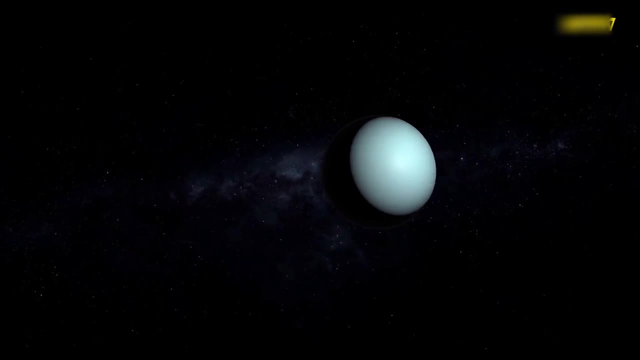 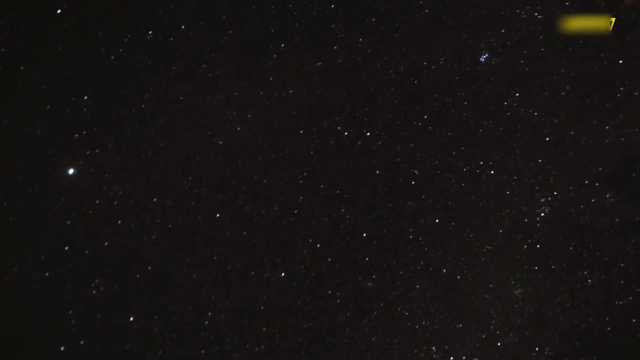 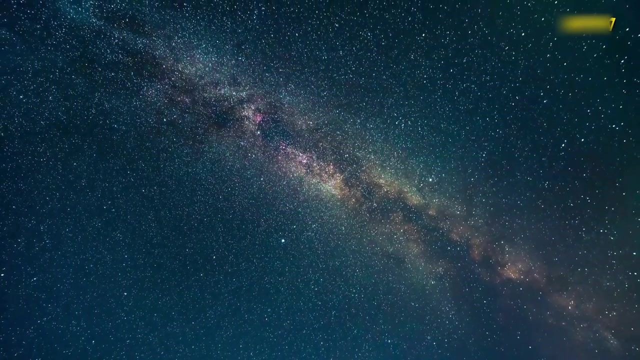 another distant world, far beyond Neptune. But hunting down such a faint object was like looking for a needle in the celestial haystack. Leading the search for Planet X over much of this time was the founder of the Flagstaff Observatory, Percival Lowell. Starting in 1906, Lowell had embarked on an obsessive pursuit of the ninth planet. 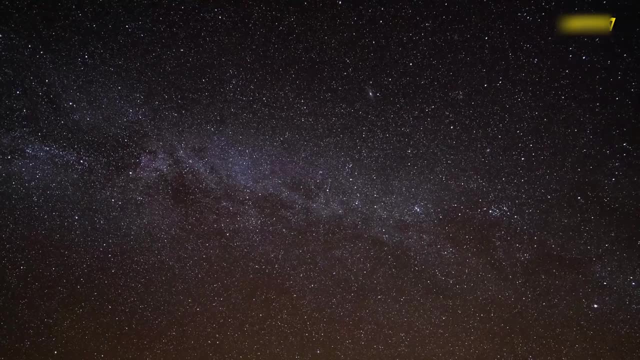 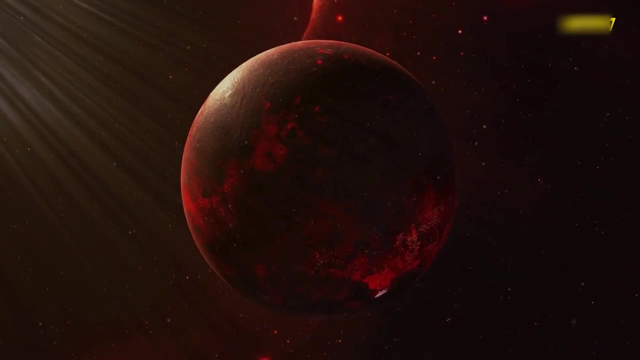 but despite years of work, he would not live long enough to see its discovery, and he would never know how close he came to finding it himself. Unknown to Lowell, an image of Planet X had been captured in two photographs he had taken just a year or so before his death in 1916. 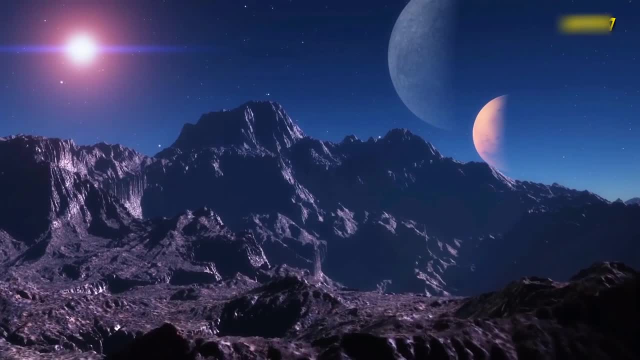 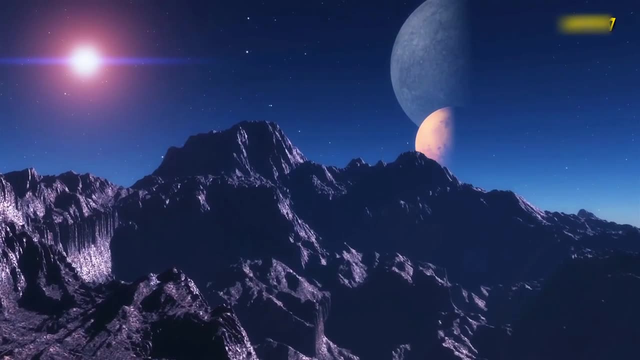 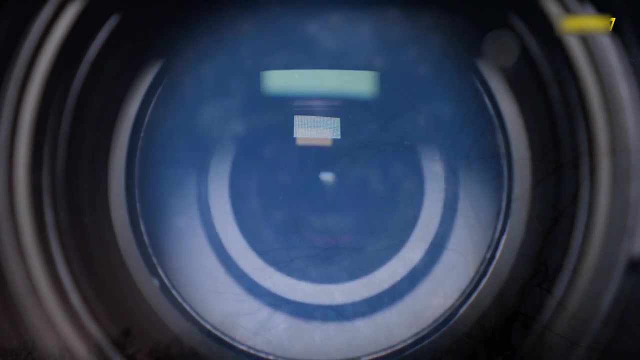 But the evidence was missed. The photographic plates were filed away and the search would go on without him for another 15 years. The logic behind using identical pairs of photographs taken a few nights apart was simple: By examining the two images for any stars that appeared to have shifted position. 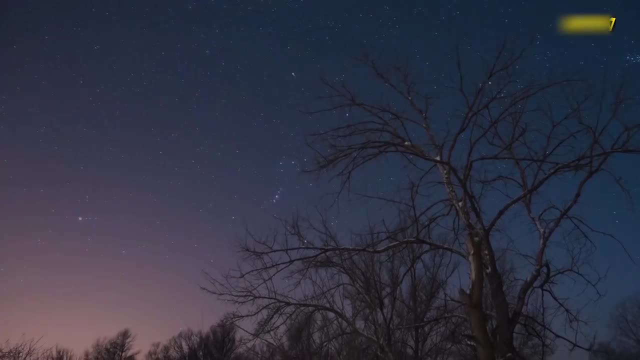 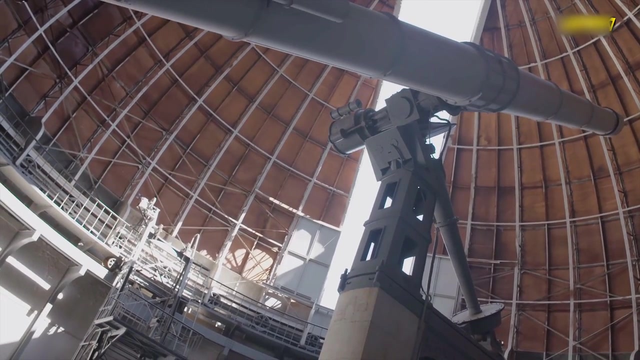 they would be able to differentiate between the distant stars in the background and anything that was orbiting closer to Earth. Hundreds of pairs of images were taken the Lowell Observatory for this purpose and analysed using a blink comparator, which helped to reveal any minute differences between the images. 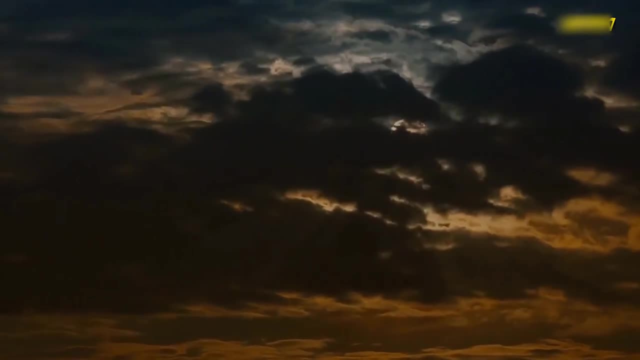 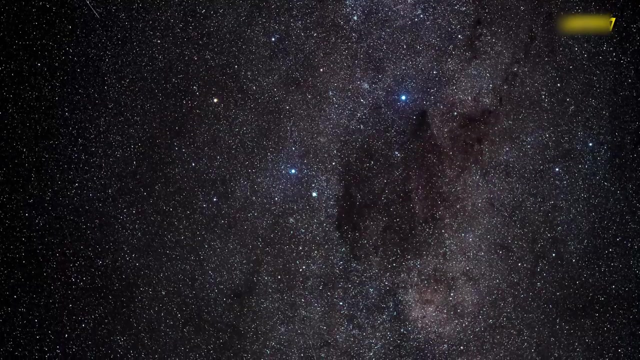 But it wasn't until the night of the 29th of January 1930 that Tombaugh would strike gold. Comparing the two images he had taken a week apart, Tombaugh discovered what appeared to be a moving object on the two plates. 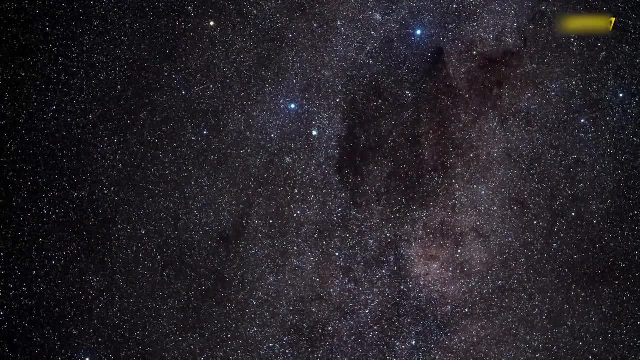 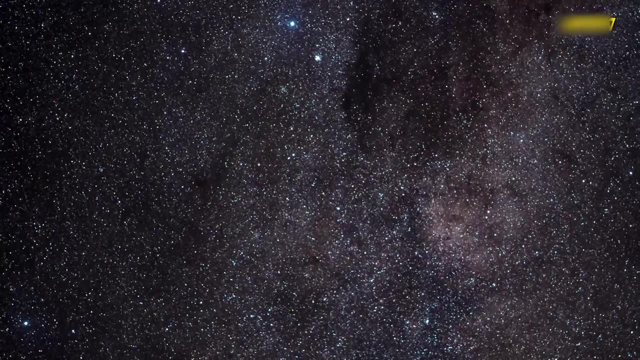 Across those few days, a dim spot had moved no more than an inch, but that movement seemed to be a moving object. This signified something profound. This was an object much closer to the Earth than the distant stars in the background, an object that had moved as our perspective had changed with the Earth's own orbit. 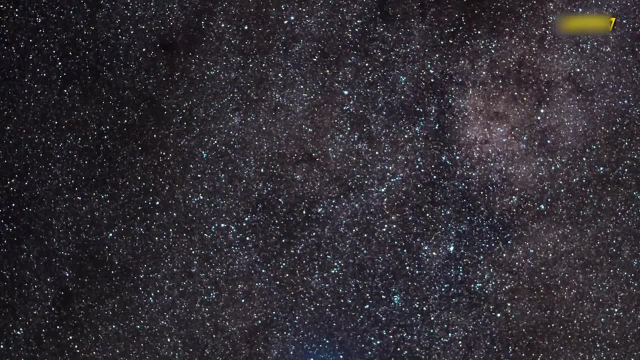 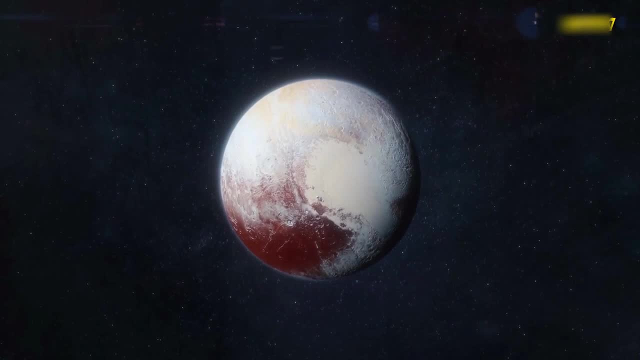 And over the course of that week this object appeared to have shifted against the distant background. Tombaugh had found Planet X, which would be named Pluto after the suggestion of Venetia Burney, an 11-year-old English schoolgirl from Oxford. 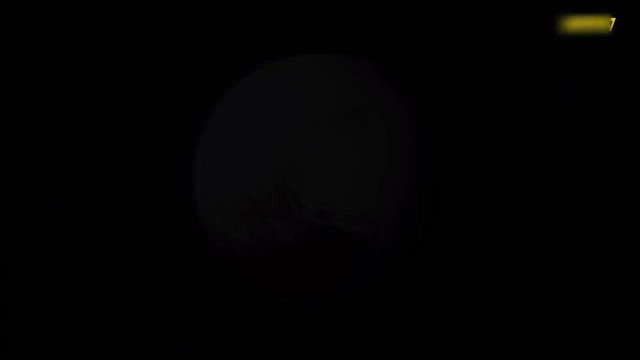 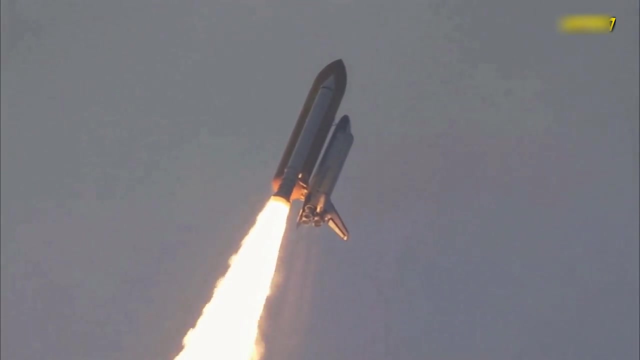 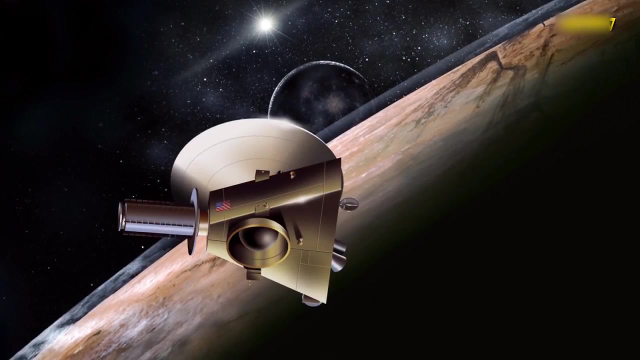 with an interest in classical mythology. Taking off from Cape Canaveral Air Force Base on the back of an Atlas V rocket, the New Horizons space probe began its epic journey across the solar system towards Pluto in January 2006.. Just nine years after the death of Clyde Tombaugh, 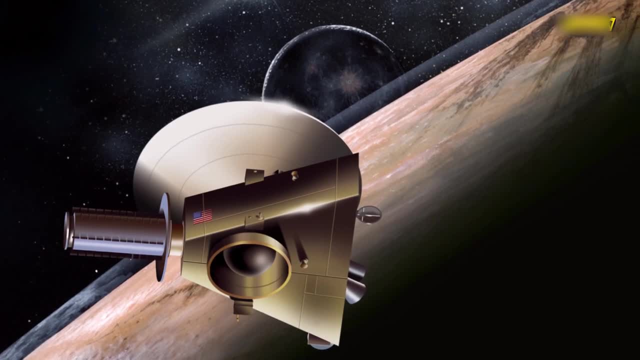 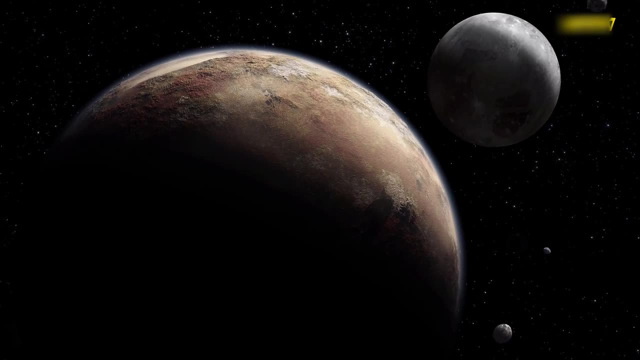 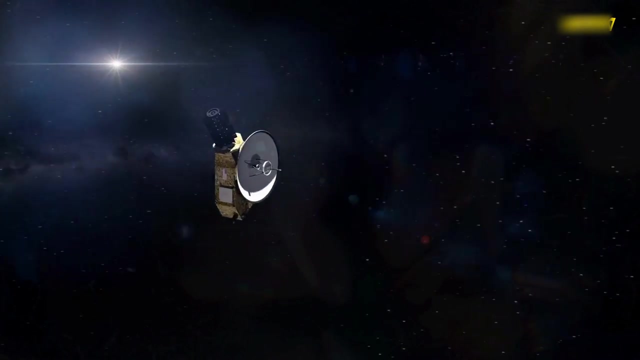 this tiny interplanetary probe, no bigger than a grand piano, made room in its payload for 30 grams of his ashes, a tribute to the man who had begun our journey to Pluto 76 years before. For Alan Stern, principal investigator of the New Horizons mission. 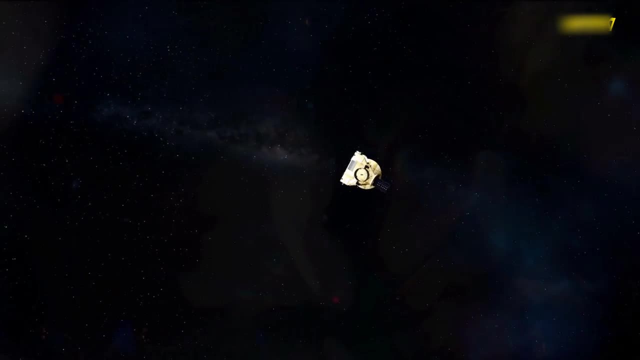 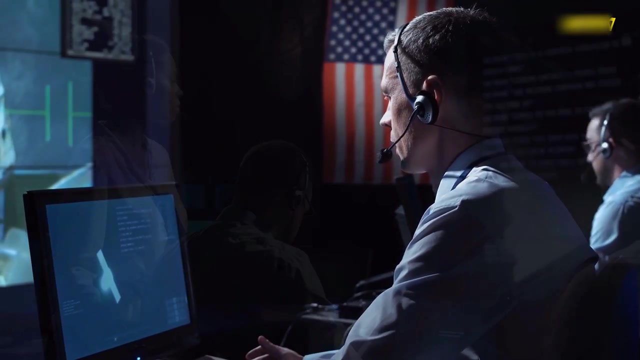 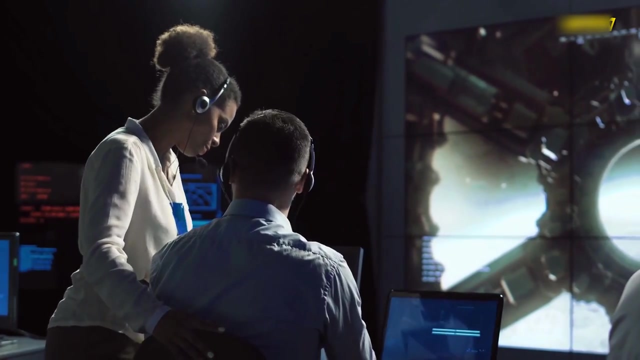 this move fulfilled a promise made to Tombaugh Shortly before New Horizons became a project. while we were still trying to get funding to fly a spacecraft to explore Pluto, Clyde died in January of 1997.. And prior to that he had asked if a mission ever did get launched. 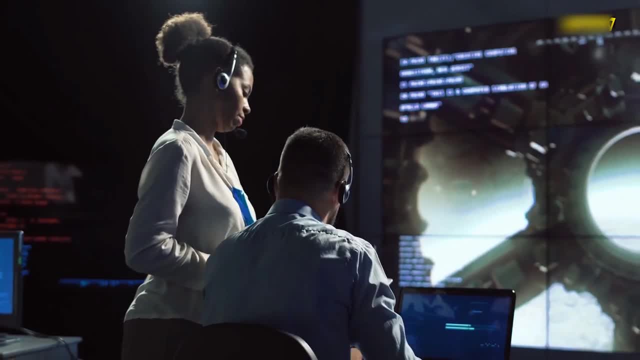 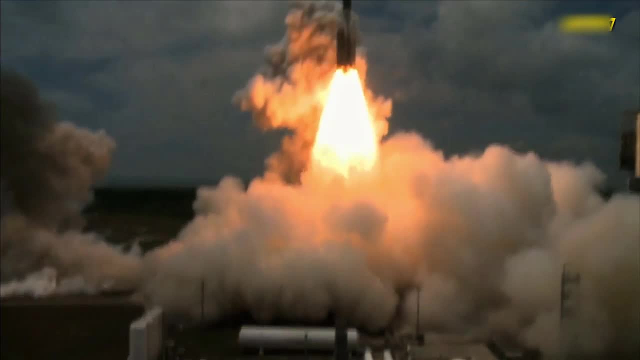 if there was a way it could be considered, if some of his ashes could be sent on the journey, And I had heard about that back in the 90s and when it came close to launching New Horizons in the summer of 2005,. 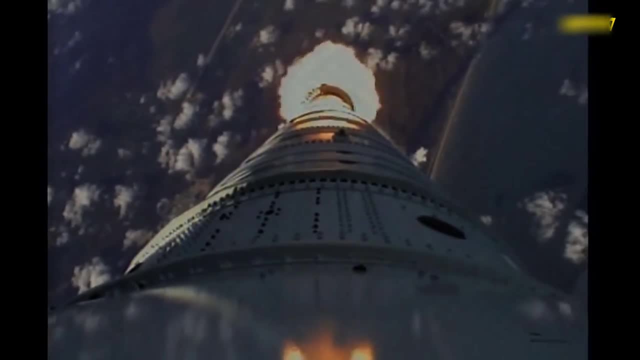 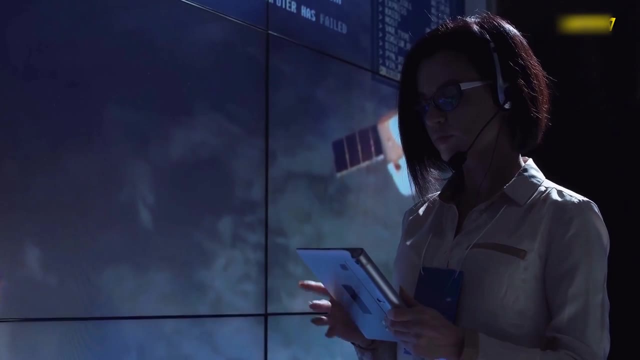 I reached out to his family to see if that's something they wanted. and it was still possible And it was, and we found a way to do it and we were very proud to be able to make it happen, Not just for Clyde Tombaugh and his family. 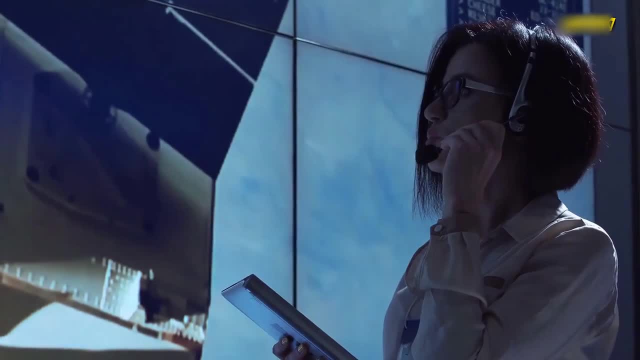 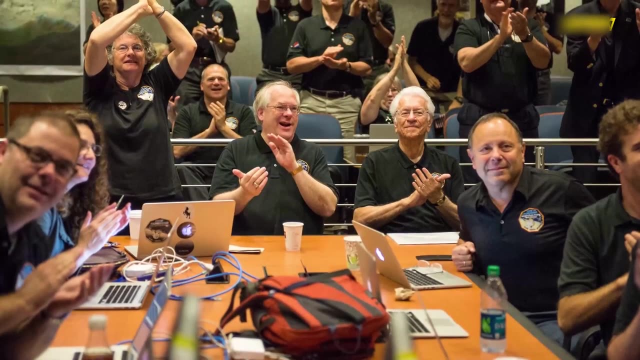 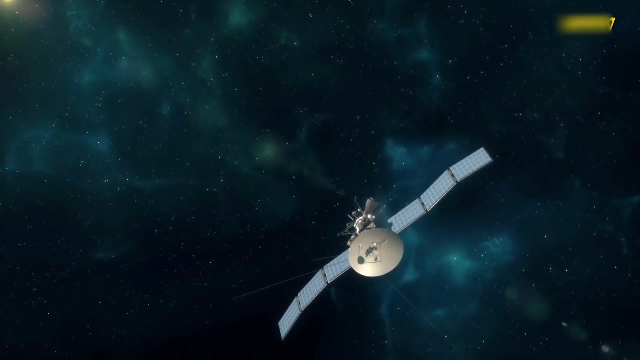 but even more so for the people of Earth, because it makes a very human connection between the discoverer of this world and those who were the explorers of it on the New Horizons team, Leaving the Earth with an escape velocity of 16.26 kilometers per second. 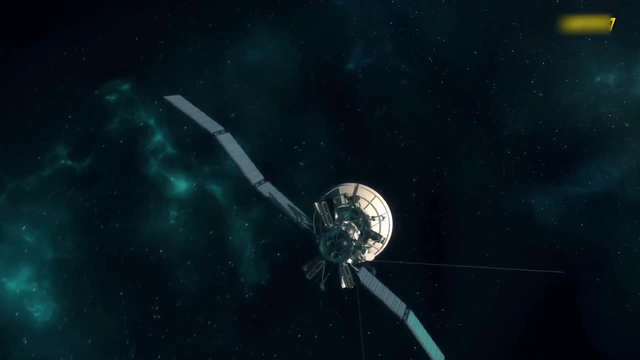 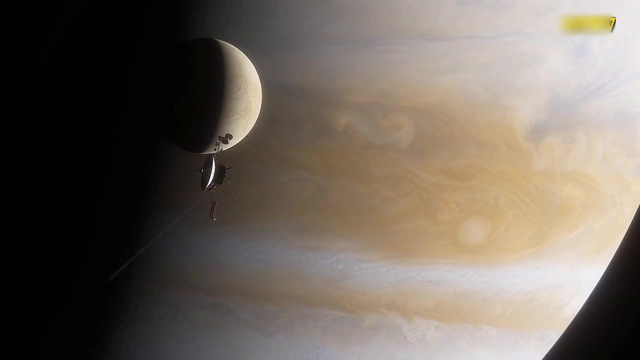 New Horizons was the fastest probe ever launched from our planet, Reaching Jupiter in just over a year. it progressed on its way with a gravity-assisted kick from the gas giant, sending it hurtling across space, With all non-essential systems shut down to conserve energy. 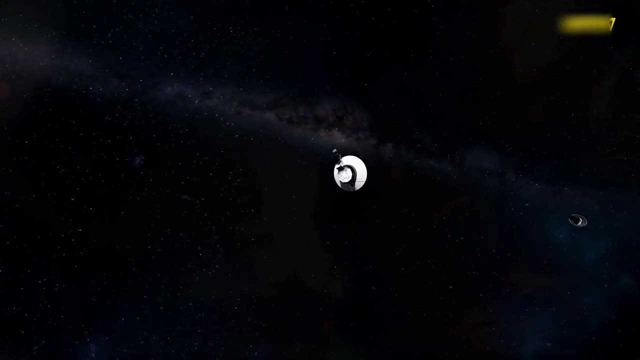 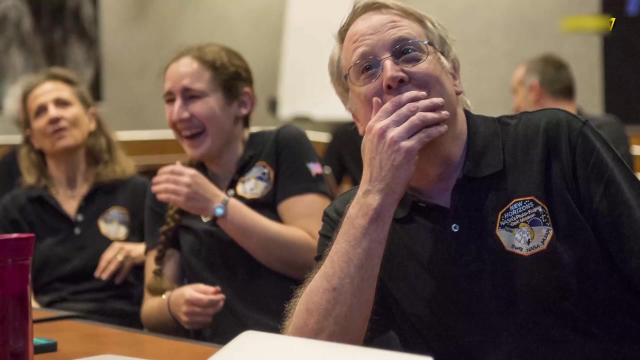 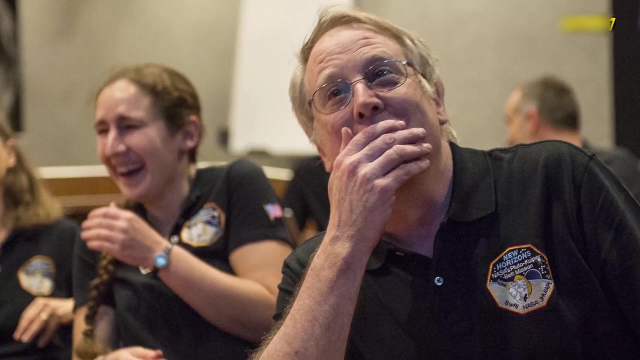 this little probe would sleep through most of its epic eight-year voyage in the dark. After 20 years of planning, building and dreaming, the New Horizons team could only wait and hope for its safe passage as it made its way towards the last unexplored world in our solar system. 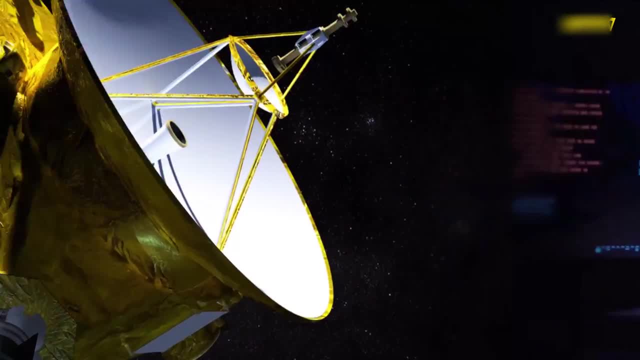 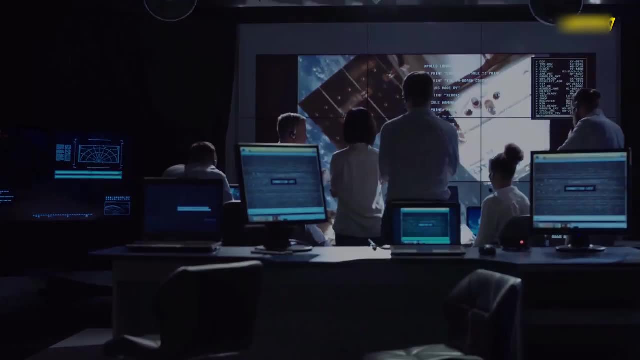 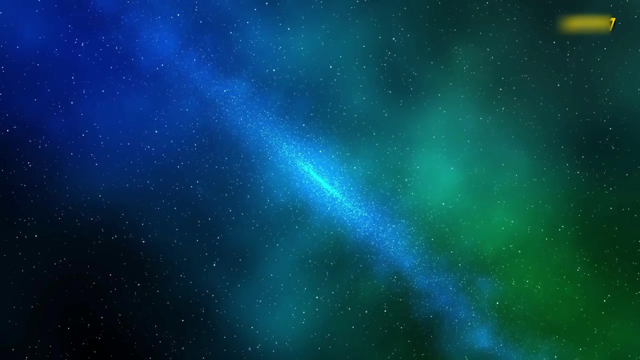 But while the voyage itself proceeded without a glitch, back on Earth, the status of the mission was about to take the most unexpected of turns, Starting with the discovery of the rocky object 15760 Albion back in 1992, the description of Pluto as a planet. 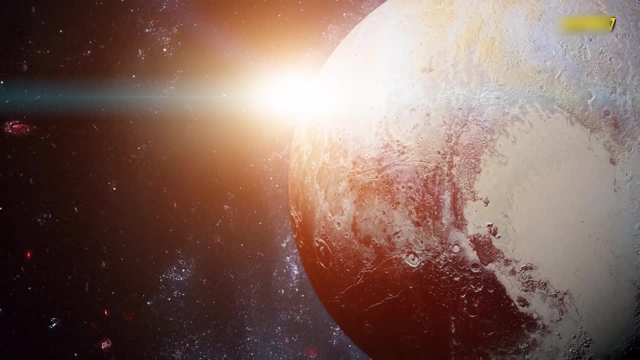 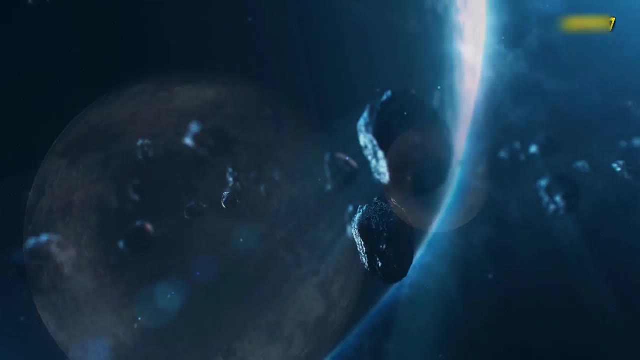 orbiting alone in the farthest reaches of the solar system would come under increasing scrutiny. Pluto, it seemed, was not so lonely. after all, This was a region of space filled with an array of orbiting objects, and, as we began to peer into the Kuiper Belt, 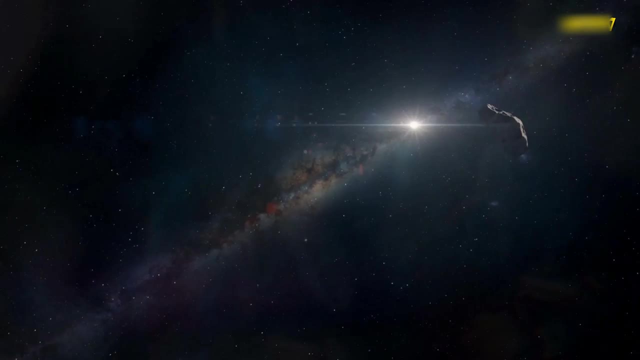 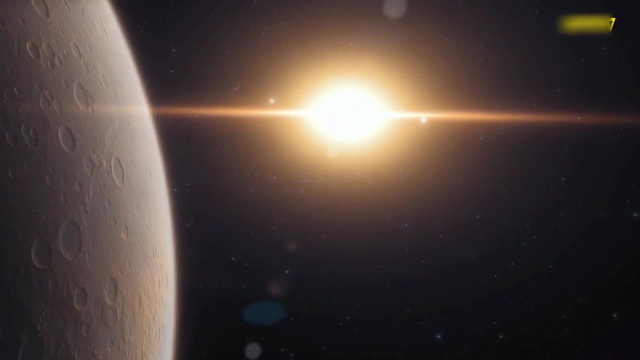 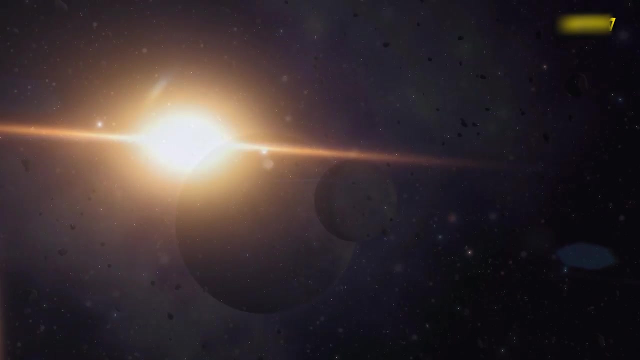 we discovered, they were far from just fragments. This was a region of space filled with Pluto-like worlds. 50000 Quawar, an object half the size of Pluto, discovered at the Palomar Observatory in June 2002.. 90377 Sedna. 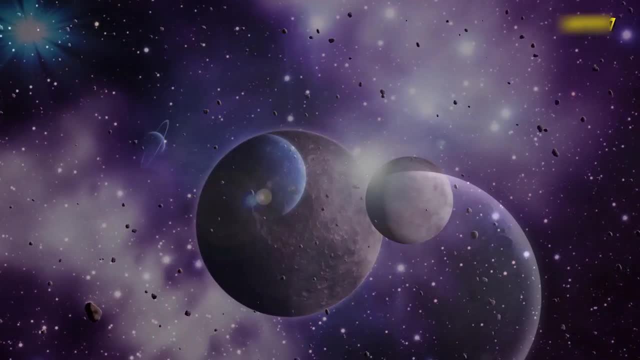 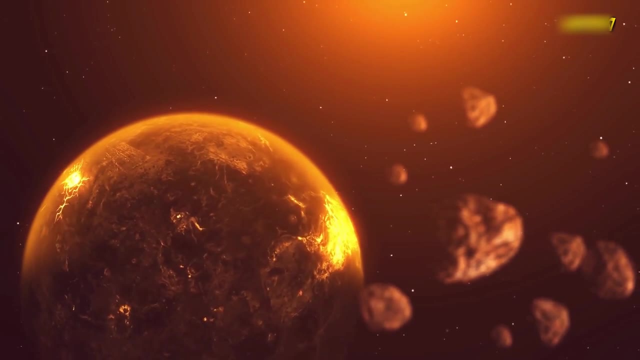 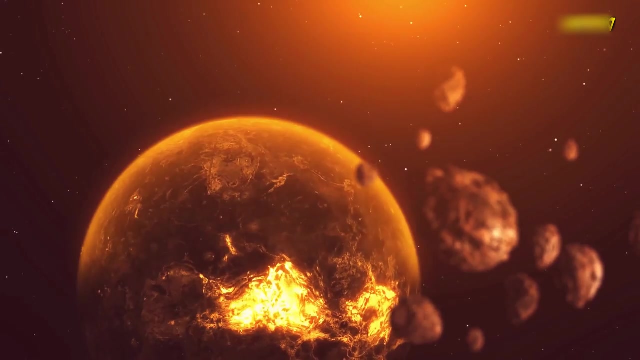 a large minor planet discovered in November 2003, on an 11,400-year orbit around the Sun. 136198 Haumea, a huge pebble-shaped world with two tiny moons in orbit, discovered in December 2004.. 136472 Makemake. 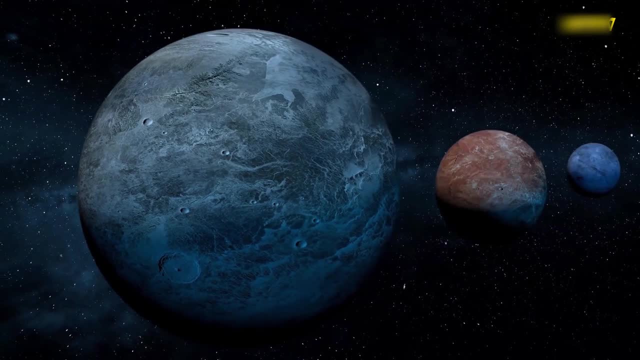 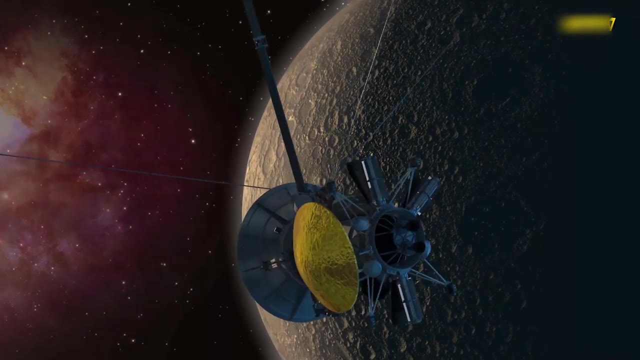 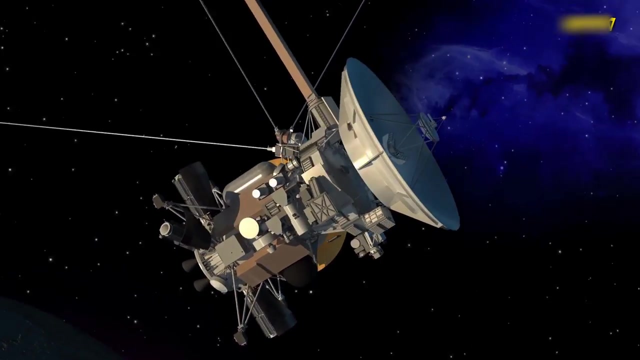 a dwarf planet, perhaps two-thirds as big as Pluto discovered in 2005.. Then, in January 2005,, we spotted 136199 Eris, a world almost the same size as Pluto itself, if not bigger. These discoveries, and the hundreds we've made since 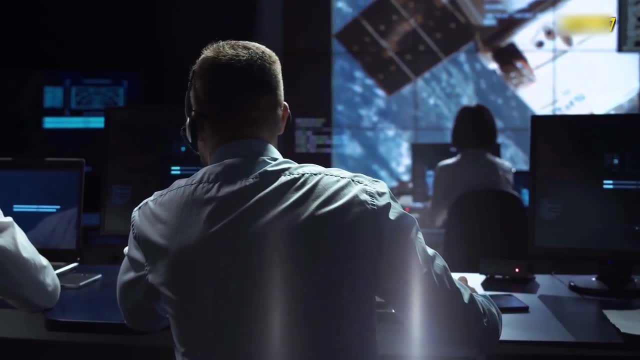 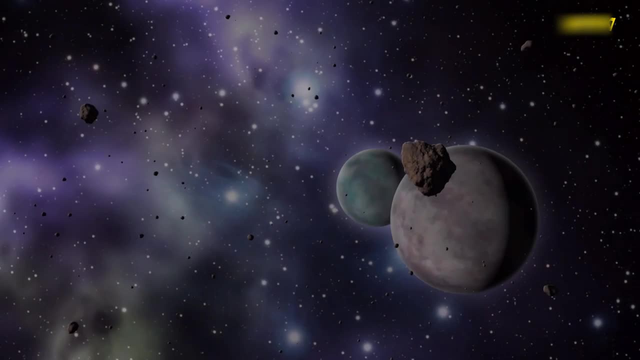 forced the International Astronomical Union, the ruling body on Earth for all things astronomical, to formally reconsider the definition of a planet. In October 2006,, they published a set of three criteria that any object in our solar system would have to fulfill. 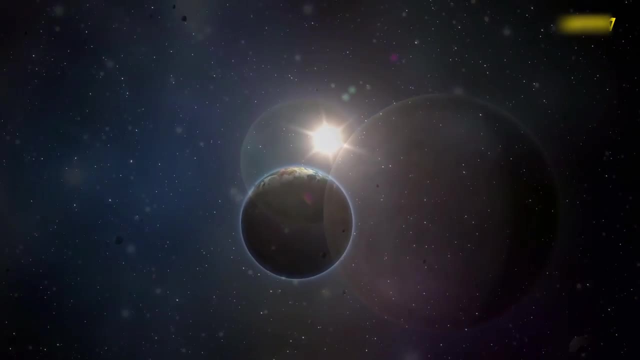 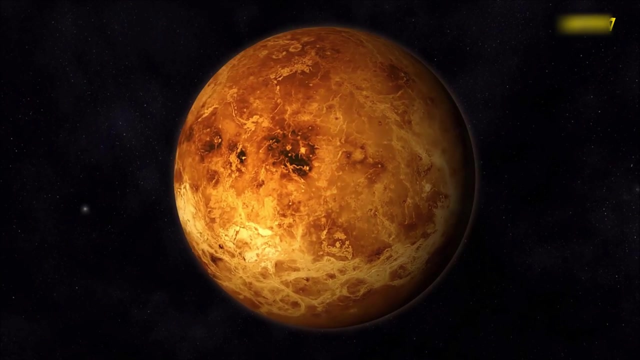 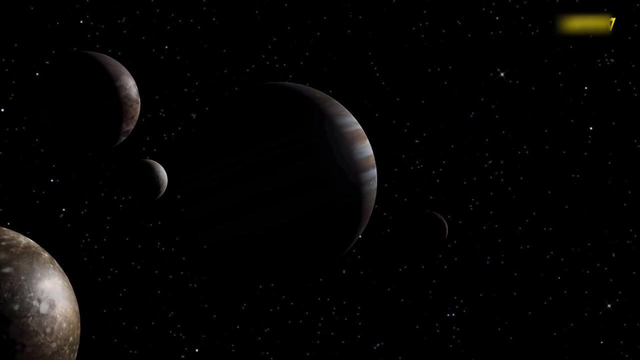 if it wanted to stake a claim of planethood, it has to orbit the Sun. it has to be massive enough for it to form a sphere under its own gravity. it has to be massive enough to clear its own orbit of any other objects, dust or debris. 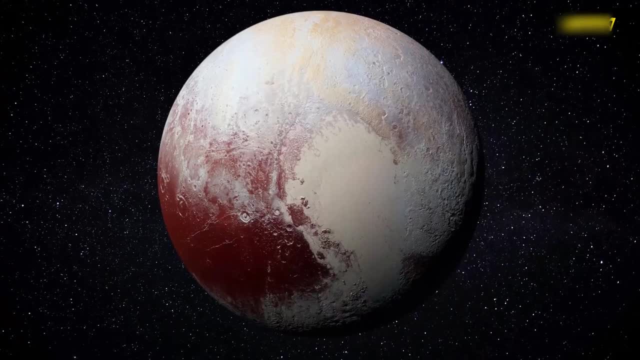 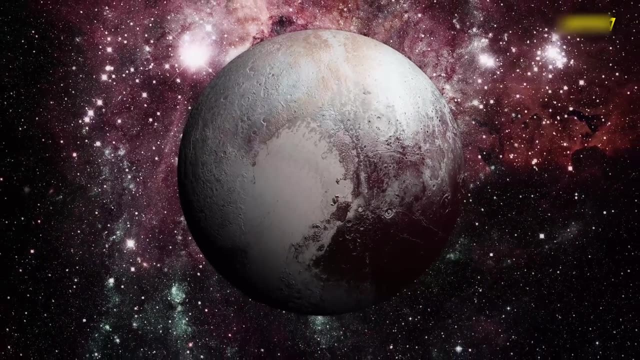 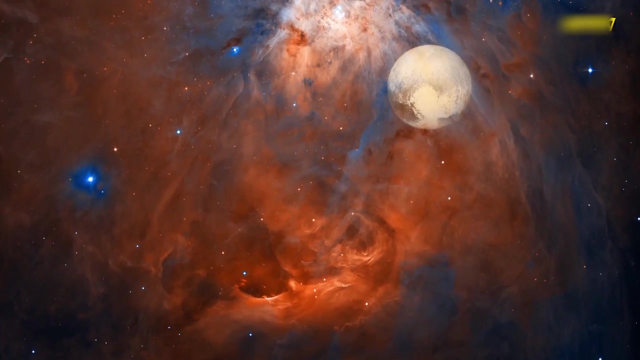 Pluto certainly ticks the first box, completing an orbit of the Sun every 248 years. We also know, even from our most distant observations, that Pluto is nearly perfectly spherical, and so the second criterion is also a clear tick for Pluto. But when it comes to the third requirement, 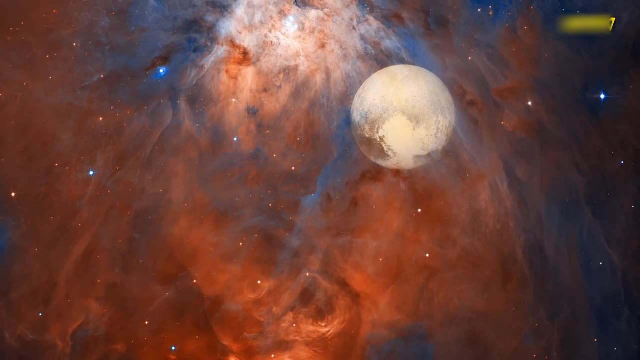 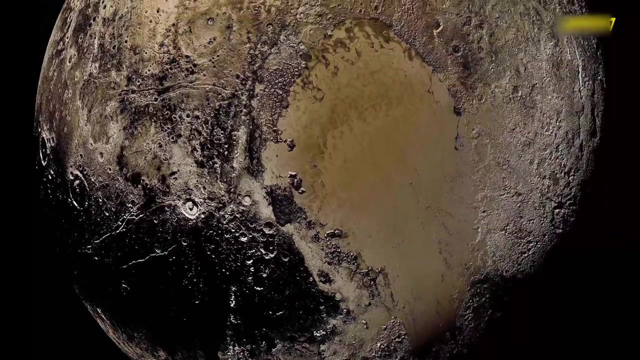 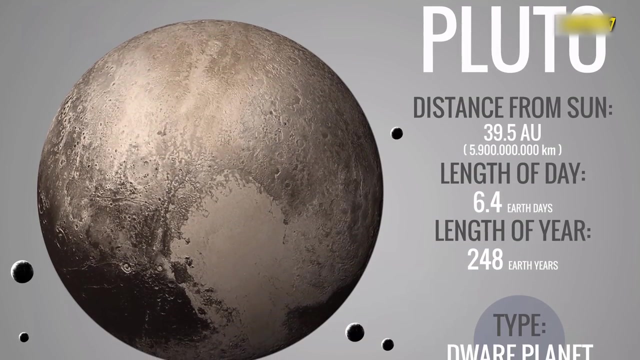 Pluto is not quite as big as Pluto. It is simply not massive enough to blow away all the bits of dust and debris in its orbit, And for that reason it fails to make the cut as a planet. Since September 2006,, Pluto has been officially designated a dwarf or minor planet. 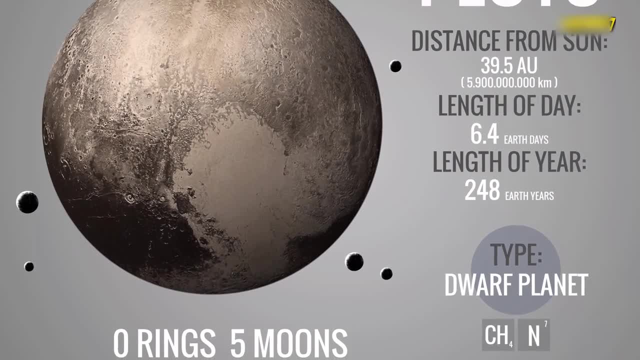 A sphere orbiting the Sun, yes, but a planet, no. The third criterion is ultimately the one that necessarily separates the chosen eight, and that is Pluto. The third criterion is ultimately the one that necessarily separates the chosen eight, and that is Pluto. 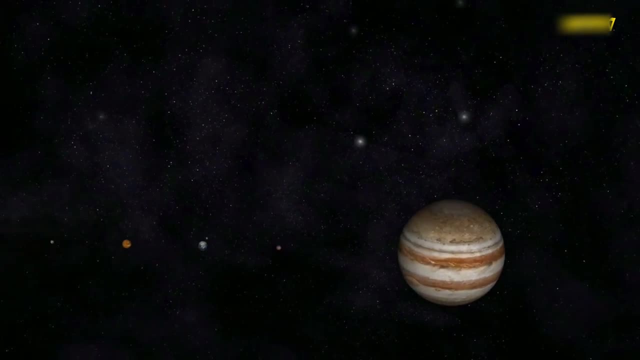 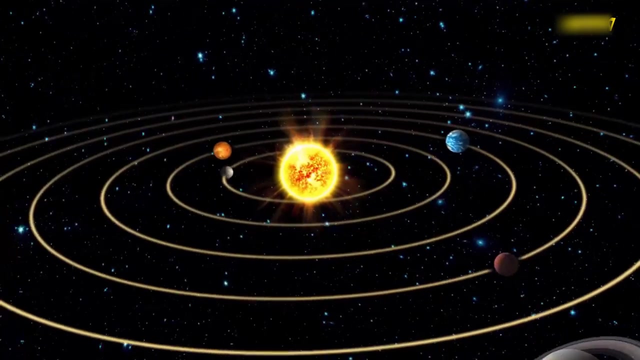 Mercury, Venus, Earth, Mars, Jupiter, Saturn, Uranus and Neptune from the rest of the globes that orbit the Sun, Because if Pluto was a planet, so too would be Sedna Eris Makemake. 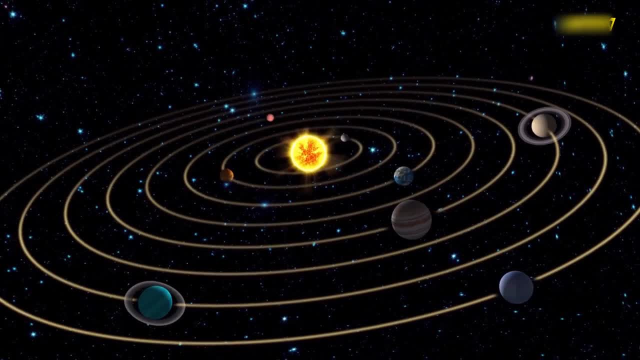 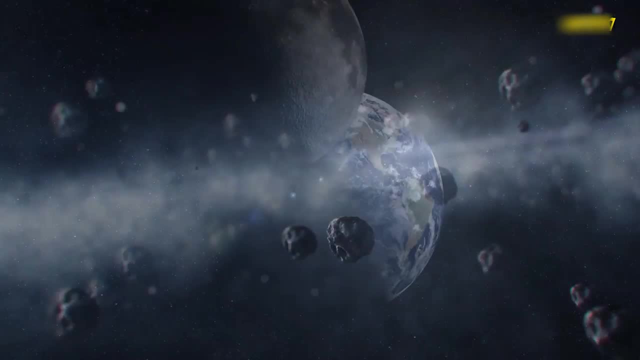 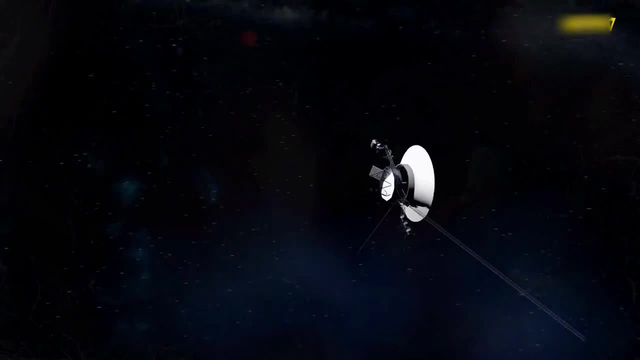 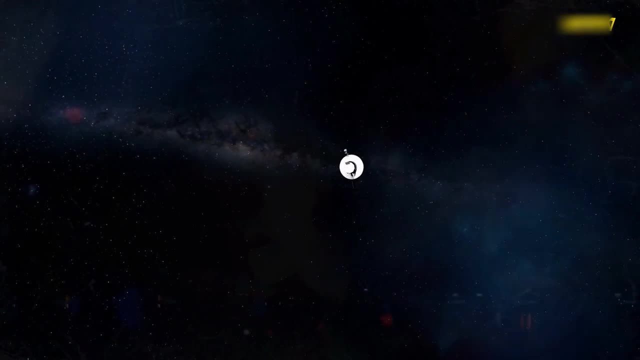 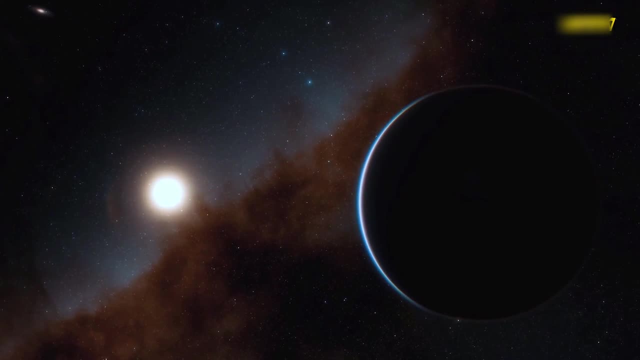 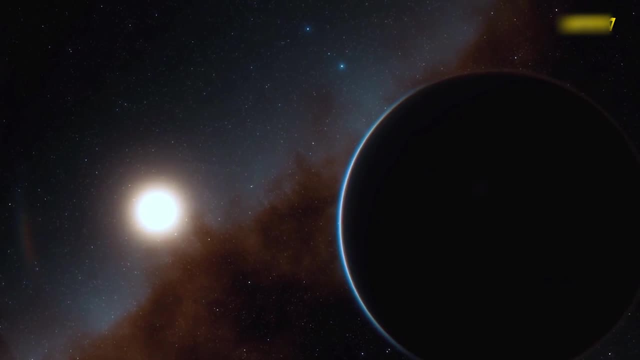 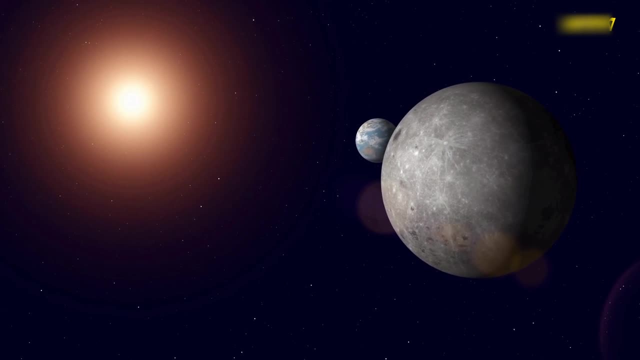 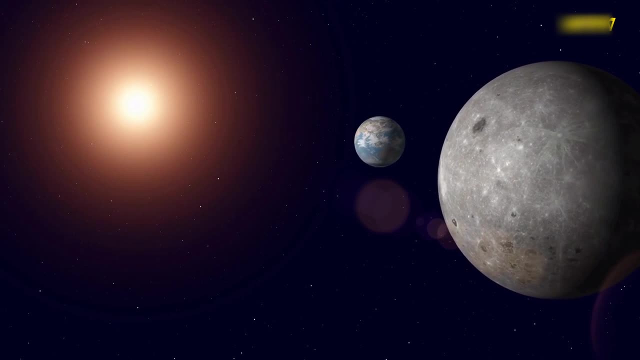 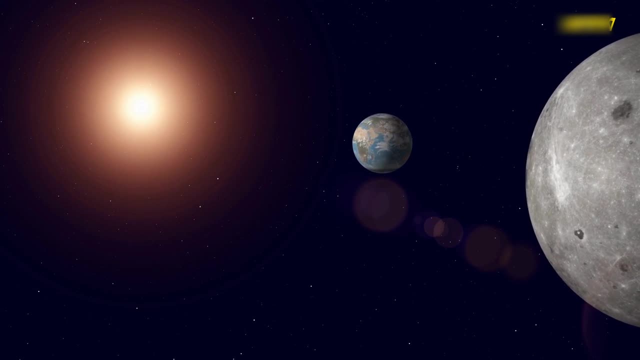 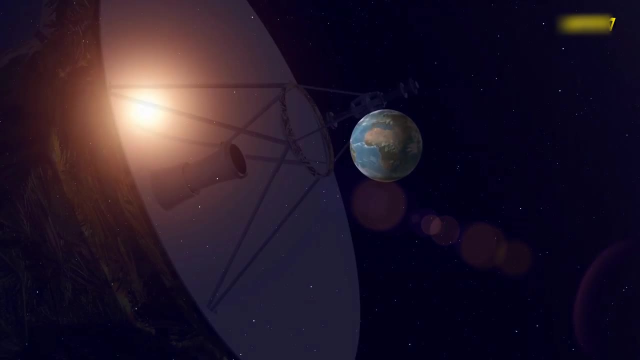 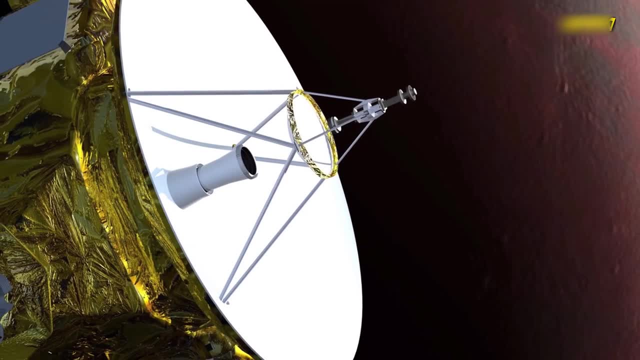 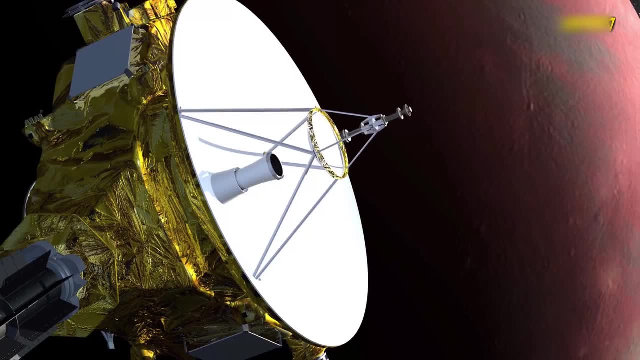 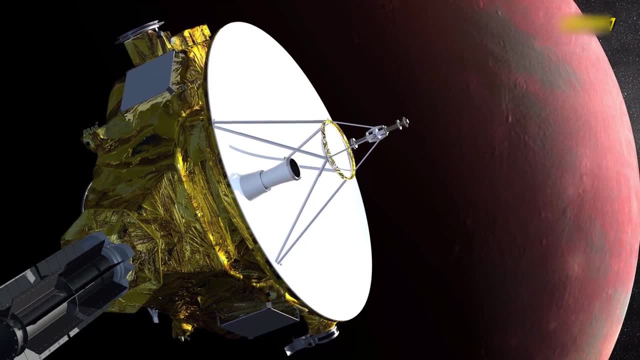 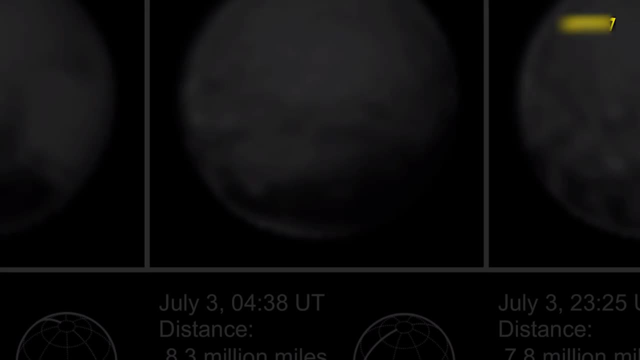 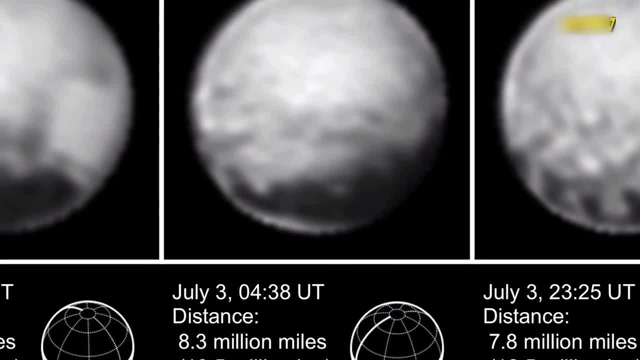 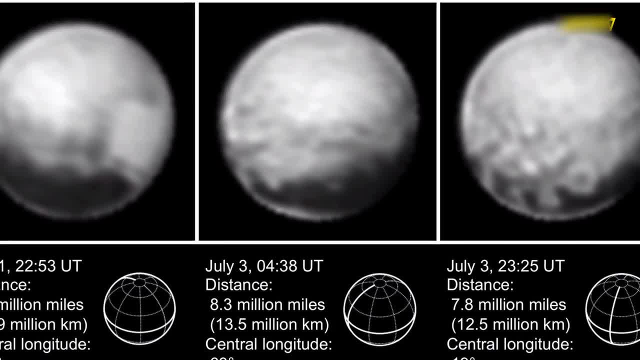 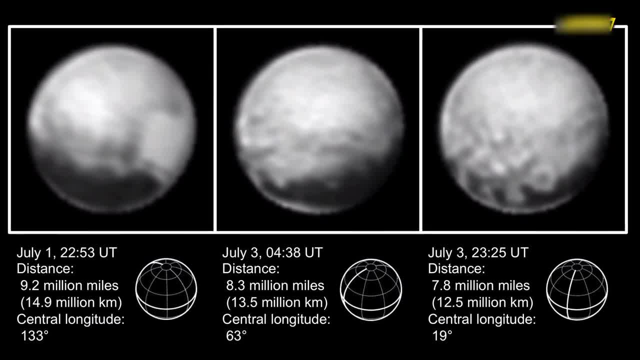 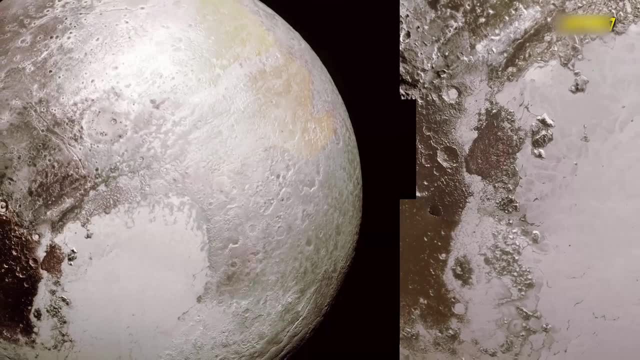 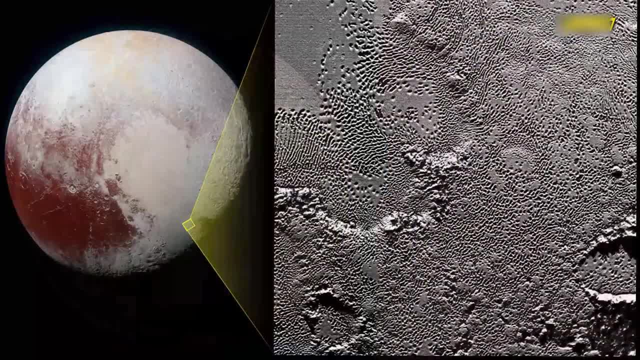 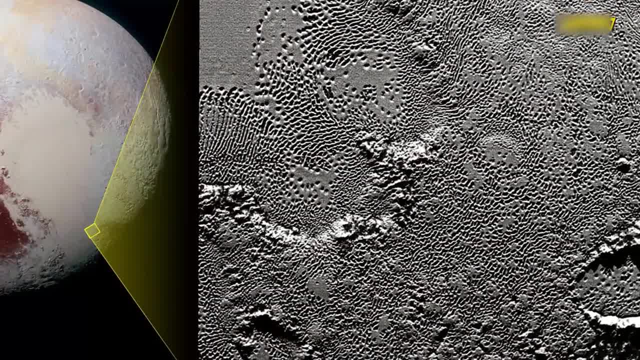 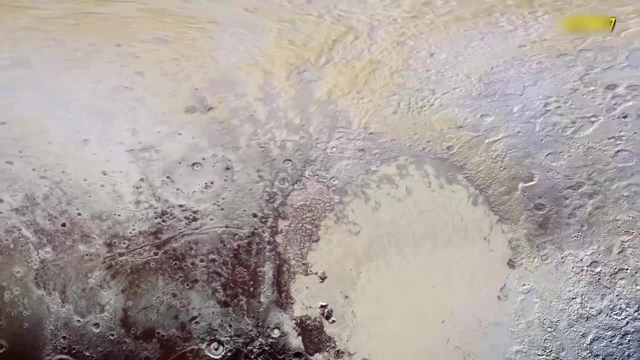 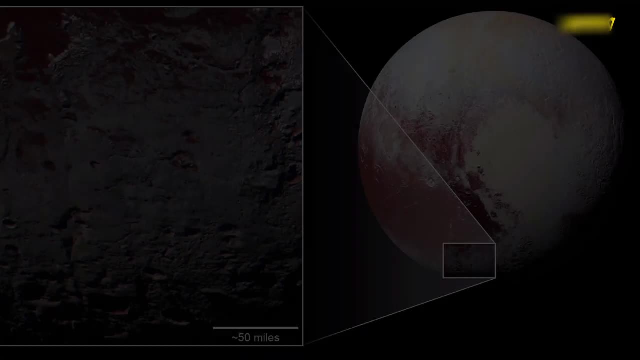 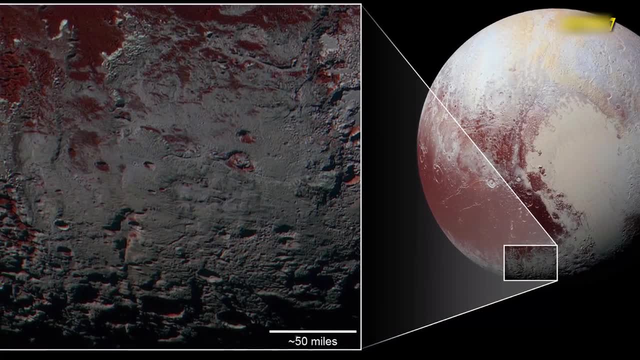 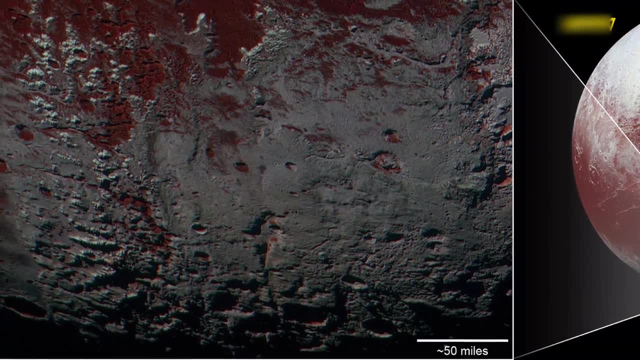 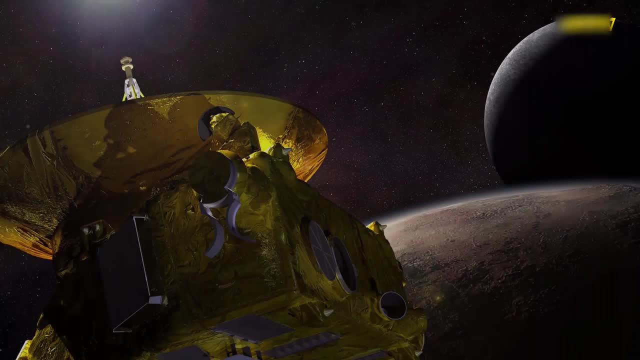 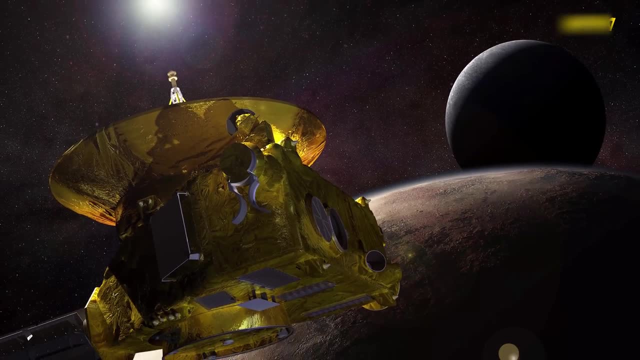 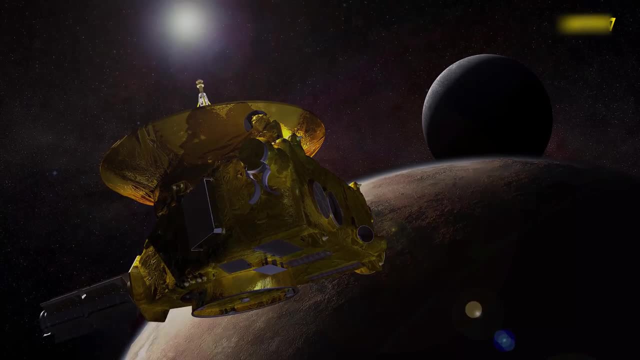 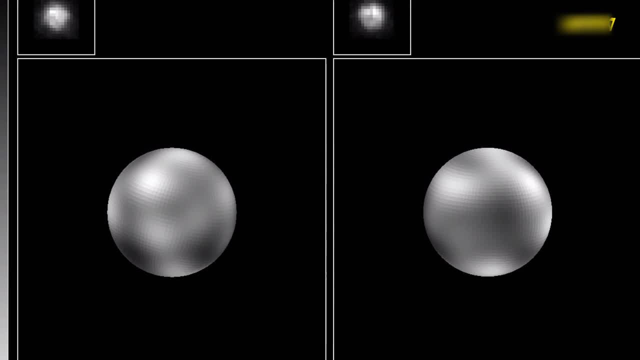 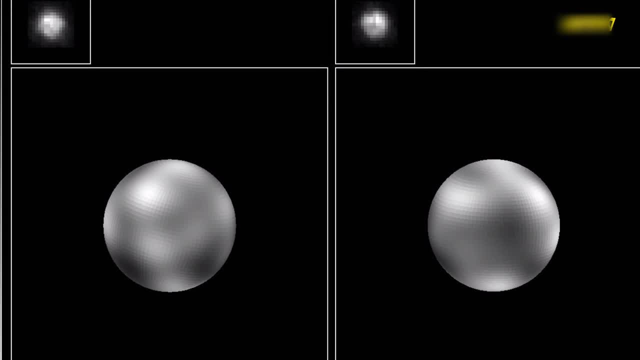 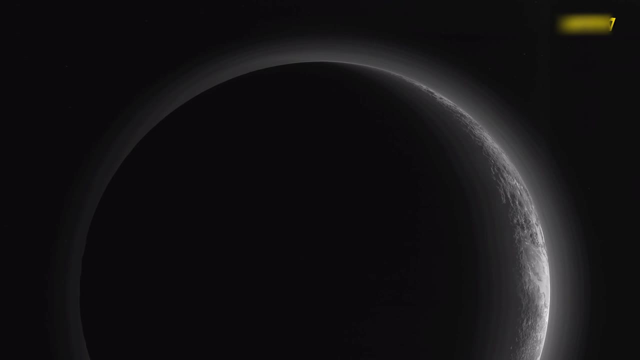 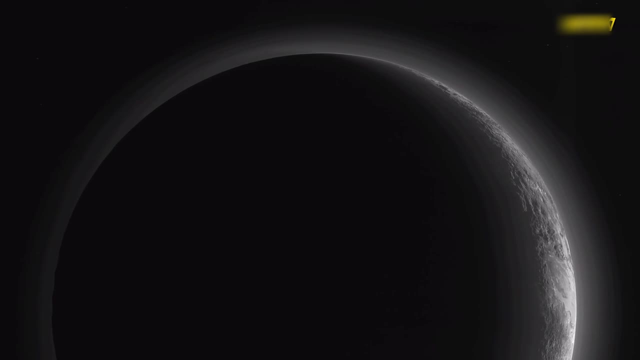 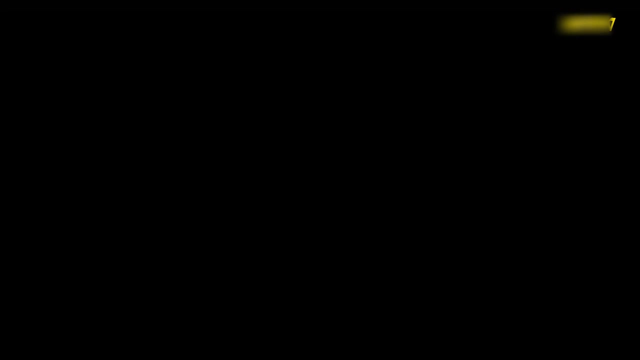 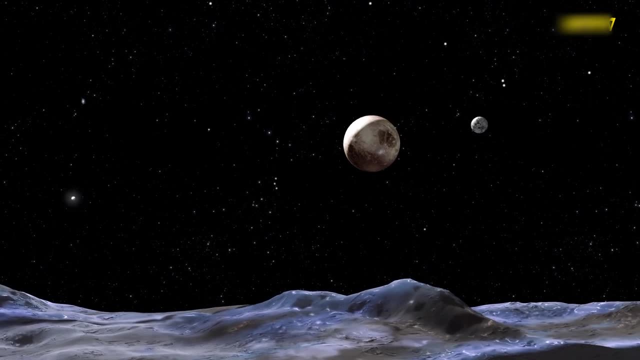 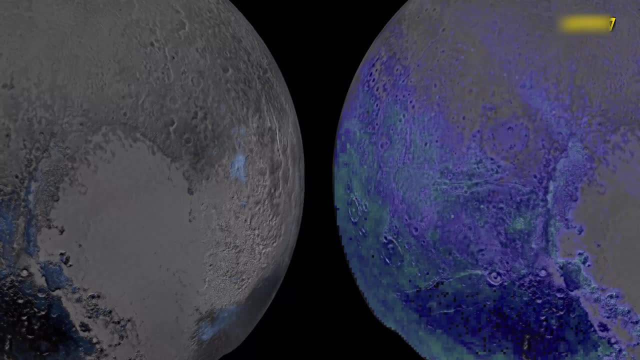 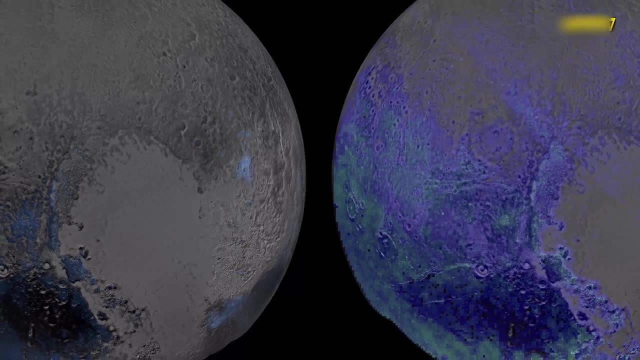 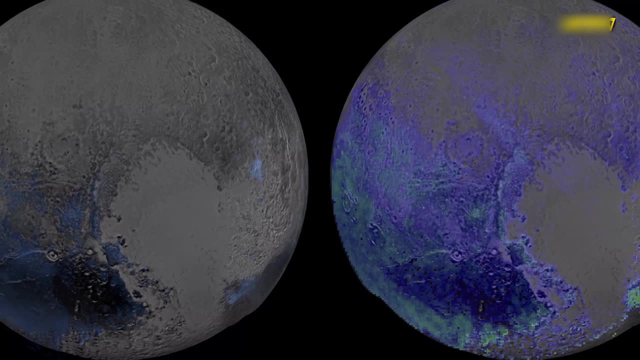 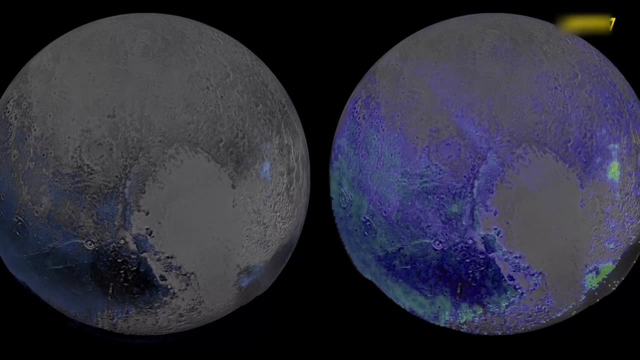 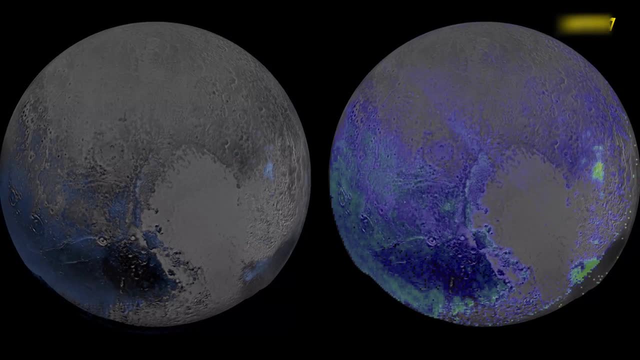 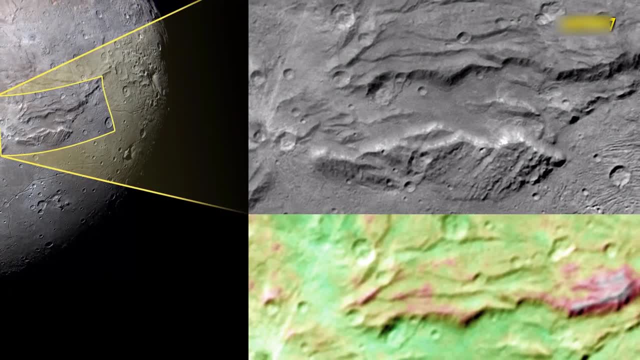 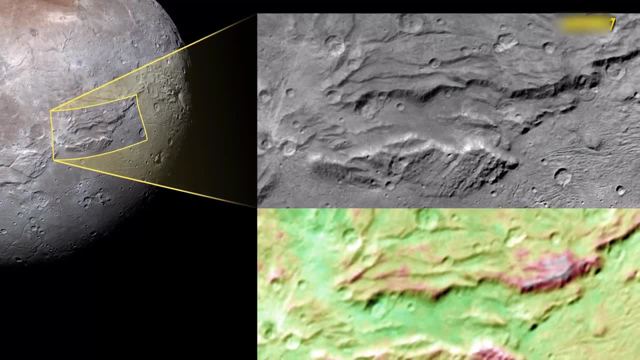 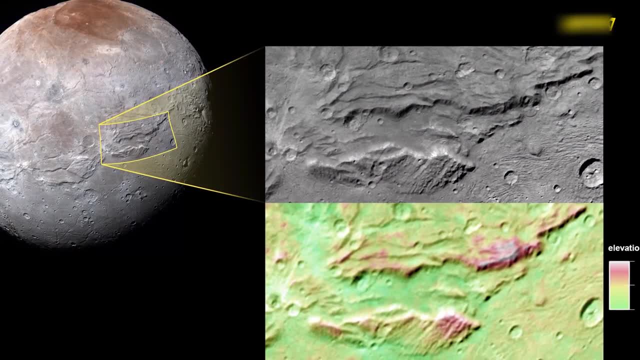 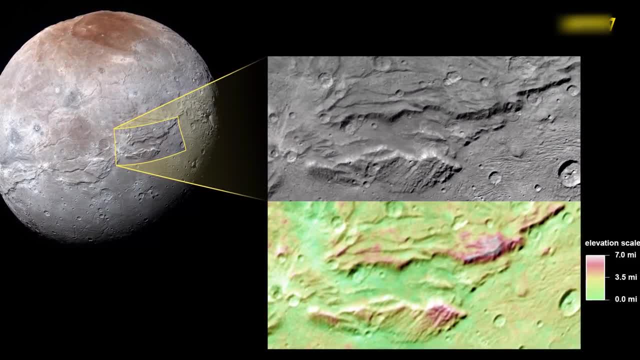 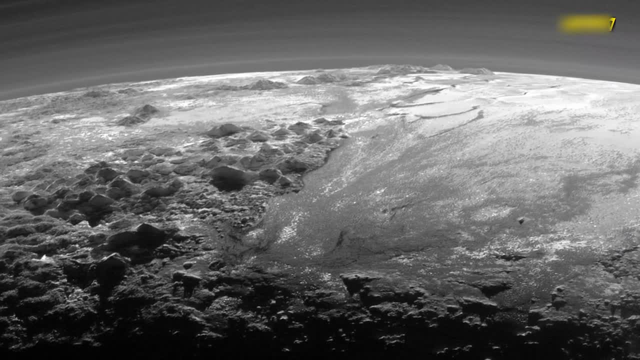 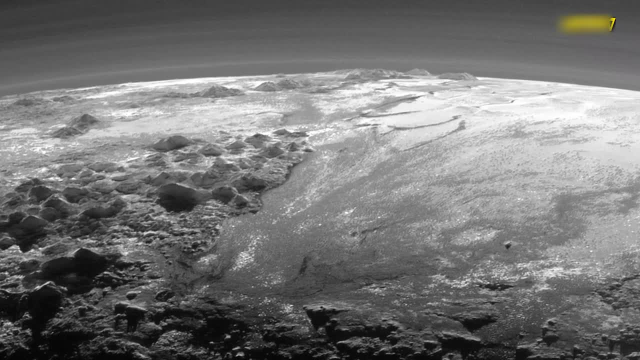 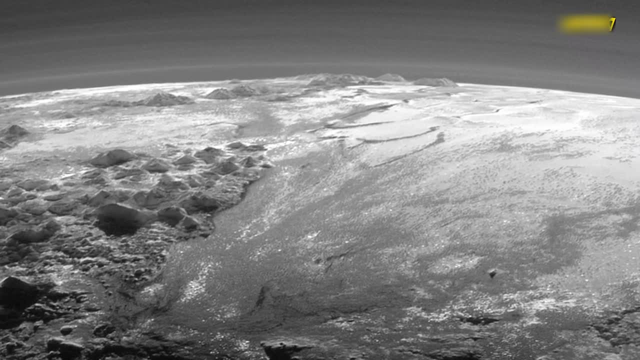 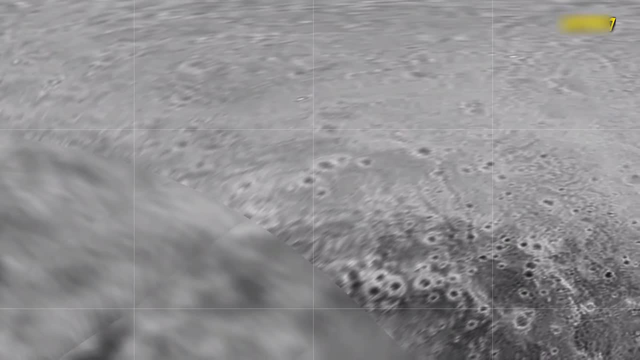 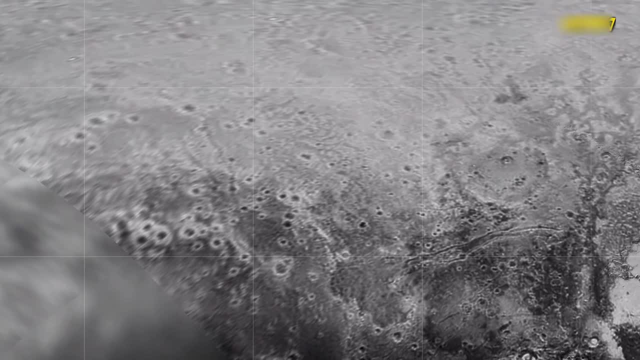 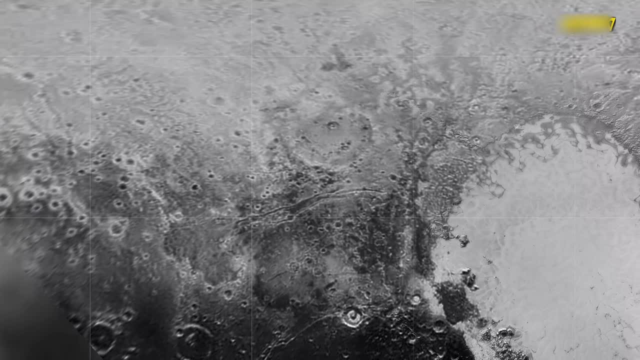 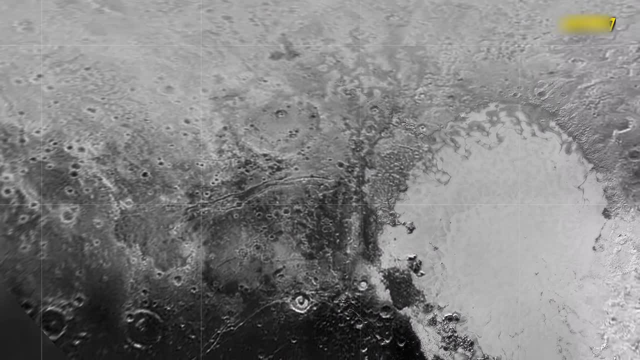 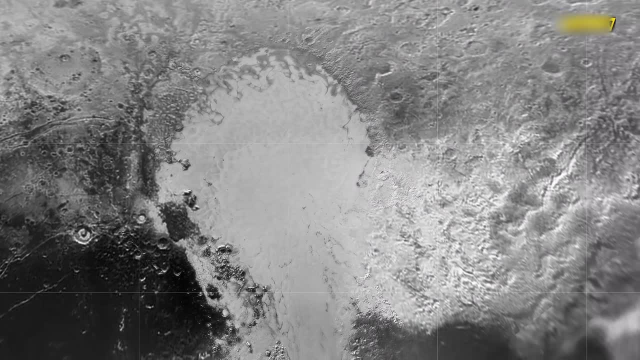 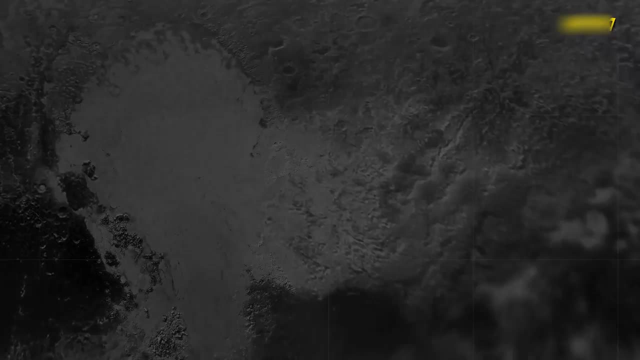 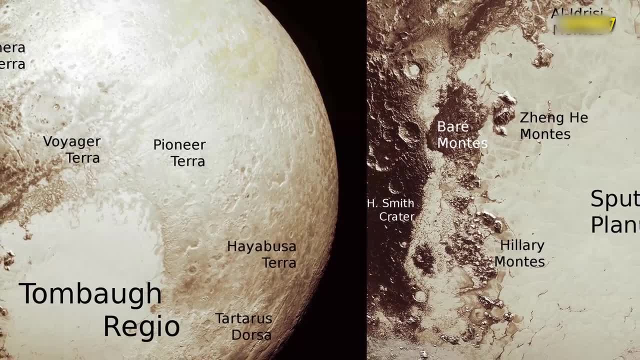 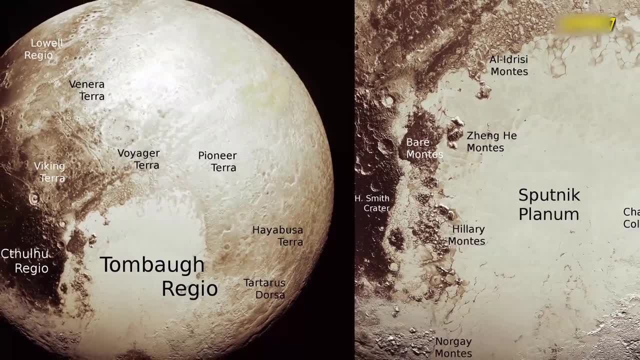 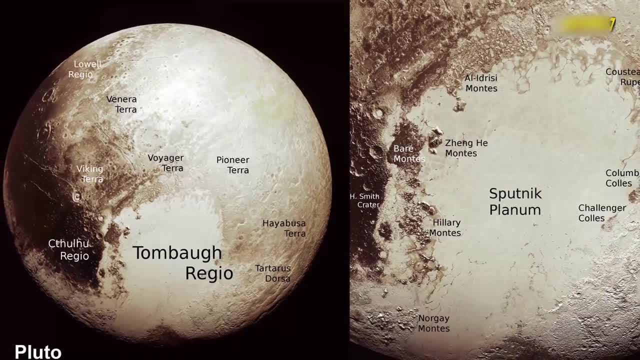 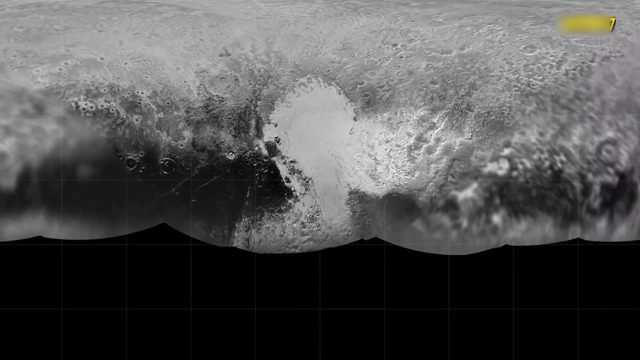 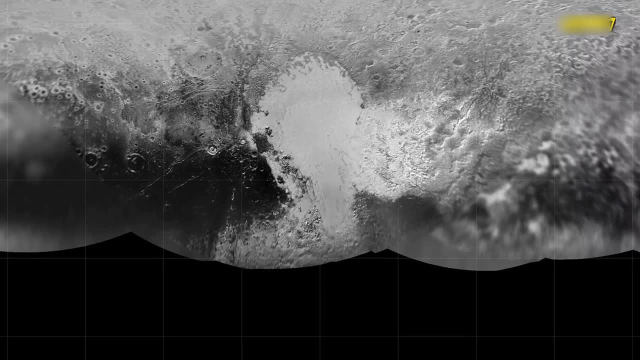 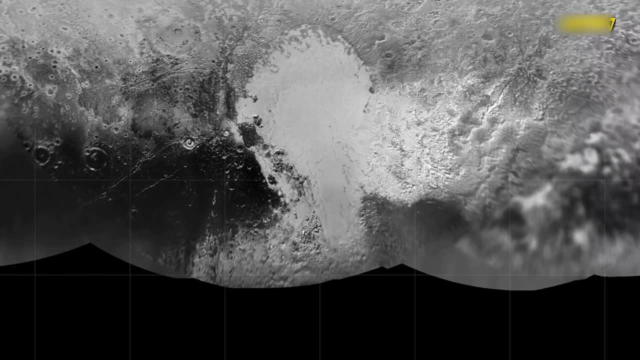 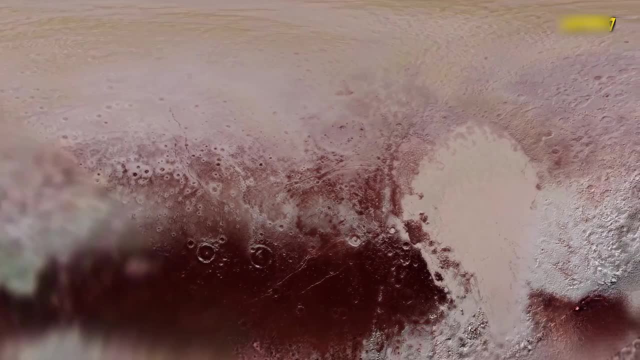 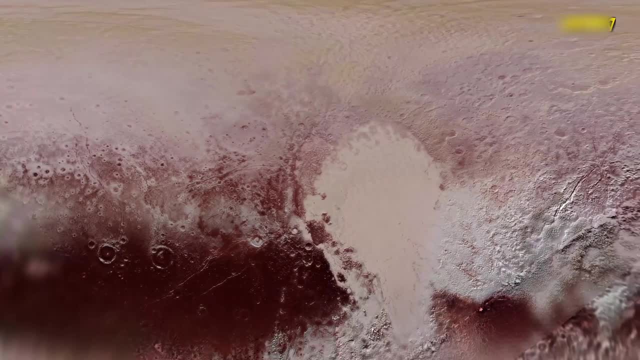 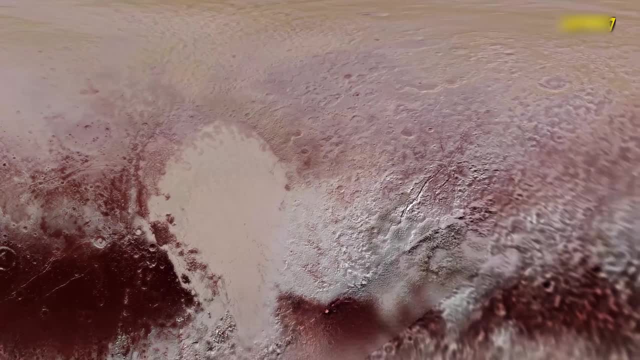 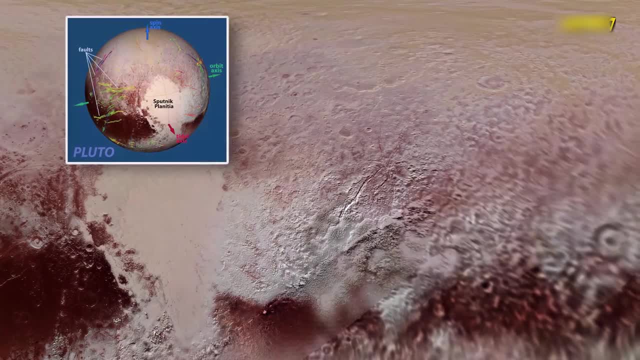 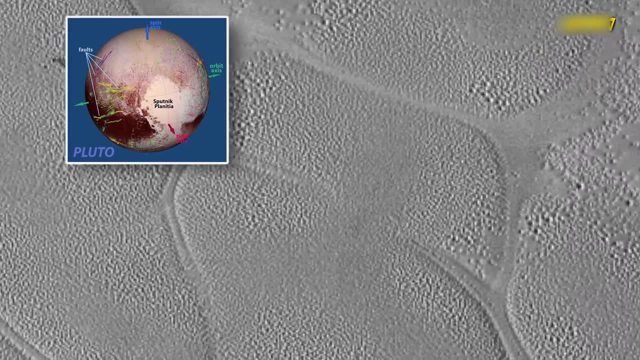 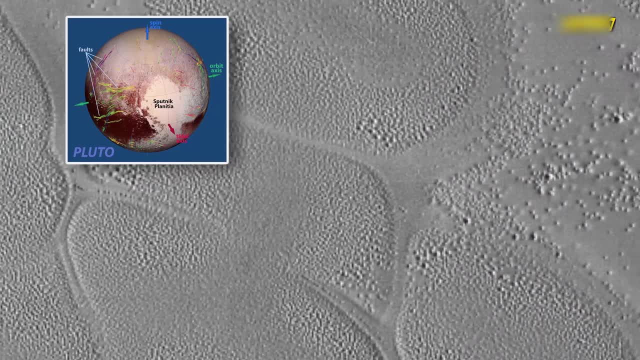 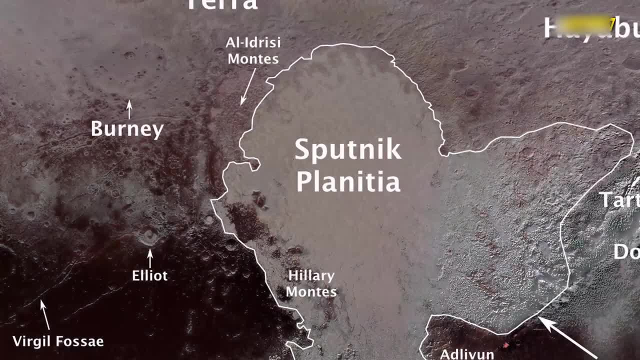 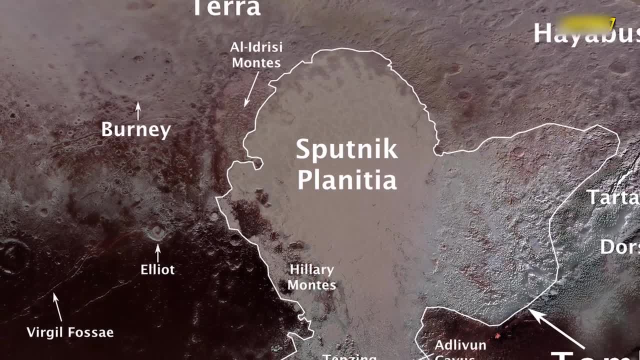 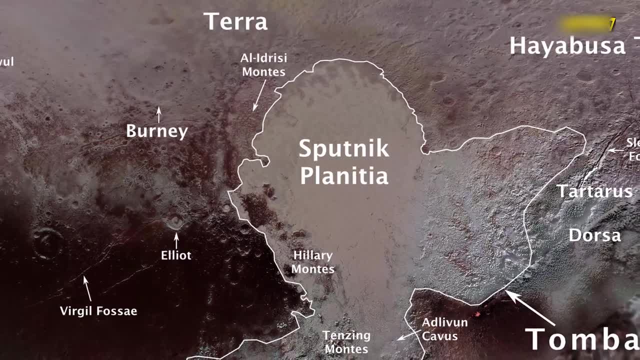 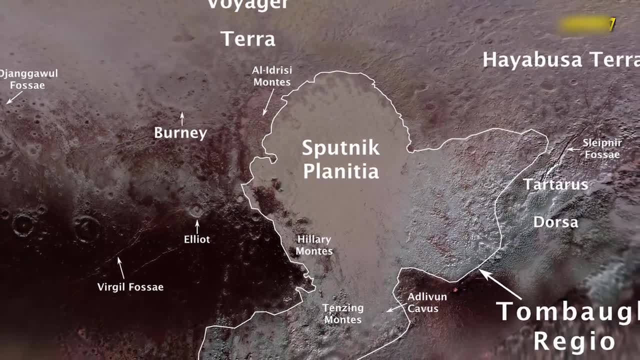 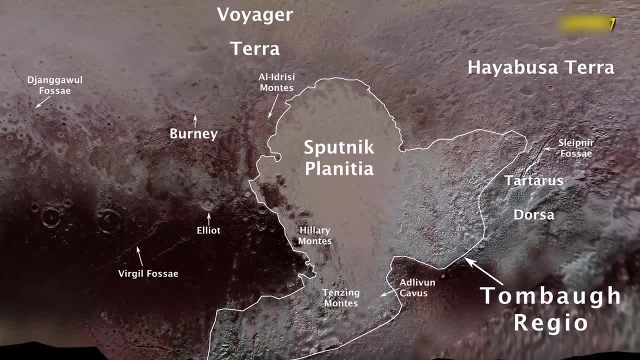 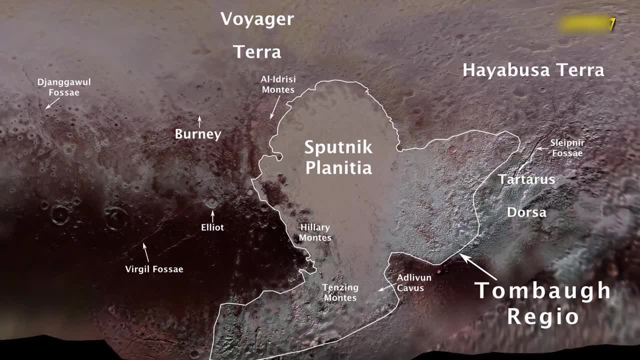 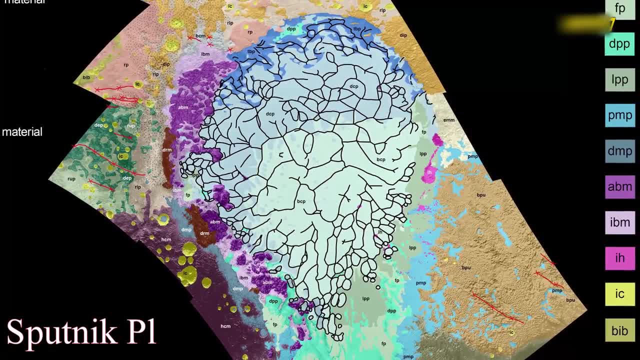 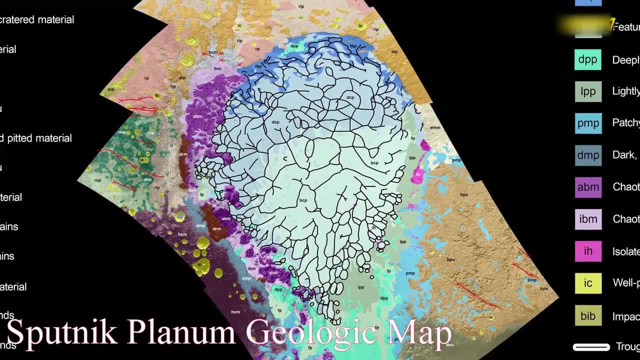 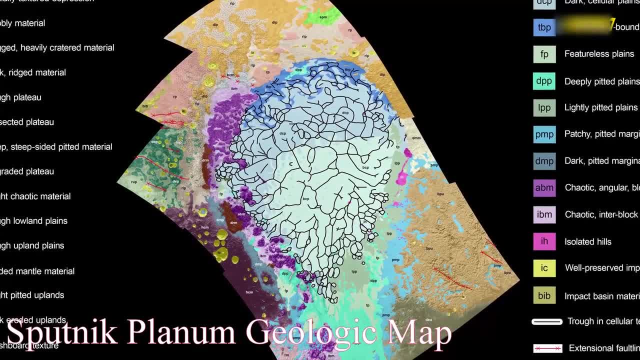 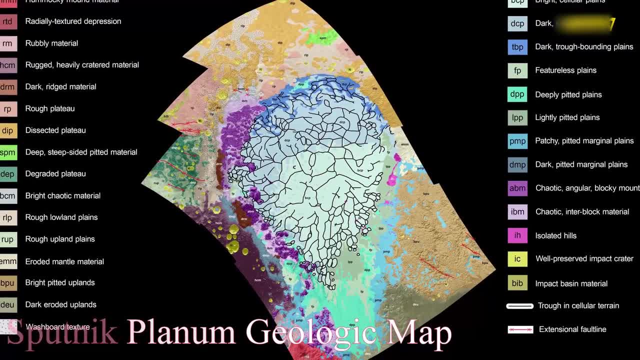 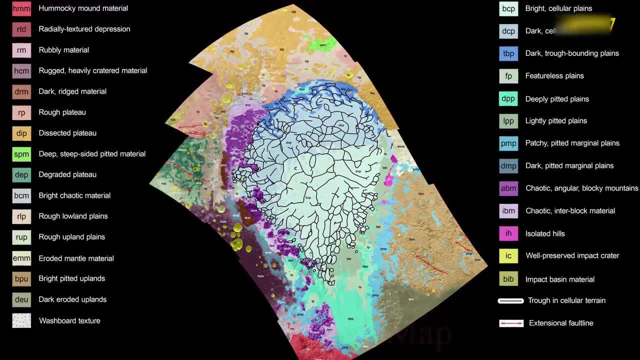 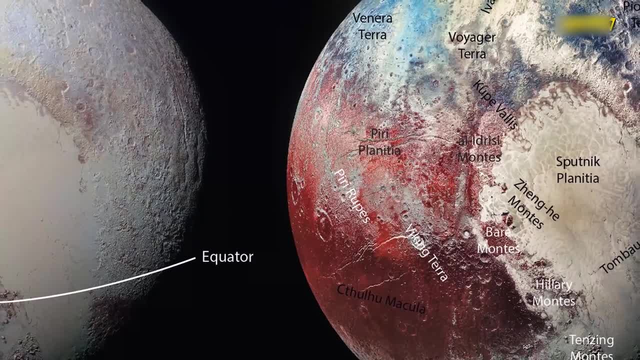 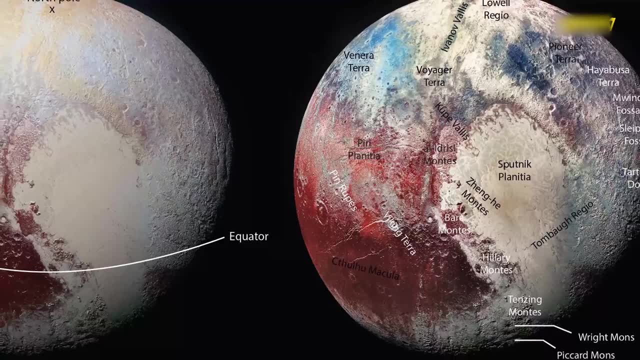 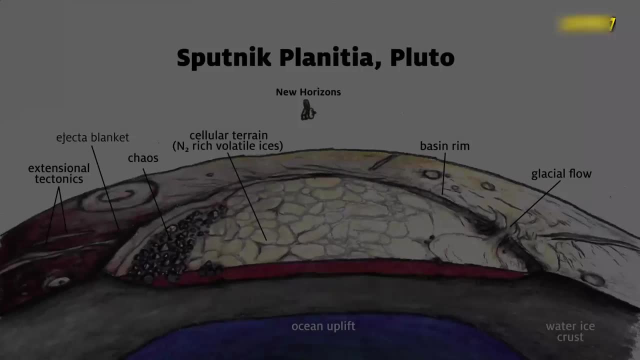 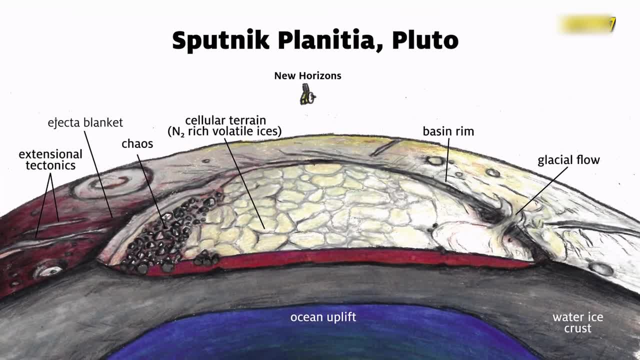 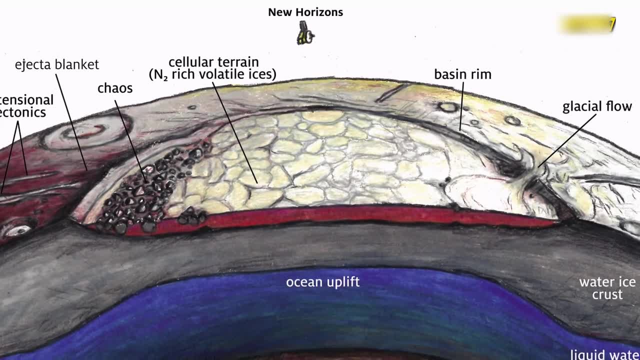 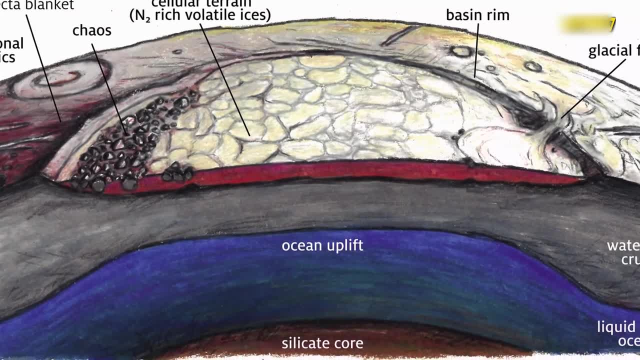 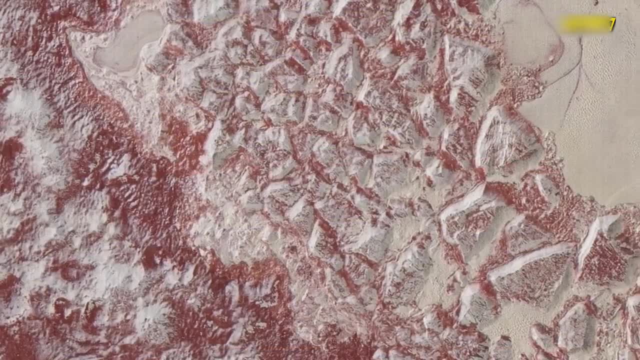 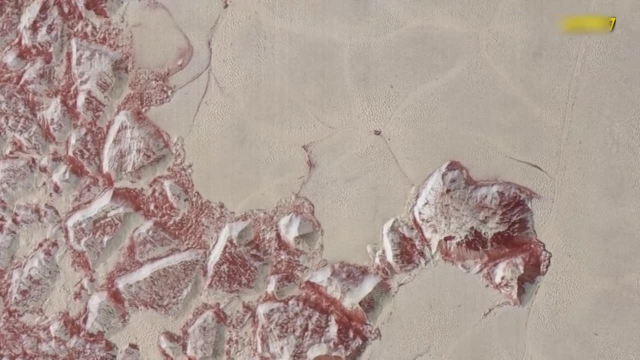 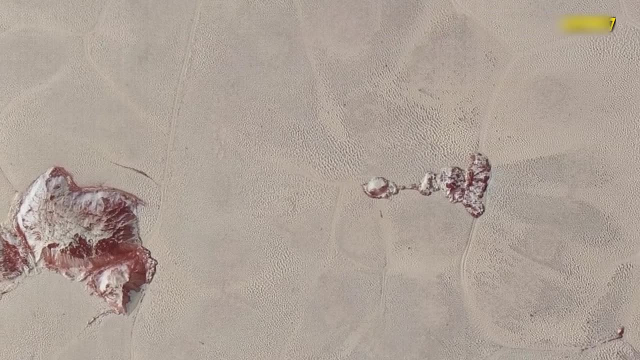 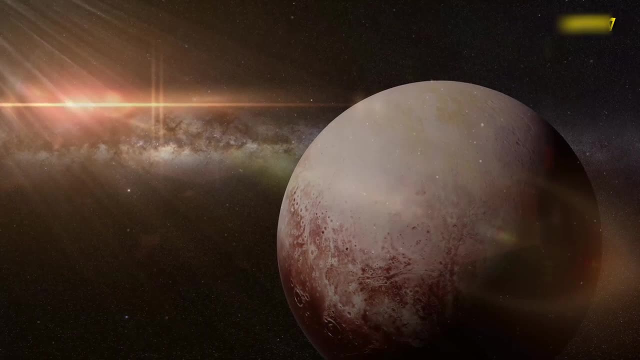 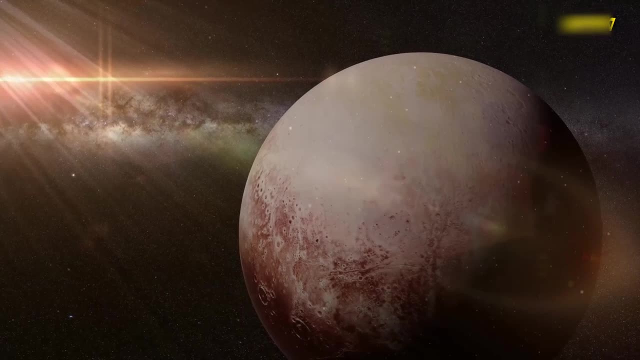 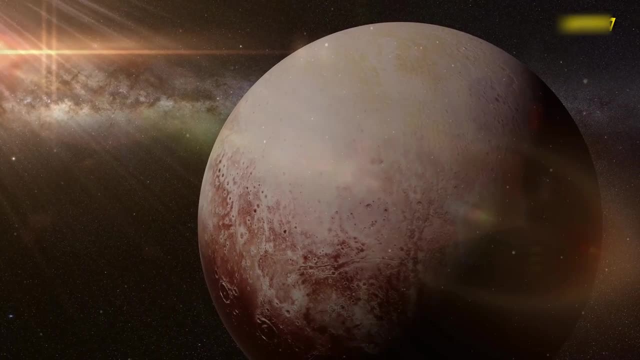 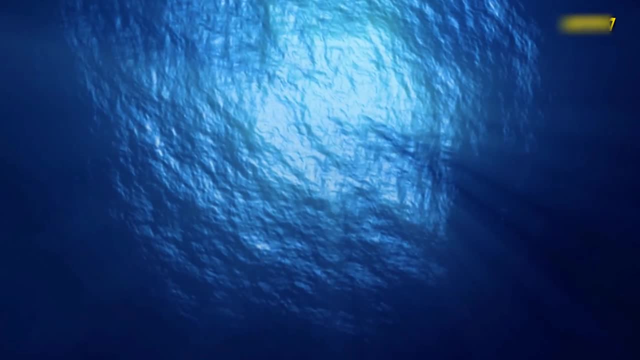 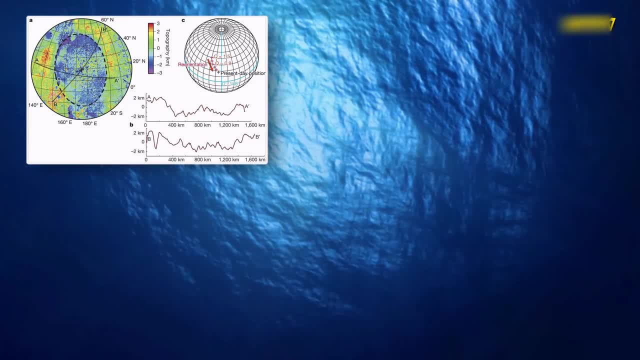 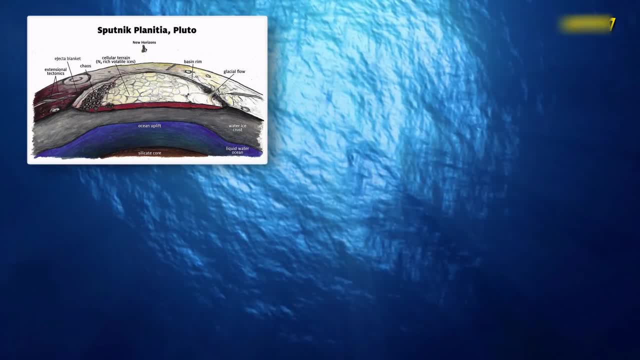 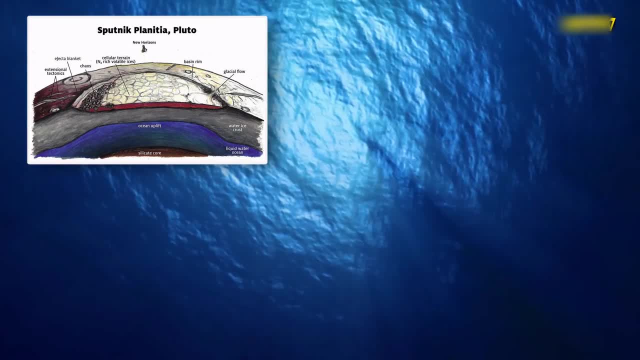 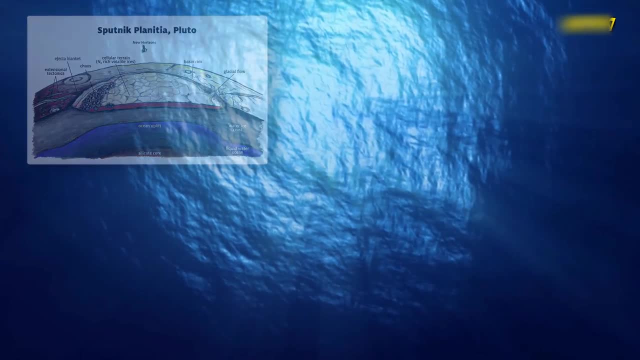 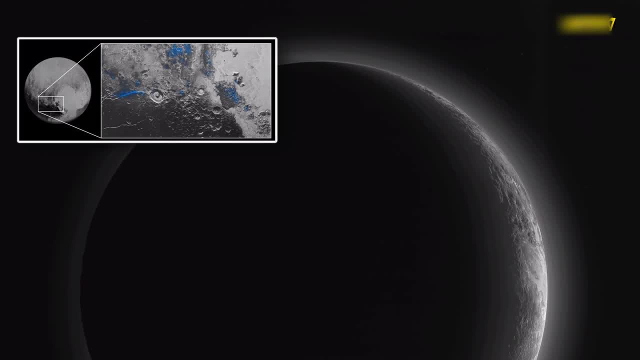 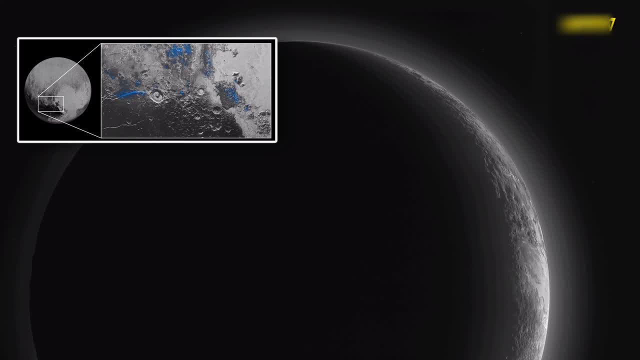 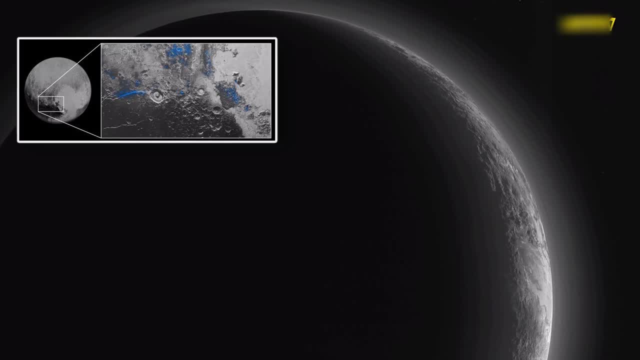 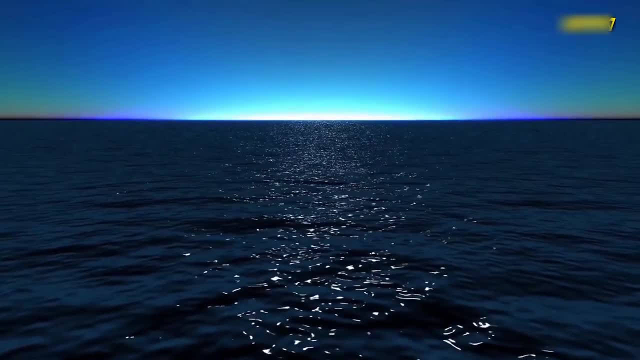 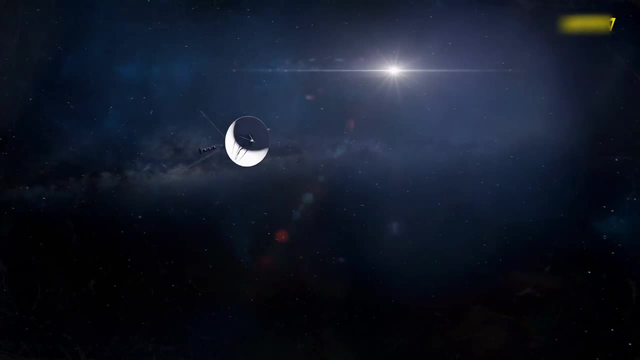 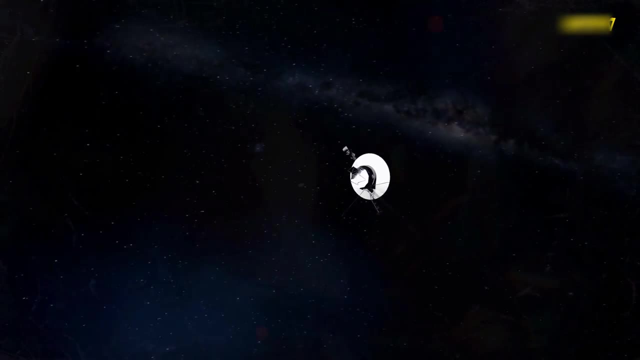 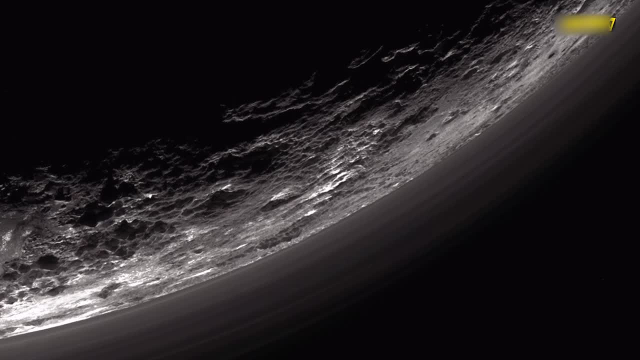 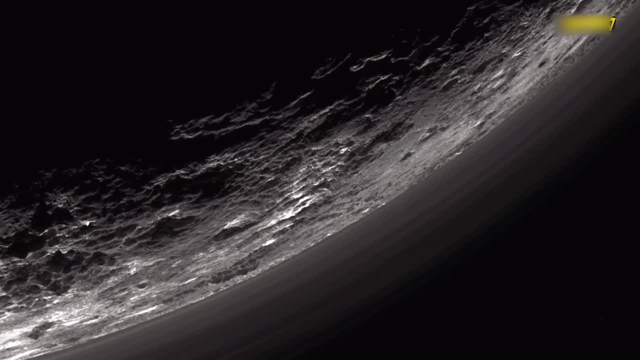 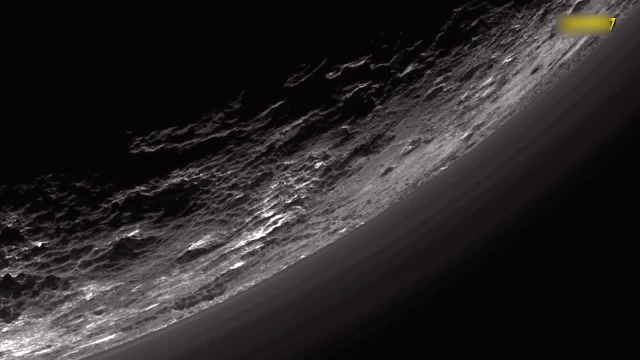 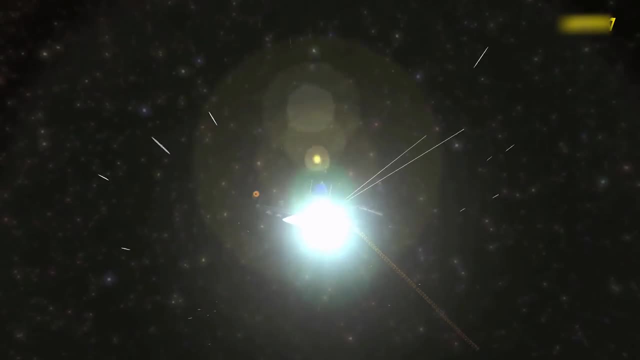 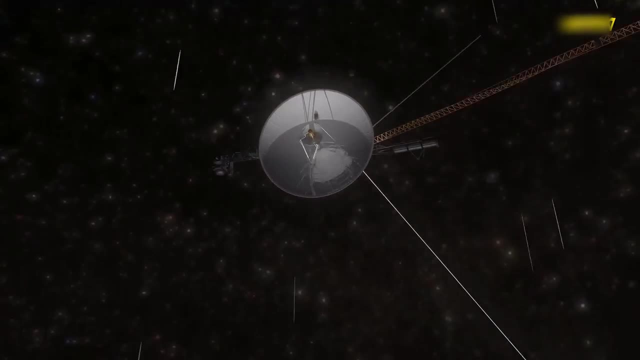 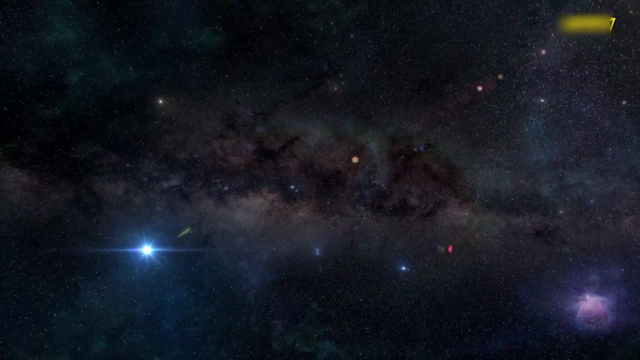 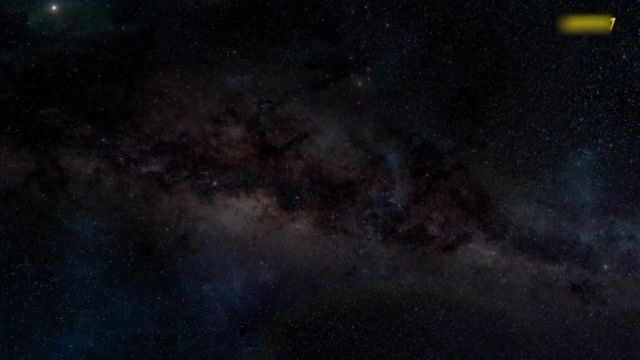 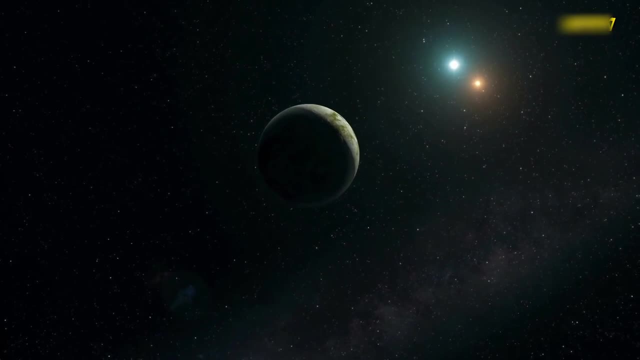 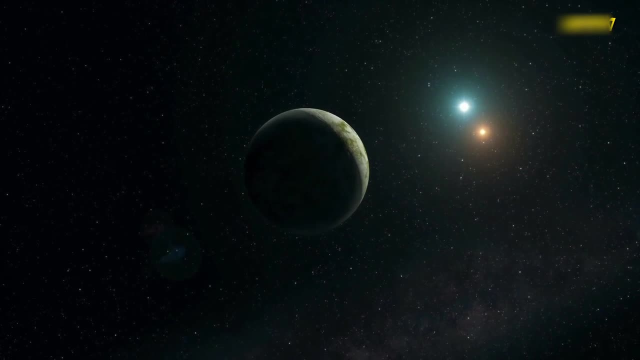 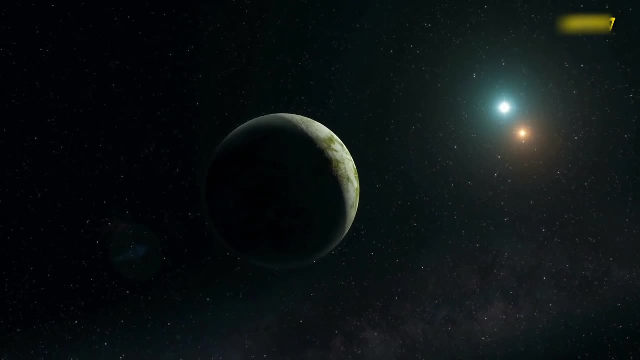 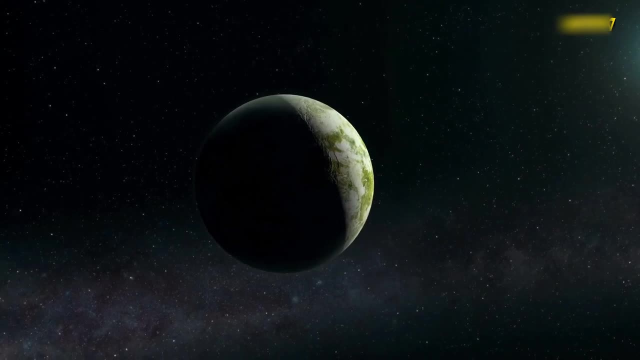 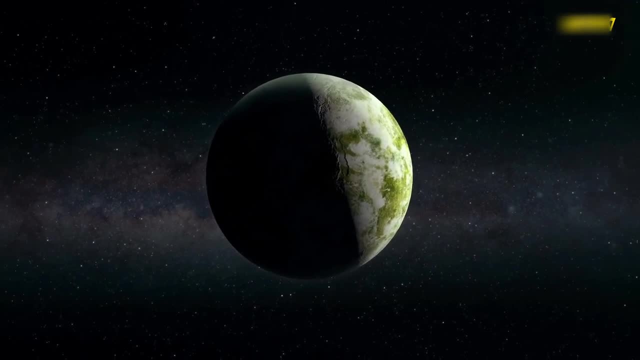 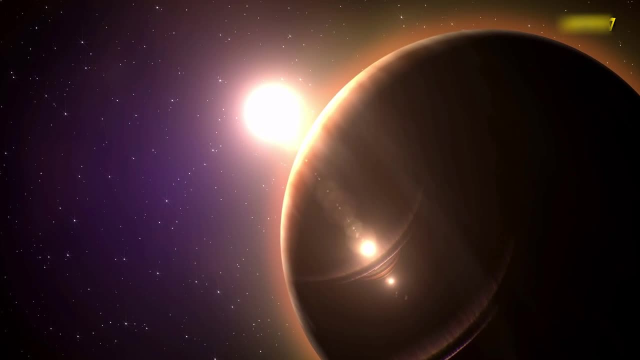 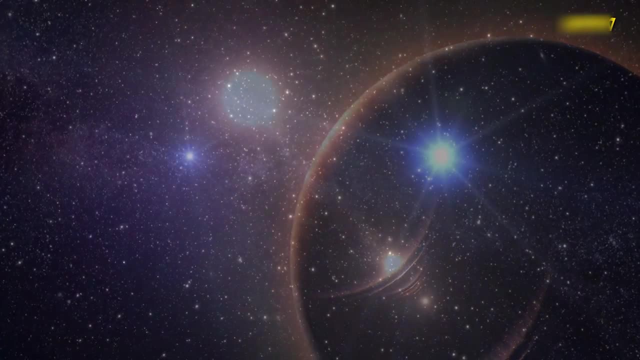 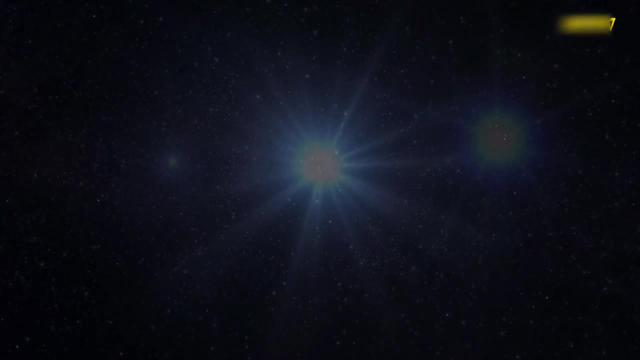 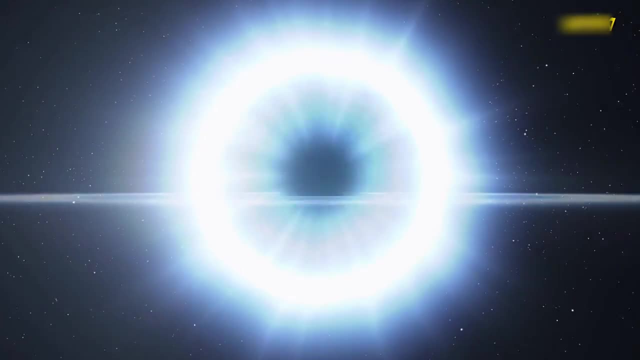 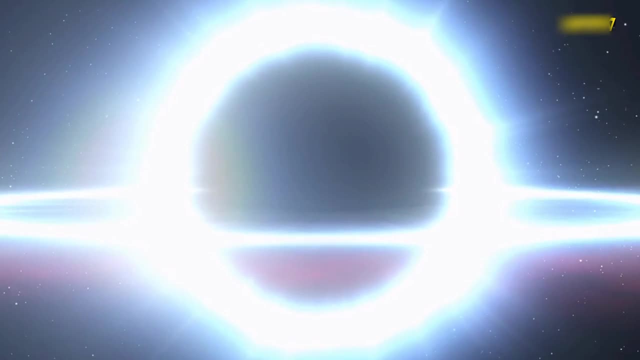 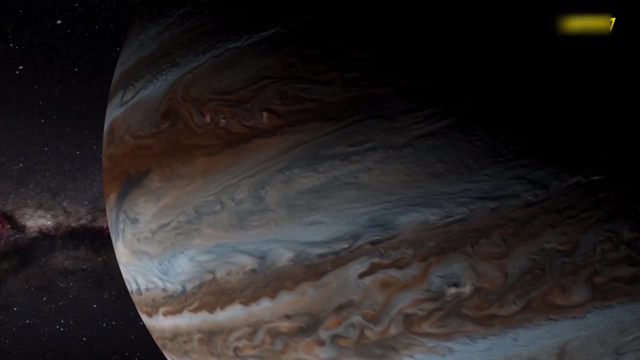 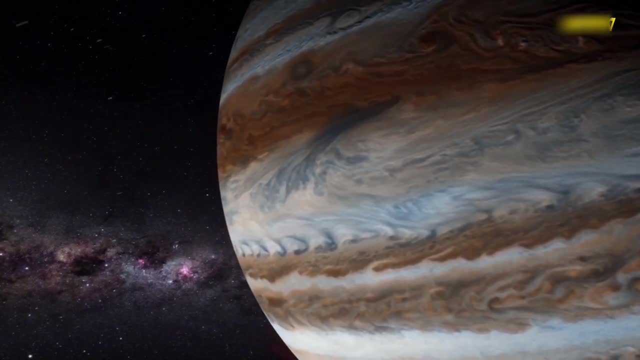 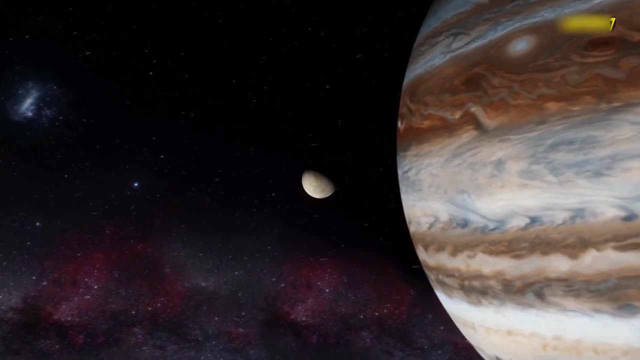 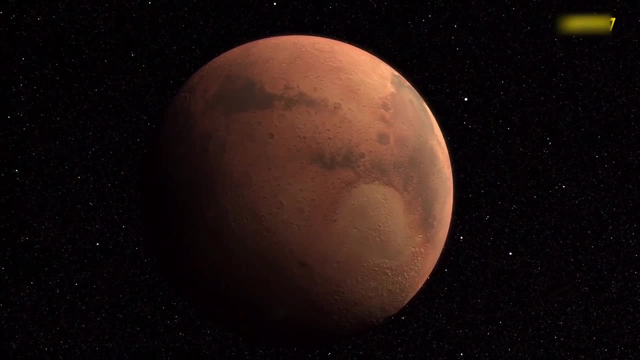 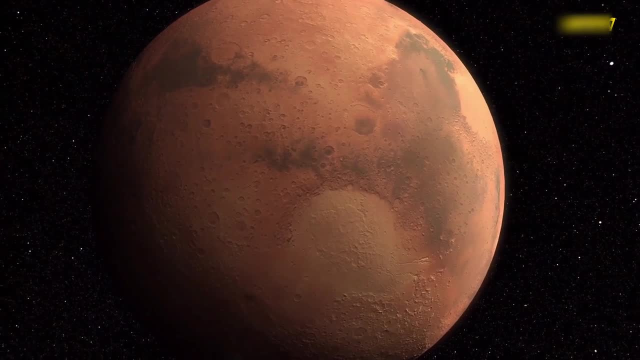 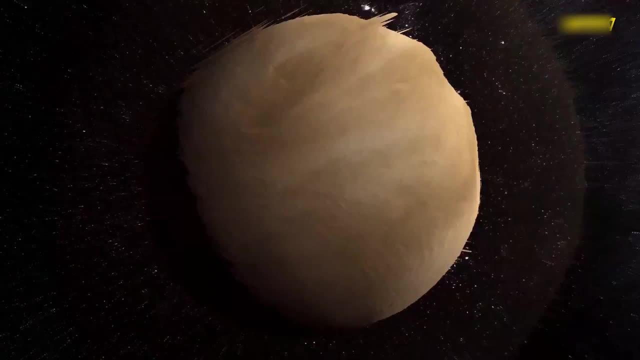 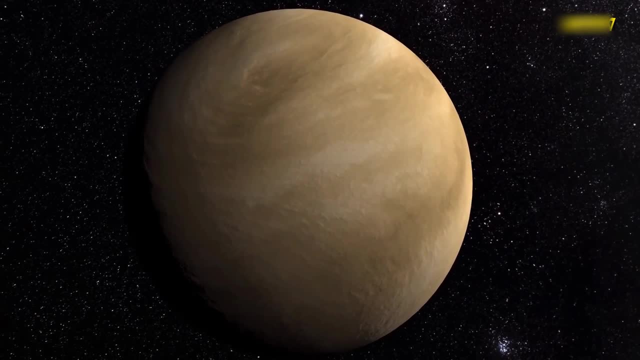 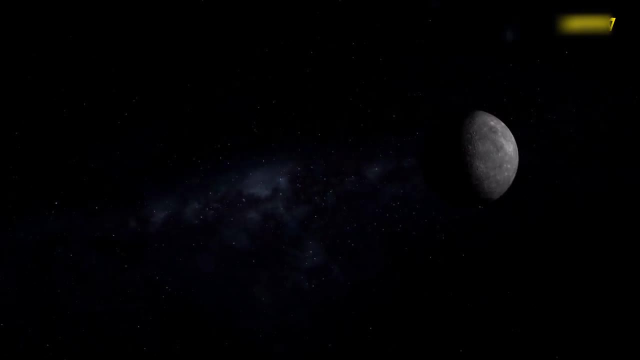 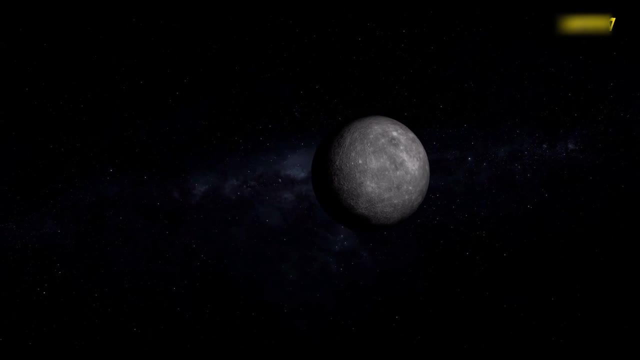 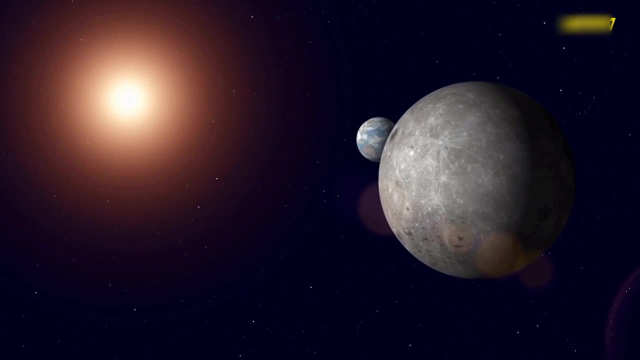 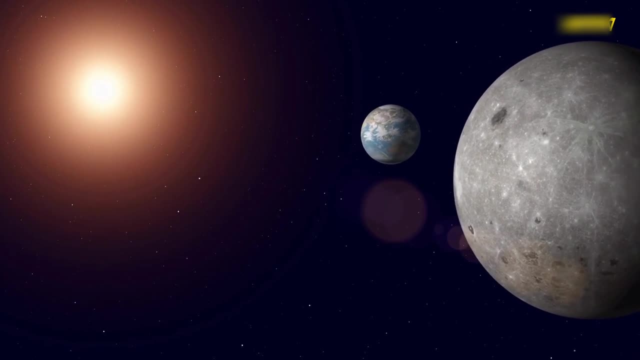 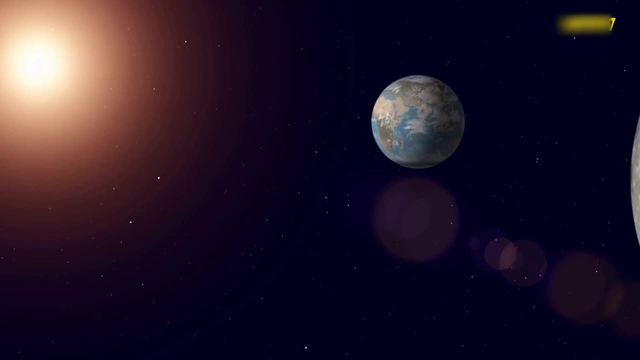 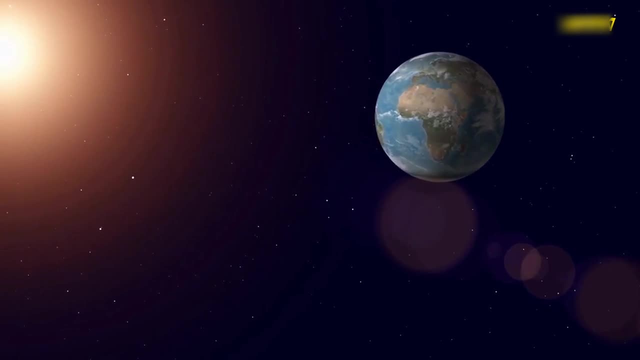 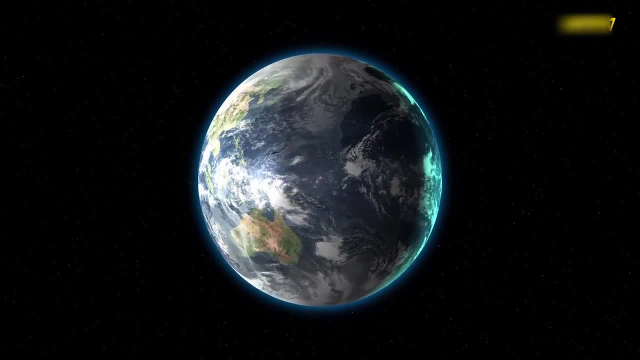 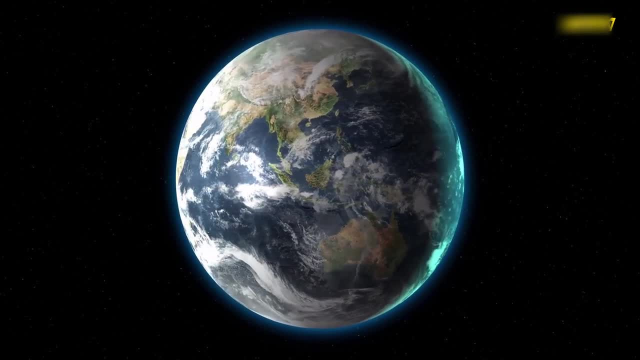 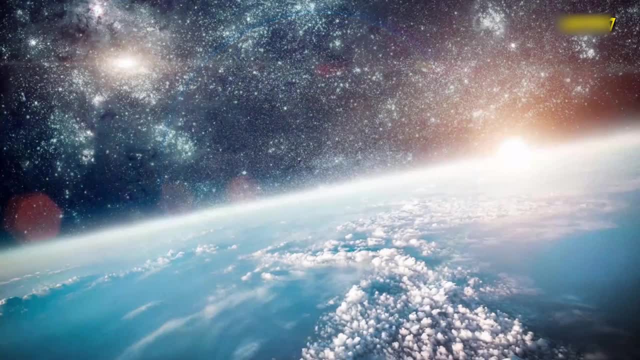 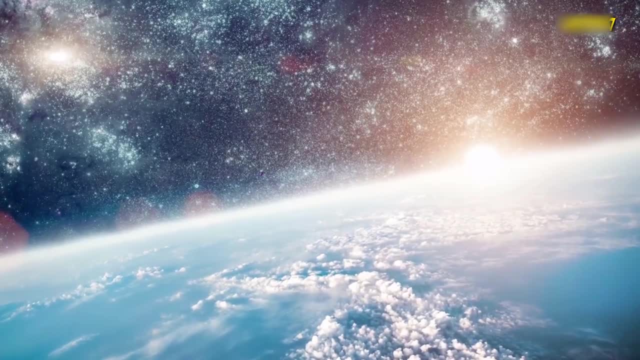 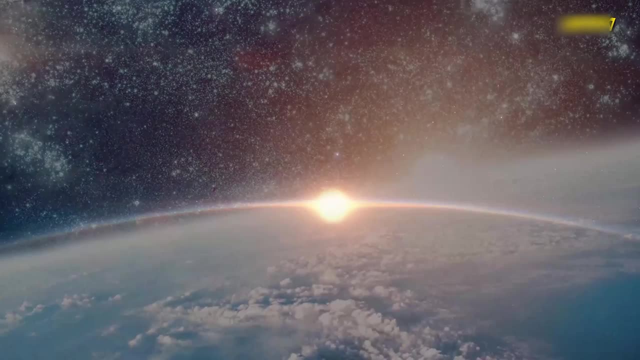 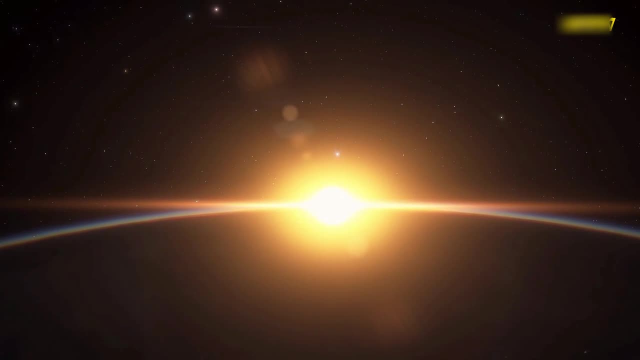 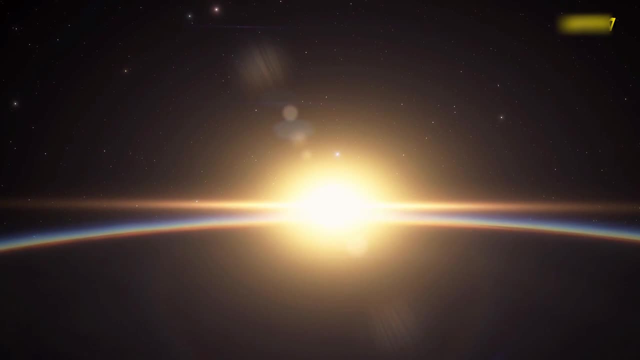 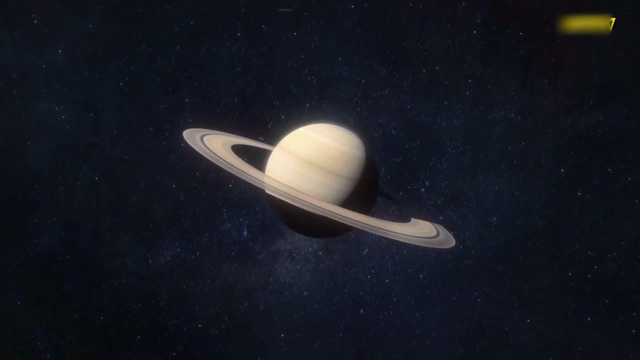 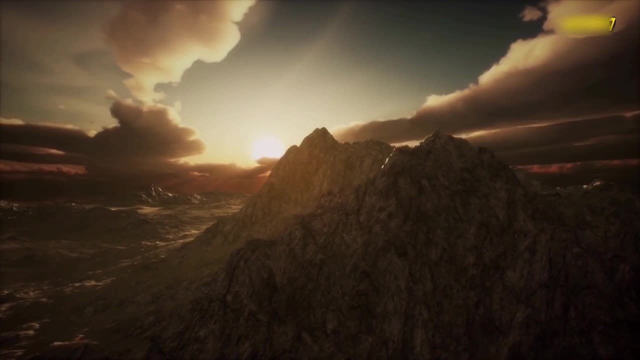 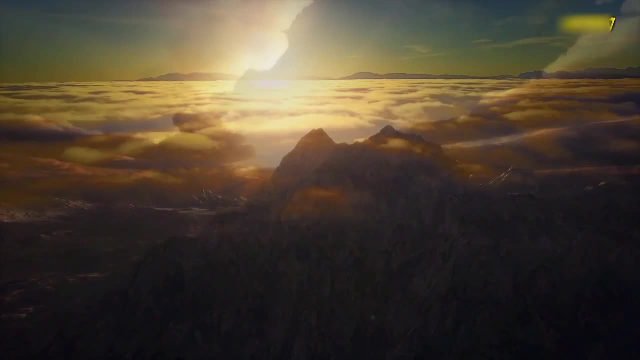 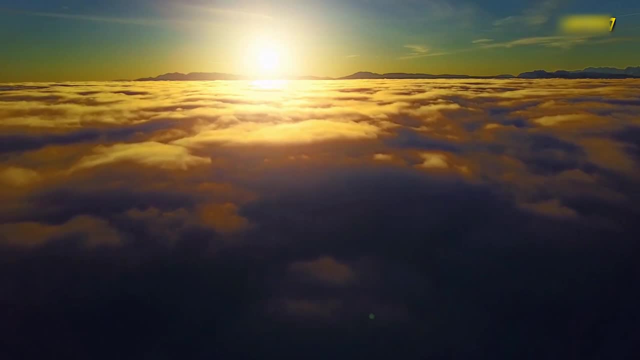 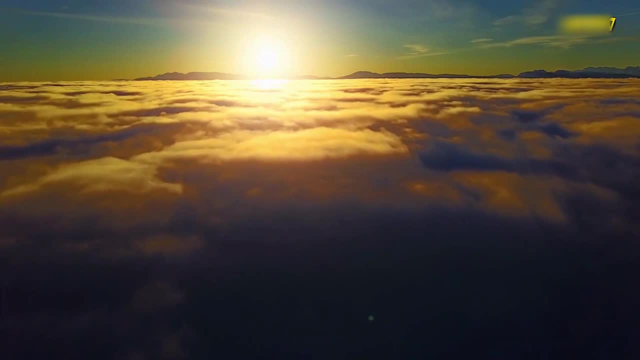 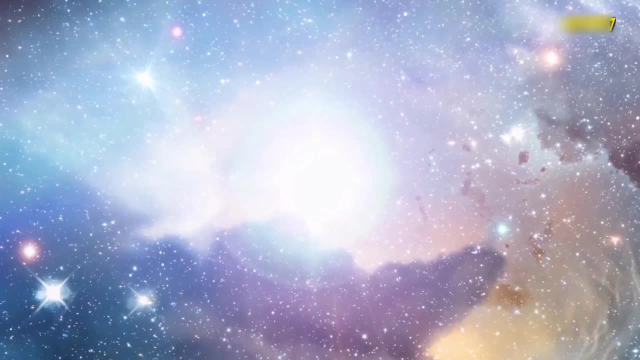 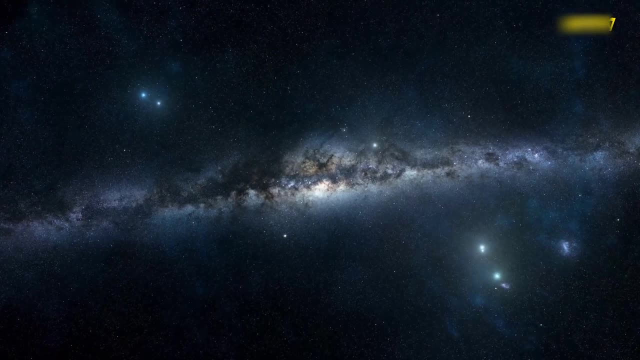 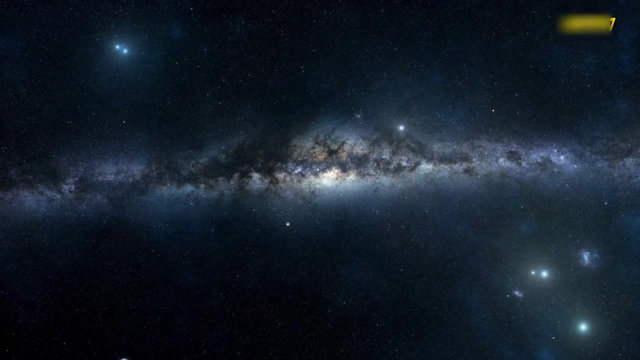 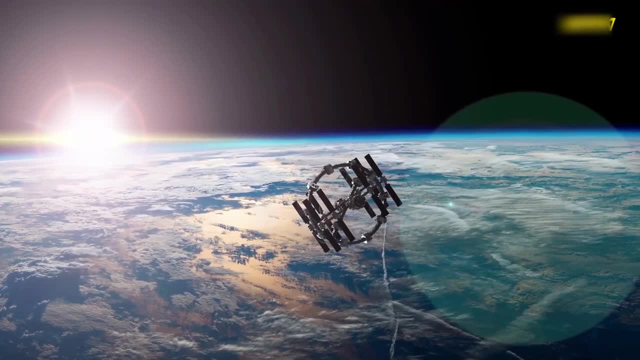 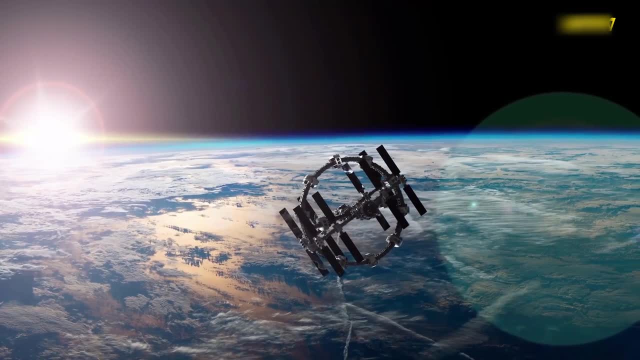 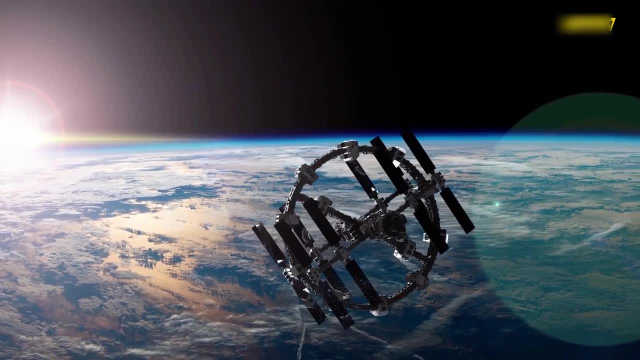 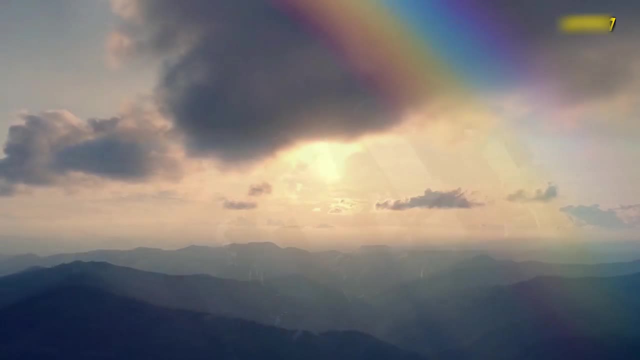 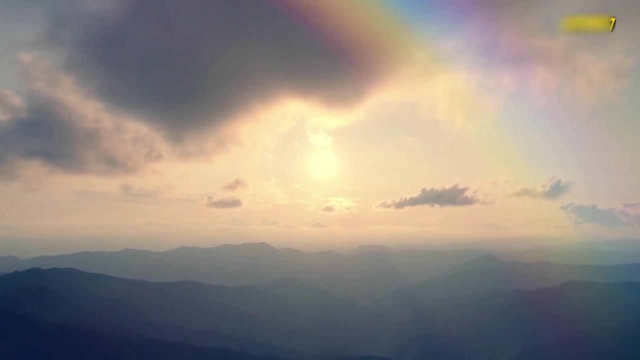 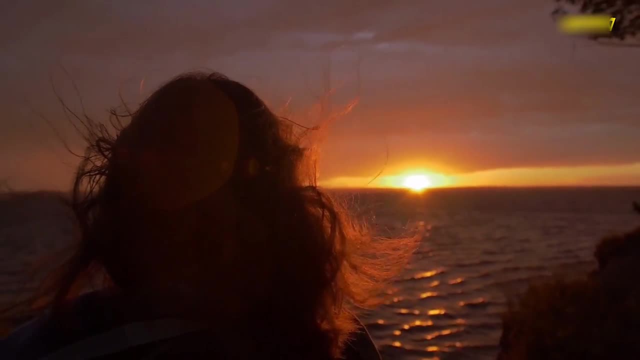 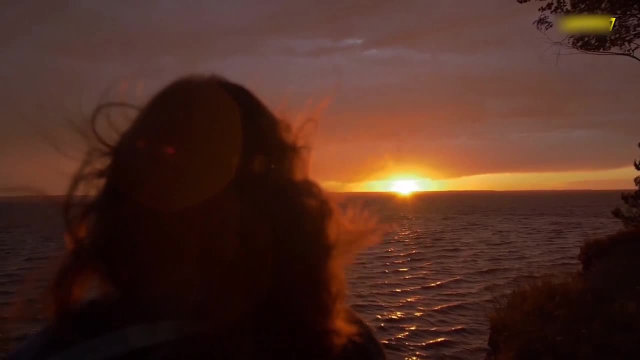 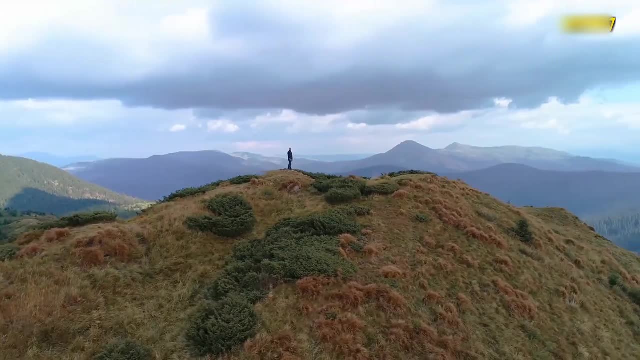 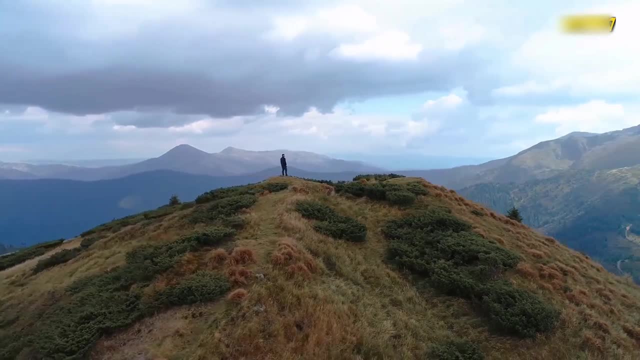 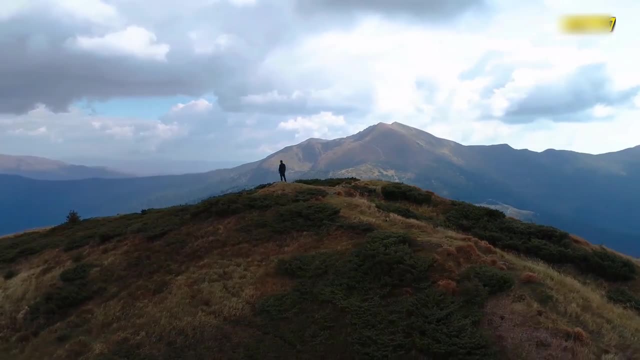 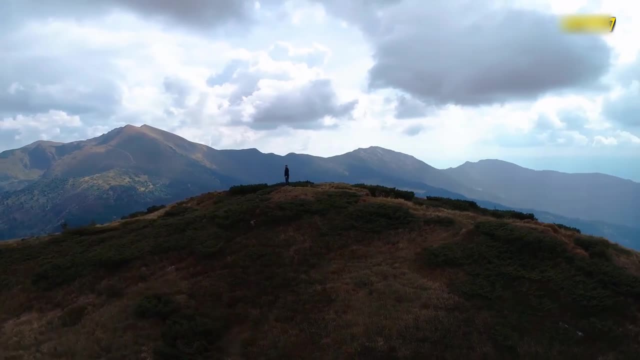 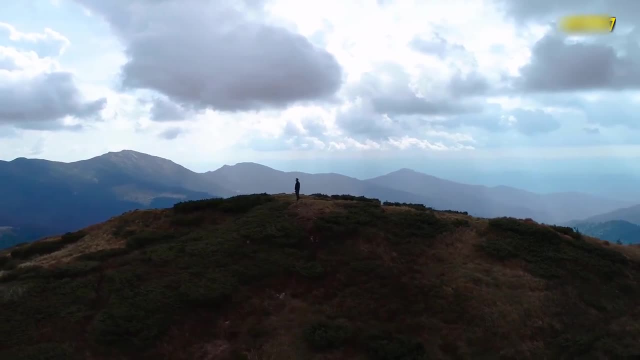 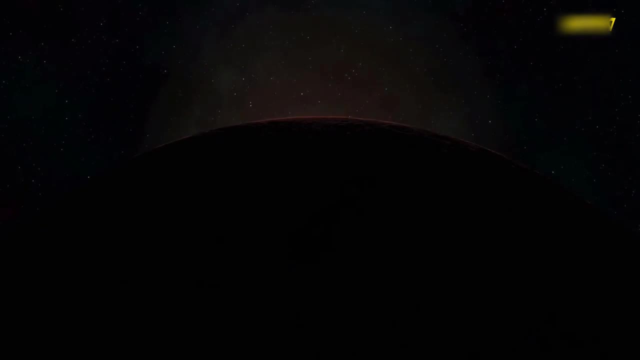 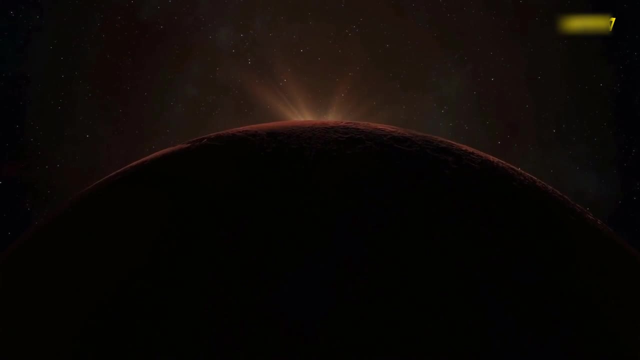 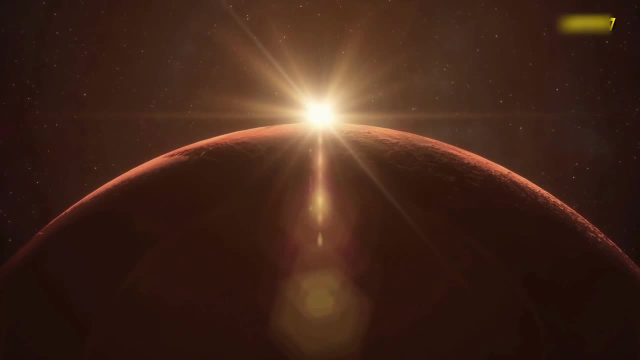 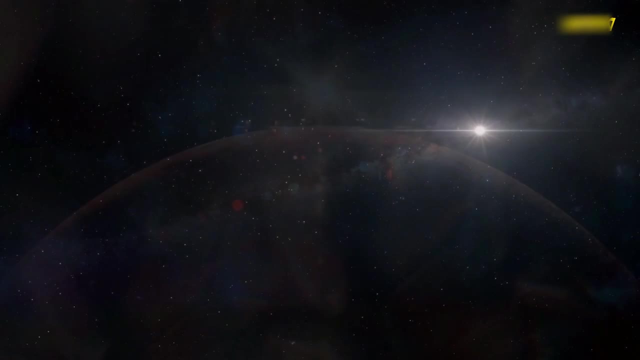 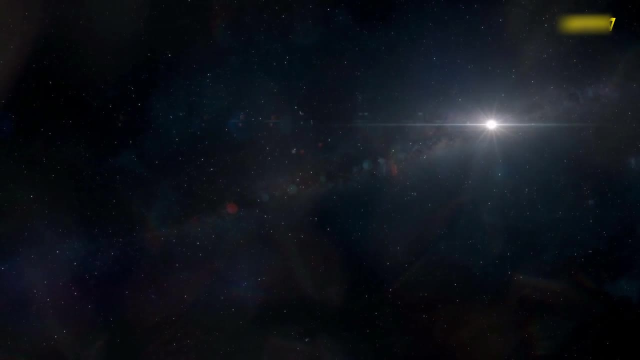 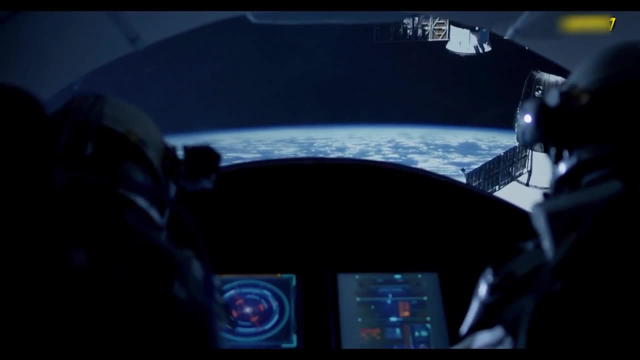 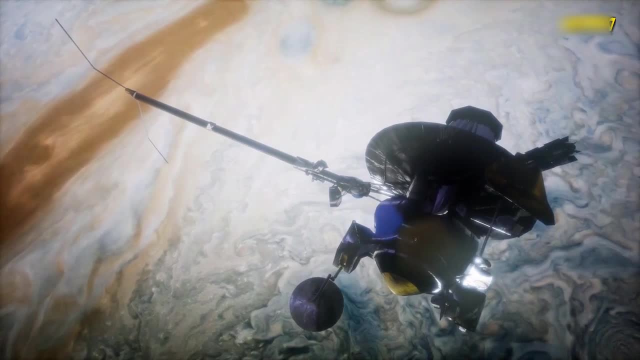 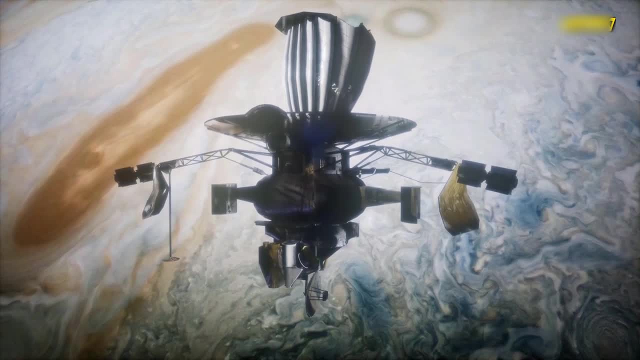 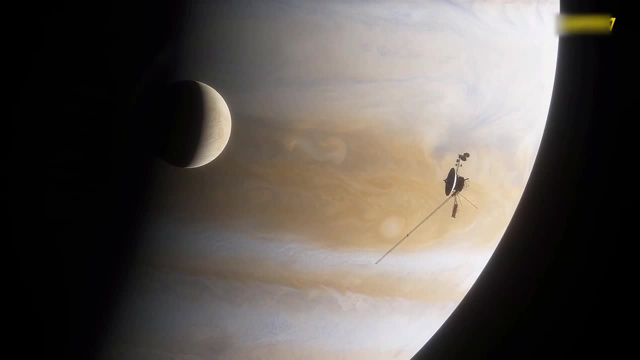 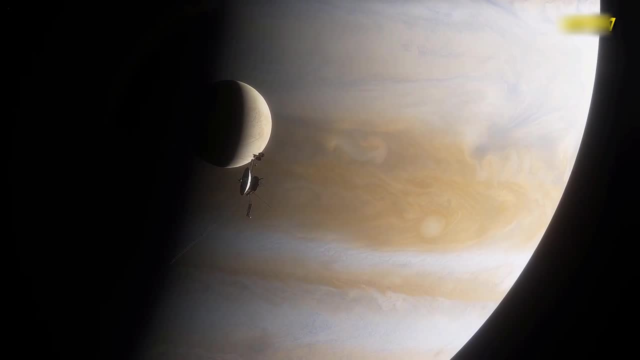 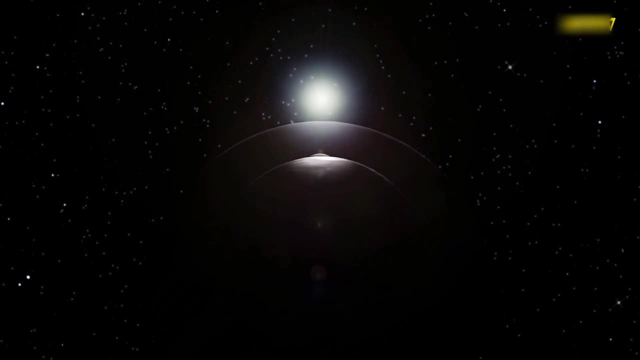 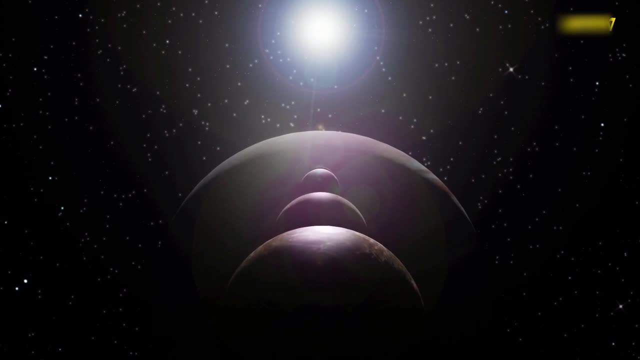 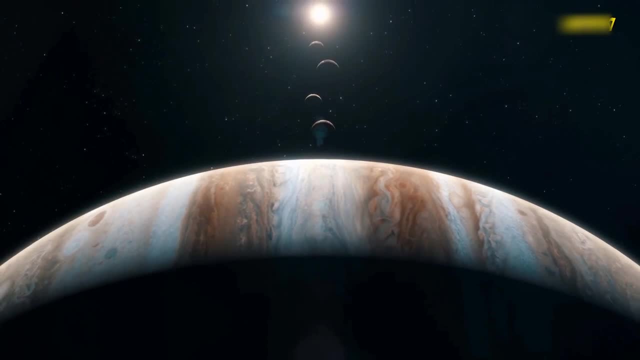 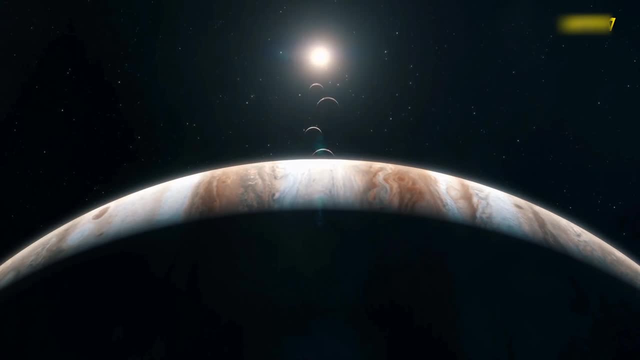 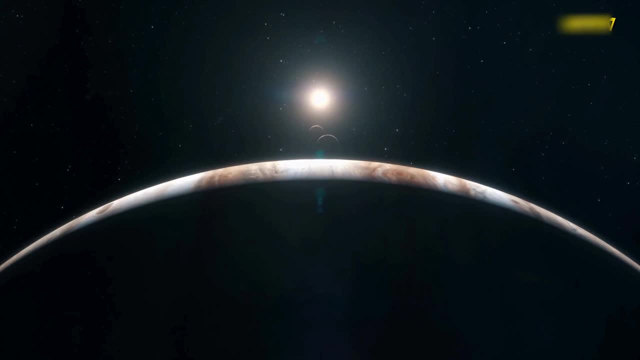 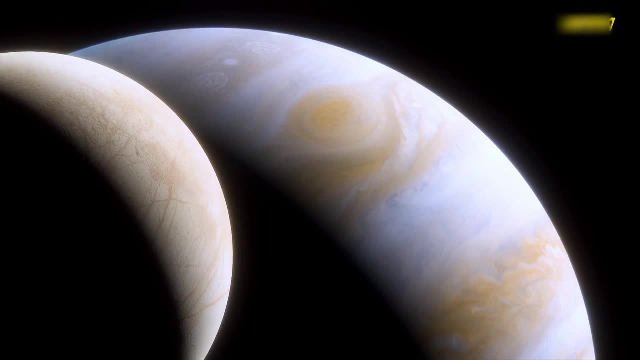 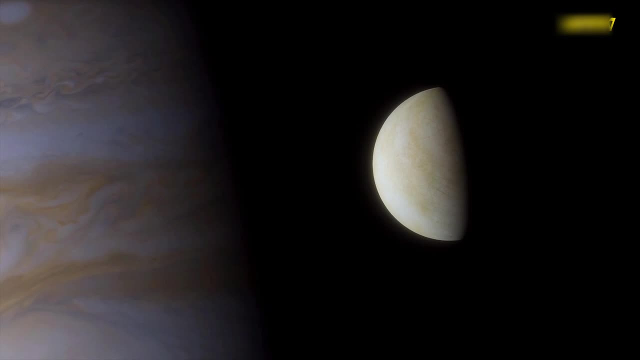 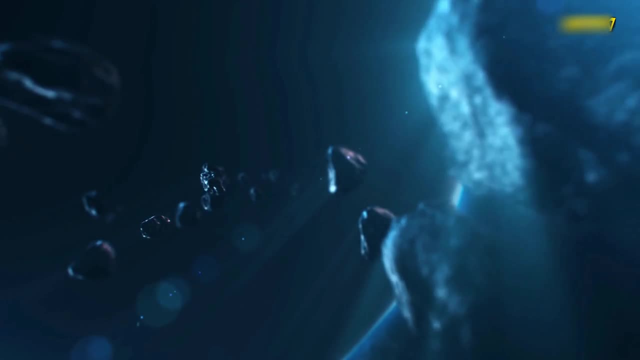 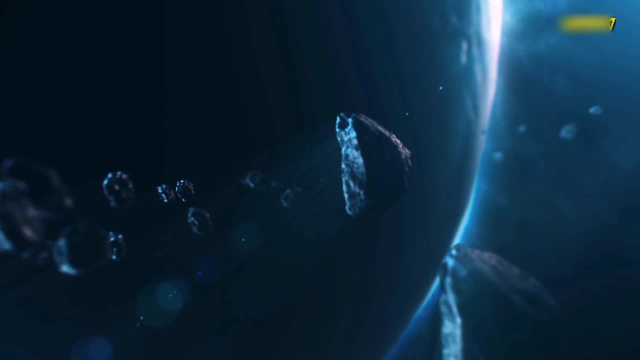 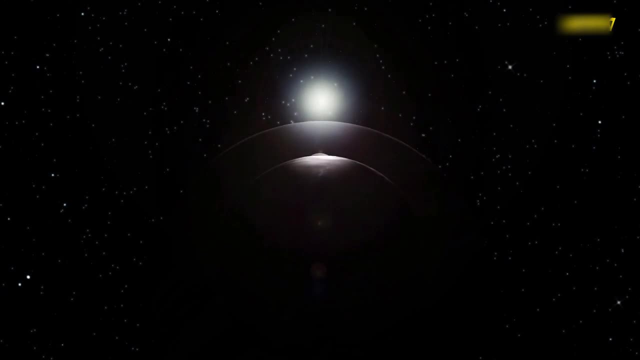 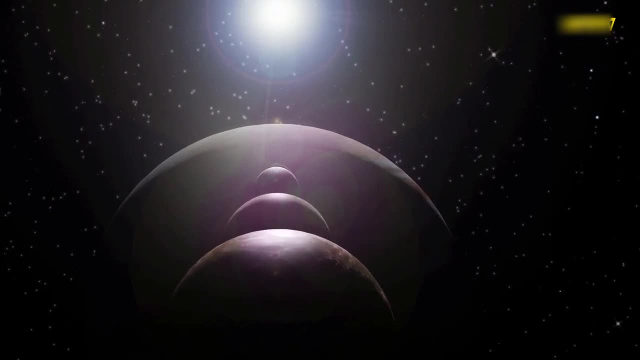 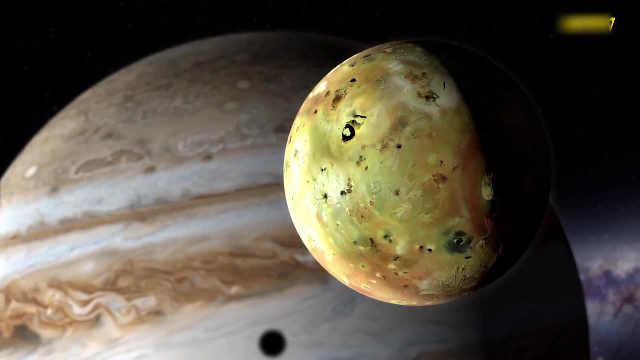 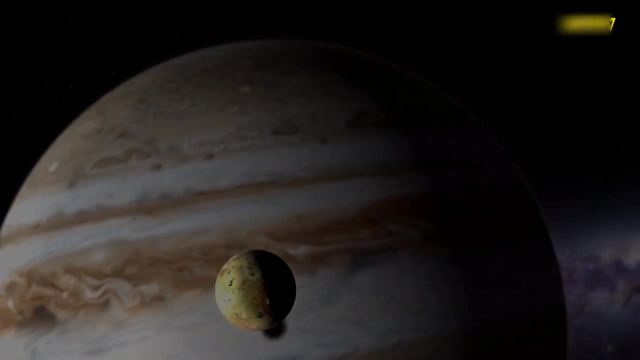 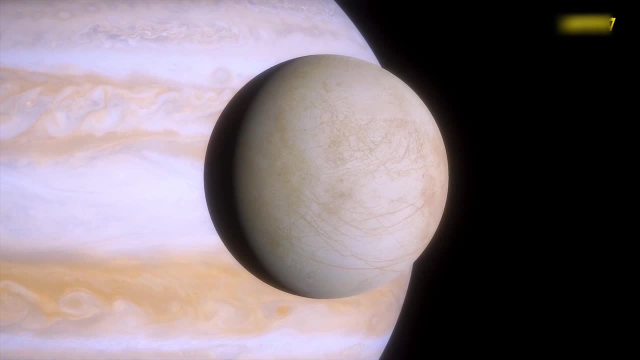 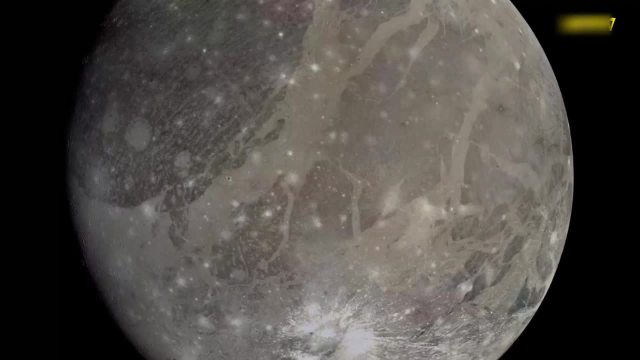 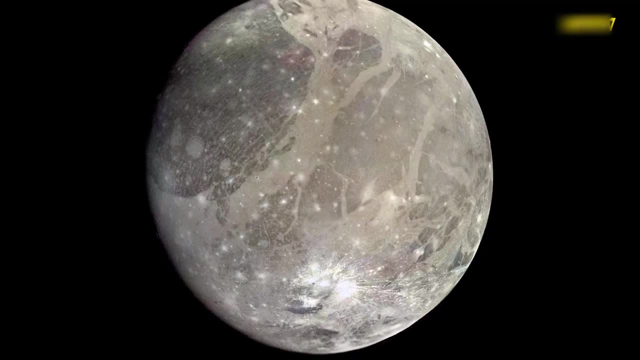 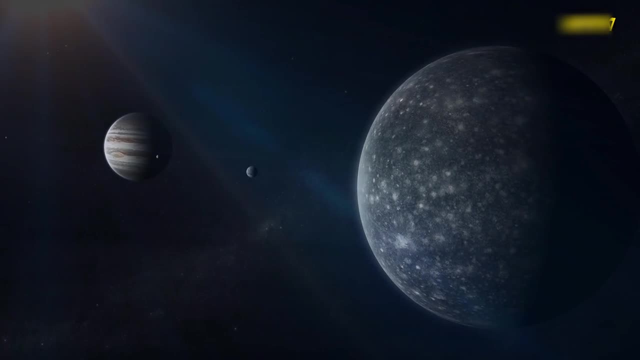 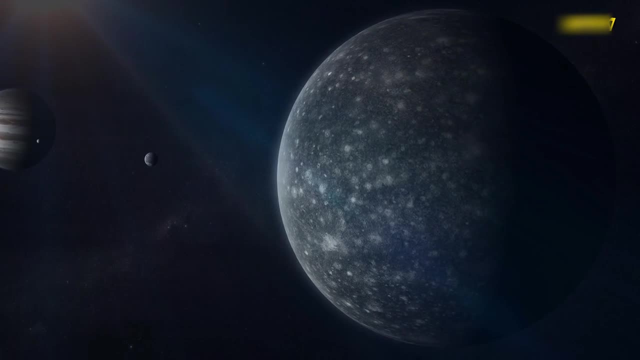 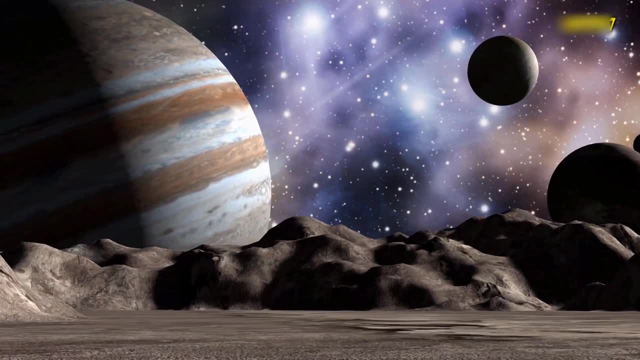 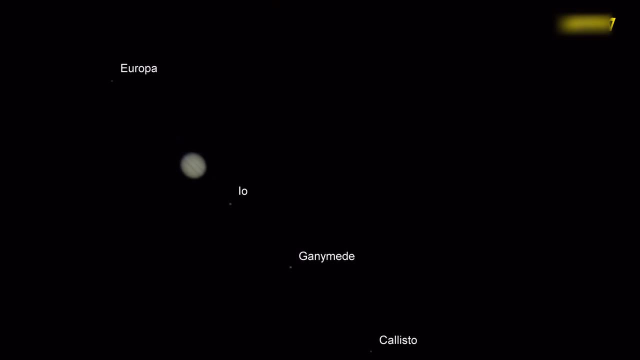 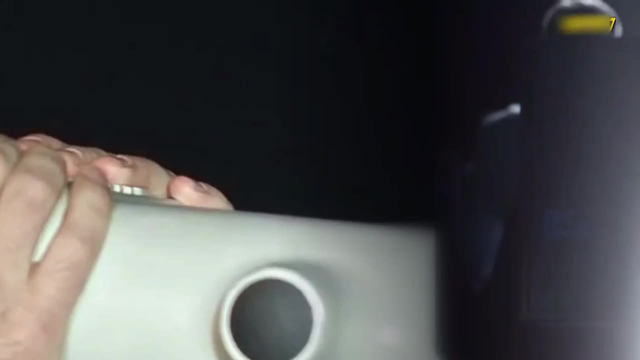 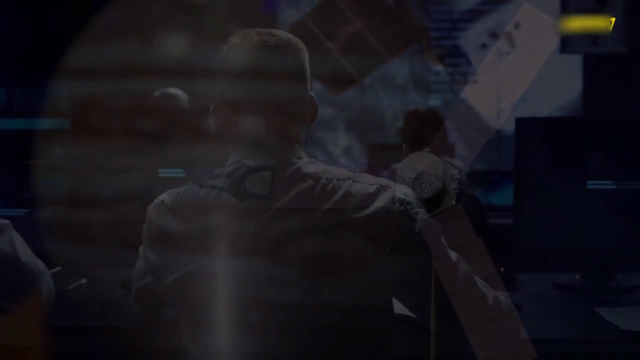 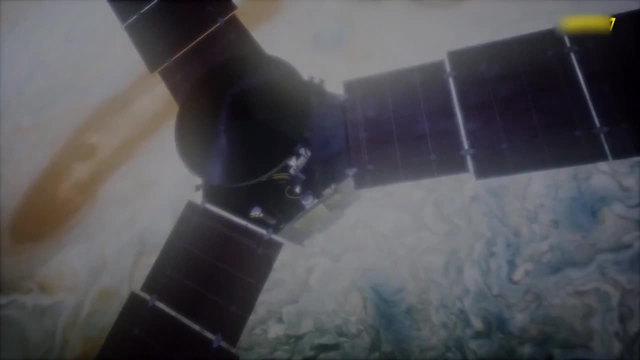 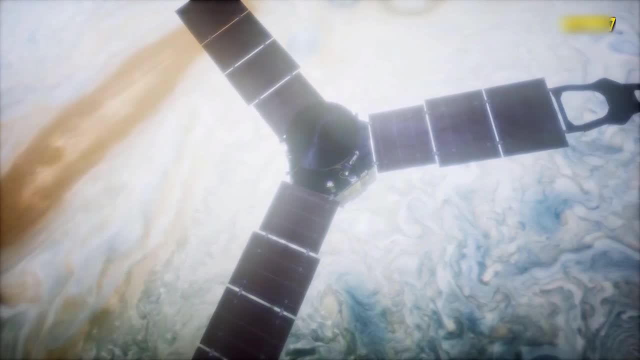 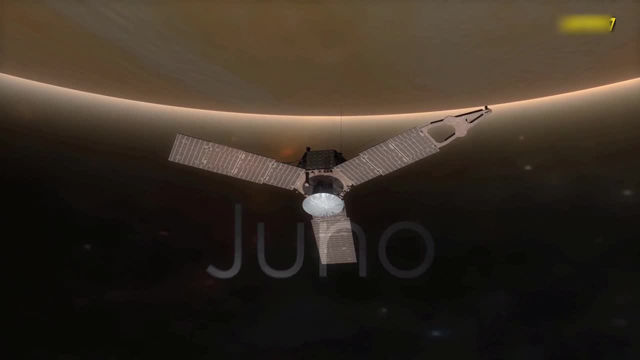 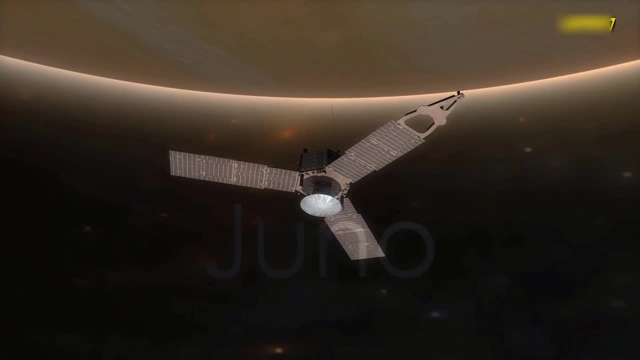 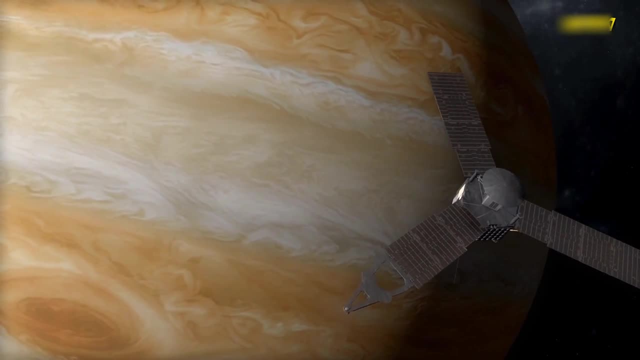 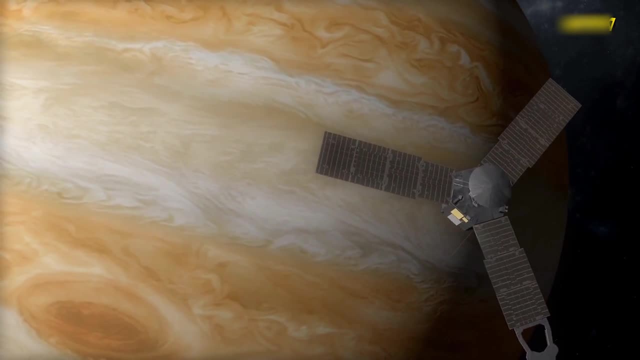 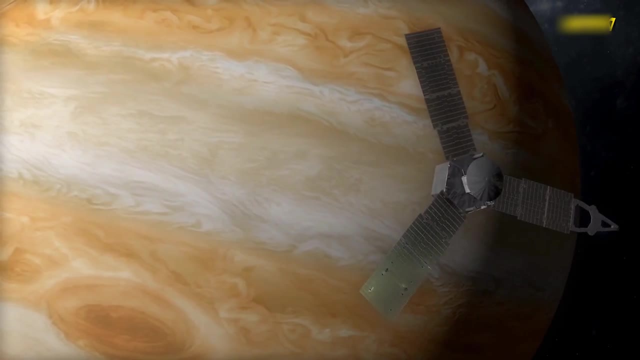 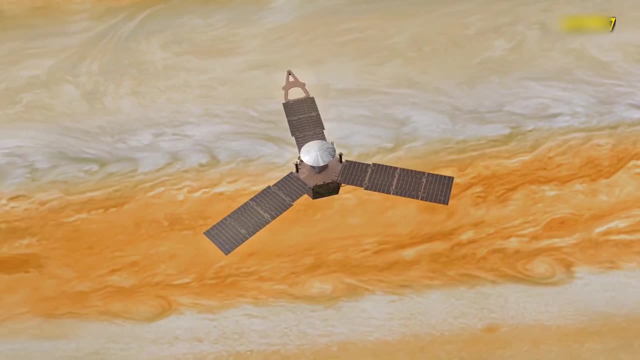 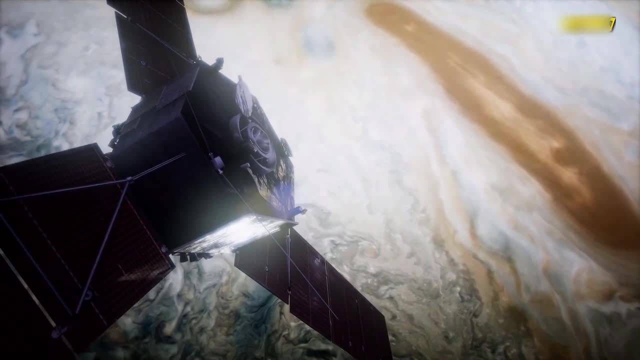 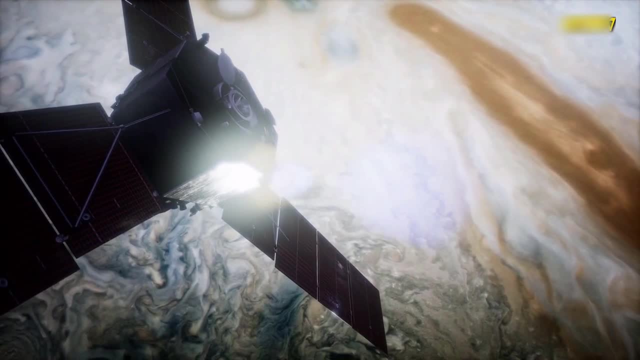 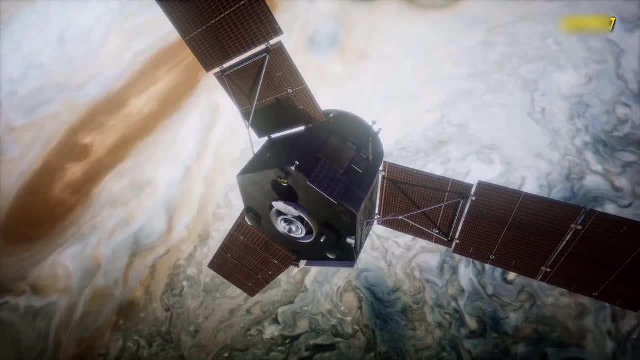 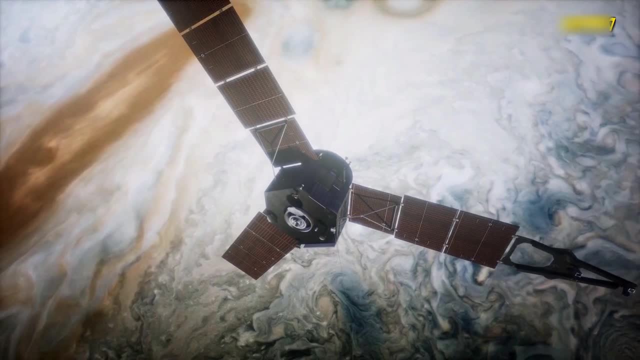 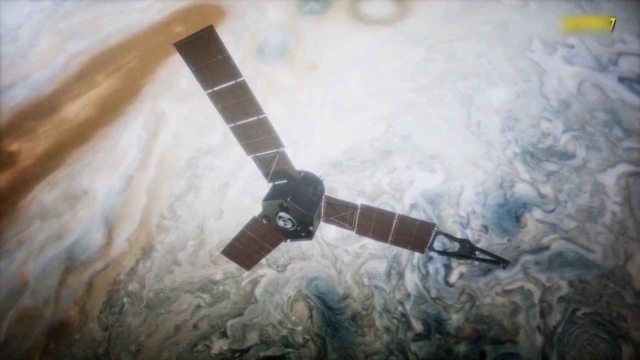 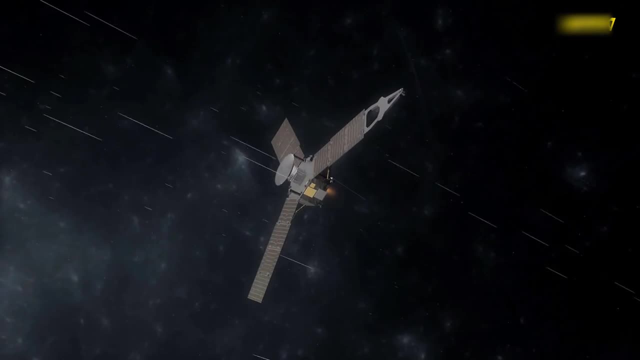 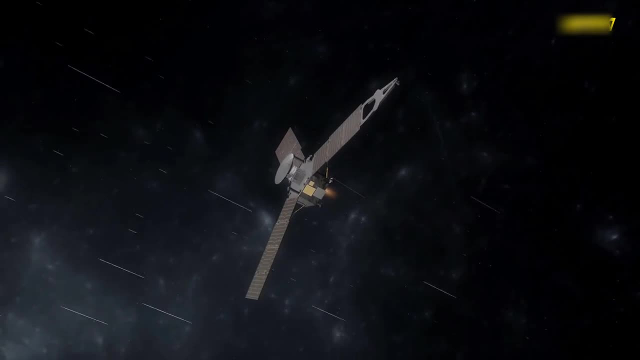 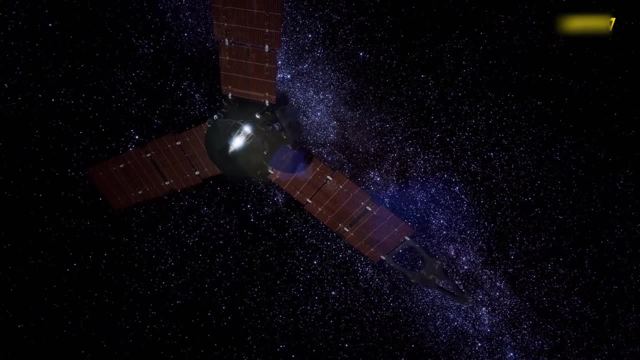 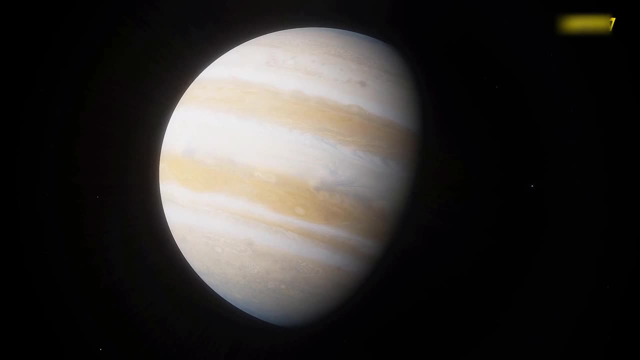 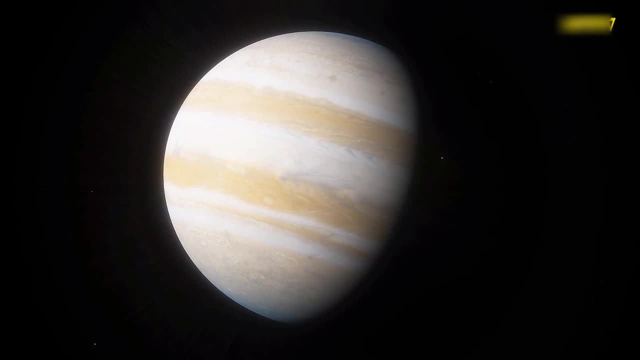 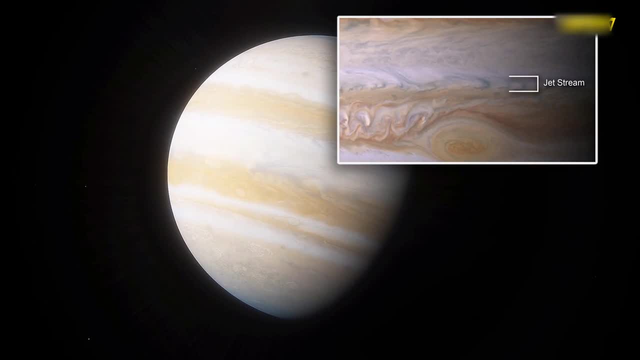 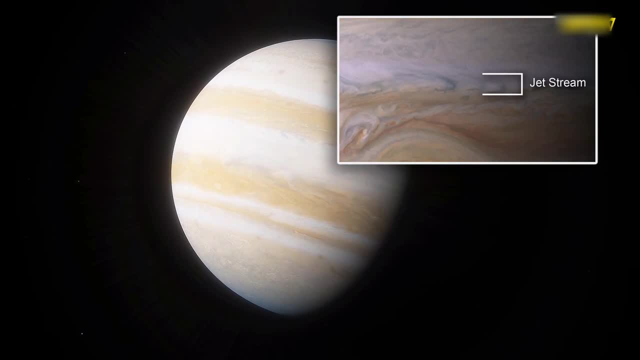 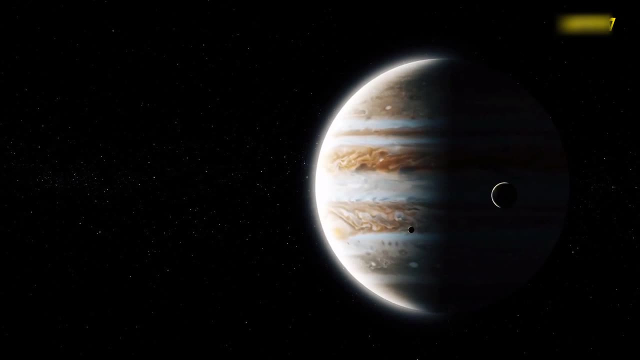 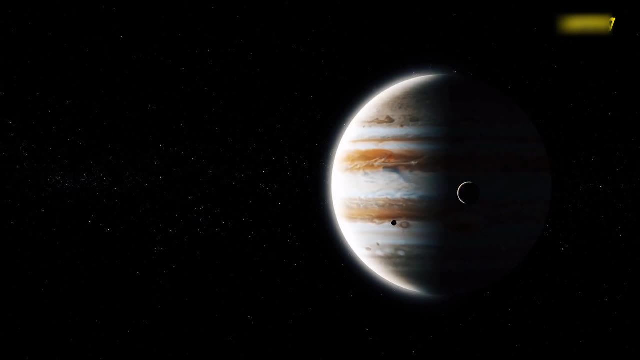 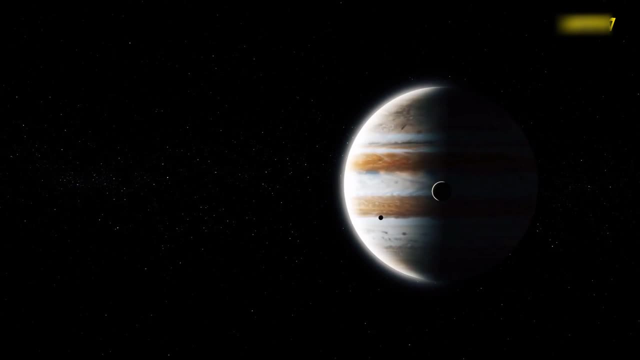 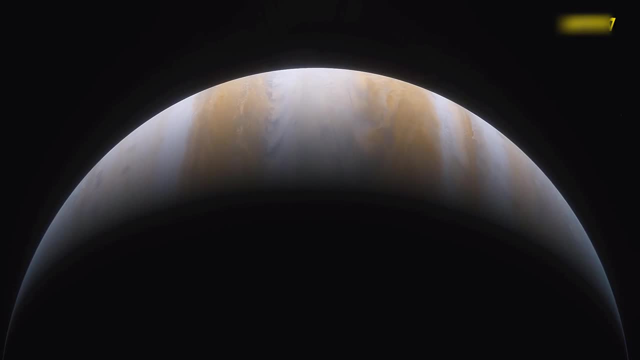 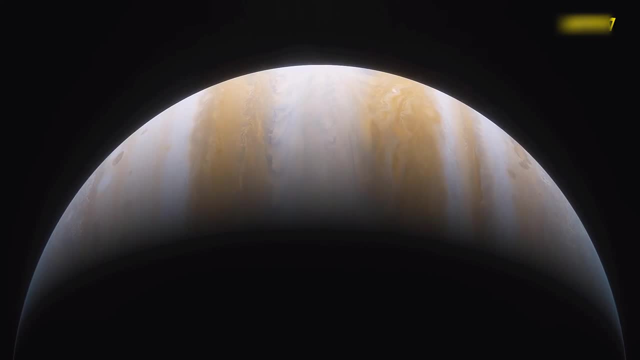 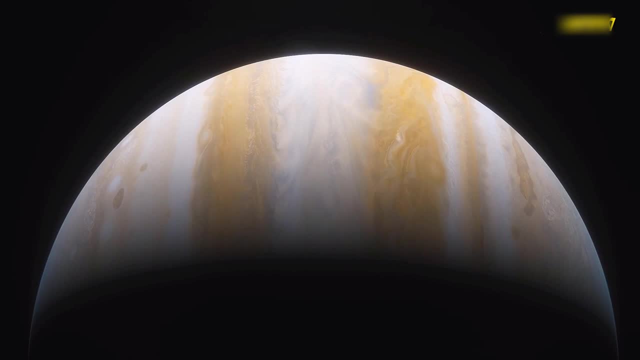 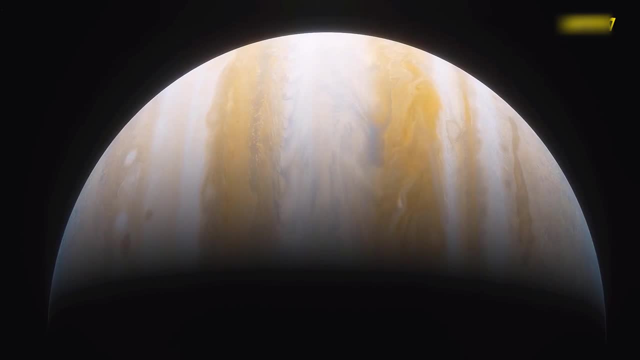 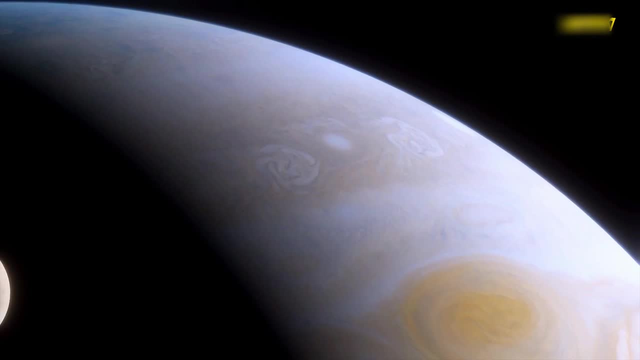 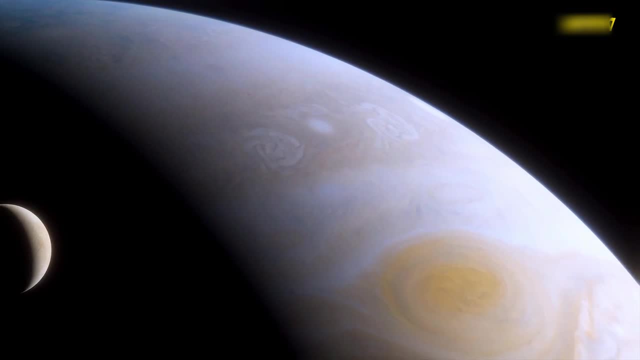 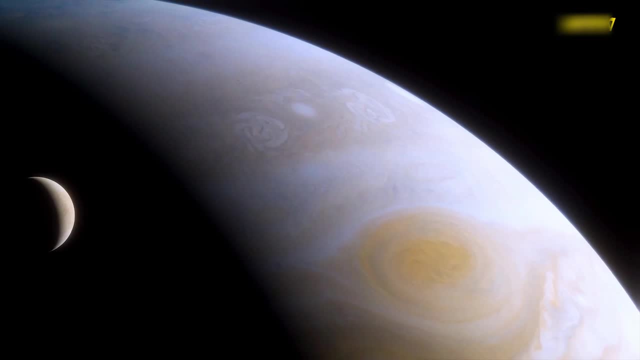 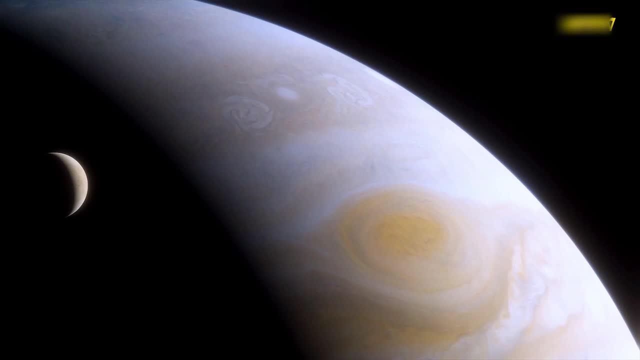 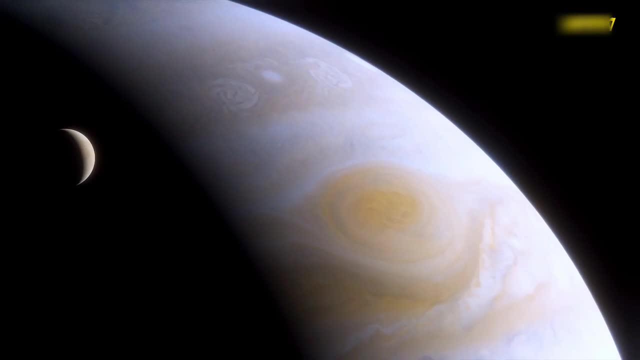 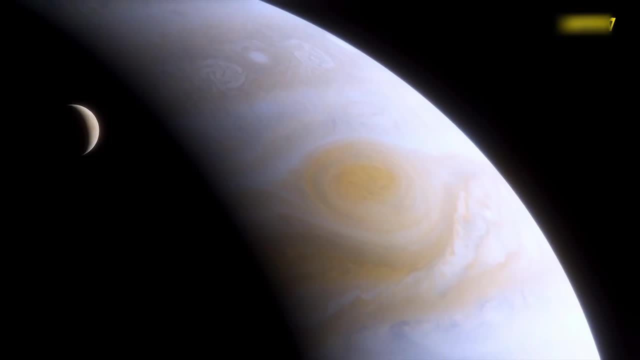 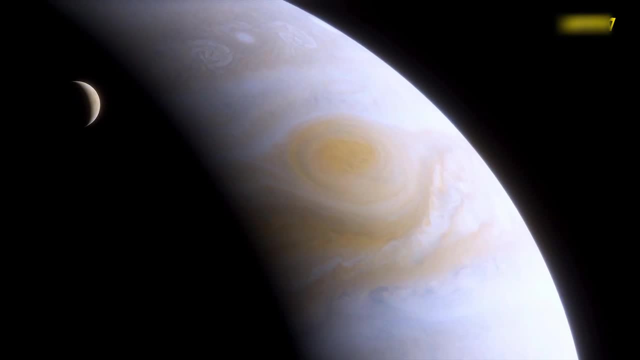 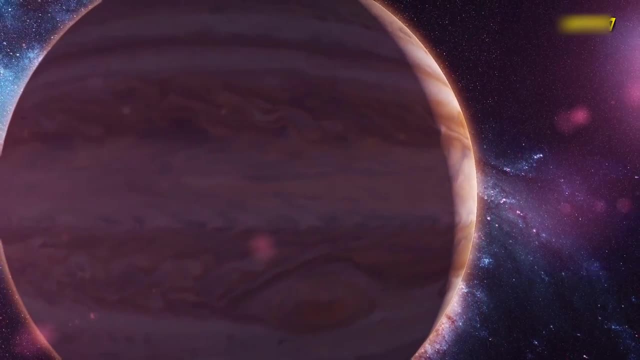 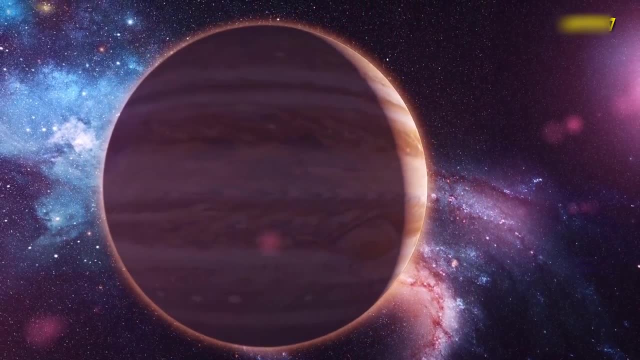 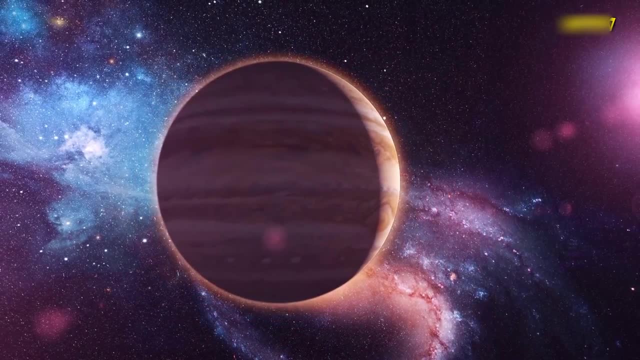 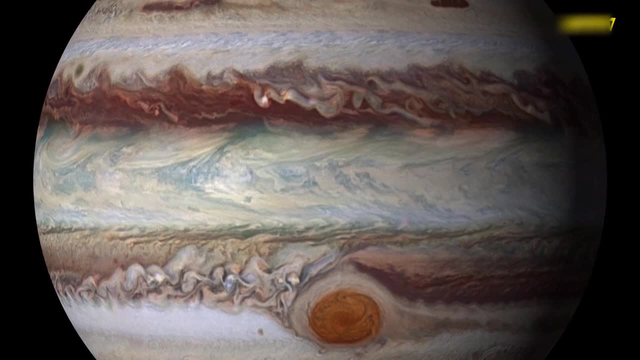 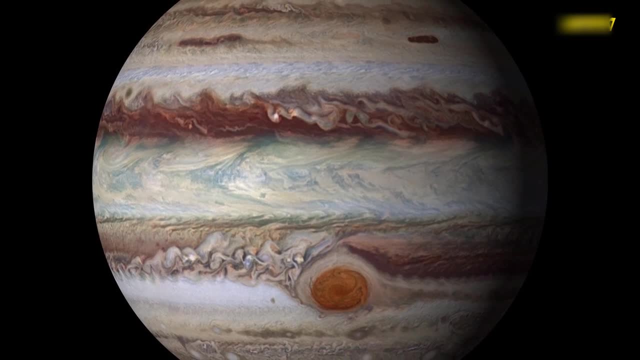 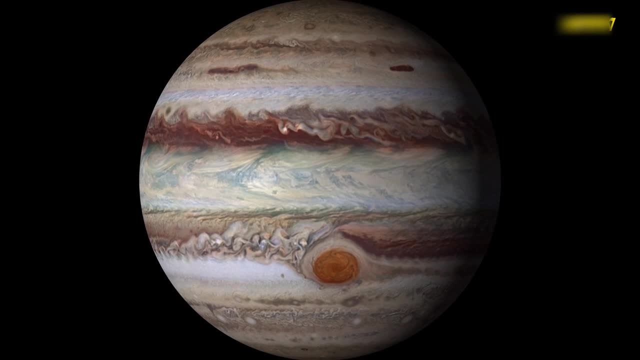 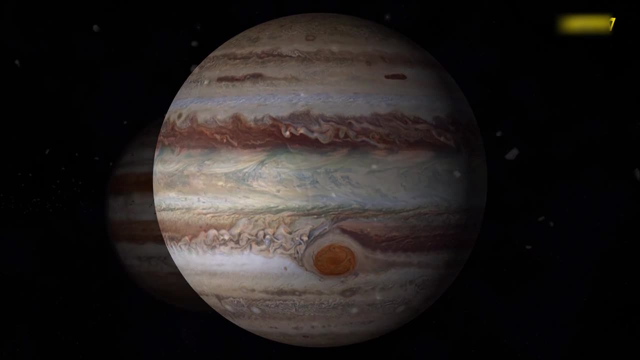 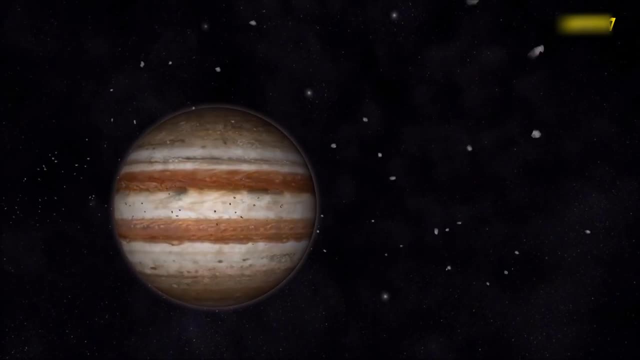 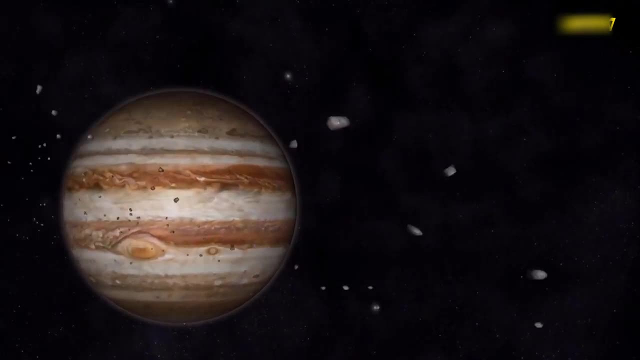 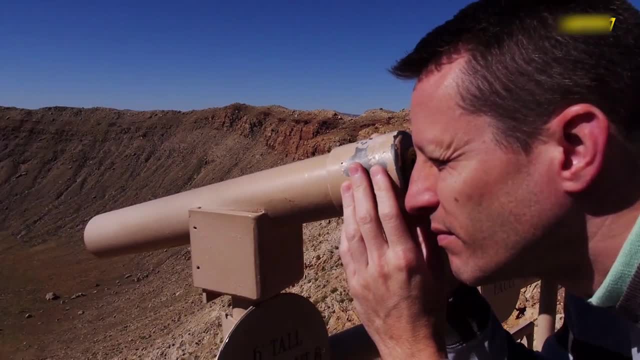 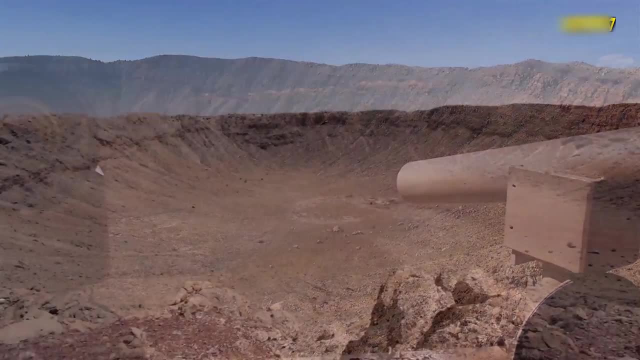 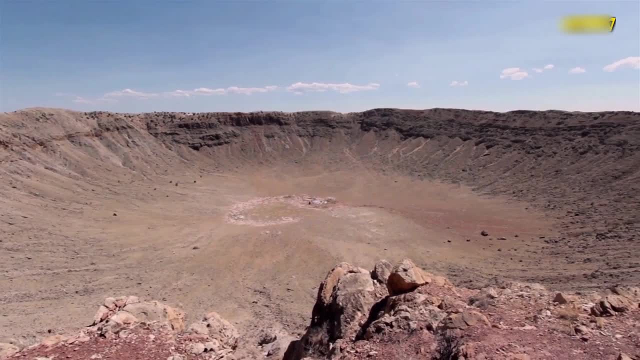 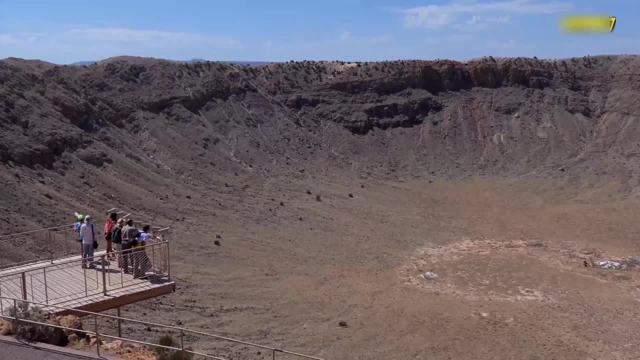 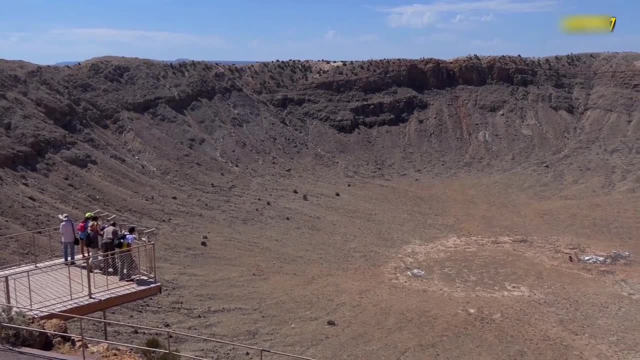 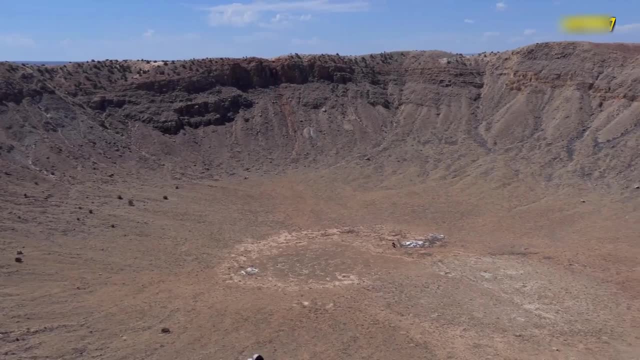 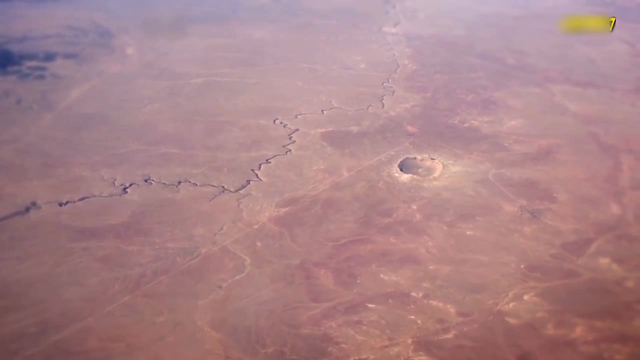 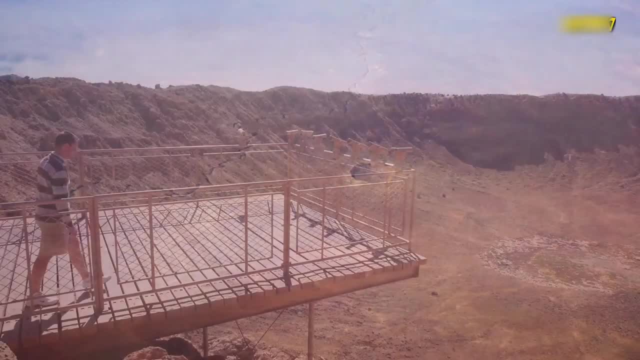 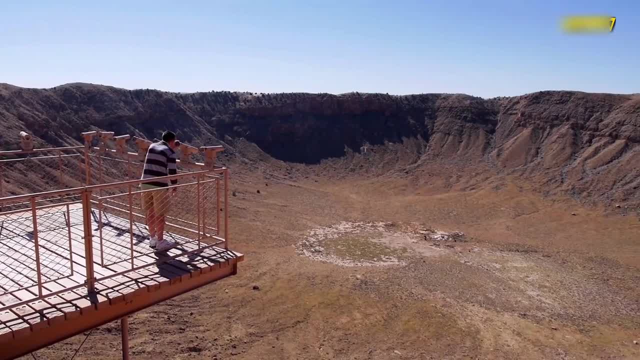 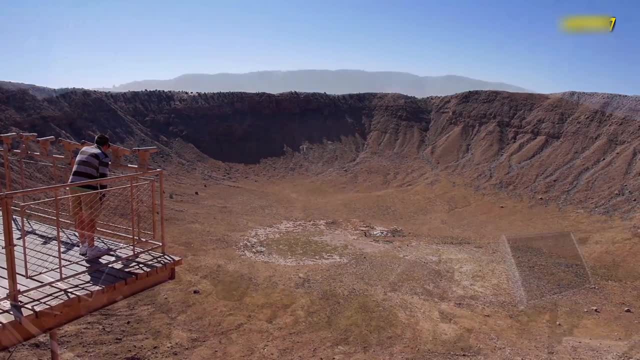 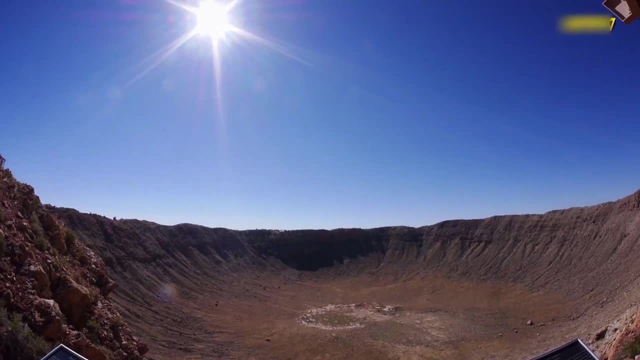 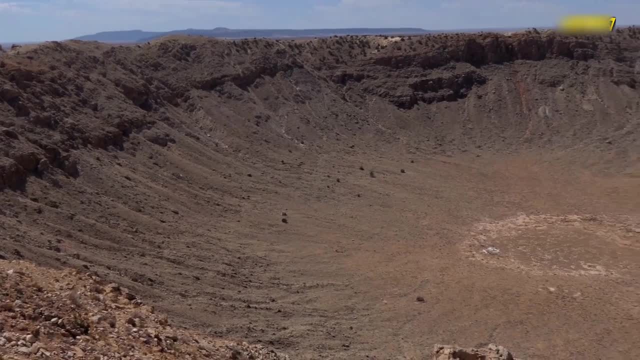 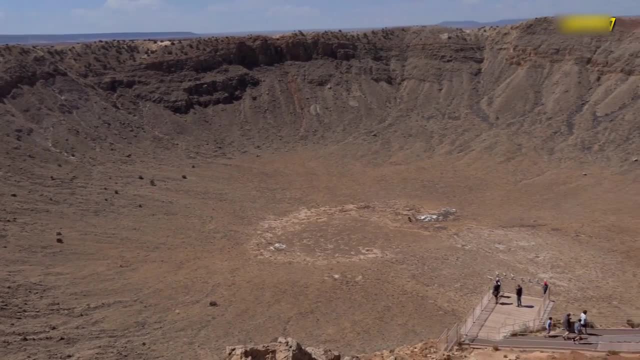 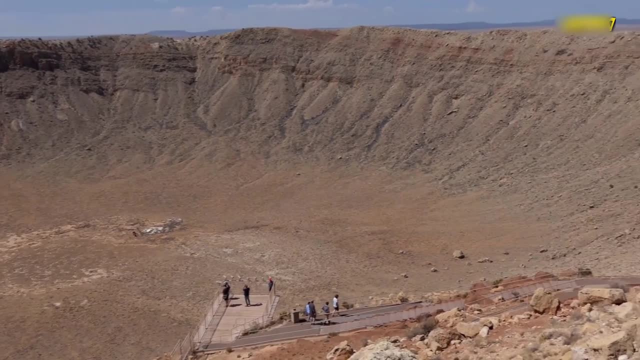 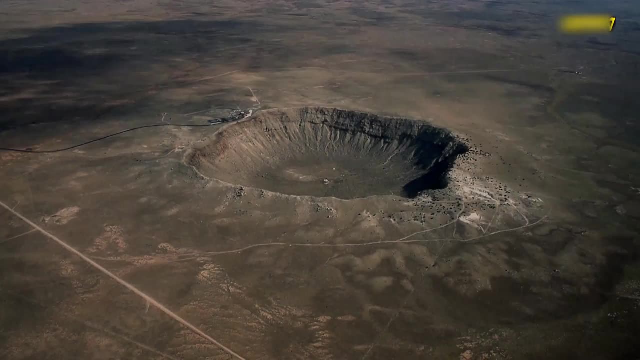 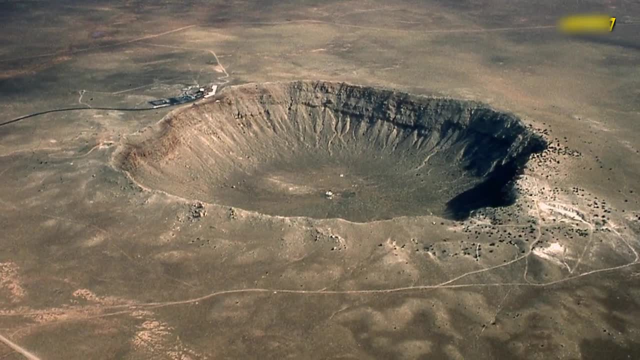 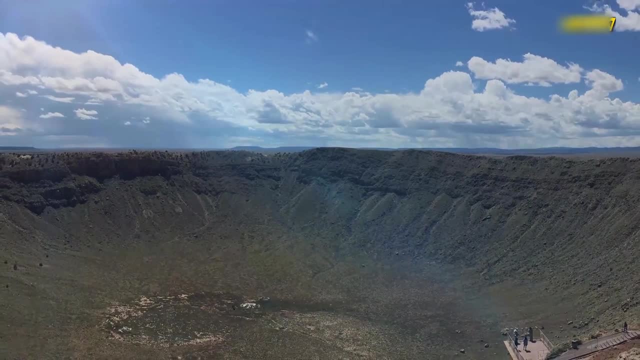 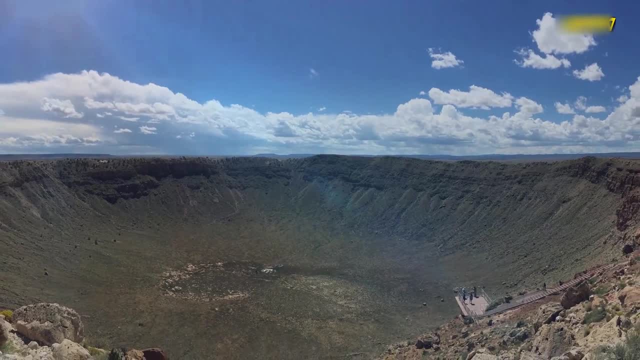 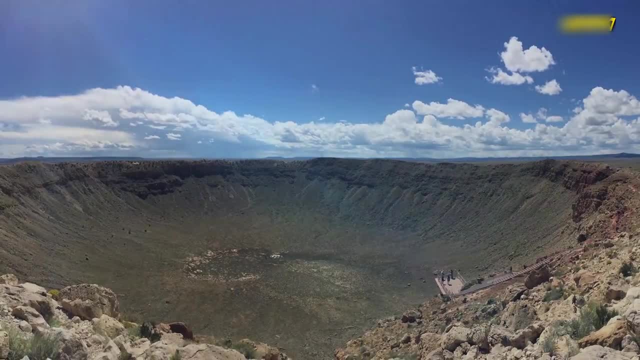 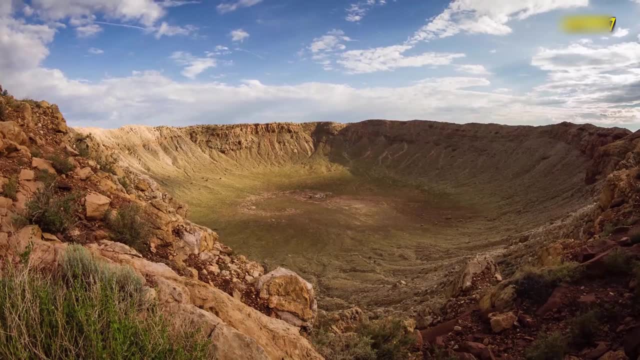 As for Pluto, despite the best efforts of complaint and protest around the world. As for Pluto, despite the best efforts of complaint and protest around the world, in the gaps launched on the 27th of september 2007, the dawn space probe took off from cape canaveral. 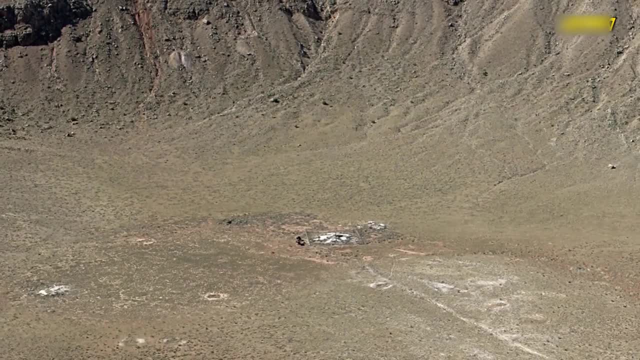 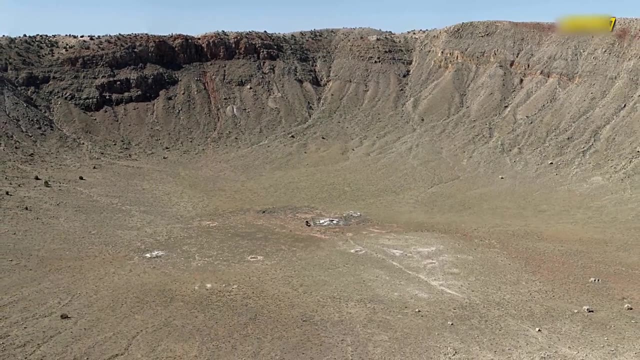 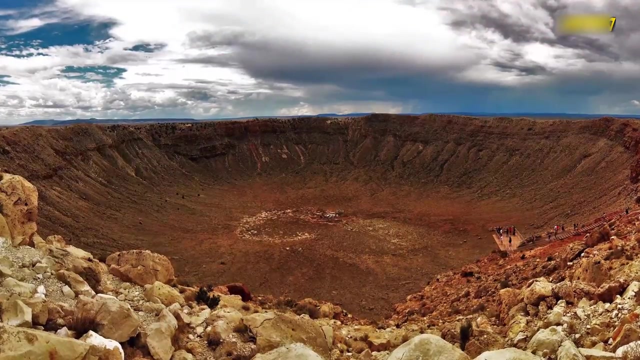 on a mission to explore the two largest objects in the asteroid belt sports car. but when it comes to efficiency, the ion propulsion system is difficult to beat. powered by a 10 kilowatt solar array, dawn's engines ran for almost six years across the 11-year lifetime of the mission. 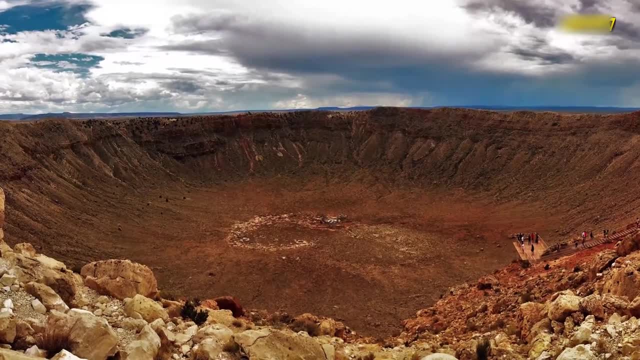 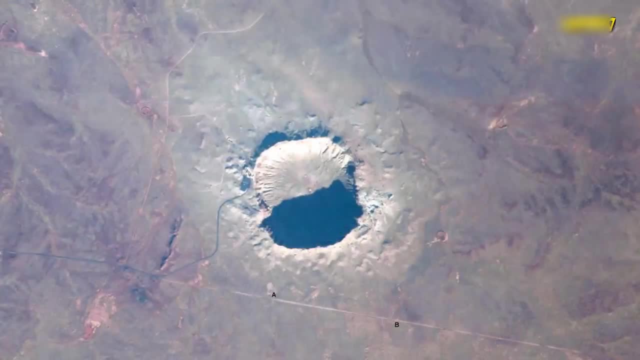 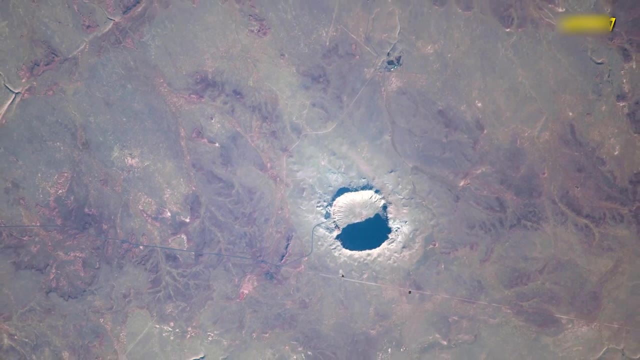 propelling the craft across space using less than 400 kilograms of its xenon fuel supply, while reaching speeds of 41 360 kilometers per hour. its trajectory took it on a 16-month journey to mars, where a gravitational kick sent it on its way out to the asteroid belt. and onwards towards vesta, its first destination, almost 500 million kilometers from the sun. the asteroid belt was the first to reach the sun. the asteroid belt was the first to reach the sun. the asteroid belt lies halfway between mars and jupiter, the boundary line between the four rocky worlds that orbit closest to the sun. 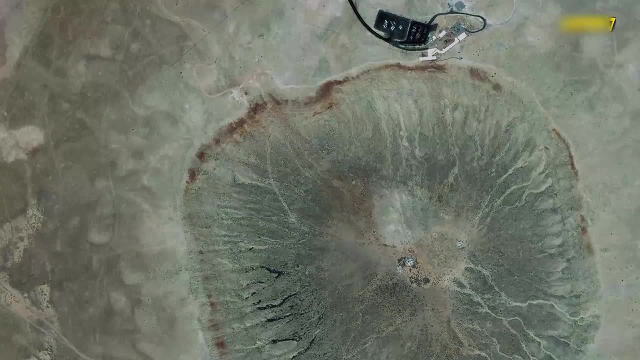 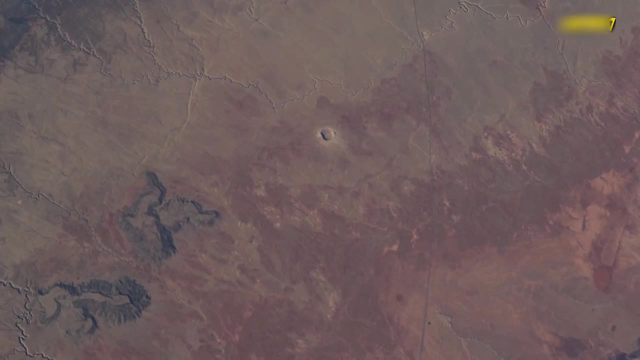 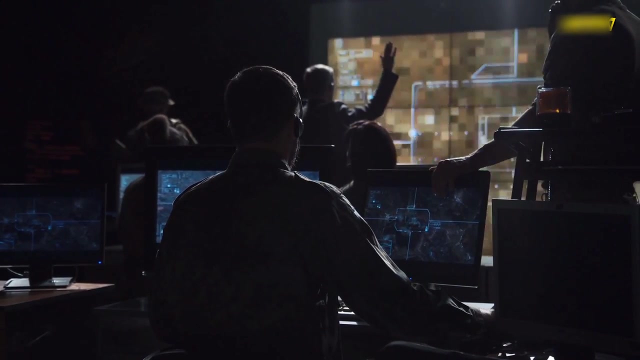 and the giant gas and ice planets that lie beyond made up of millions of pieces of rock from the dawn of the solar system. it's a graveyard of failed planets, remnants from the heyday of planetary construction. we often imagine the asteroid belt to be a dense, unnavigable mass of tumbling rock, but in reality 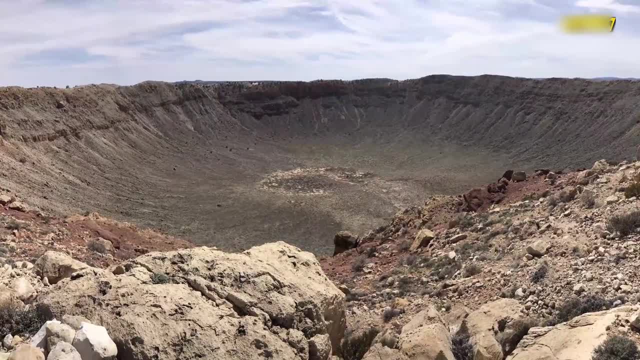 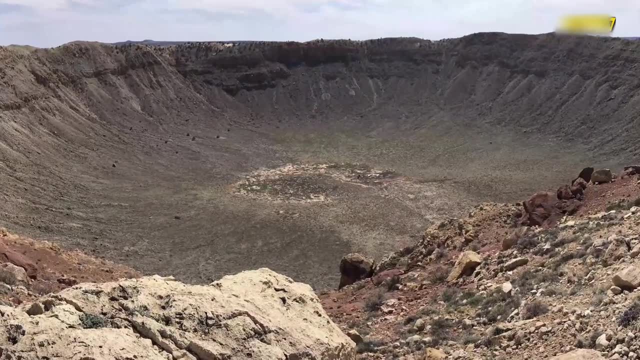 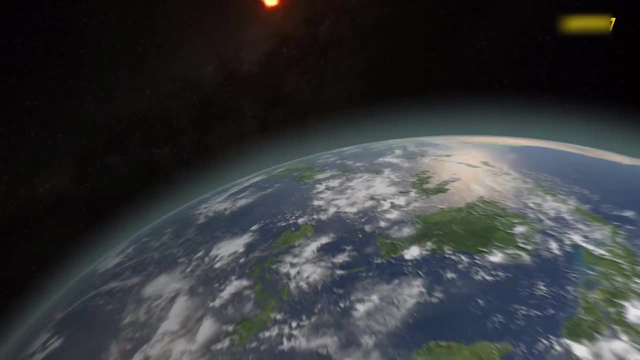 it's something quite different. the total mass of all those rocks is estimated to be three times ten to the power of 21 kilograms, which, although an enormous sounding number, is just four percent of the mass of our moon, with a third of that mass found just in the largest object series. 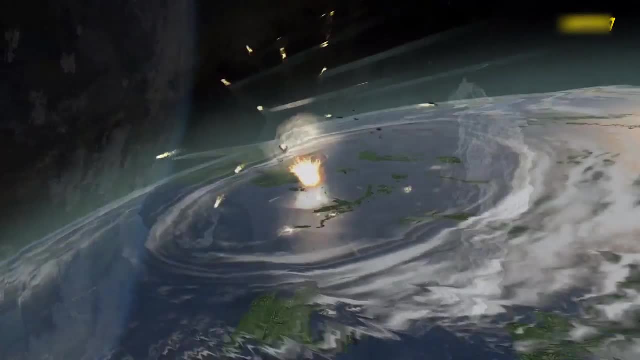 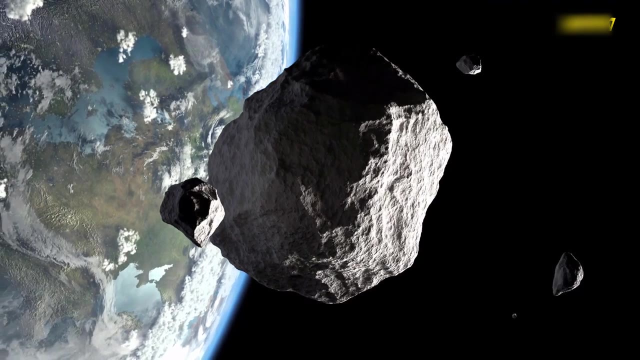 the rest of this cosmic junkyard is made up of objects covering a vast range of different sizes. on one end of the scale, we think there are at least a couple of hundred asteroids larger than 100 kilometers in size. then come a million or so stretching to at least one kilometer or more. 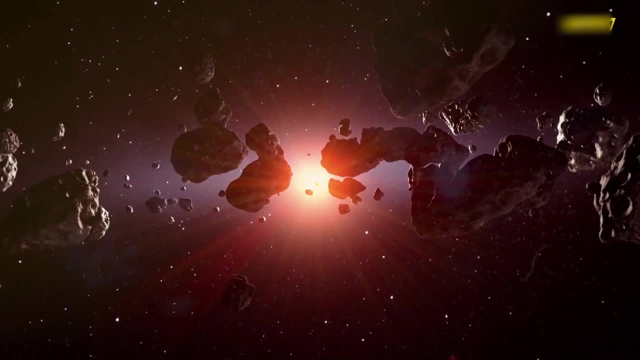 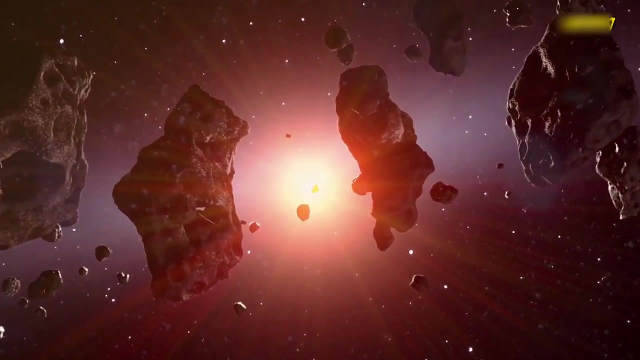 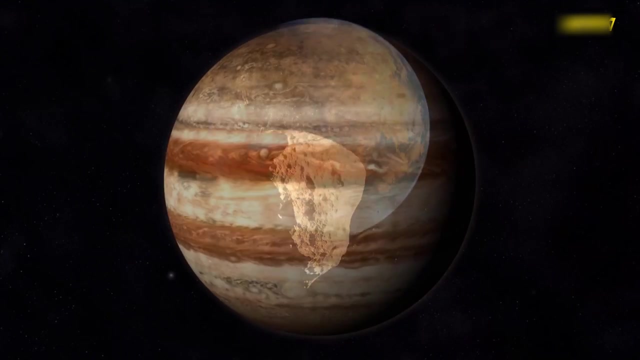 and a countless spread of smaller objects number in the millions and billions, depending on how small you want to go. all of this sounds like it should make for a crowded environment full of collisions, the perfect location to form the basis of a computer game or disaster movie. but even with that many objects, the space they occupy is so unimaginably vast. 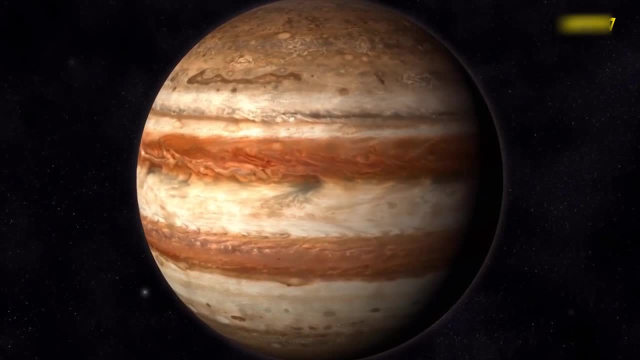 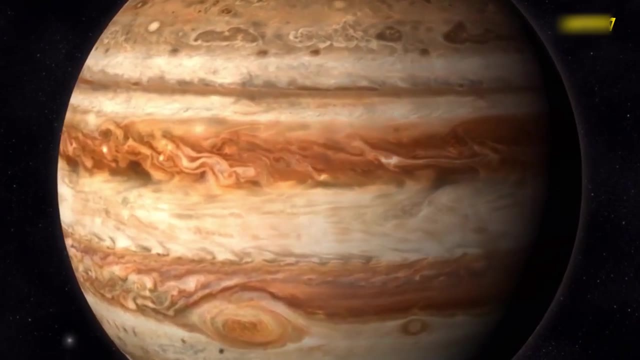 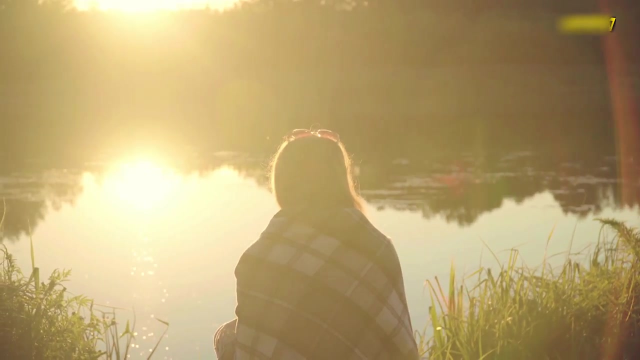 spread out across 13 trillion trillion cubic miles of space, making the average distance between any two large asteroids approximately two million miles, or eight times the distance from the earth to the moon. these distances are so large that when we send spacecraft to the outer solar system, the chances of hitting anything are so small that the engineers don't need to make any course corrections to pass through. 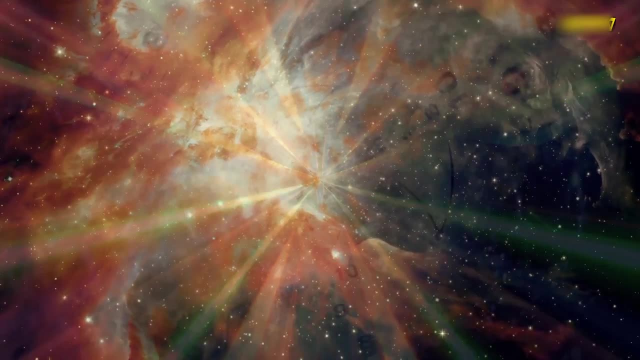 in fact, if you were standing on an asteroid, you'd be lucky to see another one, and if you did, it would appear as little more than a tiny point of light in the darkness. as it turns out, it's not just a tiny point of light, it's a tiny point of light. 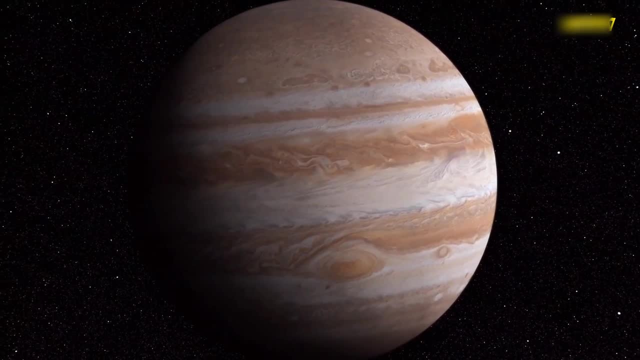 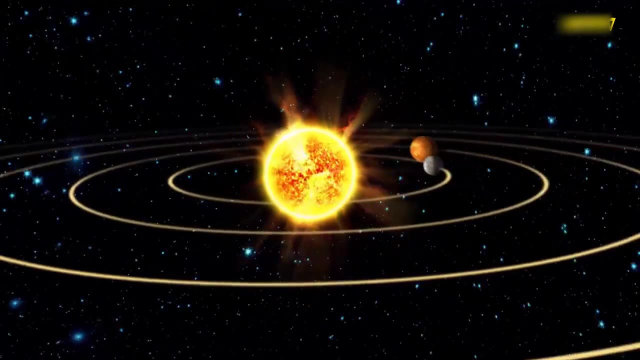 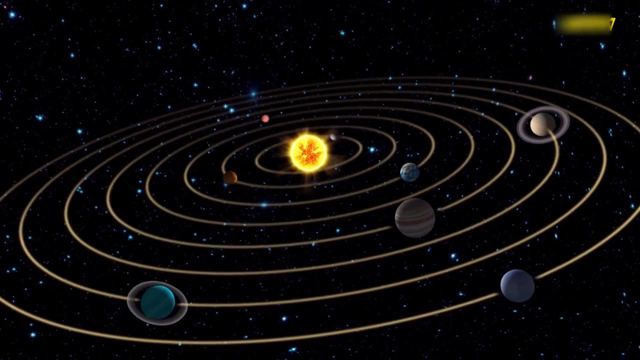 when we traveled through this vast emptiness in the early summer of 2011, the dawn spacecraft slowly began to bring its first target into view from a distance of over 1.2 million kilometers. dawn took its first photograph of vesta against the backdrop of a thousand stars. 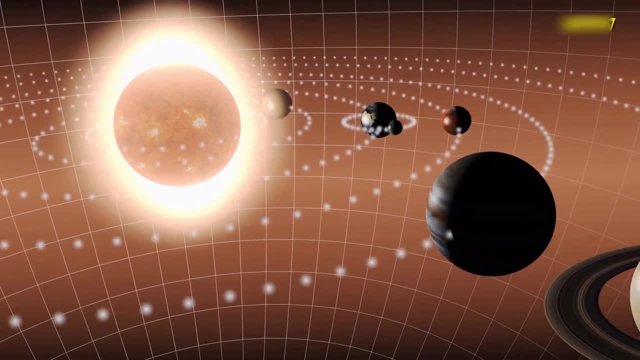 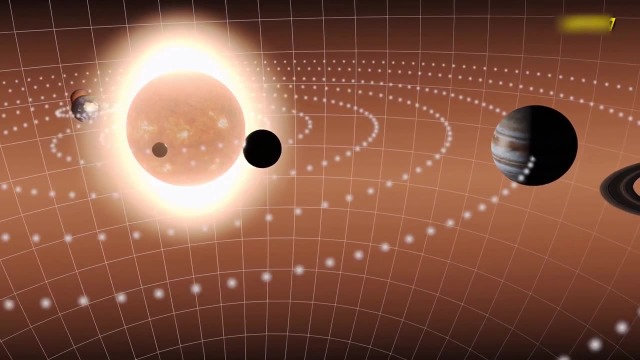 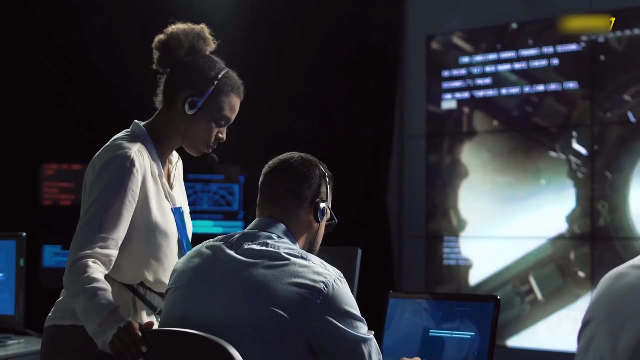 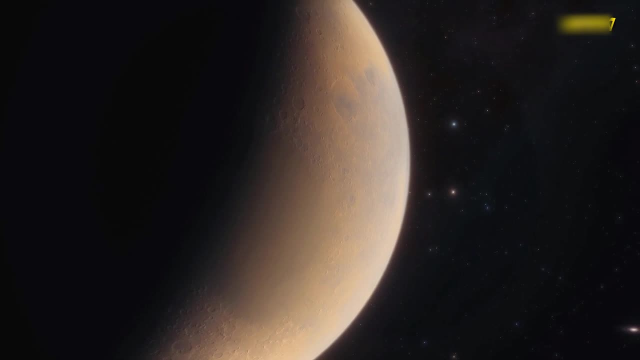 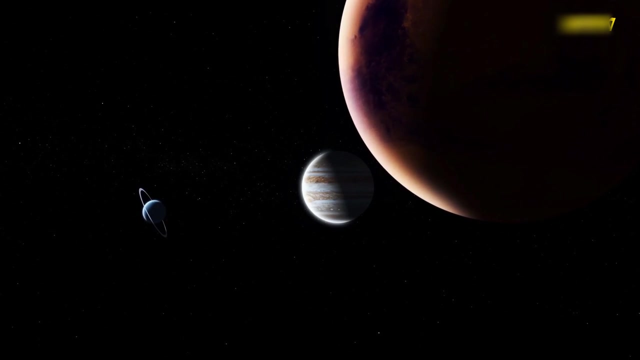 to date the formation of the asteroid to a couple of million years after the first solid objects began to take shape in the solar system. These are just two of the clues that point us to an extraordinary conclusion. Vesta is perhaps the last remaining example of a protoplanet. 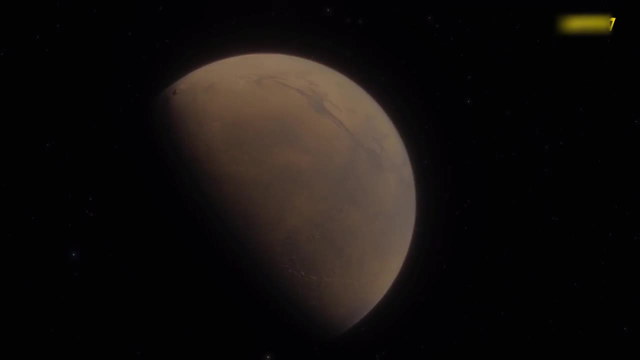 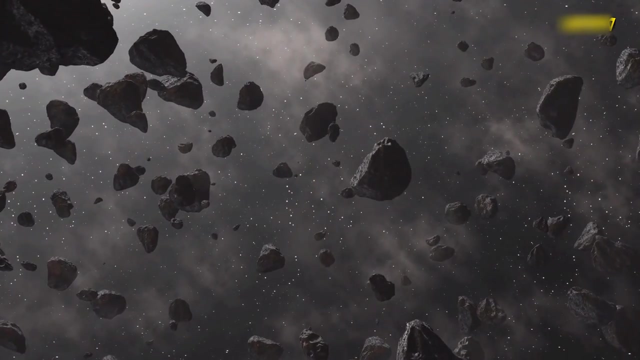 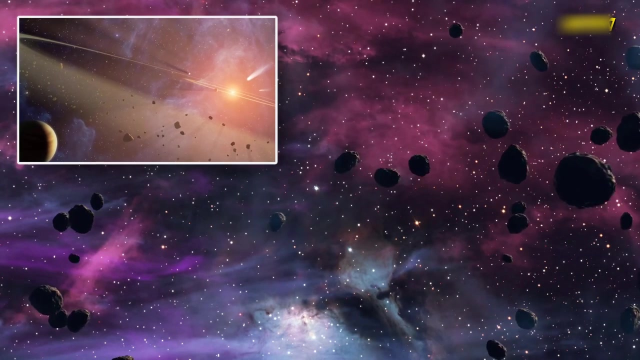 a half-formed world from the very earliest days of the solar system, Frozen in time. this is a stage that every world we know of passed through, including the Earth. Vesta was on the way to becoming a planet almost 4.5 billion years ago. 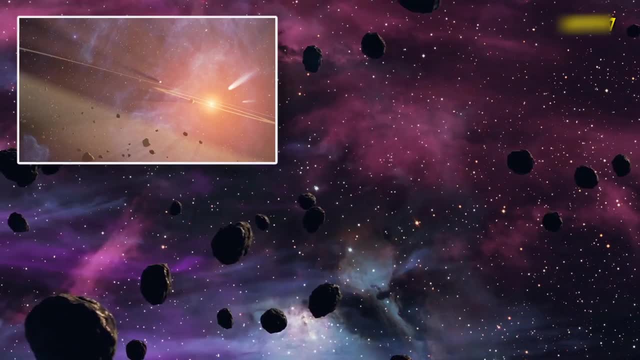 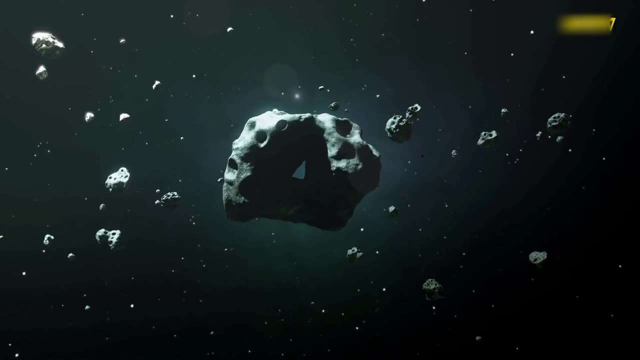 but something happened to stop its progress. While other worlds went on to flourish and other protoplanets disintegrated in the violent collisions of the early solar system, Vesta somehow seemed to survive, a fossil of planetary formation for us to not only look at. but, through a quirk of fate, actually hold. But this was not the end of Dawn's dive into our deep history. Departing Vesta after 14 months of study, Dawn fired its ion drive, leaving the orbit and heading off for its second planetoid rendezvous at the largest of all the asteroids, Ceres. 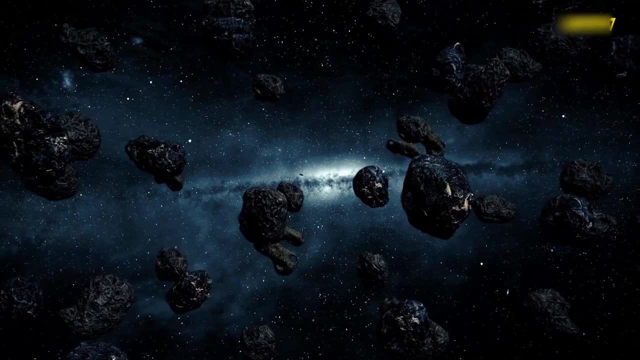 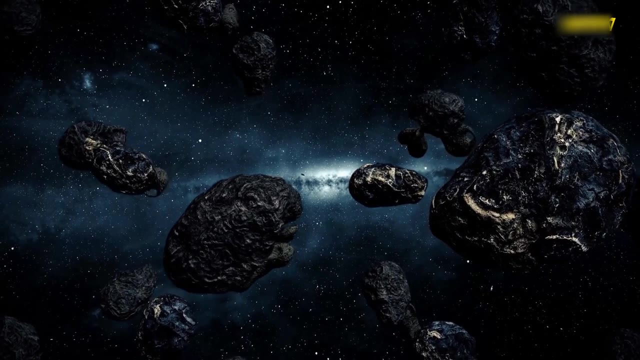 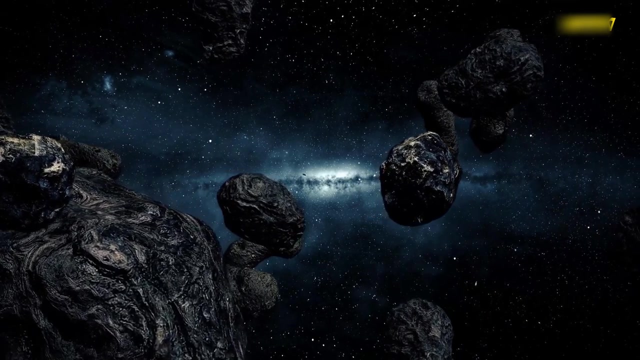 Dawn arrived at the dwarf planet Ceres in early March 2015, and from the very first moments of its observations, it sent back some astonishing images. Very little was known about Ceres before our spaceship arrived, but it soon became clear that this was a rock with far more of a story to 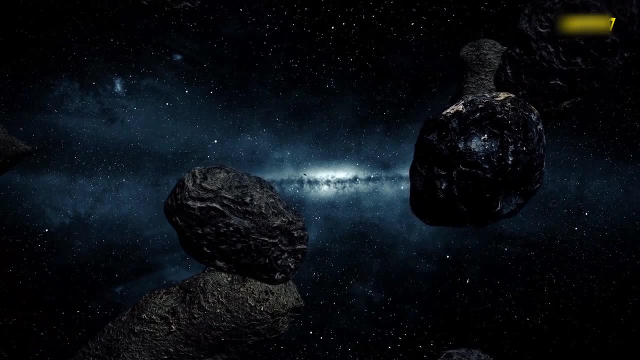 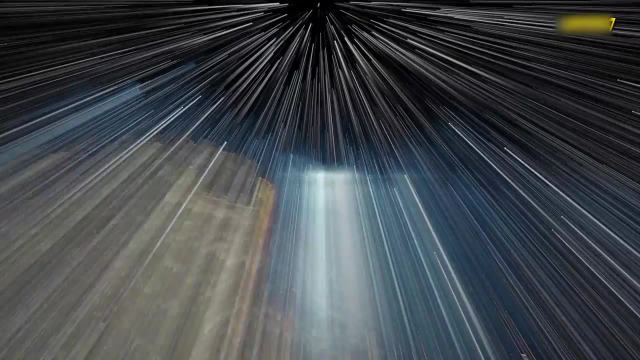 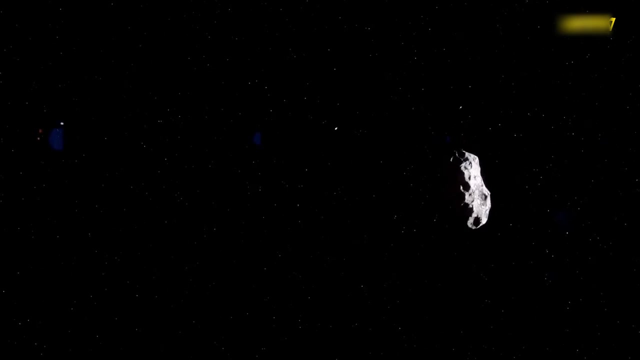 tell than we could ever have imagined, A story that would help reveal a new perspective on the deep history of our solar system and the enormous influence Jupiter has exerted over it. The Italian astronomer Giuseppe Piazzi discovered Ceres on the 1st of January 1801, and at first he 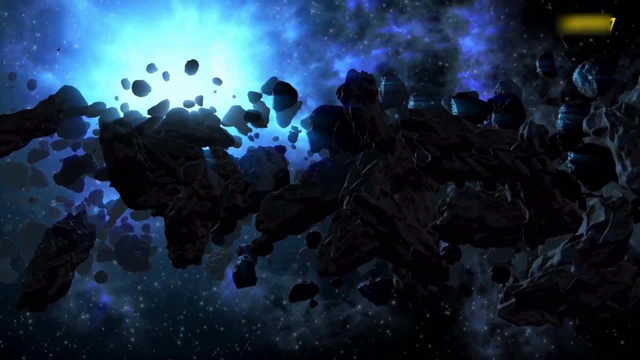 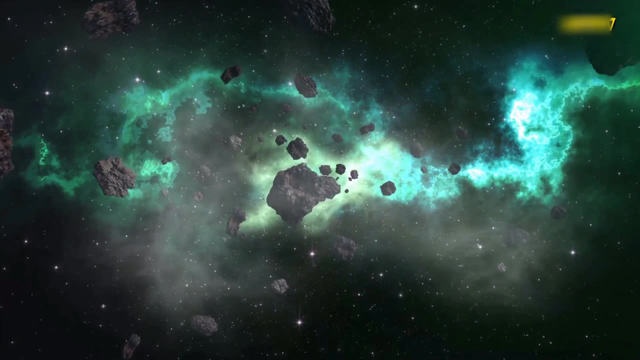 reported his findings as the discovery of a new comet in the region of space between Mars and Jupiter, But it seems from the start that all of his instincts told him this was something else. In announcing his observations in a letter to two fellow astronomers, he noted that, since its 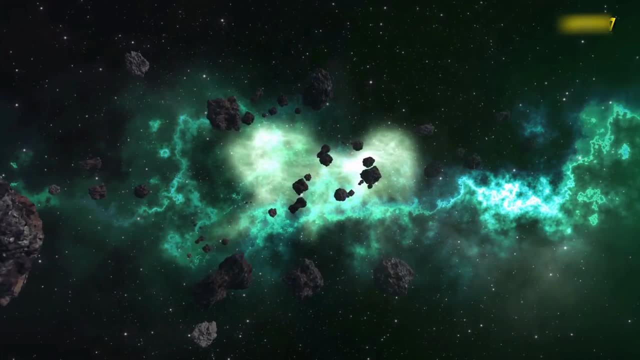 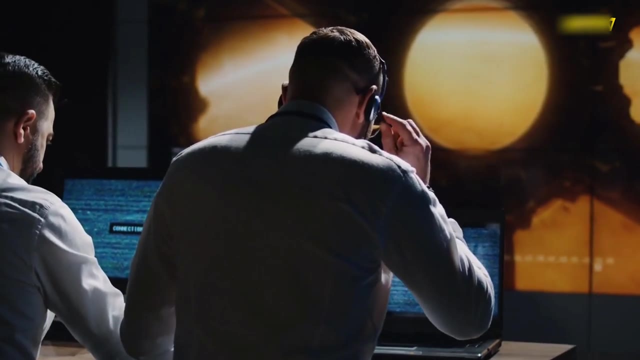 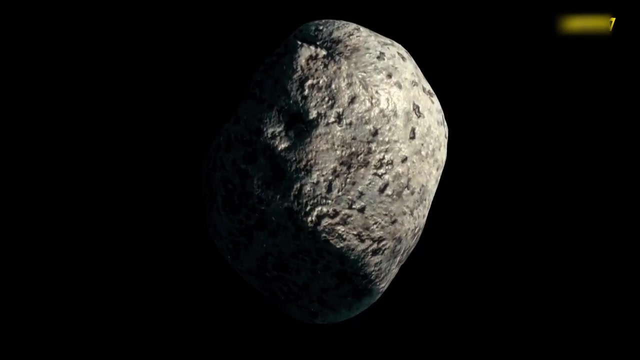 movement is so slow and rather uniform, it has occurred to me several times that it might be better than a comet. Piazzi and his colleagues speculated that rather than a comet they might have found something even more spectacular, a new planet, But after just 41 days of observation. 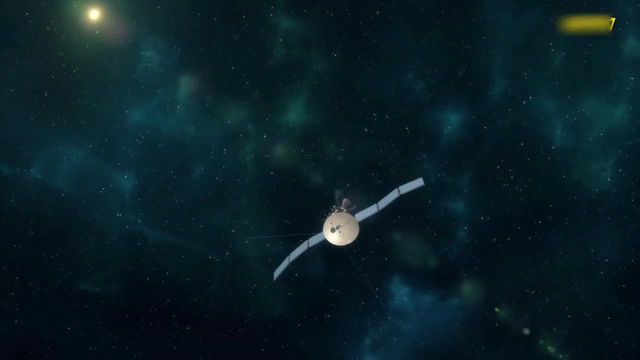 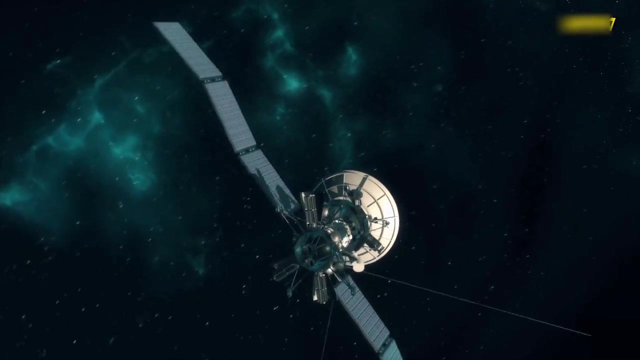 Piazzi, fell ill. the path of the newly discovered object strayed into the direct glare of the sun and, in a twist of high astronomical drama, the newly found planet Ceres was lost. With just a tiny number of objects, the new planet Ceres was lost. 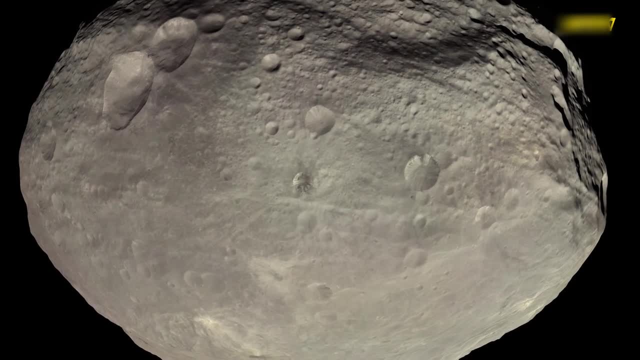 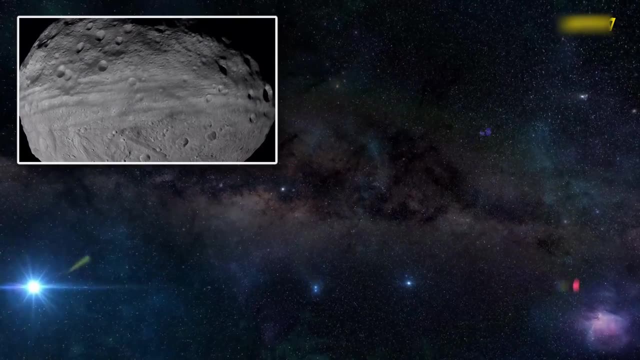 With just a number of observations across a small piece of sky. calculating Ceres' orbit was deemed impossible using the mathematics of the time, and many contemporary great mathematical minds predicted it might never be found again. It would take the work of a young German mathematician. Friedrich Gauss to solve the problem. Attracted to the difficulty and elegance of using mathematics to compute the orbit from just a few coordinates, Gauss pioneered a novel mathematical method that allowed him to calculate the path of Ceres using just three of Piazzi's original observations. On the very last day of 1801,, two astronomers, using Gauss' methods, searched the region of the sky to which the calculations guided them and, to everyone's delight and relief, recovered Ceres from the darkness. Gauss became a mathematical superstar, and Ceres firmly back in our sights. was stamped with the classification of a planet. For the next 50 years, Ceres and its companions Vesta, Pallas and Juno remained listed as planets until, as we have seen, the discovery of a raft of other objects in this region of space gave rise. 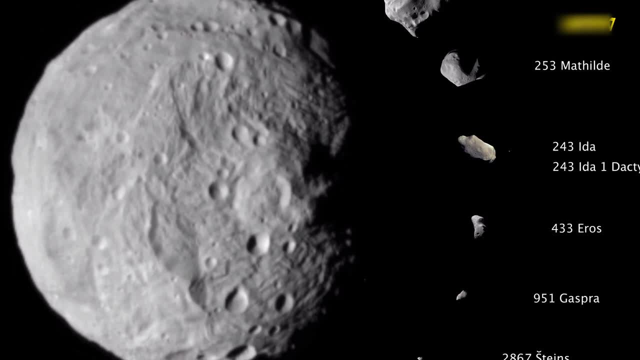 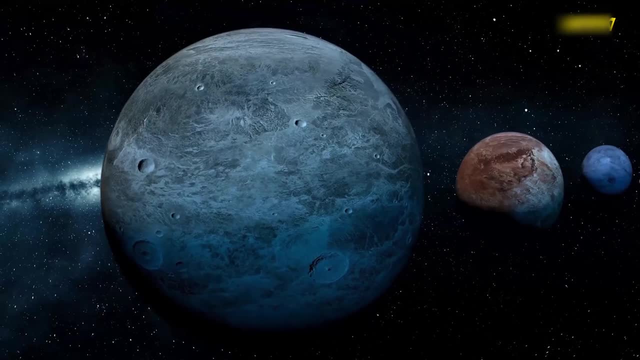 to our identification of the asteroid belt, and for Ceres it was downhill from there on. until in 2006, it was classified as a dwarf planet For the next 160 years. little was known about this tiny planet orbiting the sun at a distance of 113 million kilometers. We knew that it was the biggest object in the asteroid belt and the only object amongst the millions of asteroids that was large enough to have been rounded by its own gravity. We could also make a good approximation of its size at around 1,000. 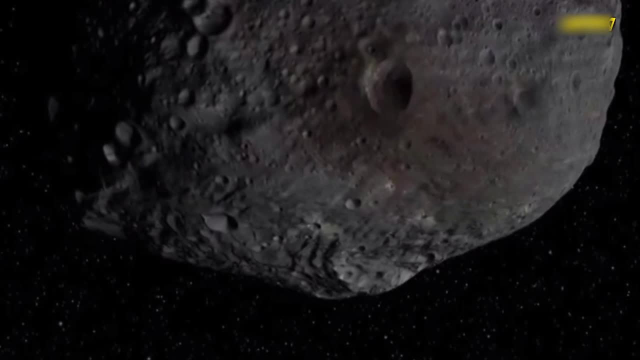 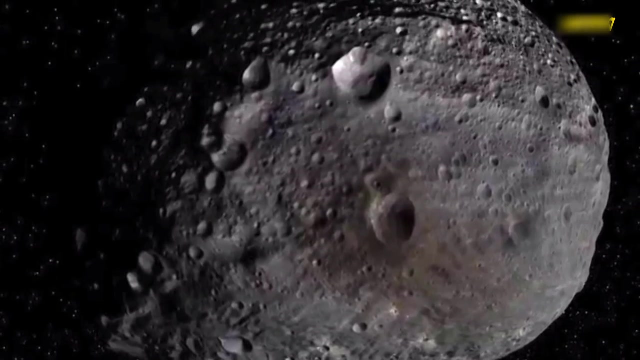 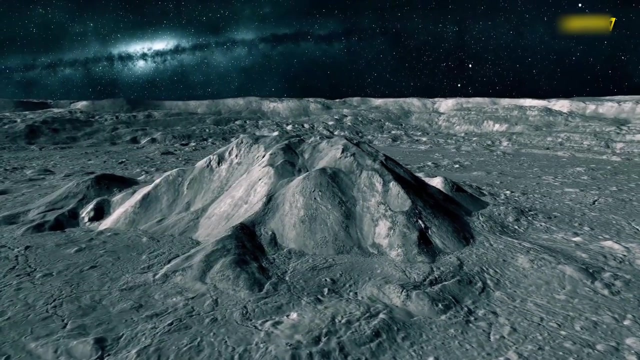 kilometers in diameter, and composition: rock and ice- what else? But when it came to surface features, even the powerful eye of the Hubble Space Telescope could make out only the vaguest of features intriguingly strewn across its surface. It would take Dawn's arrival for us to truly understand the complexity of this world and its 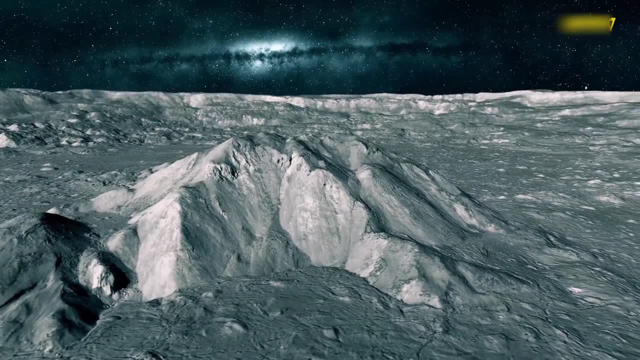 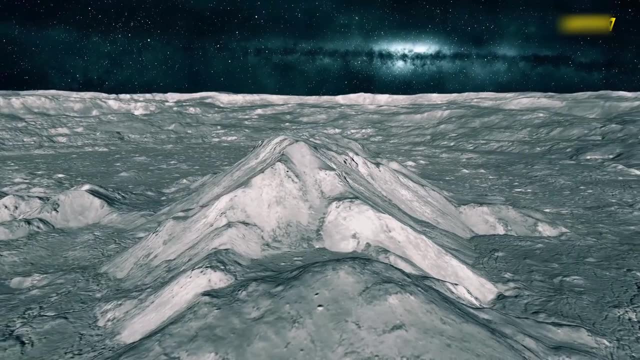 history. Even in the early approach phase of the mission, Dawn was able to capture a quality of imagery that at once gave a new perspective on the long hidden surface. It was no surprise to find it heavily cratered, but while speeding towards Ceres, Dawn beamed back a series of 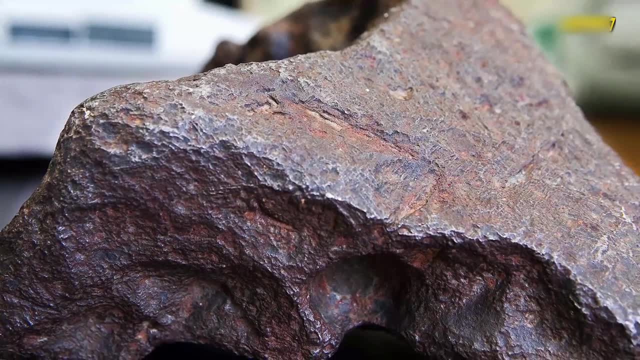 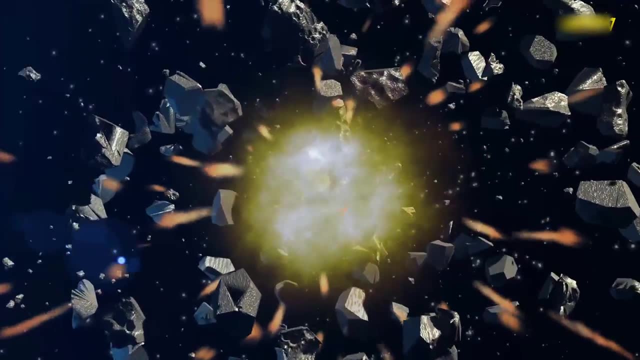 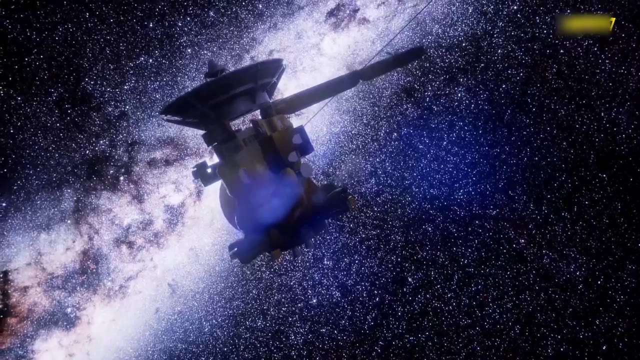 mysterious images revealing a number of bright spots on the surface of what we had thought would be a dull, dead and frozen world- Not what you would expect on a planet that was assumed to be entirely geologically inactive. The brightest of all of these highly reflective areas was imaged near a massive crater known as 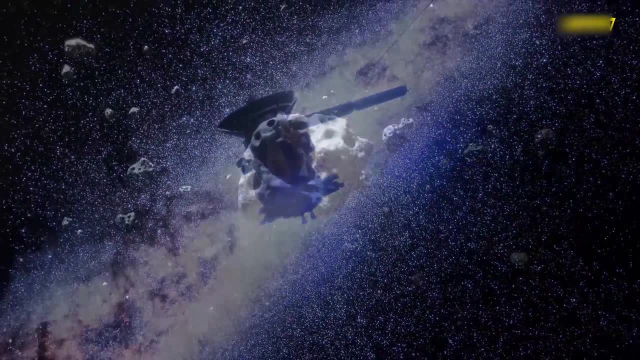 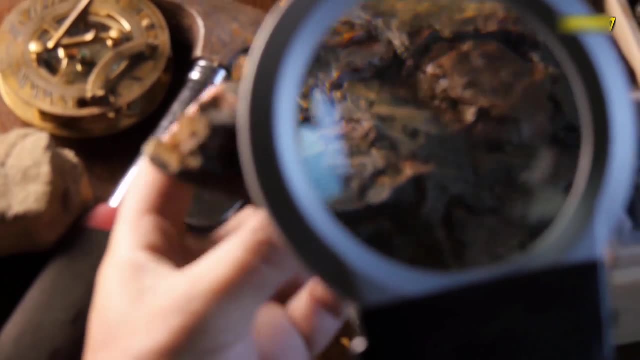 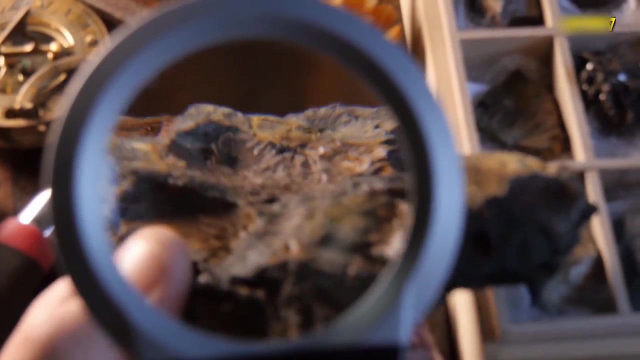 Arcata. At 92 kilometers wide and 2 kilometers deep. it's one of the biggest on the surface of Ceres. Spot 5,, as it became known, is in the center of the crater and became the focus of intense investigation as Dawn began its three-and-a-half-year residency in orbit around it. 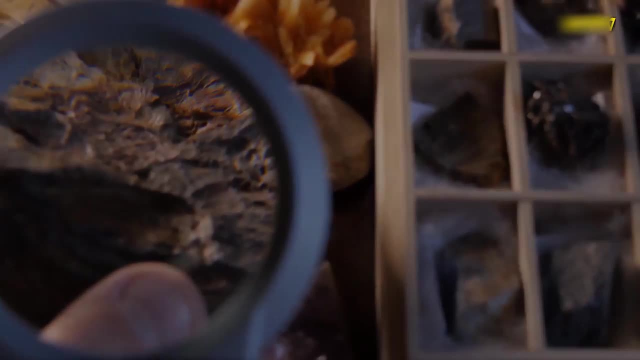 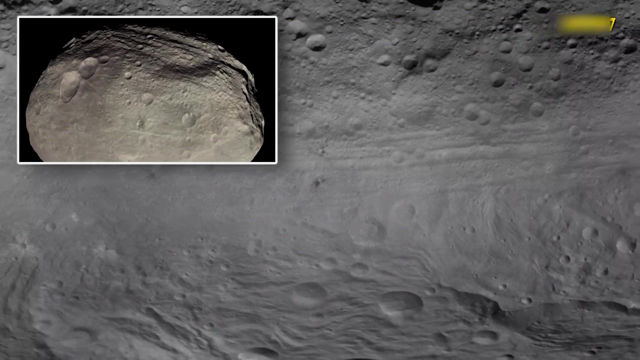 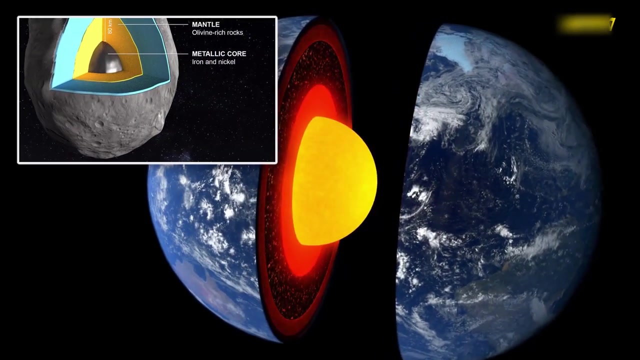 The crater is thought to have formed from a large-scale impact around 80 million years ago, and so the presence of what appeared to be geological active material on the surface was particularly surprising and at first left the mission scientists perplexed. Not only that, but a haze was also seen to periodically appear above Spot 5,. 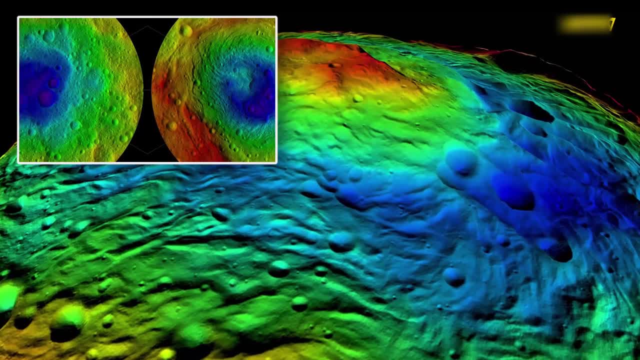 suggesting something was going on beneath the surface. After detailed analysis using Dawn's data, we were able to find out that the crater was not in the center of the crater and that it was in the center of the crater itself. With Dawn's full range of imaging and spectroscopic capabilities. 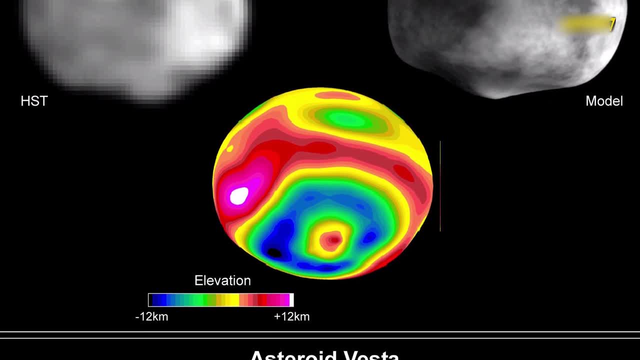 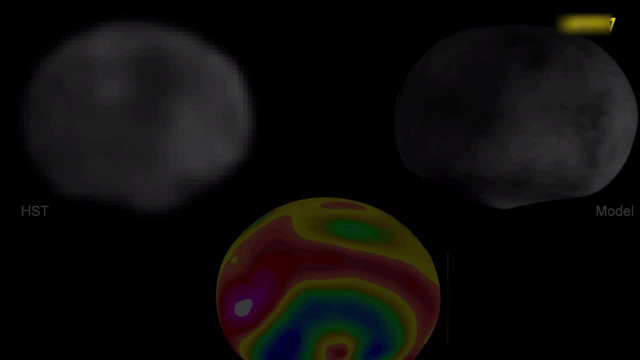 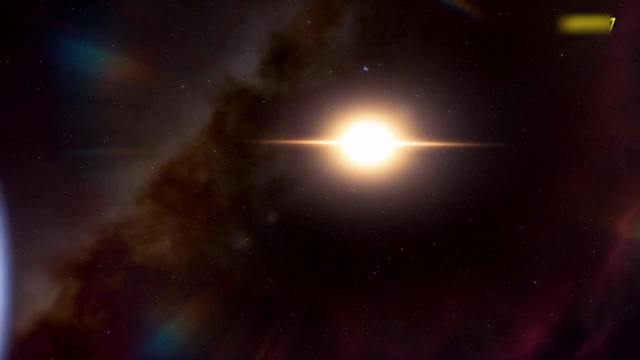 we now believe that Spot 5 is the result of a geological hotspot: the brightness created by the highest concentration of carbonate minerals ever found outside the Earth, in a dome structure right in the center of the crater. Why does this matter? Well, we know that this type of salt can only be formed in the presence 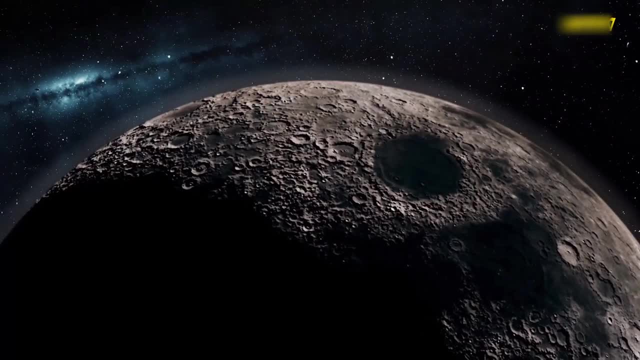 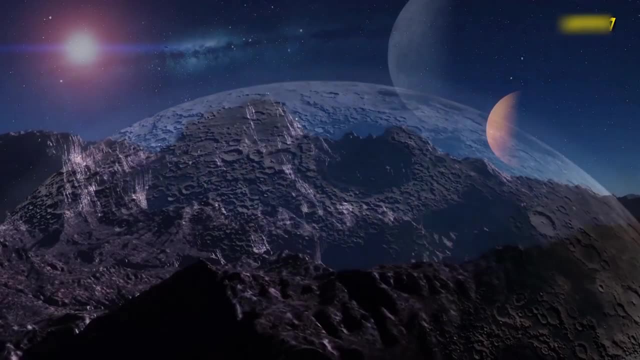 of liquid water, and it's almost certain that an impacting asteroid can only be formed in the center of the crater. The asteroid could not have delivered such material to the surface of Ceres, so the upwelling in which it's found suggests that it comes from deep within this world. 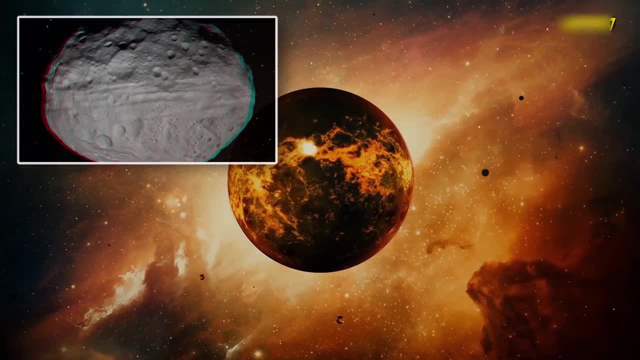 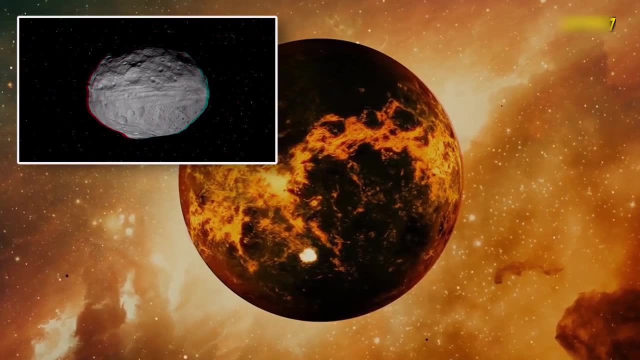 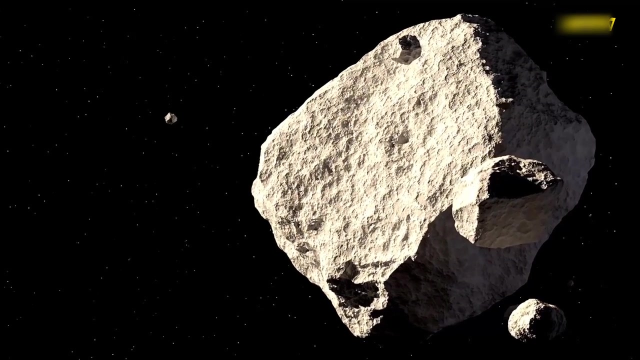 It now seems that Spot 5 is the remains of an ice volcano, one that is perhaps still partially active and thus able to create the haze we have observed. The two brightly colored patches inside it are thought to be the salty residue left by this. 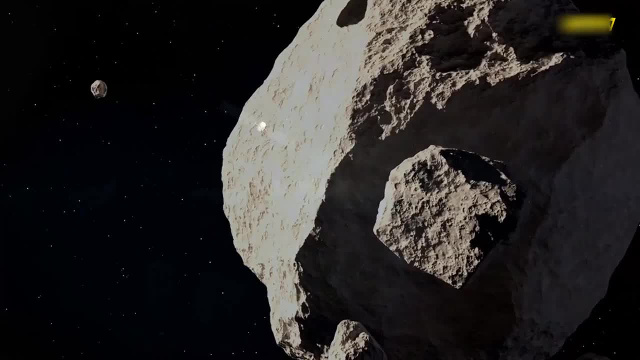 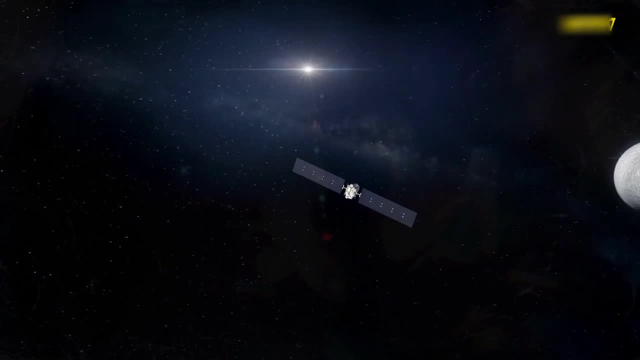 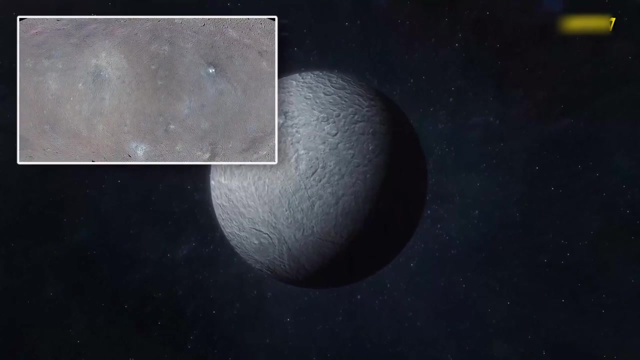 ancient formation Deposits of sodium carbonate from an erupting ice volcano that may have first been triggered by the impact that created the crater. However, the dome-like shape upon which the deposits sit is almost certainly evidence of geological activity below the surface, suggesting that. 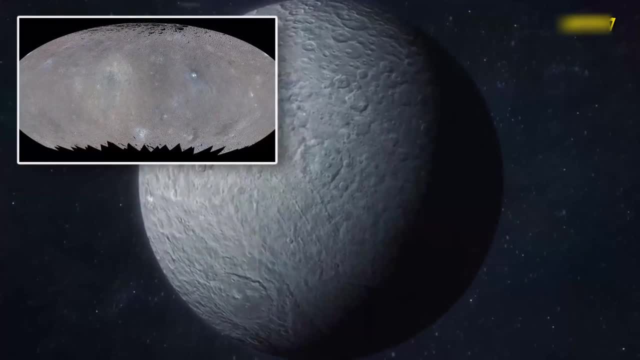 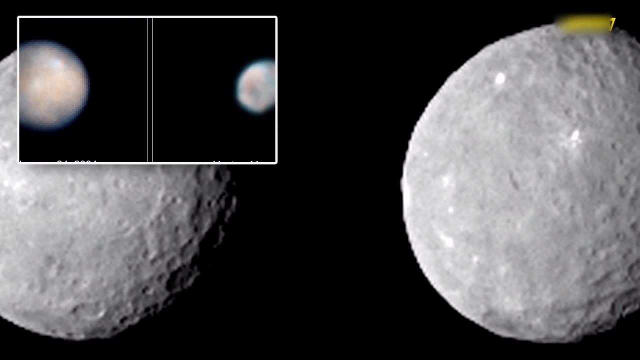 hydrothermal activity was involved in bringing the salts to the surface, And Spot 5 is far from isolated. We've now seen areas like the ones in Acata all over the surface of Ceres, and this begins to paint a tantalizing picture of the surface of Ceres. 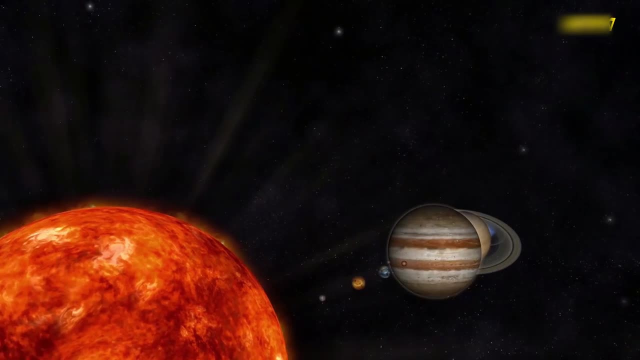 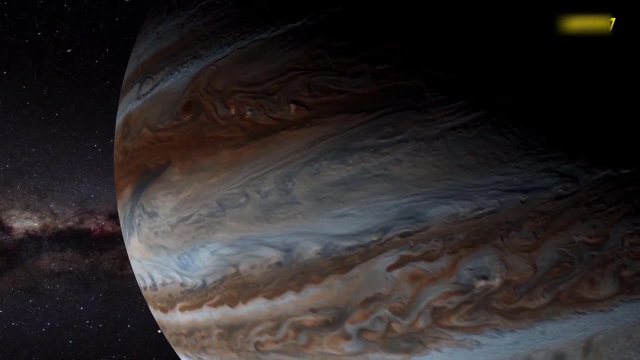 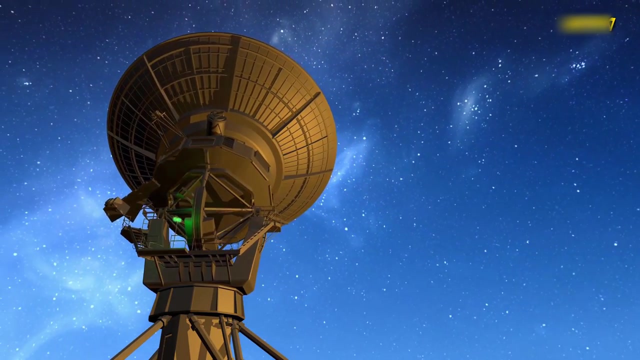 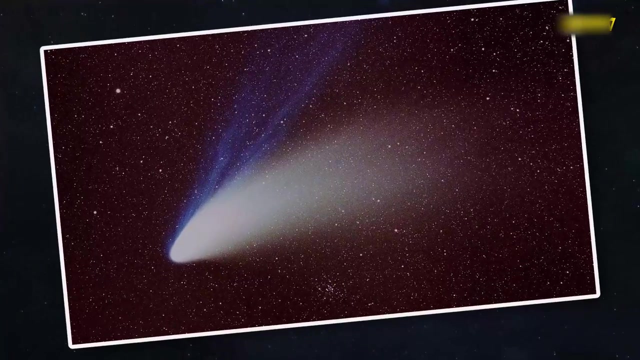 A past where heat from within the planet created a subsurface ocean, or at least localized pockets of water that surged upwards in the form of great ice volcanoes, bringing with them on the asteroid the carbonate salts that we see sparkling today As dawn delved deeper beneath the surface. the surprises kept coming thick and fast. 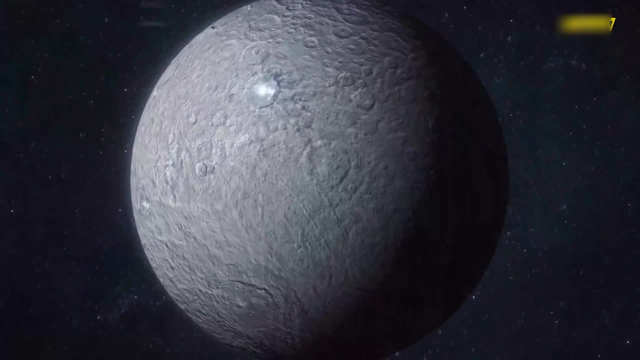 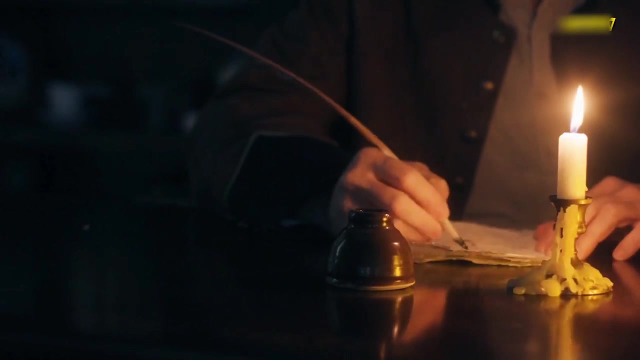 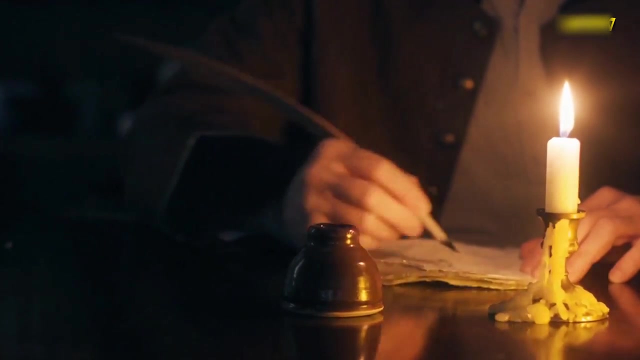 Dawn was able to accurately measure the overall density of Ceres and found it to be 2.5 times 2.16 grams per cubic centimeter, which is less than you'd expect for a rocky body. Ceres is about two-thirds the density of our moon, which suggests that, as well as rock, the asteroid must also hold. 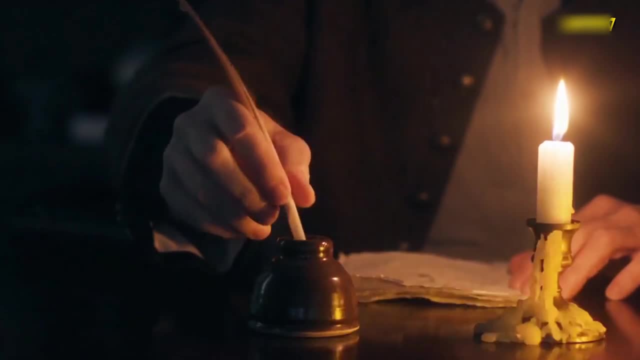 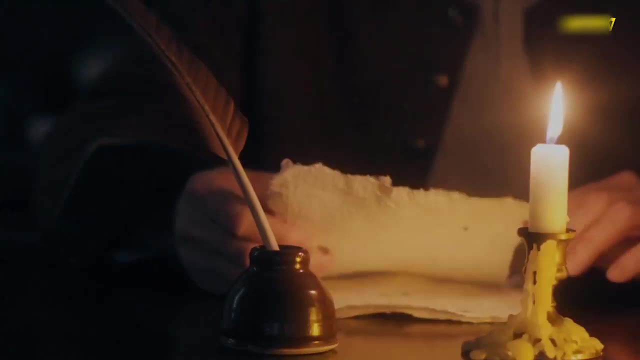 significant amounts of water ice. This had been suspected long before dawn arrived, but with our eyes and ears now at work as dawn circled, Ceres it was able to take precise measurements and so uncover anomalies in its orbit. that revealed something that was not so simple as the fact that 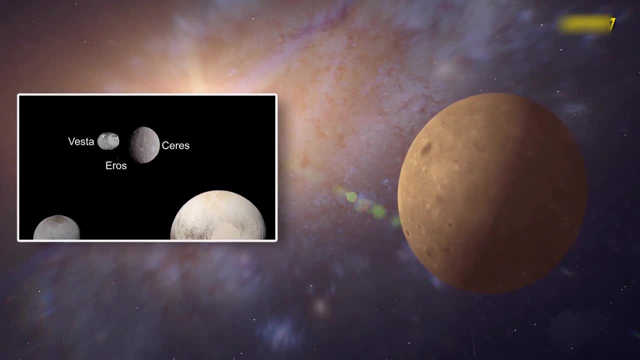 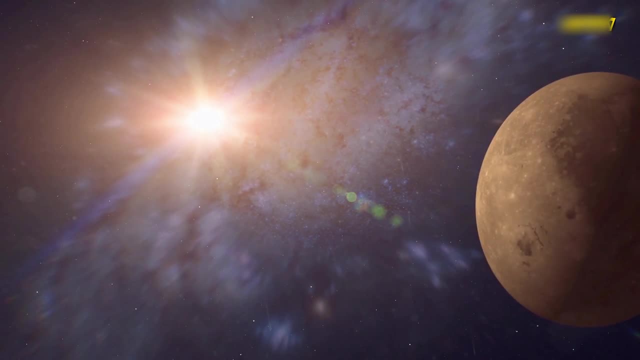 Ceres was able to take precise measurements and so uncover anomalies in its orbit that revealed something remarkable about this lump of rock and ice. By carefully mapping the shape and gravitational field, we found that the rock and ice weren't evenly distributed. It appears that Ceres' interior is nothing like that of other asteroids in the 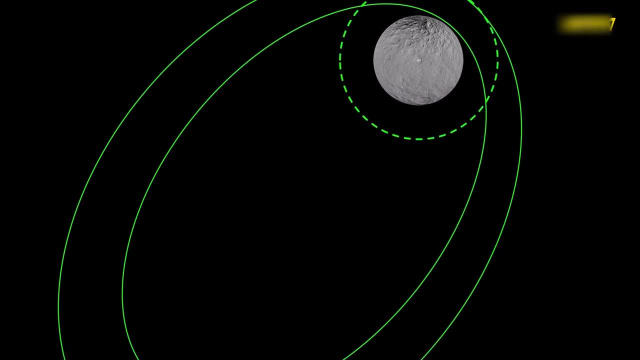 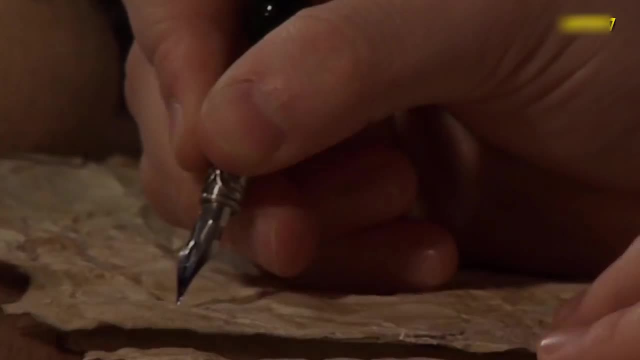 belt. Instead, it appears to have a rocky core surrounded by an ice-rich crust. This is not the jumbled structure of an asteroid. The differentiation into layers that was discovered by dawn in the discuted universe is something we only see in planets. 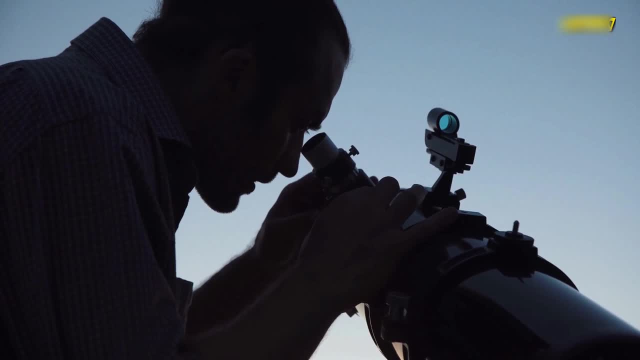 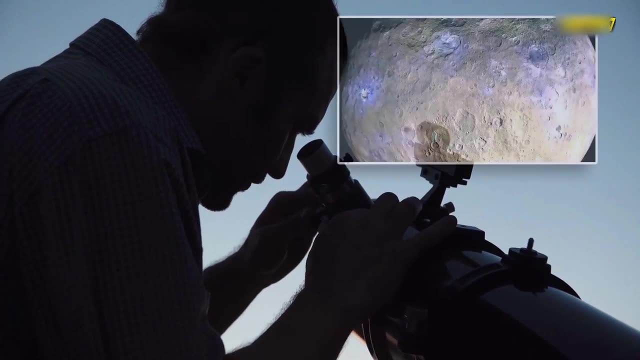 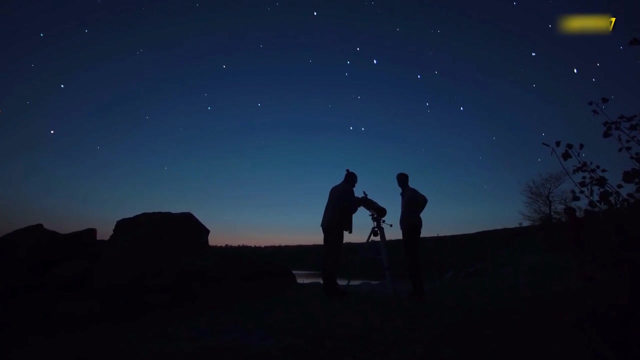 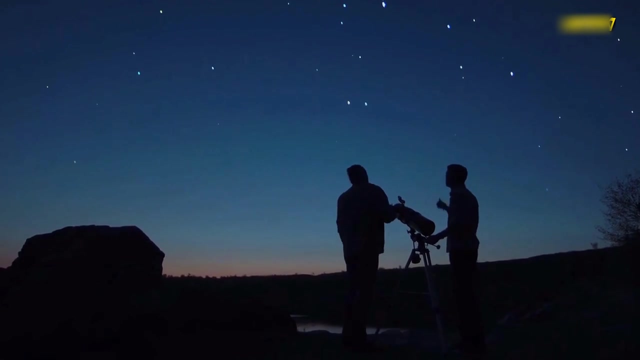 The Earth is a large asteroid with a diameter of about 2.5 billion kilometers. It is seen that it is about 4.5 billion kilometers. But this was just the start of Jupiter's reign of terror. Further and further, the young Jupiter fell until it reached the vicinity of where Mars orbits today, just 225 million kilometers or so from the Sun. This was no quiet visitor to our local neighborhood. A planet of this size can wreak havoc just by its proximity, And Jupiter's arrival in the inner solar system did just that. 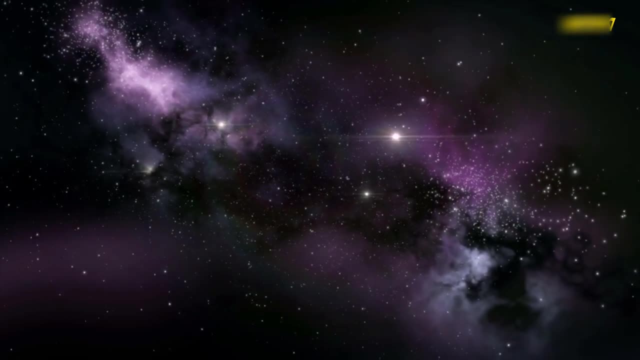 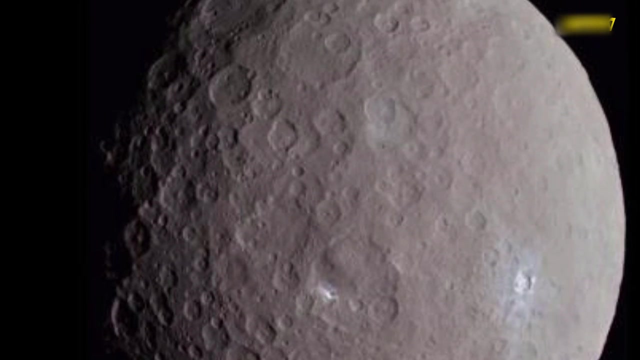 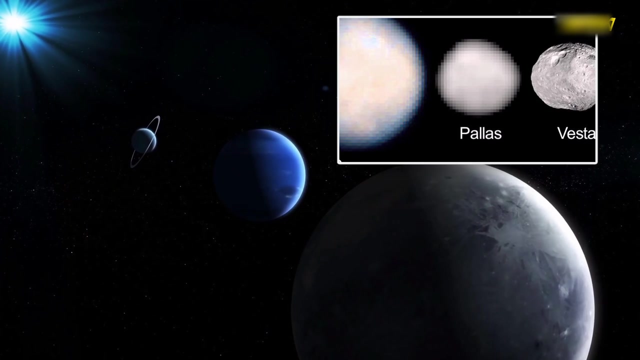 transforming the destiny of many of the emerging new worlds, including our own. Lee Fletcher, from Jupiter Icy Moons Explorer mission explains this action as a tug of war Between the orbits of Mars and Jupiter, we have a large accumulation of objects, rocky objects, mostly known as the asteroid belt. 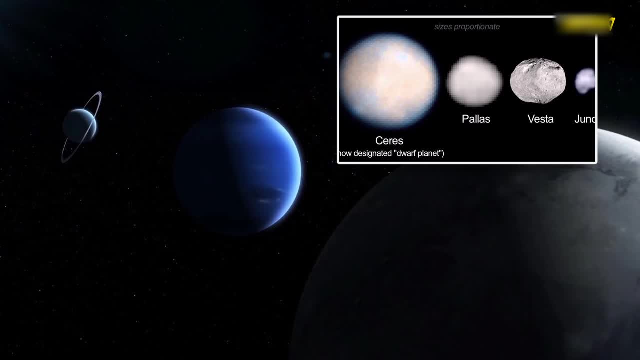 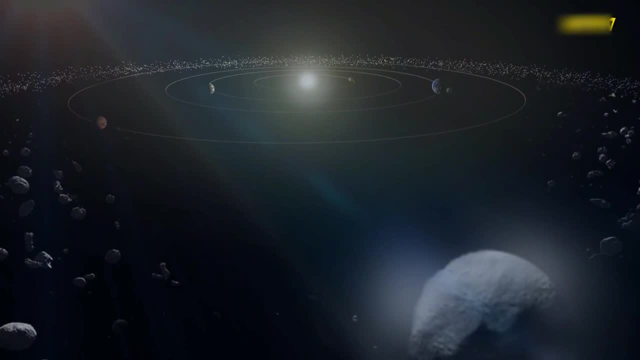 They're not able to form and agglomerate into a complete planet because of the constant tug of war between the gravitational forces of the Sun and of Jupiter. So what we see today is a large disk of objects that could be the remnants left over from the formation of our solar system. 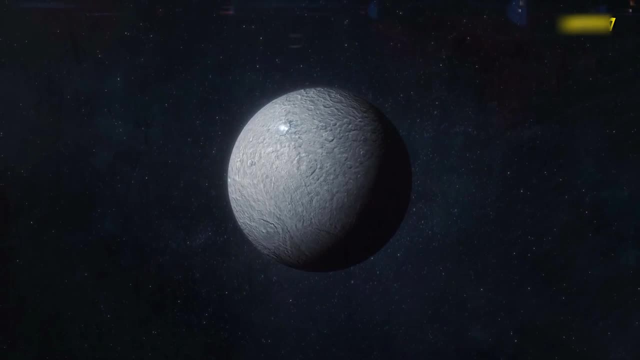 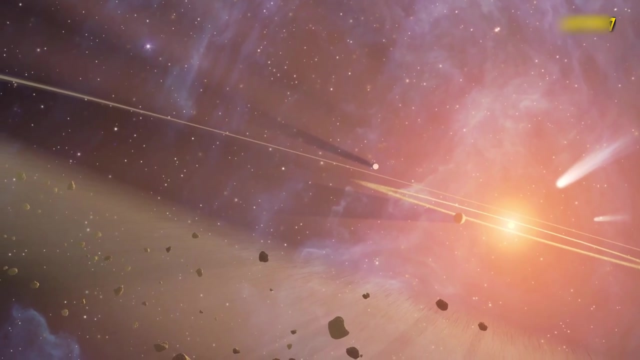 To understand just how powerful a presence Jupiter must have been as it marauded around the inner solar system, we need to look no further than the worlds it has in its iron grip today. Jupiter has, at the time of writing, 79 known moons held in its orbit by the powerful gravitational field. 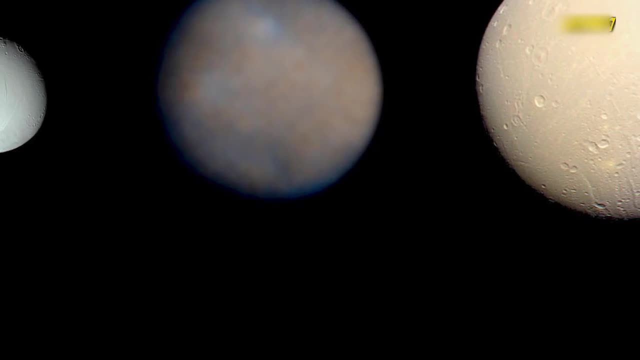 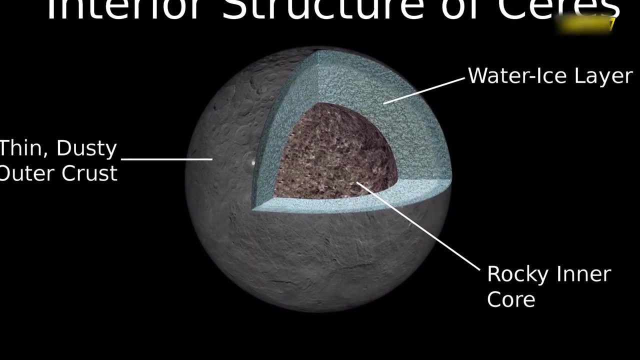 that is generated by the planet's enormous mass, a powerful force field that is generated by the force that reaches out from the planet deep into the solar system. It's what has made Jupiter so destructive in the past and through our exploration of the Jovian system. 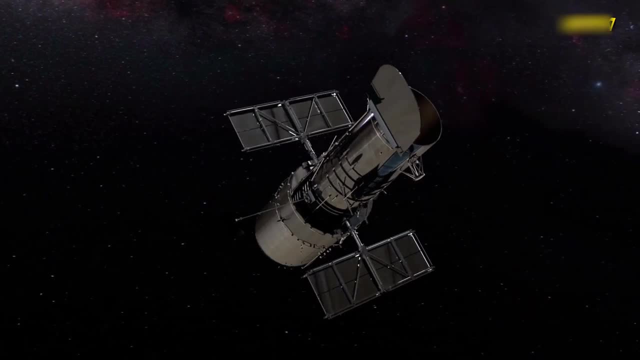 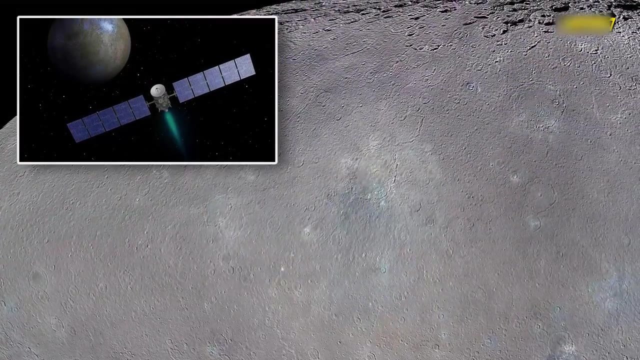 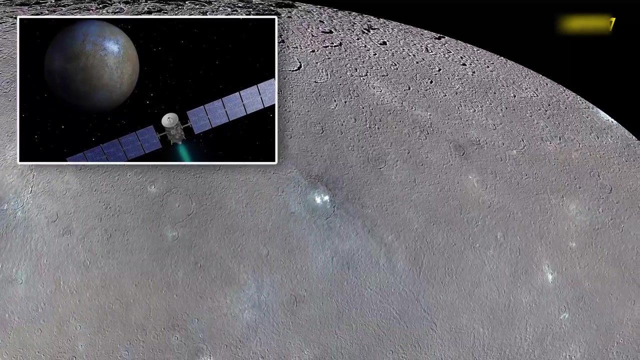 we have also witnessed its awesome power today. Nowhere is this power more dramatically revealed than on Io, the closest of all the moons to Jupiter. Io orbits just 350,000 kilometers from the cloud tops of its mother planet, a distance that makes it a gravitationally tortured world. 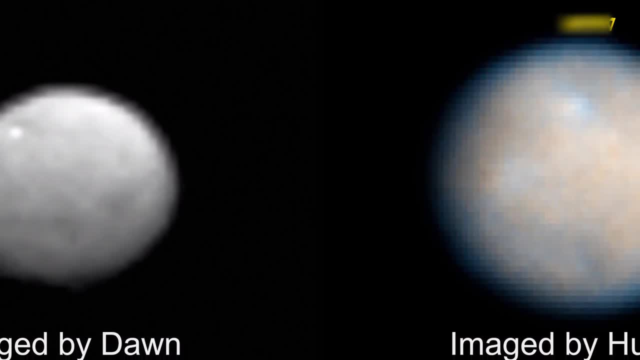 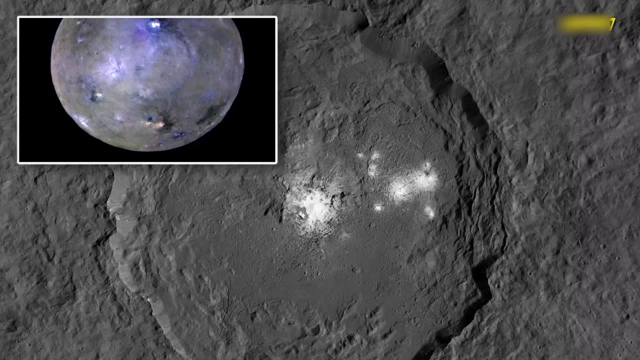 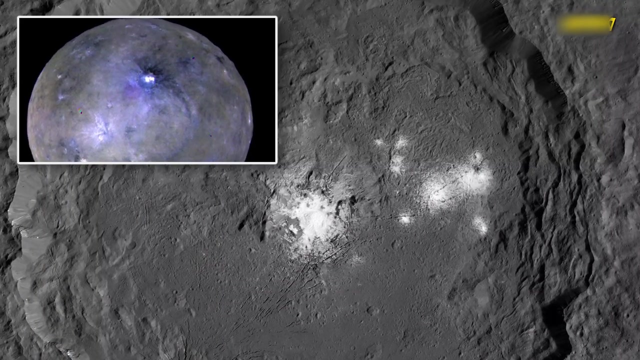 A volcanic vision of hell. this is the most geologically active object in the solar system, with over 400 active volcanoes from which lava flows stretch hundreds of kilometers across the moon's surface and vast clouds of pyroclastic material blow hundreds of kilometers up into space. 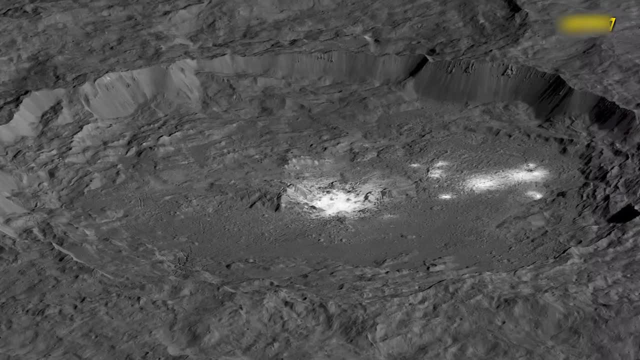 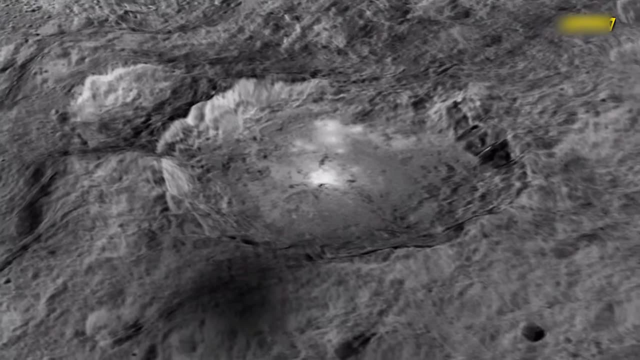 creating distinctive umbrella-shaped plumes above its surface. The surface of Io is perhaps the closest that our solar system has to offer of a vision of hell, and all of this activity is created not by ancient internal heat as we see on our planet Earth. 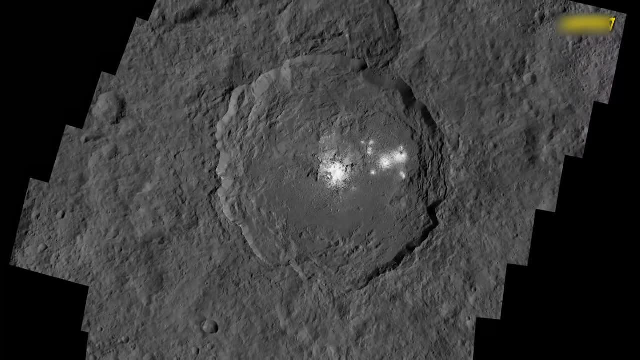 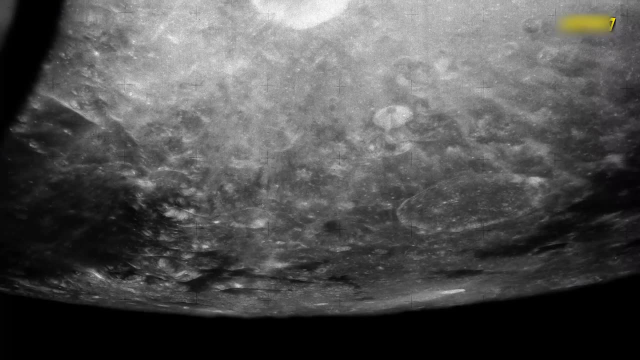 but by the power and the influence of Jupiter's gravitational pull Here on Earth. the volcanism that we see across our planet is driven by a combination of the heat that remains from our planet's violent formation and that which is released from the decay of radioactive elements. 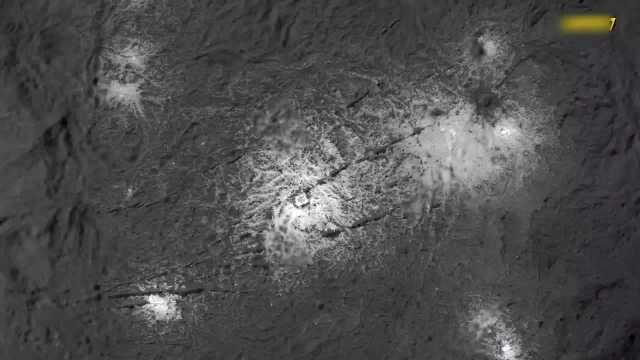 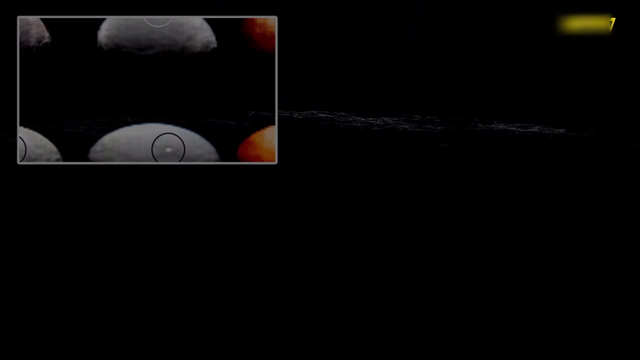 locked away in the planet's interior. This heat, combined with the high pressures below the surface, creates the molten rock that pools within the mantle layer of the Earth, and then, in certain places, this magma finds a route to the surface, creating a volcano. 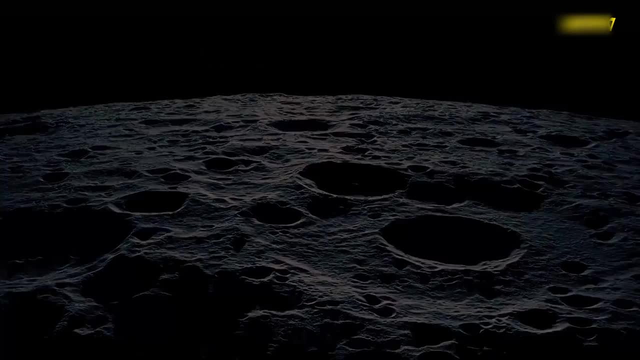 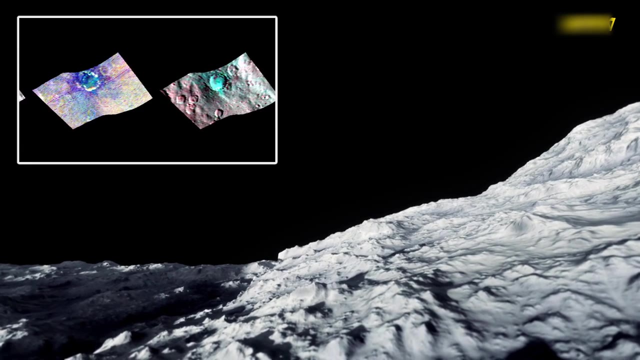 On Io. the volcanism is nothing like this. Instead, it's being generated by a completely different mechanism, a process called tidal heating, that is driven in large part by its proximity to Jupiter and the gravitational tug-of-war between other nearby moons. 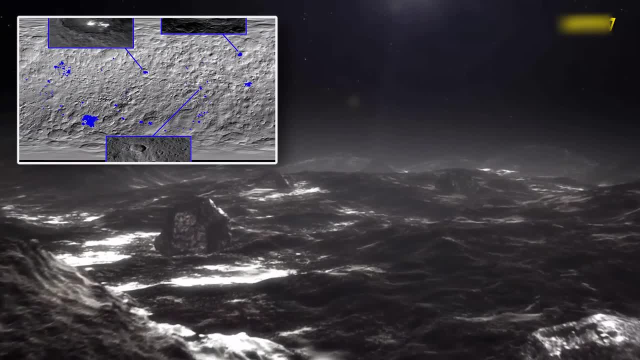 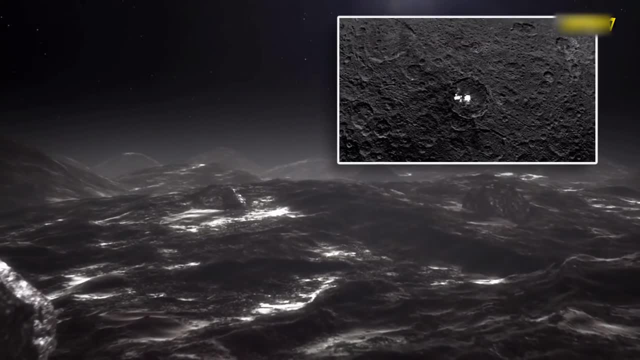 Io is caught between the vast mass of Earth and the vast mass of Jupiter on one side, and the three other- Galilean, moons, Europa, Ganymede and Callisto- on the other. a dynamic that pulls in different directions to violent effect. 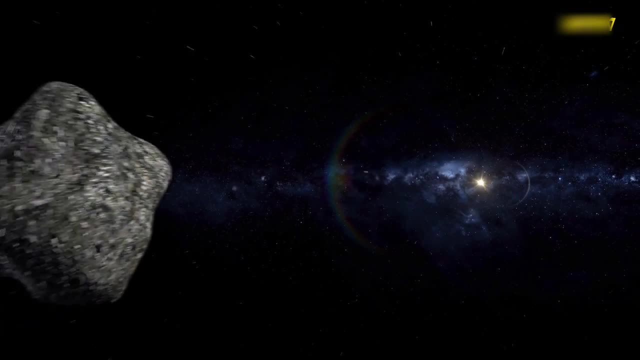 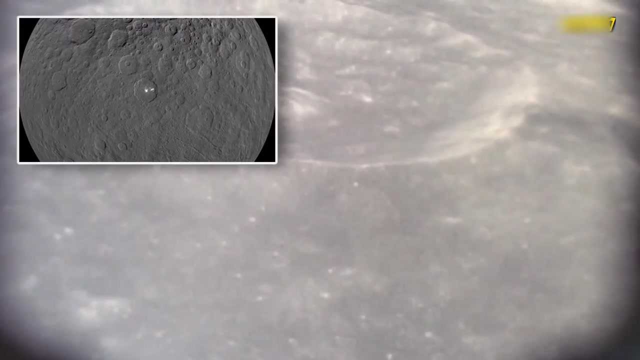 It's a dynamic that we see in part on our planet every day, as the force of gravity flexes its muscles in the interaction between the Earth and the Moon, creating the twice-daily ebb and flow of our tides On Earth: the gravitational tug of the Moon. 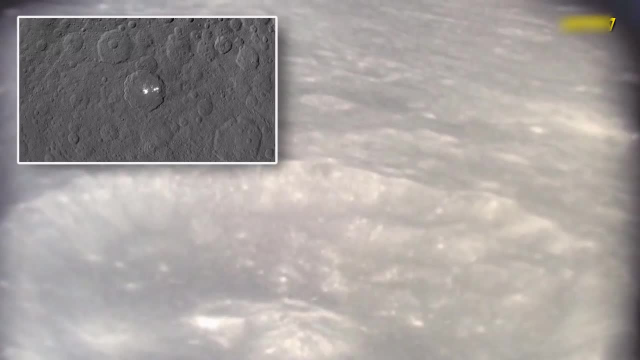 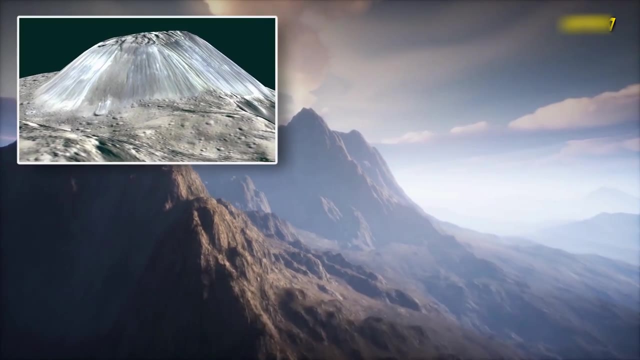 creates a tidal force that moves vast volumes of water around the planet, with the biggest difference between low and high tide, creating a shift of a maximum of 12 metres in the height of water. The same principle also applies on the surface of the Moon. 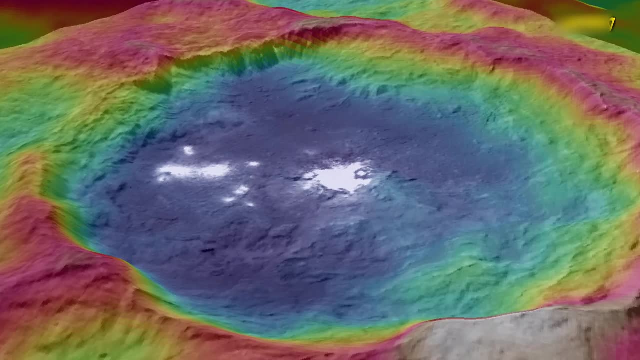 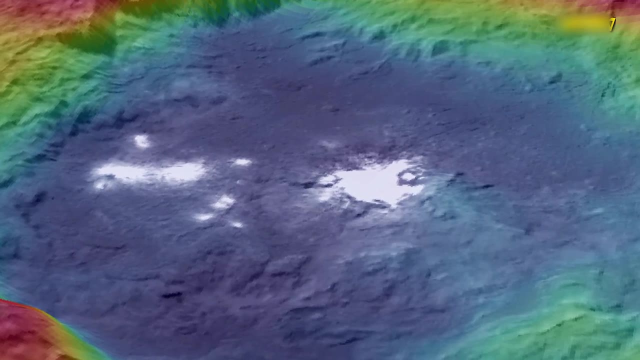 where the gravitational pull of the Earth creates tides not of water but of rock. Moon tides are small changes in the height of rocks on the lunar surface caused by the pull of the Earth's gravity. In the case of the Earth-Moon system. 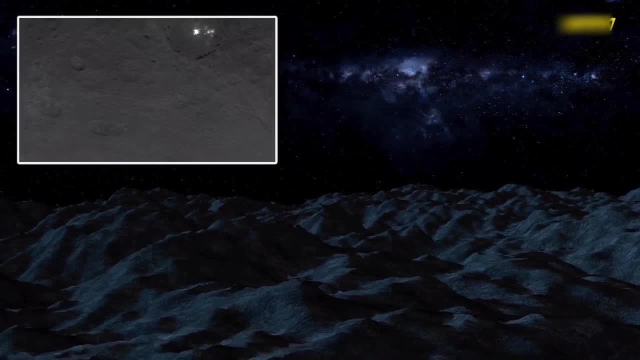 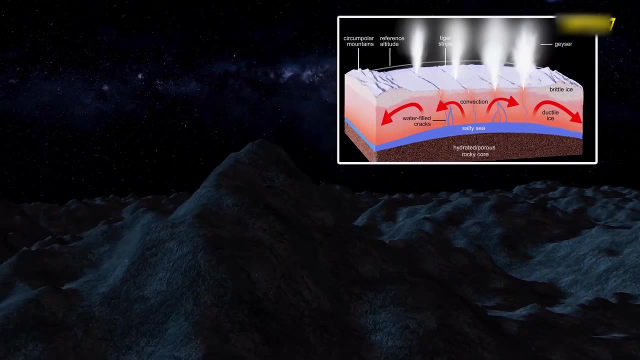 these rock tides are measured in just a few centimetres, but Io tells a very different story. Io is roughly the same distance from Jupiter as our Moon is from Earth, and both moons are of equal size, But because Jupiter is so much more massive. 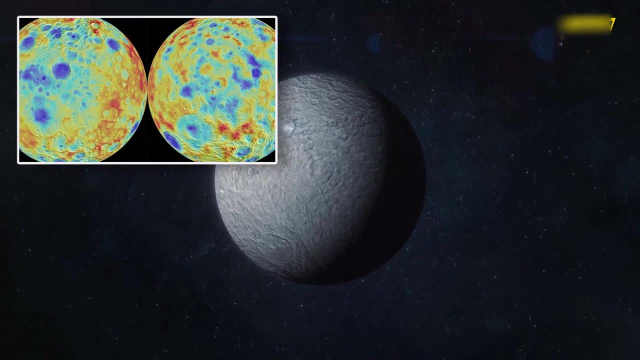 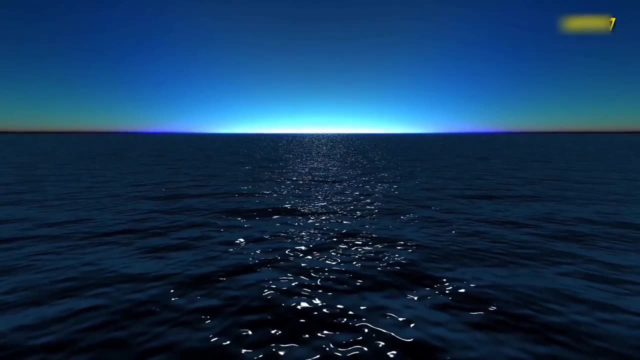 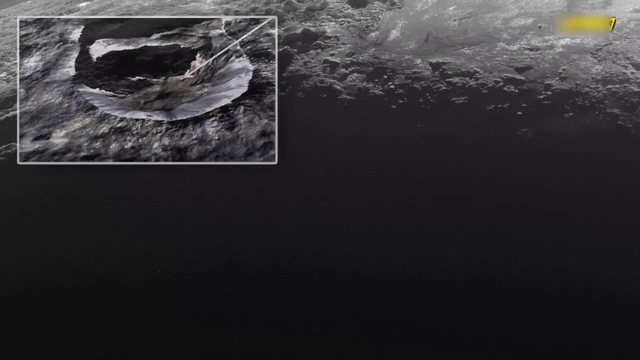 the tidal forces it generates are much greater, with the gravitational pull of Jupiter moving the bulge of rock tides up to 100 metres between low and high tide. That's five times the height of any tide here on Earth. In fact, Io contains the least amount of water. 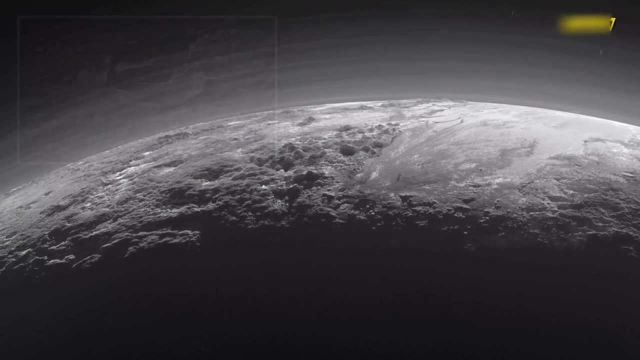 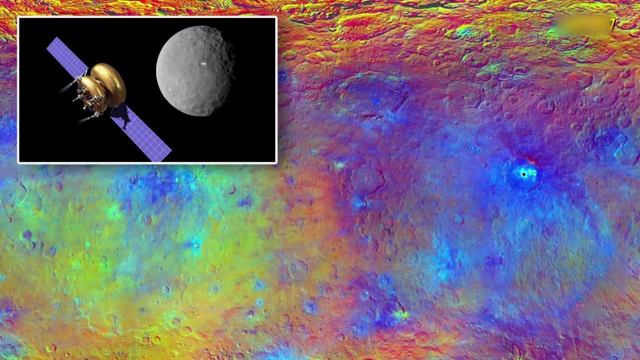 of any known object in the Solar System. But this is not the end of Io's torture. Its relationship with the other large moons, particularly the next moon out Europa, also adds to the destructive forces that are pulling the very substance of Io apart. 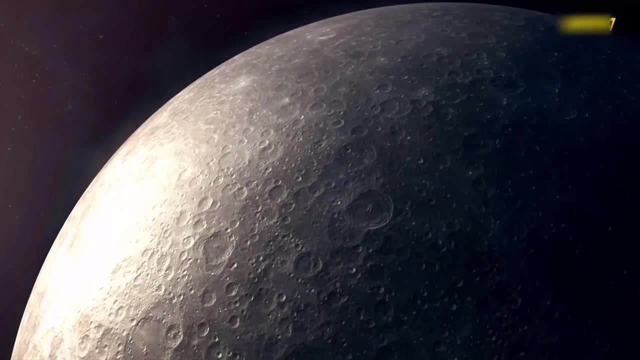 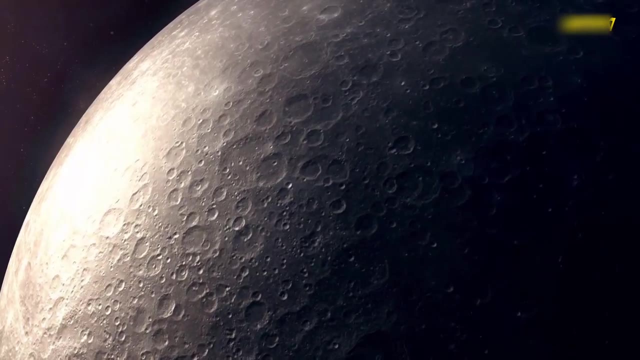 Io whips around Jupiter much quicker than our Moon goes around the Earth, once again due to the mass of Jupiter, completing an orbit once every 42 metres. But Io is much faster than Jupiter, as it does an orbit once every 42 hours. 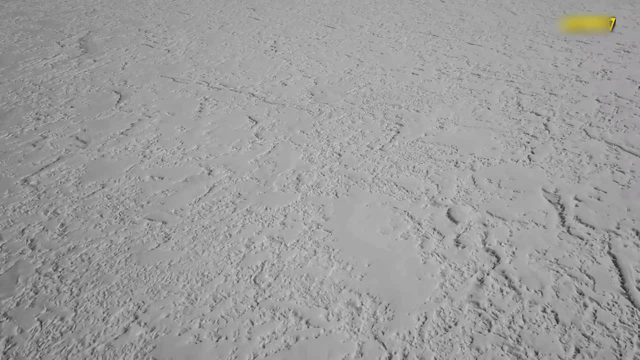 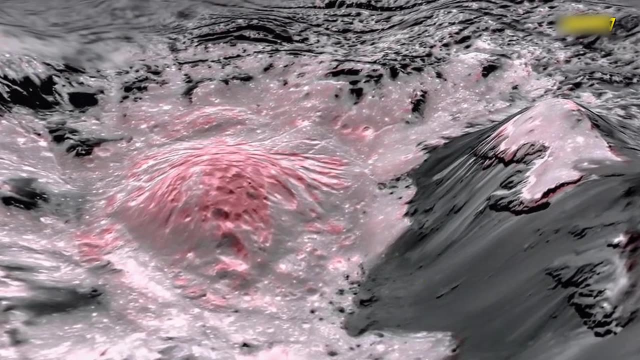 If left alone, Io would complete this orbit in a near-perfect circle around the giant planet. But Io is far from alone and with Europa circling Jupiter precisely once every two orbits of Io, it means that in every second orbit Europa and Io line up. 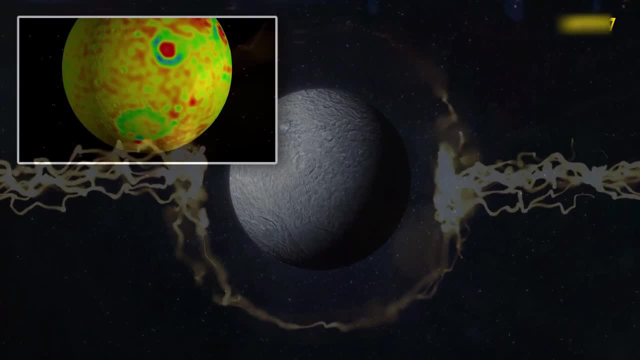 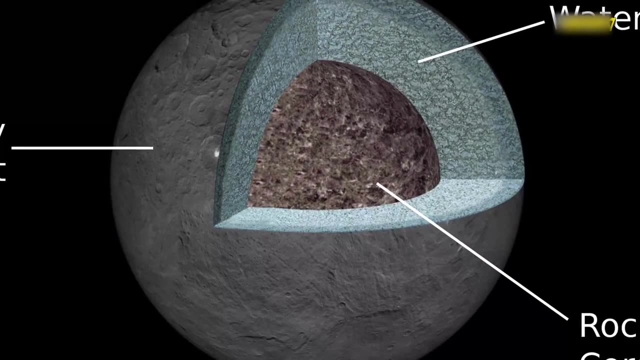 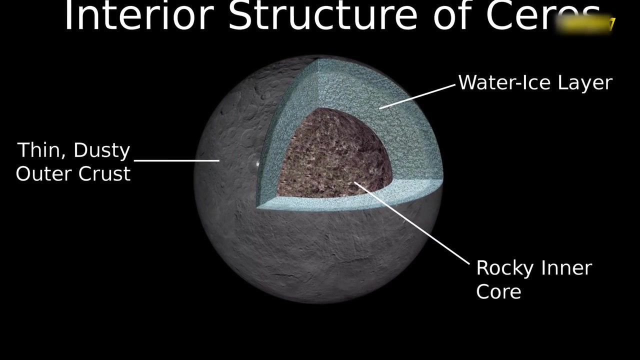 and that rhythmic orbit has consequences. This is what's known as an orbital resonance, and the result is that it gives Io a final gravitational kick that moves the Moon's orbit out of a circle and into an ellipse. Ganymede is also in a resonant orbit with Io. 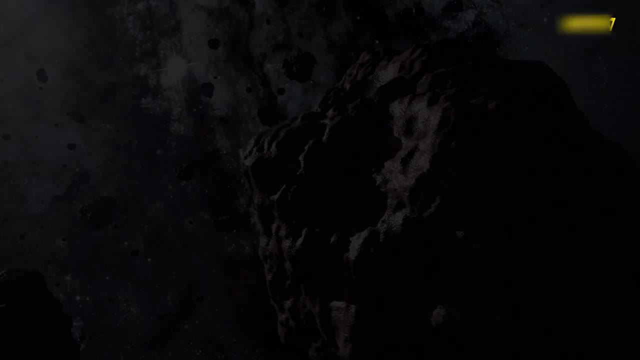 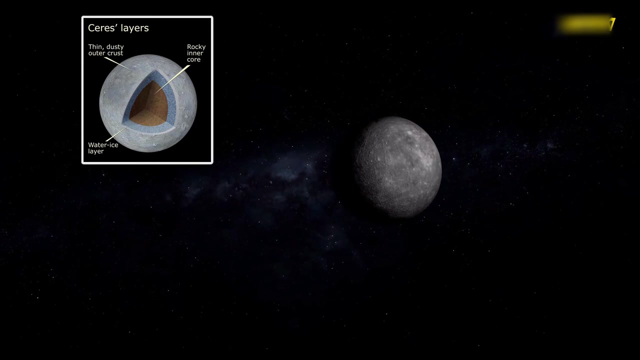 in a 1 to 4 orbital period ratio, and the outcome of this is that, as Io orbits, the gravitational forces are constantly shifting and changing, and that stretches and squashes the Moon, creating vast amounts of friction that causes its interior to heat up. It's a process called tidal heating, and it's this generation of heat that produces Io's volcanoes, raising the temperature in its interior to over 1,200 degrees Celsius and creating the violent world of lava lakes and volcanic plumes that we've witnessed through the eyes. of Galileo and Voyager. The pull of the two moons on Io also stops it gradually falling inwards to Jupiter and being completely ripped apart. Io is an extraordinary example of the power of Jupiter and a demonstration of how this planet can shape and change the destiny of worlds. Because of its huge mass and the intense gravitational force this produces, any planet or moon that gets too close to it is under threat. While Earth is at a relatively safe distance today, 4.5 billion years ago, as Jupiter moved into the inner solar system, it began to exert its power right in the spot where Mars and our own world were beginning to form. 4.5 billion years ago, the region of the solar system we call home was densely packed with gas and rock, a planetary nursery full of embryonic worlds. each with a different destiny in store. But this fertile space was about to be thrown into chaos by the solar system's most unwelcome of visitors. As Jupiter was pulled from its distant orbit and continued its inwards descent, it paused in this planetary breeding ground. The consequences of this action would be significant and far-reaching. Detailed simulations of the impact this wandering Jupiter would have made suggest that the fate of any super-Earths caught in mid-formation would have been thrown into chaos. The models suggest that Jupiter's inward journey would have driven thousands upon thousands of planetesimals, many over 100 kilometres wide, spiralling into the inner solar system. This planetary breeding ground was turned into a battleground, as Jupiter's presence threw the orbits of any newly forming super-Earths. into the overlapping paths of thousands of massive blocks of rock and ice. The result was carnage, a cascade of collisions that blew apart planets and left a trail of fragmentary worlds in its wake, a chain reaction that would culminate in the formation of a spiralling swirl. of gas, dust and rock which would eventually have swept any surviving super-Earths towards the Sun and ultimately to their destruction. In what was just a fleeting moment in the history of our solar system, its destiny changed forever. Our planet would not fit the norm. of super-Earths and the tightly packed gas giants that we see across the Milky Way. Instead, we think the inner solar system would have been swept clear of up to 90% of the rocky material thrown in by Jupiter, With just crumbs remaining. four small terrestrial planets began to form from the rubble. With Jupiter marauding in its orbit, much of the material that could have gone on to form Mars was lost, leaving the planet with enough scraps to make a planet half its potential size and transforming it from a possible habitat for life. to a world that would freeze and die in its adolescence. Just that little bit further in, Earth found itself forming in a slightly more substantial ring of gas and dust that would make it the largest of all the terrestrial planets. A lucky escape for our future home. because had Jupiter continued on its inward path, Earth might never have formed at all. But just as it looked like it would sweep everything away, Jupiter stopped in its tracks On its inward journey, Jupiter had transformed the inner solar system, sweeping away the formative giant planets. and leaving just enough material for Mars, Earth, Venus and Mercury to form. But the stage was now set for another player to enter the story and shift the destiny of both our world and the solar system, once again Waiting in the shadows of the outer solar system. another massive planet was lurking that we now think pulled Jupiter back from the brink. Saturn, a gas giant not as big as Jupiter but enormous nonetheless, began its own slow drift inwards towards the Sun, Formed much further out than Jupiter as Saturn began turning inwards. it would have a profound effect on Jupiter's trajectory. As the two giants drew closer together, they became locked in an intimate gravitational dance, an orbital resonance. that meant that for every orbit Saturn made around the Sun, Jupiter made two circuits exerting a regular, periodic gravitational force. on each other as the two giant worlds passed close by. The result of this orbital resonance between Jupiter and Saturn cleared out all of the gas and dust between the two planets, creating a gap in the disc of the early solar system. And this interaction between the two resonant planets. and the gas and dust at the edge of the gap resulted in both planets changing tack. The orbits of both Saturn and Jupiter began to move outwards, away from the Sun, preventing Jupiter from moving any further into the inner solar system. Earth was given a reprieve. and Jupiter was dragged back out into the asteroid belt once more. This change in direction has become known as the Grand Tack Hypothesis, a nod to the action of a sailboat as it tacks and changes course while it travels against the direction of the wind. Just like a sailboat. the theory suggests Jupiter tacked around 1.5 AU from the Sun in the current orbit of Mars, changing direction and pulling back out to its current orbit at 5.2 AU. It's a theory that's been driven. by using advanced computer modelling, which helps to explain many of the inconsistencies between our solar system and the hundreds of other planetary systems we've recently observed. It's the Grand Tack that accounts for the lack of super-Earths and explains the presence of only a handful. of small rocky worlds with thinner atmospheres than those observed around other stars. The Grand Tack also allows us to explain the unusually small size of Mars, which simulations predict should be at least half the mass of the Earth, if not bigger, rather than the 0.107 Earth's mass. we find it to be. It also helps explain the odd inhabitants of the asteroid belt transformed by Jupiter's journey, not just once, but twice, across this region of space. This is why we see half-finished planets like Ceres and Vesta, left starved of building material. and an asteroid belt that has a surprisingly small mass, with objects that appear to originate from both inside and outside Jupiter's orbit and have a wide range of eccentric orbits themselves. Jupiter, the father of the skies and ruler of the heavens, had spread its hand far and wide. sculpting the precious solar system we see today in the space of just a few million years. Before coming to rest, though, it would grant one more precious gift to the newly forming planet Earth, As Jupiter was dragged out crossing the asteroid belt for a second time. it encountered a region full of objects rich in water and bearing minerals, and Jupiter's trajectory caused these objects to be flung back into the inner solar system. They crashed into the young planets and moons with an intensity never seen before or since, in a period known as the Late Heavy Bombardment. It transformed the make-up of the inner solar system, delivering a large percentage of the water Earth holds on its surface today, It's extraordinary to think that it was Jupiter that was responsible for the delivery of the most important ingredient of life: the water. that provided an ideal environment. for life to spark and thrive in one unbroken line for the last four billion years. This story offers an extraordinary understanding of the power Jupiter has wielded over all of our lives, The more we learn about the formation of solar systems and the more we try to model a system like ours. with four terrestrial, water-rich planets close to the star and the gas giants further out, the more we learn that perhaps all these things had to happen, These unlikely movements and interactions between the planets were necessary to produce a system like ours and a planet like ours. So if events like the attack of Jupiter are, as we believe them to be, extremely uncommon, the conditions for the formation of Earth-like planets, terrestrial worlds with plenty of liquid water beneath the gentle pressures of a thin blue line, must be exceedingly uncommon. It's a humbling thought to begin to comprehend that the Earth may not just be a rare rock in our solar system, but a rock that only exists because of the rare system of planets within which it evolved. All the evidence is beginning to suggest that we may be living on a tiny oasis. within a vast desert devoid of life and stretching out across the Milky Way. Today, Jupiter has settled into a regular orbit at the far side of the asteroid belt. its days of marauding through the solar system at an end Established in a stable orbit for almost four billion years. it has looked down on our planet as a distant light in the sky, unchanging while the work of evolution by natural selection has transformed the first sparks of life on Earth into the endless beautiful forms that we witness today. But although Jupiter is not the only planet, that is distant and seemingly detached. Jupiter's influence has been far from benign. The history of life on Earth has been interrupted by numerous cataclysms, impacts with asteroids that have fundamentally shifted life again and again, And the hand behind these disruptions, It's Jupiter. that has continued to hold immense sway over our planet, exerting its influence on the asteroid belt with just the smallest of nudges: The difference between existence and extinction. At 1653 UTC on the 18th of October 1989, the space shuttle Atlantis took off from the Kennedy Space Center in Florida. carrying the Galileo spacecraft, carefully packed away in its hold. Released into Earth's orbit from the cargo bay just a few hours later, the probe would begin a six-year journey to Jupiter that would utilize flybys of Earth and Venus to propel it on its 4.6 million kilometers. The probe would then be able to fly a six-year-long, 10-kilometer voyage across the solar system. Entering orbit around the giant planet on the 8th of December 1995,, Galileo would not only become the first spacecraft to orbit Jupiter. but also the first craft to orbit any of the outer planets. It spent nearly eight years in the Jovian system and explored the giant planet and its menagerie of moons in intricate detail for the very first time, revealing a host of new discoveries. 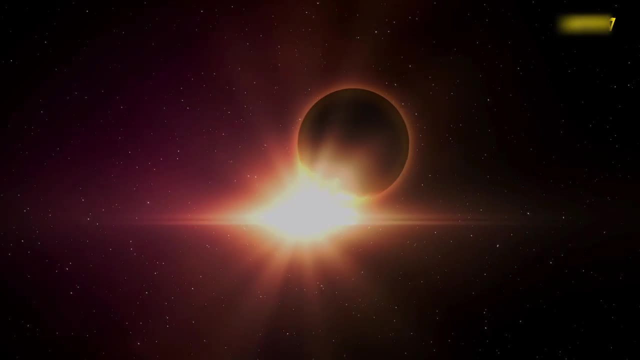 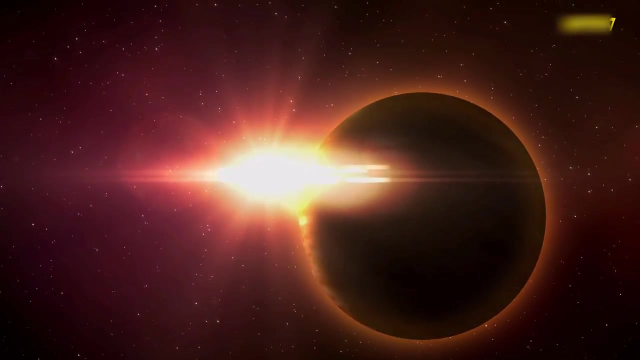 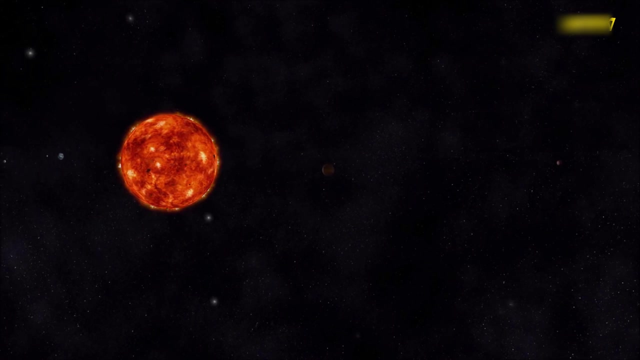 From precise measurements of Jupiter's atmosphere and observation of its giant thunderstorms to discovering liquid water under the surface of the moon Europa and the first detailed studies of the intense volcanic activity of Io. this was a mission that opened our eyes to the beauty and diversity of the Jovian system. 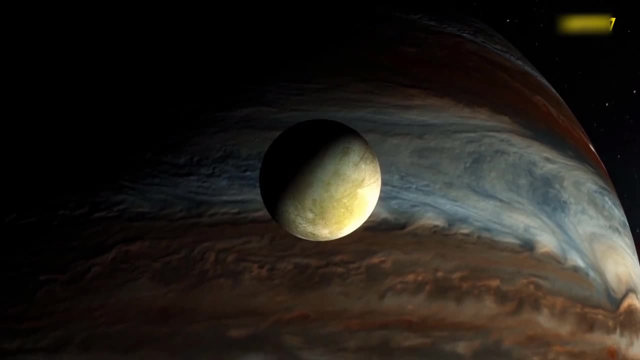 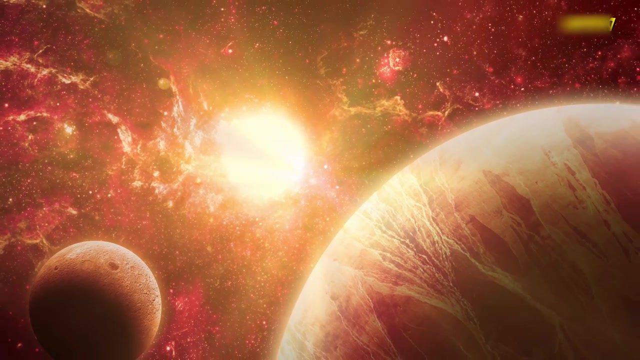 in a level of detail that we could scarcely have imagined possible. But long before Galileo even arrived, this two-ton explorer would already have changed our lives. It was only a matter of time before Galileo would be able to take a close-up view of the solar system. 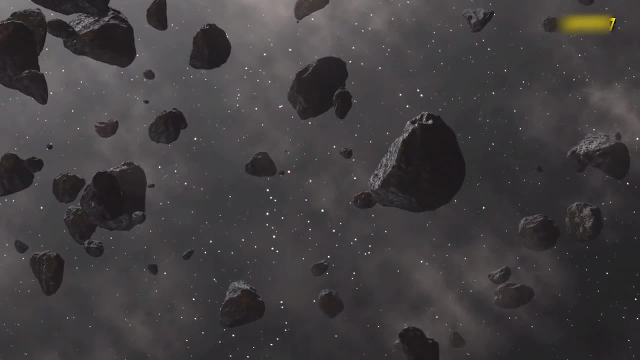 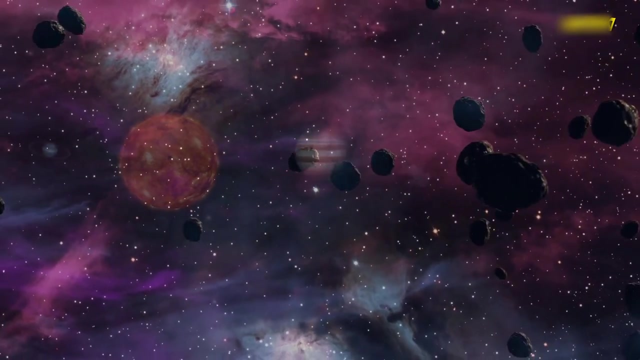 Entering the asteroid belt. in August 1991, Galileo performed the first close-up flyby of an asteroid passing within 1,500 kilometers of 951 Gaspra and returning the first detailed images of this rocky remnant back to Earth. 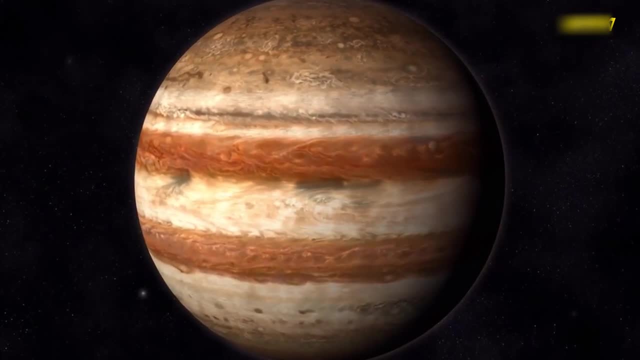 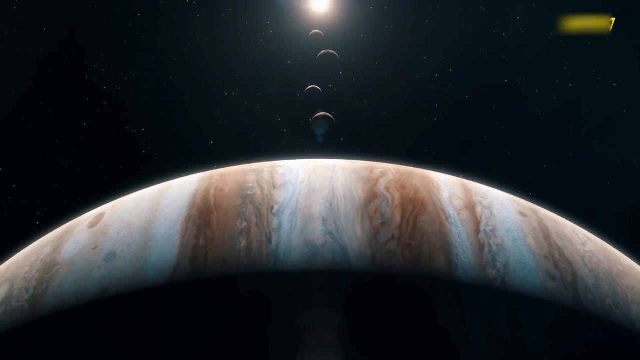 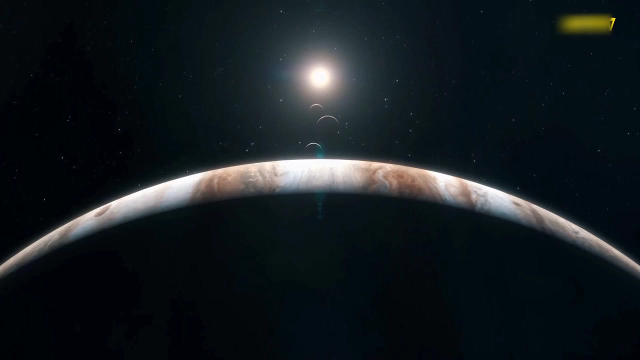 Its next close encounter would come almost two years later, when flying past 243 Ida. the probe discovered that this asteroid had its own moon, which was the first asteroid moon ever to be discovered, And the images are beautiful: a tiny, 1.5 kilometer wide object. 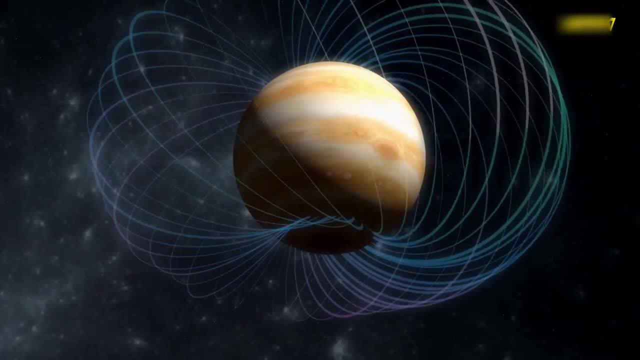 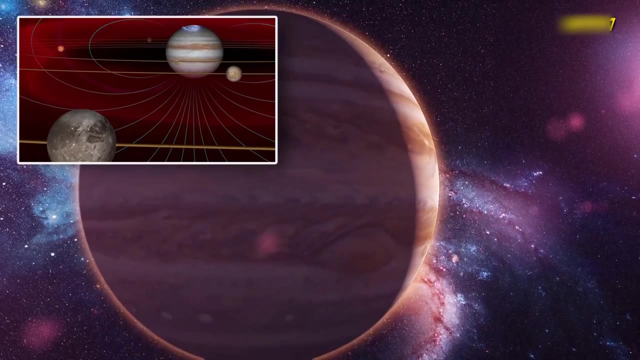 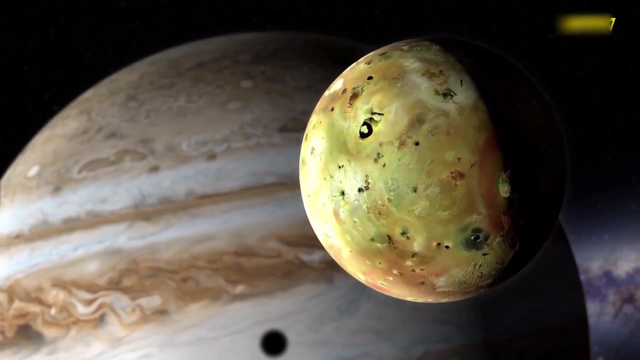 in a chaotic orbit around its parent rock. After this unexpected encounter, Galileo continued its long journey across millions of kilometers of empty space, still four years away from its ultimate rendezvous with Jupiter. But by luck, rather than judgment, this tiny probe happened to be traveling towards Jupiter. 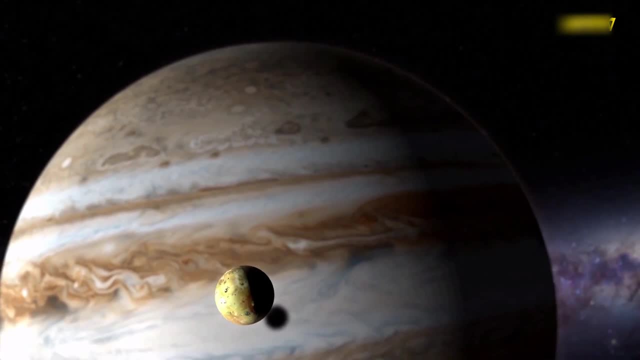 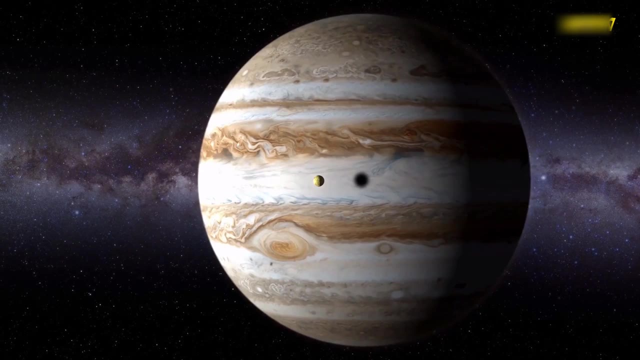 at the precise moment it would be able to witness one of the rarest of shows our solar system has to offer. On the night of the 24th of March 1993, as Galileo sped across the solar system, three astronomers working at the Palomar Observatory in California. 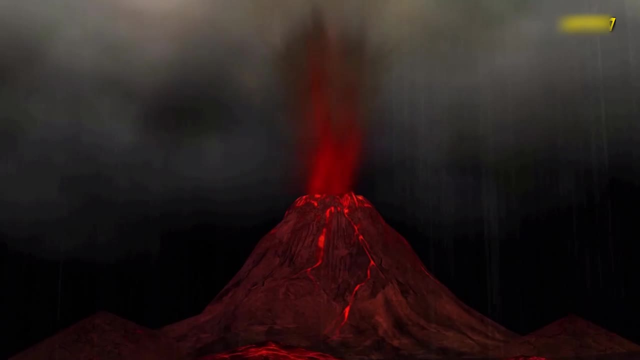 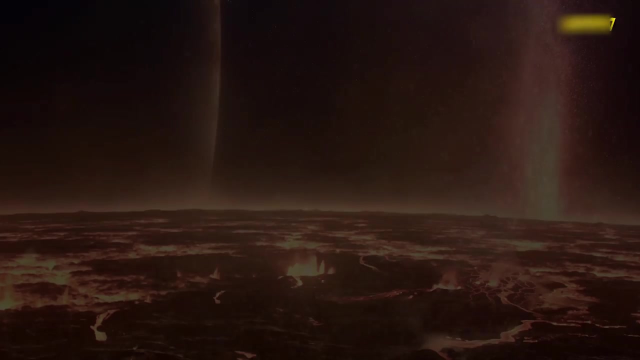 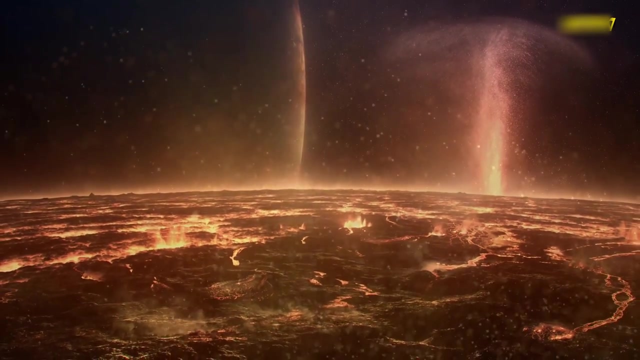 were attempting to spot and track what are known as near-Earth objects: undetected meteors that might be of potential threat to our planet. That evening, David Levy, along with Carolyn and Eugene, took a series of images using the 1.5-foot Schmidt telescope. 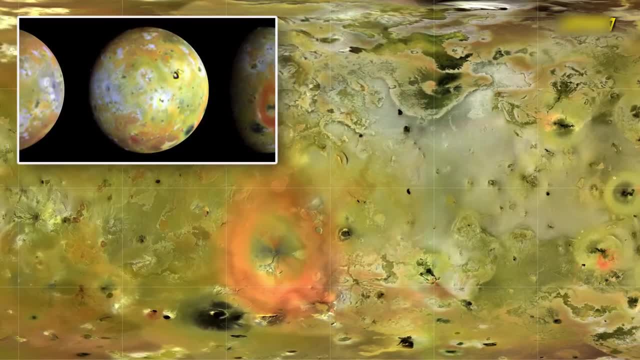 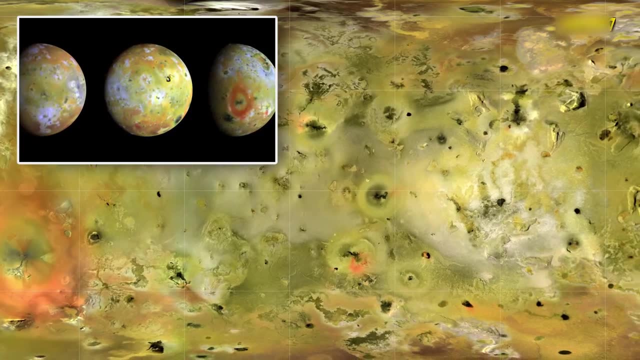 Lurking in one of them was an unusual artifact that grabbed the attention of the team. Streaking across the image was an object that, although nowhere near the Earth, was of immediate and immense interest, A comet that appeared not only to be unusually close to Jupiter. 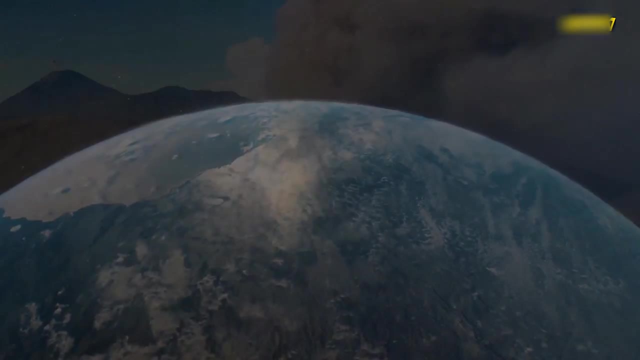 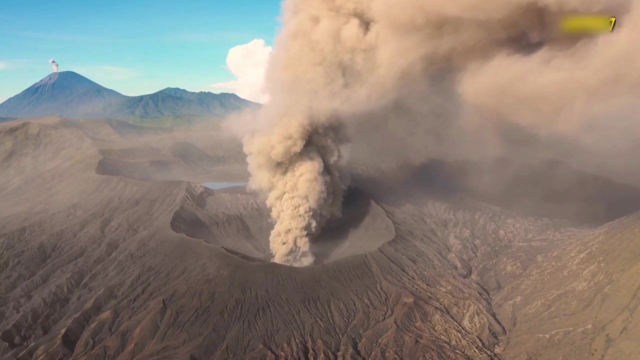 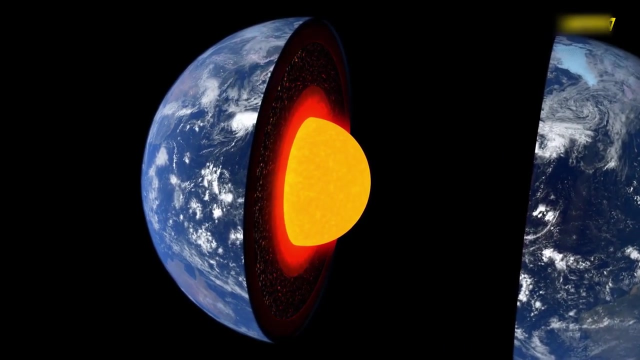 but also seemed to have multiple nuclei, A fragmented series of rocks trailing across one million kilometers of space. In a moment of wondrous astronomical serendipity, the team had discovered the first-ever comet in orbit around another planet, A comet that had not only been captured by Jupiter's immense gravity, 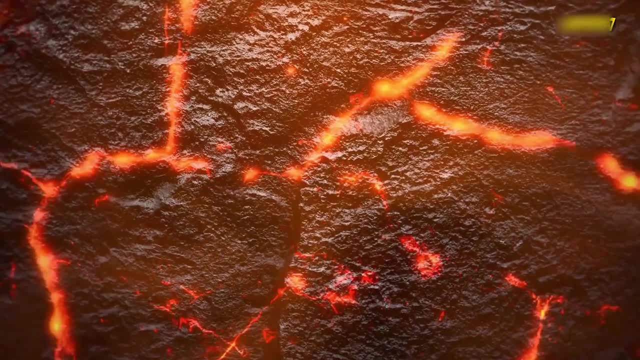 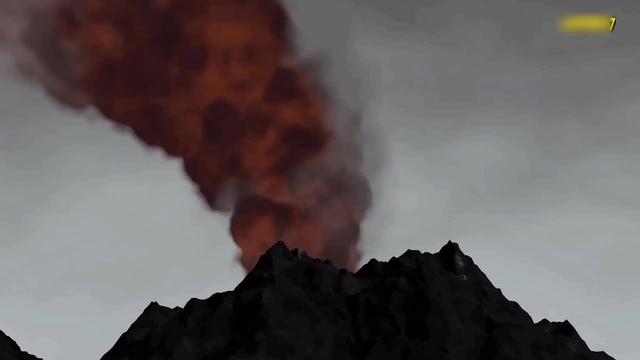 but had also been pulled apart by it. Shoemaker-Levy 9,, as it became known, because it was the ninth comet this team had found was a comet unlike anything we'd seen before, Quickly confirmed by further studies to be orbiting Jupiter. 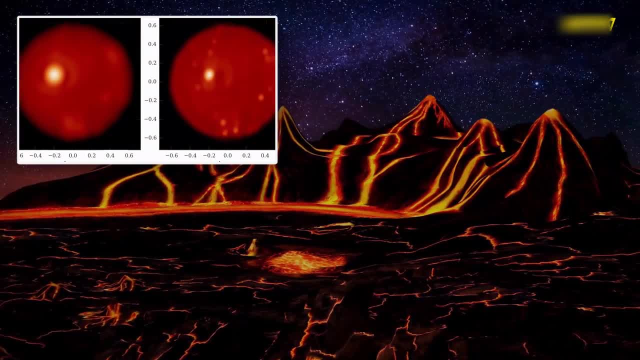 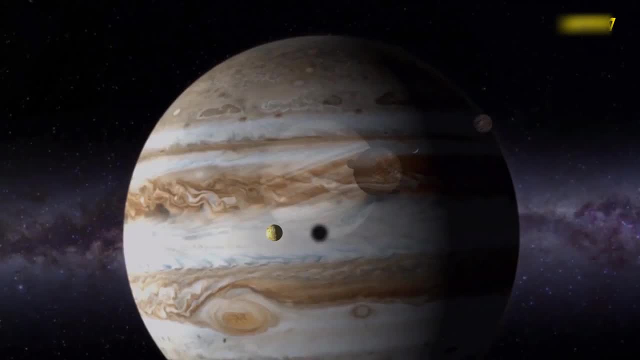 and thought to have been captured from its solar orbit back in the late 1960s or early 1970s. astronomers were able to wind back through its orbital history and calculate the precise moment the comet was ripped apart, Passing just over 40,000 kilometers above Jupiter's cloud tops. 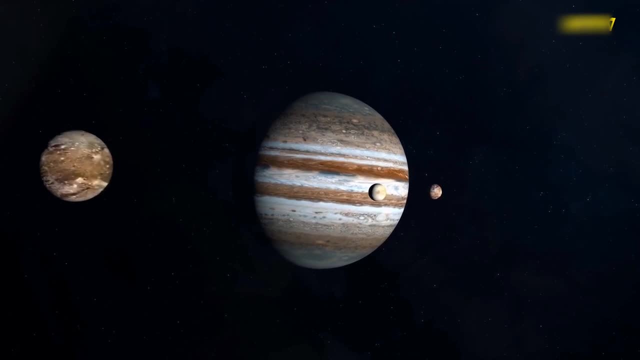 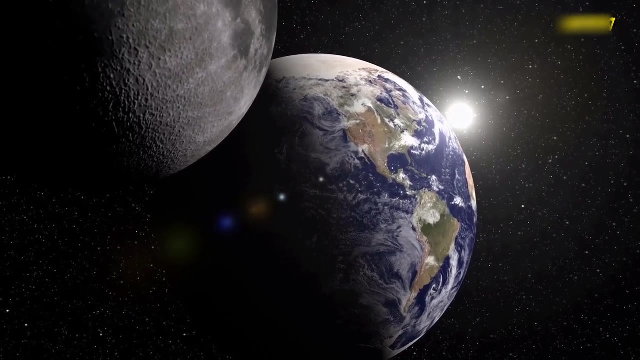 on the 7th of July 1992,, we think, Shoemaker-Levy 9 fell within the planet's Roche limit and this five-kilometer comet was ripped apart by the huge tidal forces generated this close to the planet. 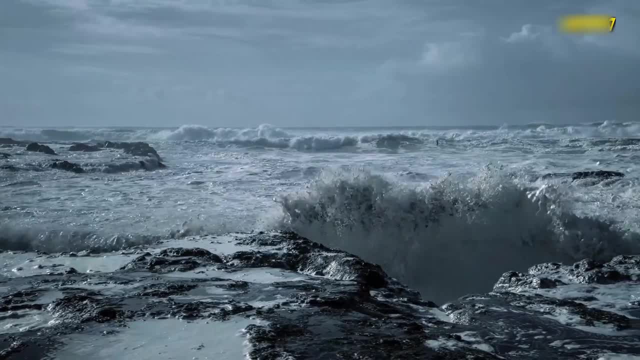 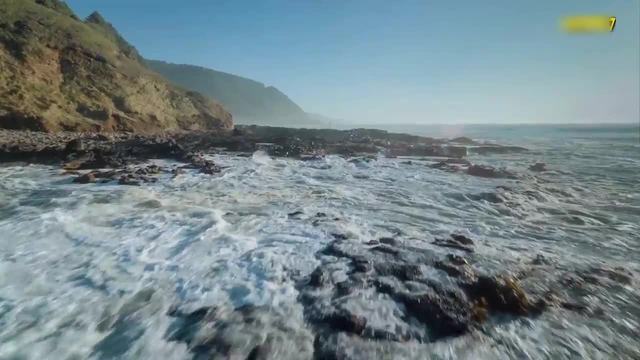 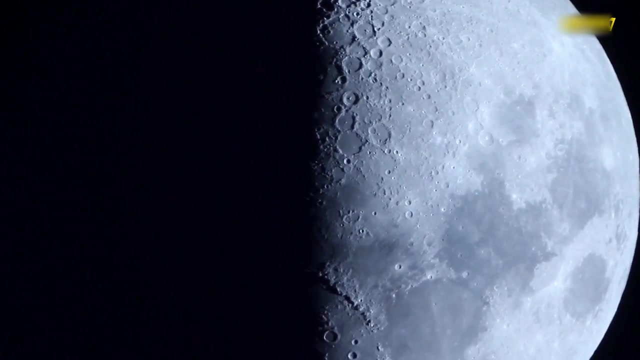 It disintegrated into 23 pieces visible to us here on Earth, labeled fragments A to W, with the biggest up to two kilometers in diameter. This alone was a remarkable discovery, a visual representation of Jupiter's colossal gravitational power. But if that wasn't enough, 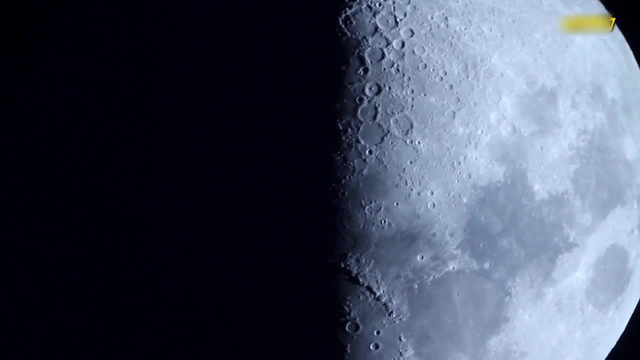 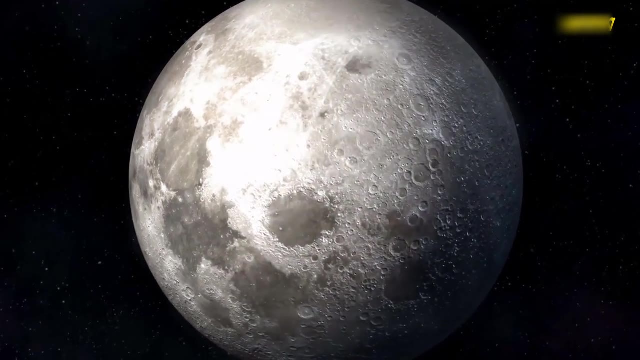 it quickly emerged from orbital calculations that the comet seemed to be on a trajectory that would ultimately take it straight through the center of the planet. Shoemaker-Levy 9 was on a collision course with Jupiter, and as if we had scheduled it ourselves. 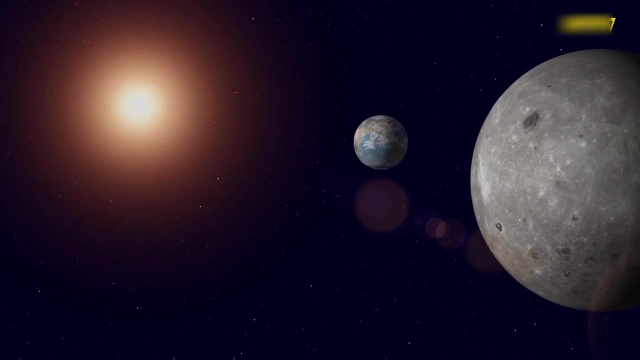 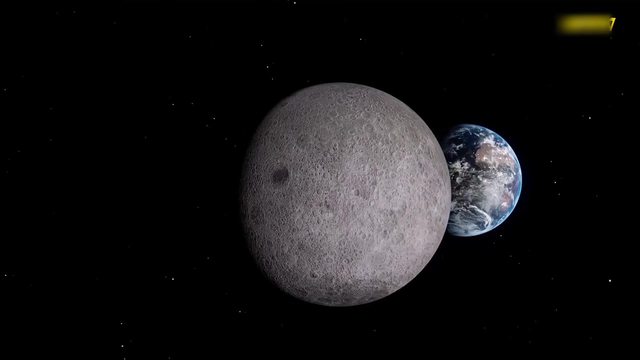 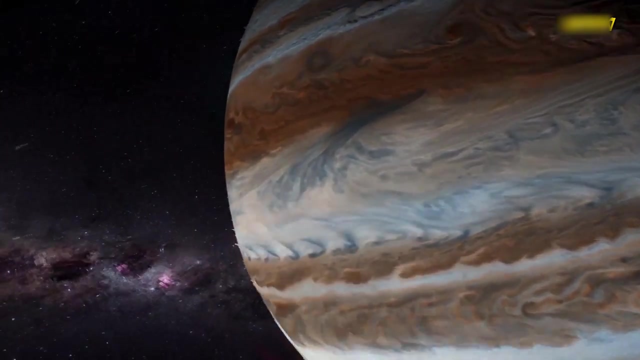 the date of the predicted impact was July 1994, perfect timing for the spacecraft we already had en route By the beginning of July 1994,, Galileo was 238 million kilometers from Jupiter, on the very edge of the asteroid belt. 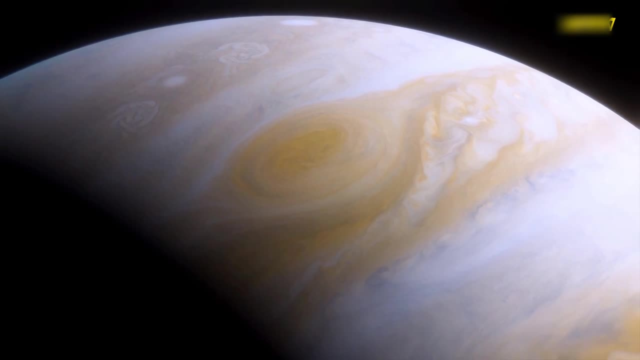 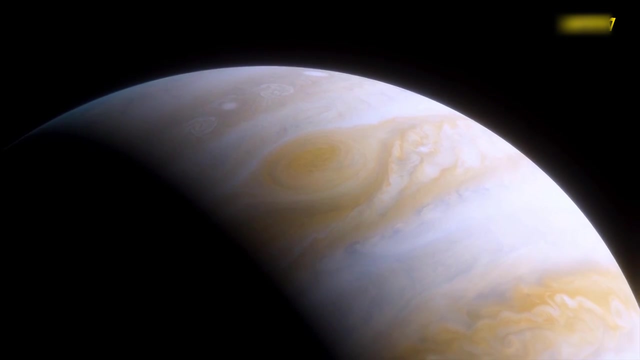 leading through space towards its final destination. Ahead of it, Comet Shoemaker-Levy 9 was entering its final few days in orbit around the planet, With the first impact expected on the 16th of July. the world's most powerful terrestrial telescopes were trained here. 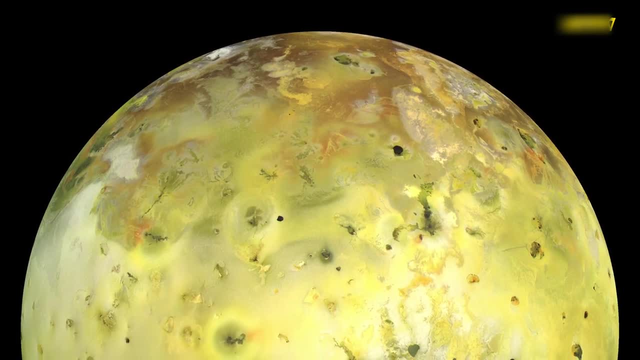 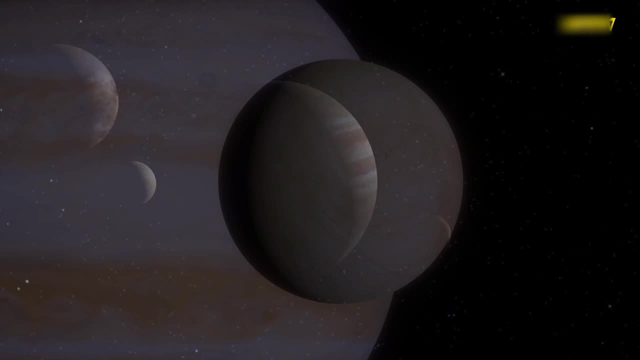 as well as some of our space observatories, from the newly fixed Hubble Space Telescope to the Ulysses spacecraft, which turned its gaze from its primary job of watching the Sun, Even the distant Voyager 2 probe, 6.6 billion kilometers away beyond Neptune. 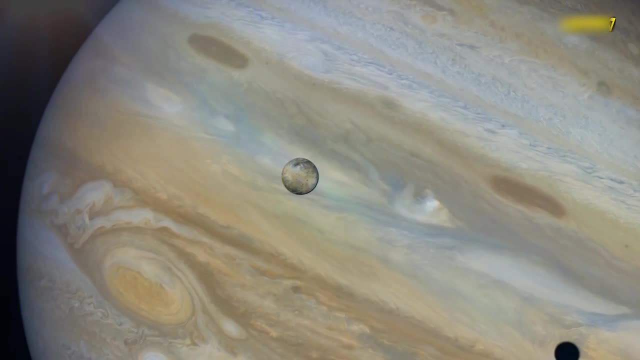 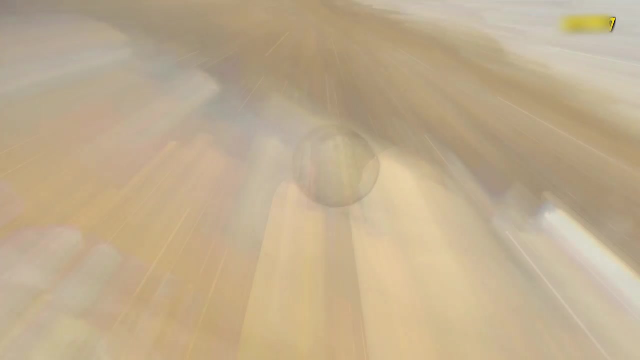 was able to look for radio wave emissions from the impact and employ its ultraviolet spectrometer to make distant observations. But for all of this technology peering across the solar system, there was only one set of eyes that would be able to see the actual first impact. 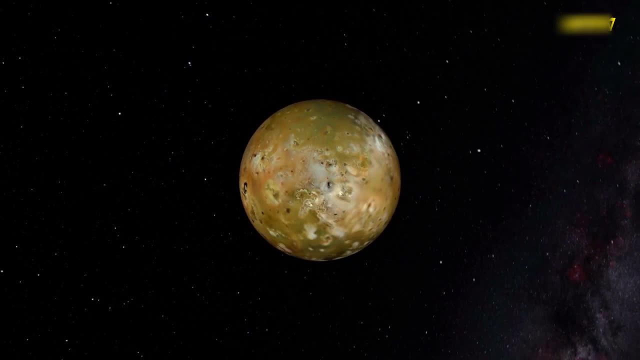 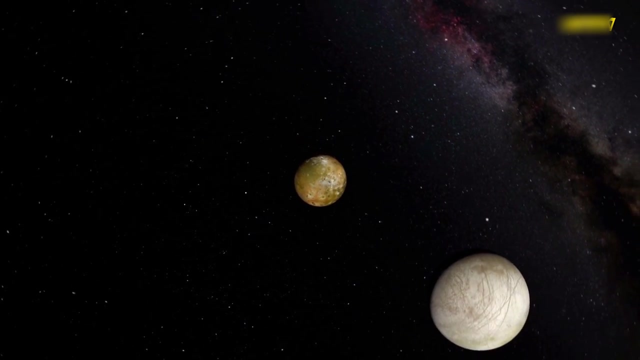 The comet would first hit Jupiter on the side, turned away from the Earth, but Galileo was approaching on the night side of the planet, which would give us a unique view, not visible from Earth, of our first ever observation of a collision between two objects in the solar system. 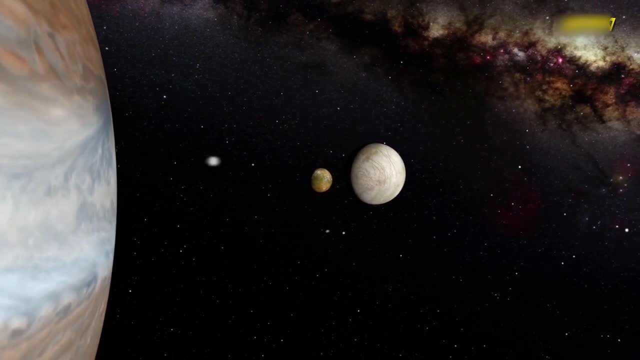 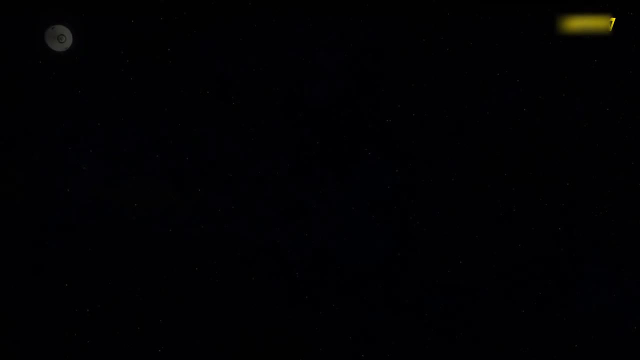 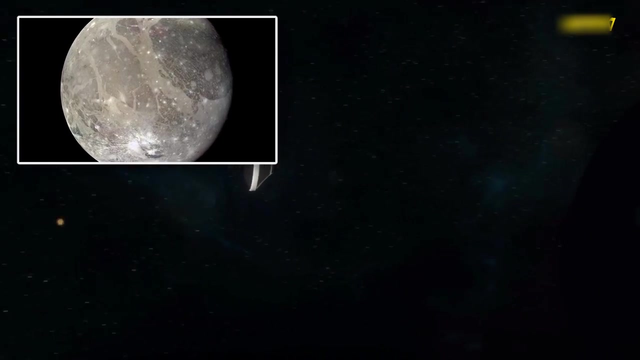 The first impact occurred at 2013 UTC, on the 16th of July, when fragment A entered Jupiter's southern hemisphere traveling at 60 kilometers. a second hitting the planet with an estimated force of 300 million atomic bombs, With its instruments trained on the impact. 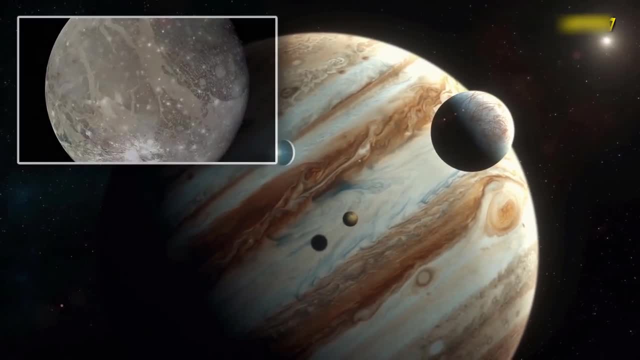 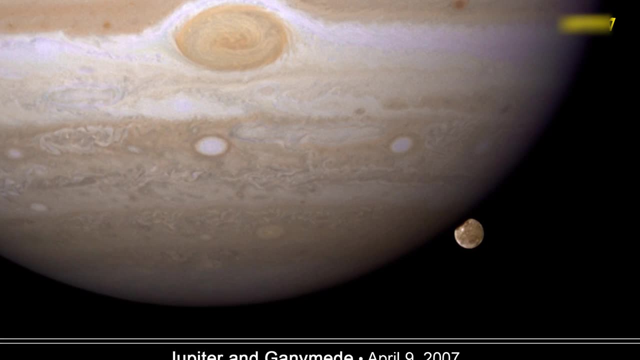 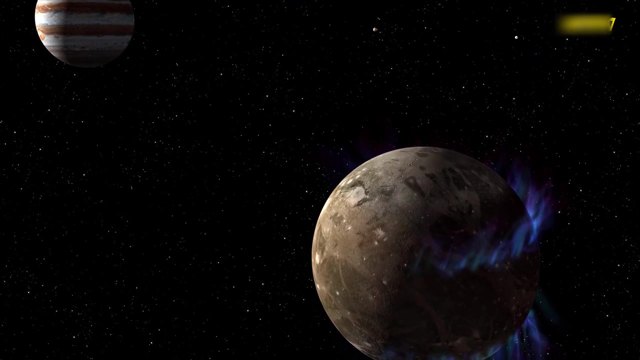 Galileo recorded the subsequent fireball, which reached temperatures of over 24,000 degrees Kelvin, creating huge plumes that stretched over 3,000 kilometers high. It was a breathtaking spectacle that quickly came into view from Earth, as the rapid rotation of Jupiter brought the impact. 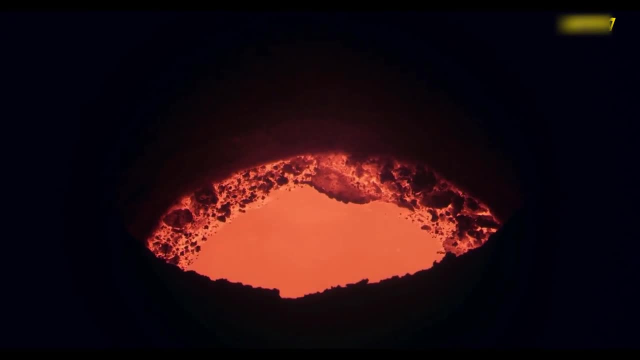 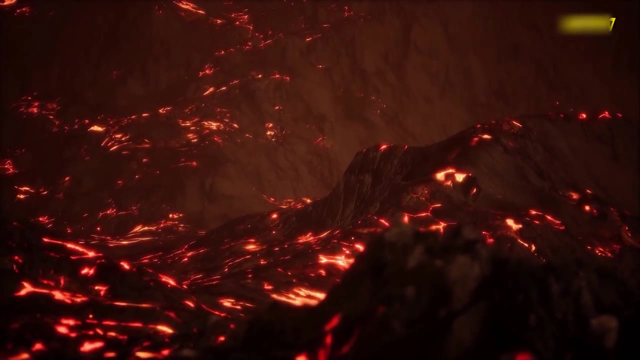 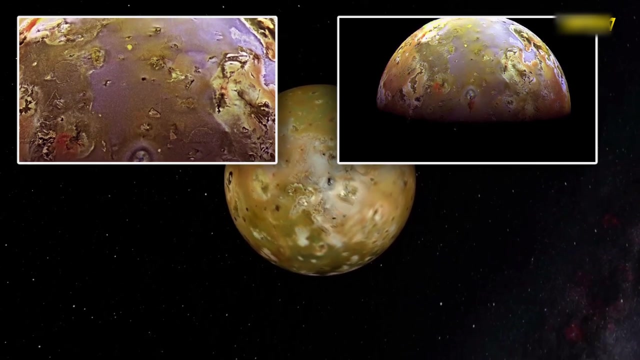 There's an unbroken chain of life stretching back 4 billion years here on this planet, But, having said that, there are major events that affected life, and one of them, without doubt, is the asteroid that wiped out the dinosaurs, And so, in that sense, it is true to say that without Jupiter, we wouldn't be here. 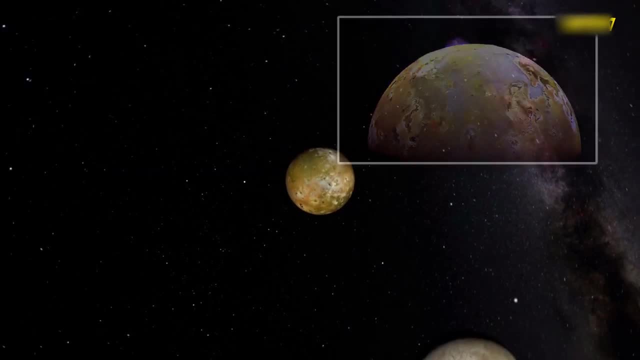 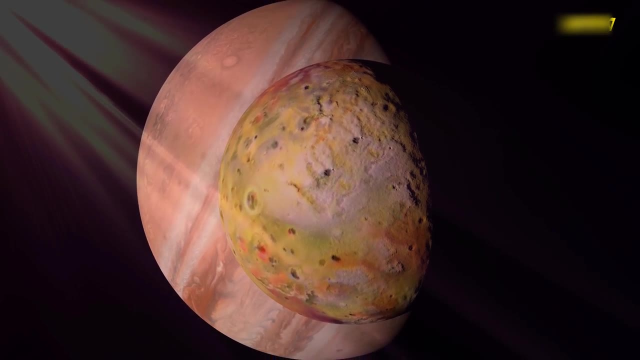 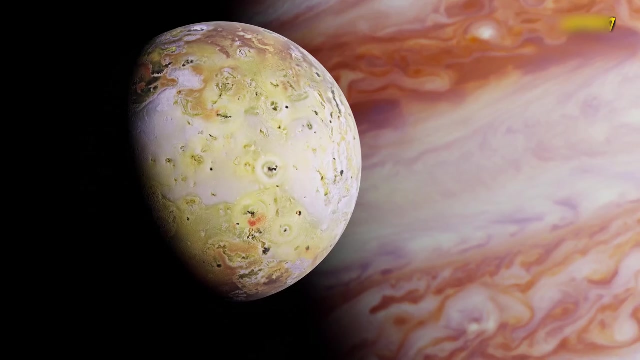 The godfather of the planets, paved the way for humankind to inherit the Earth, And it has looked down on us benevolently ever since, using its immense power to keep us safe. A sleeping giant with its power undiminished An asteroid impact like the one that cleared the way for us to evolve 65 million years ago. 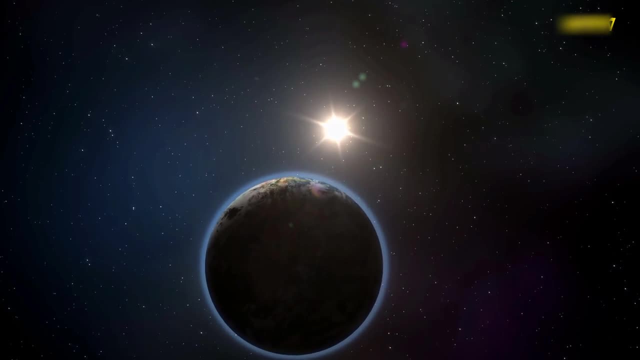 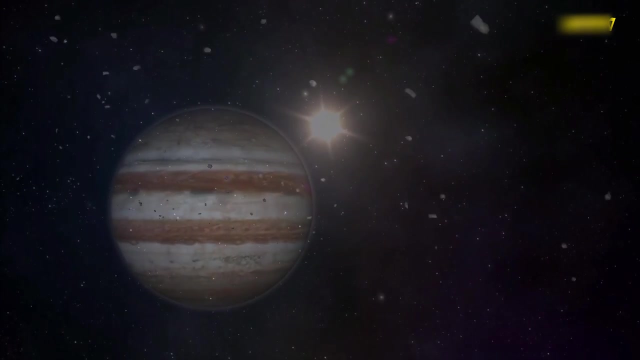 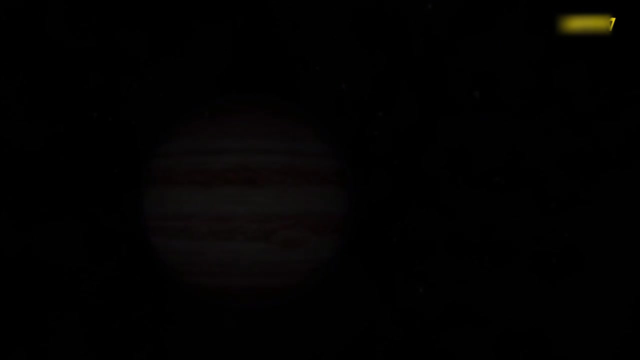 would have catastrophic consequences for our civilization, or something similar to strike today To the naked eye. Jupiter is one of the brightest points of light in the night sky And through a small telescope it is a beautiful banded world. It feels distant, eternal, disconnected from events here on Earth. 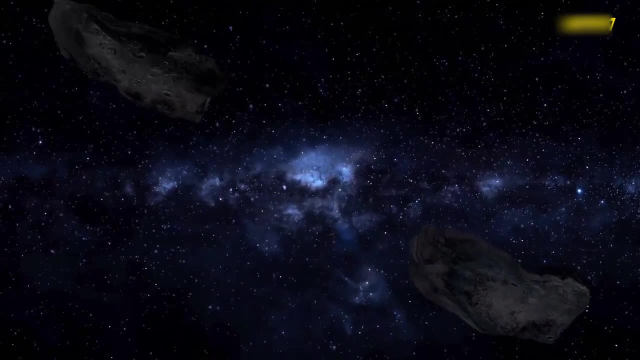 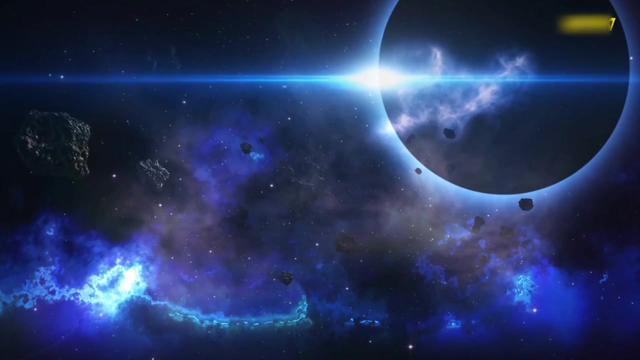 But the more we've learned about the history of the solar system, the more we've come to understand that that is not the case. Jupiter has played an important, and perhaps decisive, role in the stories of all the planets, including Earth. You see, the solar system is just that. 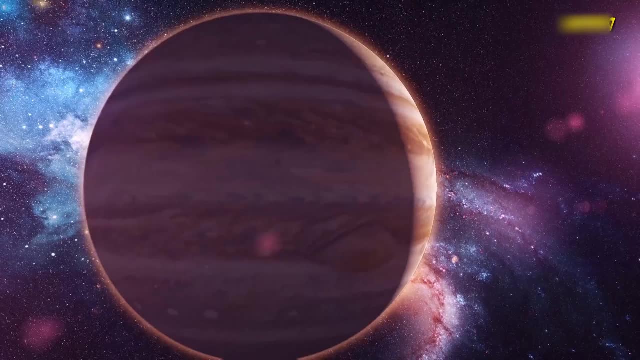 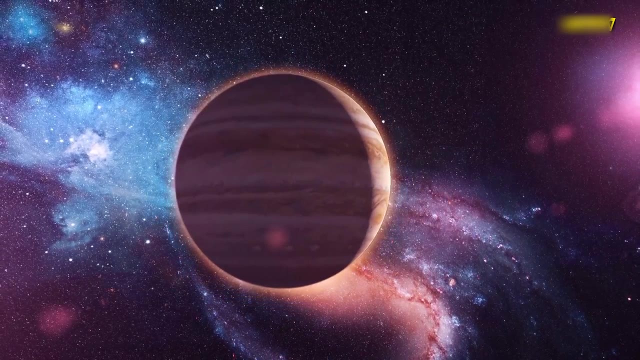 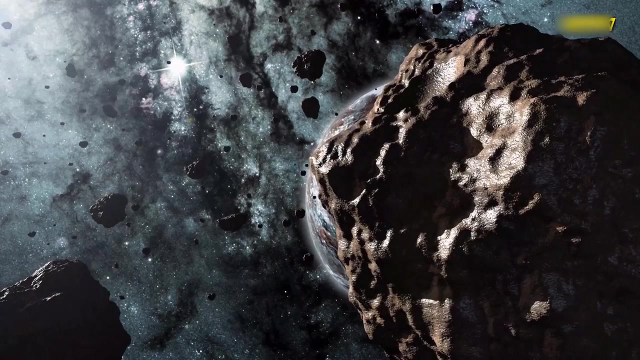 It's a system, Complex, interconnected and interdependent. So the next time you see Jupiter, just hold your gaze and think for a while about the fact that it is so much more than a point of light or a planet. even Jupiter is the great sculptor of the solar system. 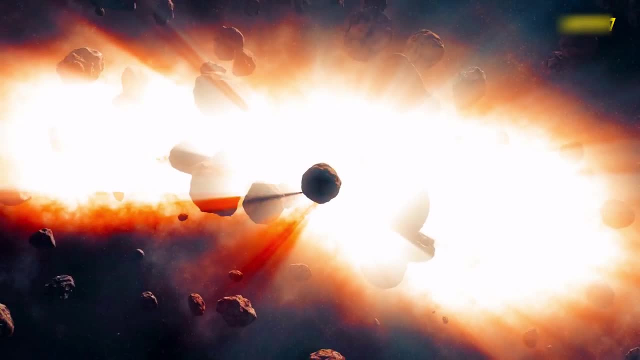 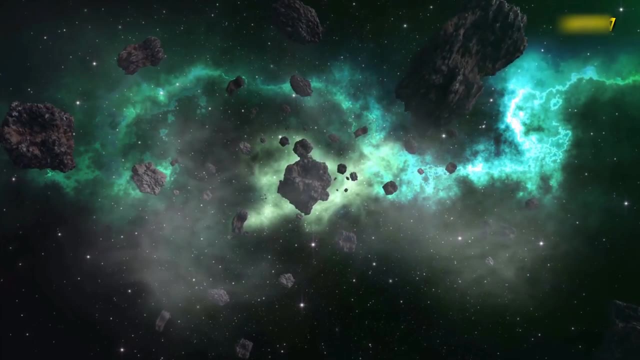 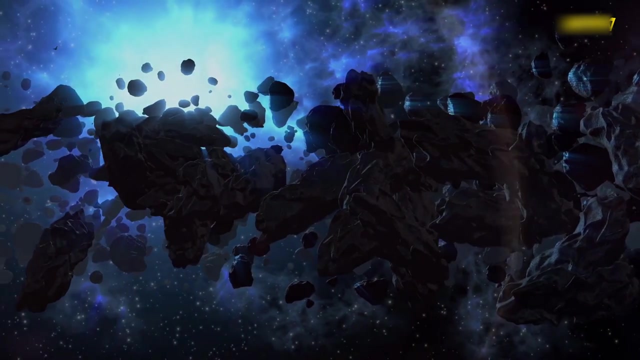 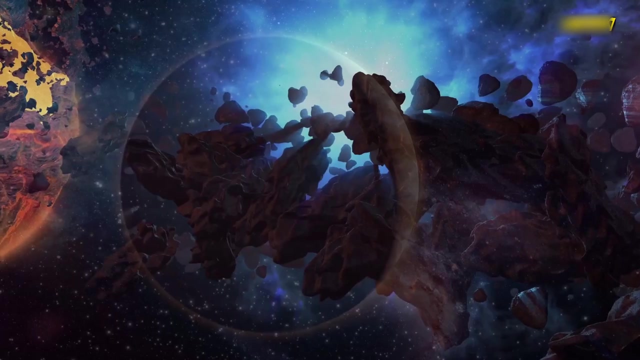 The destroyer and creator of worlds. Saturn is a gas giant alive with storms of unimaginable ferocity, A world of alien weather where diamonds rain down from the sky and bubbling vortexes whip around the planet so fast they catch up with their own tails. 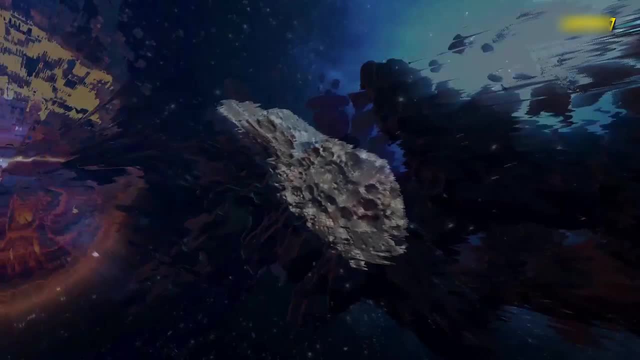 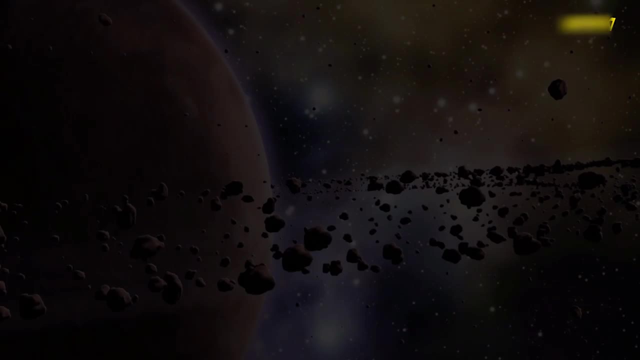 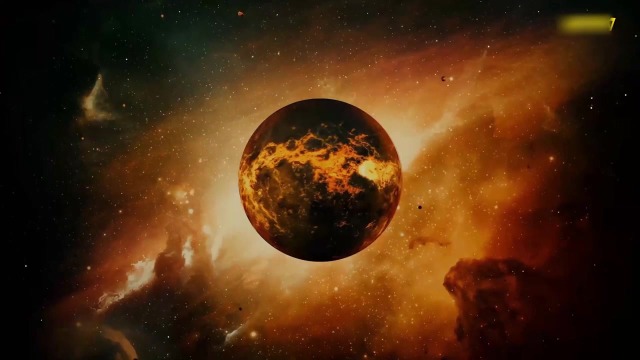 And glistening in the distant light of the sun, is a 500,000 mile ring of almost pure frozen water, broken into millions of individual pieces. This structure is unique in our solar system, sculpted by the delicate hand of gravity. Yet, for all of their iconic beauty, 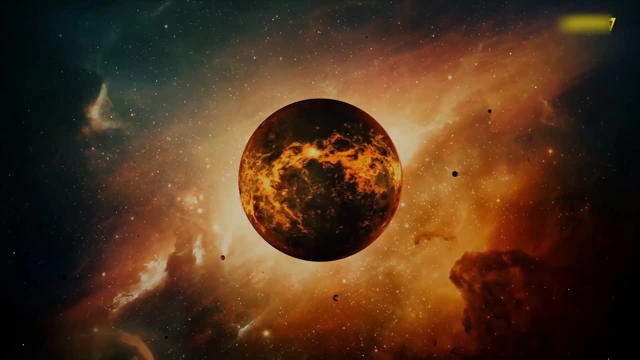 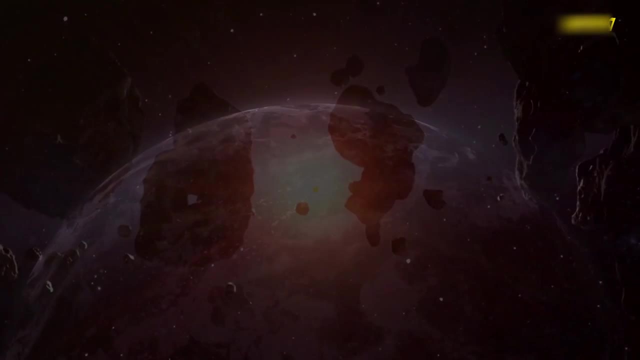 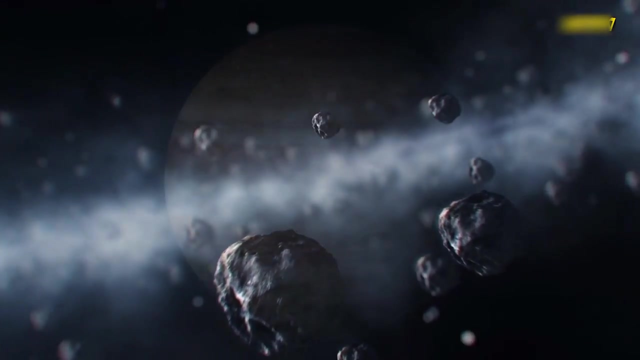 the rings are just a fleeting shadow, an echo of Saturn's past and an ephemeral structure that has adorned the planet for a brief moment in its history and will soon disappear again. Saturn is a place of many worlds, encircled by at least 62 moons. 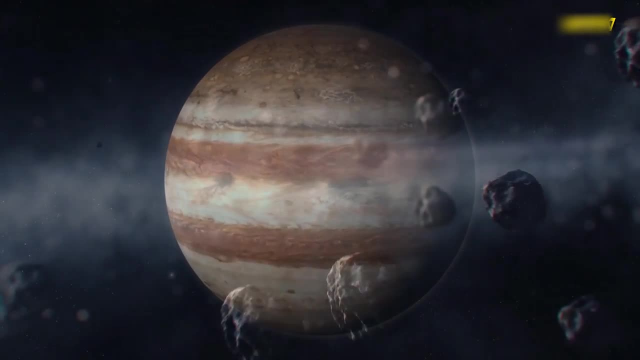 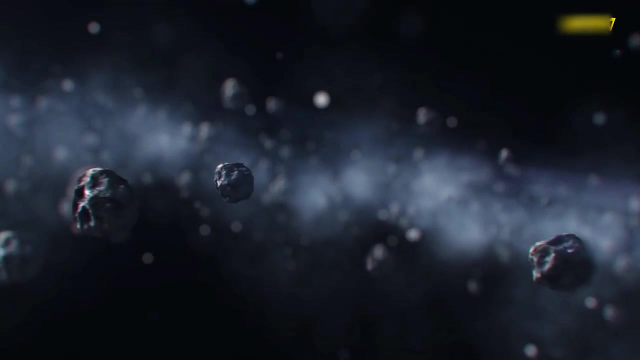 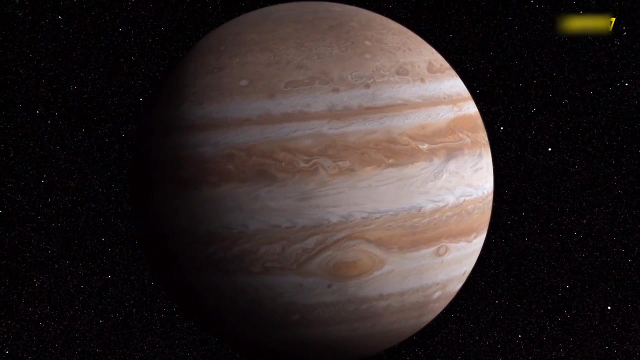 This menagerie of satellites boasts worlds of astonishing variety. Titan, bigger than the planet Mercury, is the only moon in the solar system to have its own substantial atmosphere, while Mimas is the smallest body in the solar system. Perhaps most astonishing of all, though, is Enceladus. 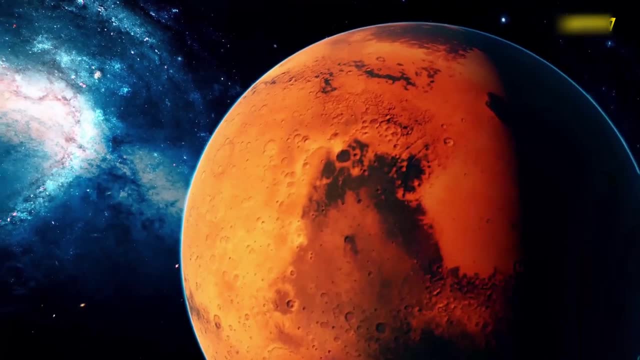 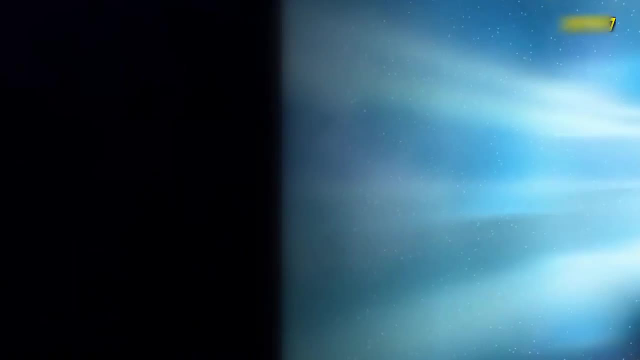 an ice moon with an ocean of liquid water inside that seems to contain all the building blocks of light. It is the only planet in the solar system to have an atmosphere of this size, composed of 96% hydrogen and 3% helium. Saturn has a diameter at its equator. 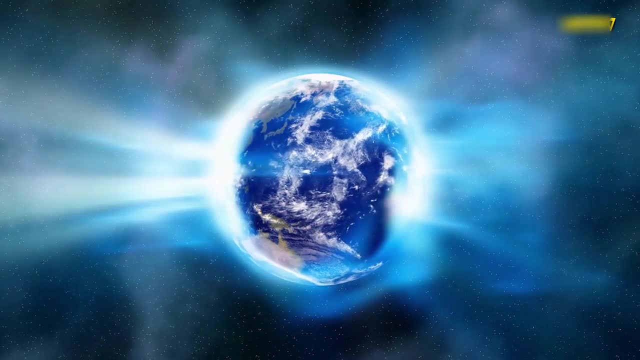 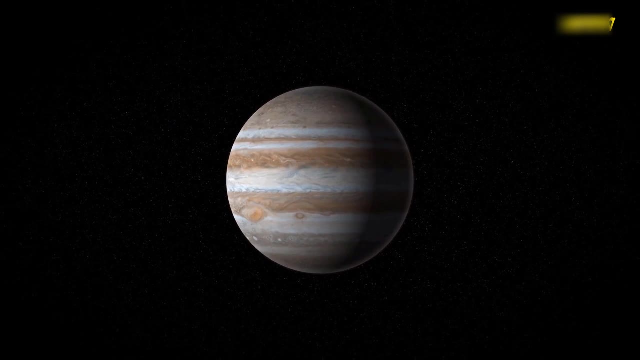 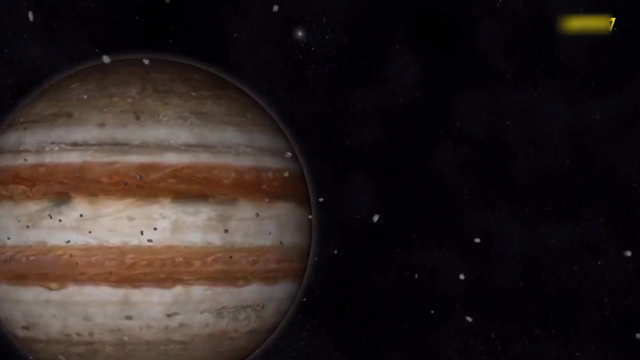 almost ten times the size of the Earth. at 120,536 kilometers, Its volume would hold 800 Earths. However, with a mass made up predominantly of gas, the planet's density is remarkably low, As the only planet in the solar system less dense than water. 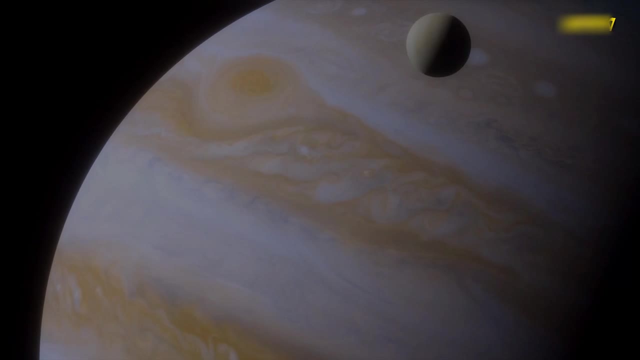 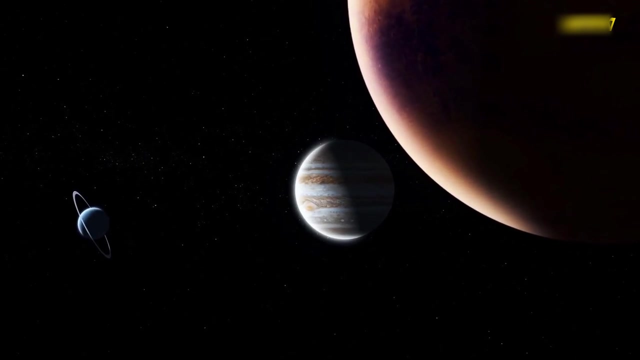 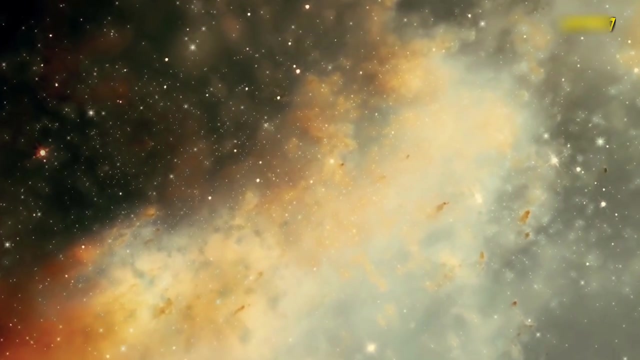 if you could find a bathtub big enough to hold it, Saturn would literally float in it. Beneath the frosty minus-178 degrees Celsius cloud tops, the pressure rapidly increases under the huge weight of Saturn's dense atmosphere, The hydrogen gas of the upper layers. 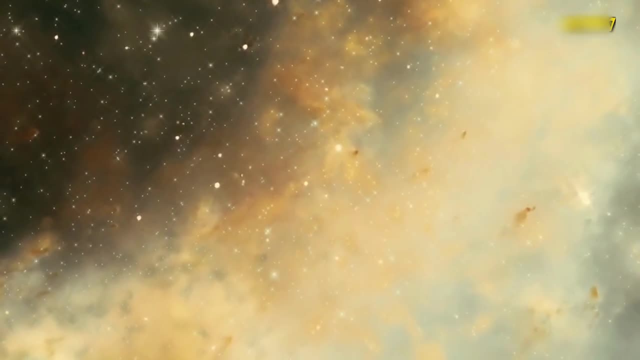 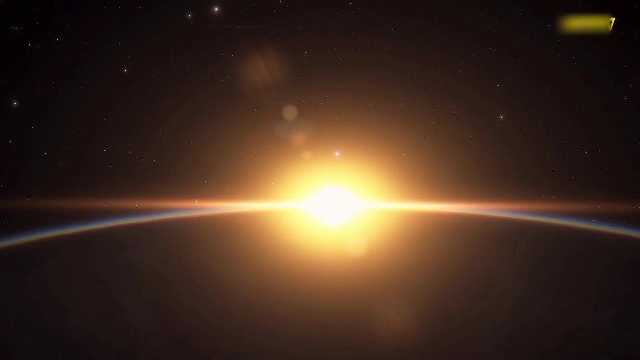 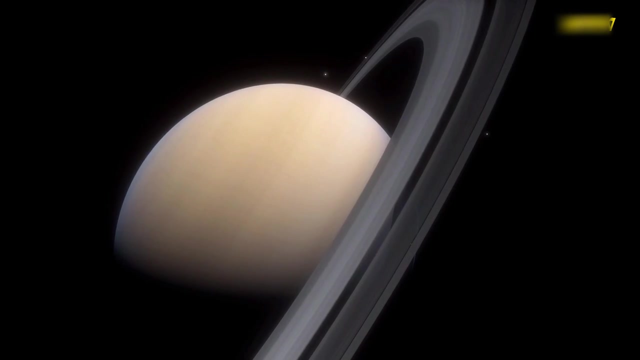 turns at first into liquid and then, hundreds of kilometers further below the planet's cloud tops, into slushy metallic oceans of hydrogen. We can only make an educated guess at the structures that lie within Saturn's unreachable core, With temperatures at its center exceeding 11,000 degrees Celsius. 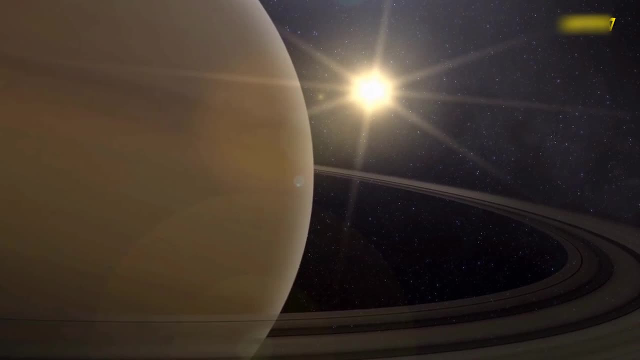 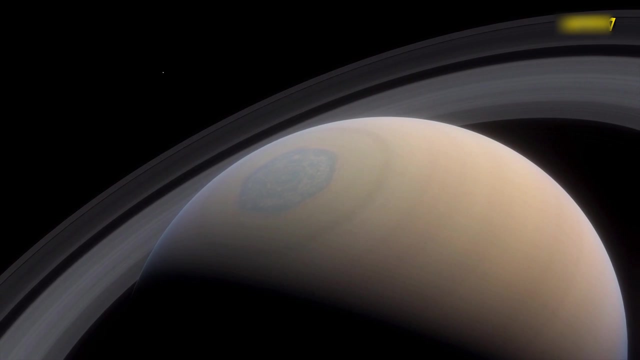 Saturn generates far more heat from within itself than it receives from a sun that sits, on average, 1.4 billion kilometers away, meaning that it must be generating its own heat. With such extreme temperatures and pressures, the structural makeup of this planet is uncertain. 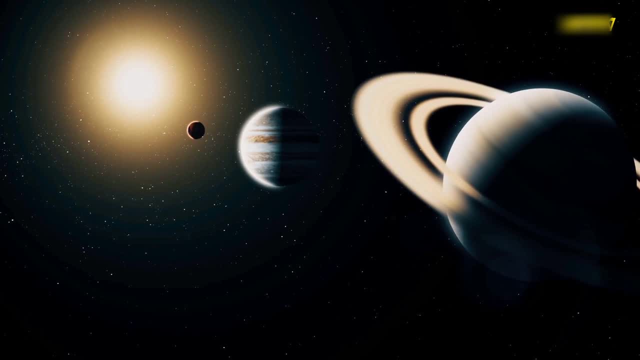 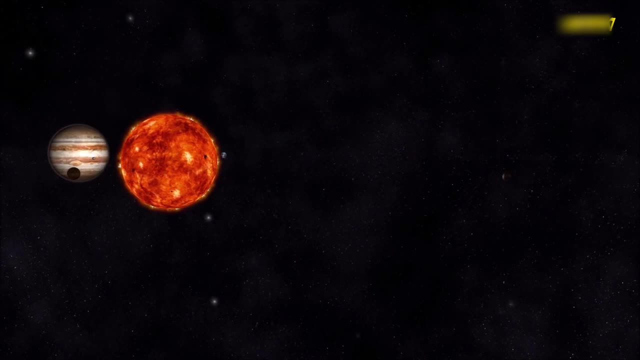 and hotly debated. According to planetary scientists and geophysicist Jonathan Lanine, if you go down, down, down, through the hydrogen, through the helium rain, to this core of rocky and icy material, it's not rock and ice. 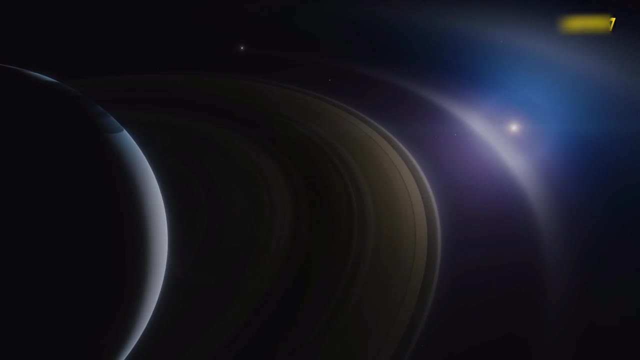 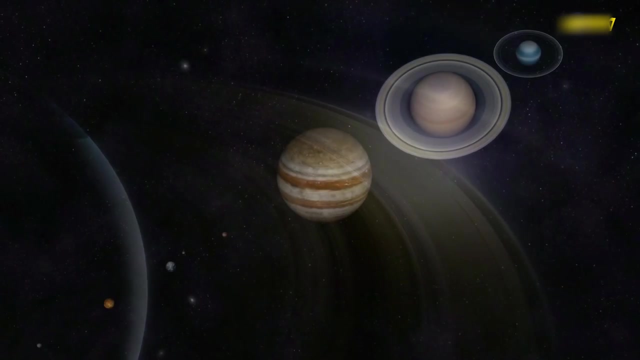 It's some sort of atomic crystal where the elements of rocks and ice, the silicon, the oxygen, the magnesium are all together in a structure that doesn't exist in the rocks on the Earth. Now, in the case of Jupiter, it might actually be warm enough. 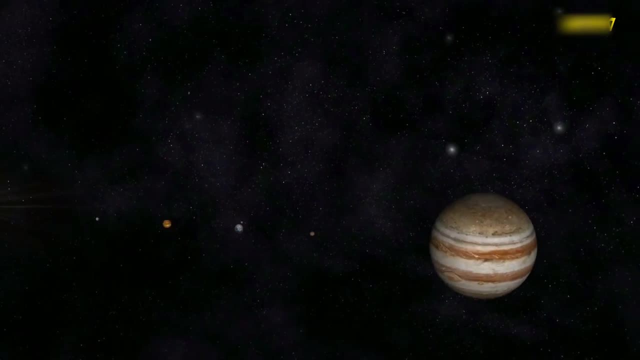 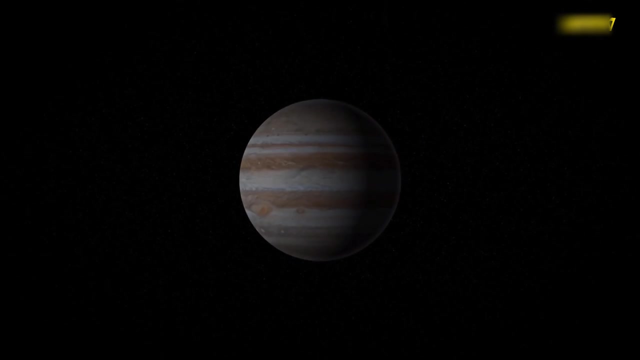 that the core is a liquid, that it's molten, But in the case of Saturn, it's probably a solid core, but definitely an exotic one. Undoubtedly, there is a dense core at the heart of Saturn, one that is almost certainly composed of iron-nickel alloy. 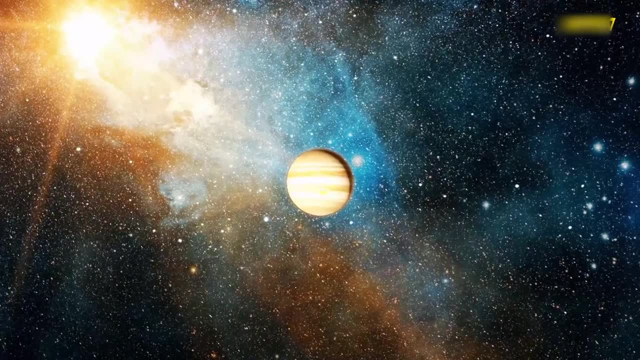 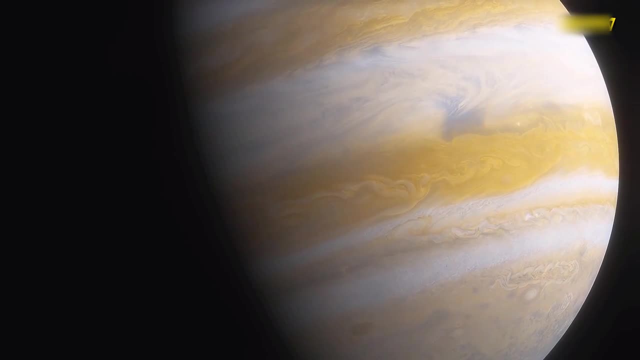 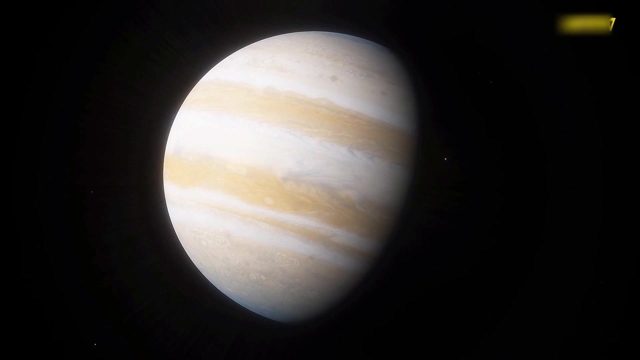 and rocky silicon-based compounds. But exactly how this material behaves at such extremes remains a mystery. From its surface all the way down to its center, Saturn is a world of mystery. This gas giant, along with its sister planet Jupiter, is worlds apart in character. 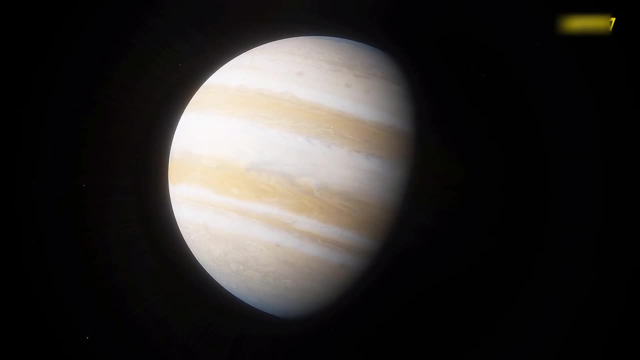 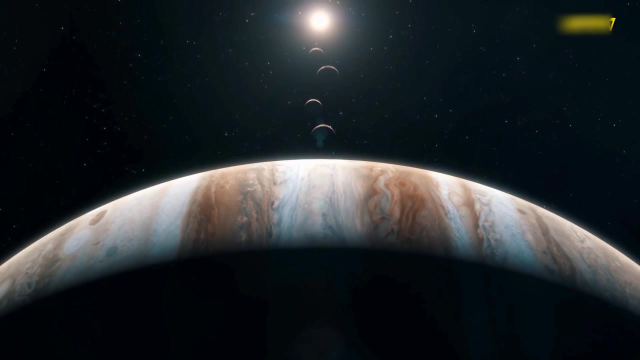 from Mercury, Venus, Earth and Mars, the terrestrial planets of the inner solar system. It's hard to imagine how they could all have been created from the same ingredients, the singular cloud of gas and dust that gave birth to every planet in our solar system. 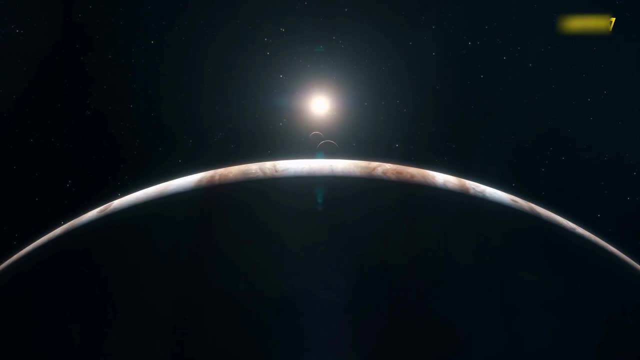 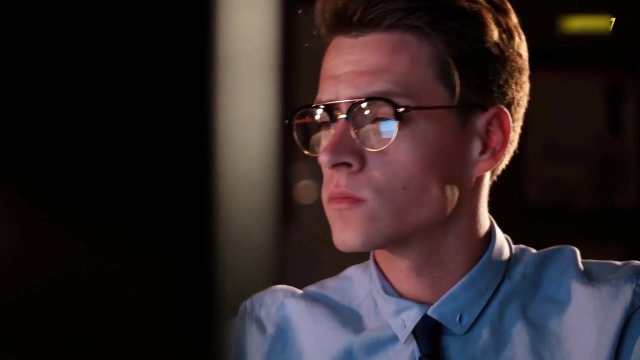 But if we go back far enough in time, we begin to uncover a history with a surprisingly familiar origin. The beginning of Saturn's story is far more recognizable than its present-day character would suggest, because at the heart of all the ringed planets' beauty. 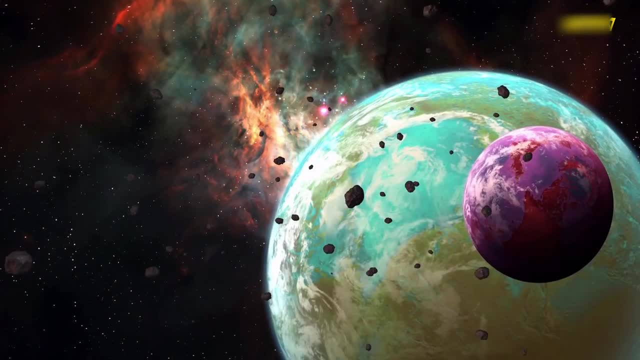 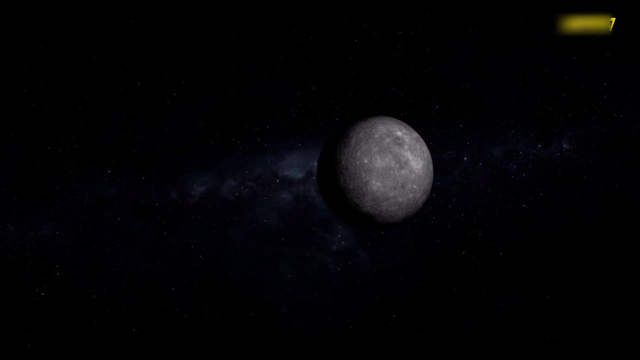 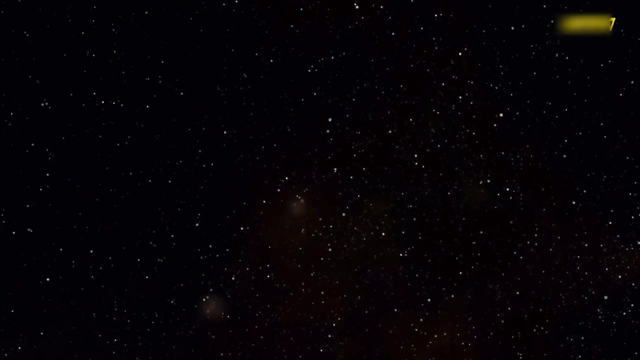 lies a lost world, a primordial one that disappeared from view billions of years ago and yet was the seed for everything that Saturn was to become. Without this early world, there would have been no gas giant, no rings of ice and no hope of an orbiting oasis of life. in the far distant reaches of our solar system. The story of Saturn, like that of all the planets, began around 4.5 billion years ago In the light of the awakening sun. a vast cloud of gas and dust swirled around our newly formed star. 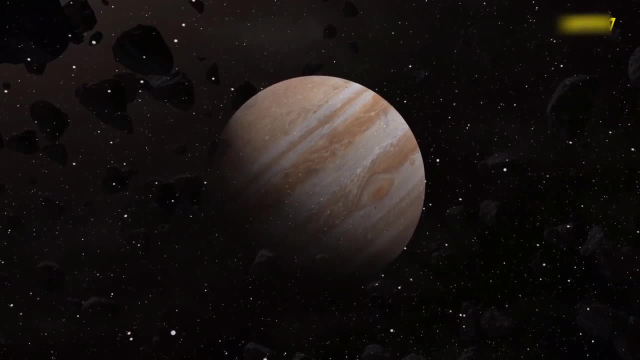 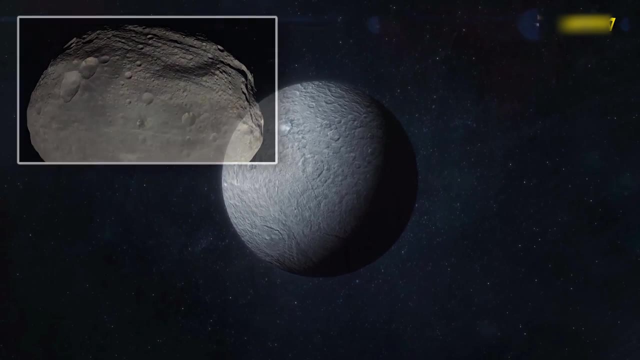 and that protoplanetary disk of gas and dust clumped and coalesced until it slowly began to form into a collection of embryonic worlds that would go on to become the four rocky planets sitting closest to the sun, Millions of kilometers further out. 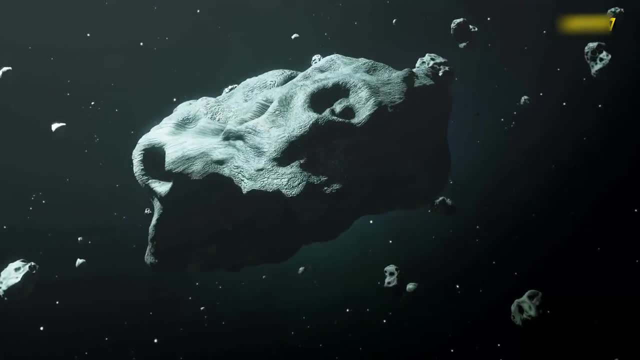 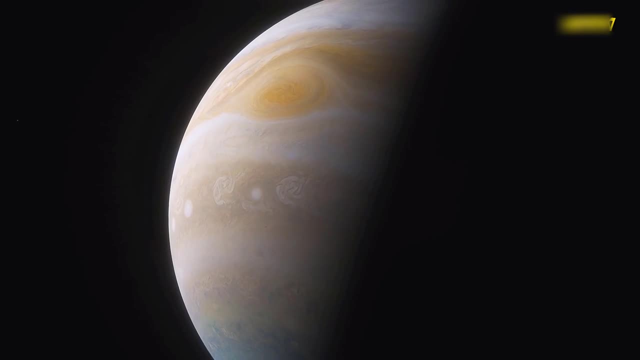 in the cold, distant reaches of the solar system, a similar story was playing out, but this tale of planetary formation would follow a very different path. That's because Saturn was molded beyond a boundary called the ice line, sometimes also called the snow line. 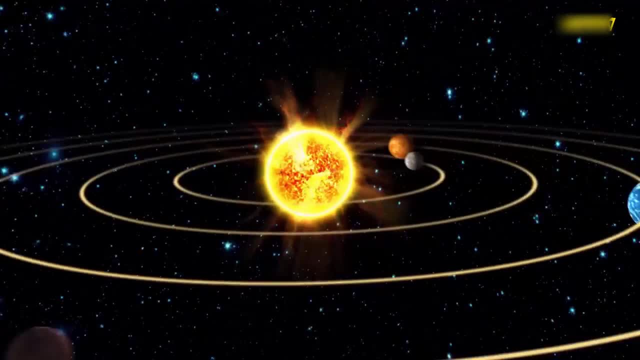 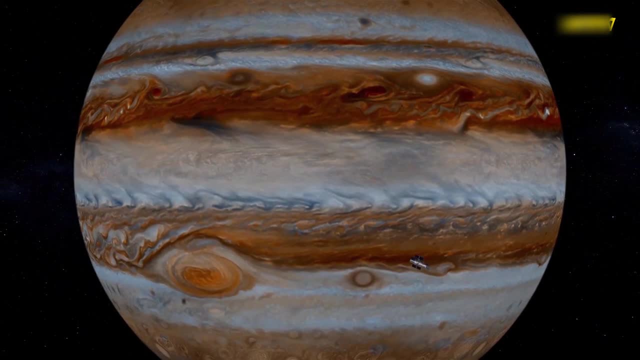 which is a frontier that marks the divide between the terrestrial planets and the gas giants. Respective proximity to this line would lead the evolution of Saturn and that of its neighboring planet Jupiter to play out in the future The ice line, as you might expect from the name. 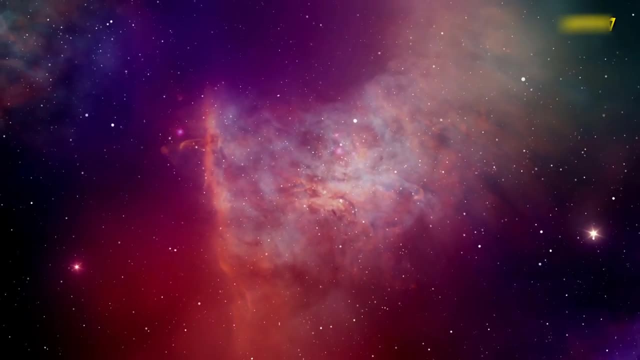 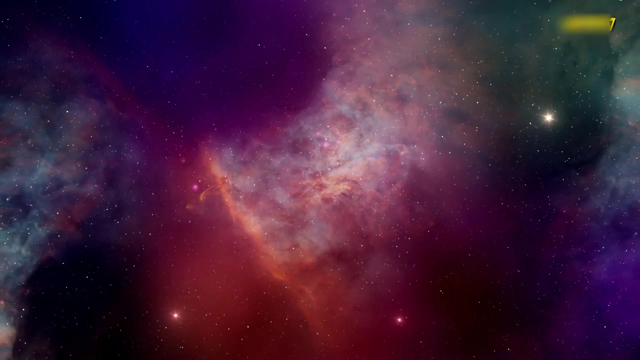 is a way of dividing a solar system into two broad zones based on temperature. Inside the ice line, the strength of a star is strong enough to keep things pretty warm, But step onto the other side of the line and you've crossed a boundary. 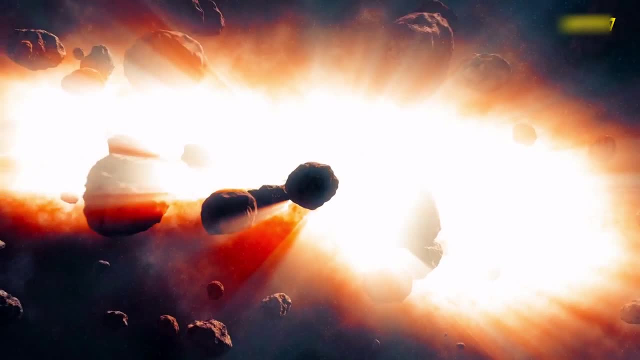 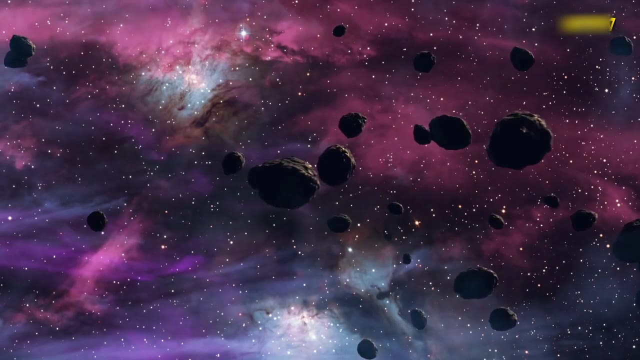 where it becomes cold enough for volatile compounds like water, methane, ammonia and carbon dioxide to condense and freeze solid. Each of these compounds has its own temperature and temperature. Each of these compounds does, of course, have its own precise ice line. 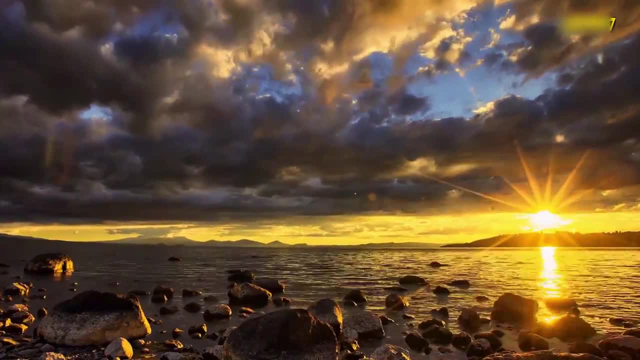 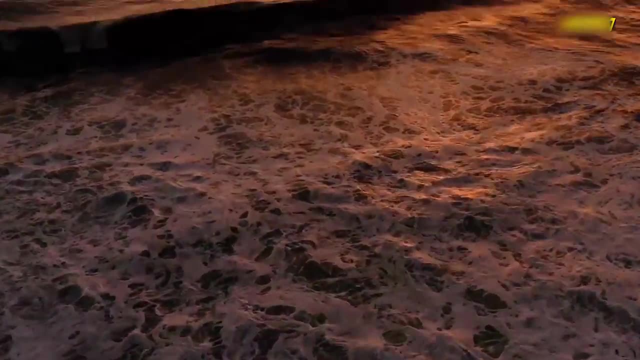 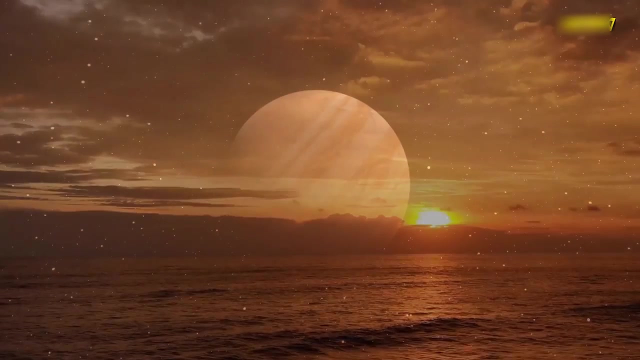 due to the different specific freezing points of each individual compound. But beyond a certain point, the boundary begins to incorporate the freezing points of a large number of compounds. Today, the ice line is thought to be around 5 AU, That's around 750 million kilometers from the Sun. 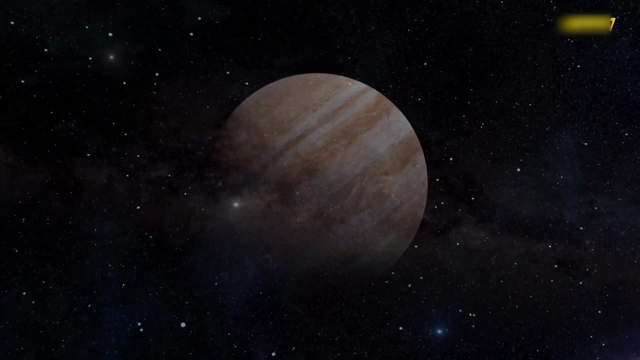 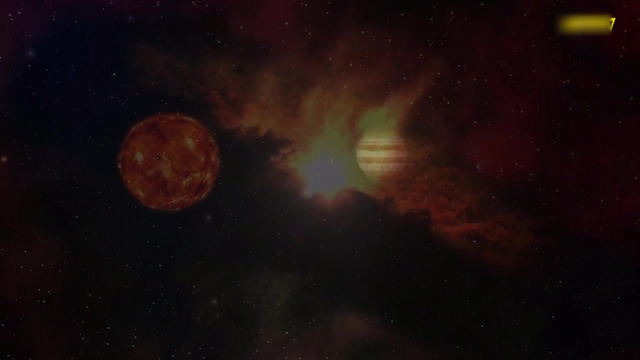 which means it lies well beyond the asteroid belt, at a distance just before the orbit of Jupiter. But in the infant days of the solar system that distance would have been much less, With a weak young Sun shrouded in an opaque cloud of dust and gas. 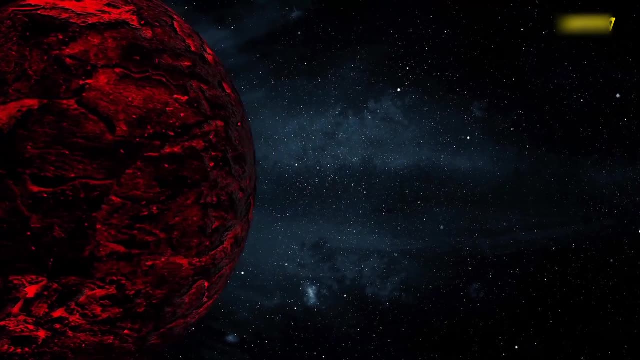 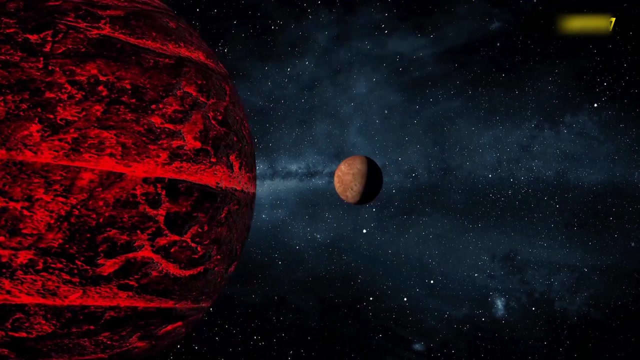 the early ice line would have fallen about 2.7 AU from the Sun, smack bang in the middle of where we find the asteroid belt today. We know this because we've been able to explore the makeup of the asteroids on either side of this line. 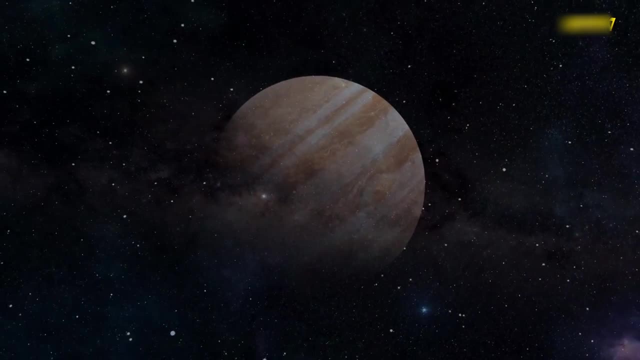 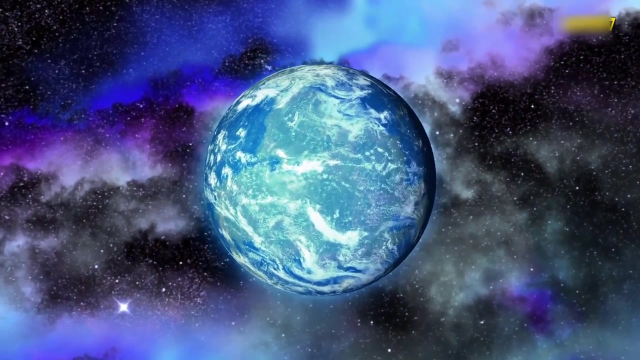 Beyond the 2.7 AU line, we've discovered the asteroids to be icy objects with large amounts of water ice locked away within them, While on the inside of this line we find a very different class of asteroid, dry and largely devoid of water. 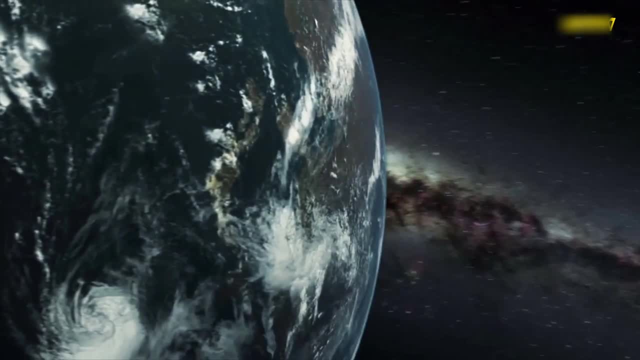 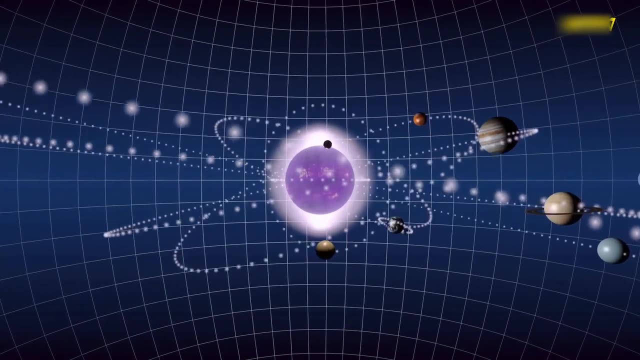 It seems these bodies formed in a region of space that was simply too warm to allow substantial amounts of ice to exist. Why does the ice line matter in the story of Saturn's evolution In the early solar system, as the protoplanetary disk swirled around the young Sun? 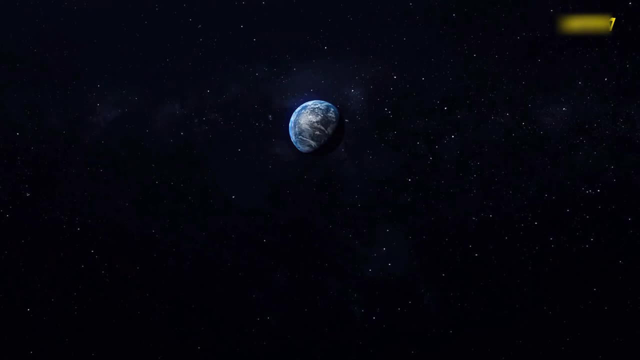 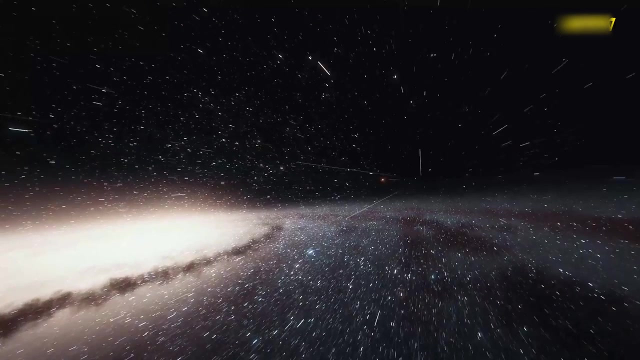 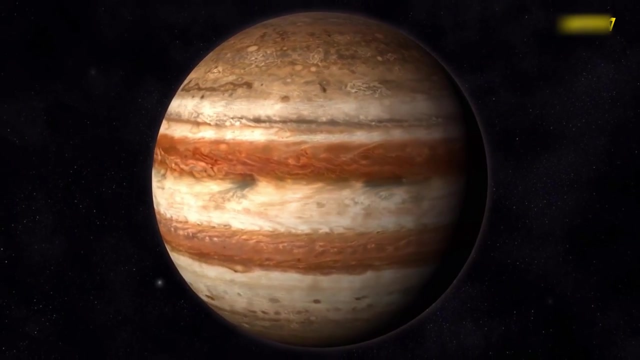 the ice line moved not only defined an important boundary in terms of temperature, but it also created a dramatic difference in the abundance of material available to build a planet on either side of the line. Beyond the ice line, the lower temperatures meant that all of those frozen volatile compounds 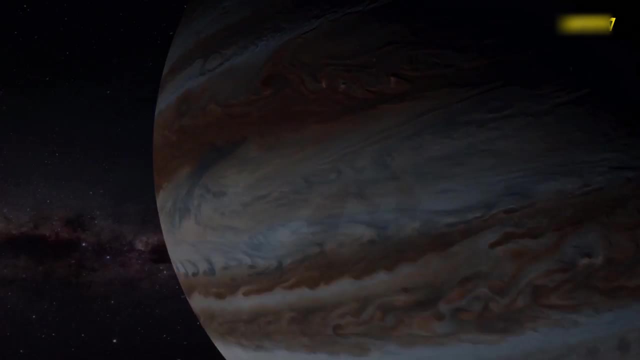 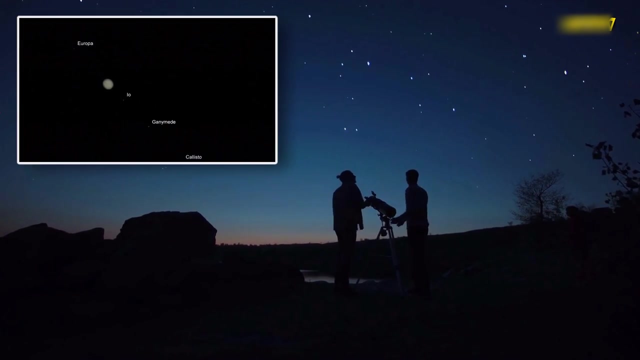 were swirling around in the cloud of gas as solid grains, building blocks that provided vast amounts of additional material to feed into the process of planetary accretion, And the impact of this simple physical difference was profound On our side of the line. 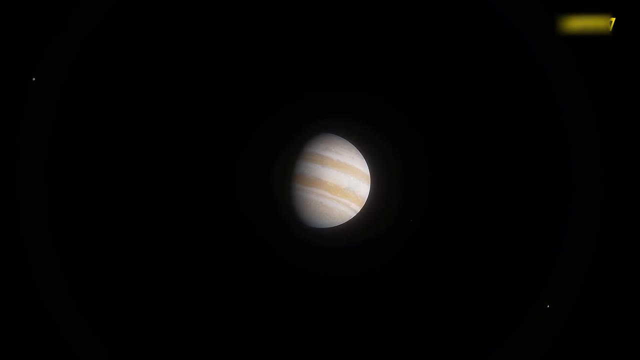 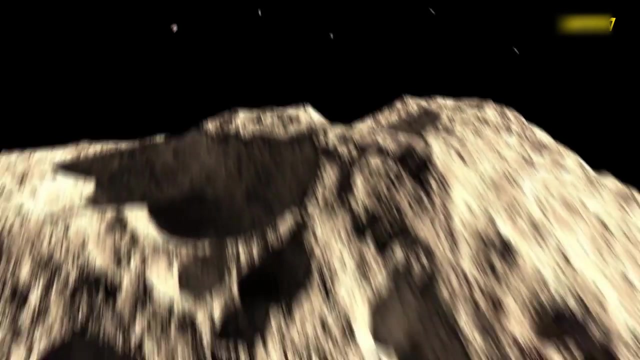 we find only rocky planets like Earth, Venus and Mars, while on the other side of the line there is not a single planet that we recognise as terrestrial, just the gas giants of Saturn and Jupiter and the ice giants of Uranus and Neptune. beyond, 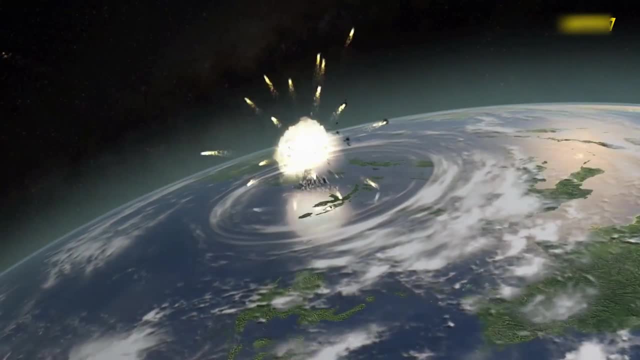 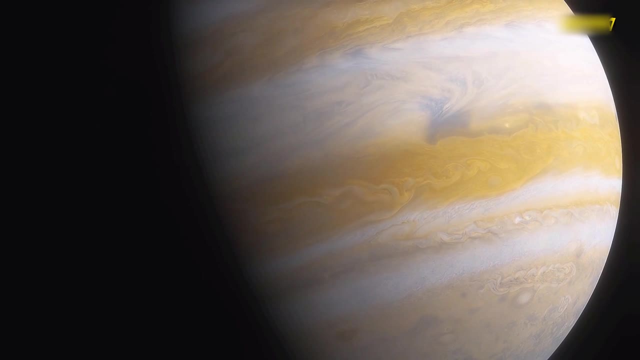 To understand the reason for this stark delineation, we need to look back to a critical time in Saturn's history, to the moment where the paths of the planets either side of this ice line began to diverge. Saturn began its life not as a beautiful jewel. but as a tiny, ugly ragged world, Just like its terrestrial cousins. the origins of this gas giant planet began with the clumping together of tiny specks of gas and dust that slowly grew into bigger and bigger clusters As this embryonic new world tumbled wildly through space. 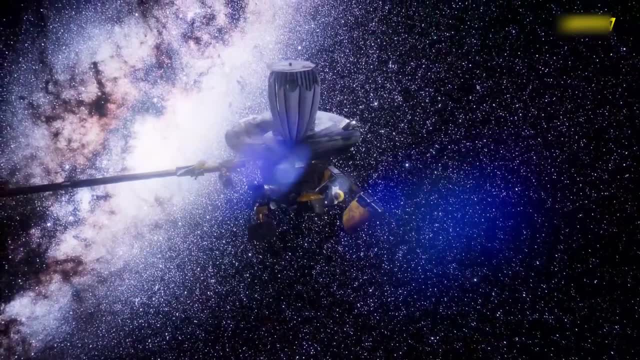 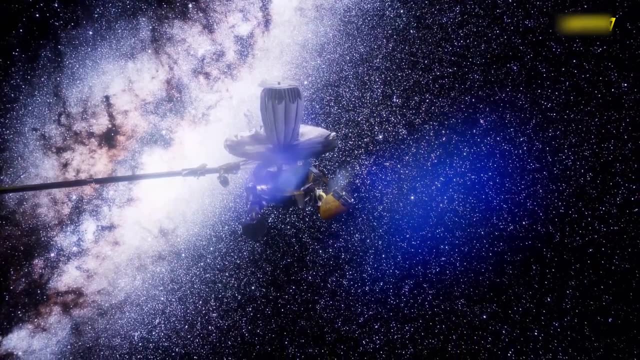 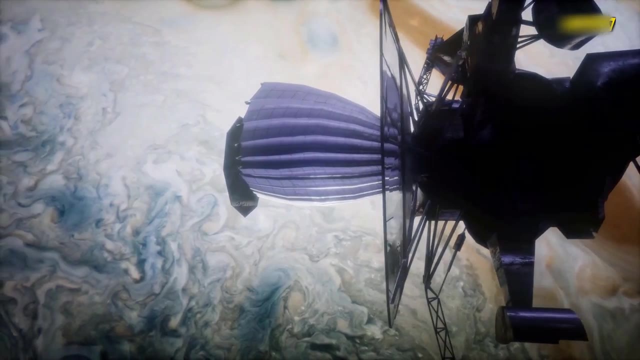 days would have lasted minutes as the distant sun lit its twisted surface, rising and falling in chaotic rhythm repeatedly. Eventually, as it grew, this ragged rock began to transform itself, taking the new shape of a spherical world as it went from planetesimal to protoplanet. 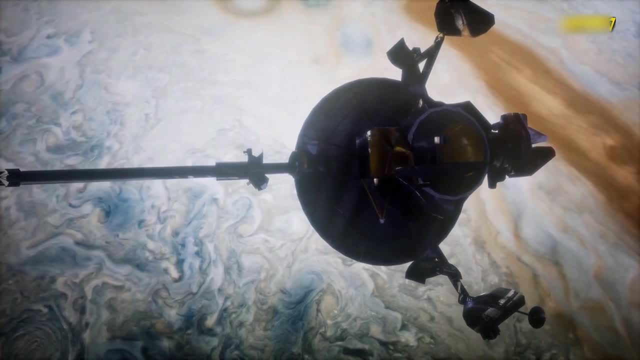 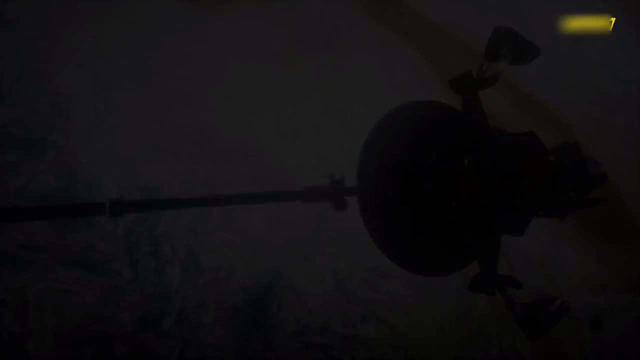 On the warm side of the ice line. the growth of the terrestrial planets came to an abrupt halt. As these planets had secured stable orbits and began clearing their way through the protoplanetary disk, the supply of raw ingredients ran dry, and so their growth simply stopped. 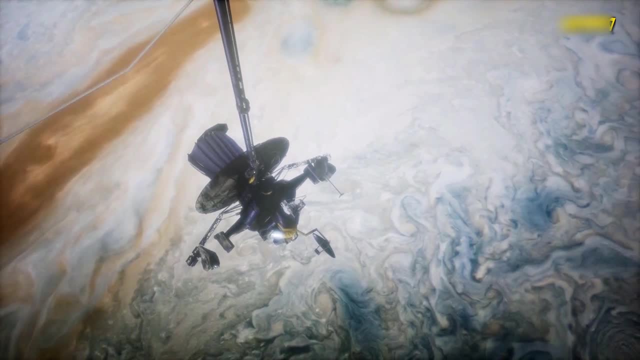 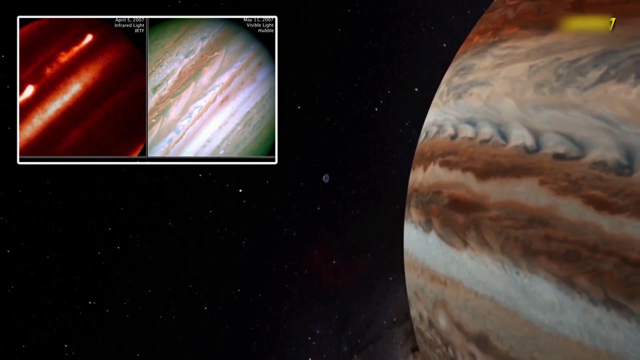 starting with the runt of the litter, Mars, followed by Venus and then our planet Earth, the largest of the rocky planets. But on the other side of the ice line it was a very different story, With no shortage of building material. 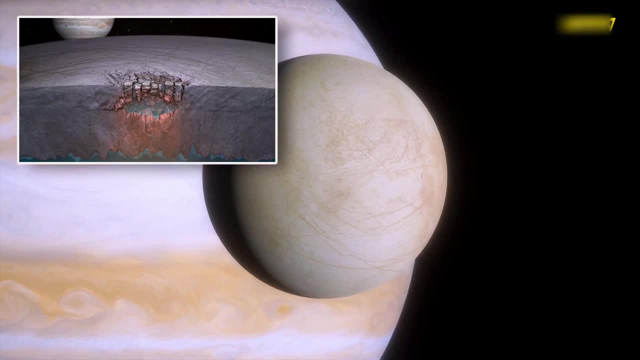 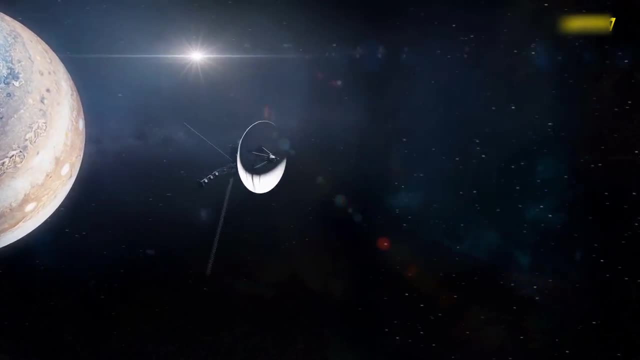 the growth of the protoplanetary Saturn was able to progress at a rapid rate, With abundant amounts of rock and ice. the young Saturn continued to grow quickly, dwarfing any of the terrestrial planets that were forming in the far distant glow of the warming Sun. 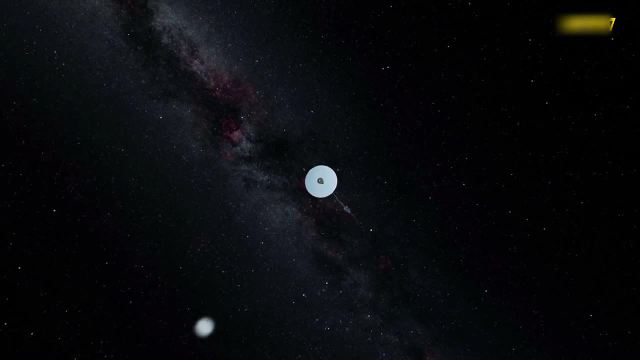 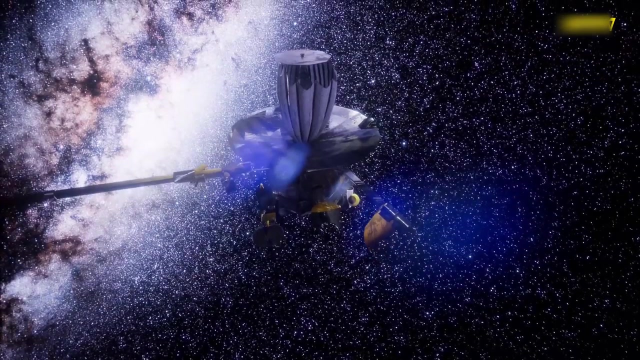 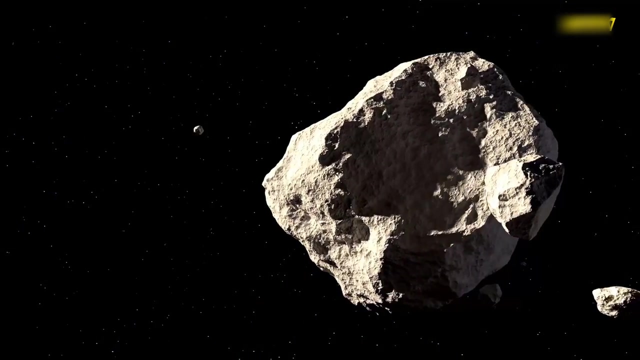 Over a relatively short period of hundreds of thousands of years, this plentiful supply of material smashed and clumped and grew until, through a series of planetary-scale collisions, Saturn became the largest object for millions of miles in any direction. The bigger it got, the stronger its gravitational field grew. 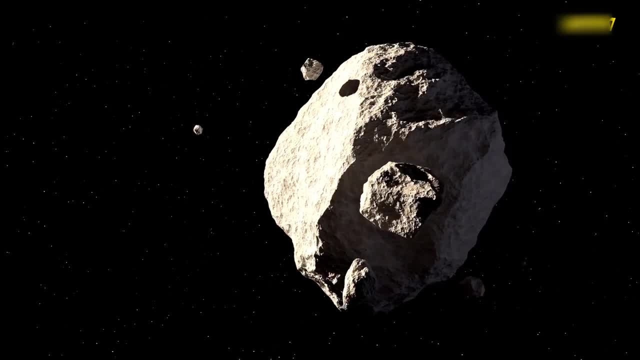 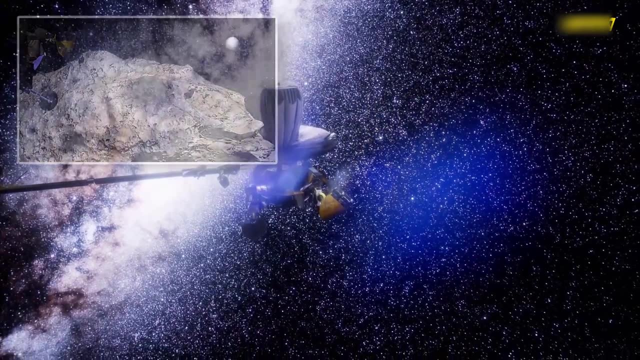 and so it could attract ever more material into its grasp. Eventually, the violence of its early life allowed Saturn to grow into one of the biggest worlds of rock and ice the solar system had ever seen. What did this world look like? We simply do not know. 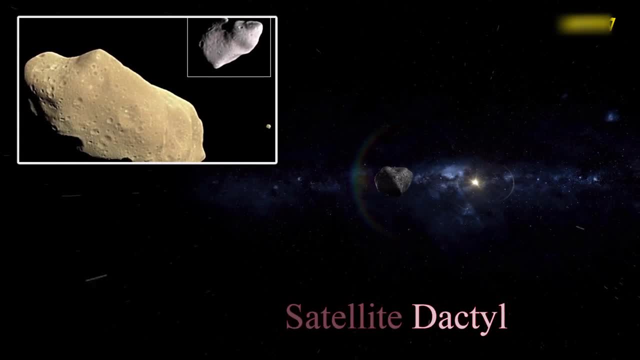 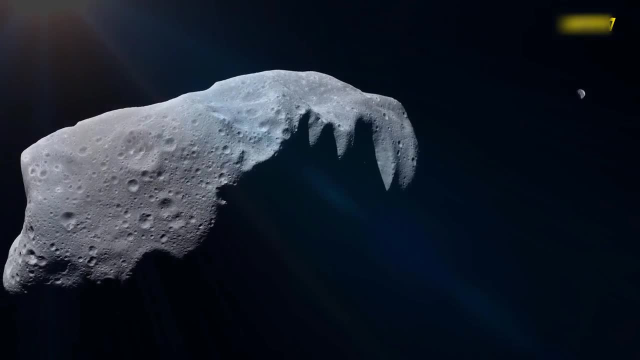 The detail of how any of the planets formed in the solar system is only sparingly understood. These are events that happened 4.5 billion years ago and it's very much still cutting-edge scientific research trying to piece together the barest of timelines. 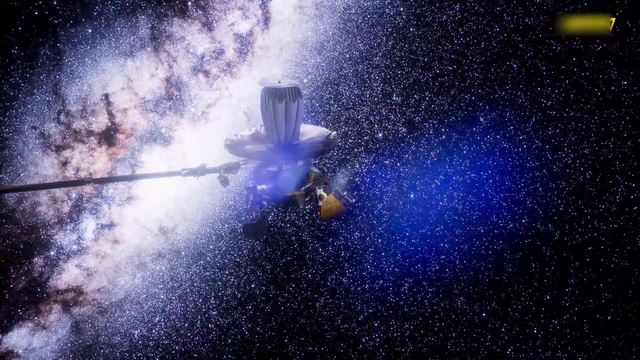 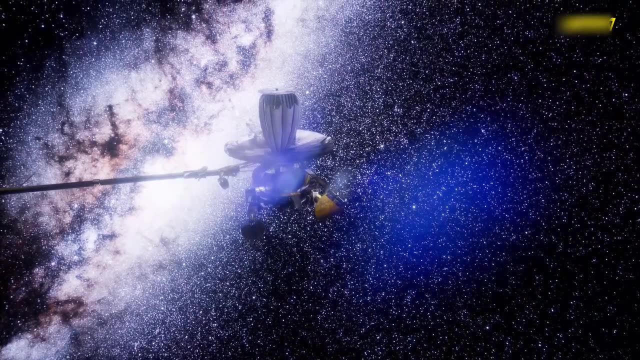 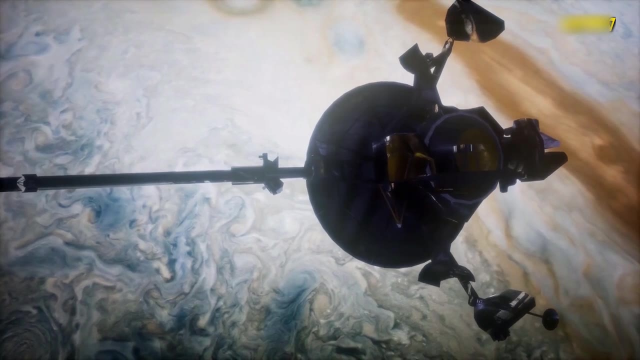 let alone the intricate details of these distant events. Much of what we do understand of the evolution of our own solar system and the planets within it has been supported by our recent ability to study worlds outside it, in neighbouring systems. The study of exoplanets has allowed us for the first time. 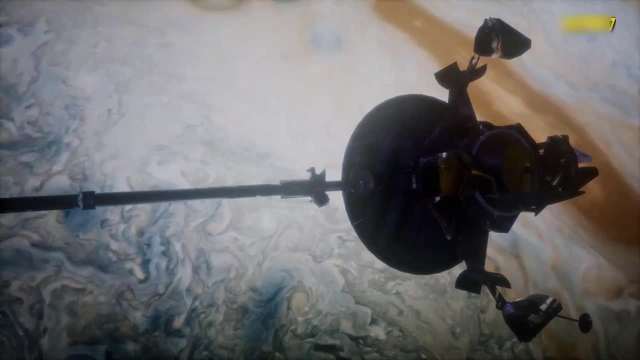 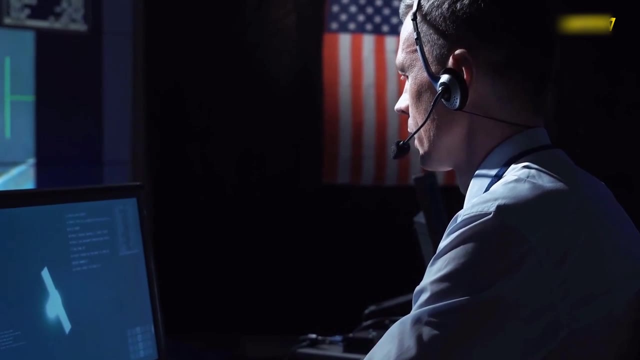 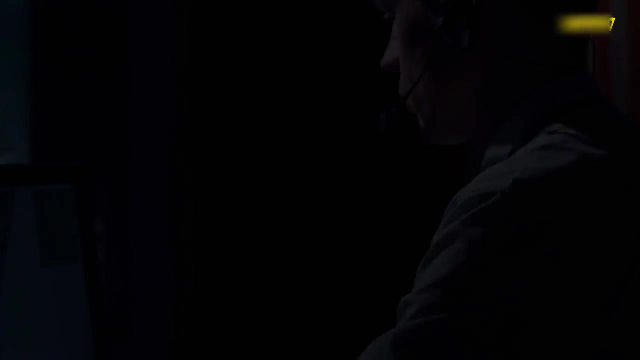 to peer into the evolution of other star systems and witness the formation of hundreds of different planets, rather than the eight in our own backyard. Much of this evidence supports the idea that Saturn was once a world of rock and ice, a world that grew to perhaps 10 or even 20 times the mass of the Earth. 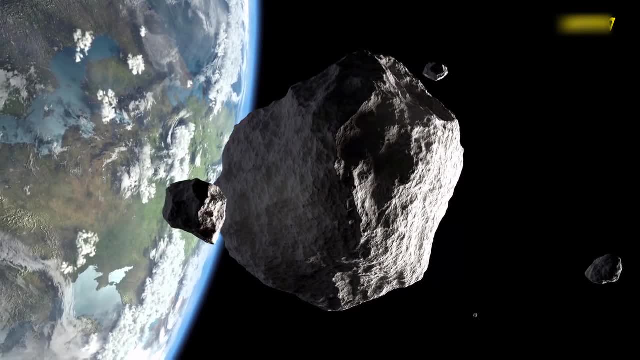 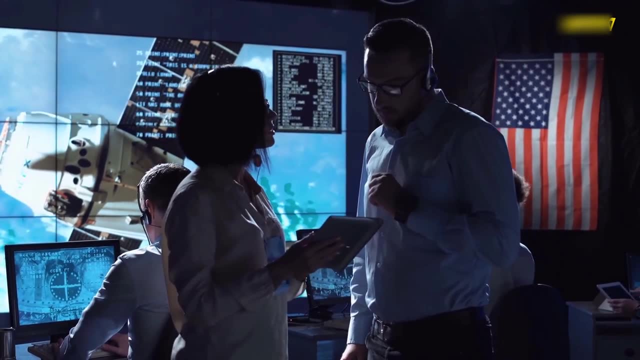 as it gorged itself on the available matter. This was a world we would at least have vaguely recognised a place. it is almost possible to imagine, a world that you could stand on and survey, but it was a world that wouldn't last. 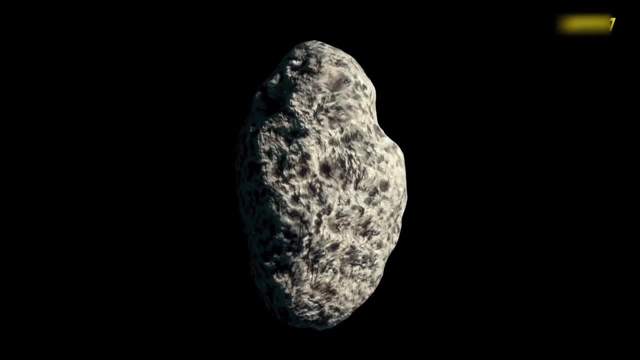 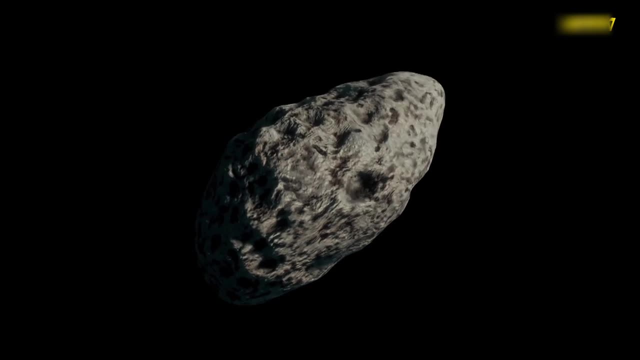 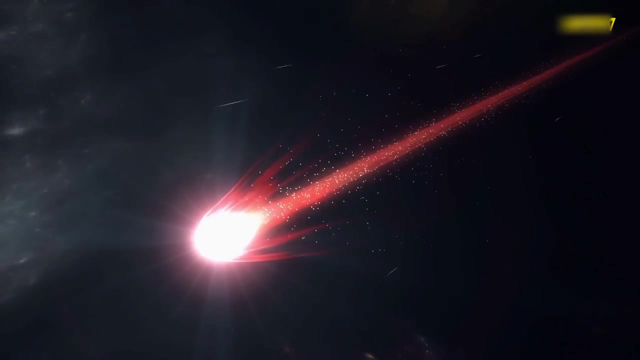 The fact that Saturn grew to such a size had significance beyond just scale. Its size pushed the planet towards a very different evolution, Changing its relationship with the environment and ultimately sending it on a completely new path. It's because of its immense mass and its place in the solar system. 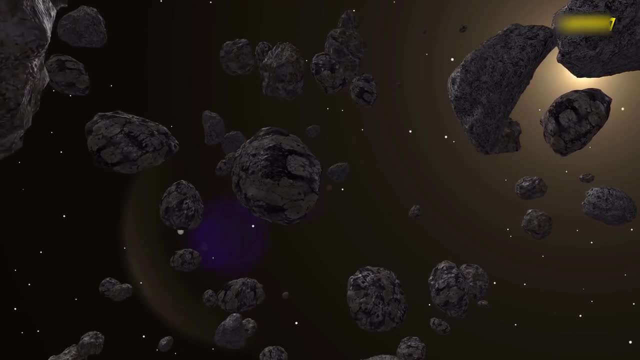 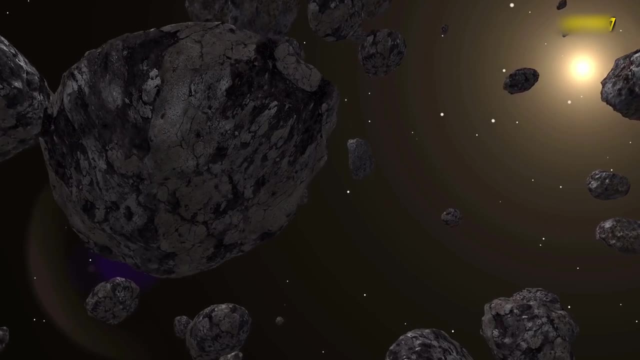 that Saturn wouldn't remain a rocky world for long. The history of the exploration of Saturn is littered with many of the greatest names in the field of science. Galileo Galilei was the first to peer at her through a telescope in 1610,. 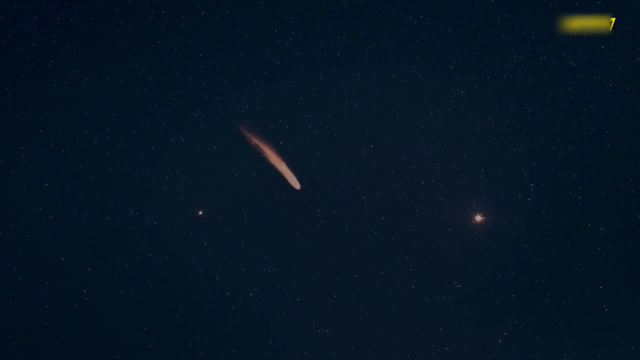 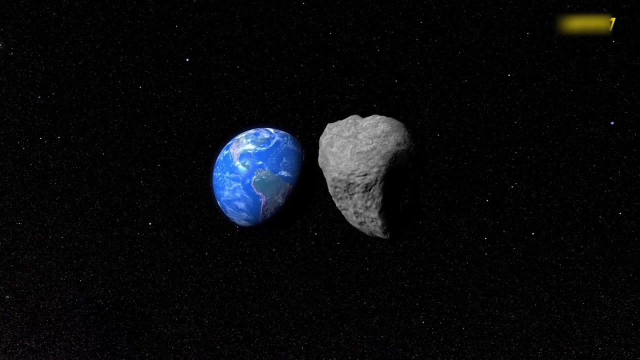 mistaking the faint outline of the rings for two moons on either side of the planet. He famously reported the planet appeared to have ears. Two years later, however, when he looked up again, the peculiar structures on either side of the planet had disappeared. 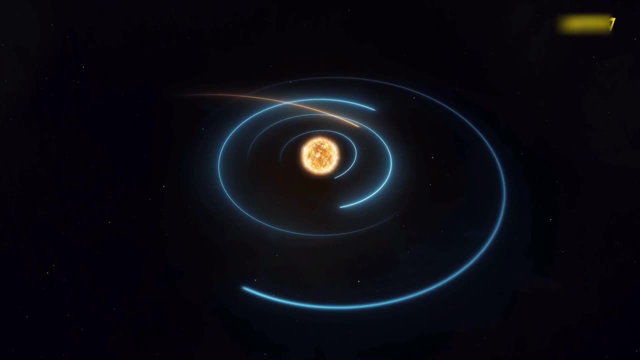 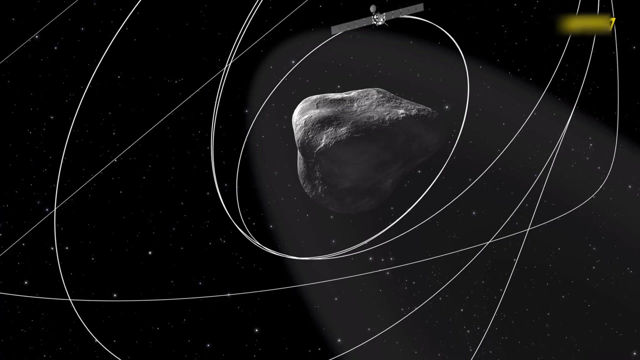 We now know this is because the rings were facing the Earth edge-on at the time of observation, but for Galileo this was a strange and mysterious anomaly. It would take almost 50 years and the more powerful telescope technology of Christian Huygens to solve the problem. 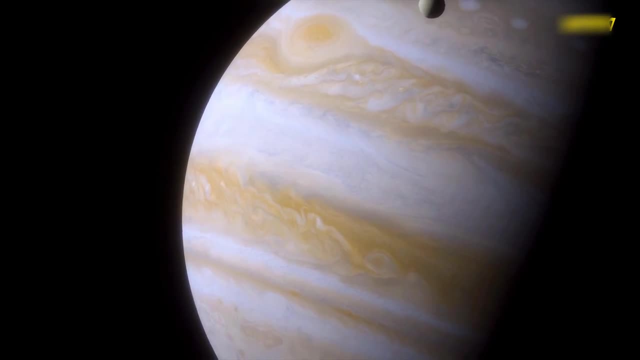 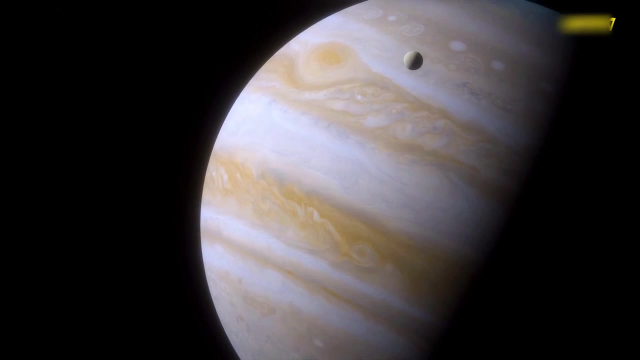 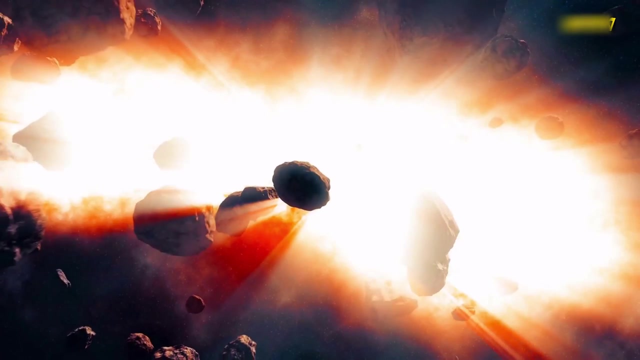 Using a 50mm refracting telescope, Huygens was the first to spot a moon of Saturn, publishing his discovery of Titan in 1656.. At the same time, his observations led him to begin formulating a theory to explain the strange ears that Galileo had first seen. Not moons but a ring around the planet. Uncertain that he had enough proof to convince the scientific community of his hypothesis, Huygens did what was common at the time: He published his thinking, not as a preliminary hypothesis or even as a line of investigation. 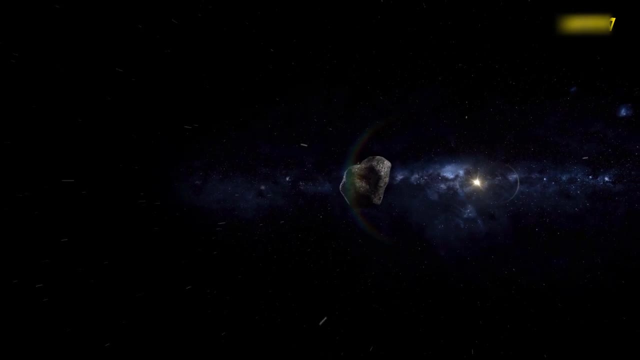 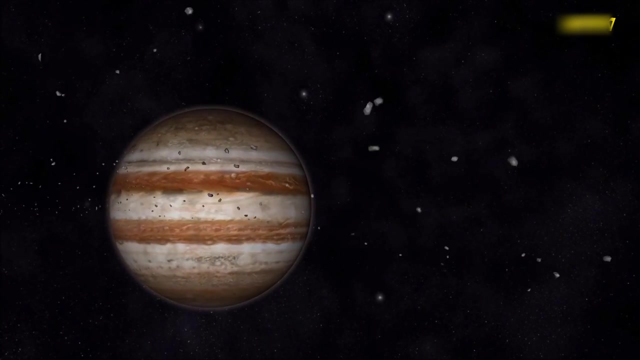 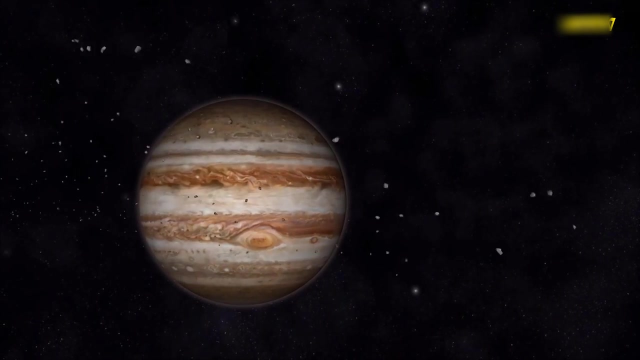 but instead, in order to mark the territory and protect his reputation, He announced his discovery in the form of an anagram: A-A-A-A-A-A-A, C-C-C-C-C-D, E-E-E-E-E-G-H- I-I-I-I-I-I-I. 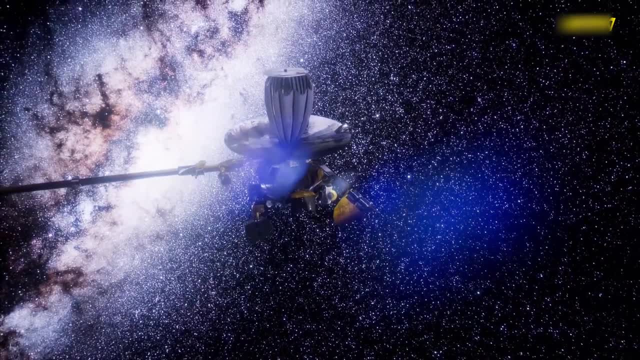 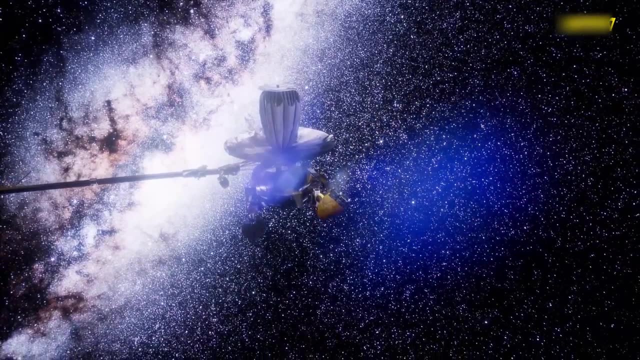 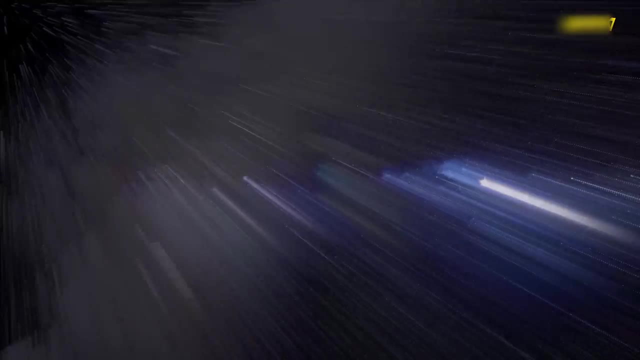 L-L-L-L, M-M, N-N-N-N-N-N-N-N-N, O-O-O-O, P-P-Q-R-R-S, T-T-T-T-T-U-U-U-U-U. For two years, the anagram remained unbroken, protecting Huygens' claim to be the first to identify the rings. 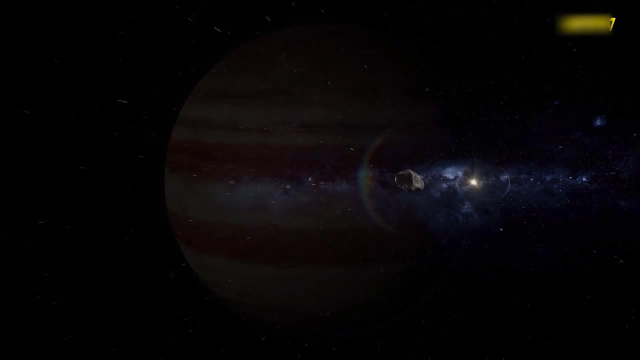 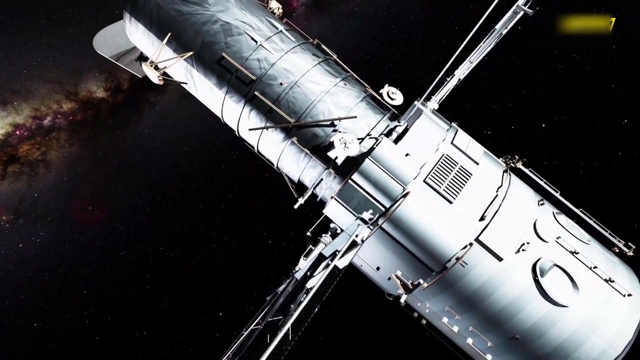 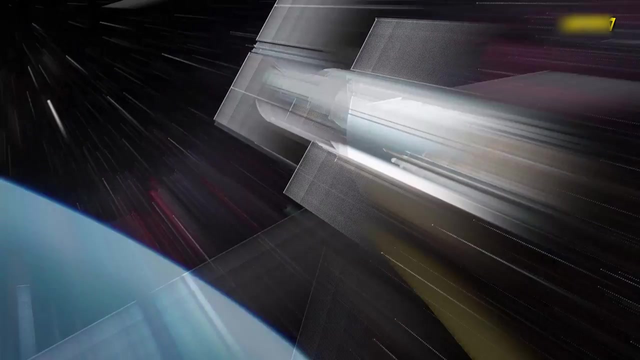 while also giving him enough time to build the evidence to make the hypothesis defendable. It wasn't until 1658 that Huygens revealed the meaning of the anagram to be a Latin sentence: ANNULO CINGITUR TENUI PLANO NOSQUAM COHAERENTE AD ECLIPTICAM INCLINATO. 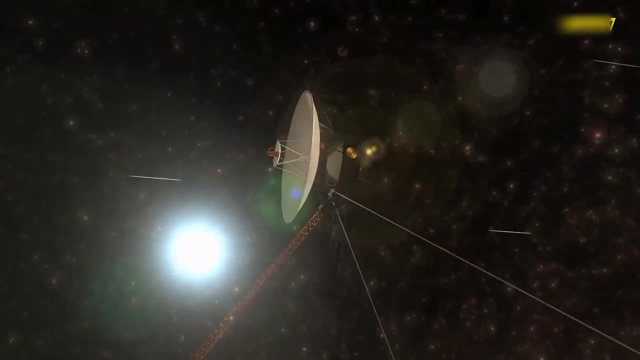 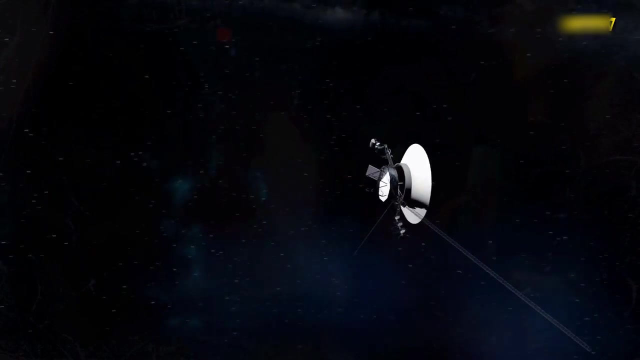 Which means it is surrounded by a ring, thin and flat, never touching oblique in relation to the ecliptic, With the rearrangement of 62 letters, one of the most beautiful structures in the solar system: the rings of Saturn. 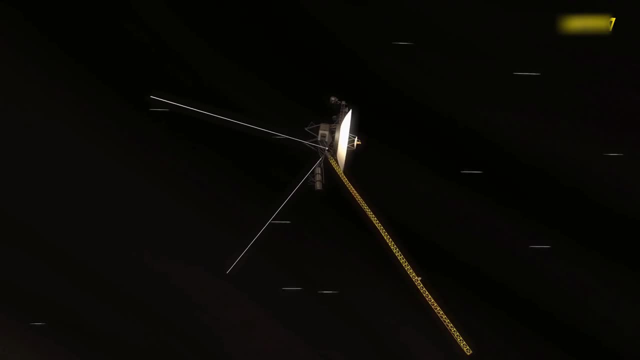 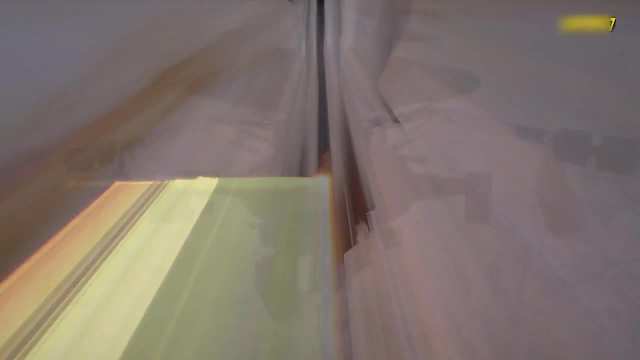 had been revealed to the world, If not yet understood, While Giovanni Cassini and William Herschel went on to discover more moons of Saturn and to detail structures within the rings, including the 4800 km gap between the A and B ring. 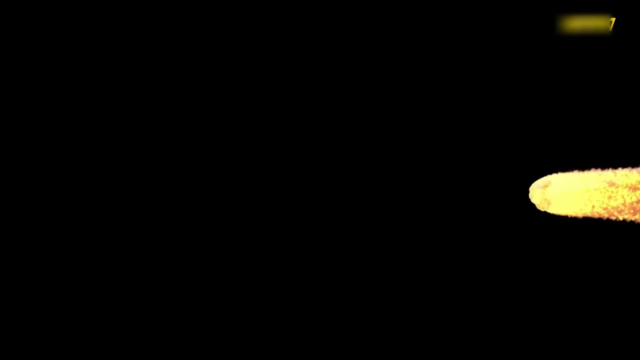 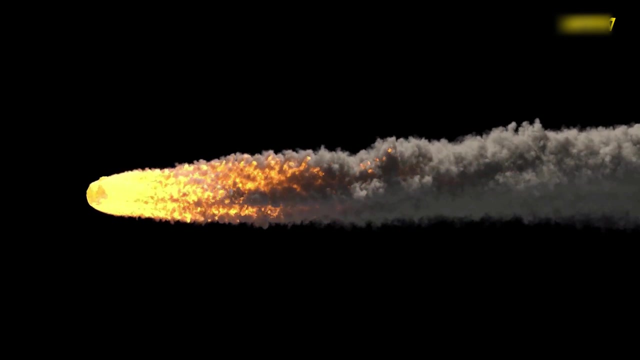 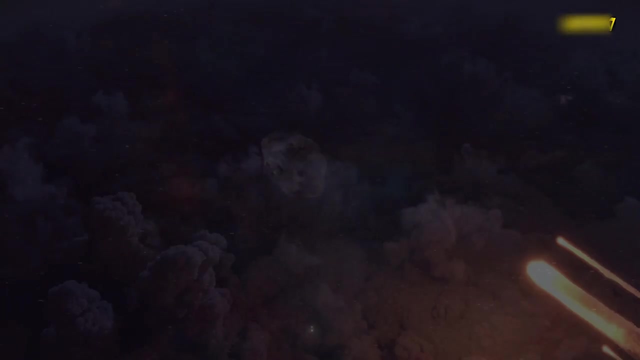 that would later become known as the Cassini division. we still imagined the rings as one great disc, a flat, solid circle of material encircling the planet within. It was Pierre-Simon Laplace, the French Newton, who was the first to suggest, in 1787,. 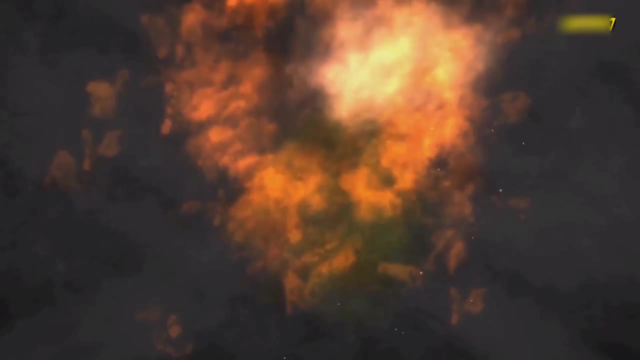 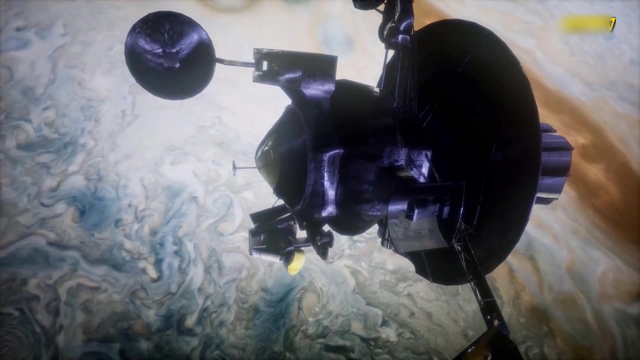 that such a singular structure around a planet would be unstable and instead was more likely to be comprised of a number of solid ringlets. By the mid-19th century, it was the turn of the great mind of James Clerk Maxwell to investigate the rings. Unpicking centuries of conjecture around the nature of the rings, he demonstrated for the first time, through a series of mathematical proofs, that any solid structure, be it single ring or ringlets, would be unstable and so unable to exist around the distant planet. Therefore, Maxwell concluded, the rings must be composed of a huge number of small particles all orbiting the planet independently. In his words, every particle of the ring is now to be regarded as a satellite of Saturn, disturbed by the attraction of a ring of satellites. at the same mean distance from the planet, each of which, however, is subject to slight displacements. The mutual action of the parts of the ring will be so small compared with the attraction of the planet that no part of the ring can ever cease to move around Saturn as a satellite. With Maxwell's publication On the Stability of the Motion of Saturn's Rings in 1859, our modern understanding of this distinctive feature of Saturn had begun. But it would be another 120 years before we'd get the chance to explore the most remarkable bodies in the heavens. as Maxwell described them up close, At 1426 Universal Time. on the 1st of September 1979, after a six-year journey from Cape Canaveral across over a billion kilometres of space, the Pioneer 11 spacecraft took us within touching distance. of the rings of Saturn for the very first time. As our first explorer to cross the boundary of the rings, Pioneer flew across the ring plane beyond the outer ring, enabling it to photograph the Saturnian system in extraordinary detail, sending back a series of images. that revealed the ringed planet in greater resolution than we could ever have seen from Earth-bound observations. On its way through the ring plane, Pioneer was able to take the first close-up measurements of the rings and in doing so discovered not only a new ring system, the F ring, but also two new moons of Saturn. In fact, the spacecraft flew so close to the as-then-unknown moon, passing at a distance of just 6,676 kilometres. it was lucky the mission didn't abruptly end with a massive collision. We now know Pioneer had encountered either Epimetheus or Janus, but we're still not sure which one of these two similar-sized moons it was, as both sit in the same orbit around Saturn, Travelling at a speed of 114,100 kilometres per hour. Pioneer passed within 21,000 kilometres of Saturn's cloud tops, making its closest encounter at 1629 UST on that September day, before speeding off beyond the rings and onwards on its journey to the outer solar system, As well as taking 440 images of the Saturnian system. Pioneer measured the characteristics of Saturn directly. An array of sensors were able to confirm that this giant planet was a bitterly cold world, with an average overall temperature of minus 180 degrees Celsius and a composition made up almost entirely of liquid hydrogen. But beyond the basic data, perhaps Pioneer's greatest achievement was to plot a course through the Saturnian system and make its way safely through the ring system while returning data back to Earth. Now the stage was set for the two Voyager probes already well on their way across space, speeding towards the ringed planet. equipped with an even more advanced array of technology, ready to probe even deeper into Saturn's mysteries. The rings were named essentially in order of discovery. In terms of the main rings, it starts at the outermost, which is the A ring, and then goes into B ring, where most of the mass is. And there's a faint C ring and an even fainter D ring inside that. Then the E ring was discovered around 1980, when the rings, as viewed from the Earth, were edge-on. That's the one that's clearly associated with Enceladus. Then Pioneer 11 discovered the F ring and then Voyager discovered the G ring. And the G ring we know is associated with a moon called Aegeon, which is the source material for the ring. At that stage we stopped using the letters as a nomenclature. So there are other individual rings that have been named, but they tend to be rings or ringlets that are in the main ring system itself. Karl Murray Cassini Mission on the organisation of Saturn's rings Just over a year after Pioneer had exited the Saturnian system. early in November 1980, Voyager 1 swept in with its high-definition cameras, primed and ready for action. As it sped past Saturn at 17 kilometres per second, it was able to produce a wealth of new data about the planet, rings and moons. One of its key discoveries was the identification of three new moons: Prometheus, Pandora and Atlas. The mission revealed detailed relationships between these moons and the ring system within which they sat, which also confirmed a long-standing theory about the structure of the rings. At least the first two of these moons are shepherding moons. satellites that exist within the narrowest rings of Saturn and play an essential role in keeping the delicate structures in place by their gravitational interactions with the billions of particles within the rings. With its wide and narrow-angle cameras, Voyager 1 was able to take a series of pictures. showing in incredible detail Prometheus acting as a shepherding moon to the F ring and Atlas as a shepherd to the A ring. This first Voyager craft was also sent by the team at NASA's Jet Propulsion Laboratory to investigate one of Saturn's most intriguing moons up close. for the very first time, Titan had already been identified as potentially the only moon in the solar system with a thick Earth-like atmosphere, and Voyager was set on a course that enabled it to pass by within just 6,400 kilometres of its surface. As it flew on the dark side of the moon, looking back at Titan's atmosphere through the haloed light of the sun, it was able to accurately measure, for the first time, the density, composition and temperature of the atmosphere, and also obtain a precise measurement of Titan's mass. This mysterious moon, the largest of all Saturn's satellites, was found to have an atmosphere almost entirely composed of nitrogen, just like the Earth, with a surface pressure just 1.6 times that of our planet. Voyager opened our eyes to this curious world for the first time. a world we would come to explore in even more detail with the Cassini-Huygens mission, which would touch down on the surface of Titan. As well as exploring the rings and moon systems of Saturn, Voyager 1 was able to deploy its array of sensors and cameras. on the planet itself. With its closest approach on 12th November 1980, Voyager came within 77,000 miles of the Saturnian cloud tops and was able to measure powerful winds travelling at 1,100 miles per hour, whipping around the planet's equator and aurora. But most intriguing of all was the discovery that Saturn's upper atmosphere was composed of only 7% helium, while the rest was mostly made up of hydrogen. Scientists had expected Saturn to have the same atmospheric helium levels as Jupiter and the Sun, at 11%. So this much lower level suggested something intriguing was going on deep within Saturn's internal structures. Where was the missing helium? The lower levels in Saturn's upper atmosphere suggested that the heavier helium might be slowly sinking through Saturn's hydrogen, But it would take the arrival of Voyager 1's sister craft nine months later. to enable scientists to further probe the inner workings of Saturn and to begin to reveal the fate of the rocky ice world that had been lost inside this planet billions of years earlier, While passing behind Saturn and so shielded from the view of the Earth. Voyager 2 used its radio science system to probe Saturn's upper atmosphere, gathering information on its atmospheric temperature and density. It was an ingenious dual use of its telecommunications system that allowed Voyager to create a temperature profile of the planet. that provided the first direct evidence of something that scientists had long suspected. At the uppermost level of its atmosphere, Saturn's temperature was 70 K minus 203 degrees C, While at the deepest levels, around 120 kilopascals, the temperature increased to 100 degrees C, with increasing altitude becoming progressively thinner. until by the time you get 100 kilometers up, you'll have 99.999997% of the atmosphere below you. This essentially arbitrary line between the Earth and space is known as the Kármán line. It's a line that was calculated by the Hungarian-American engineer and physicist Theodor von Kármán to be the altitude at which the air becomes simply too thin to support aeronautical flight, where, as he wrote, aerodynamics stops and astronautics begin. Cross this line and you have officially gone from being a pilot to an astronaut. And you get to join a club that still only contains 561 members at the time of writing. The number of humans who have made it over the line is still so small, because traveling the short hop into space might be slightly less than that, But it is large in terms of the power and technology needed. 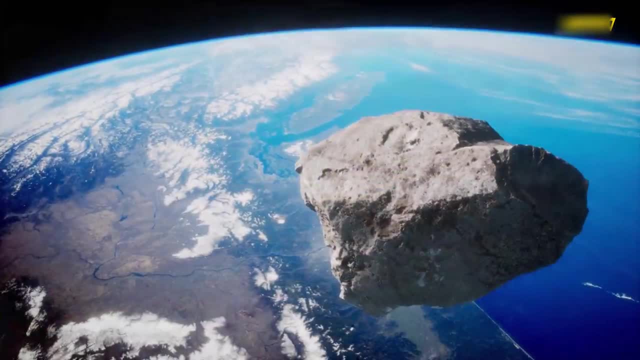 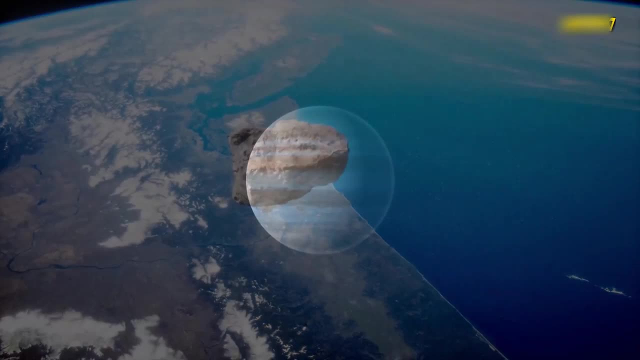 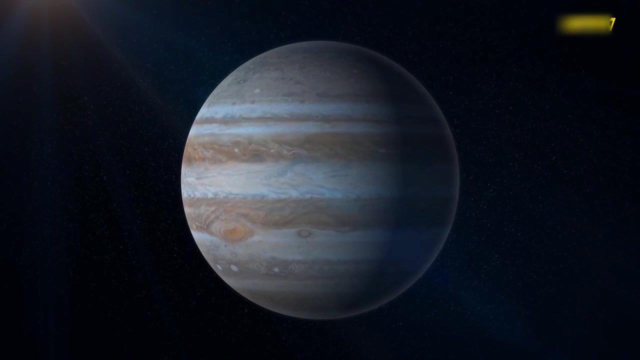 to lift anyone or anything that far from the Earth's surface. Gravity binds us tight to our little rock and despite over 60 years of space travel, it means almost all of us are still very much rooted to the ground, The reason we find it so tough to leave the Earth. 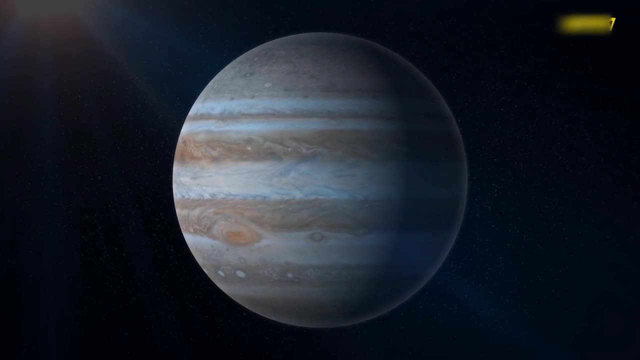 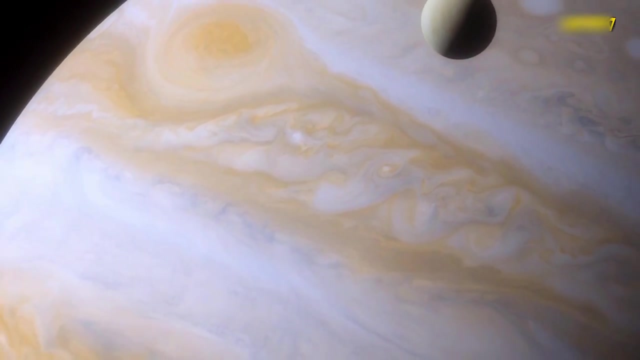 is because of the mass of the planet- all 5.9 sextillion tons of it- which creates a gravitational pull so strong it requires an escape velocity of around 11.186 kilometers per second to make it off the Earth and into space. 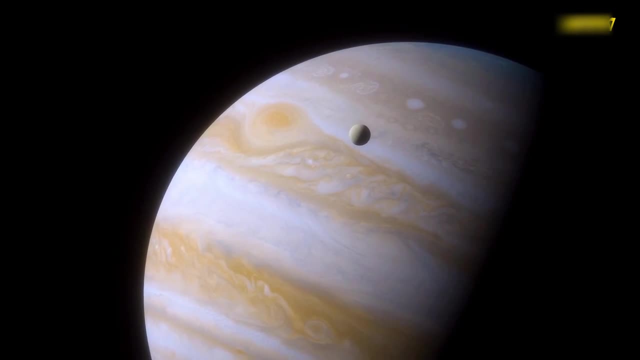 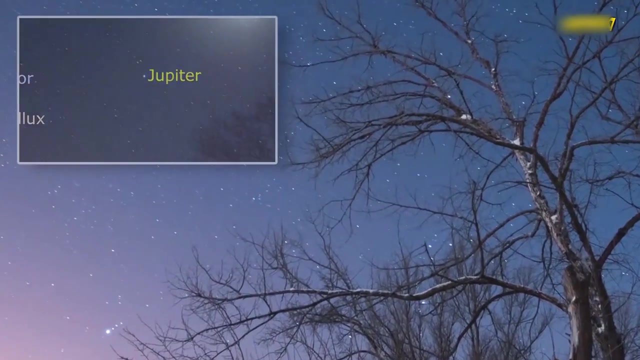 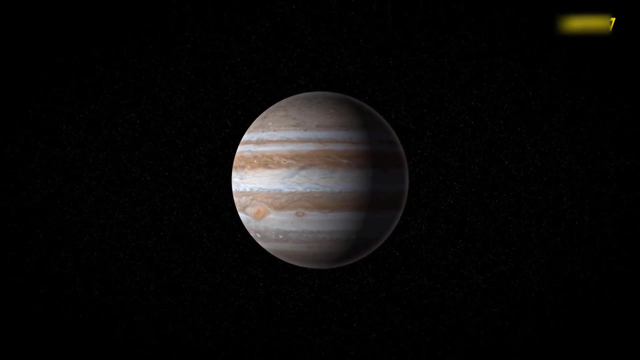 That's a lot of speed to counteract the 9.8 meters per second squared of gravitational force that is continually tugging us down. Gravity keeps our species firmly locked to the surface of the planet, but it also keeps a tight grip on everything else on the surface of the Earth. 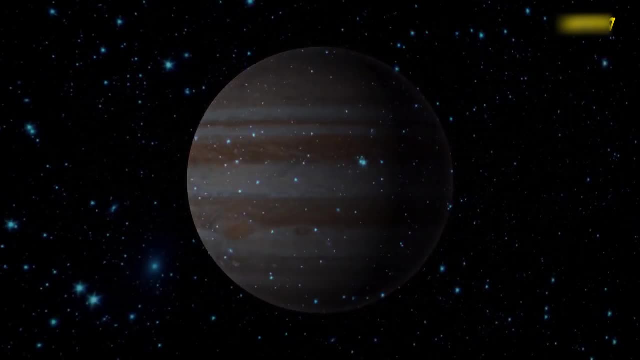 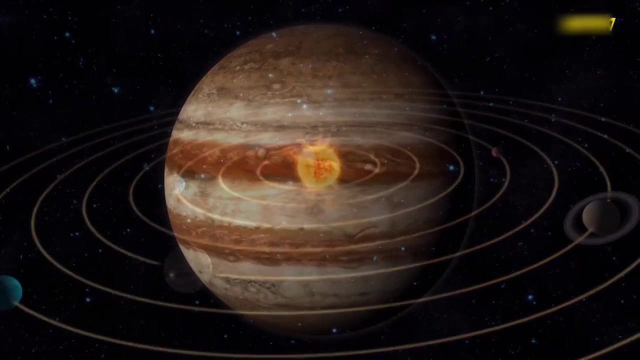 solid liquid or gas, including the 5.5 quadrillion tons of nitrogen, oxygen, carbon dioxide and other trace gases that together make up the Earth's atmosphere- In the very simplest terms, the size of the atmosphere of any planet. 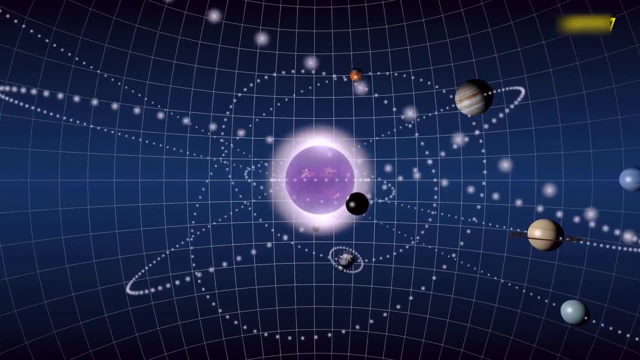 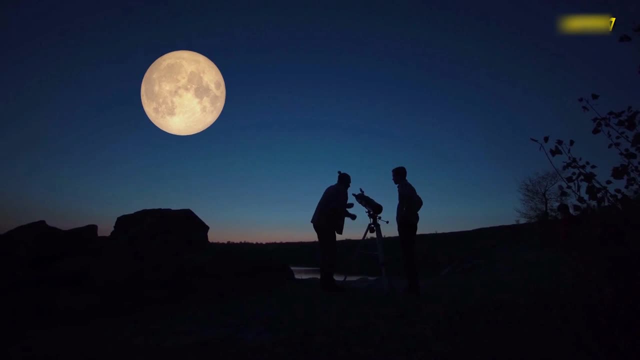 is intricately linked with the mass of that planet. The bigger the mass of a planet, the greater the attraction of gases to its surface. But that's not the end of the story. The ability of a planet to retain an atmosphere is also dependent on a multitude of other factors. 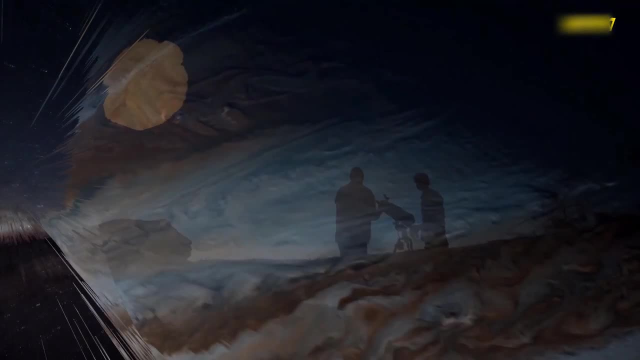 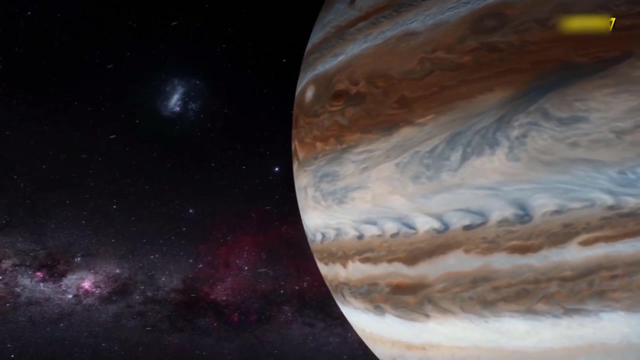 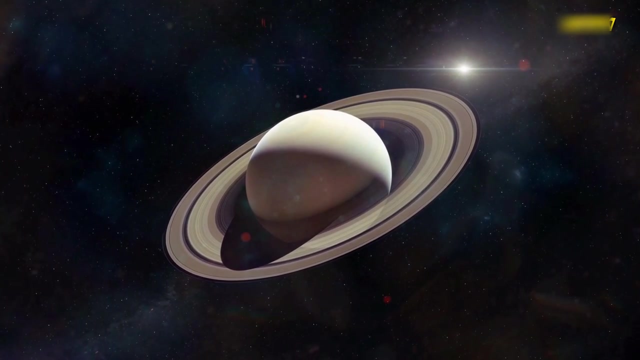 including the composition of the atmosphere, its temperature, proximity to the sun, geological activity, the ability of the planet to protect itself from the ravages of the solar wind and, finally, the impact of life itself, which has seen our atmosphere gradually pumped full of oxygen. 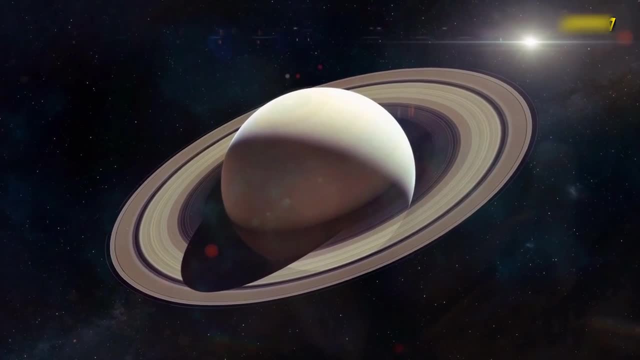 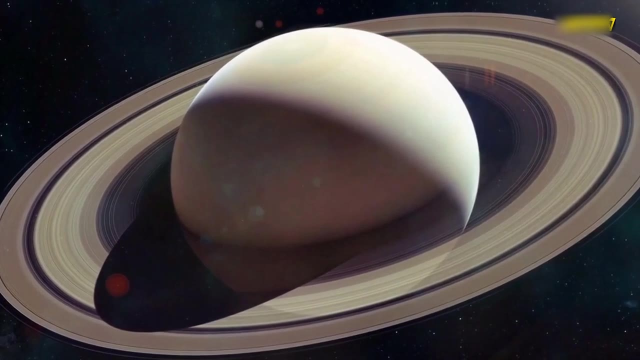 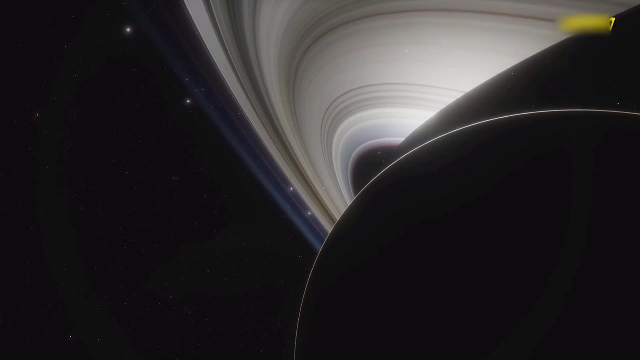 It's the intricate balance of these factors that dictates the endurance and composition of the gases around a planet, Each one a unique atmospheric fingerprint. Fast forward through the history of the solar system and we see a familiar theme again and again around the inner rocky planets. 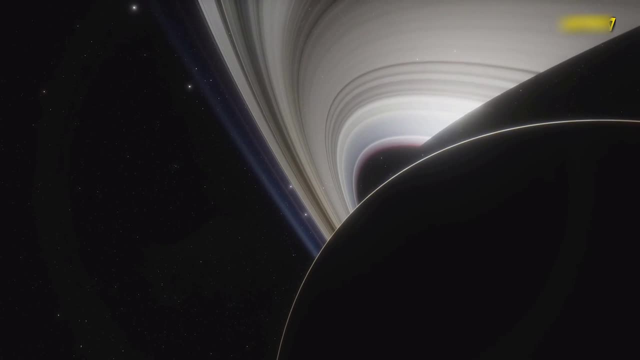 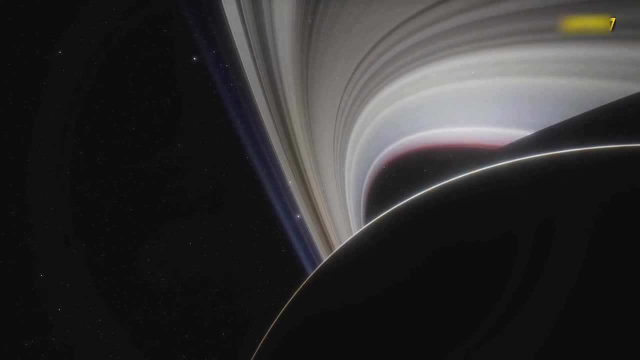 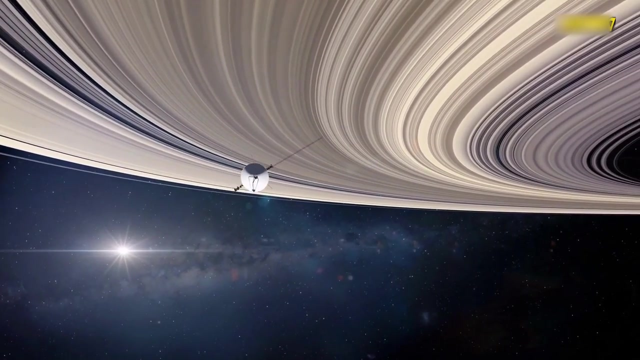 Each of the four planets grabbed onto a thin atmosphere, but then the individual characteristics of each planet set in motion its own individual evolution. Mercury, the smallest of the planets and closest to the sun, lost its atmosphere long ago, with only the merest whisp. 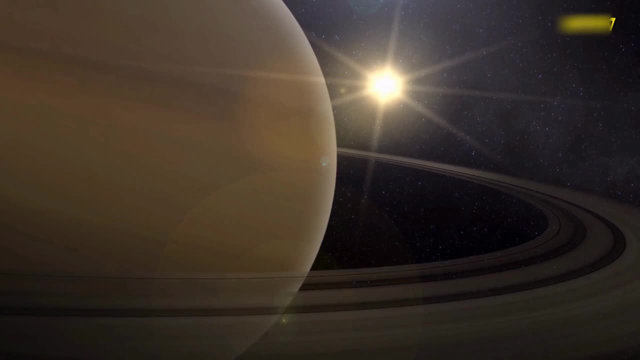 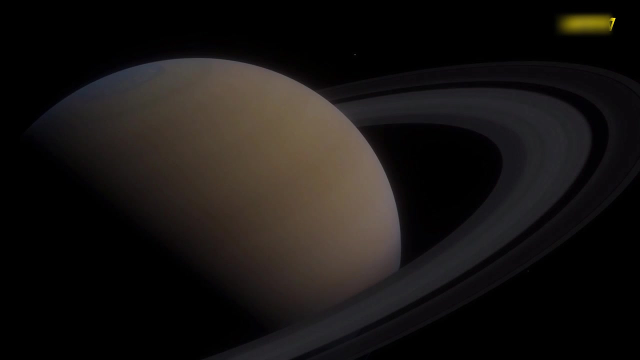 perhaps remaining today. Next, there is Earth sitting in the Goldilocks glow of the sun. We have clung on to our 100 km of atmosphere in one form or another for billions of years, allowing life to thrive under its warming embrace. 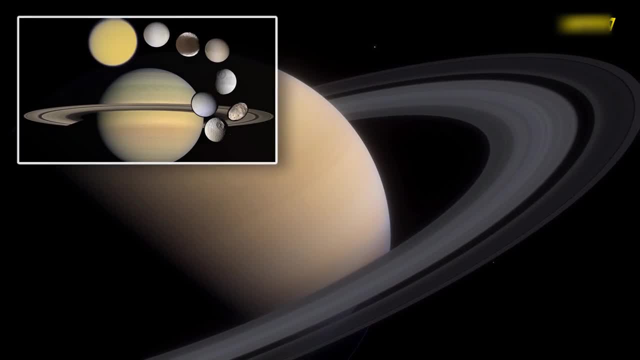 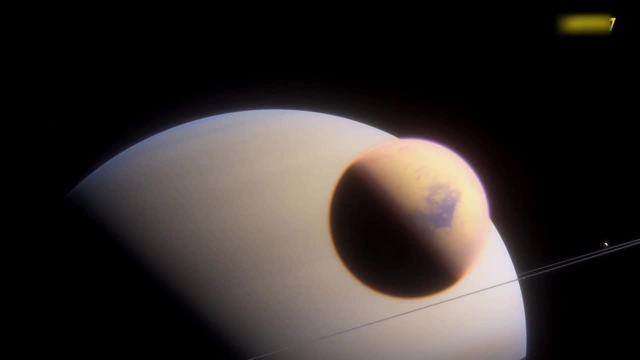 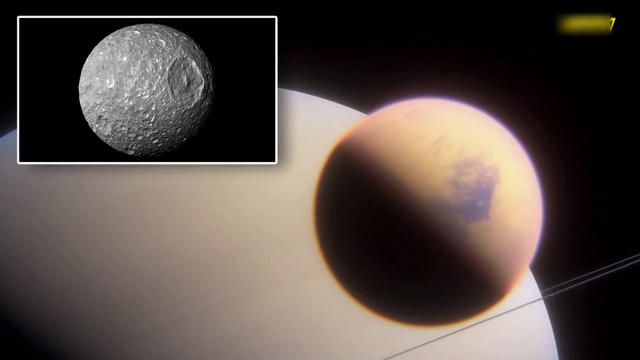 Venus, on the other hand, despite starting with an atmosphere likely very similar to our own, has now choked on the 250 km deep toxic atmosphere that blankets its surface today. Each of the four rocky worlds has seen its atmosphere ebb and flow over time. 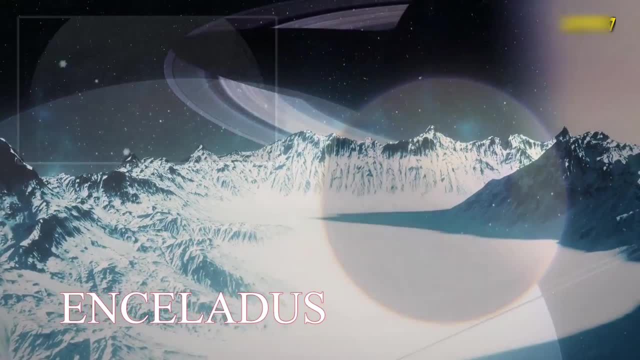 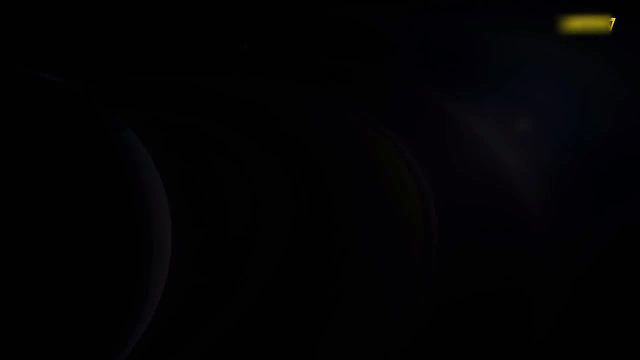 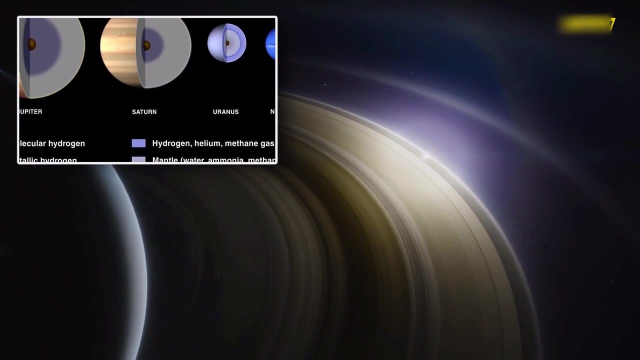 But no matter what twists and turns the story of each planet may have taken, there has always been, and will always be, a limit to the size that any atmosphere can grow around these relatively small lumps of rock. Before we return to Saturn to understand how its atmosphere grew, 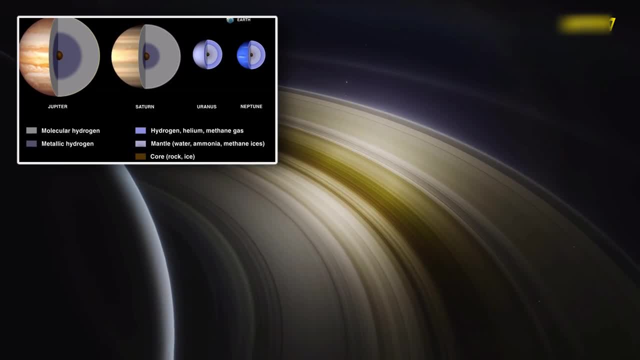 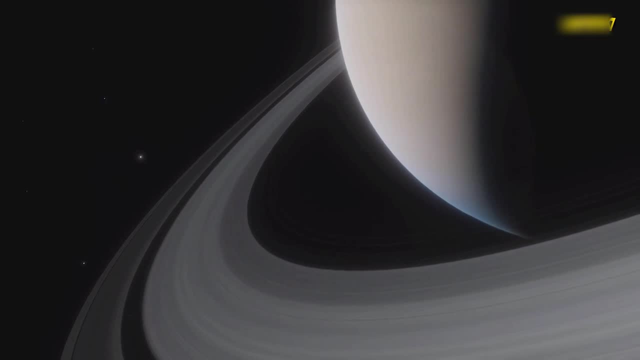 in a very different way to those of the rocky planets. we should take a swift look through the history of the Earth's atmosphere in more detail To establish how it began and evolved, Using a combination of geology, climatology and paleontology. 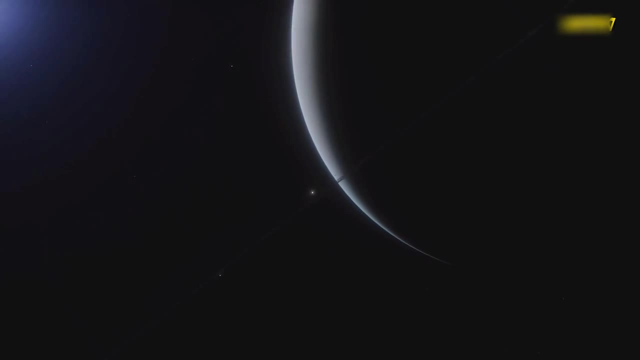 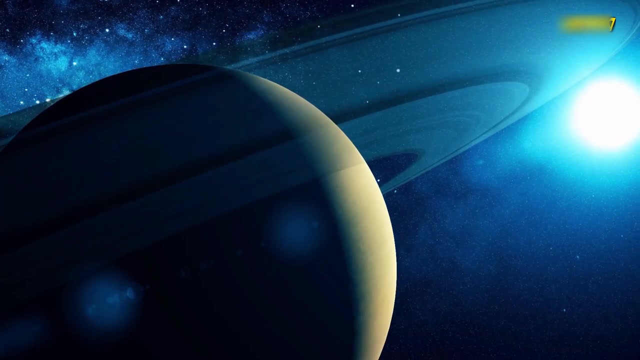 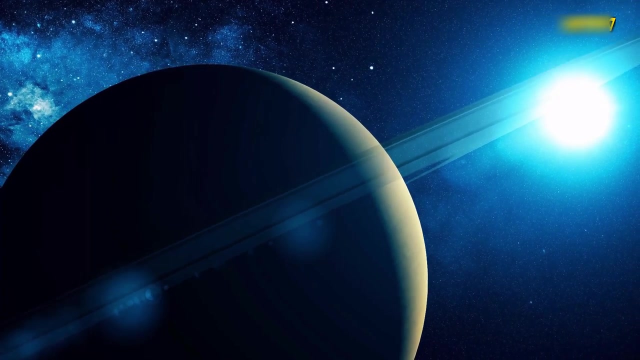 scientists have been able to piece together an immensely detailed picture of the Earth's atmospheric evolution. Far back in the Earth's history, a very different type of atmosphere to the one we see today surrounded the primordial planet. The newly formed Earth had grabbed on to gases. 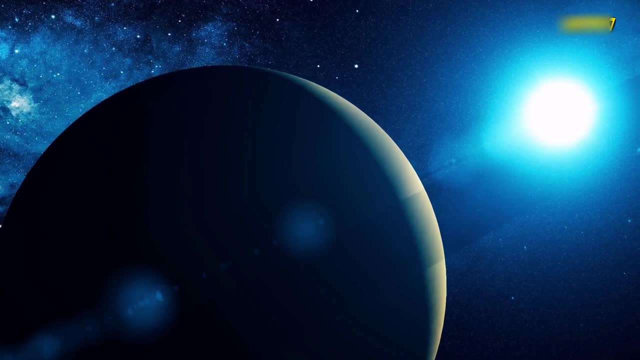 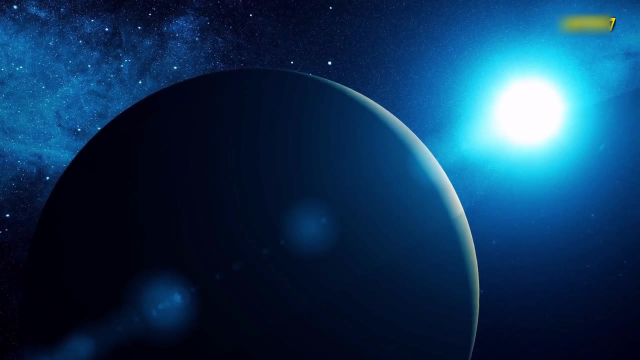 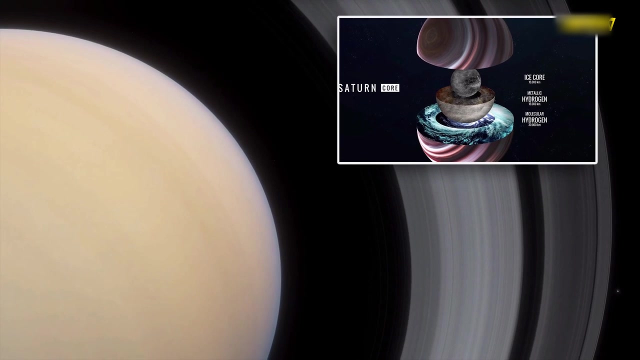 from the billowing vapours of the solar nebula, the cloud of gas and dust that the planet had formed from, consisting almost entirely of hydrogen and simple hydrogen-based molecules such as water, methane and ammonia, This primary atmosphere would have been entirely created. 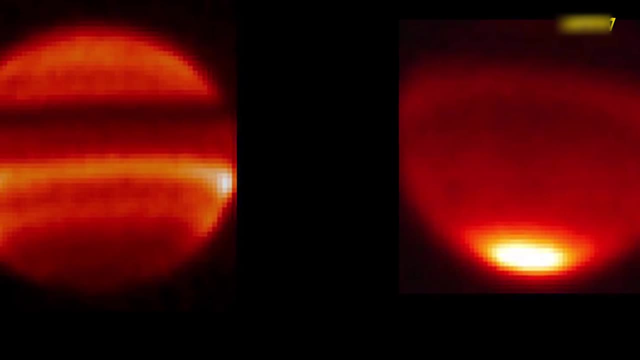 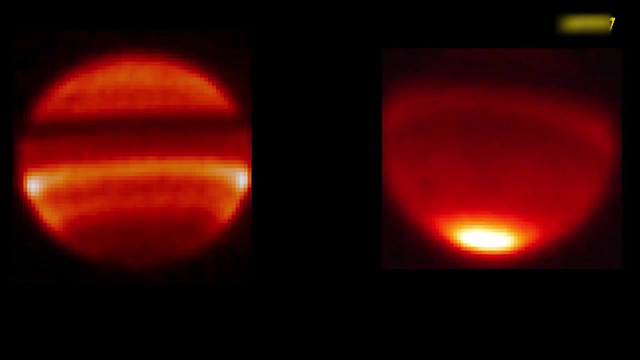 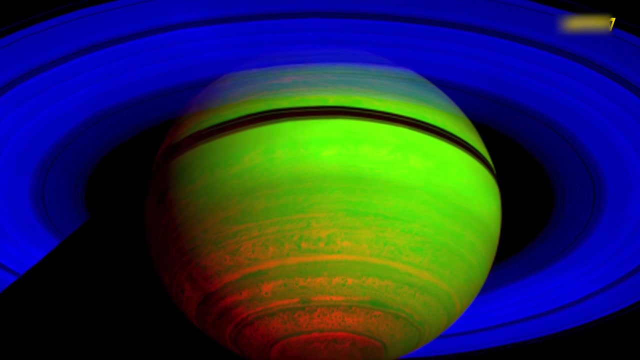 by the capture of the nebulous gases by the gravitational attraction of the planet. Slowly, over time, the composition of the atmosphere changed from a hydrogen-based one to one rich in nitrogen and carbon dioxide. We think this shift to the secondary atmosphere was at first triggered by the giant impact. of the planetesimal Thaya on the early Earth and then driven by a combination of gases produced during the late heavy bombardment, while asteroids rained down on our planet for millions of years and the geological activity within the Earth sent vast quantities of gas upwards. 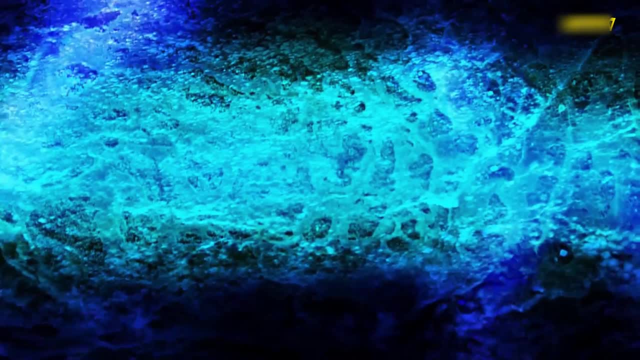 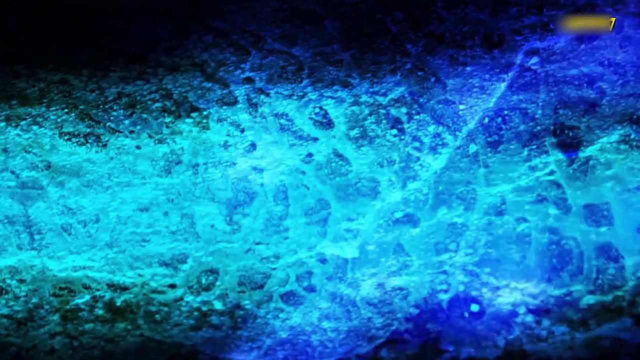 through all-encompassing periods of volcanism. By the time first life appeared on the planet, the nitrogen-rich atmosphere was stable, But gradually, as life took hold, a new component would begin to appear in the Earth's atmosphere Two and a half billion years ago. 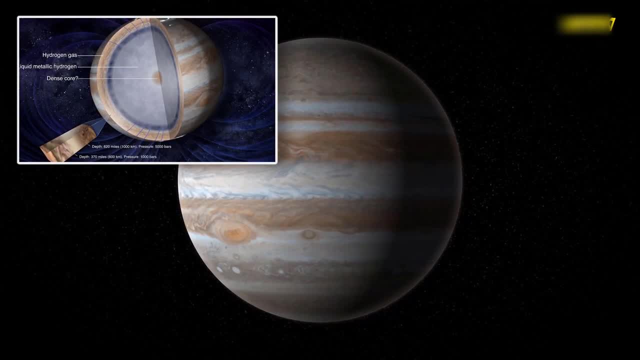 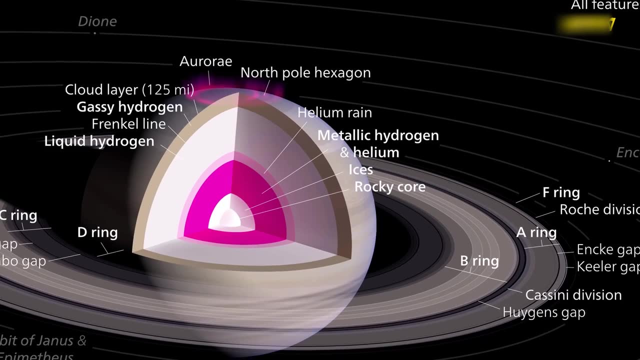 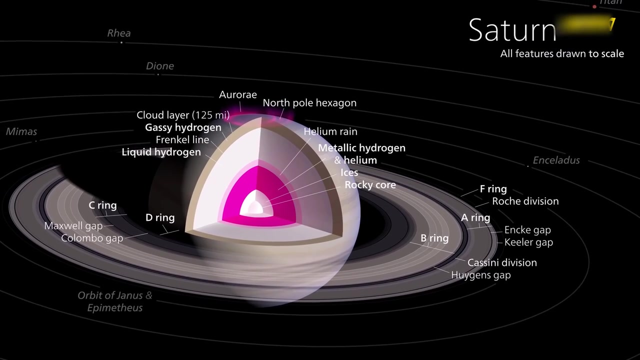 photosynthetic life had become so prevalent, it triggered a tipping point known as the Great Oxygenation Event, during which oxygen was produced by living things at such a rapid rate it far exceeded the amount of oxygen that was captured from the atmosphere in Earth's geological chemical reactions. 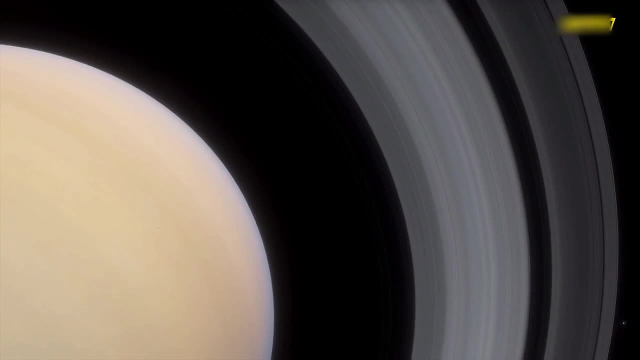 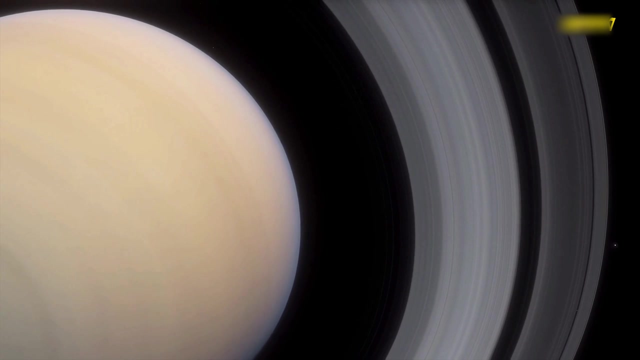 The result of this shift to the third atmosphere has been the presence of free oxygen in our atmosphere ever since, providing the energetics to support the rapid evolution of life on Earth. And, of course, one of these life forms has become so dominant. 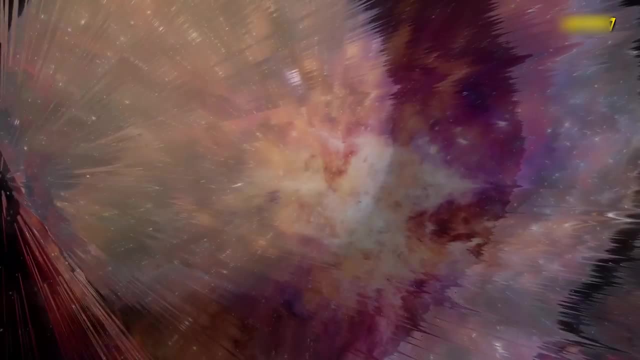 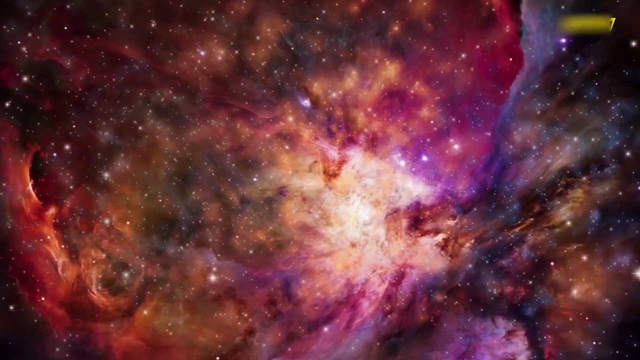 we've developed a way of life that is now fundamentally changing the atmosphere of our planet for a fourth time, but not for good. Now, with this history of our planet's atmospheric evolution in mind, let's return to the earliest days of the Solar System. 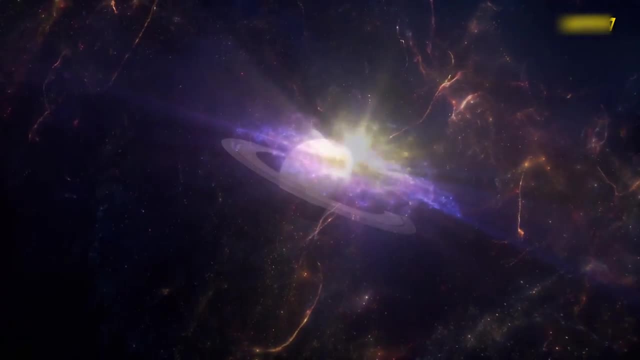 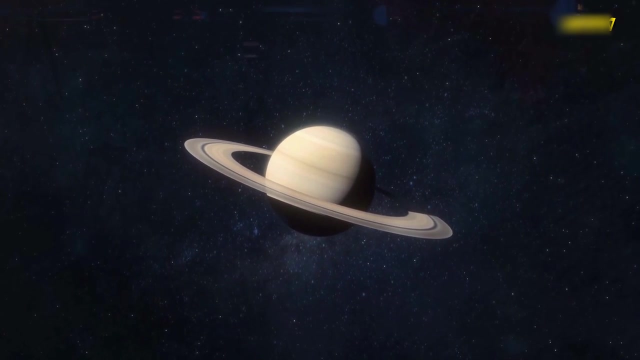 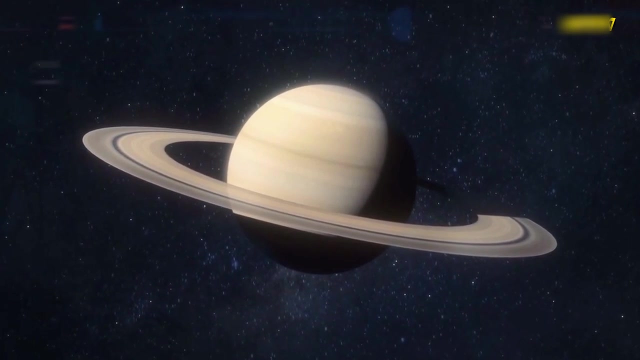 and explore the very different path taken by Saturn Around. four and a half billion years ago, the young Saturn had grown to become one of the largest rocky bodies in the history of the Solar System, At least ten times the mass of the Earth. it found itself far beyond the warmth of the Sun. 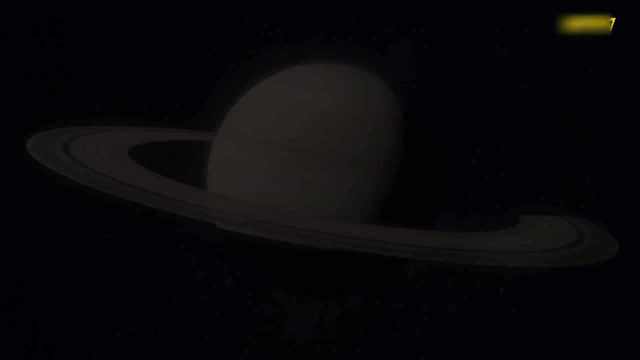 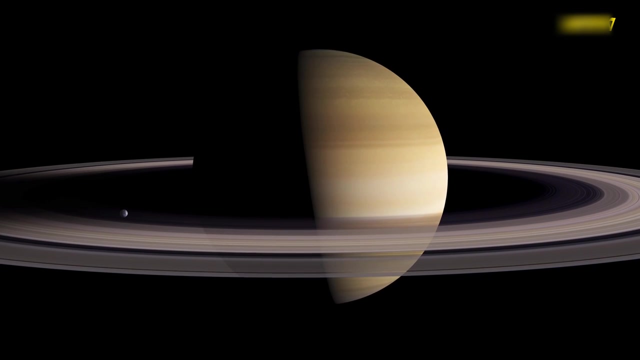 locked in its icy orbit a frozen, rocky world on a scale unlike anything we've ever seen. But time would not stand still for this world, Having grown as large as it could from rock and ice alone, its barren surface would not stay lit. 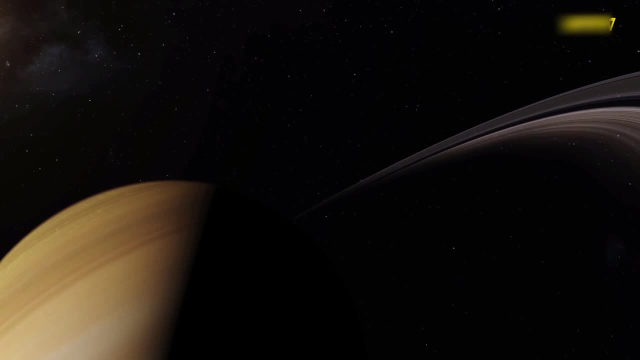 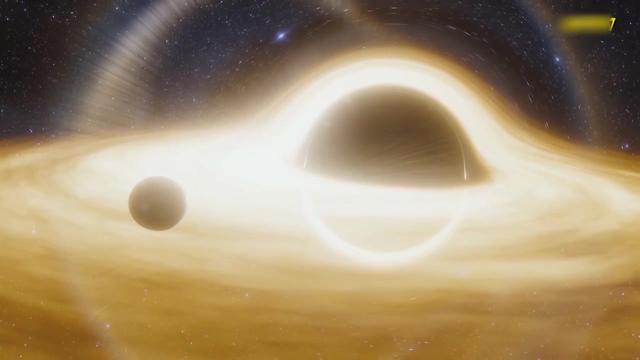 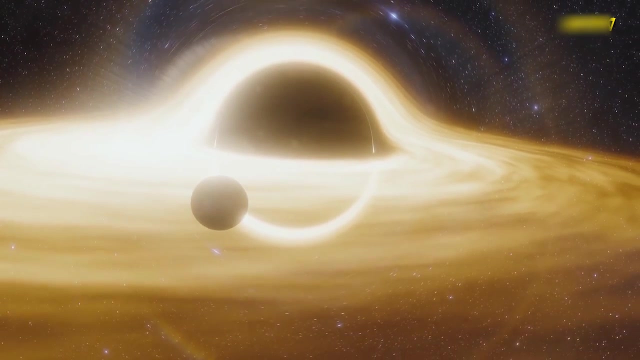 by the dim light of the Sun. for long. As it continued to grow, Saturn would become a radically different kind of planet, defined not by its rocky surface, but by an atmosphere that would bury it beneath vast volumes of gas, an atmosphere that would not just enwrap the planet. 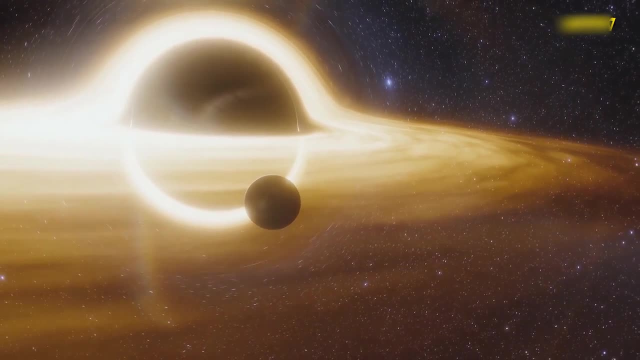 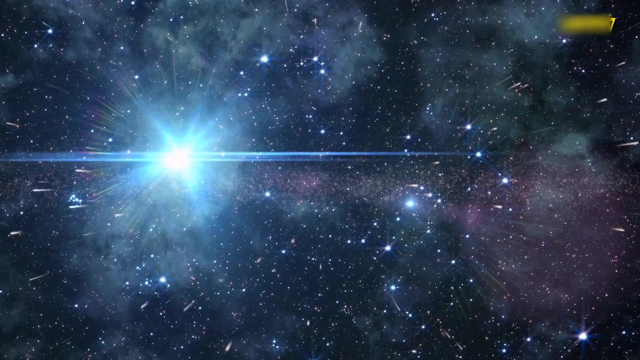 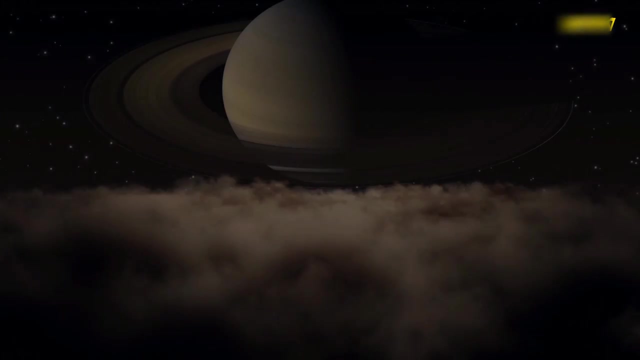 but engulf it, Just like the Earth in its earliest days. as Saturn continued to grow, it drew not just solid material but also gas towards it from the vast clouds swirling around the embryonic Solar System. Huge amounts of the hydrogen and helium left over from the formation of the Sun. 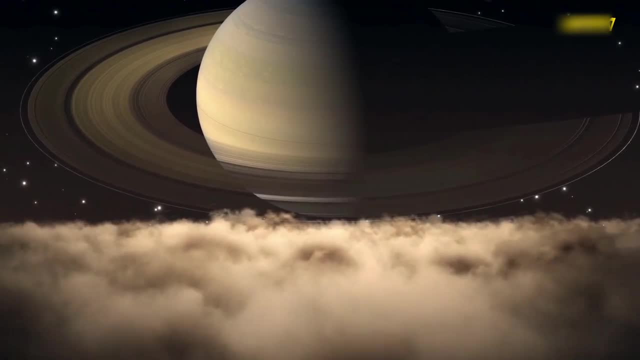 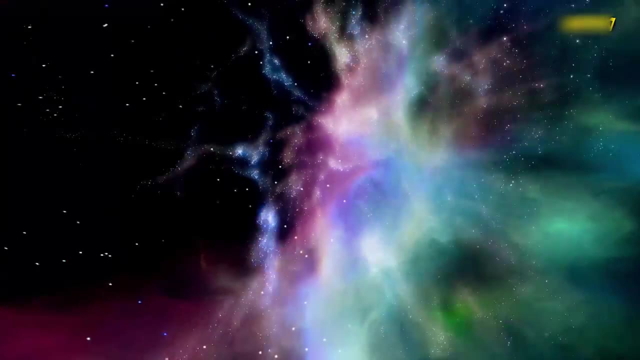 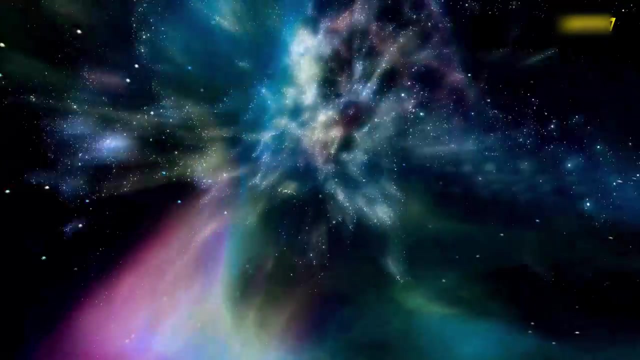 clung to the vast planet, creating a first atmosphere that may well have been very similar to the earliest one on Earth, But Saturn's early atmosphere would follow a very different course, as it was driven by two key differences between the young worlds. First, Saturn had grown far, far bigger than Earth. 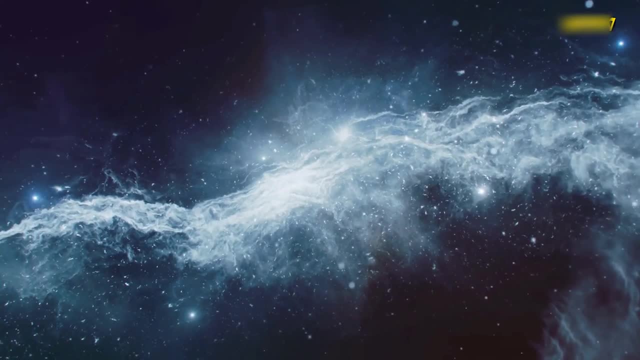 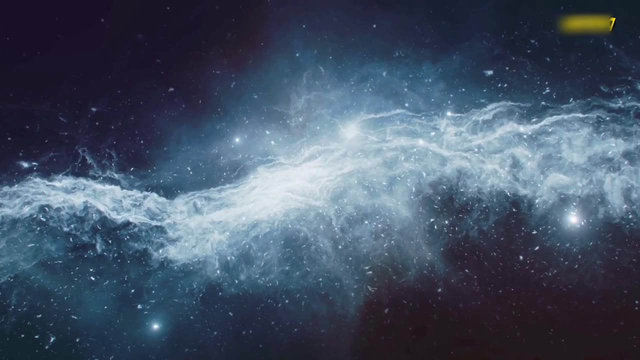 so by gravitational attraction alone, the volume of gas it could attract towards itself was far greater than anything the diminutive Earth was able to. But it wasn't just size that drove Saturn's atmosphere to grow so rapidly. Located this far from the Sun, 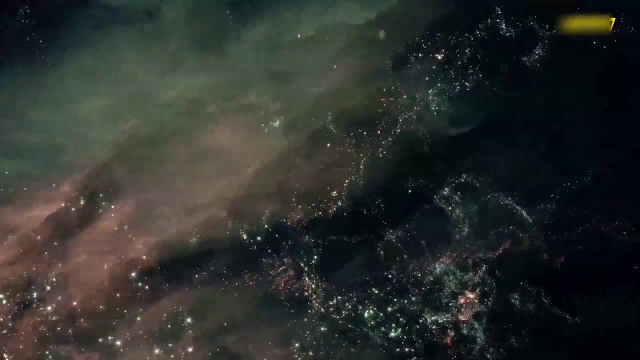 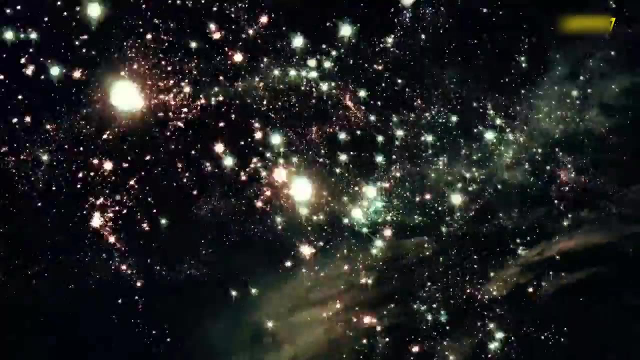 the freezing temperatures meant that even the most volatile of gases could cling onto the planet without being driven off by the heat of the Sun: Hydrogen, helium, ammonia, methane and many other gases that were too light for the smaller worlds of the inner Solar System. 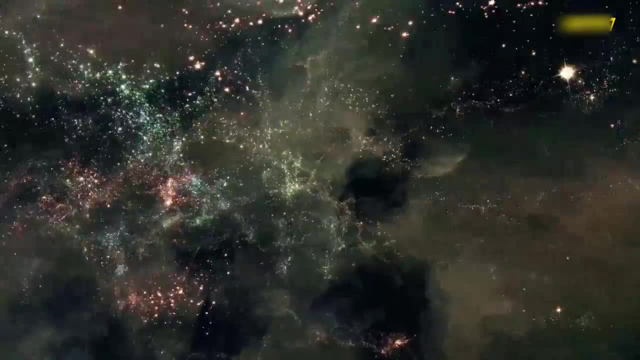 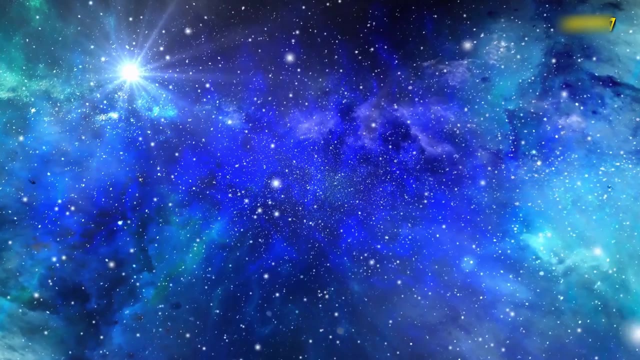 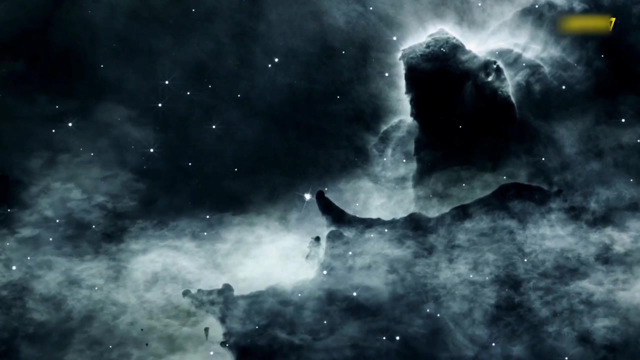 to hold onto were able to accumulate out here, with Saturn's vast mass and the freezing temperatures being enough to draw them in. Trillions upon trillions of tons of gas began to envelop the planet, reaching depths first of hundreds of kilometers and then thousands. 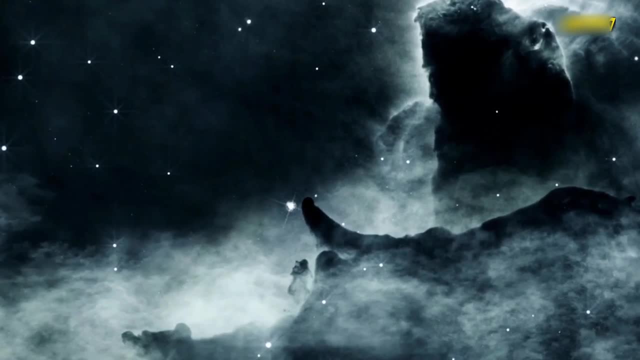 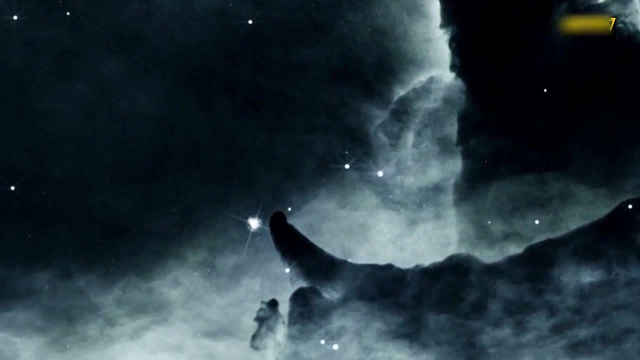 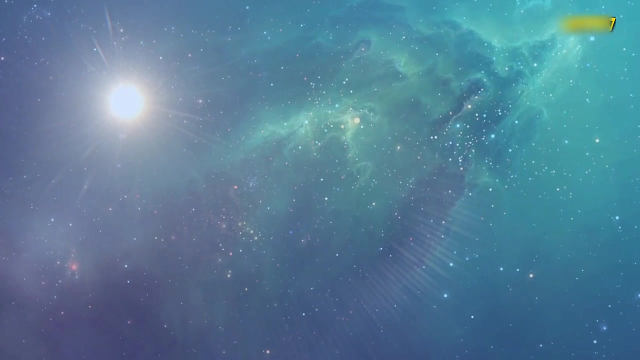 And as this new atmosphere grew, it transformed the surfaces below On Earth, under our canopy of air. it's easy to forget that all of those molecules sitting above your head right now have a weight If you draw a one centimeter square on a piece of paper. 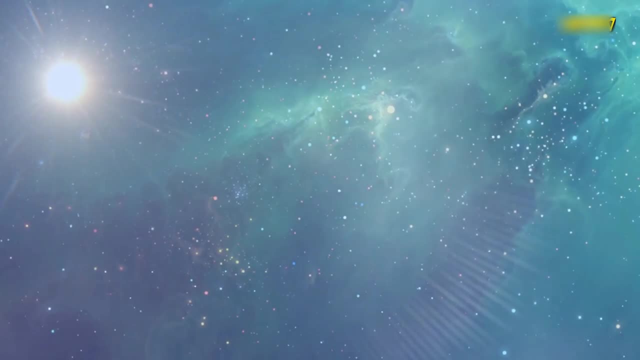 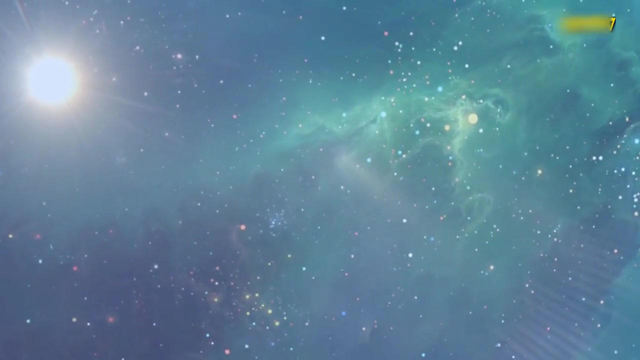 at sea level, and imagine a column of air stretching all the way up from the square to the top of the atmosphere. it will have a mass of, on average, just over one kilogram, Exerting a downwards force of ten newtons onto the paper. 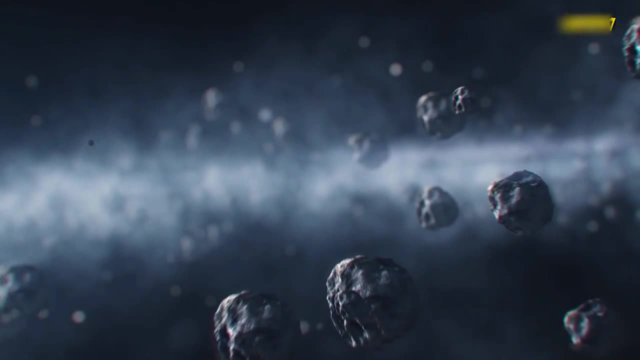 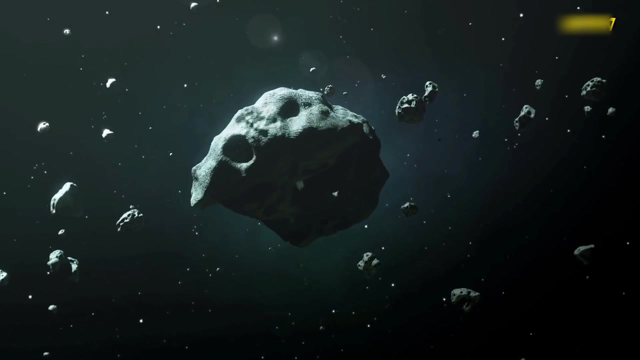 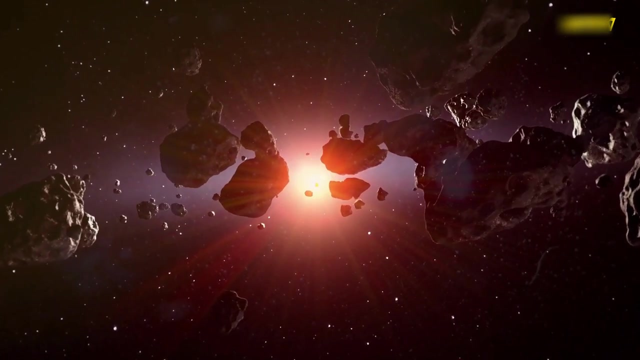 a pressure that we call 100 kilopascals or one bar. That might not sound like much, but all of that weight reveals itself in the subtle and not-so-subtle effects of atmospheric pressure that we can see all around us. For example, the simplest of classroom experiments. 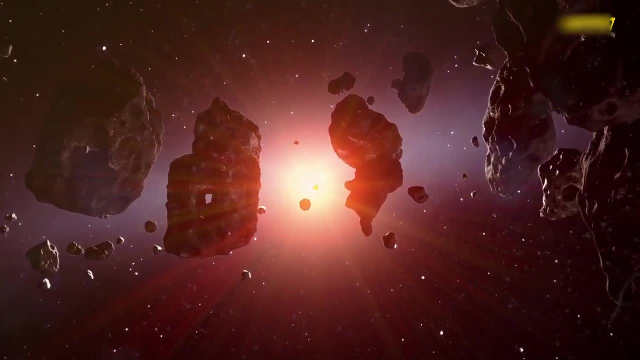 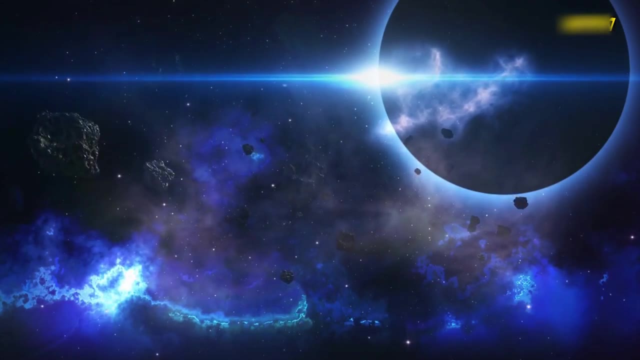 can reveal the power of the atmosphere by the process of just removing the air from a plastic bottle. The bottle collapses not because of the vacuum that it creates, but because the bottle cannot withstand the pressure of the atmosphere that is pushing down on it. 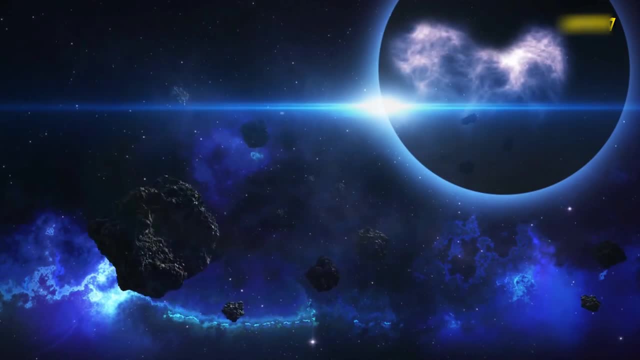 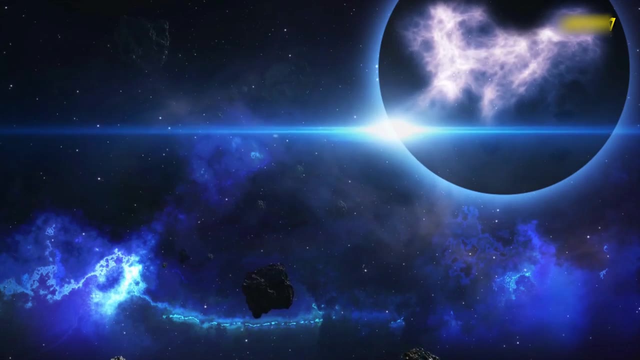 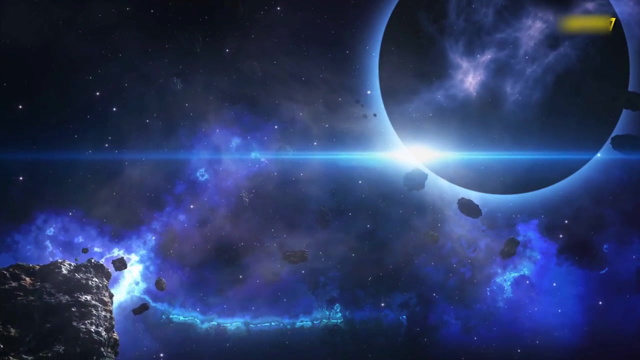 While 100 kilometers of atmospheric pressure can quickly crush a bottle here on Earth, a much bigger atmosphere can exert pressures that not only are able to shape things on the surface, but also have the power to transform an entire planet, And that's exactly what we think happened to Saturn. 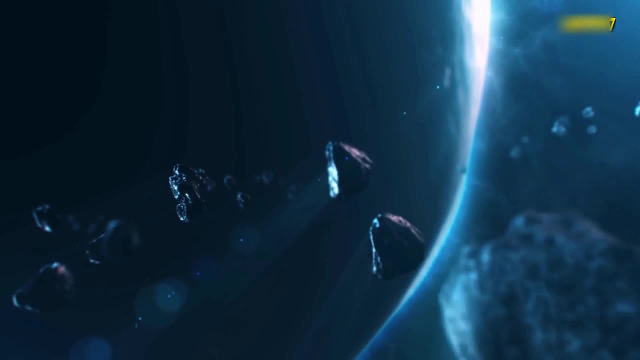 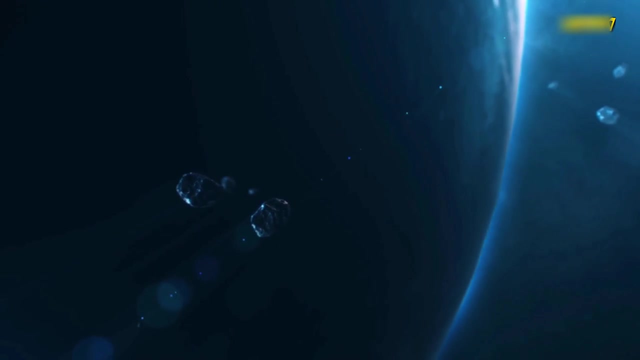 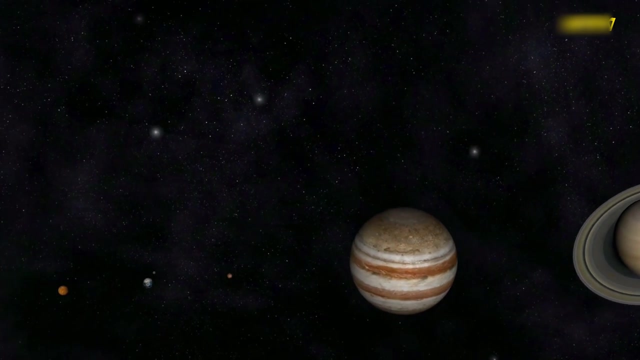 4.5 billion years ago, As its atmosphere deepened, the thousands upon thousands of kilometers of gas weighing down on its surface began to generate incredible pressure, heating the rock and ice so much they began to glow. It's thought, perhaps, that for a brief moment in time, 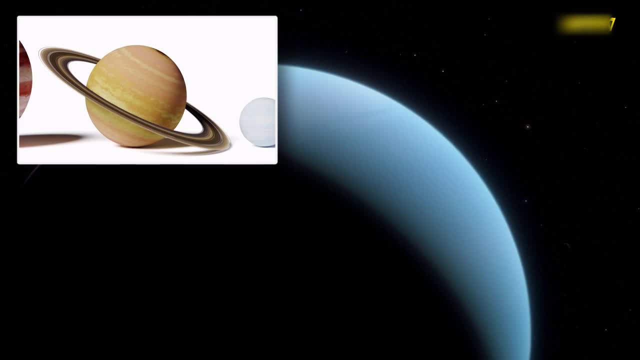 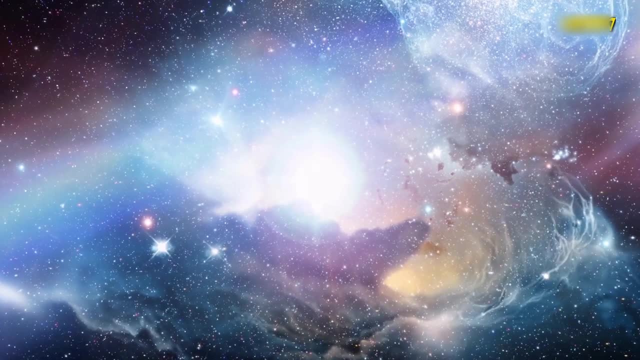 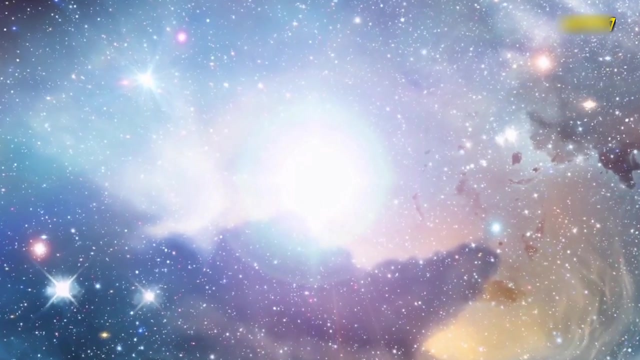 the heat generated on the surface of Saturn by these extraordinary pressures meant that the glow of the planet even outshone the sun. But this was just the beginning. As Saturn matured, the pressure at its core grew to 10 million times the level we experience on Earth. 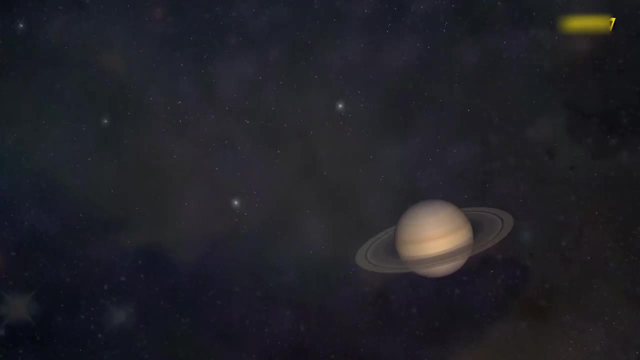 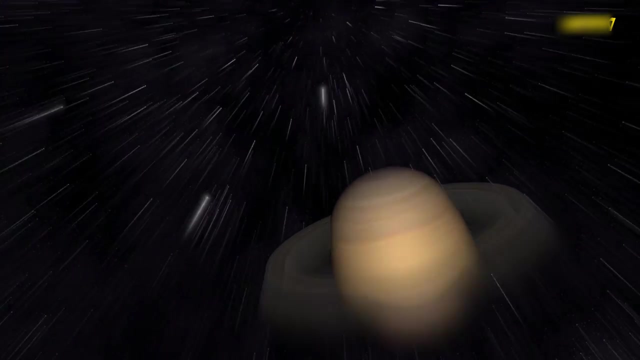 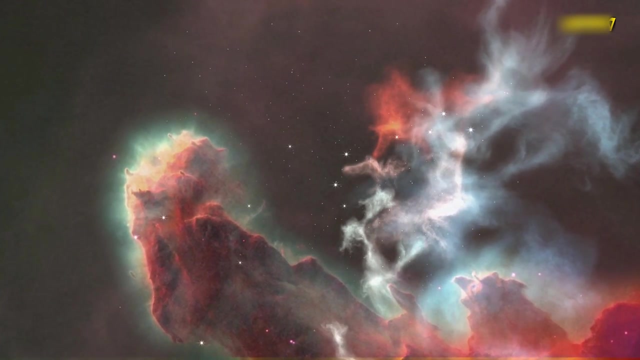 At that level of pressure, matter behaves in extremely strange ways and the very idea of a planetary surface becomes meaningless. As Saturn took on its new form, the enormous pressures generated, crushed and melted its solid core, destroying the rocky world it had been and replacing it with a new world. 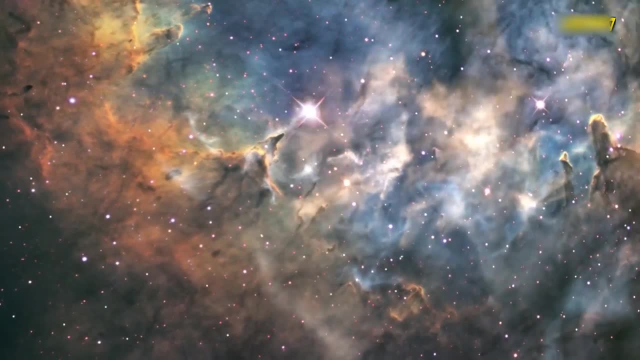 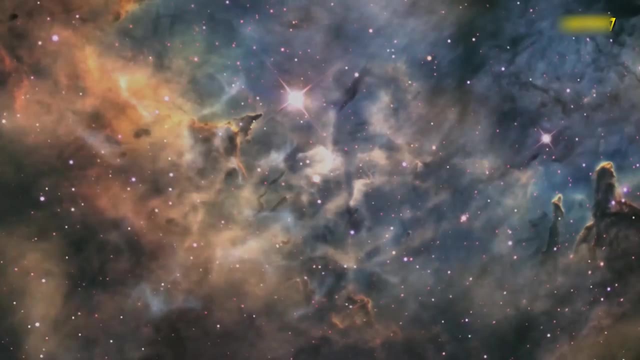 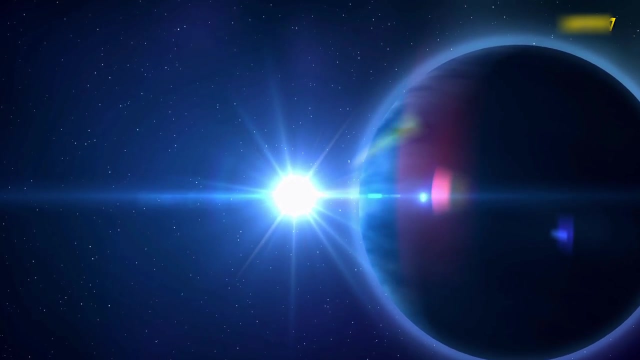 utterly alien in its characteristics. Saturn had transformed from a world of rock and ice into a wholly different class of planet, a gas giant, a ball of gas so big it could contain 800 Earth-sized worlds inside it, making it the second largest planet in the solar system after Jupiter. 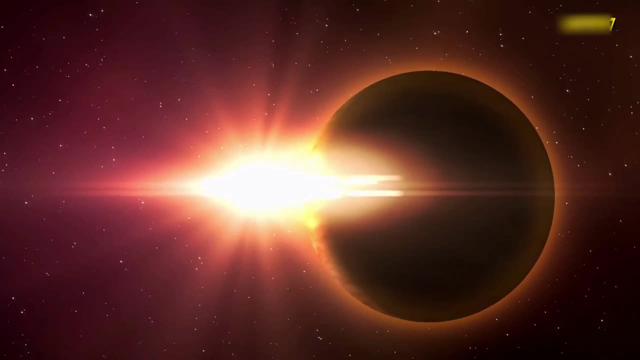 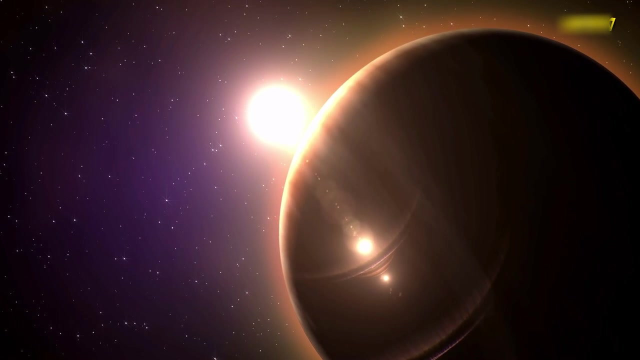 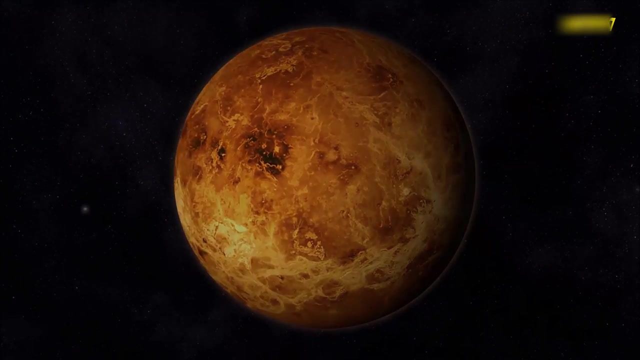 At 7.55 and 46 seconds AM Eastern Daylight Time on the 15th of September 2017, NASA's Deep Space Network antenna complex in Canberra, Australia, received notification that contact had been lost with one of our greatest space explorers. 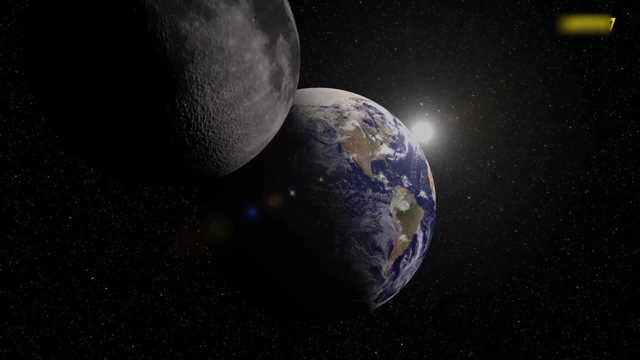 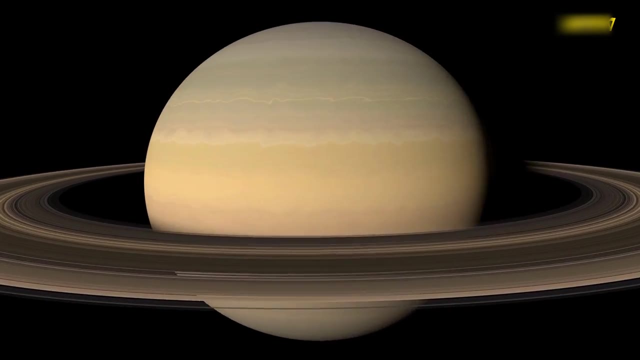 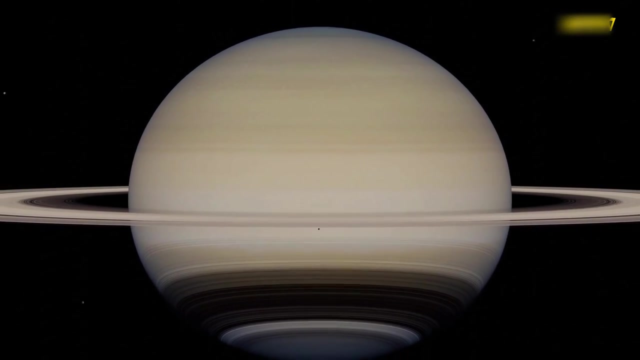 After 13 years of extraordinary encounters, the Cassini spacecraft had made its last fateful maneuver, plunging headfirst into the atmosphere of Saturn. 45 seconds later, the craft would be gone, crushed by the atmosphere of the planet it had spent over a decade so carefully exploring. 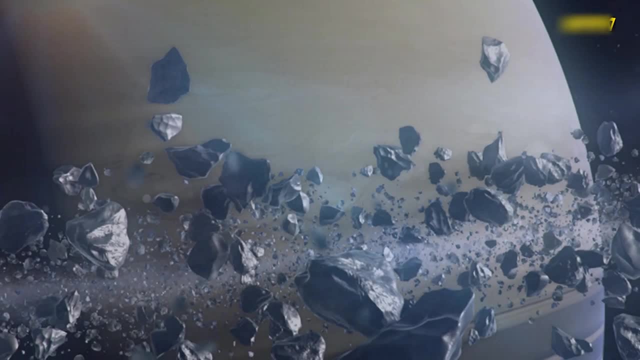 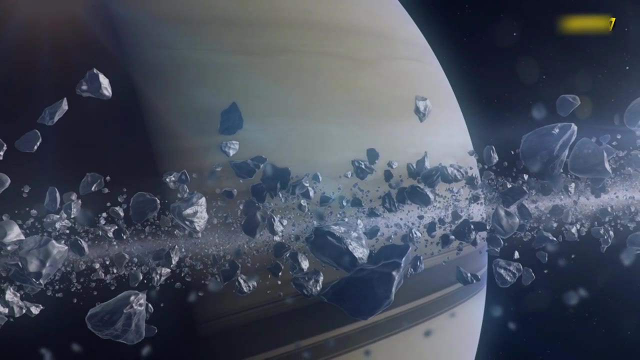 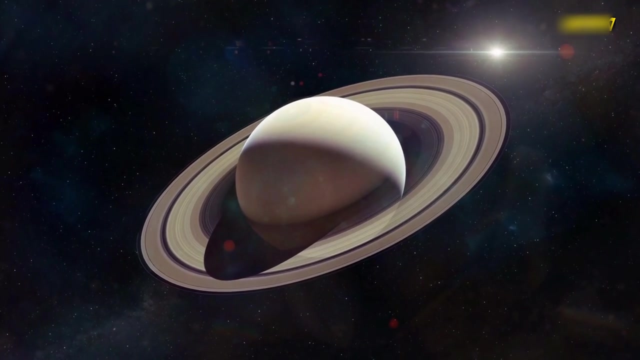 Its last image, a monochrome view of the planet's night side, lit by the reflected light of the rings, was a picture of its own grave, revealing the location towards which the spacecraft would plummet in its final act of self-destruction, as it entered the planet's atmosphere just a few hours later. 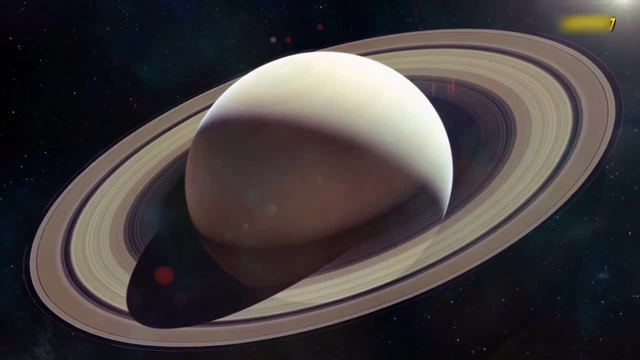 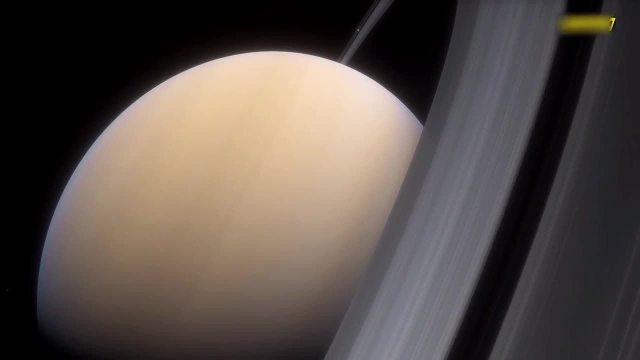 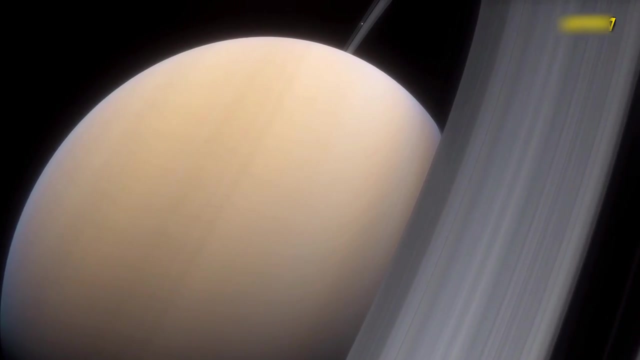 This was the end of a 20-year mission that had exceeded all expectations. The fourth spacecraft to enter the Saturnian system, following after Pioneer and the Voyagers Cassini, was the first to live there, ultimately spending 13 years and 76 days in orbit around Saturn. 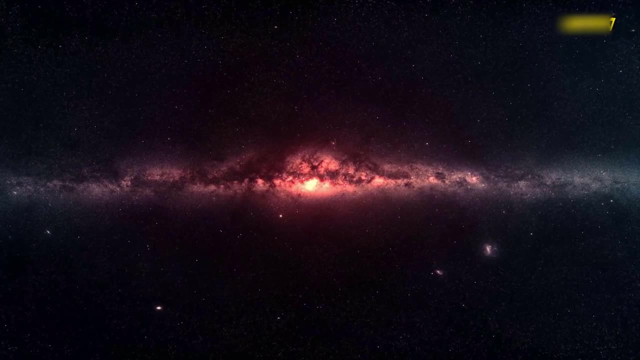 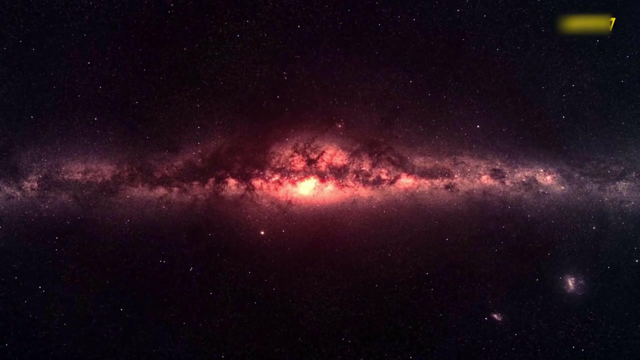 During this time, it explored the planet, its rings and its moons, and relayed images and information in a level of detail that would change our understanding not just of the Saturnian system, but of the whole solar system and our place within it. 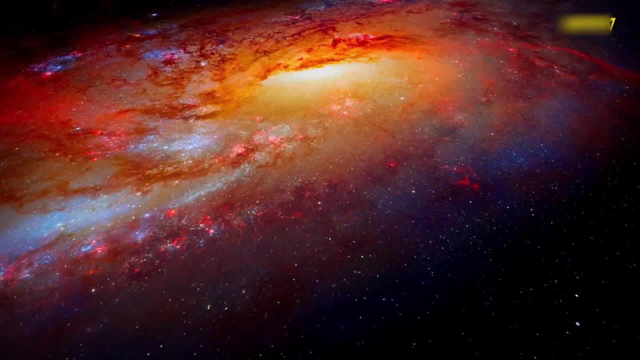 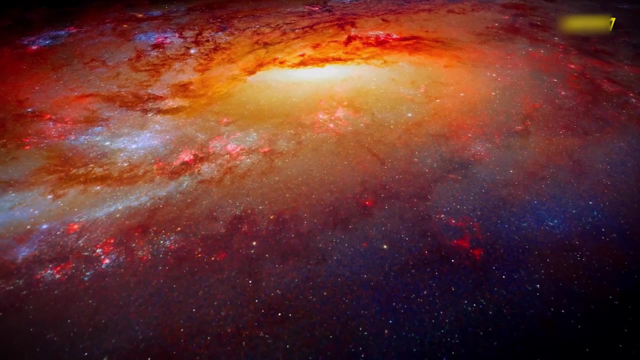 It all began on 15 October 1997 at Cape Canaveral, with the launch of the spacecraft aboard a mighty Titan IV rocket. To get to this moment had taken the best part of 15 years, the combined efforts of 28 countries. 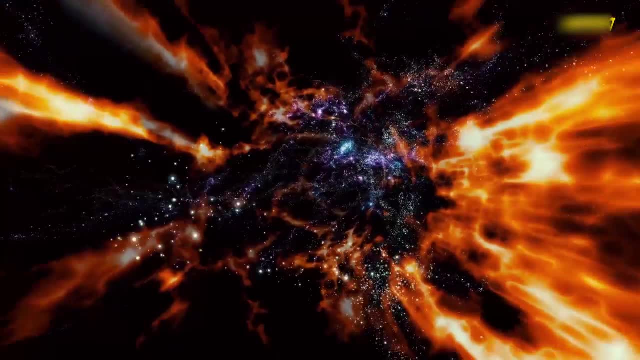 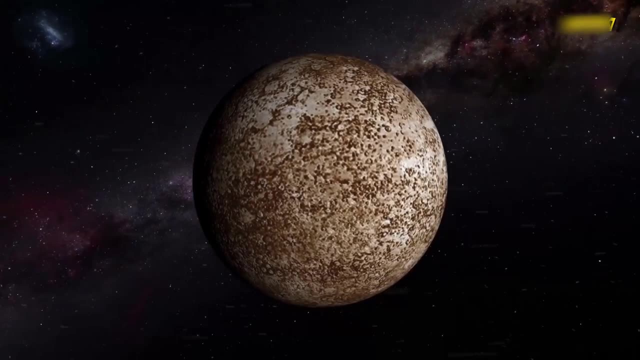 and a budget of $3.26 billion, But even then it would be another seven years before Cassini could truly begin its mission objectives. Getting this 5.5-tonne machine across 1.6 billion kilometres of space would require a complex trajectory. 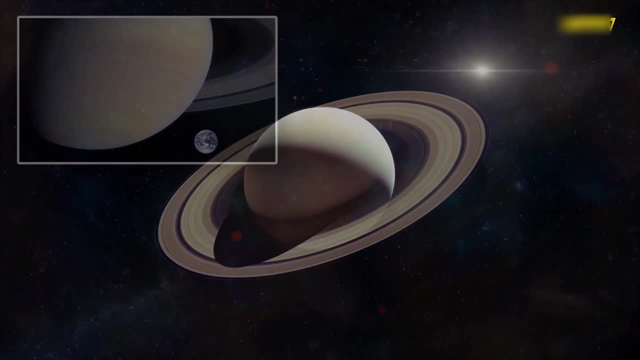 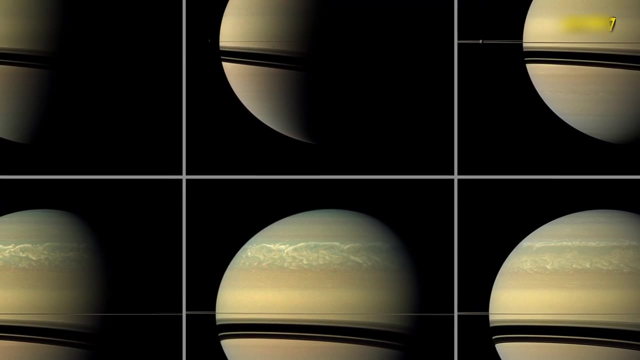 that would take it on two flybys of Venus and out to the asteroid belt before returning to the Earth two years after take-off for a final slingshot from its home planet. that would send the craft hurtling at speeds of 98,346 miles per hour. 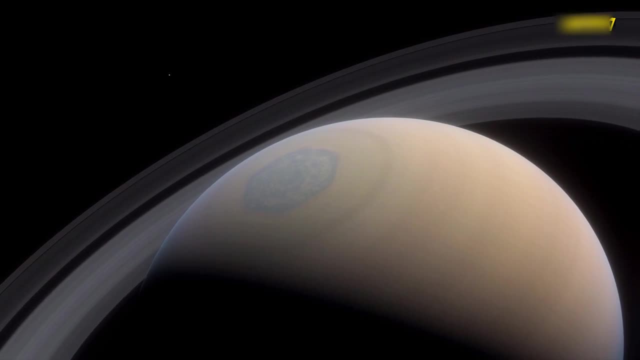 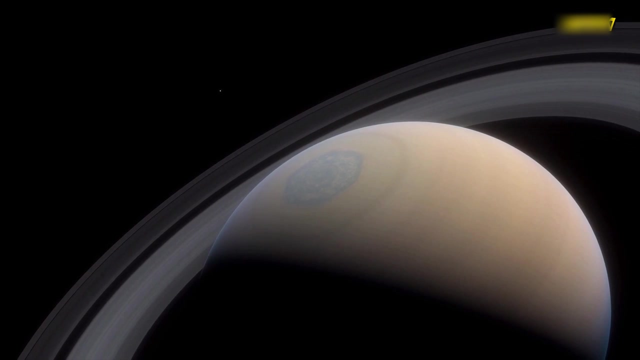 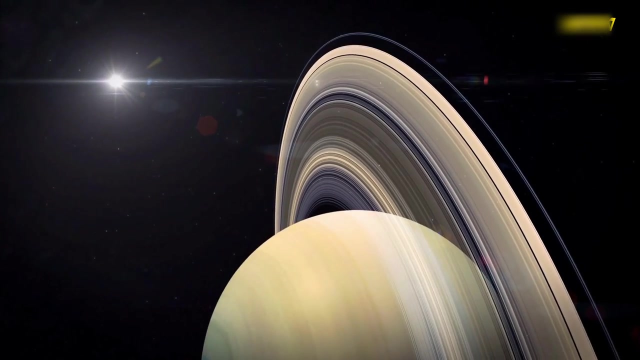 outwards, past Jupiter and on towards its final destination. This complex and high-risk trajectory was designed to exploit the orbital momentum of Venus, Earth and Jupiter to enable the spacecraft to accelerate, which helped keep the amount of fuel, and hence the launch weight, to a minimum. 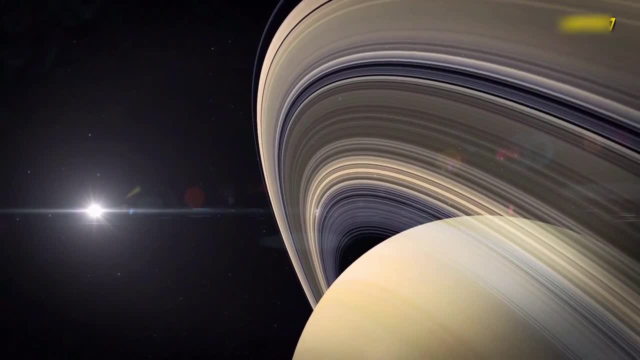 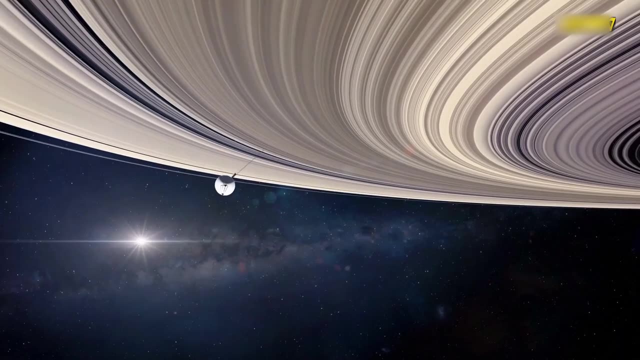 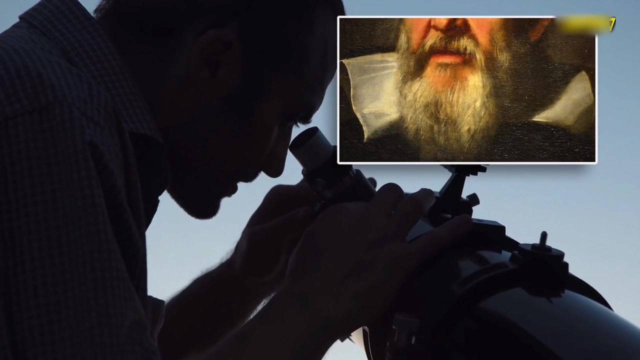 while making sure the craft could pick up enough speed to complete its epic journey. However, the trade-off of using this VVEJGA Venus-Venus-Earth-Jupiter-Gravity-Assist trajectory was a nervous six-year, 265-year and 61-day wait for the team back on Earth. 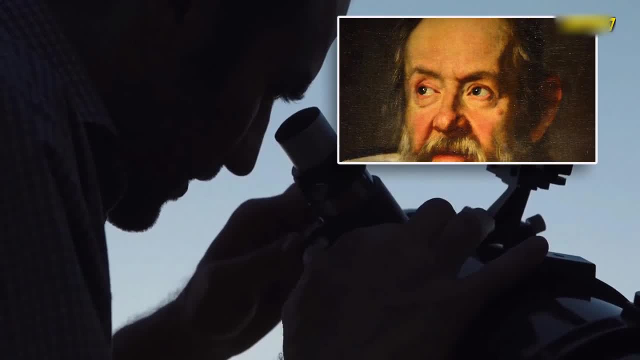 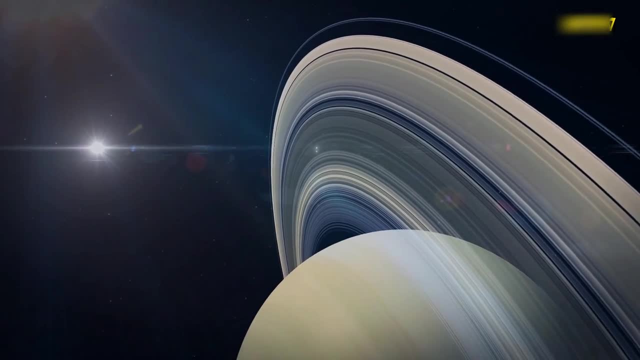 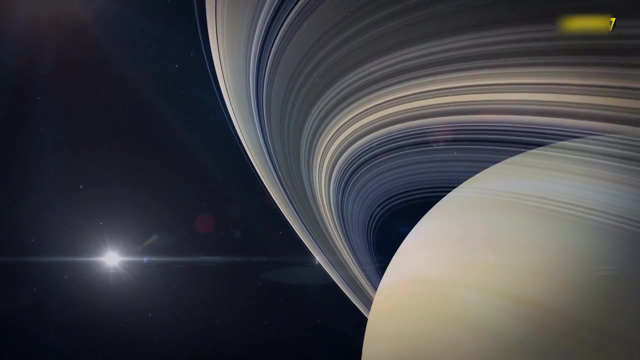 as the craft made its convoluted voyage across space Primary voyage complete, Cassini now faced the life-or-death challenge of slowing itself down with enough precision to enter orbit around Saturn. The tiniest miscalculation would have seen billions of dollars. 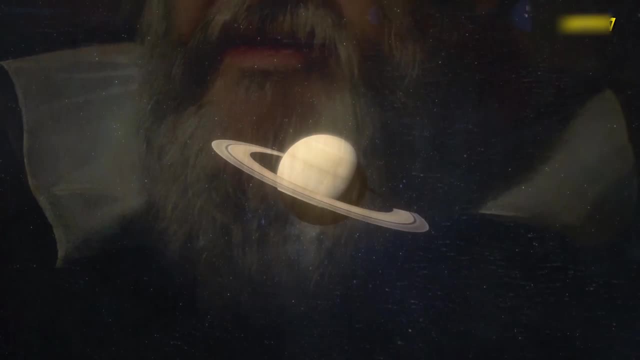 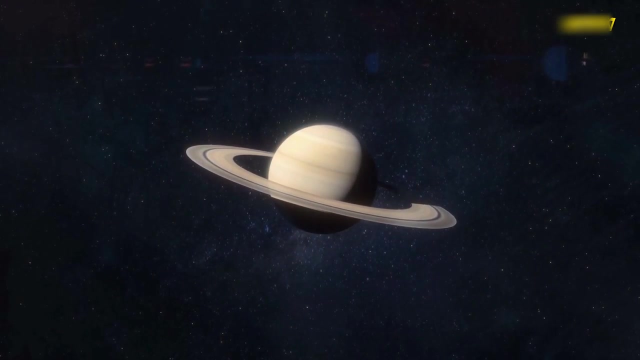 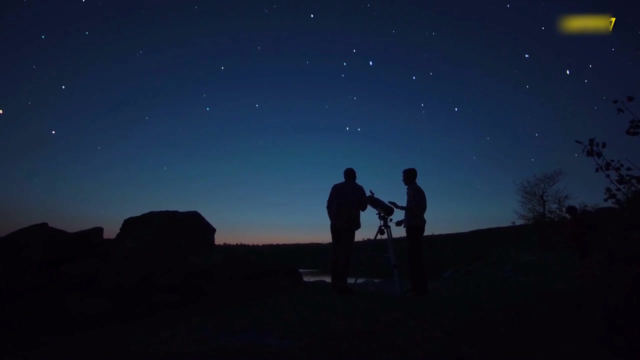 flung into the outer reaches of the solar system and decades of work lost forever. On 20th June 2004,, the spacecraft began its complex Saturn Orbital Insertion maneuver by flying through the gap between the F and G rings. This maneuver alone was not without serious risk. 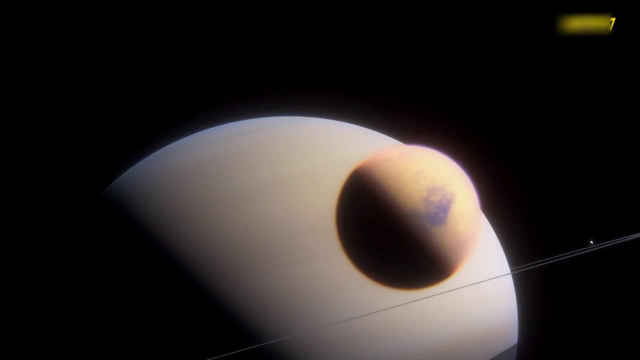 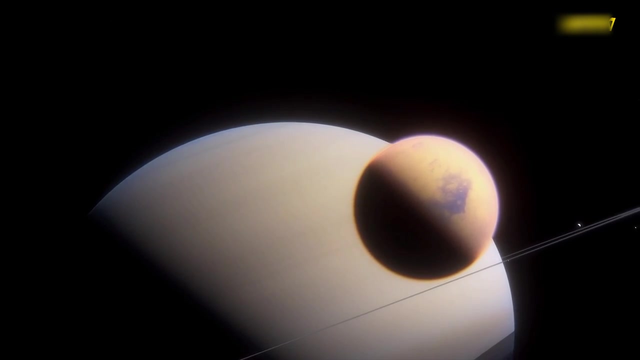 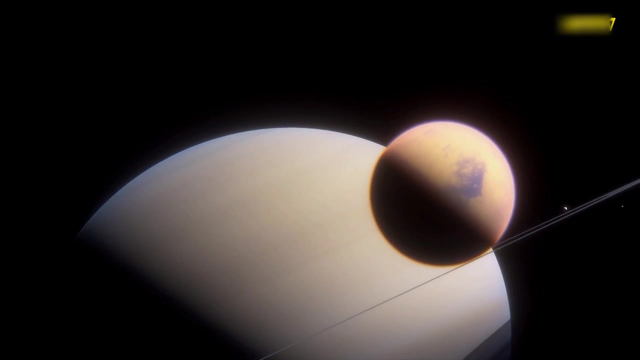 from the potentially devastating impact of particles in the rings colliding with the craft. so Cassini had to carefully orient itself to protect its instrumentation. Once through the ring plane, the spacecraft had to rotate itself once again to point its engine directly along its flight path. 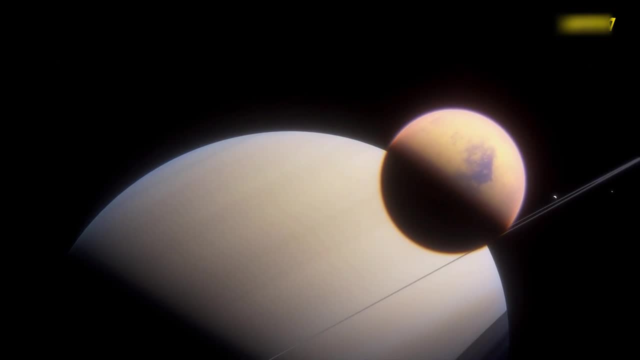 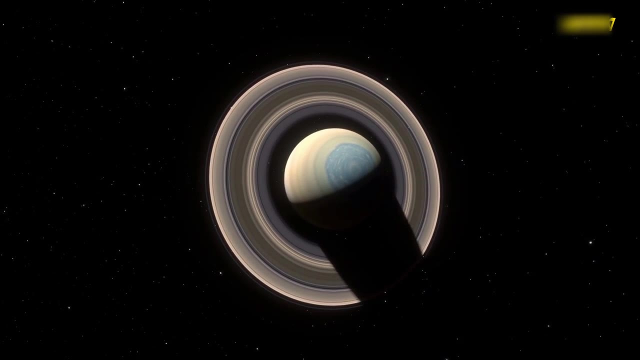 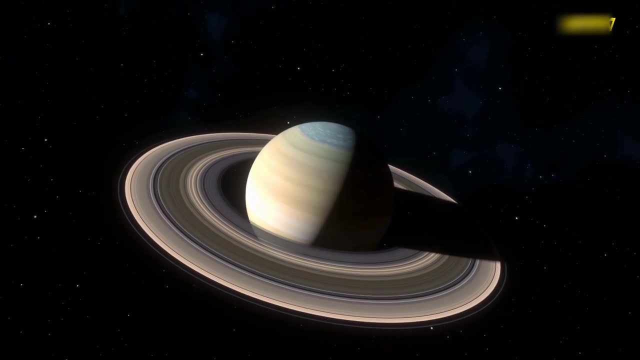 so that when the engine fired, it would decelerate the craft by a precise velocity, 622 meters per second, allowing it to fall into the gravitational hand of Saturn. Decelerate too much and the craft would fall into Saturn Too little and it would fly off into outer space. 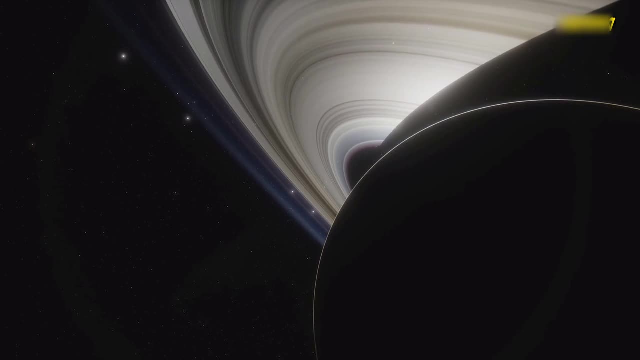 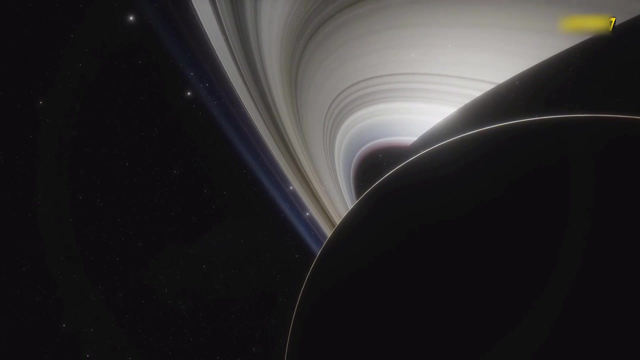 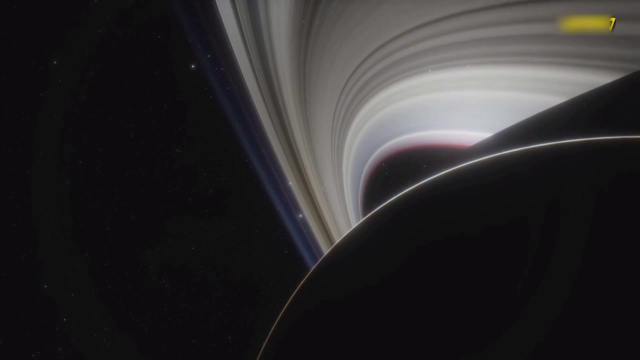 At 8.54 pm PDT, Cassini was finally captured by the gravity of this gas giant, becoming the first spacecraft to ever orbit Saturn. A new age of exploration had begun And over the next 13 years, Cassini would provide an extraordinary return on investment. 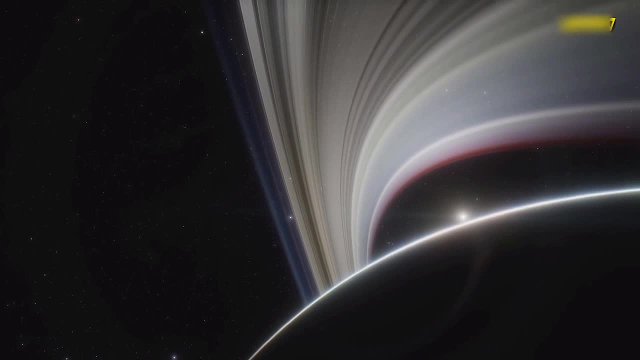 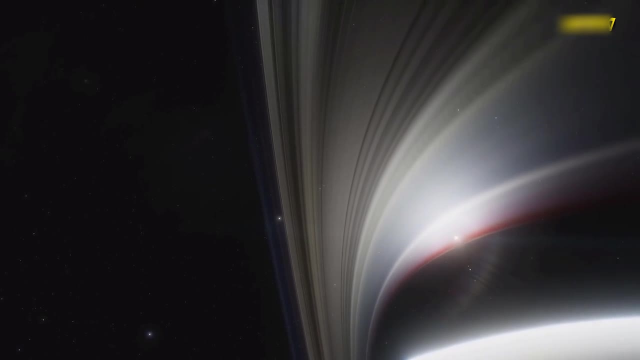 The Voyagers and Pioneer had given us our first rough glimpses of Saturn's moons, but during its 13 years in orbit round the planet, Cassini did so much more. Not only did it discover a whole host of new moons, it also helped solve countless mysteries. 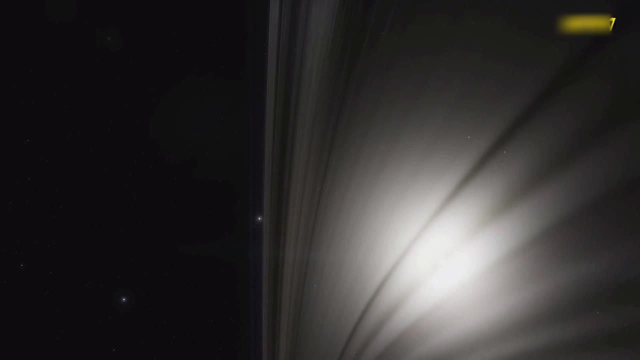 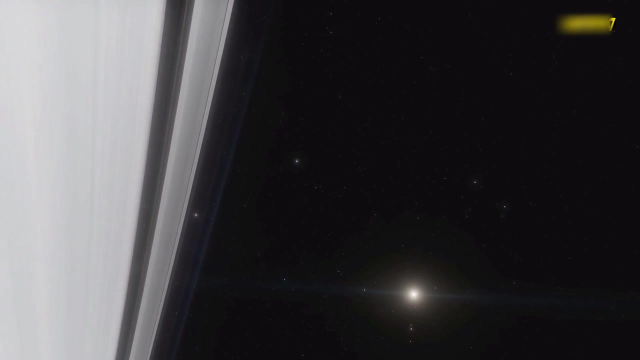 around moons we already knew existed, such as Titan and Enceladus, and revealed just how varied the characteristics of the 60-plus moons of Saturn really are. Cassini also allowed us to study for the very first time the interactions between Saturn's menagerie of moons. 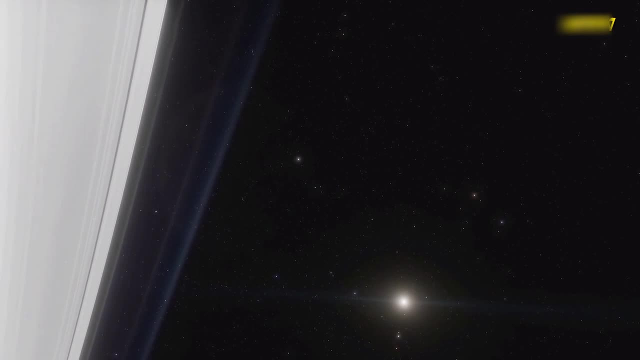 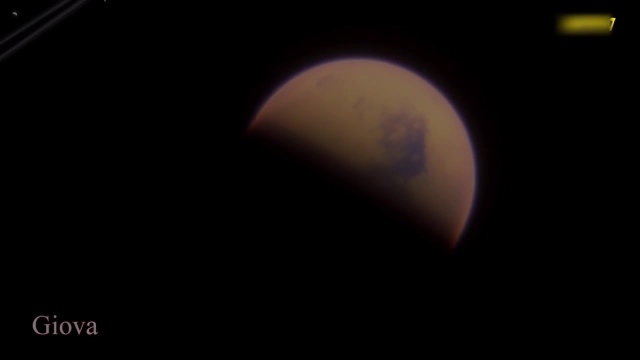 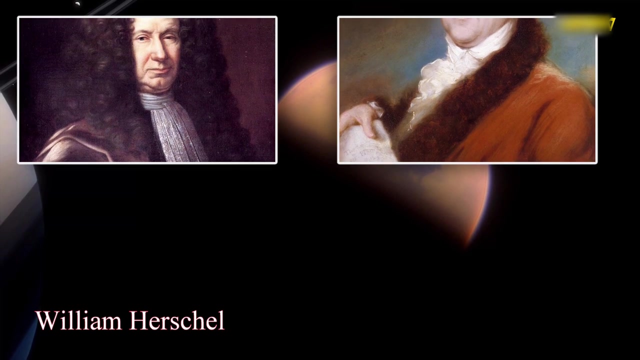 and the ring system within which they sit, as well as the structure and history of the ring system itself. One of Cassini's key mission objectives was to explore the characteristics and activity of the vast atmosphere that makes up most of Saturn. Voyager 2 had revealed the presence of a heat source. 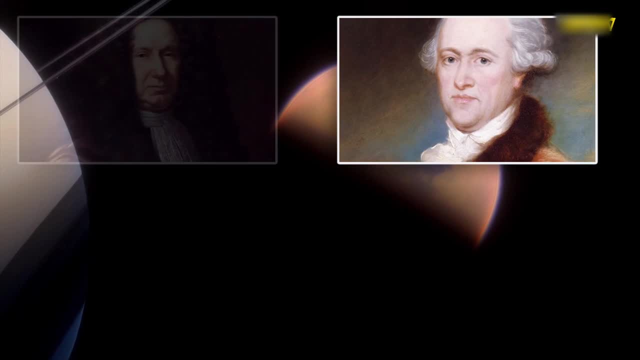 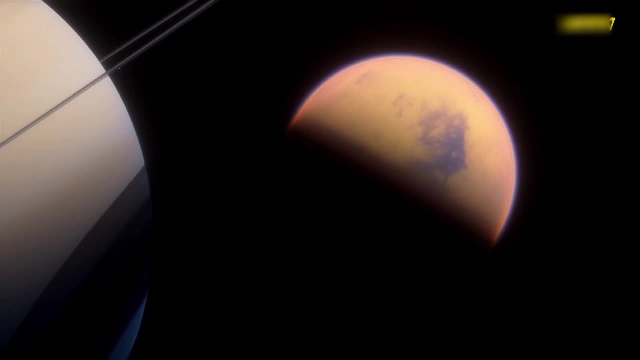 buried deep beneath the planet's cloud tops that seemed to be producing vast amounts more energy- up to 87% more, in fact- than the planet absorbs from sunlight. But what was the source of this heat, And how did Saturn's immense atmosphere? 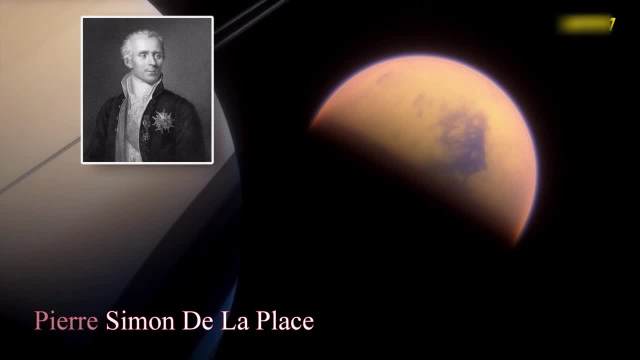 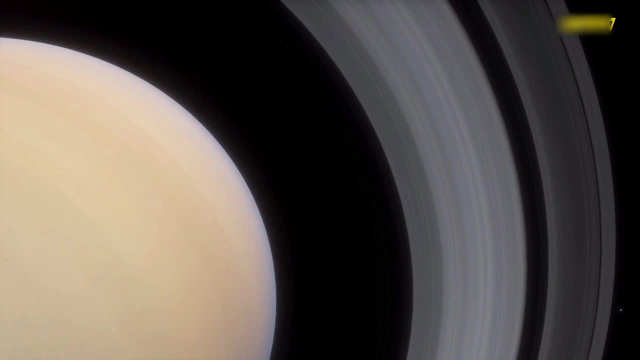 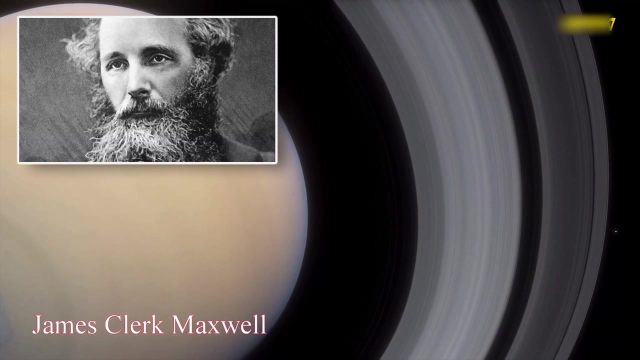 organise itself into the vast and intricate weather systems like the huge hexagon. This remained a question that Cassini was charged with solving. Atmospheres can be some of the most spectacular and complex environments found on any planet, from the crushing intensity of Venus's choking atmosphere. 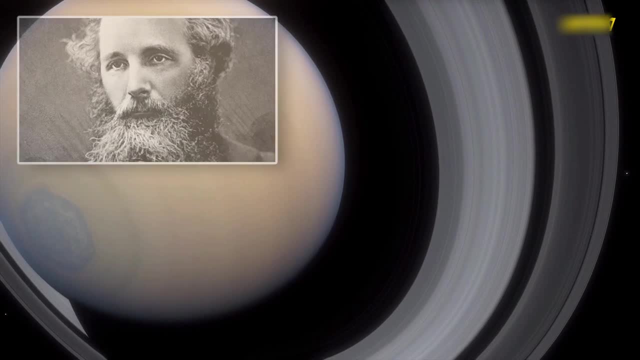 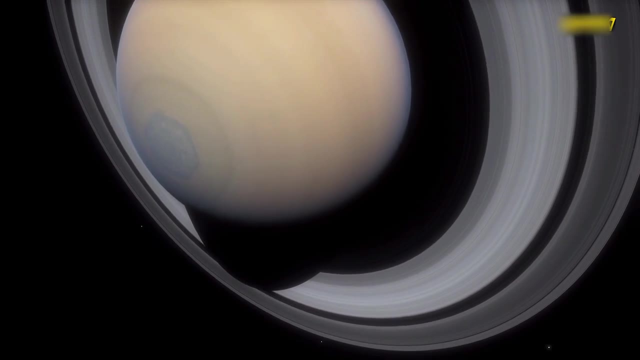 with its raging winds and sulphuric acid rain, to the thin blue line of Earth, where, even on our somewhat milder planet, we see endless storm systems In the inner solar system, the atmospheres of the rocky planets and the weather systems they contain. 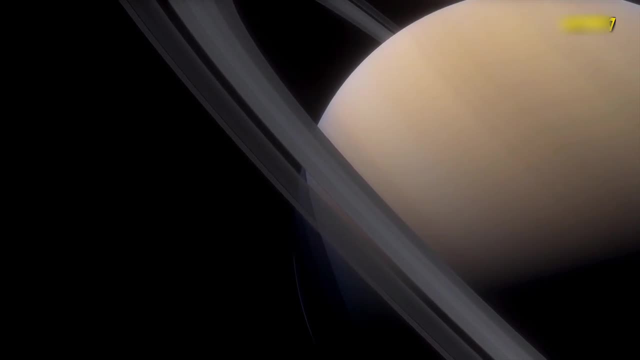 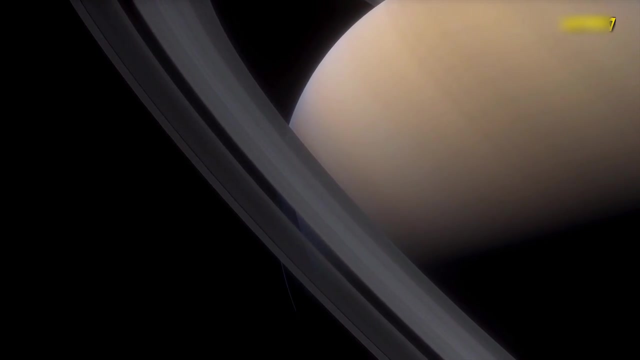 are all powered by a single source: the relentless heat of the sun. All the weather we see on the rocky planets, whether it's a dust storm on Mars or a hurricane on Earth, are driven by the same simple process. It begins with the sun beating down onto the planet's surface. heating the ground, which in turn radiates back, heating up the air closest to it. That air expands, which means it becomes less dense, and so the hot air closest to the ground rises. The result of all this rising air is that you get thermals. 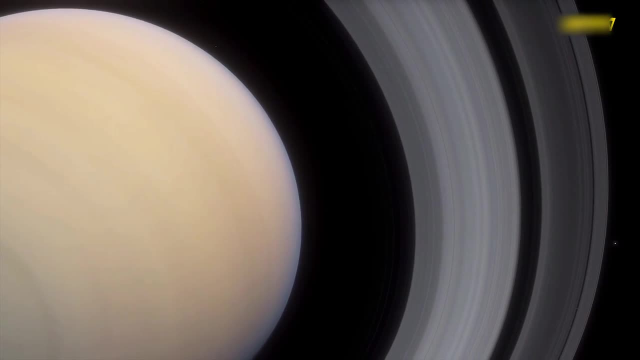 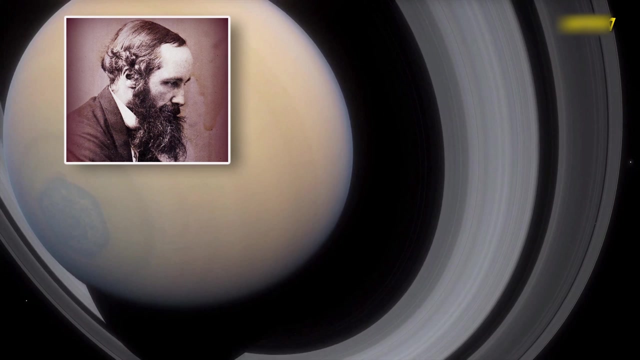 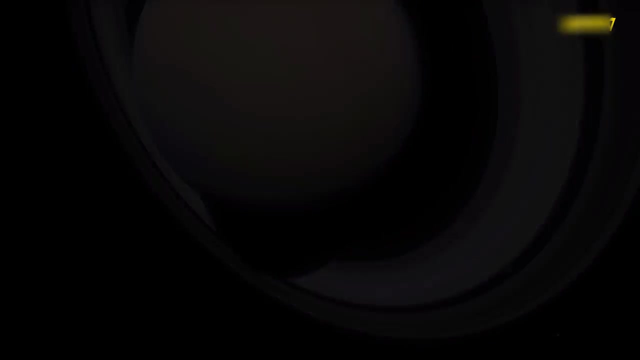 energetic movement of air from the ground into the upper atmosphere Over the oceans. exactly the same process occurs with the heat of the sun evaporating vast amounts of water and lifting it up into the atmosphere. So, in the very simplest terms, all of the extraordinary weather systems. 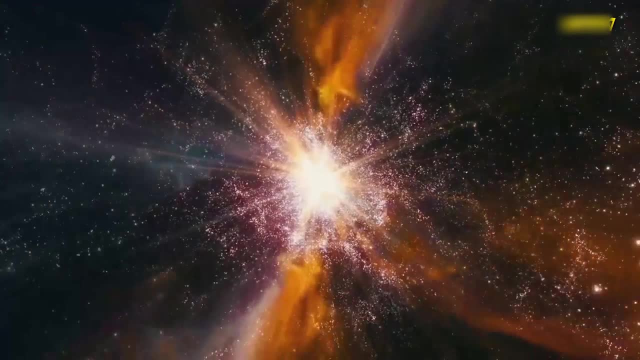 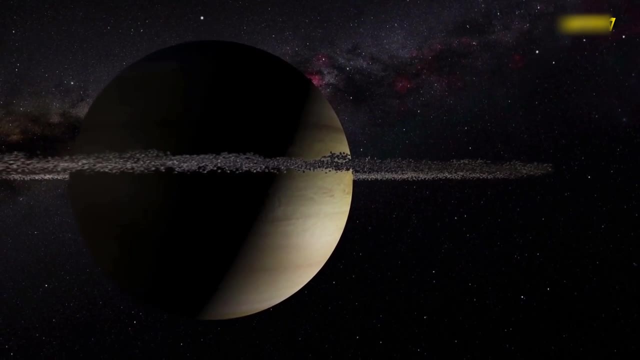 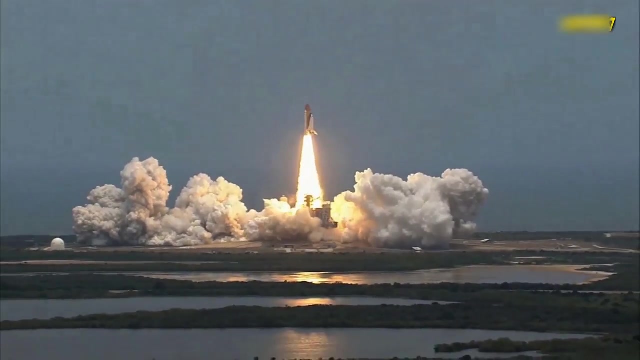 we see on Earth or any of the other terrestrial planets, is driven by the sun, heating the land and sea and causing the air to move around, Travel further out into the solar system, however, and the character of any atmosphere radically changes. The storms on Saturn are among the most violent. 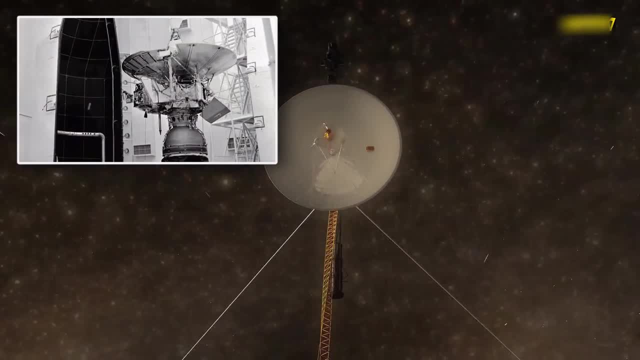 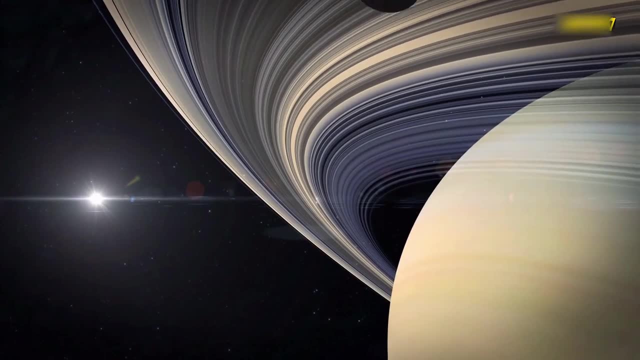 found anywhere in the solar system, Generated by rich, complex and powerful weather systems. we've been witnessing these giant storms from afar for almost 150 years. Asaph Hall, the great American astronomer and discoverer of the two moons of Mars. 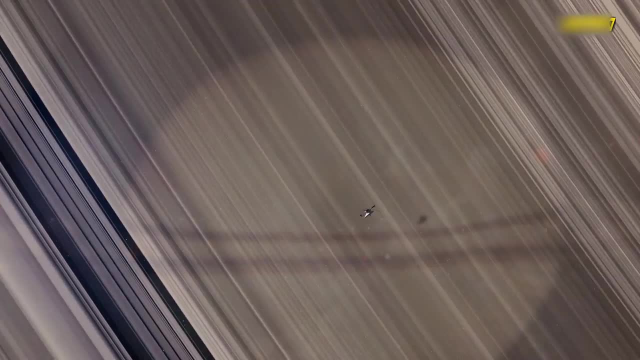 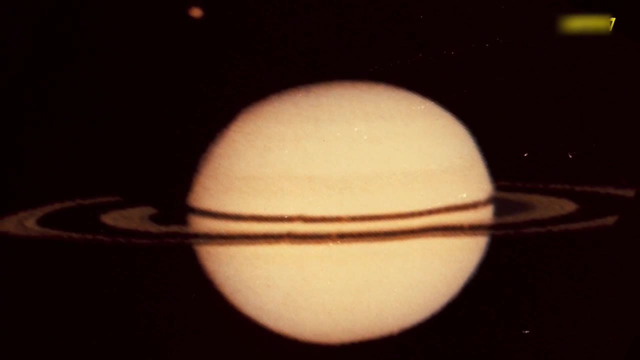 was the first to observe one of these storm systems back in 1876.. Looking through the largest refracting telescope of the time, the United States Naval Observatory's 66cm telescope, located in Washington DC, he was able to make out a great white spot. 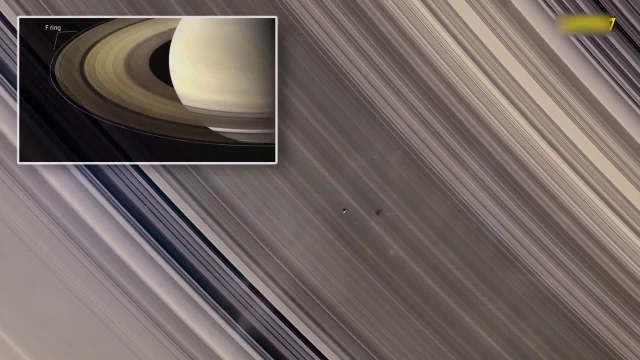 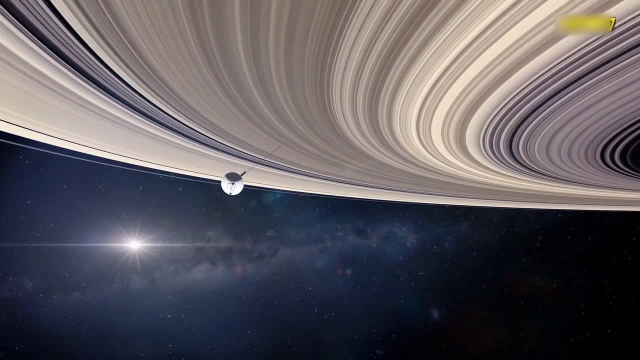 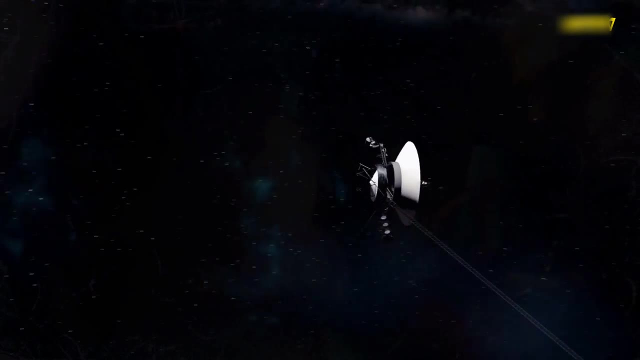 sitting in the northern hemisphere of the planet. At the time, Hall wouldn't have known much at all about the phenomenon he was looking at. It was intriguing simply because it enabled him to make the first estimate of the rotational period of the planet Over the following decades. however, 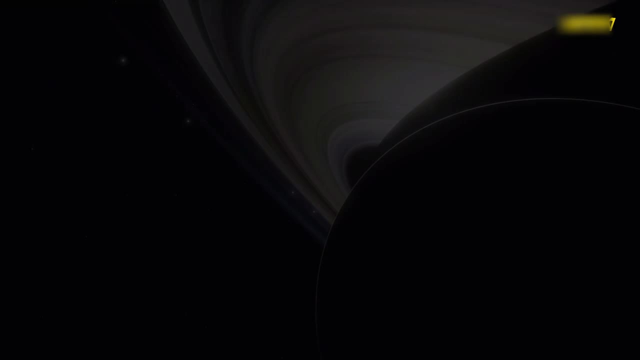 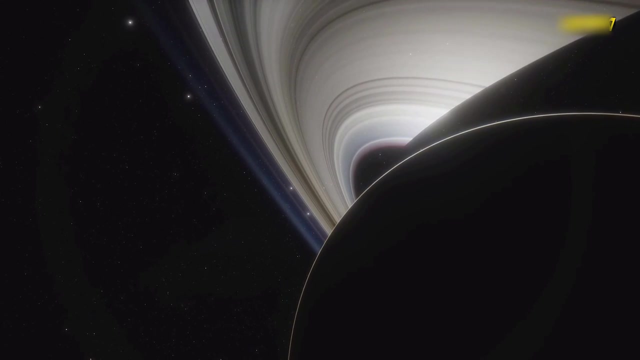 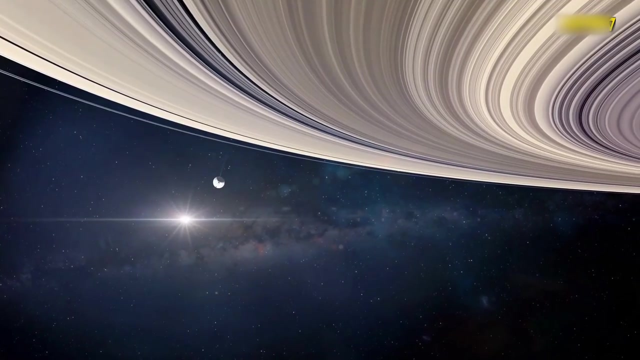 this great white spot was observed again and again, roughly falling into an appearance every 20 to 30 years before slowly fading away. Fortunately for us, the long gaps between each appearance were cut short in December 2010,, when a great white spot appeared just four years after the previous one. 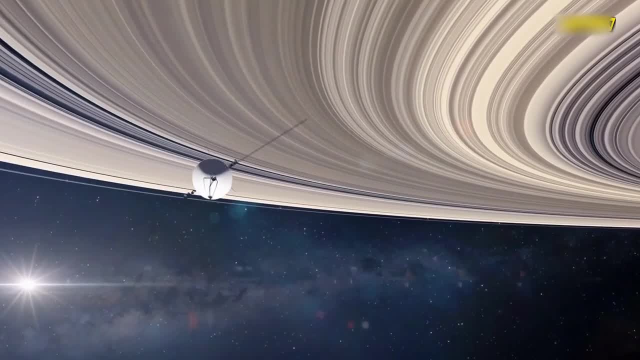 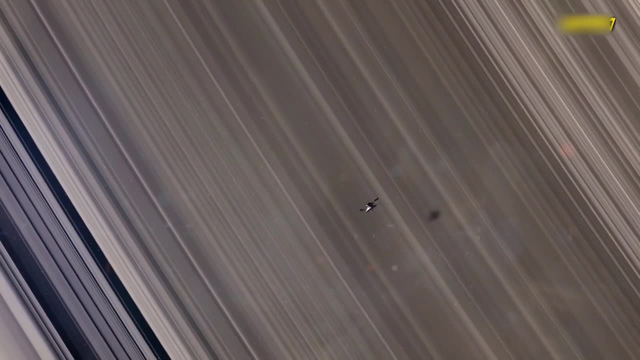 This time with the Cassini probe in orbit. we had the opportunity to track the evolution of one of these storms close up, from its birth in early December 2010 to its disappearance eight months later. This vast storm system, resembling in many of its characteristics- 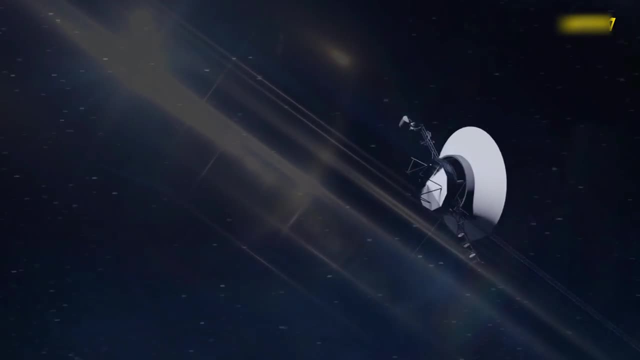 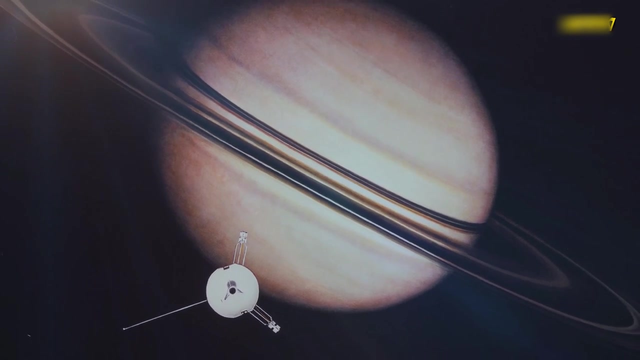 a simple thunderstorm here on Earth emerged as a single white spot, 1,300 km from top to bottom and 2,500 km from bottom to top. Over the ensuing months, Cassini was able to follow the storm as it stretched out around the planet. 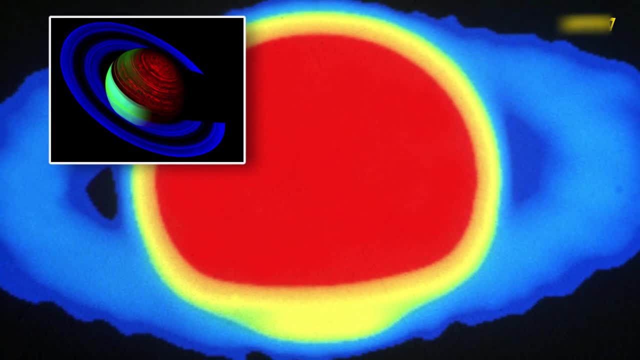 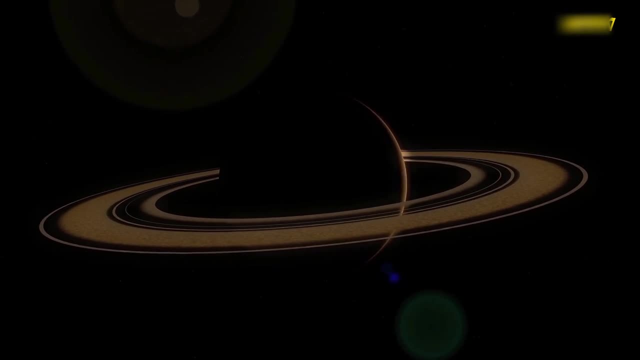 Just a few weeks after its formation, the tail of the storm had extended across 100,000 km, And within six months this great storm had stretched so far it encircled the whole planet. Cassini was able to image directly for the first time. 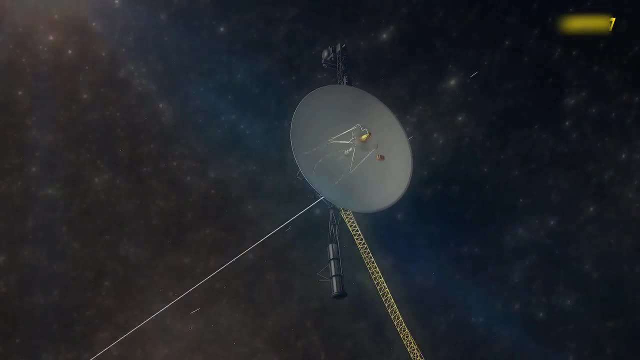 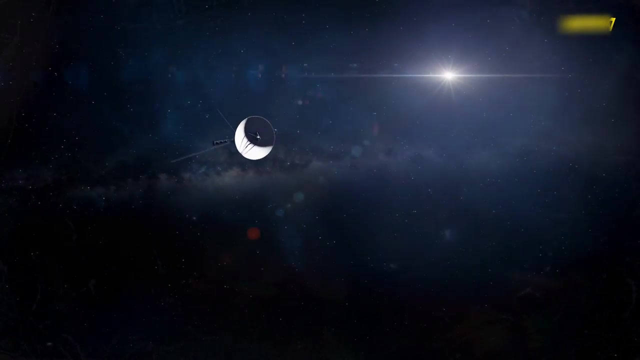 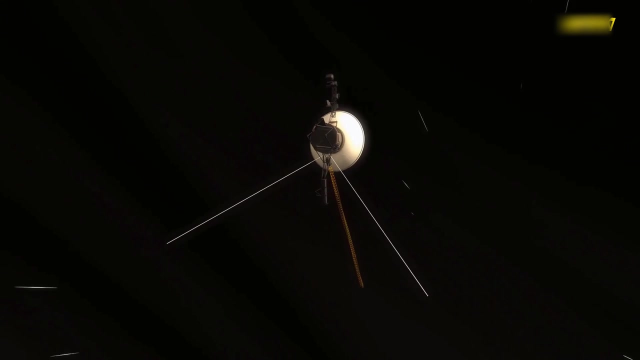 lightning occurring in the middle of this giant storm. The storm was so strong it was almost impossible to imagine the scale of this giant storm in broad daylight. The fact that the lightning could be detected on the day side of the planet surprised the Cassini team. 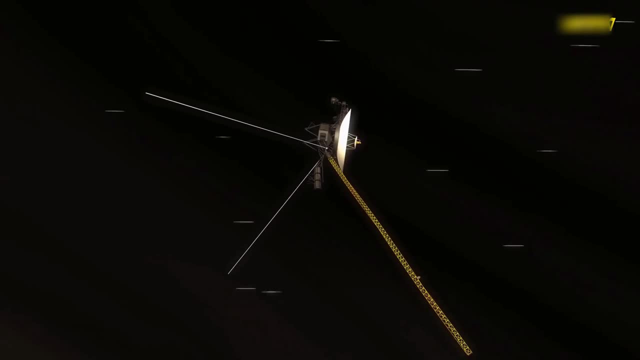 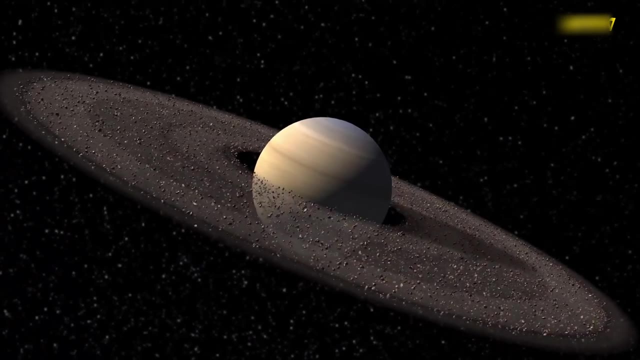 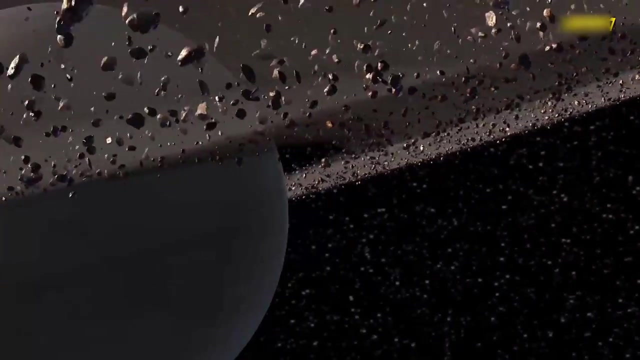 and suggested that the lightning must be particularly intense to make it visible. in such bright light The lightning flashes are comparable to the strongest lightning flashes that we see on Earth. That was a joy just to finally witness lightning on Saturn, And we could tell that it was coming from the cloud layer. 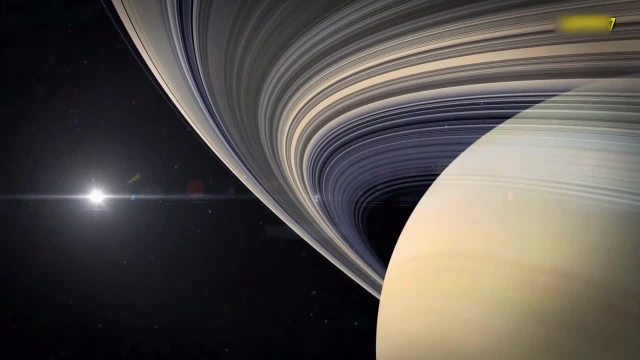 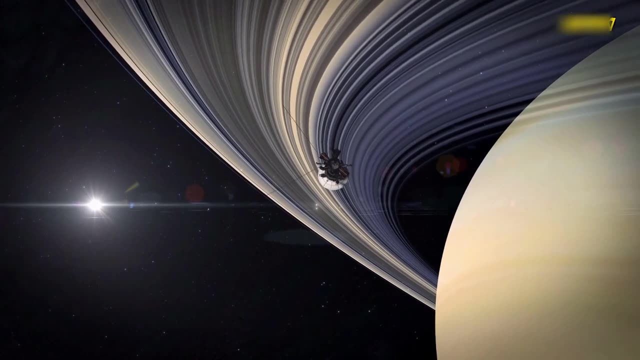 the deepest cloud layer, which is about 60 miles down, and is the water cloud, the water-ice cloud. And that makes sense, because lightning is produced on Earth because of updrafts and particles being elevated through an atmosphere rising, through an atmosphere, because they're convecting. 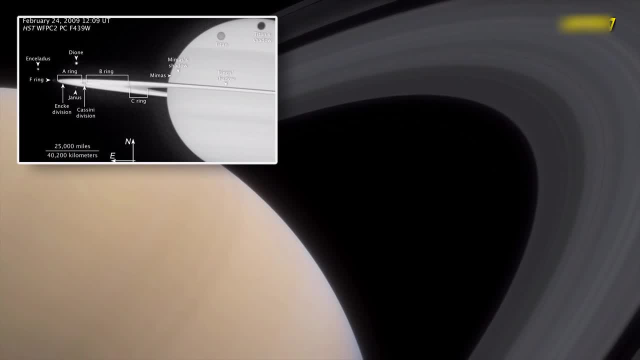 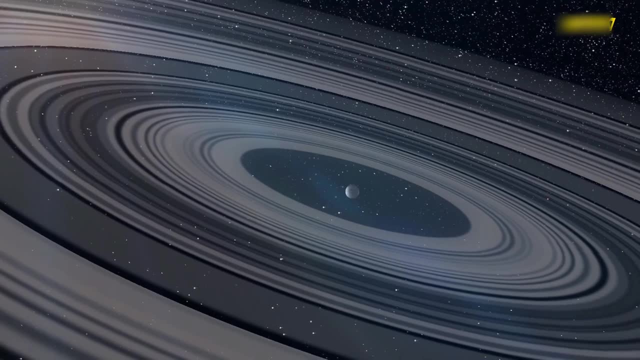 We had a whole variety of scientific goals at Saturn and one of the main ones was to understand the meteorology of the Saturn atmosphere and what energizes the winds that we see on it and so on, And we have affirmed now the belief that the atmospheric systems on Saturn 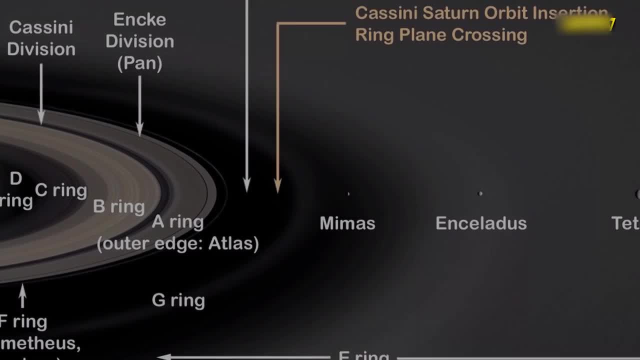 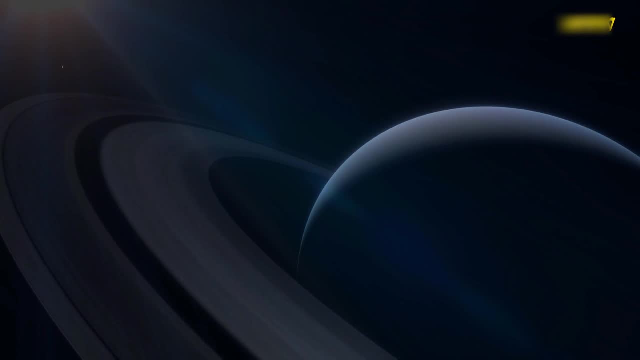 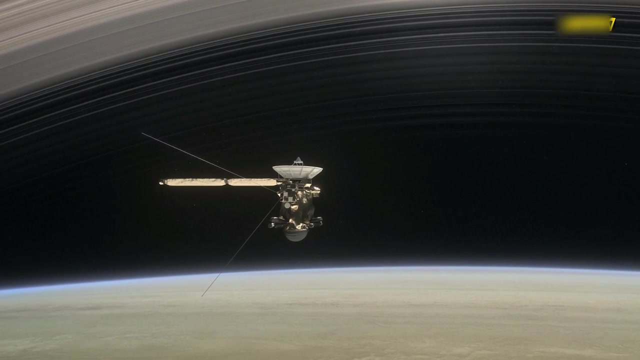 are actually powered by energy from below, from an internal source on Saturn. They're not powered by sunlight like we have on Earth. Carolyn Porco Cassini mission Cassini was also able to turn its cameras onto the giant hexagon structure that Voyager 2 had first photographed over 30 years before. 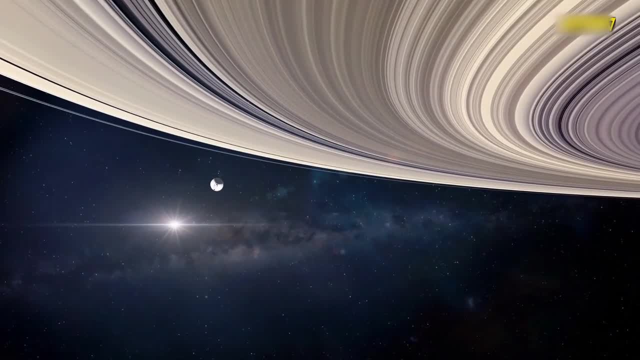 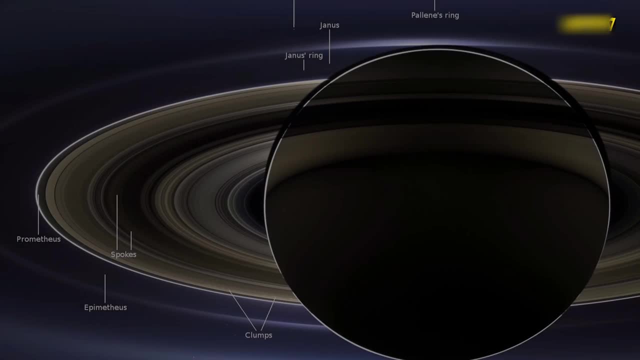 This time with its high-definition narrow-angle cameras trained on the enormous feature around the North Pole of the planet, Cassini was able to capture the giant hurricane-like storm in extraordinary detail. This vast vortex was measured as 2,000 kilometres across. 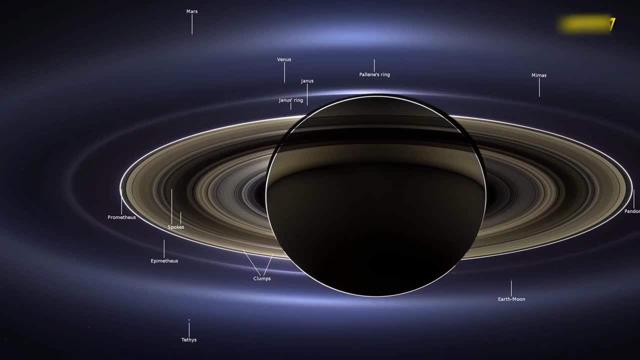 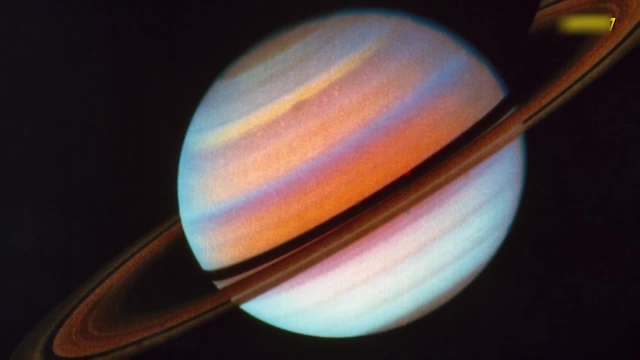 at just the eye of the storm And with cloud speeds travelling at over 150 metres per second, it's rotating far faster than any hurricane we've ever seen on Earth. Exactly what causes this or any of the giant storm systems we've witnessed on Saturn? 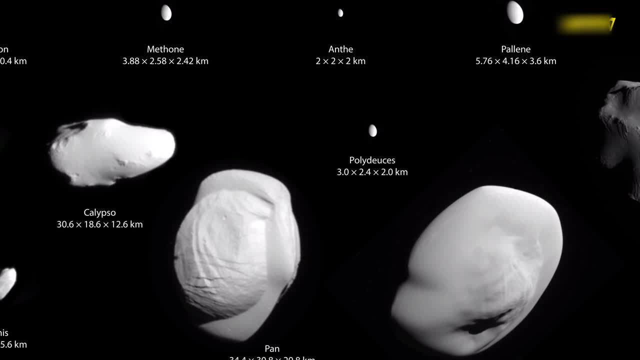 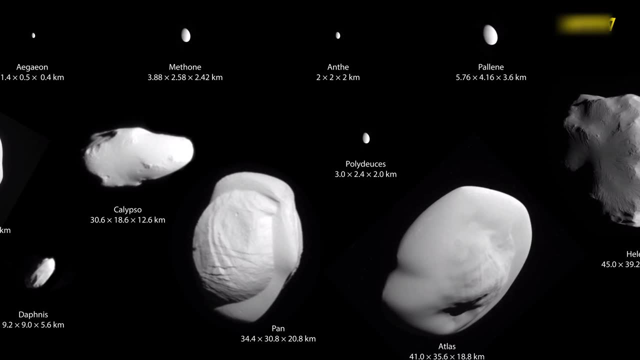 is still not fully understood, But one thing we absolutely know is that, this far out from the Sun, these weather systems cannot be driven primarily by the Sun's heat. With Saturn receiving 100 times less of the Sun's energy than Earth, something else must be driving its weather. 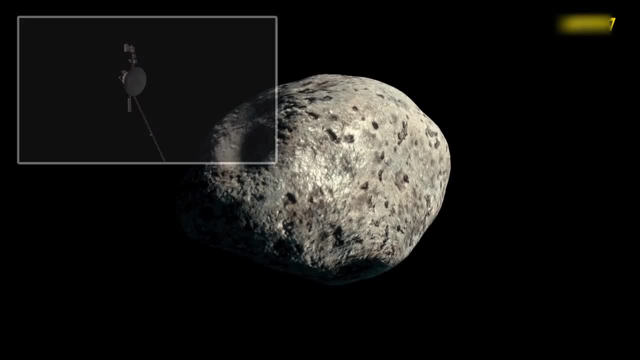 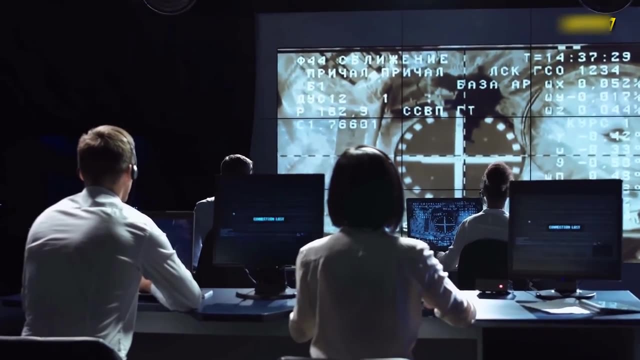 something that creates the same great upswellings of heat we see on Earth, but that on Saturn is entirely generated from the interior of the planet. As yet we've not been able to peer deep enough into Saturn's interior to see directly what happens inside this strange vortex. 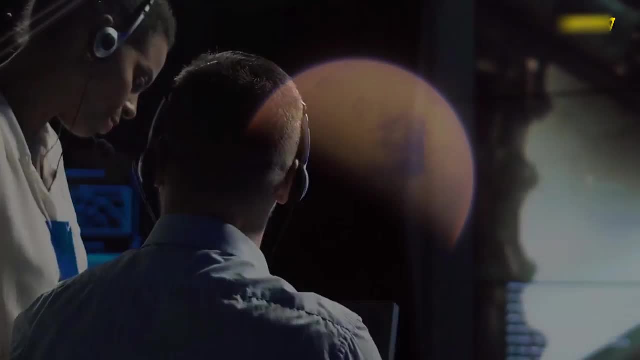 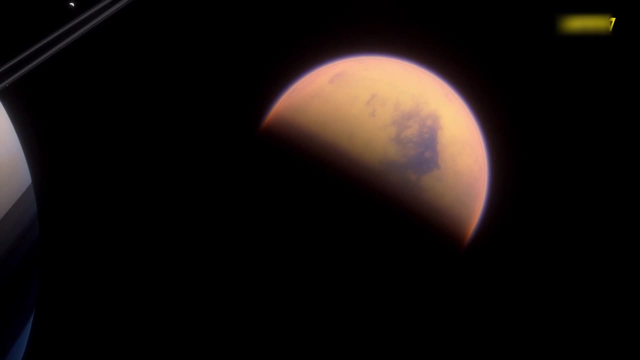 But in the last couple of years we've come closer than ever. As we've accumulated evidence from Pioneer, Voyager and, of course, Cassini and combined it with our increasingly sensitive ground-based observation, we've been able to start piecing together. 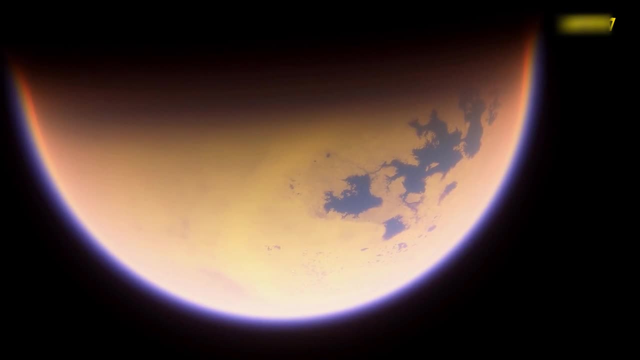 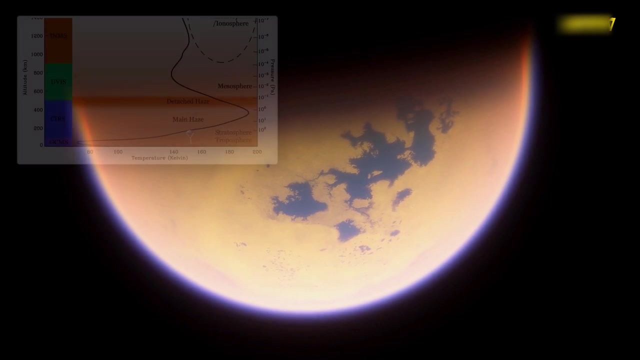 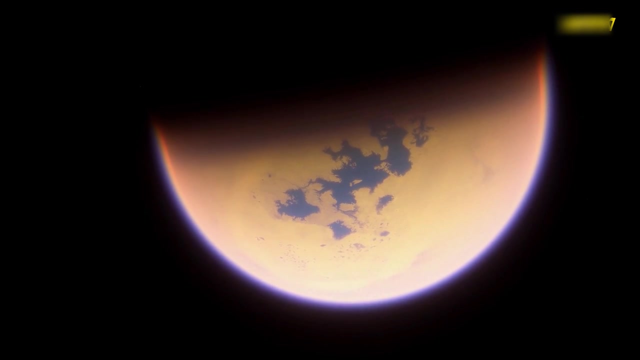 a detailed journey into the heart of the planet. By just touching the cloud tops of Saturn, alive with great storm systems and flickering with immense bolts of lightning, they have given us the first hints into the truly strange world that must lie beneath and the mysterious energy source that brings this planet to life. 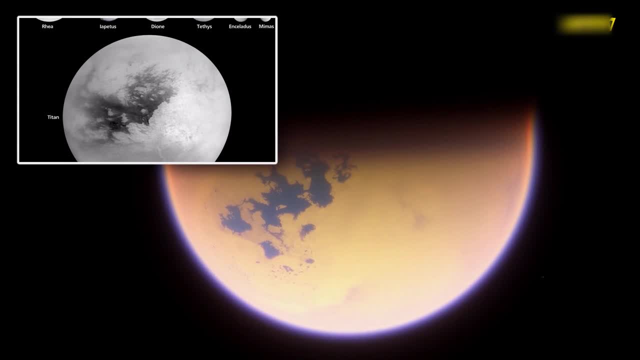 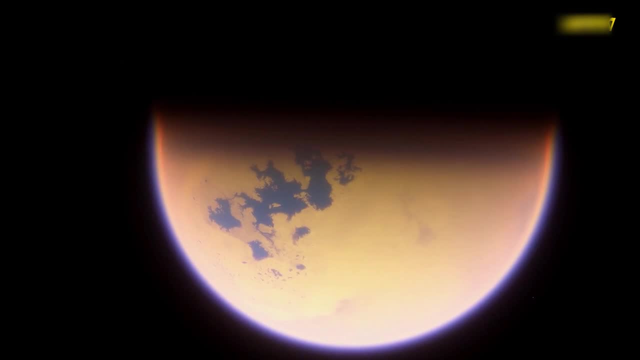 Our journey deep into the interior of Saturn begins not with clouds, but with rain At the very outer edges of its atmosphere. in the space between the closest ring, the D-ring, and the planet itself, we've discovered the phenomenon of ring rain. 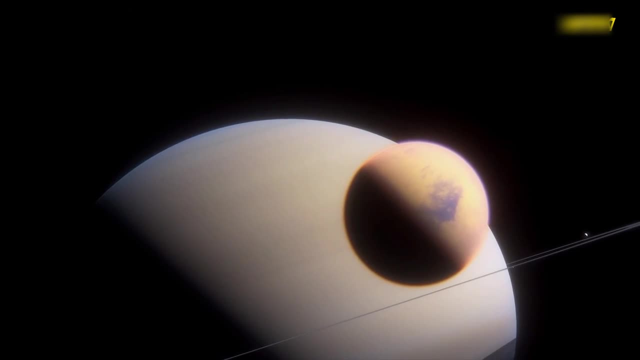 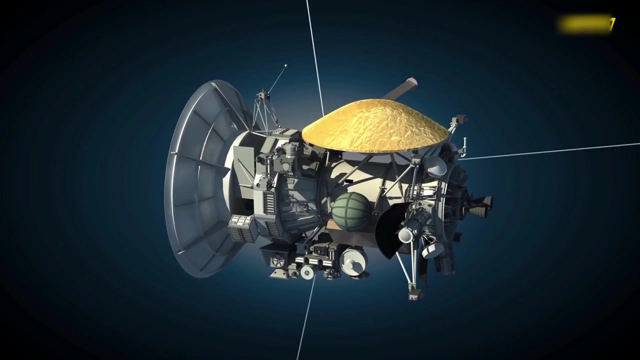 an endless downpouring of material falling from the rings into the upper atmosphere of the planet below. We know this because, as Cassini took its final fatal plunge on 15th September 2017, it flew through this uncharted no-man's land. 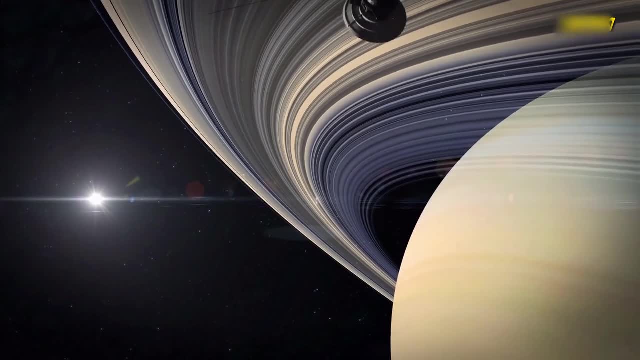 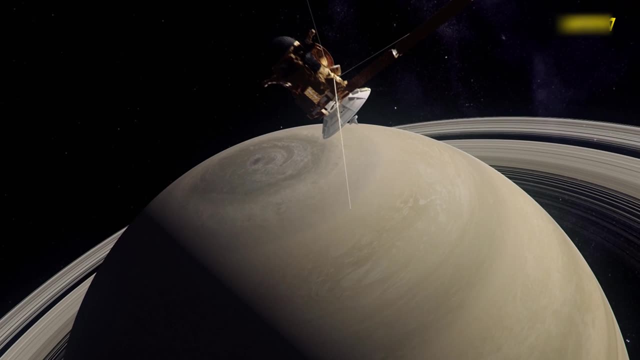 and was able to make the first direct measurements of the rain falling from the rings. Using the ion and neutron mass spectrometer, it measured the rate at which the rain was falling from the rings: a staggering 10,000 kilograms of material every second. 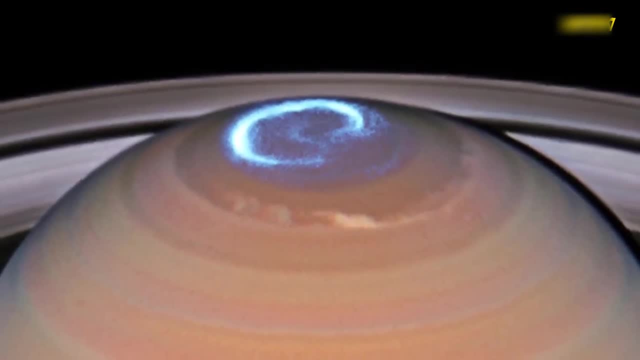 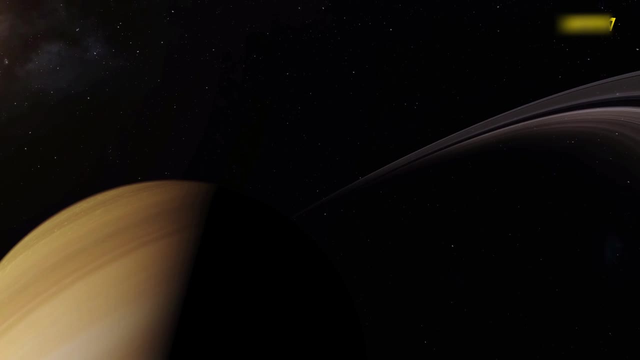 It was also able to reveal that the ring rain is comprised of a mix of hydrogen, water, ice and a surprising quantity of complex organic compounds like butane and propane, all showering down onto the planet and changing the chemistry of its upper atmosphere. 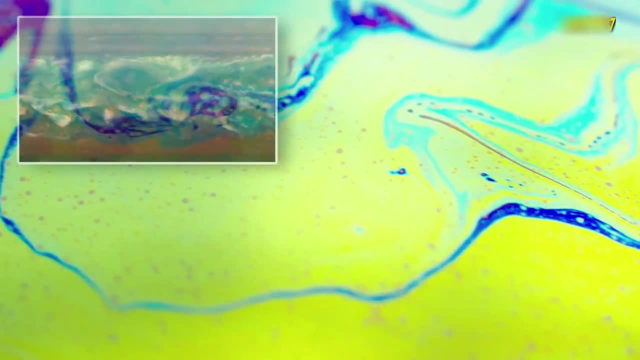 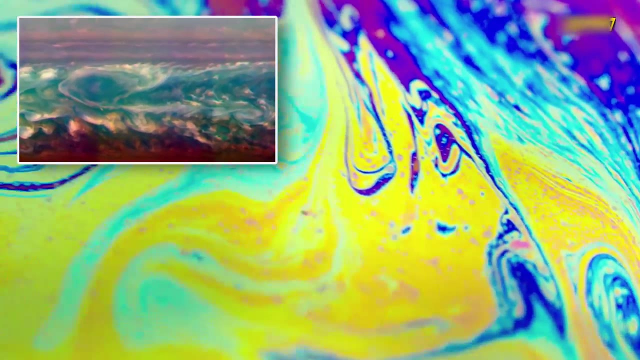 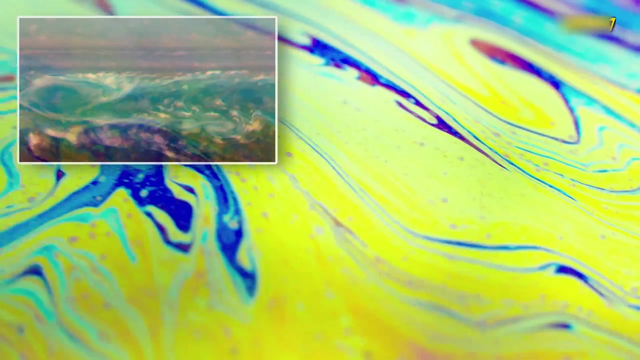 in ways we are only just beginning to understand. Cassini then began its final historic dive into the upper atmosphere of Saturn, struggling to keep its antennae pointing towards the Earth as it was buffeted by the rain, The increasing turbulence, while continuing to send a stream of precious data back to us. 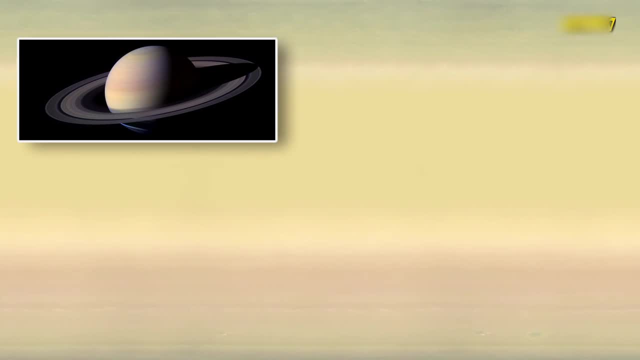 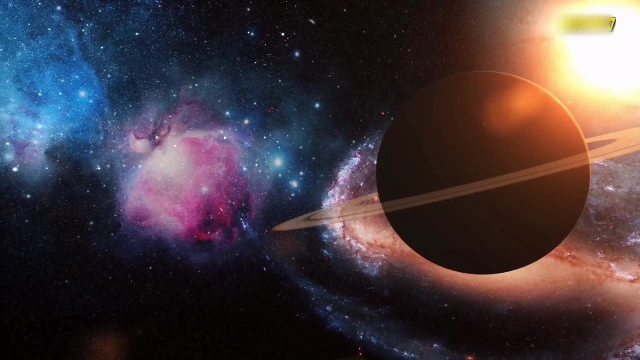 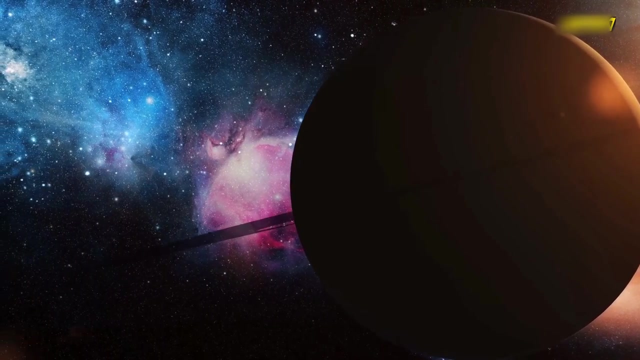 right until the very end. Travelling at around 123,000 kilometres per hour, Cassini entered Saturn's upper atmosphere at 3,3050 PDT, 1,900 kilometres above the planet's cloud tops. This was the first time scientists had ever been able. 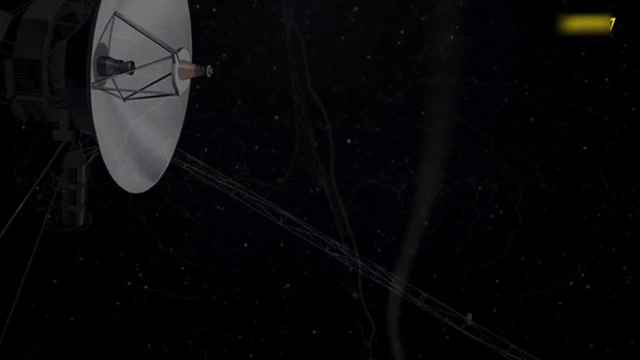 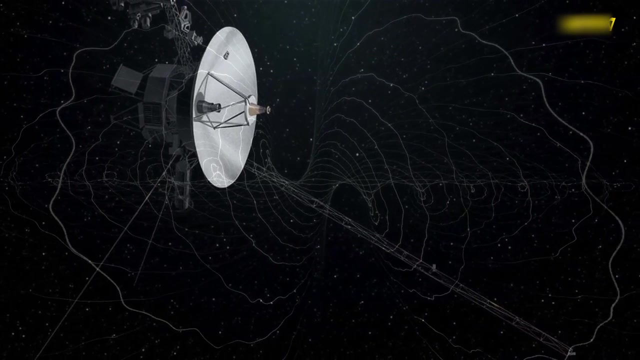 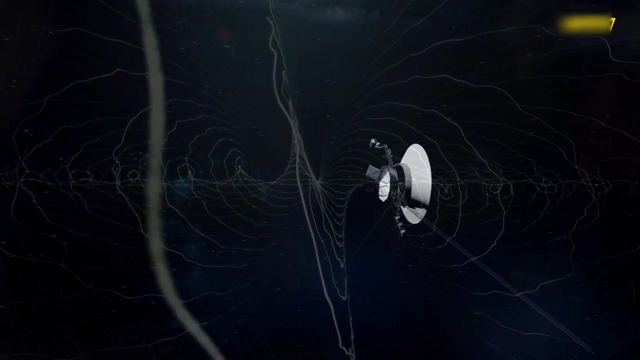 to sample the atmosphere directly. Cassini was touching the gas giant for the very first time. Over the next few seconds, Cassini increased the use of its altitude control thrusters to steady its rapid descent into the thin outer reaches of Saturn's atmosphere and keep the antennae pointing towards Earth. 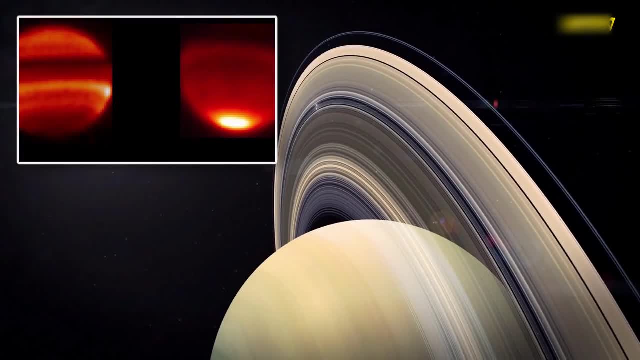 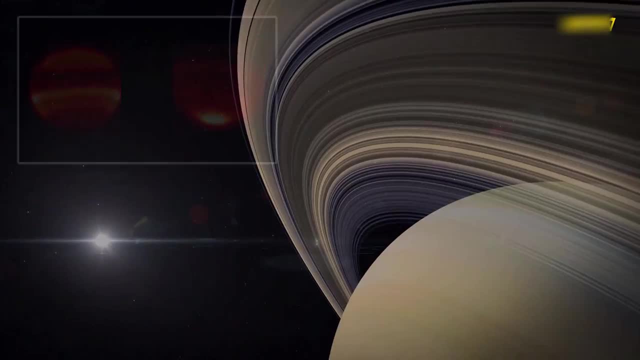 for a final few seconds of contact. But this was a losing battle. Over the next minute and a half, the growing density of the upper atmosphere rapidly began to increase the friction with the forward-facing surfaces of the spacecraft, raising the temperature at high speed. and creating an unfolding thermodynamic situation that Cassini had not been designed to withstand. At precisely 3,30 PDT, 1,500 kilometres above the cloud tops, Cassini finally lost its battle for control After 20 years in space. 13 of which were spent exploring Saturn, and having travelled a distance of 7.9 billion kilometres, this battered explorer was no longer able to maintain a stable flight path through the increasingly dense atmosphere, Beginning to tumble and roll. the last few bytes of data left its antennae. streaming the 90-minute journey back to Earth, and the mission was long over before that final contact reached our planet. Precisely what happened next to the little spacecraft as it fell into the grip of this giant planet remains no more than well-informed conjecture. Using computer models to predict its final seconds. the Cassini team were able to watch only in their mind's eye as the craft tumbled chaotically through the atmosphere, Travelling at 144,200 kilometres per hour, just 1,100 kilometres above the cloud tops. and with temperatures rapidly increasing, every component of this unprotected machine began to disintegrate, With all computer systems failing and the spacecraft, blind and deaf to its surroundings, it began to break up its gold insulation blanket, rupturing first, before the external carbon fibre structures. of the spacecraft itself began to fracture and fragment. Then, with the rings gleaming in the sky above it and the yellow cloud tops beckoning below what was left of Cassini, streaked across the Saturnian sky, blazing with temperatures higher than the surface of the Sun. The gas tanks of propellant that helped steer the spacecraft on its epic voyage blasted apart the remaining structures into a million different pieces which, in a final spectacular moment, lit up a little corner of the majestic planet with the burning debris of its greatest explorer. Cassini was dead. but its final journey was far from over. Over the following minutes, the debris scattered and fell through the cloud tops deep into the planet's interior, until, finally, the atoms of this beloved machine built by human hands, millions of kilometres away on a faraway world. came to rest in the heart of the planet: Cassini and Saturn, inseparable forevermore. Where the debris of Cassini finally ended up, we can only imagine But the data from this extraordinary mission that was collected right up to its very end. has helped us to dive deeper into the detail of Saturn's interior than ever before. As the wreckage scattered and fell from the upper atmosphere, it would have fallen through the very first cloud tops of the planet here, with temperatures ranging from minus 170 to minus 110 degrees Celsius. 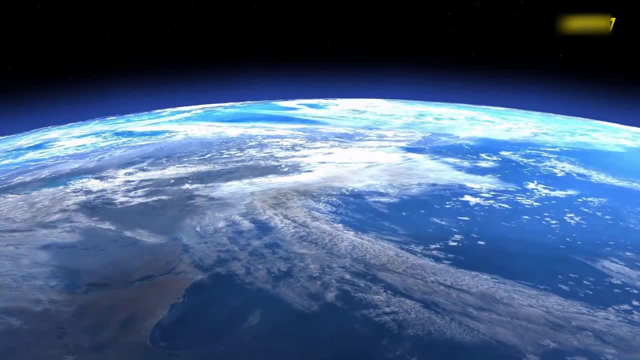 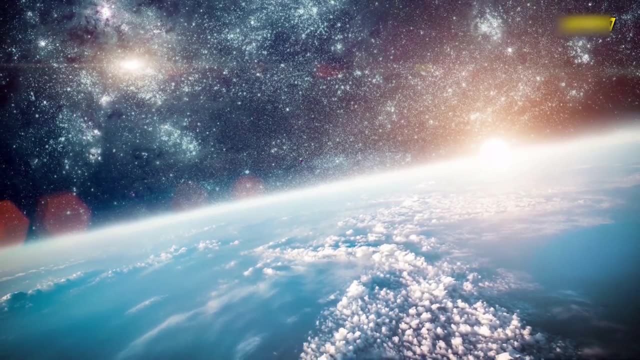 The clouds are made not of water ice, but frozen ammonia. It's these ammonia ice crystals that give Saturn its characteristic pale yellow colour, a colour that we can see shining back at us with even the most modest of Earth-bound telescopes Beyond this upper layer of cloud. as the pressures begin to increase and the temperature rises, huge clouds of water ice form a thick layer, the water molecules, perhaps long-lost remnants of the building blocks of the icy world that Saturn once was. It's here amongst the vast cloud systems. 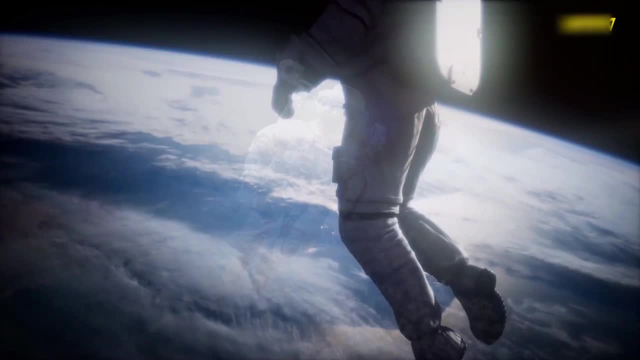 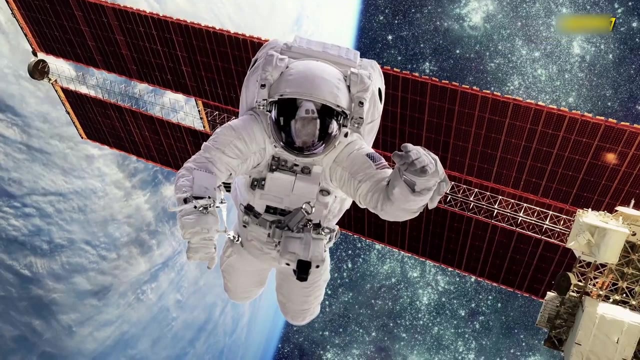 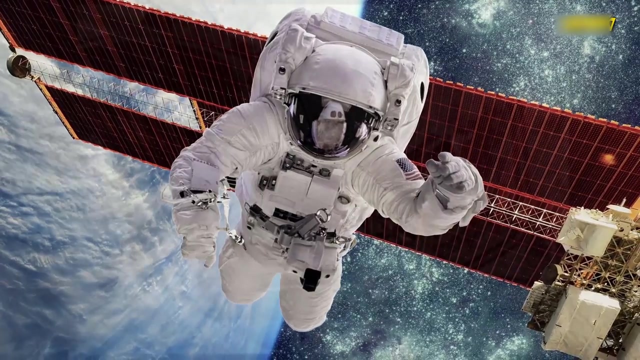 that lightning, more powerful than anything we see on Earth, illuminates the sky within storm systems that rage for months on end. Cassini gave us the first still and moving images of these lightning storms And enabled us to predict the next great transformation that will happen within the planet's interior. 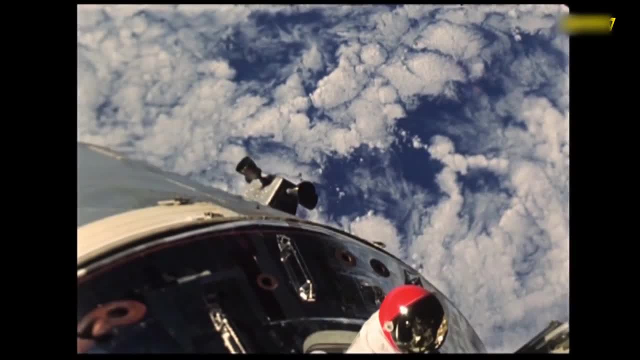 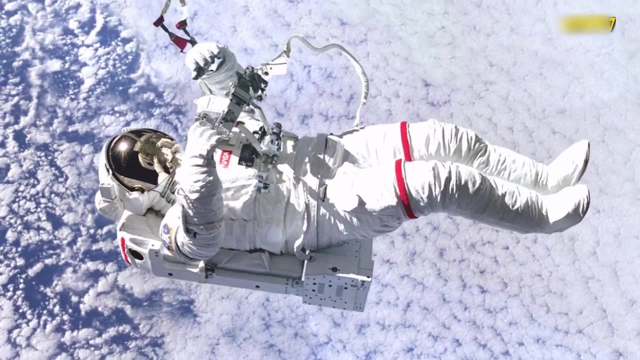 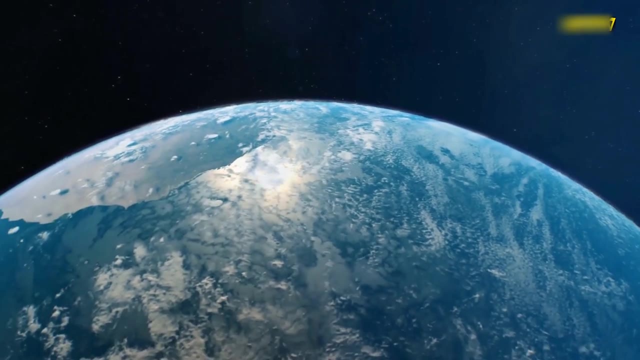 Every couple of decades, Saturn surprises us and breaks into a fit and actually erupts with really major storms. These are global storms and they last for about six months to a year. The one that we saw with Cassini in 2010 was so powerful that our calculations show. 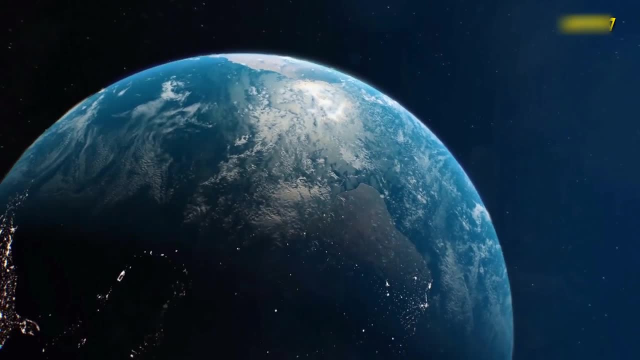 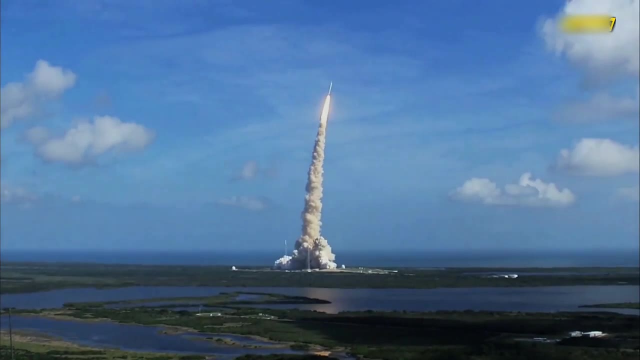 it was the most powerful storm we've ever seen anywhere in the solar system, Even Jupiter, in terms of its central conductive storm system. We had an amazing chance to see that during the Cassini mission And then when we looked at those clouds that it was forming. 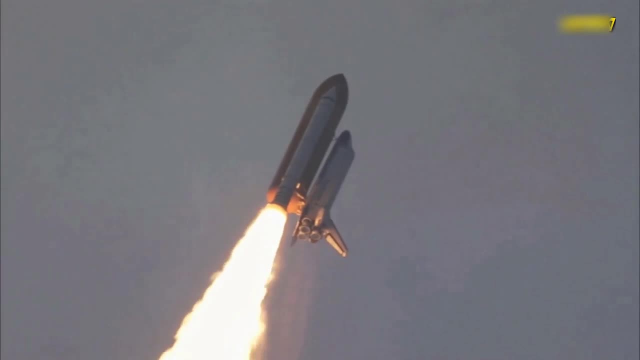 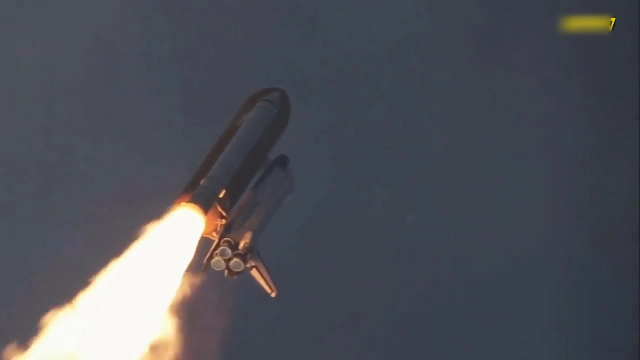 we found amazing things in the cloud, in the storm clouds of Saturn. We found that it had water ice, And this really blew our minds, because water should be sequestered deep down in the atmosphere. You should not find it at the top of the atmosphere. 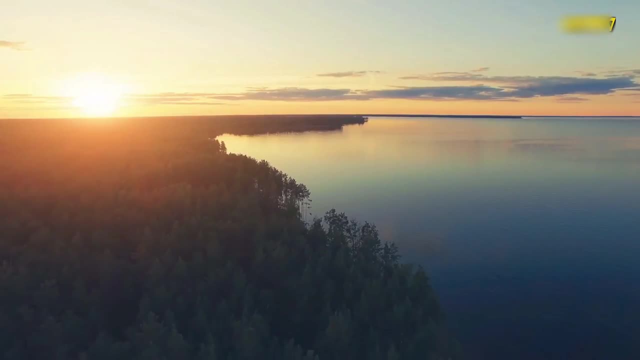 It only gets there when you have huge convective updrafts, And we're talking updrafts that bring gas up from 100 miles down, And on the Earth we only see gas going up and convection going up only about 10 miles. 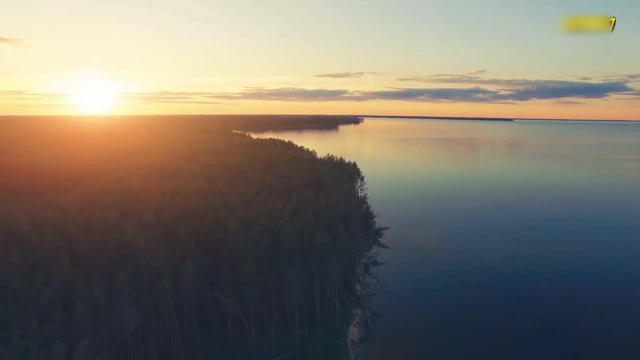 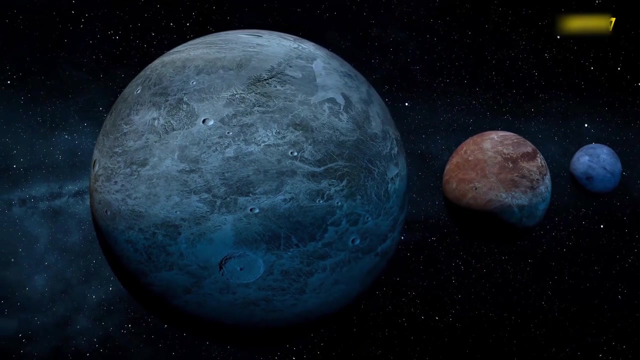 Here you have storms 10 times bigger, Very powerful storms, lifting things up from 100 miles down and bringing up the water from below, which was probably actually a mixture of gas and water, But then it brought it up and it turned into ice. 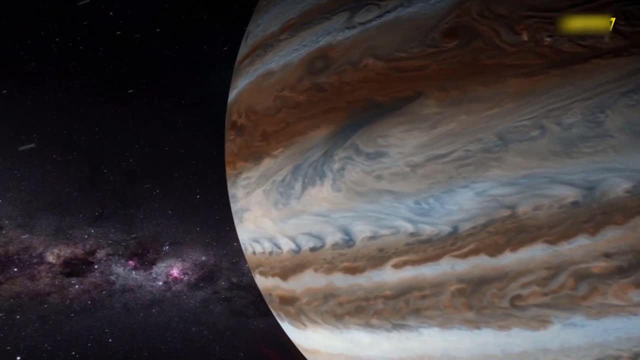 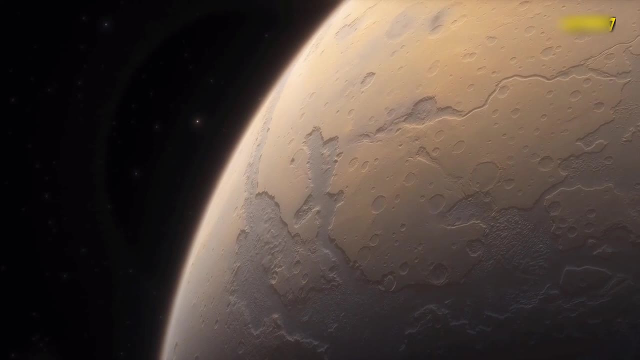 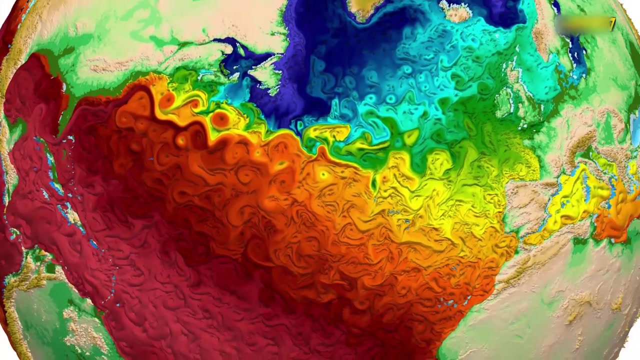 and the component of water ice in it really shocked us. Kevin Bain's Cassini Mission. We now think that around 100 kilometres below the visible atmosphere, the same distance from the surface of Earth to space, with temperatures inside Saturn's lightning reaching almost 30,000 degrees Celsius, 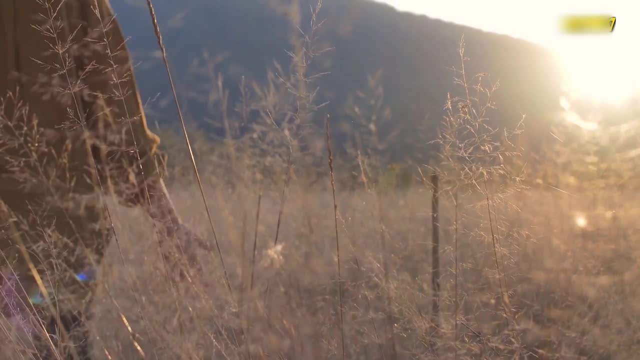 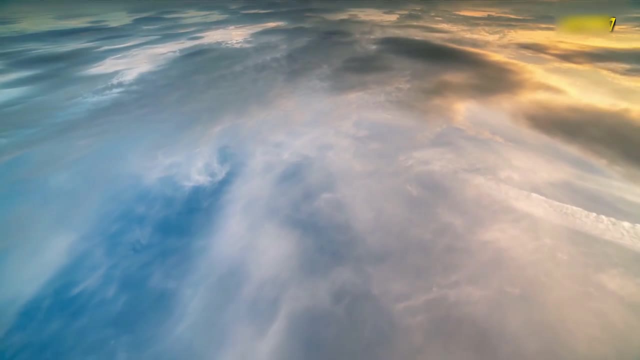 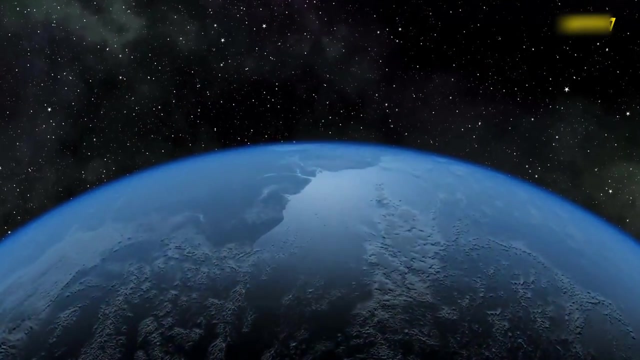 this lightning transforms methane gas in the atmosphere into huge clouds of carbon soot carried higher into the atmosphere on great convection currents. We think that it's these specks of carbon-producing lightning that can explain the mysterious dark clouds that Cassini was able to observe and image over many years. 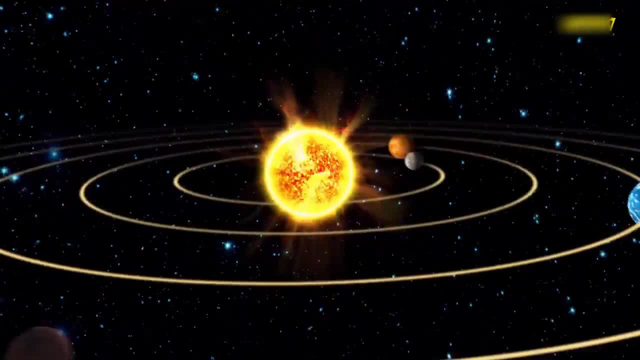 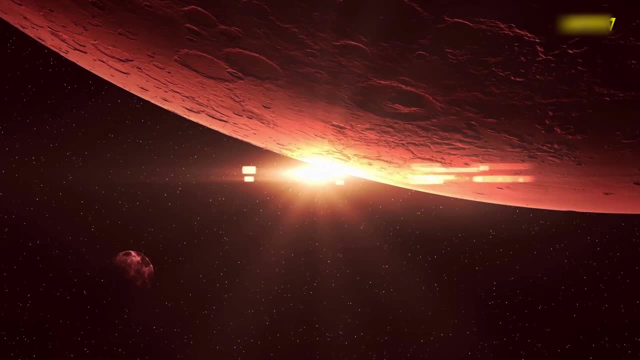 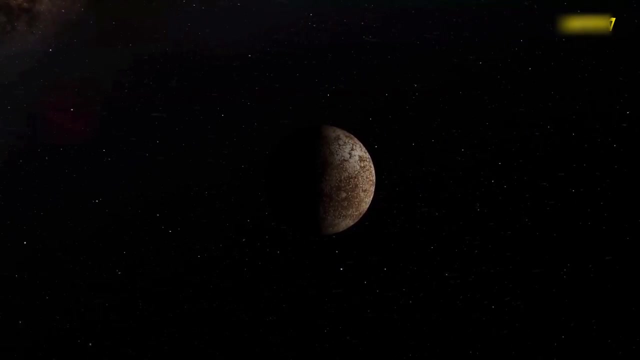 This particulate matter rains down from the upper cloud layers until at a depth of 1,500 kilometres, We think the enormous pressures begin compressing this soot into graphite, which then falls further into the depths of the planet. We then think that at around 6,000 kilometres down, 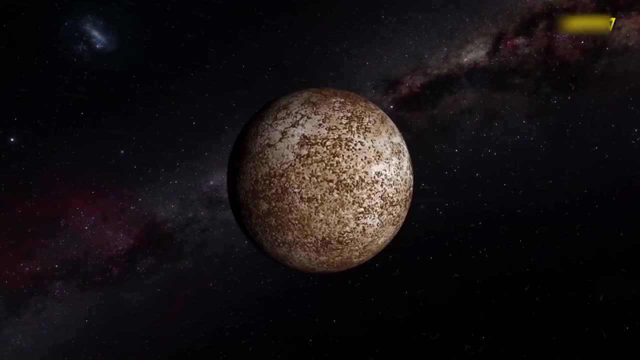 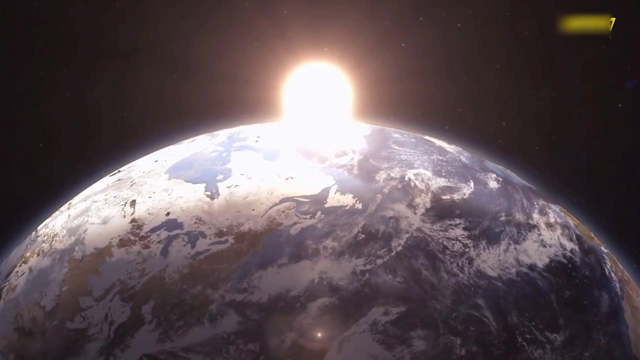 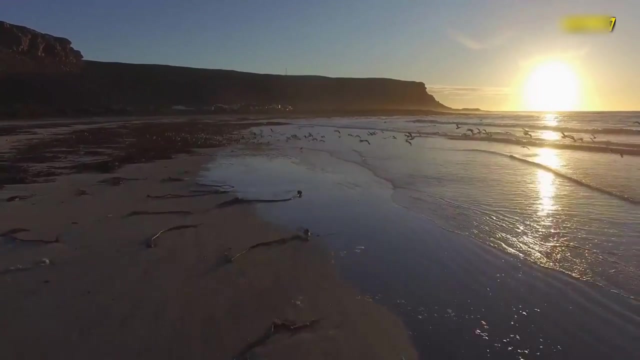 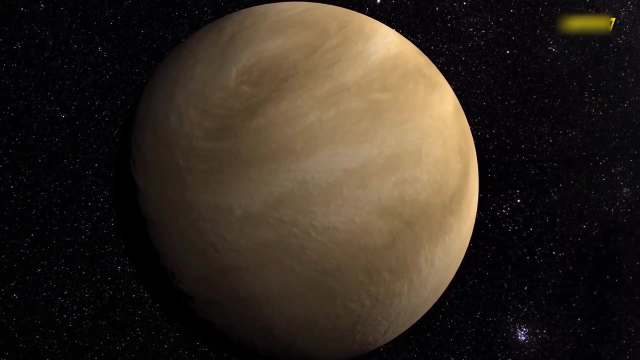 this graphite undergoes a truly extraordinary transformation, With pressure and temperatures rapidly increasing. the graphite is compressed into solid diamond that rains down for at least 250,000 kilometres. Estimates suggest at any one time 10 million tonnes of diamond hail is raining down within the planet. 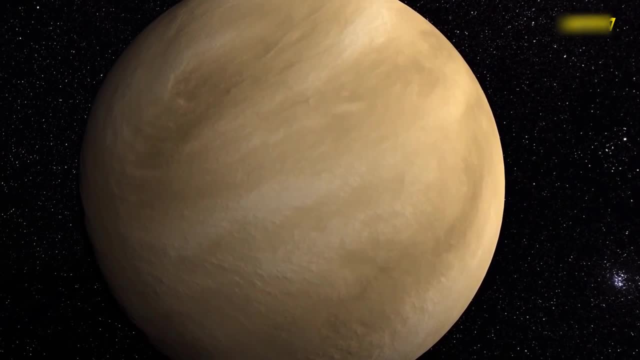 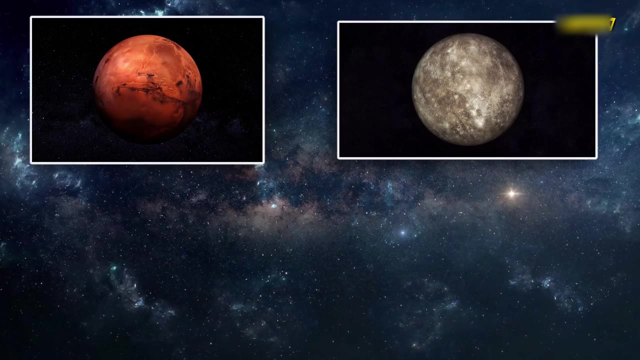 from specks of diamond dust just a millimetre across to chunks as big as 10 centimetres. Perhaps even for a brief moment in time. some of the charred, carbonised remains of the Cassini probe made it down into these depths. 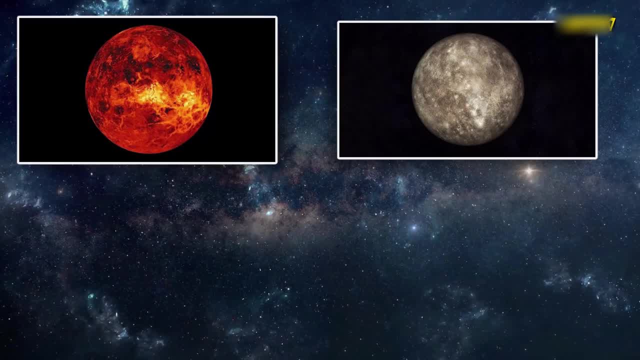 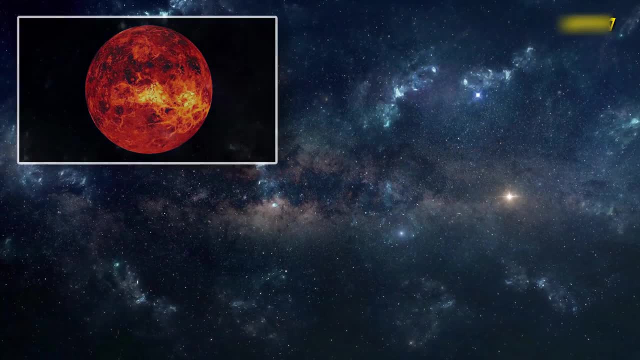 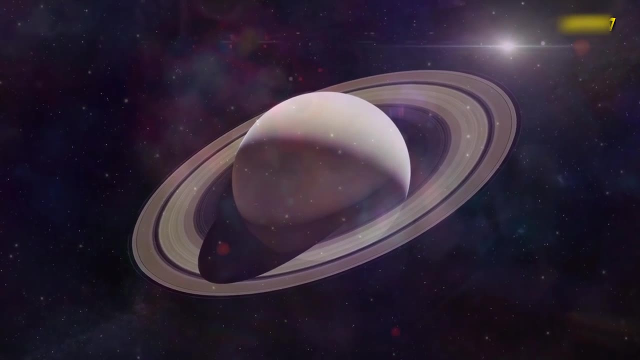 and transformed into diamonds as well, falling further into the planet. it had helped us understand, But eventually, even these diamonds will ultimately succumb to the enormous pressures of Saturn's interior, Around 30,000 kilometres into the atmosphere, where temperatures reach 8,000 degrees. 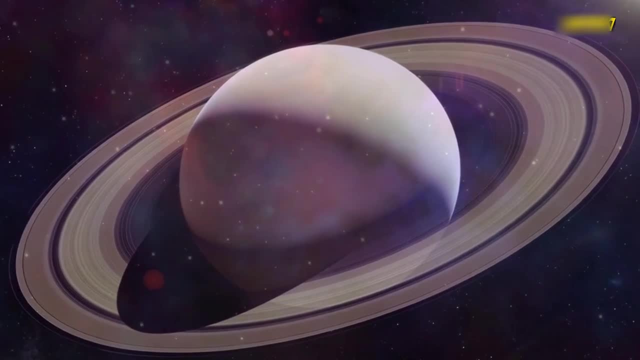 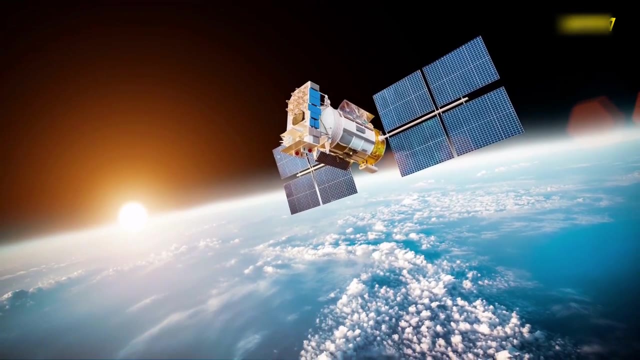 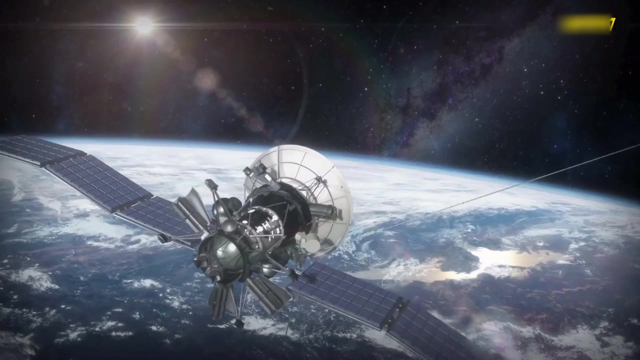 Celsius, the diamond melts and forms liquid diamond raindrops that continue to descend into the abyss. It's here, around 40,000 kilometres down into Saturn's interior, that we believe the source of Saturn's energy, the energy that drives all the storms and weather. 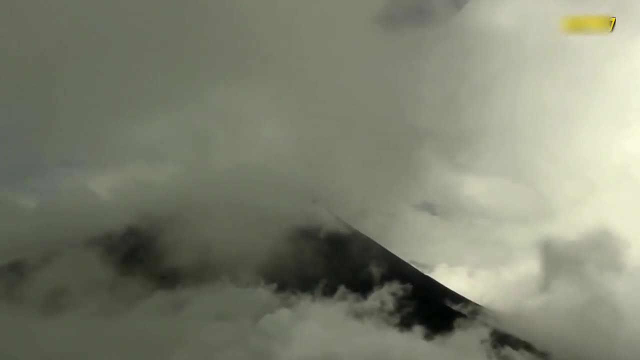 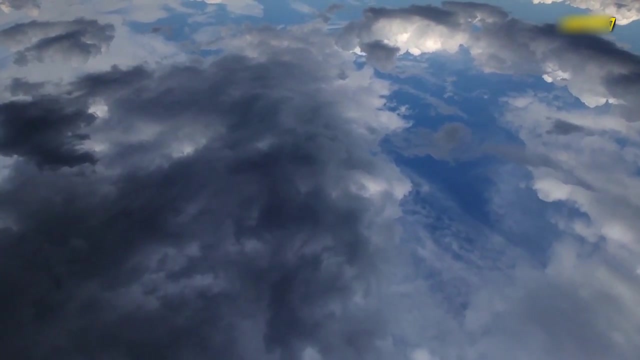 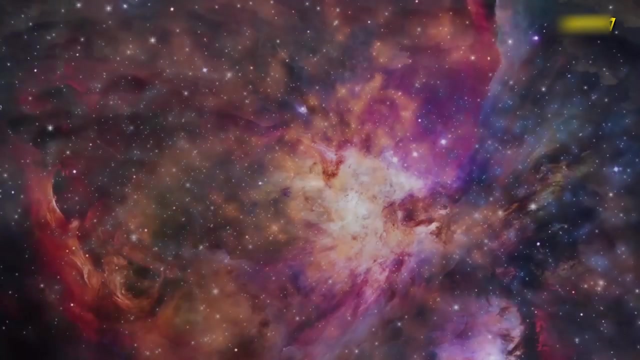 we see playing out on its surface is finally revealed Here. the pressures are so intense that the hydrogen that makes up over 96% of Saturn's mass is compressed into a vast ocean of liquid hydrogen that is saturated with helium gas. Under these enormous temperatures and pressures, 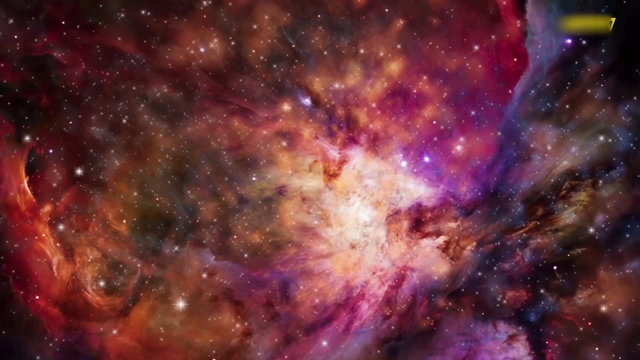 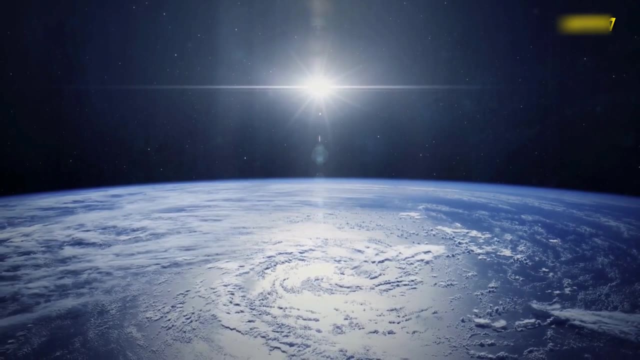 the helium precipitates out and falls like rain through the ocean, depleting the levels of helium in Saturn's outer layers, which explains the lower-than-expected amount of helium first measured by Voyager 1 in 1980.. It's a process that, through the simple action of friction, 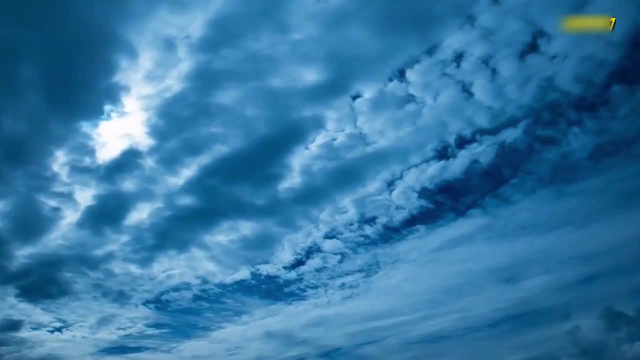 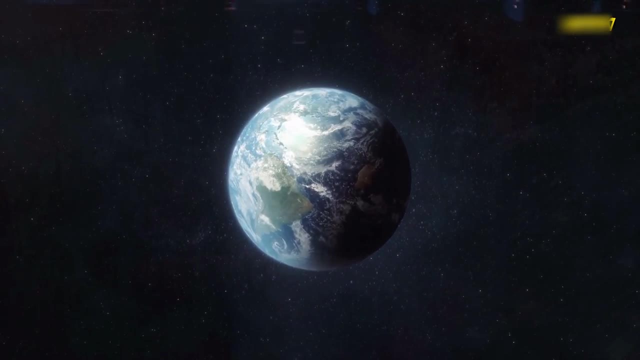 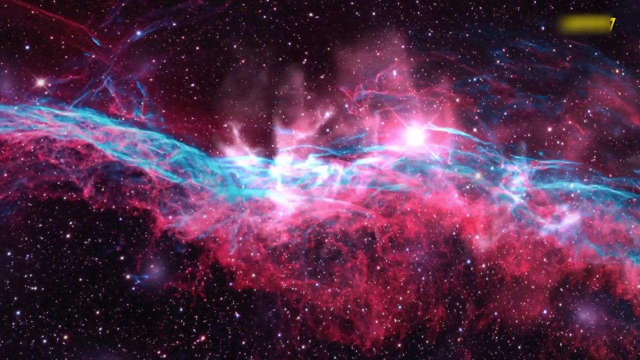 as the molten helium rain falls, creates an incredible amount of heat, and we think this is the engine, the energy source that helps power Saturn's ferocious weather and drives its entire atmosphere for tens of thousands of miles in every direction. Finally, we reach the interior of Saturn. 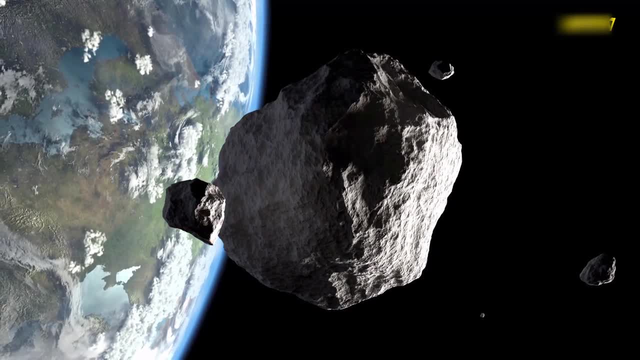 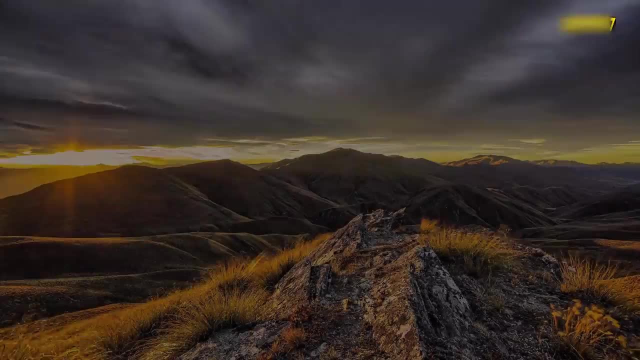 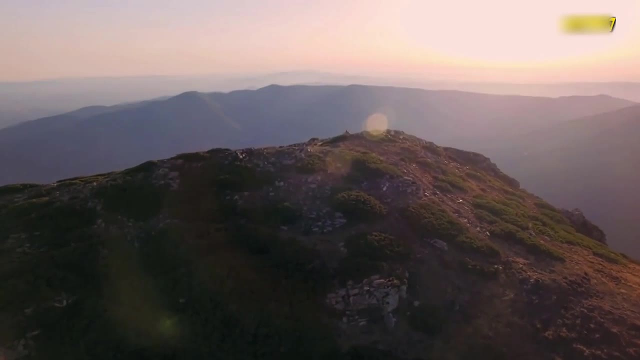 a layer where the liquid hydrogen is so compressed it starts to behave like a liquid metal and the helium itself may accumulate into a metallic shell surrounding the core. Beyond here, we do not know if a rocky core remains as a remnant of Saturn's long-lost past. or whether, under these enormous pressures, the possibility of solid rock is no longer viable. Whatever lies at the centre of Saturn, we estimate that this core region has a mass of around 20 times that of the Earth and a diameter of around 25,000 kilometres. 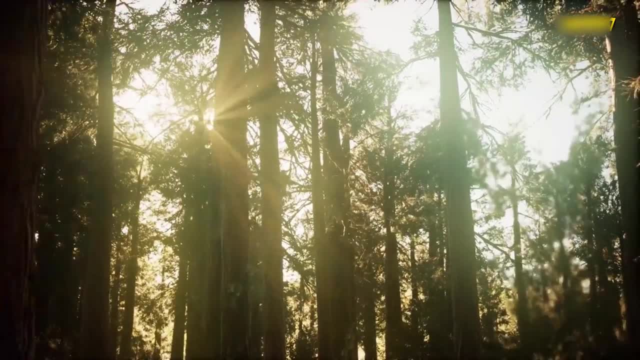 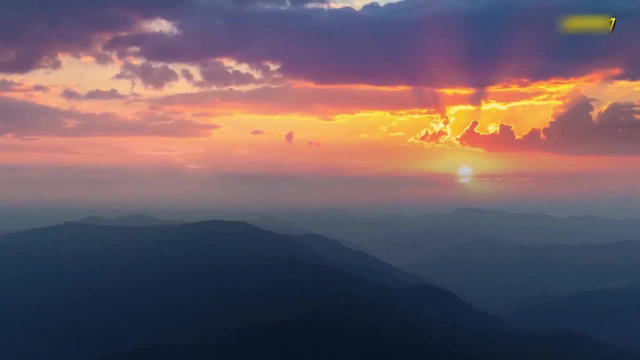 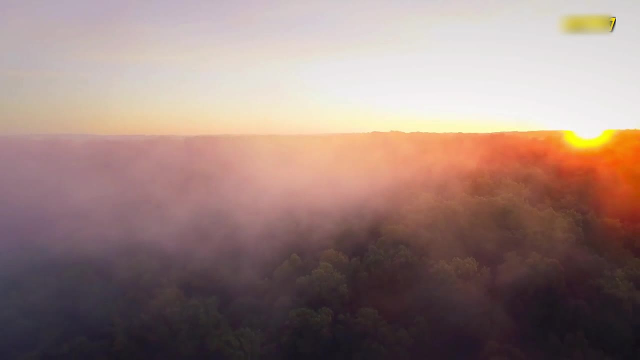 And here perhaps a few tiny fragments of Cassini might have come to rest in the ancient heart of the planet. Saturn has lived a life of incredible drama. The evolution from rocky beginning to the extraordinary gas giant we see today took just a few hundred million years of rapid transformation. 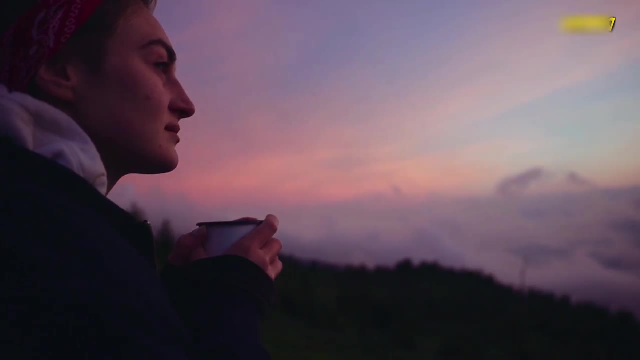 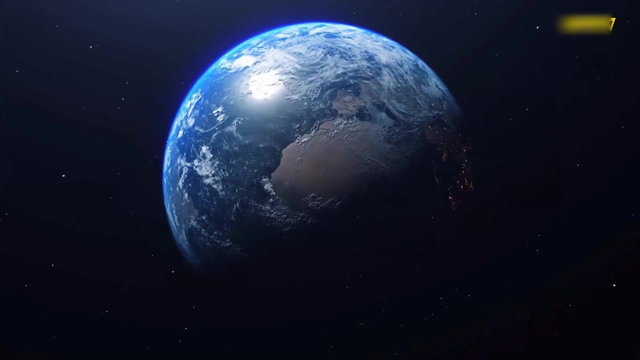 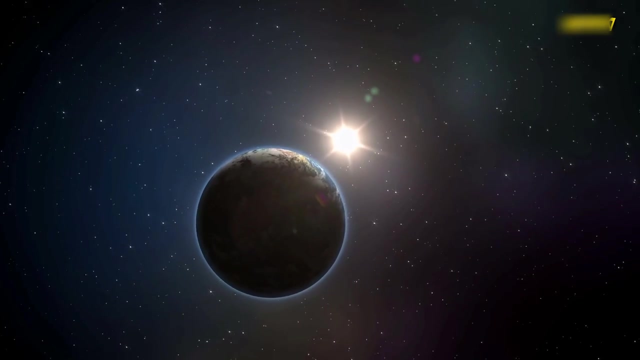 And yet, throughout almost all of this time, one thing has been missing. We now think Saturn was born naked and has lived out the vast majority of its existence without the structure that makes it more iconic than anything else. Saturn is a world defined by its rings. 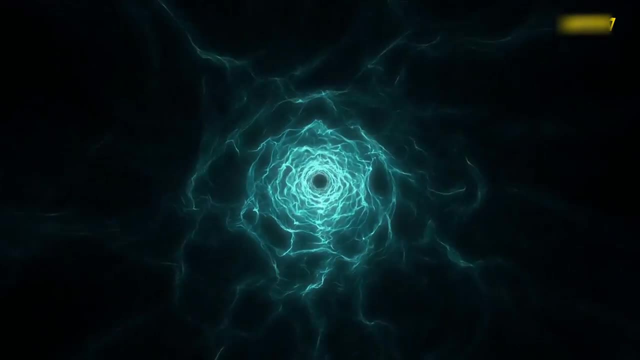 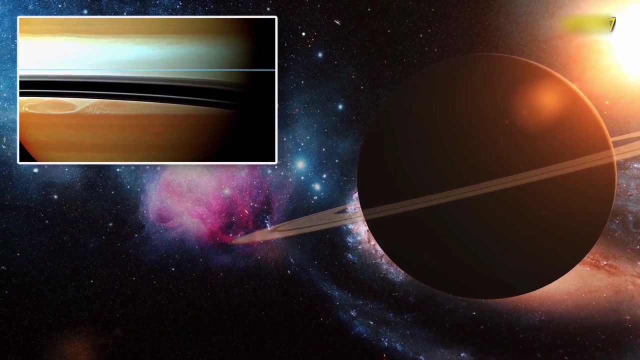 Ask a child to draw a planet, and more often than not they'll draw something that looks remarkably like Saturn. The particles in the rings of Saturn are almost impossibly delicate and intricate. Most of them are no bigger than snowflakes, but some are as large as houses. 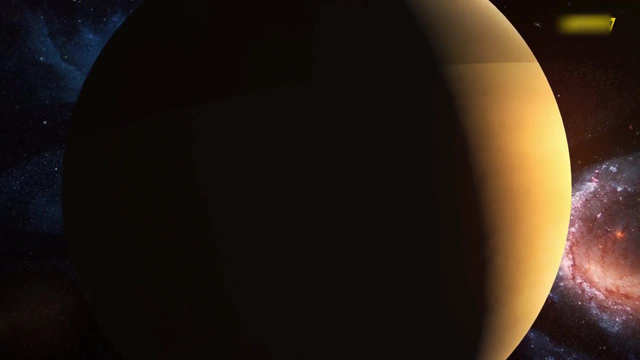 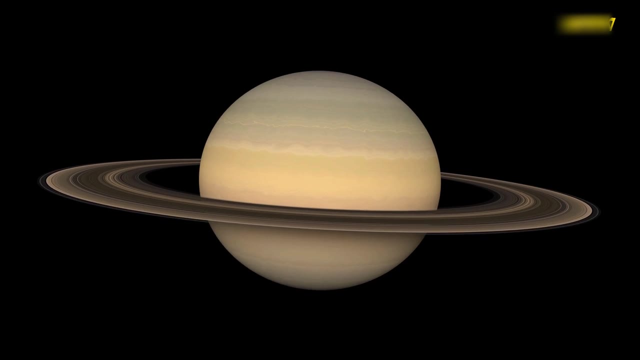 orbiting the planet at 1,800 kilometres per hour in one of the most beautiful structures we have ever laid eyes on. One of the reasons why the rings have captivated us for so long is that, despite their vast distance from the Earth, 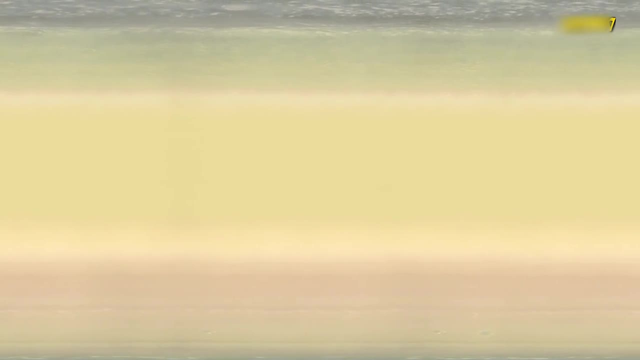 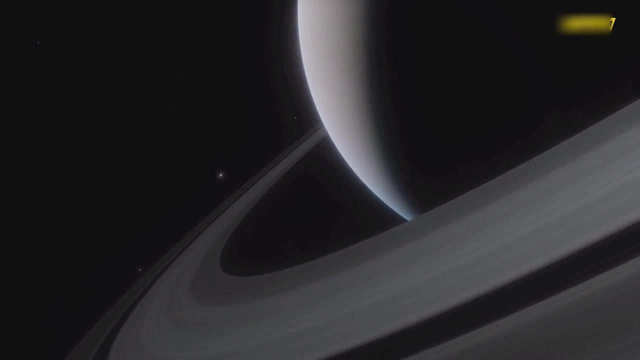 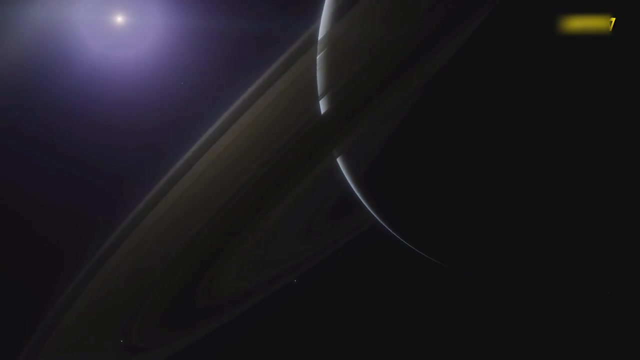 if you look through a simple telescope, they shine back at us bright against the night sky, reflecting the sun's light as powerfully as the planet itself. For years, the age and origin of the rings has been argued over, with conflicting evidence supporting two very different hypotheses. 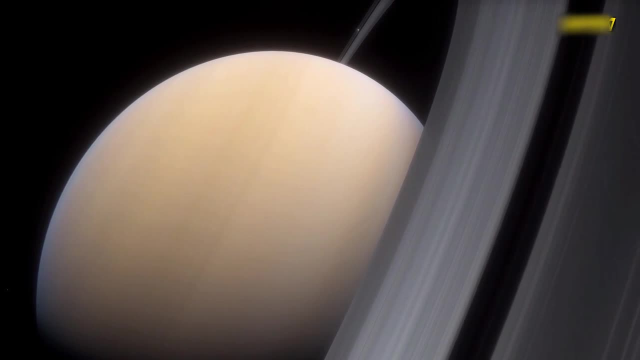 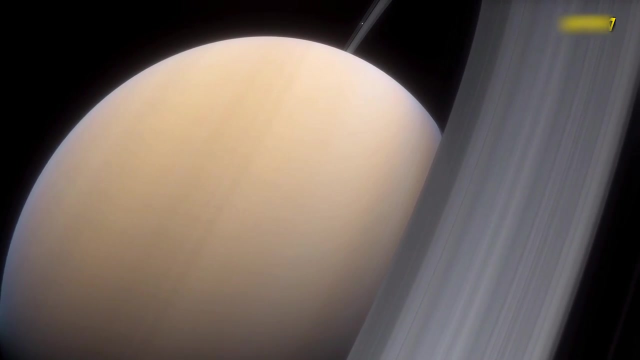 On one side, the argument has been made that a ring system as dense as Saturn's must be an ancient structure shaped from the remnants of the planet's formation. On the other side of the fence, the evidence has been used to suggest that the rings must be youthful. 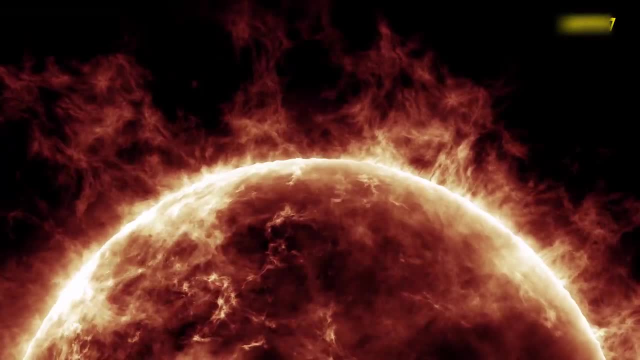 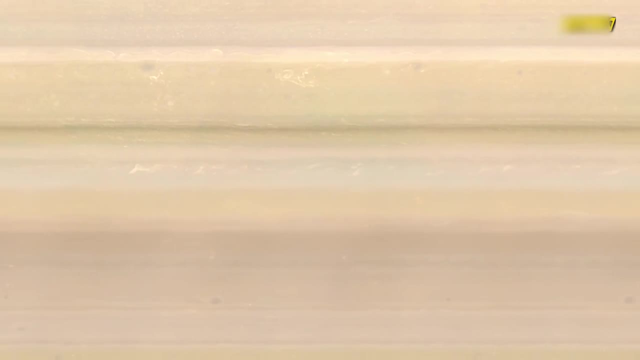 a relatively recent addition to the ancient planet. The brightness of the rings is not only beautiful, but also rather surprising. The solar system is not a very clean place. In fact, it's full of dust and dirt, and so we would expect any ice crystals. 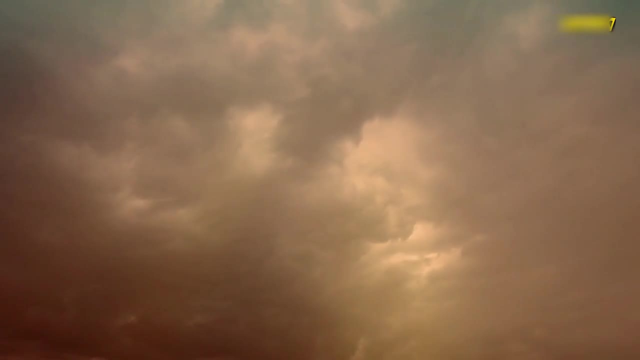 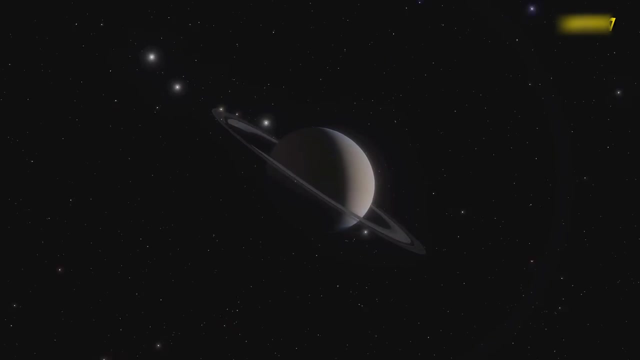 that hang around for any length of time to inevitably get dirty. We also know that if ice gets dirty, it doesn't reflect sunlight anywhere near as brightly. So in the case of the rings, we would have expected if they had been present. 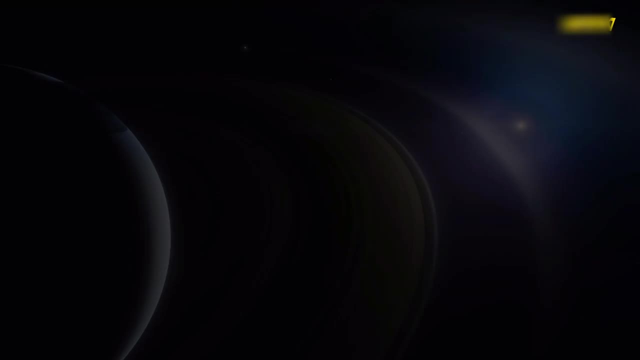 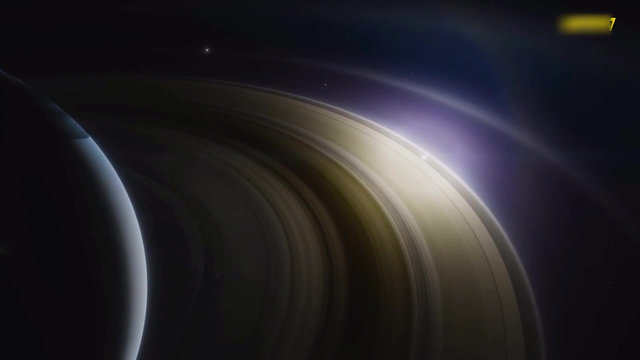 over the lifetime of the planet, all of those particles and blocks of ice would have become increasingly beautiful, But they are increasingly less reflective. If they had formed anywhere near the birth of Saturn, they would almost certainly be invisible to us now, or at least incredibly faint. 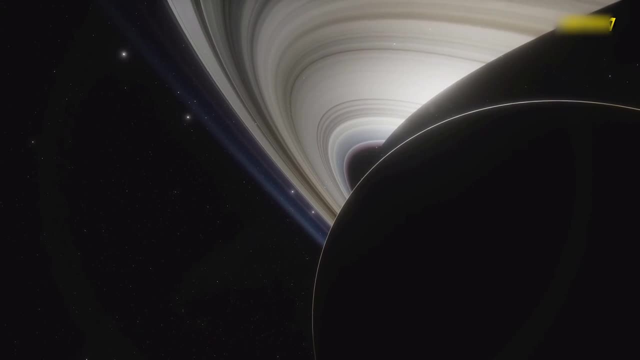 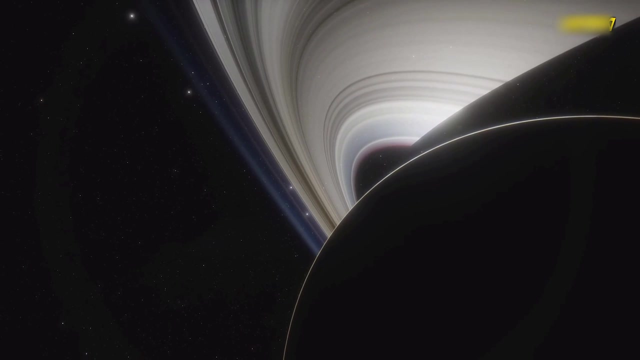 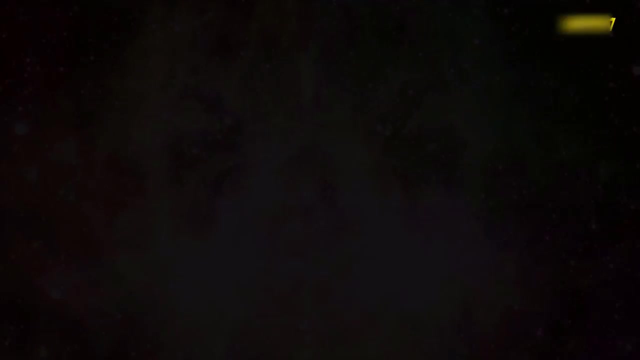 And yet they shine brightly as if they were made just days ago. Variations of this debate have been rumbling since the 18th century, But that all changed with Cassini. During its 13-year tenure around the planet, Cassini was able not only to see Saturn's rings like never before. 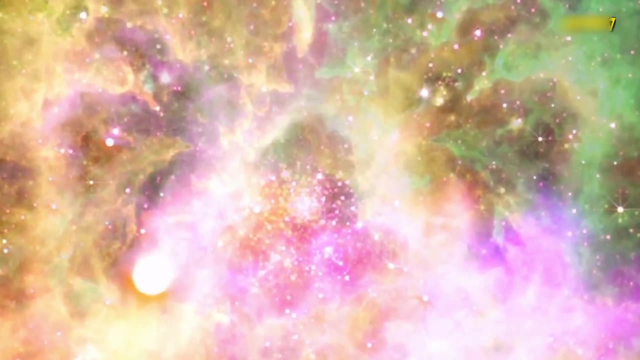 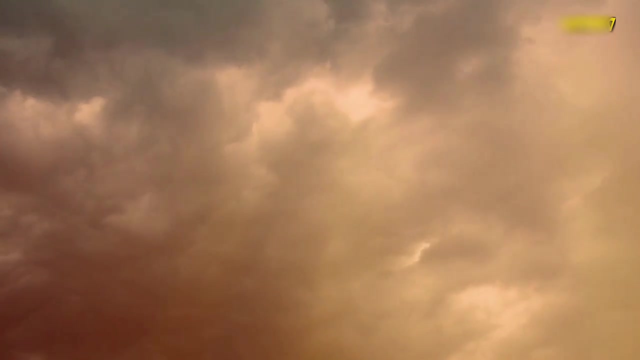 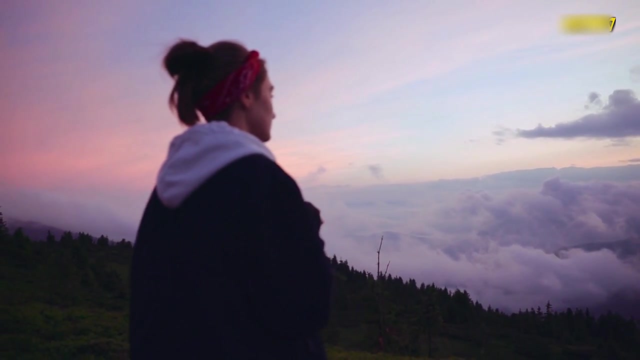 but also provide us with direct evidence about their density and composition, And this information is helping scientists to solve the puzzle of the rings once and for all. For the very first time, Cassini was able to take physical samples directly from the rings and surrounding dust. 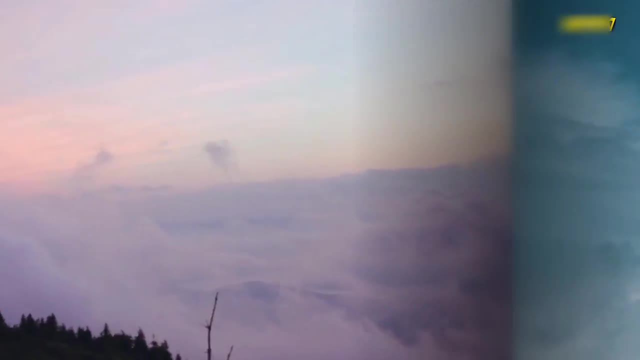 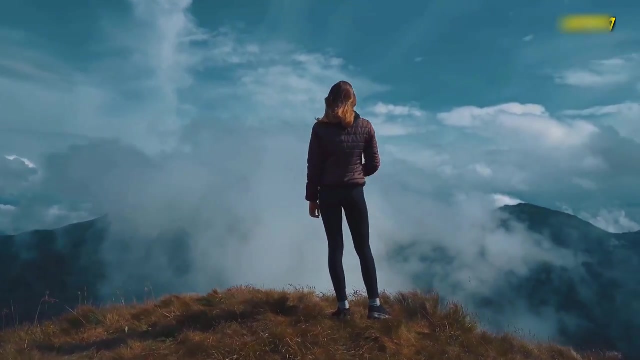 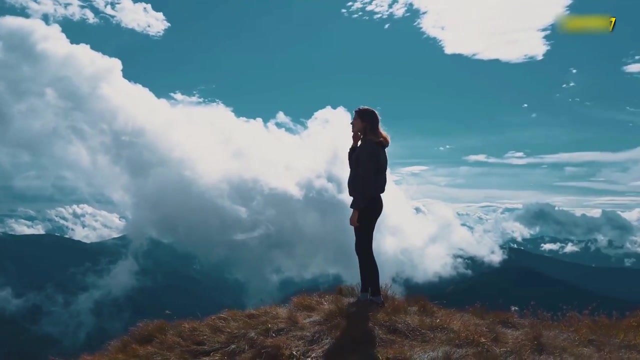 using the Cosmic Dust Analyser CDA mounted on its exterior. This highly sophisticated piece of technology is basically a multimillion-dollar bucket, but a bucket that can detect particles one millionth of a millimetre wide. That's smaller than a virus. 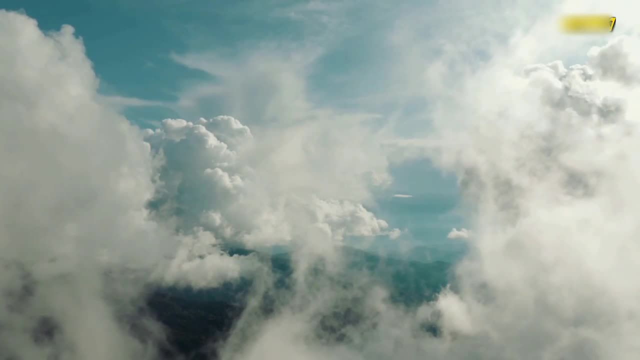 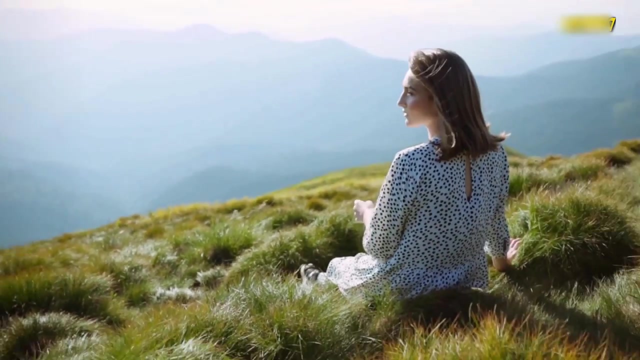 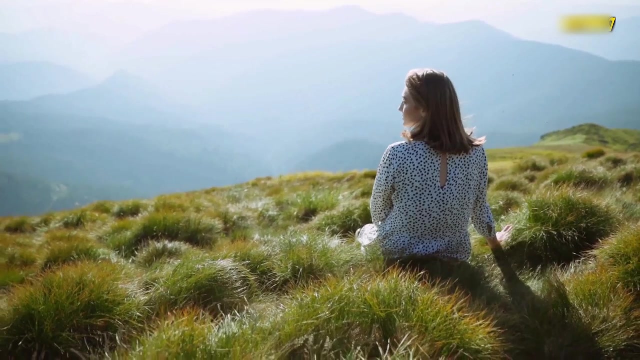 And determine the particles' size, speed and direction of travel, as well as their chemical composition. By measuring the dirt and dust from the Saturnian system falling onto the rings, Cassini has allowed scientists to rewind the clock on the rings and provide direct and compelling evidence. 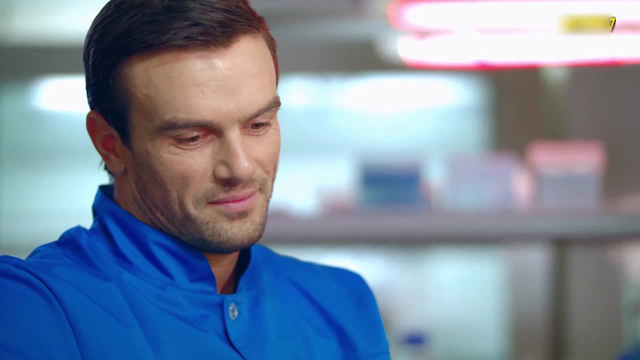 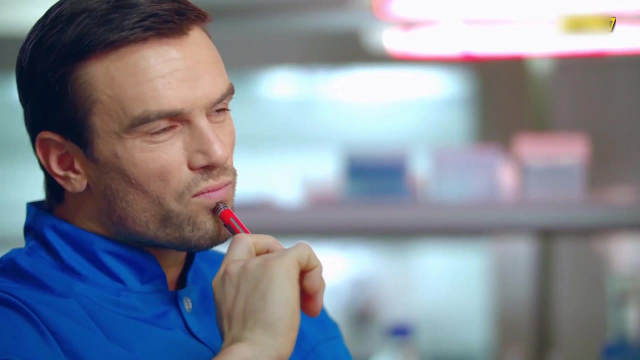 that the ice particles are nowhere near as dusty as they would be if they were an ancient part of the planetary system. This confirms the long-held belief that the rings are so bright because they are young And, in fact, the evidence gained from Cassini's CDA. 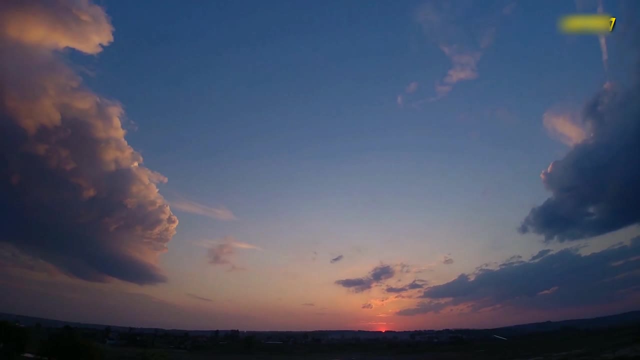 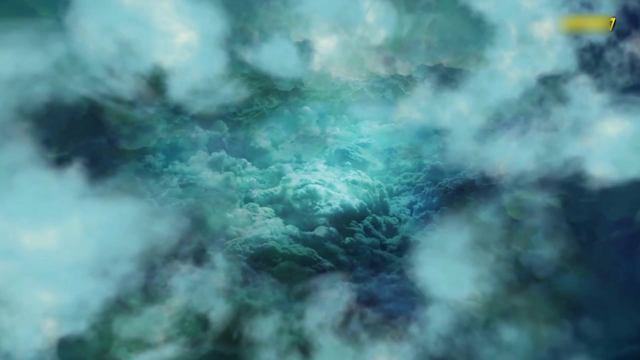 suggests they are far younger than we ever imagined. Latest estimates suggest they're somewhere between 10 to 100 million years old. That's nearly 4.5 billion years old, 15 years younger than Saturn itself. So where did they come from? 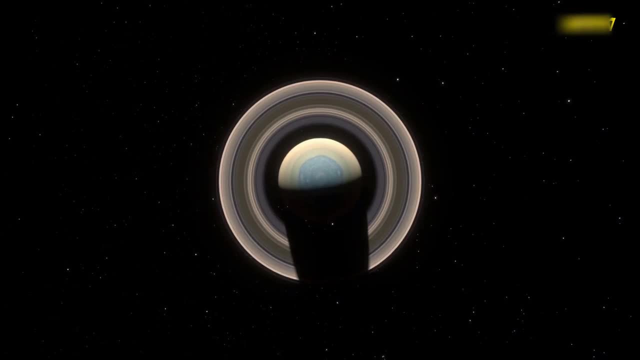 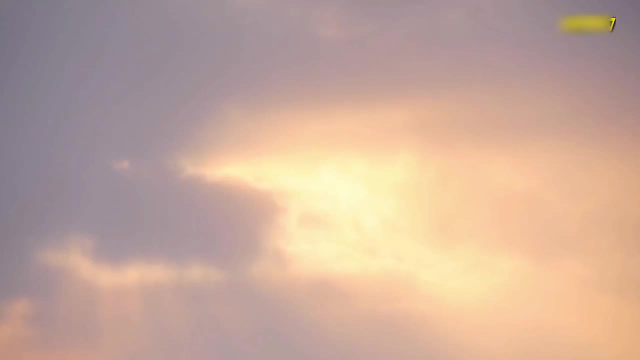 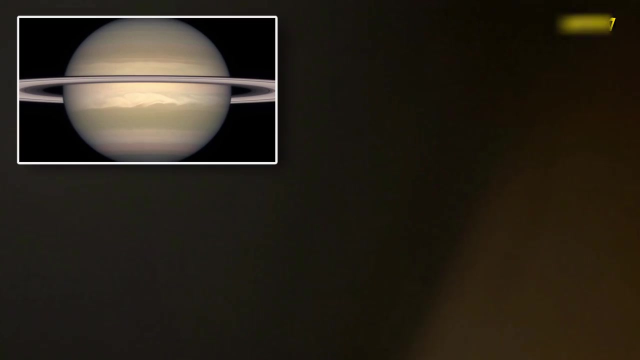 Once again, Cassini provided a tantalising clue. In its final few days, Cassini embarked on a series of almost reckless orbital trajectories that were so risky to the spacecraft's safety they would never have dared to be attempted earlier in its mission, Taking the probe closer to the planet than ever before. 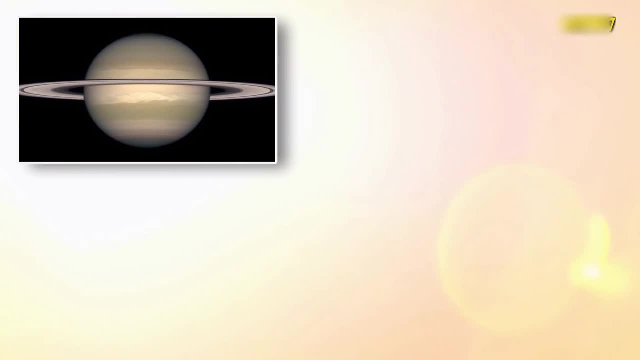 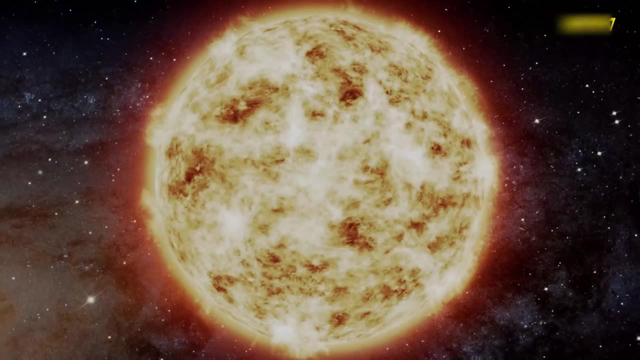 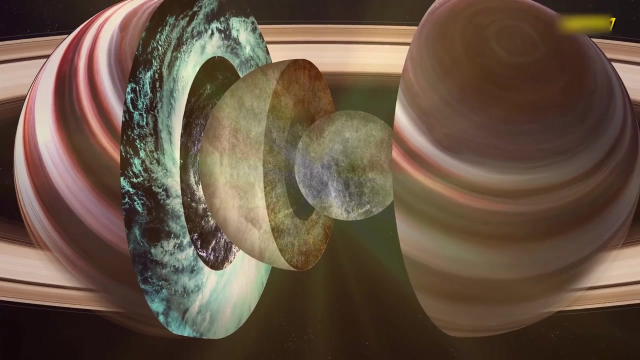 the team flew Cassini repeatedly through the gaps between the upper atmosphere of the planet and the inner rings Throughout September 2017, as it performed 22 of these perilous dives, Cassini was able to take measurements of the gravitational tug of both the planet and the rings. 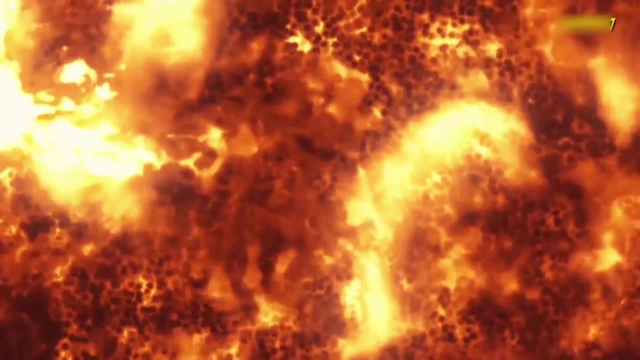 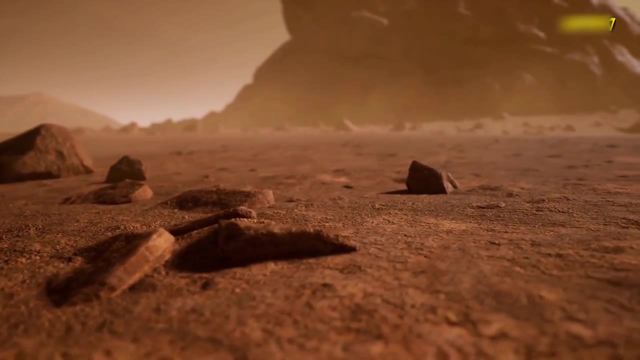 This data was then used to calculate the mass and density of the most substantial ring in the Saturnian system. The B ring makes up 80% of the mass of all the rings, and yet Cassini's measurements suggested that the total mass of the ring was surprisingly low. 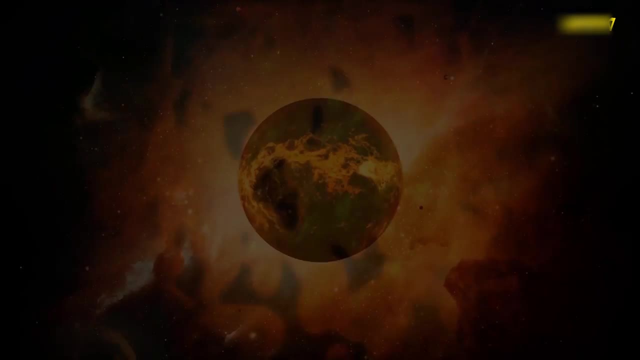 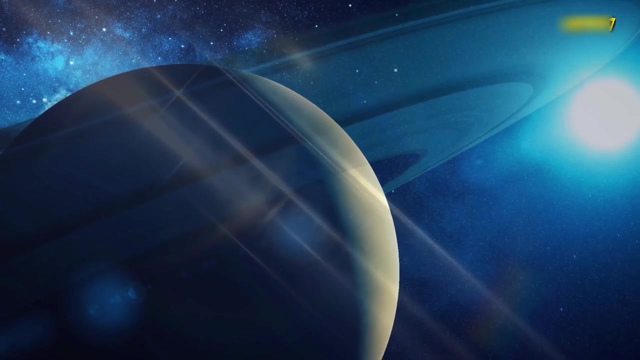 This result, although not conclusive, strongly points to the fact that the rings' origins lie not in the ancient past, during the formation of the planet itself, but to a far more recent and dramatic event involving one of the worlds trapped in orbit around it. 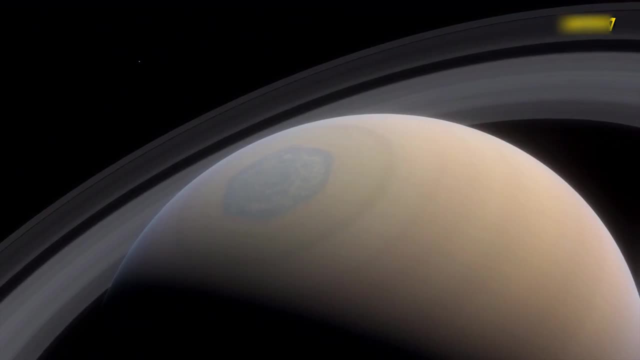 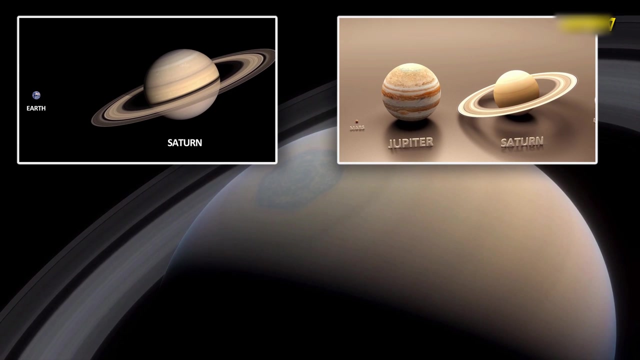 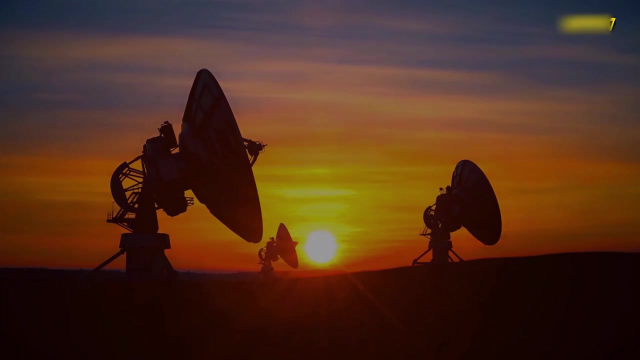 The rings, it seems, were born of a moon. Saturn has 62 large moons and countless smaller ones that range in size from planetary-scale objects like Titan to smaller irregular lumps of rock like Aegeon, And we're still hunting for new moons to add to the list. 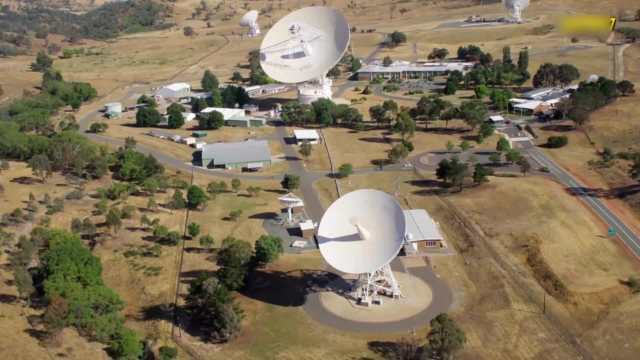 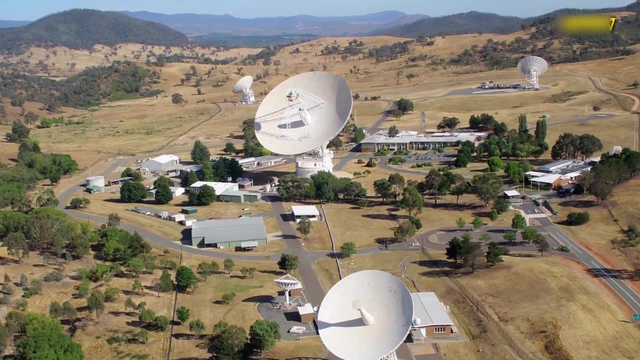 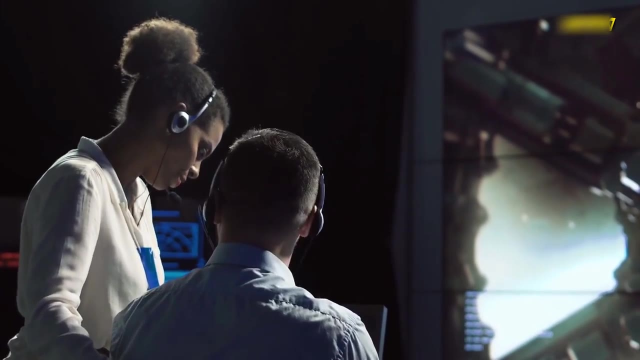 On its travels, Cassini spotted two objects within the F ring that are potential candidates for moonhood, but as yet, S-stroke-2004-S6 and S-stroke-2004-S3 remain unverified and unconfirmed. Within this menagerie of worlds, 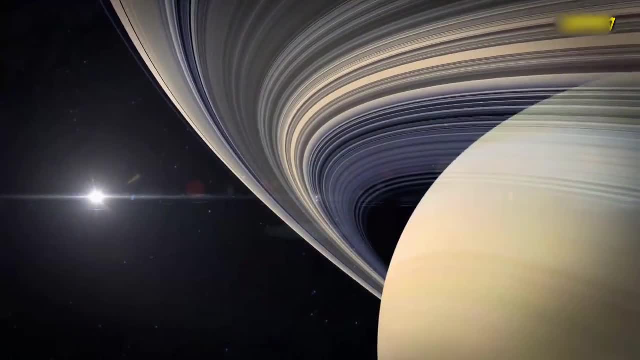 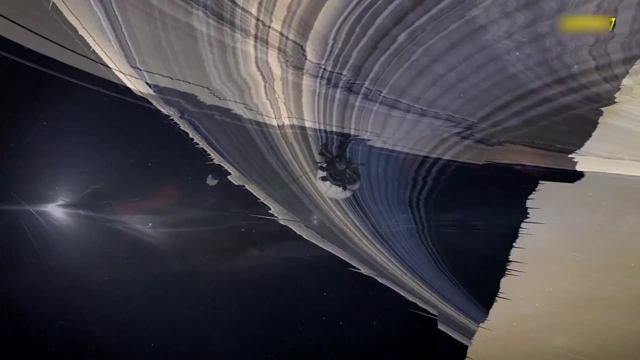 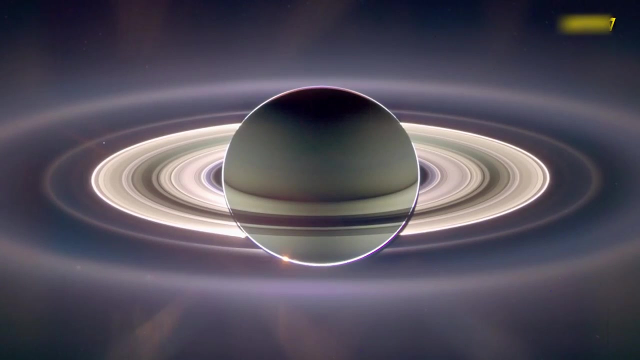 are an endless variety of clues written into the size, form and surface features of the moons that allow us to read the history of the Saturnian system, revealing the often violent and volatile events in its past. Mimas is otherwise known as the Death Star Moon. 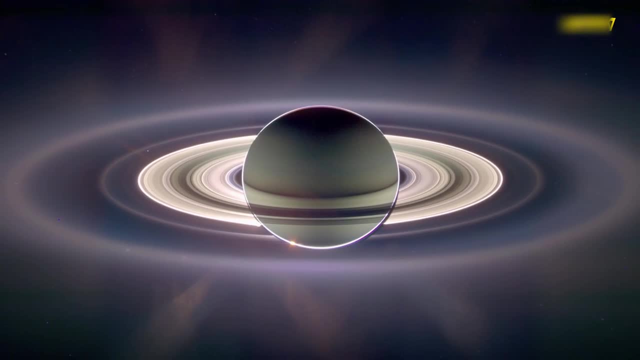 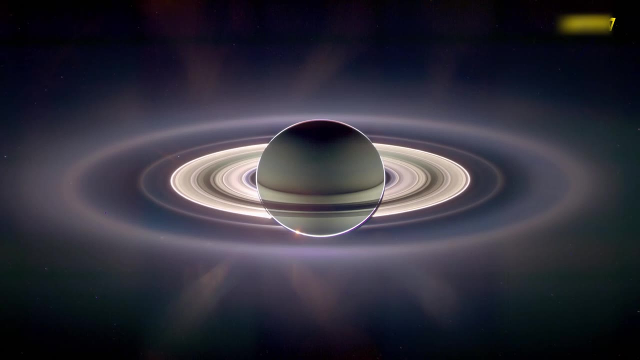 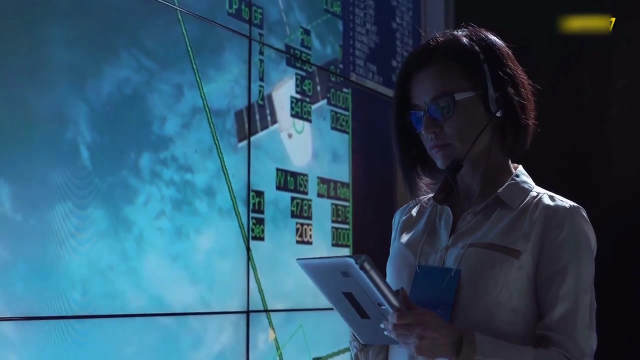 and was first spotted in 1789 by William Herschel, who is immortalised in Mimas's eponymous book. the enormous, huge impact crater Mimas is just 396 kilometres across and the Herschel crater covers 130 kilometres of that surface. 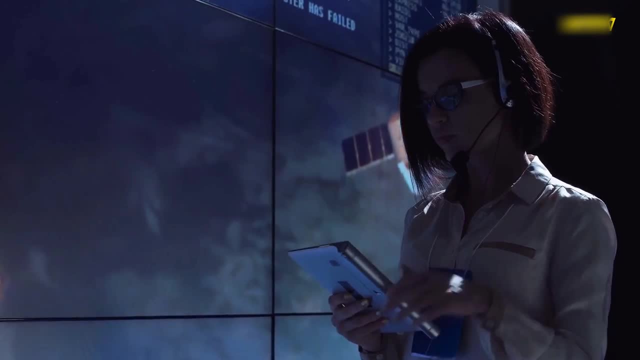 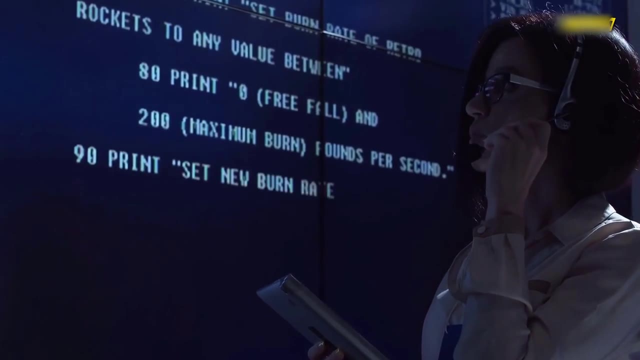 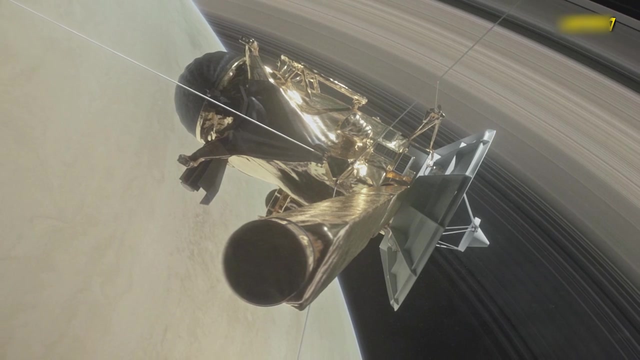 a deep scar that tells us that once, long ago, there was a giant impact that almost destroyed the Moon. Iapetus, the third largest of Saturn's moons, at 1,500 kilometres across, is almost planetary-sized and has a distinctive two-tone colouration. 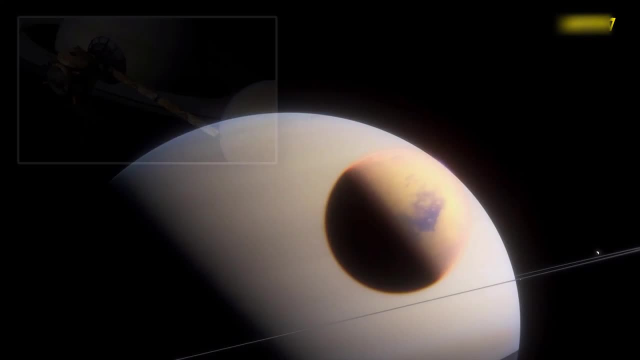 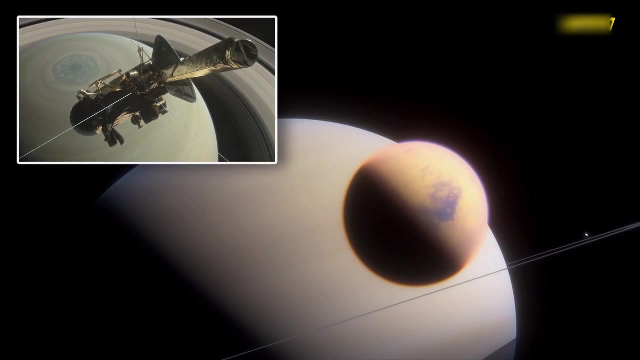 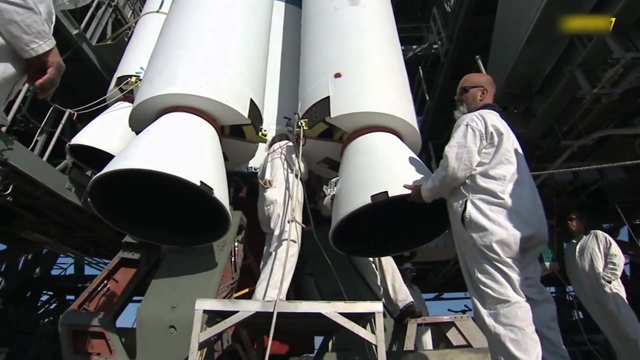 half light and half dark. Iapetus was discovered by Giovanni Cassini himself in 1671 and has another distinctive feature that we have long puzzled over: Running around three-quarters of the Moon's diameter is a massive equatorial ridge. It's one of the highest mountain ranges in the solar system. 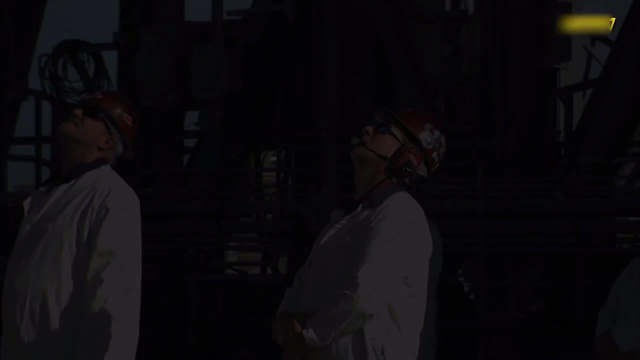 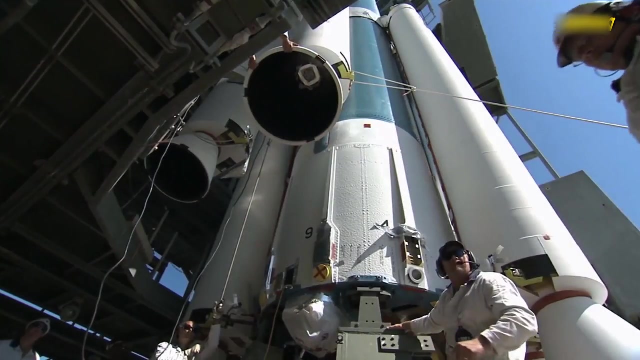 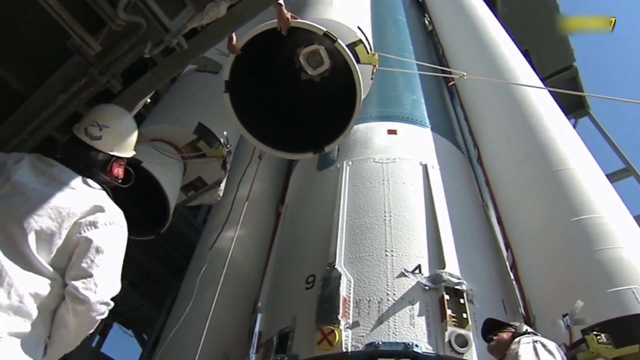 20 kilometres from the peaks to the ground below, and it's thought this may have formed because a ring that once circled the Moon collapsed onto its surface. Hyperion is the strange sponge-like Moon that tumbles around in Saturn's orbit, which, in 1848, was the first non-spherical Moon ever to be discovered. 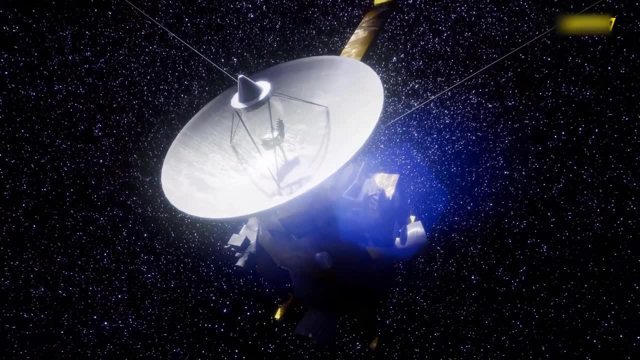 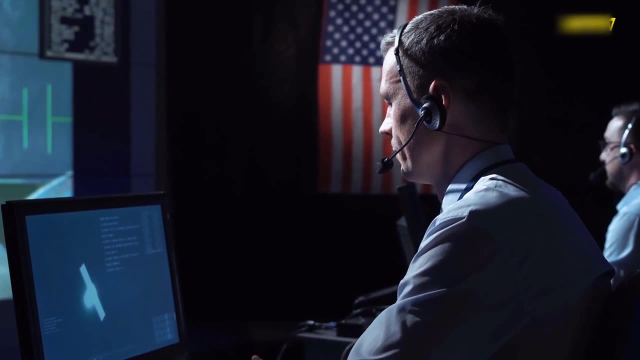 To this day, it remains a mystery as to what caused its punctured surface and irregular shape, and it's been suggested that Hyperion is in fact a remnant of another Moon that broke up long ago: Pan, the small walnut-shaped Moon that was discovered less than 30 years ago. 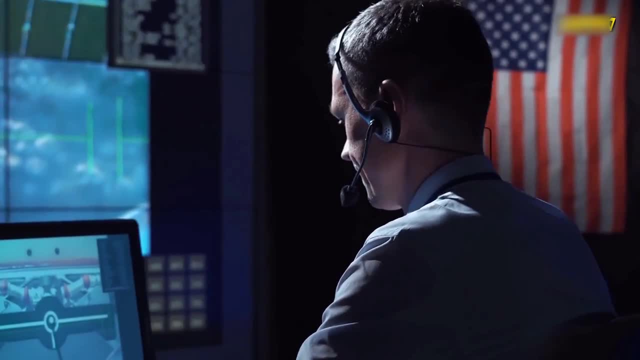 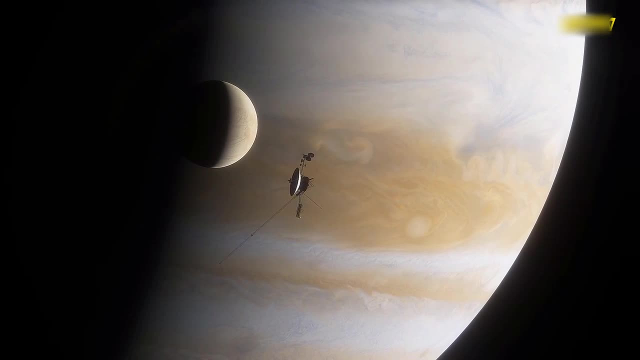 from the analysis of images taken by the Voyager 2 probe, is named after the Greek god of shepherds. It's so named because Pan is a shepherd Moon clearing the orbit of the Enker Gap, a 325-kilometre space within the A-ring. 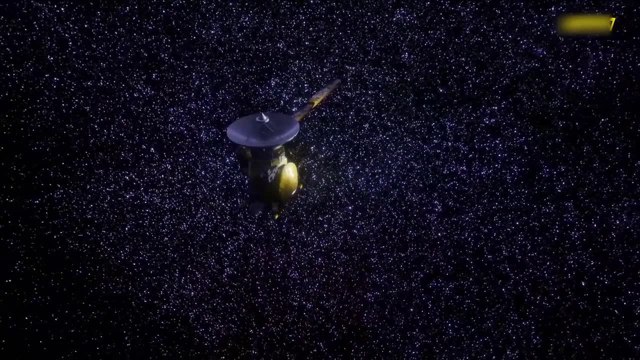 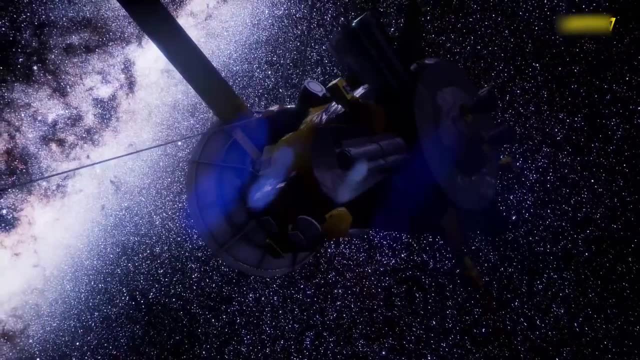 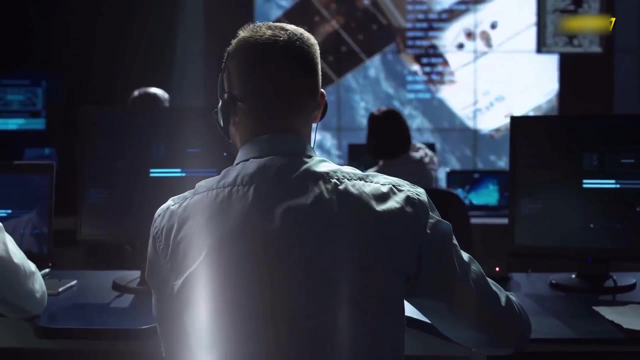 Its distinctive equatorial ridge is thought to be made of material that's been swept up and accumulated as it clears its path through the ring. Cassini's endless stream of images and data until 2017 has enabled scientists to analyse each of the Moons in ever more detail. 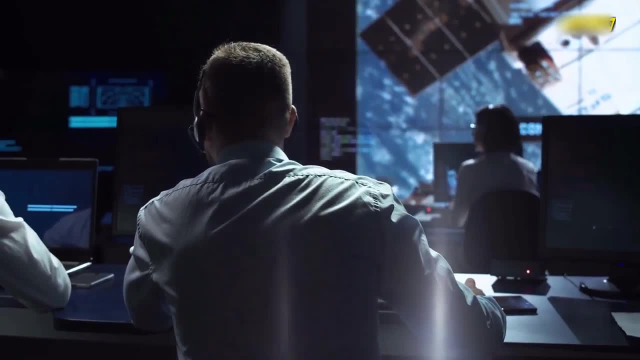 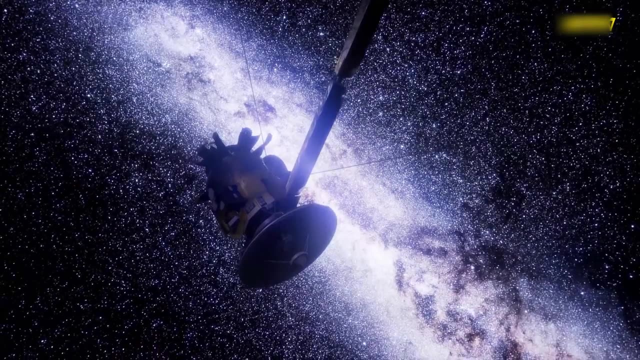 and it's become increasingly apparent that they are intimately linked with the ring system they orbit. Many of the Moons are made of exactly the same material as the rings themselves. Mimas, Iapetus and Hyperion are ice Moons composed almost entirely of frozen water ice. with only the smallest amounts of rock in their make-up. From the evidence that we've been able to read on Earth's surface, it seems almost certain that through 4 billion years of violent interactions, at least some of the Moons of Saturn must have both come and gone over the planet's history. 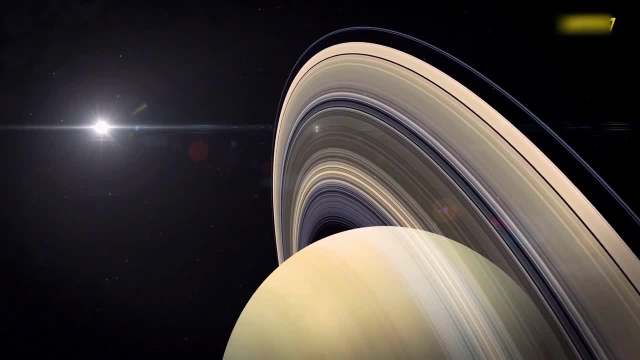 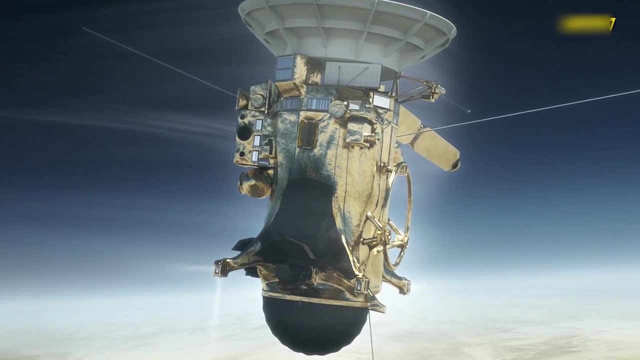 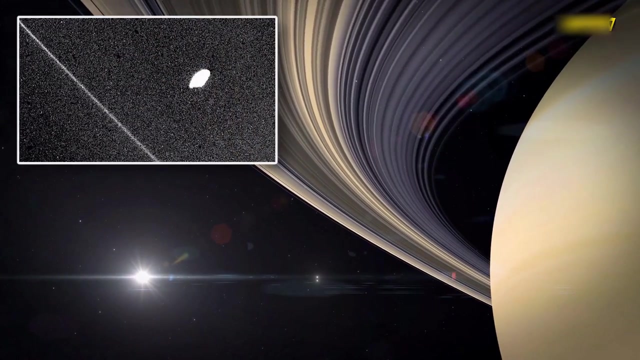 All of this begins to point us towards the idea that perhaps the most intriguing Moon in Saturn's long history is one that is now entirely missing. Around 200 million years ago, as dinosaurs roamed the Earth, we now believe a long-lost Moon. 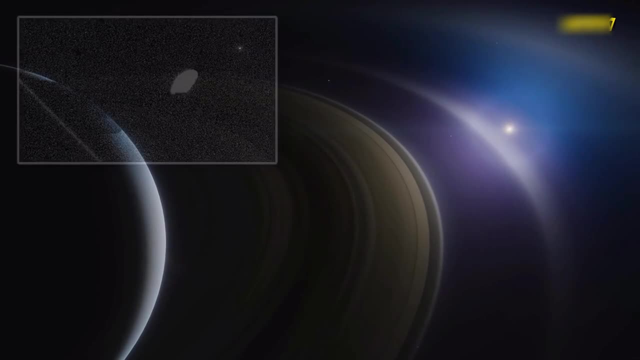 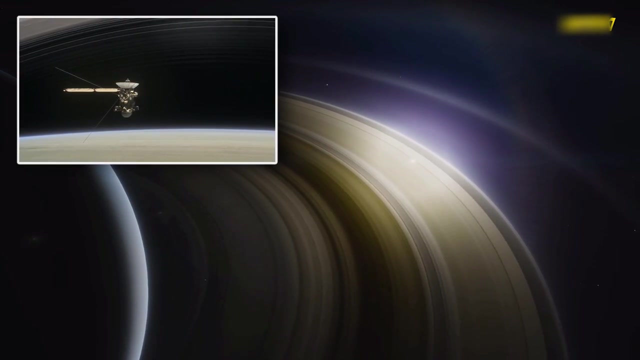 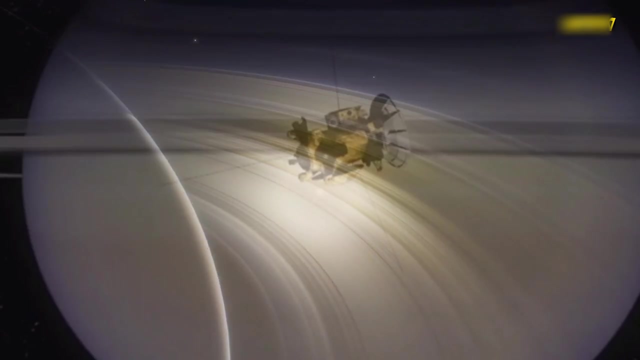 orbited close to the planet Saturn, a Moon perhaps 400 kilometres across and formed almost entirely of ice. This was a doomed world, orbiting too close to resist the immense pull of Saturn's gravity, its fate sealed at the moment of its birth. 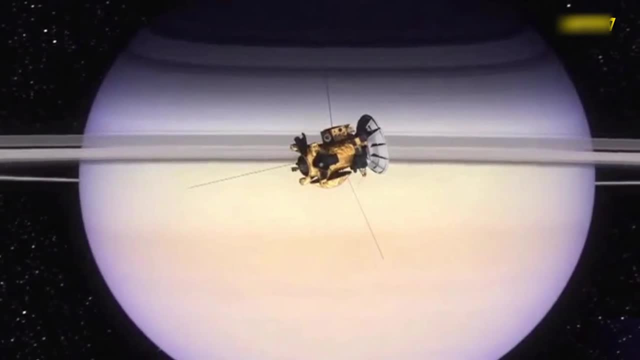 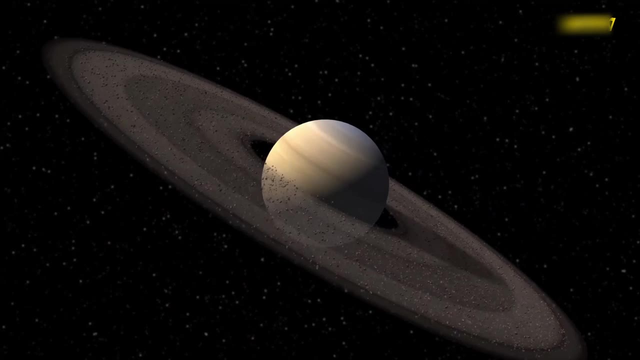 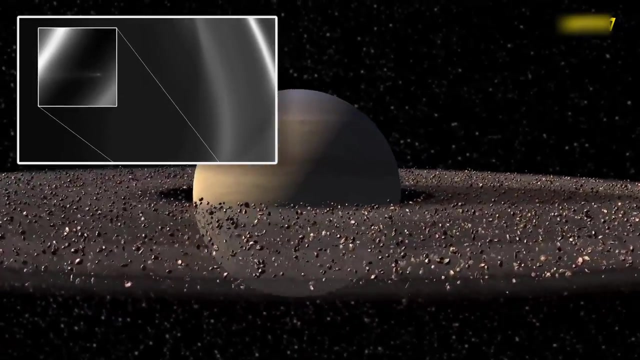 It was the French astronomer and mathematician Edouard Roche who first suggested the existence of this long-lost Moon in 1848.. He christened it Veritas after the Roman goddess of truth, though according to legend is supposed to have hidden in the bottom of a holy well. 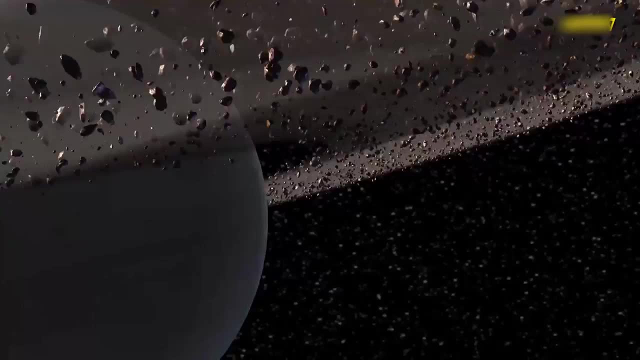 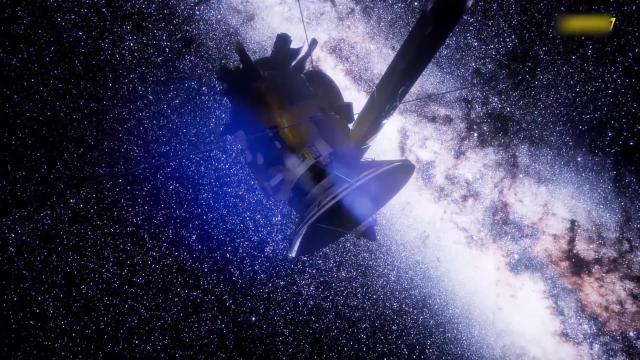 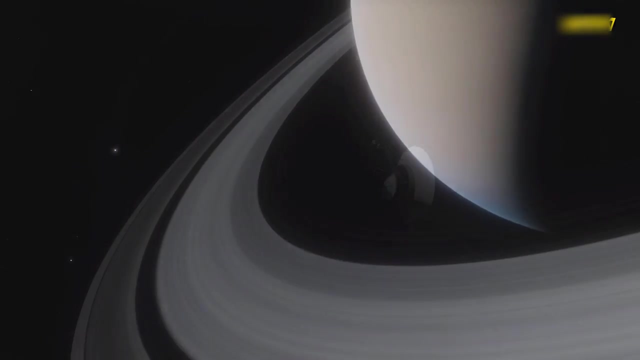 Roche had postulated the existence of this Moon. while exploring a particular dynamic of celestial mechanics that describes the potentially violent gravitational relationship between two celestial bodies, He was able to demonstrate that when a Moon moves within a certain distance of the planet, it is orbiting. 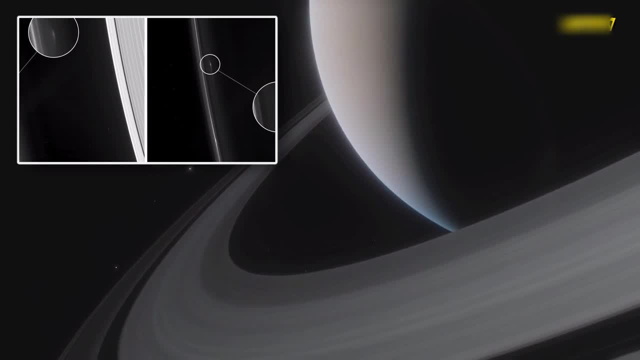 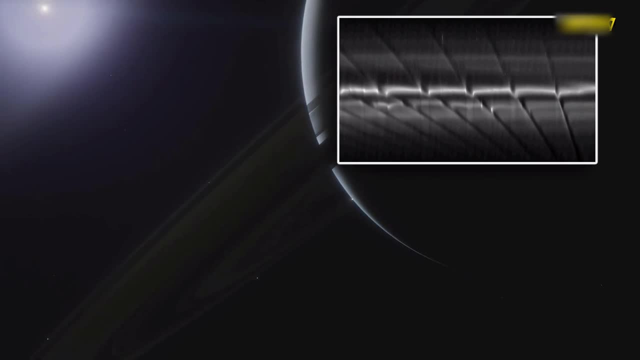 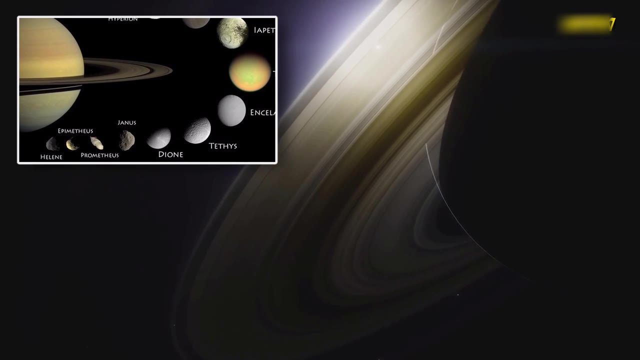 it can cross a threshold where the force of gravity is so strong, the Moon will be ripped apart. This distance has become known as the Roche limit and is dependent on many factors, including the mass, radius and physical characteristics of the Moon and planet. 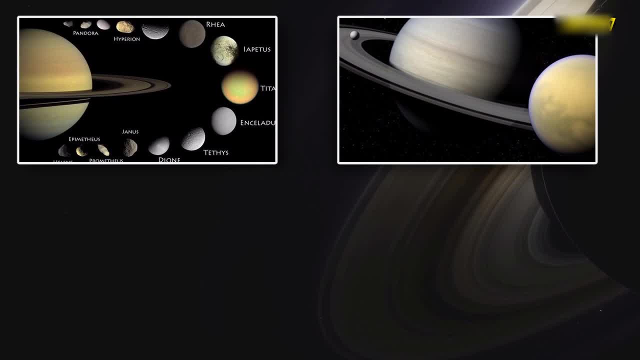 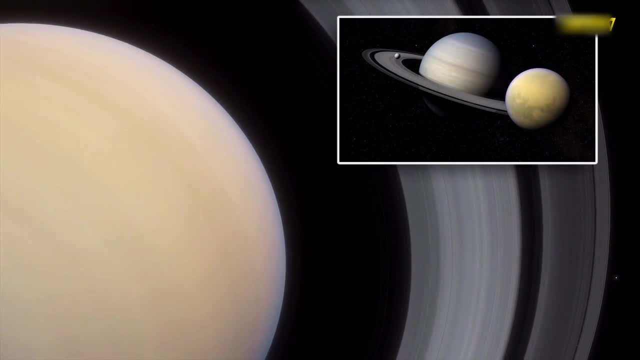 Outside of the Roche limit, a Moon can exist in happy equilibrium with its planet, orbiting in the gravitational grip of the larger body while maintaining its physical integrity, But if that same Moon's orbit degrades to the point where the Roche limit is crossed, 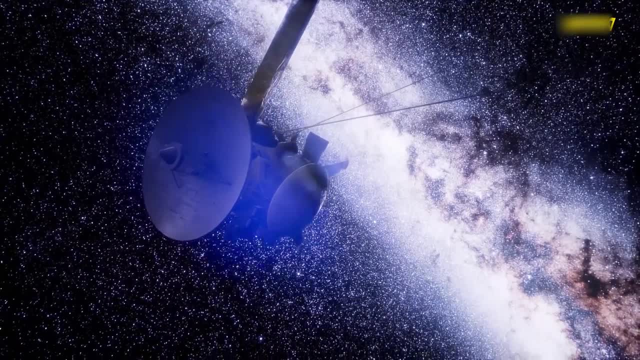 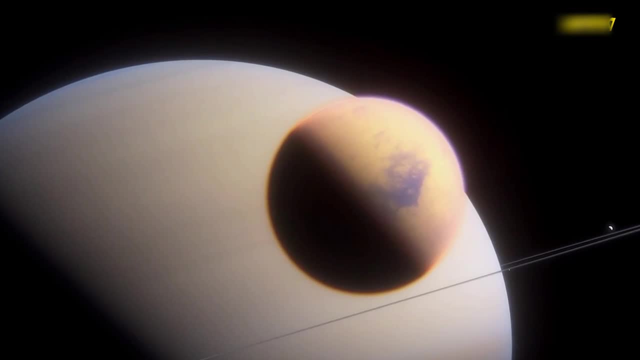 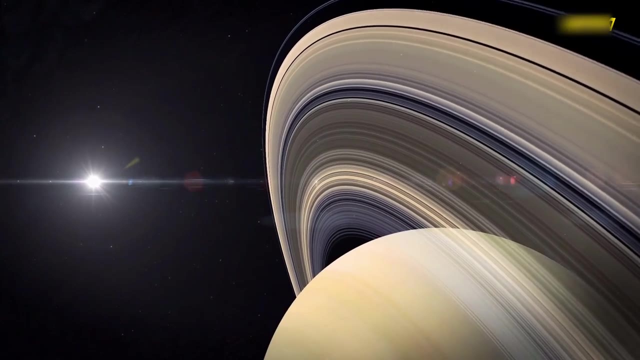 the tidal forces exerted on the Moon exceed the gravitational attraction that holds the Moon together in a sphere, resulting in the Moon's destruction. This relationship applies to any Moon-planet system, including our own. Here on Earth, we see the relationship between our planet and Moon on a twice-daily basis. 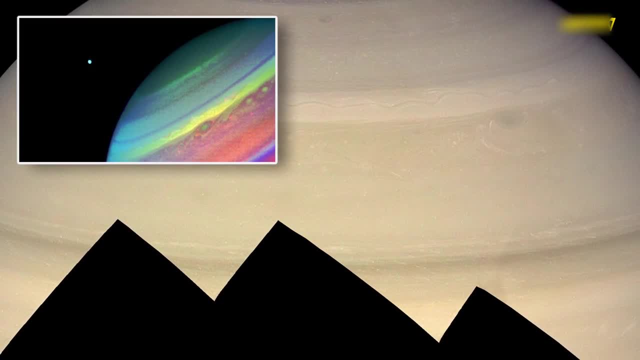 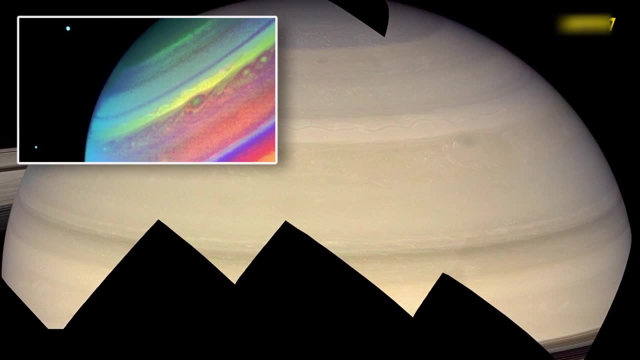 as the tides ebb and flow across the planet. These tides are caused by the difference in the gravitational pull of the Moon from one side of the Earth to the other, And that difference, although subtle, is powerful enough to move entire oceans. 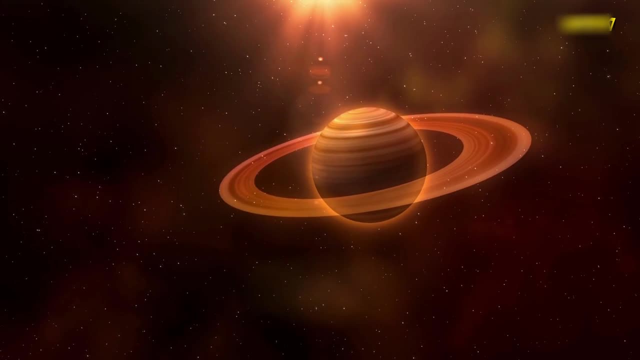 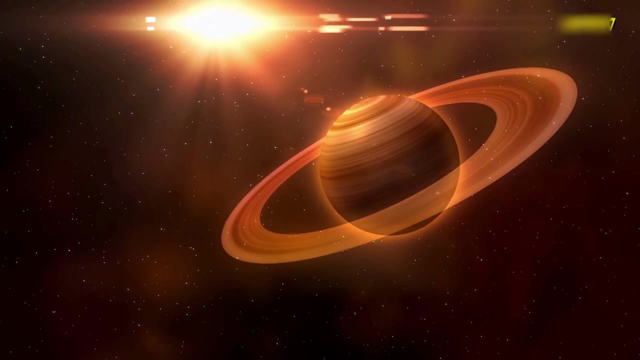 with the forces of tidal gravity. Just as the Moon creates tides on Earth, so the Earth also has a tidal effect on the Moon, And because the Earth is much greater in mass, that effect is more powerful than you might think. The Earth's pull is in fact powerful enough. to deform the Moon's surface. even today it causes moon tides on the lunar surface, where it causes the rock to rise and fall. But the effect was even stronger 4 billion years ago, when the Moon was nearly 17 times closer to the Earth. 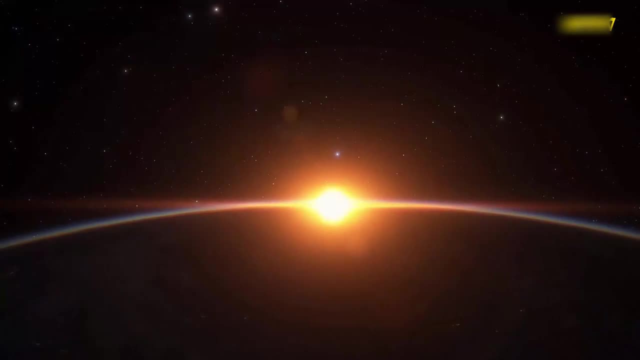 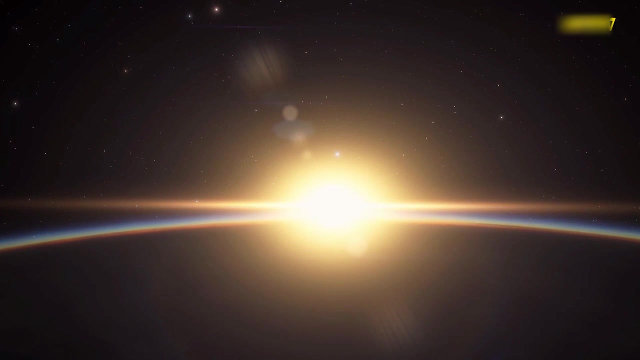 Back then, the pull from our planet caused a tide of solid rock to rise and fall by many metres, and if the Moon had ever come any nearer, it would have crossed the Roche limit and been ripped apart When Édouard Roche first formulated the expression. 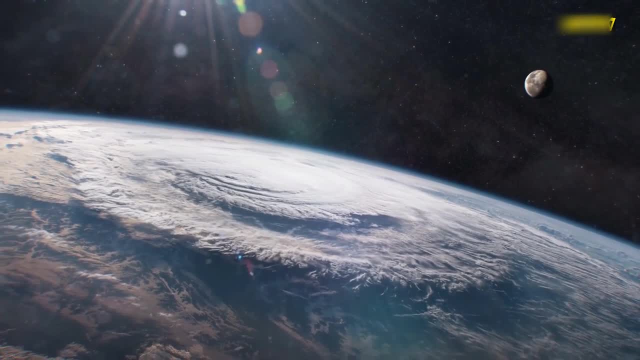 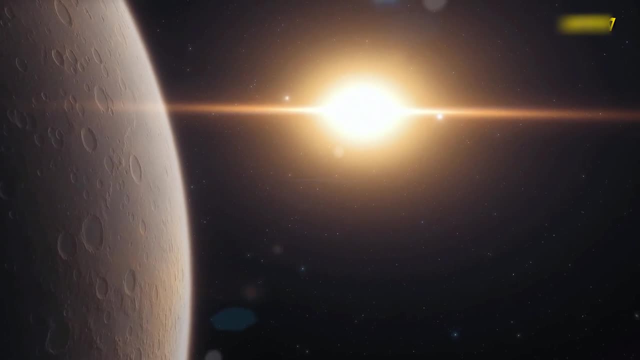 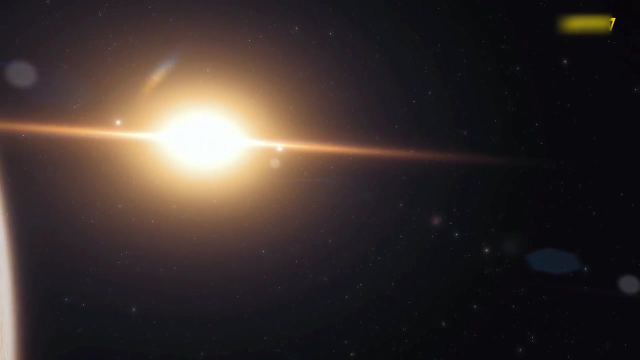 of the equations calculating this line. he realised that the result of such destruction would not just be the obliteration of a Moon, but also the creation of millions upon millions of fragments, the debris of the Moon orbiting around its destroyer. He also deduced that, in time, these fragments would form once again. 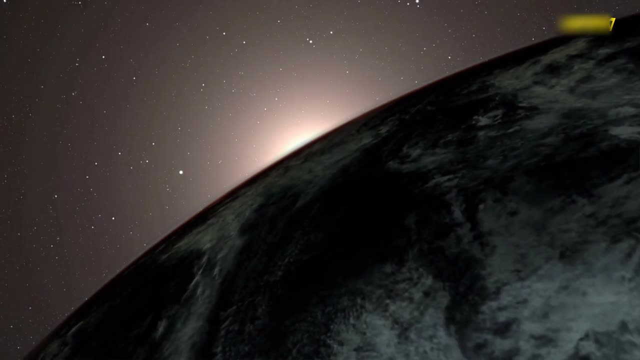 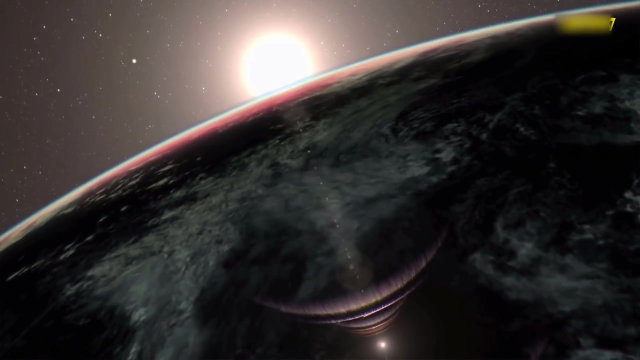 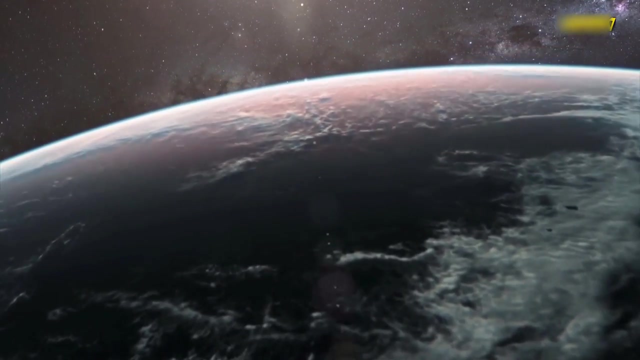 into the most delicate of structures, a system of rings, under the influence of the planet's gravity. In one of the more gruesome tales from classical mythology, Saturn, the Roman god of time and harvest, actually ate five of his newborn babies to prevent them taking his power. 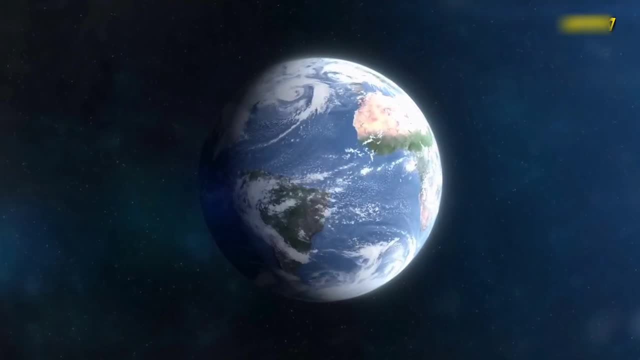 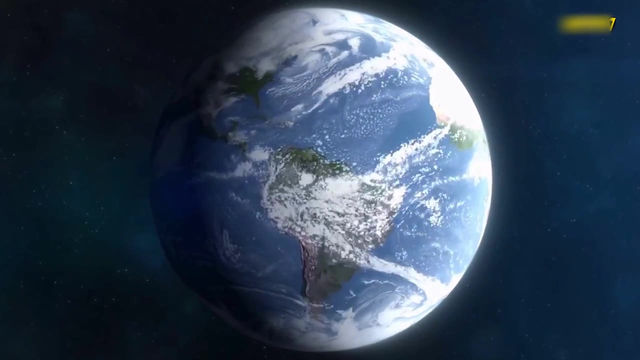 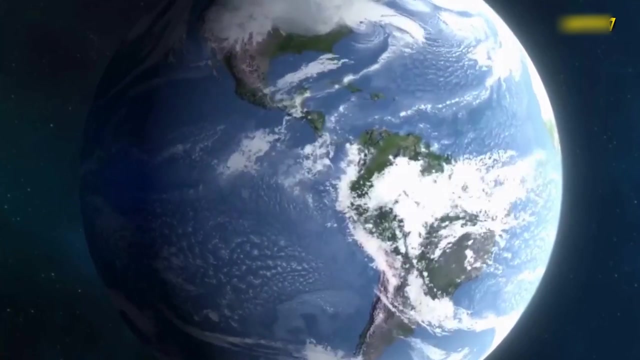 Now Cassini has shown us that, at least metaphorically speaking, they weren't far wrong. We now think that 10 to 100 million years ago, just beyond the outer reaches of Saturn's vast atmosphere, an icy Moon orbited, gradually, edging closer and closer to that tipping point, the Roche limit. 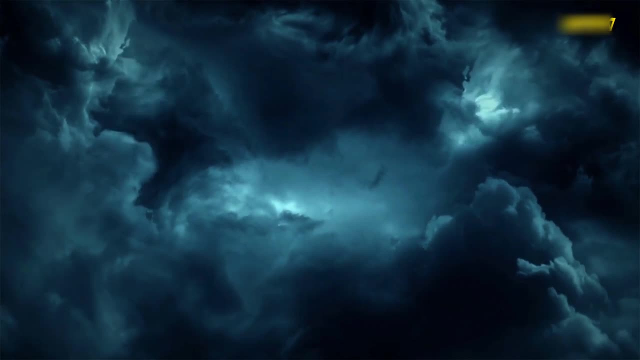 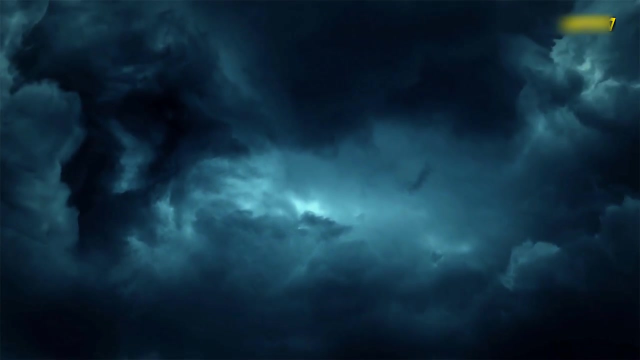 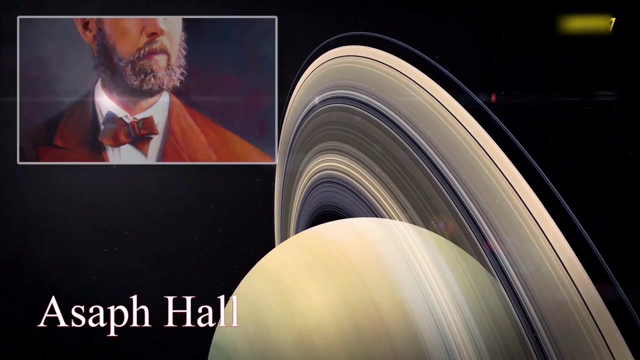 As Saturn's immense gravitational force pulled at it, this great Moon began to rupture And, in a moment undoubtedly worthy of even the greatest of mythological stories, up to 30 million trillion tonnes of ice, more than 30,000 times the weight of Mount Everest. 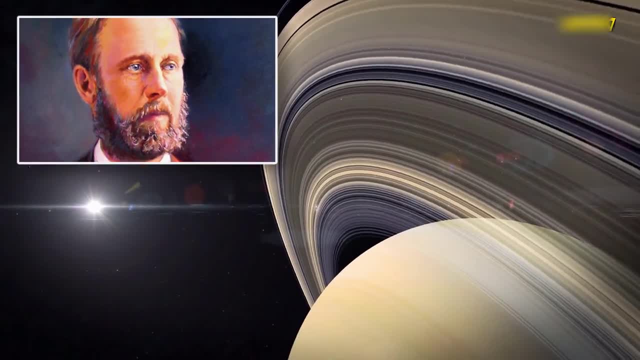 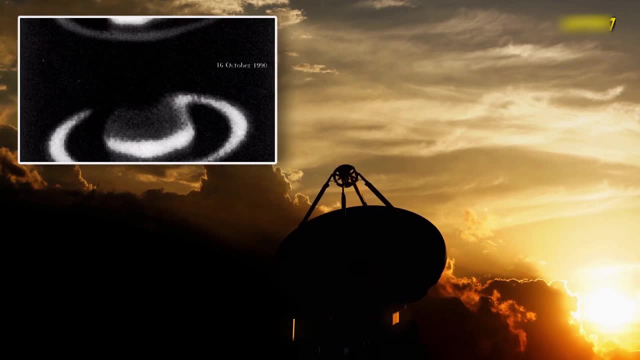 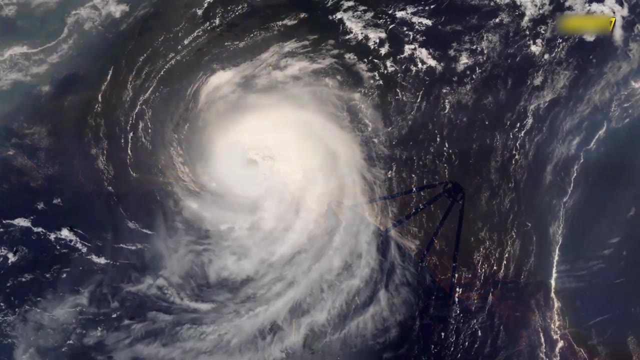 broke apart in orbit and spread out around Saturn, Travelling at tremendous speed around the planet. it's likely that this debris quickly disappeared and was only scattered to encircle the giant planet, And in the space of no more than a few days, Saturn's iconic rings had been born. 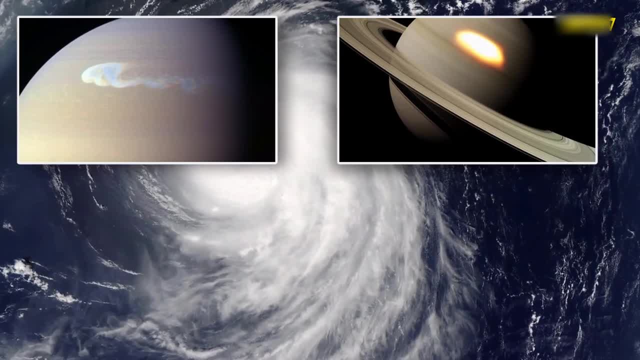 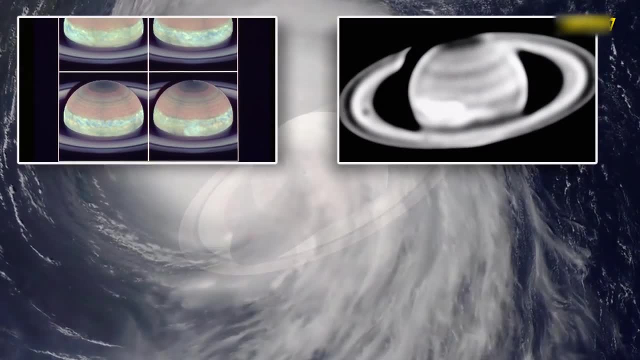 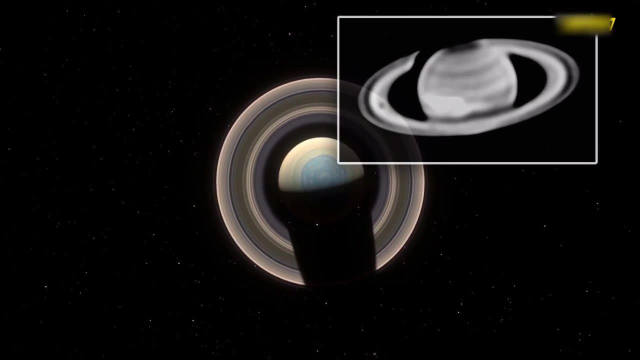 Today, this giant ring system has evolved into the intricate structures we can see in the night sky. Saturn's powerful gravity has helped keep its near-perfect elliptical shape, but an endless series of collisions have caused it to gradually flatten out. Now this debris forms a disk wider than Jupiter. 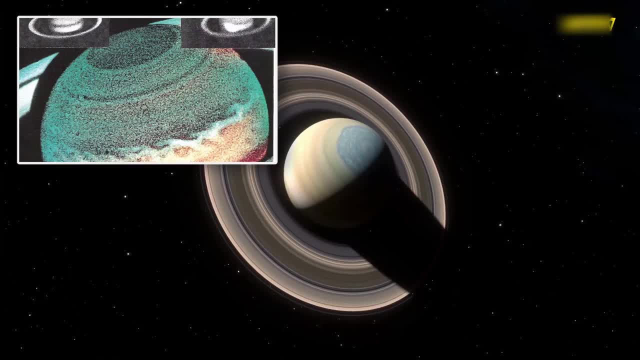 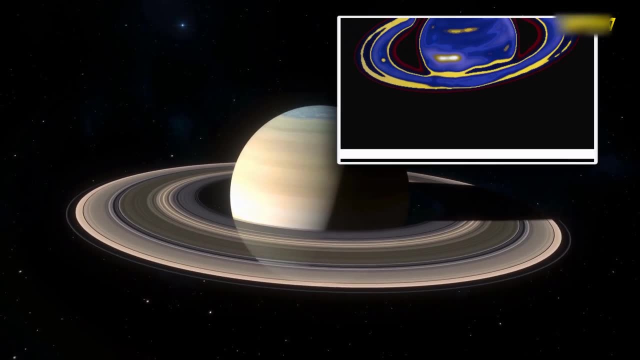 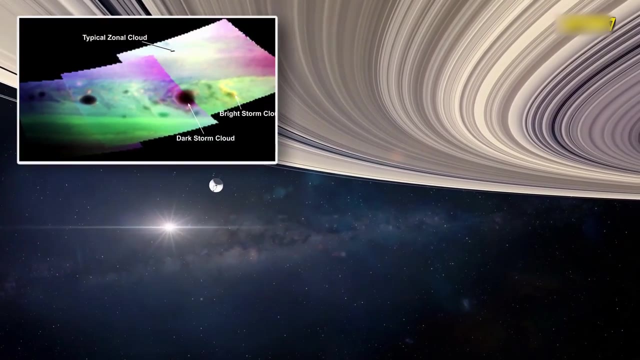 yet on average, just 10 metres thick, With Moon-sized chunks of ice orbiting through this structure. great voids have been cleared, turning one ring into many. In places, Moons have pulled particles of ice upwards to create strange peaks over a kilometre high. 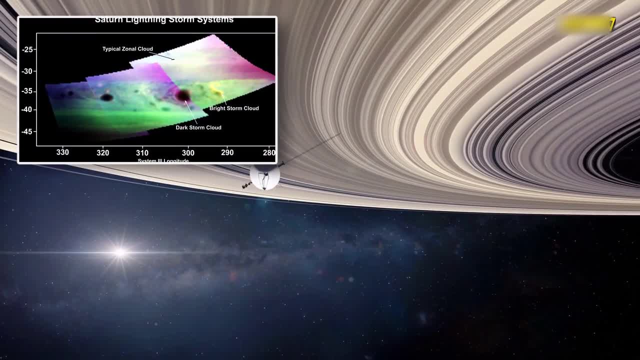 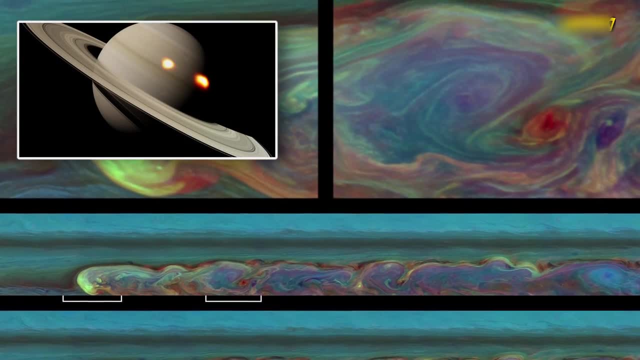 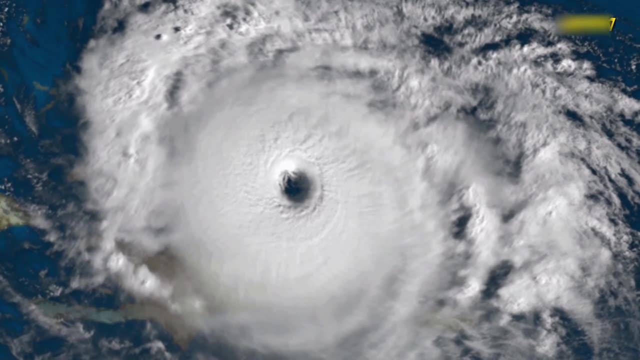 which cast spectacular shadows across the rings. Saturn, once a tiny world of rock and ice, a world that has undergone repeated transformations, has today, by chance, become the solar system's greatest jewel And Cassini, our most intrepid of explorers. 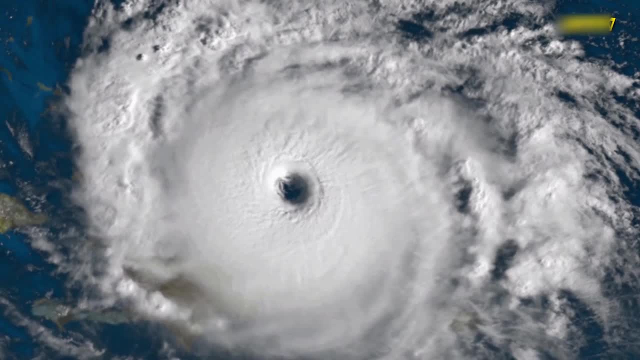 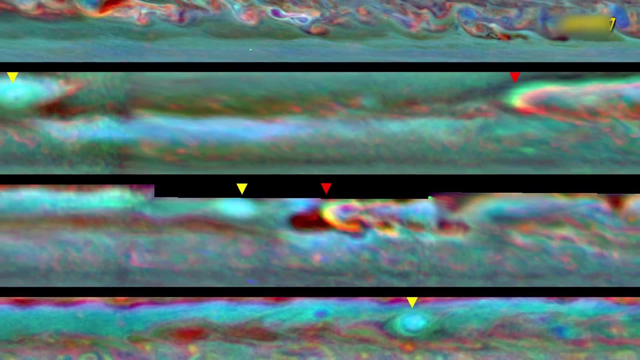 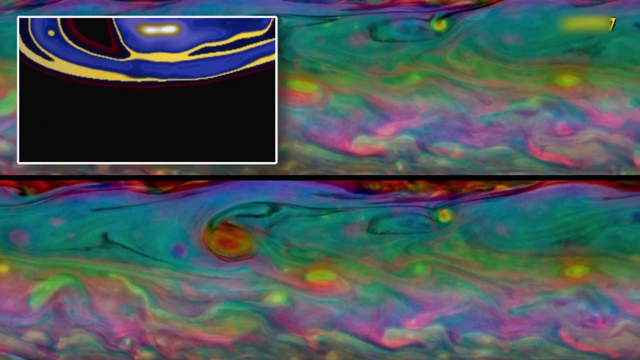 has forever deepened our understanding of the life story of this planet. Yet perhaps Cassini's greatest gift is not in its revelations of the past, but in the glimpse it has given us of the future, Because just beyond Saturn's rings, Cassini would discover a hidden treasure. 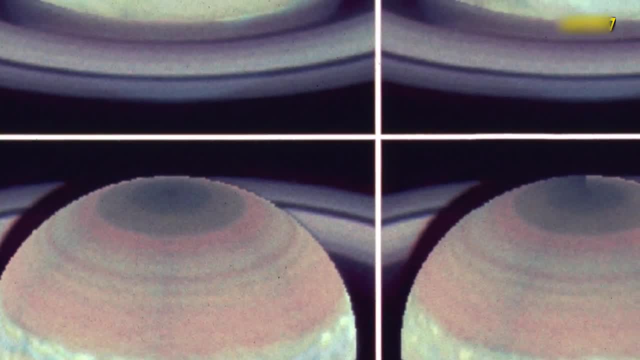 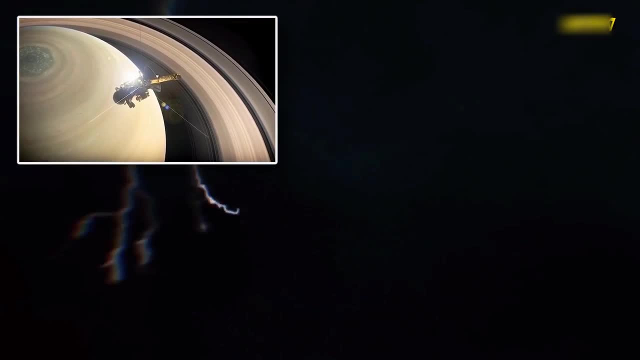 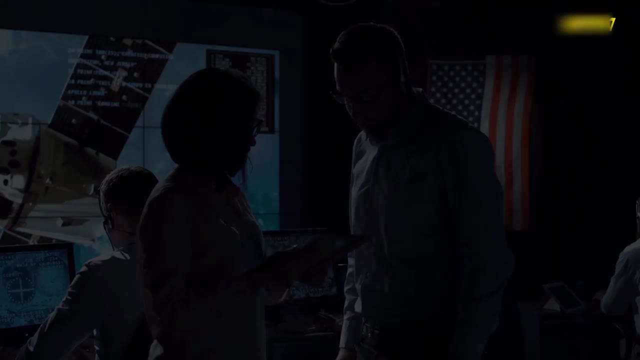 a world that may hold answers to some of our deepest questions about our place, not just in the solar system, but in the universe. One of the unmistakable jewels of the Saturnian system is Titan, A giant. it is the second largest Moon in the solar system. 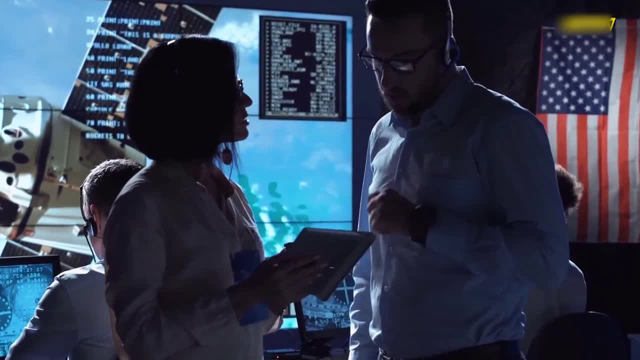 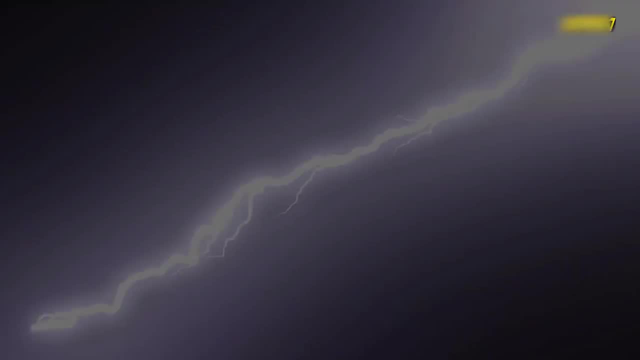 and this planet-sized satellite is larger than the smallest planet, Mercury, and 50% bigger than our own solitary Moon, Discovered by Dutch astronomer Christian Huygens in 1655,. it has held its secrets close for centuries, cloaked by thick clouds. The only Moon in the solar system with a dense, distinct atmosphere of its own. From afar, Titan hinted at being far more like a planet than a Moon. It would take a mission of breathtaking ambition to finally peer under her veil and see the wonders that lay beneath. 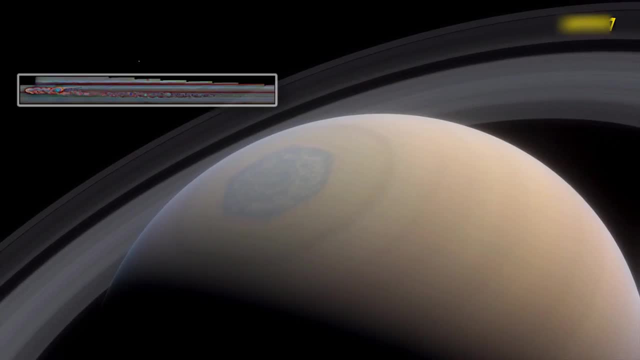 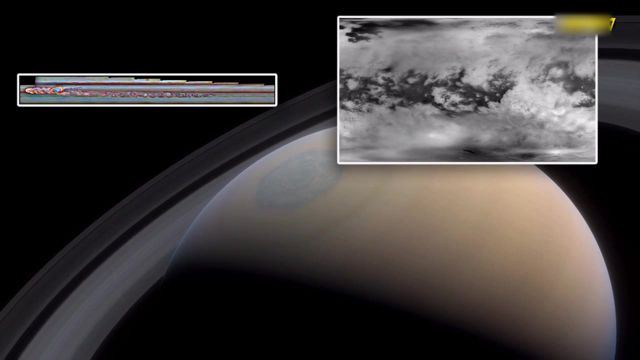 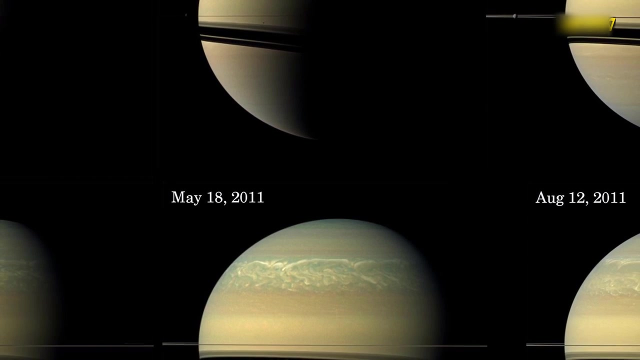 On Christmas Day 2004,, after a seven-year journey across the solar system, the Cassini probe released its sibling craft, Huygens, setting it off on a four-million-kilometre path to Titan. Simple in appearance, Huygens looked as if it had borrowed its design. 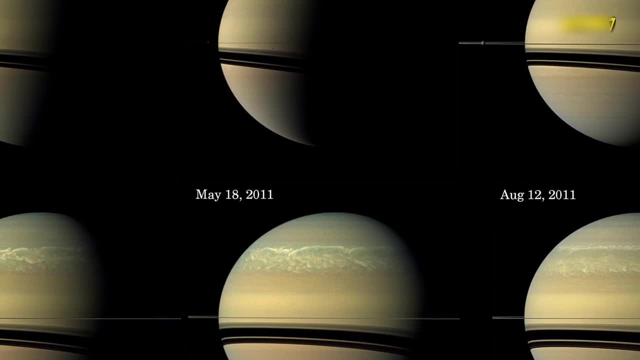 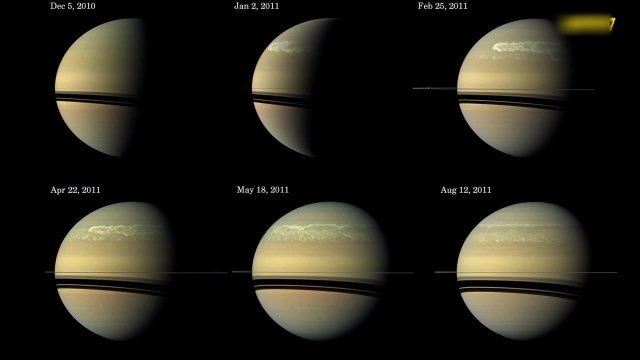 from the classic cartoon UFOs of the 1950s. But nothing was simple about Huygens. This was a highly advanced spacecraft about to begin one of the most complex manoeuvres ever attempted in the history of human space exploration, As it made its way to Earth. 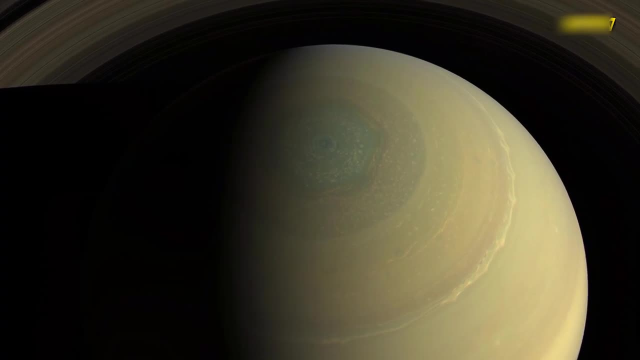 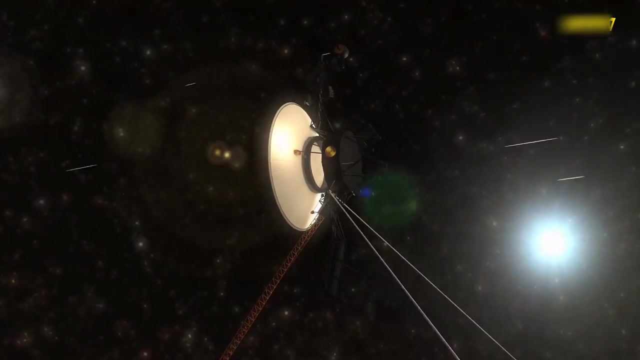 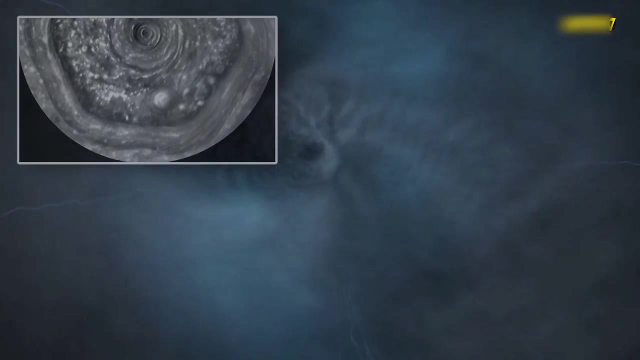 on its three-week journey towards Titan. the team of ESA- European Space Agency- scientists, who had dedicated a lifetime's work to the project, watched on hopeful but helpless. From the moment of release. they had lost direct control of the probe and were unable to send it commands. 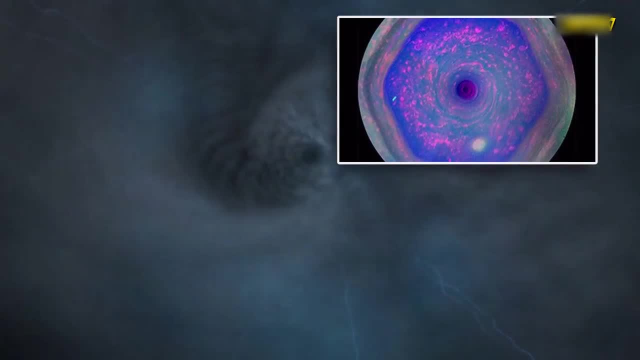 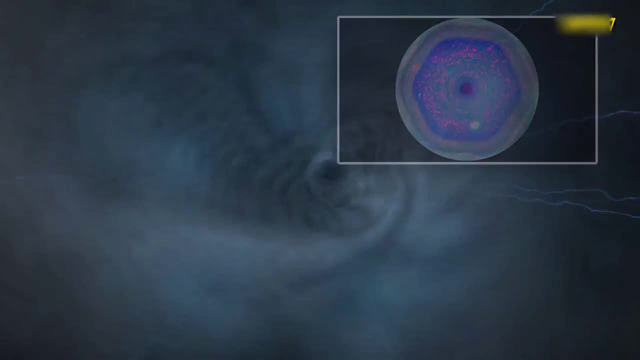 Instead, as planned in the mission protocol, Huygens was now entirely controlled by the on-board autonomous computer systems. All they could do was watch and wait to see if Huygens could fulfil their ambitions by becoming the first probe to land in the outer Solar System. 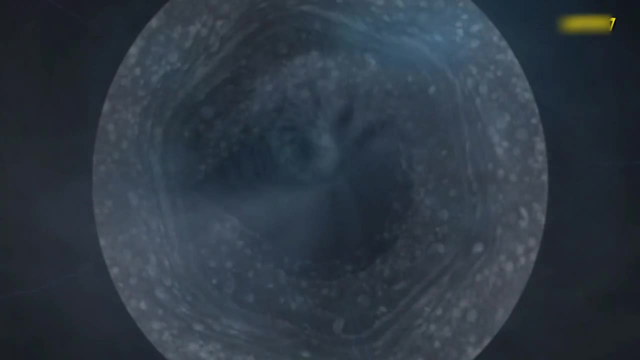 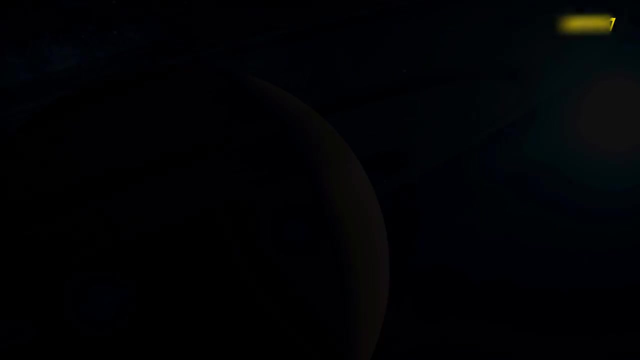 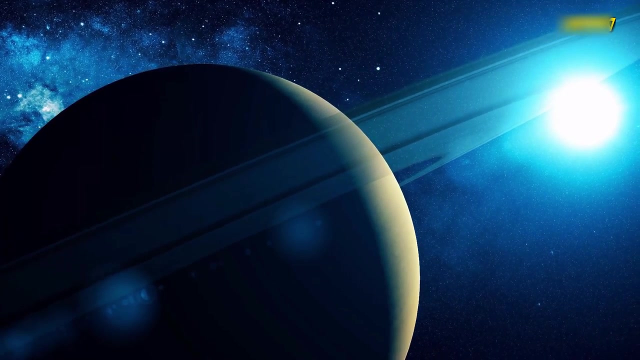 on a Moon other than our own in the most distant landing of any spacecraft. To succeed, Huygens would have to execute a perfectly controlled landing protocol designed to use Titan's atmosphere as an aerobrake, before employing a parachute system to deliver the scientific instrumentation to the surface. 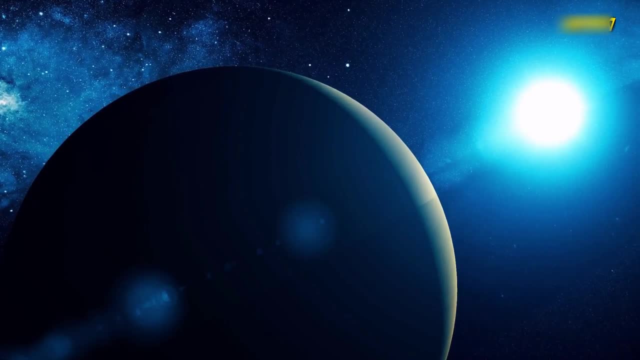 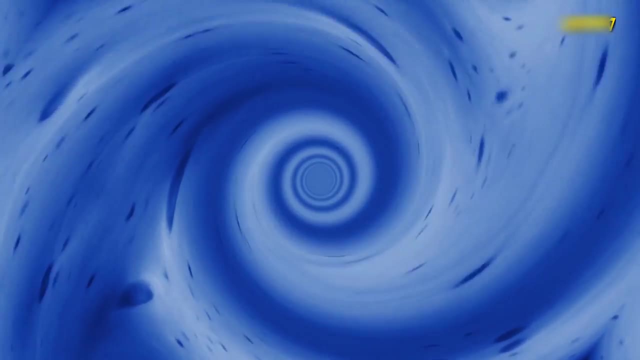 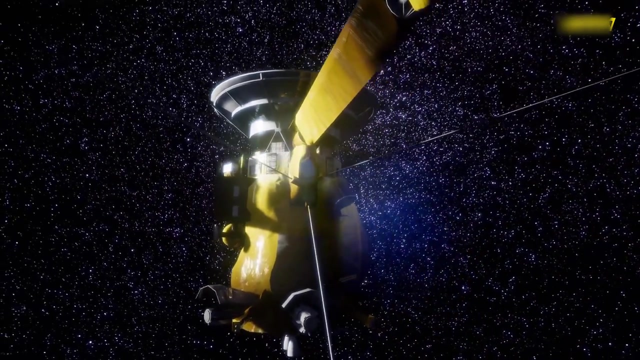 And all after awakening itself from a 6.7-year intergalactic sleep. The probe had remained in an entirely dormant mode except for a six-monthly self-health check, and only at the point of separation from Cassini was the timer set to wake the probe up. 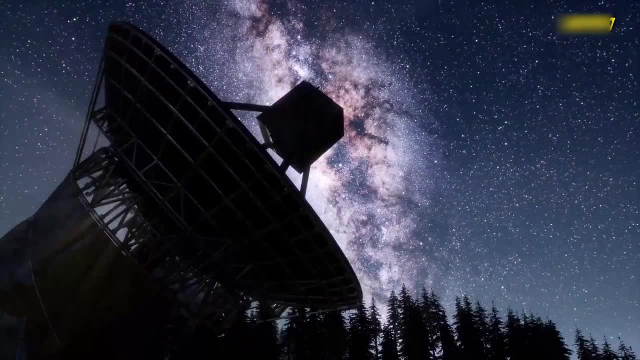 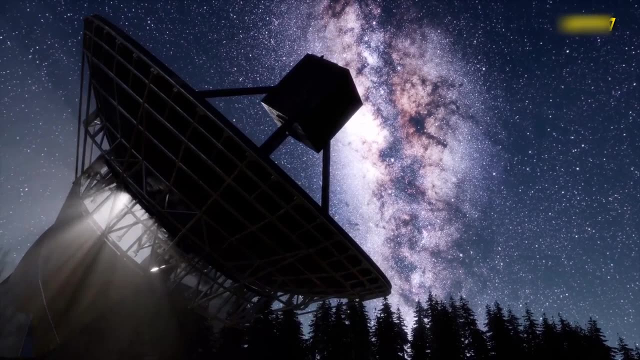 15 minutes before entering the atmosphere of Titan. The proposed landing site for Huygens also held much uncertainty, Chosen to be in the southern hemisphere of Titan, 192.3 degrees west, 10.3 degrees south to be precise. 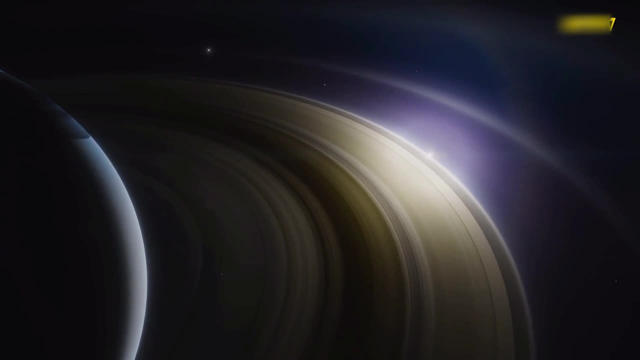 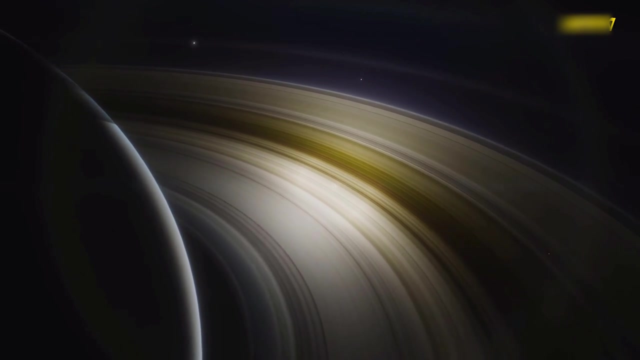 The area was surveyed by Cassini's cameras from an altitude of 12,000 kilometres and appeared to be near a site that had many of the characteristics of a shoreline. Landing into an extraterrestrial ocean had been part of Huygens' original design. so in theory the craft was expected to survive any splashdown into a liquid surface on Titan. On 14th January 1916, or 2005,, the 318-kilogram probe entered Titan's atmosphere 1,270 kilometres above the surface. 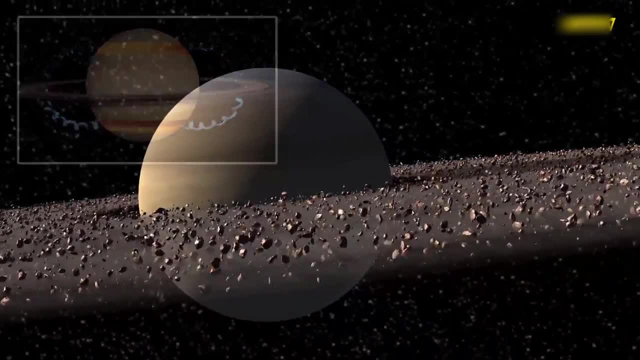 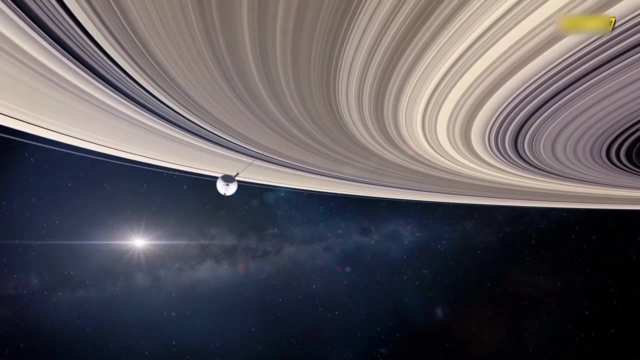 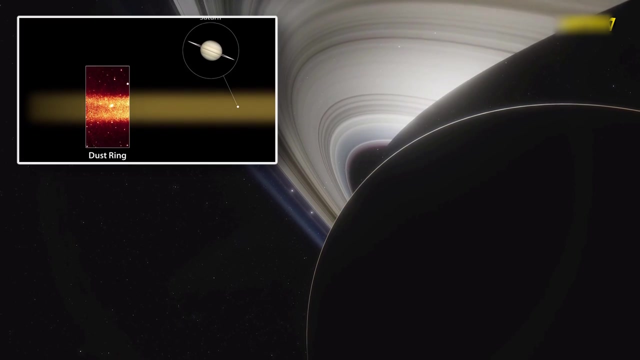 and began its descent protocol. On-board accelerometers monitored the craft's deceleration, waiting for the precise moment to trigger the explosive bolts that would blow off the front heat shield and back cover and release the pilot parachute, which would then pull out the main parachute. 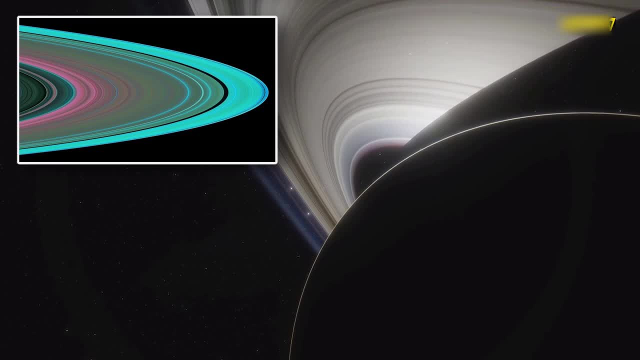 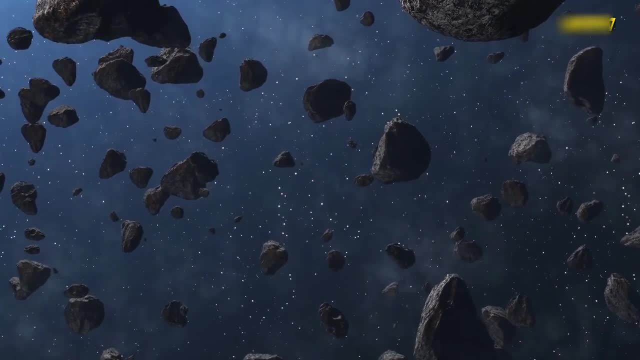 slowing the 2.7-metre rocket from its nearly 2,000-kilometre-per-hour descent and allowing it to drift safely to the surface. All of this would need to play out perfectly while more than a billion kilometres away. 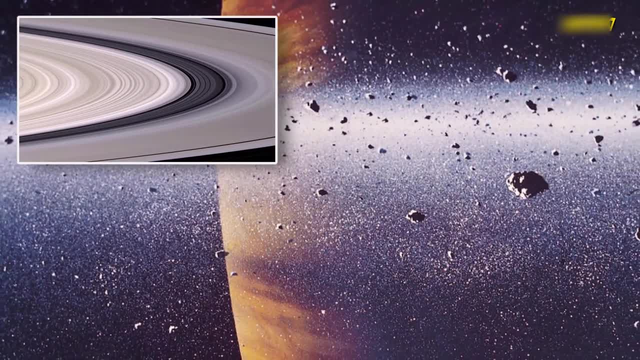 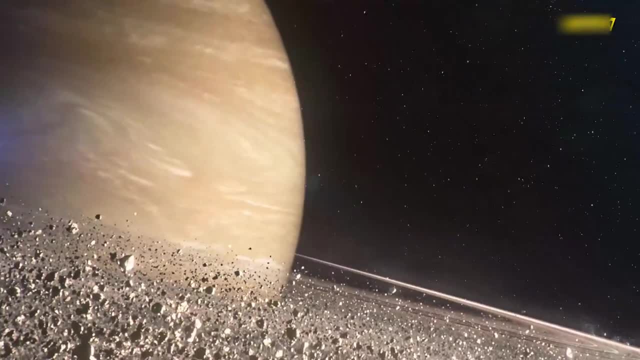 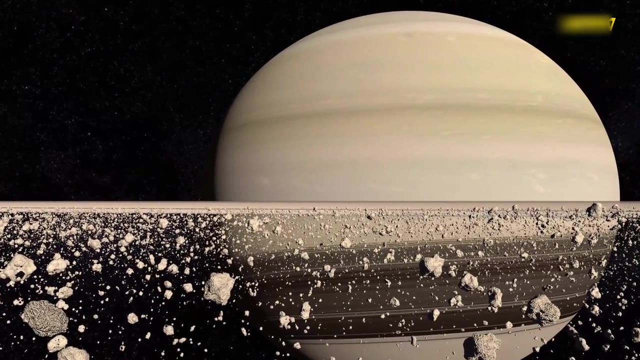 a group of nervous humans sat in near silence in mission control waiting for the first telemetry to confirm that Huygens was safely on the ground. Every second was utterly critical because Huygens had no more than three hours of battery life and with an expected 150-minute descent. 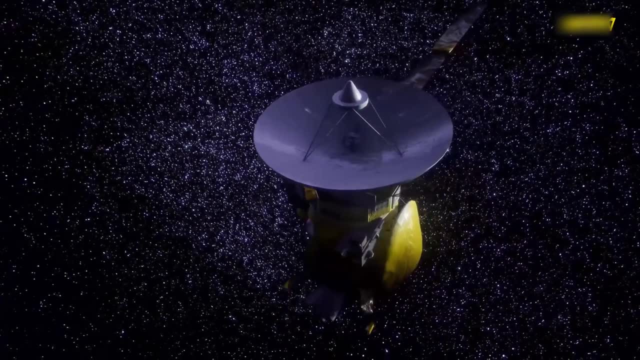 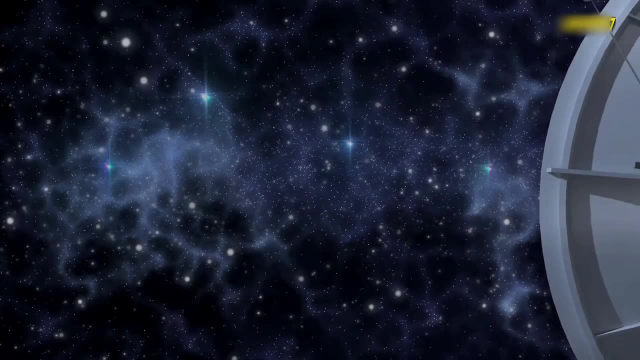 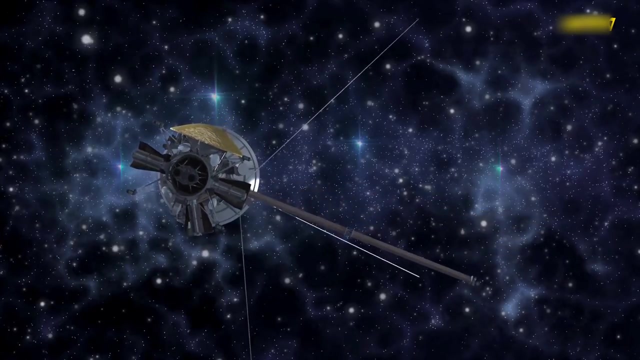 that meant not much more than half an hour's activity on the ground For a mission that had cost millions of dollars and taken decades to plan and execute. its success would depend on this incredibly short window of exploration. Despite its sophistication, Huygens could not communicate directly in any detail with Earth. 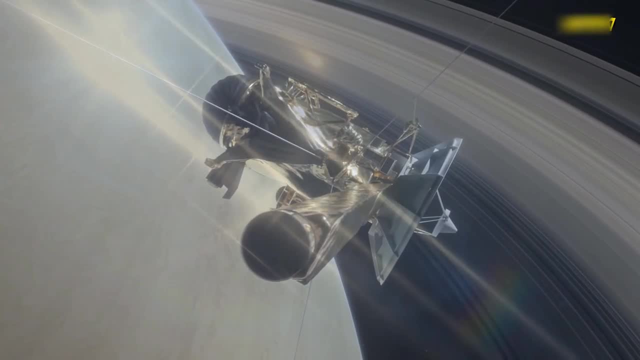 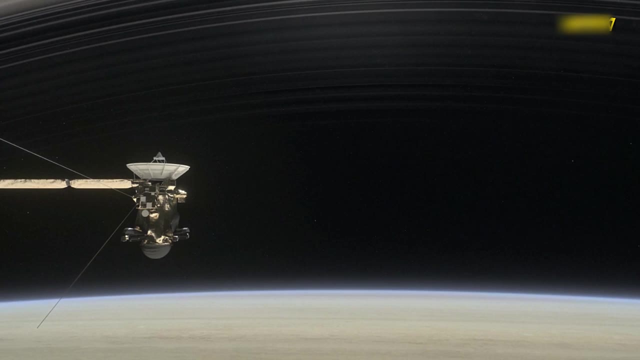 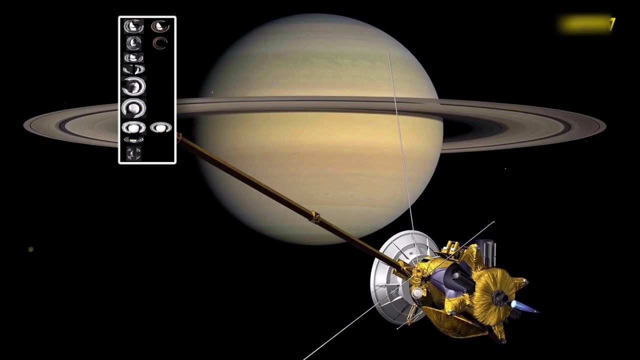 Instead, all of its detailed telemetry would need to be relayed to Earth or sent back to Earth via Cassini's communications system. This meant very little was known about the probe's status during the two-hour and 27-minute descent, But at precisely 11.38 UTC. 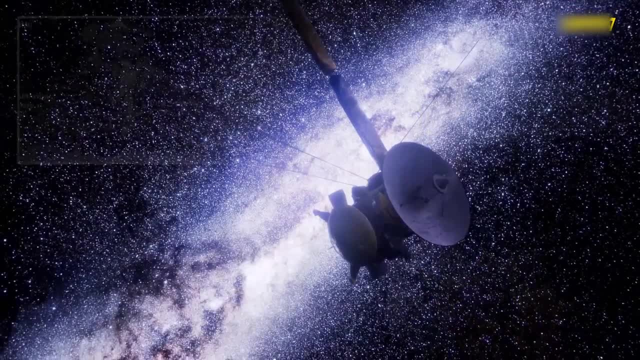 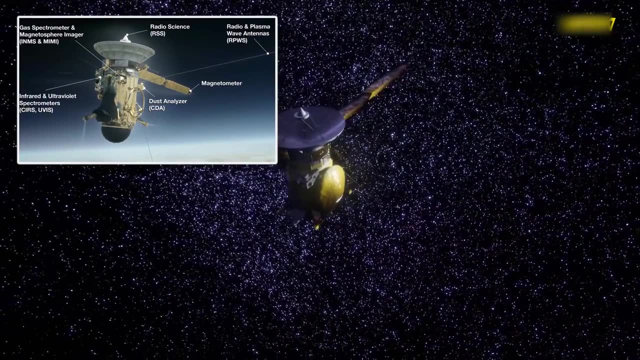 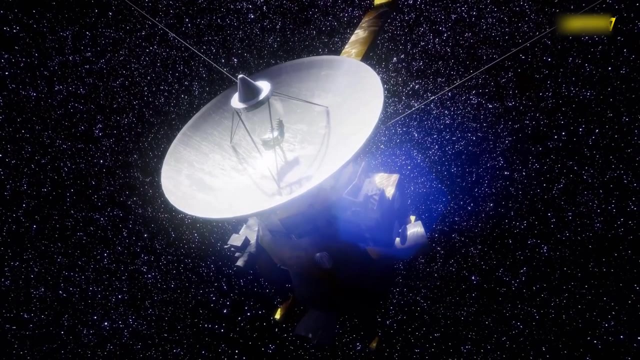 the Robert C Byrd Green Bank Telescope in West Virginia picked up the weakest of carrier signals generated by Huygens' 10-watt internal transmitter, to confirm that Huygens had arrived safely on the surface. This extraordinary probe was now alive and active. 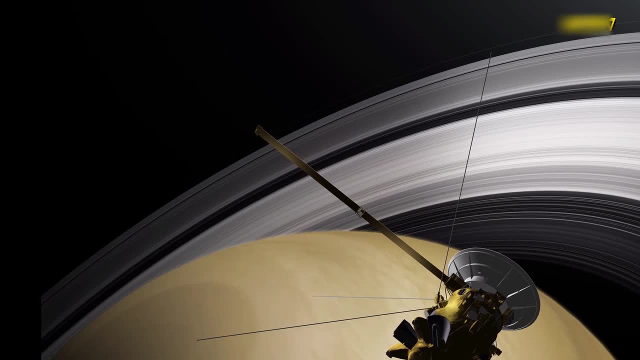 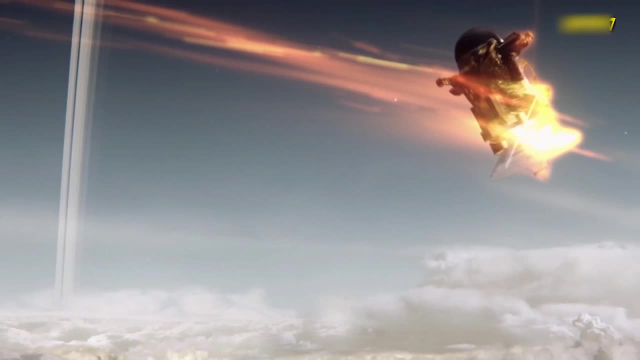 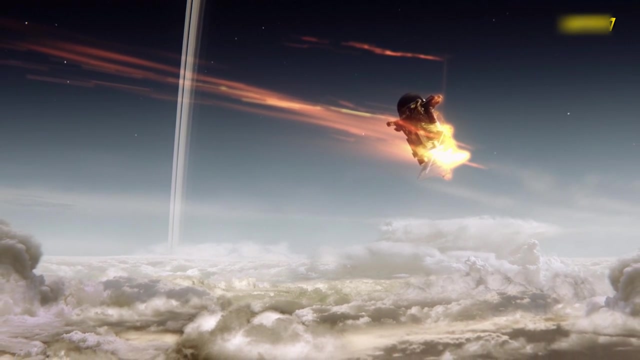 on an alien moon orbiting Saturn. Just under five hours later, the Cassini probe, orbiting far above the moon's surface, began relaying the precious data from Huygens back to Earth, And by 1945, that evening, the first extraordinary picture was released. 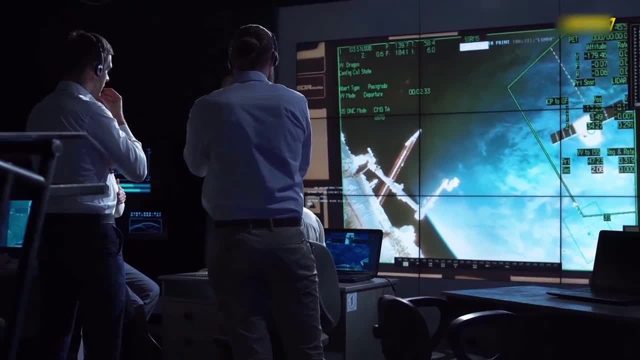 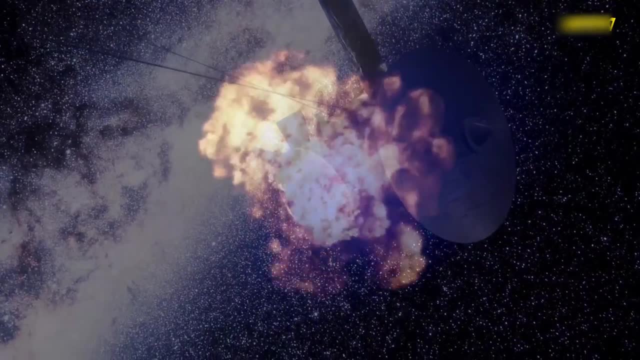 showing a view from Huygens about 16 kilometres above the fast-approaching surface. This was sped up with space exploration on an awesome scale: A photograph taken by a tiny space probe floating down on a parachute to the surface of a moon. 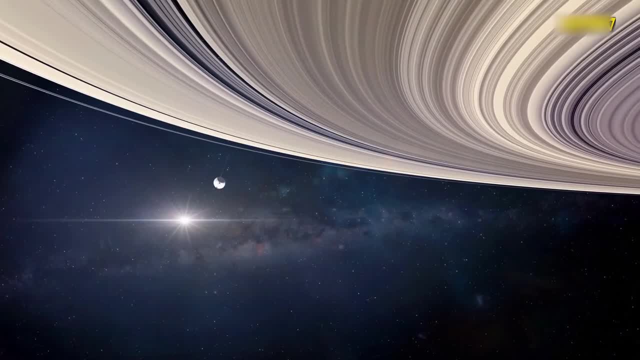 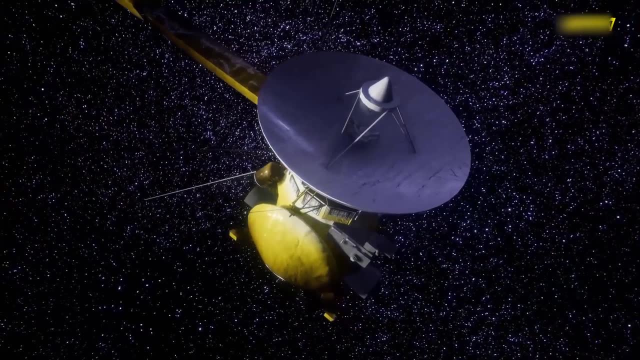 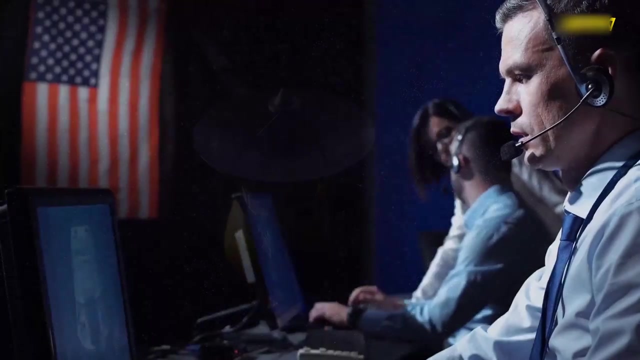 orbiting a planet over a billion kilometres from Earth. It's instantly apparent that this is no featureless rock. The channels running across this picture are recognisable as the geology of a world shaped by liquid covered in drainage channels crossing the landscape into what looks like a lake bed or sea. 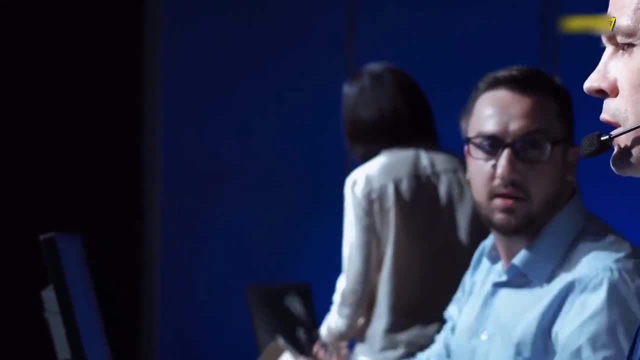 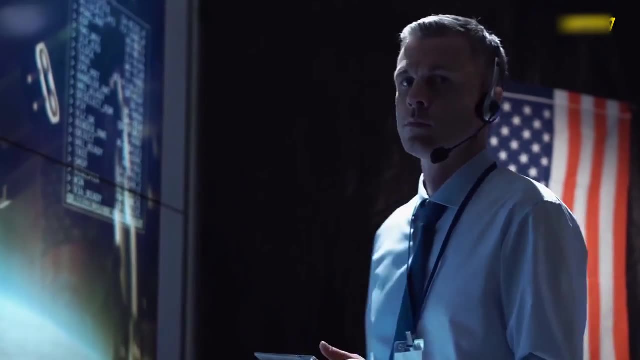 And more was to rapidly follow. Just a few minutes later, the first image from the surface arrived on Earth, The first view of the surface of a world in the frozen far reaches of the solar system. It's an image that is worthy of the very closest of inspection. 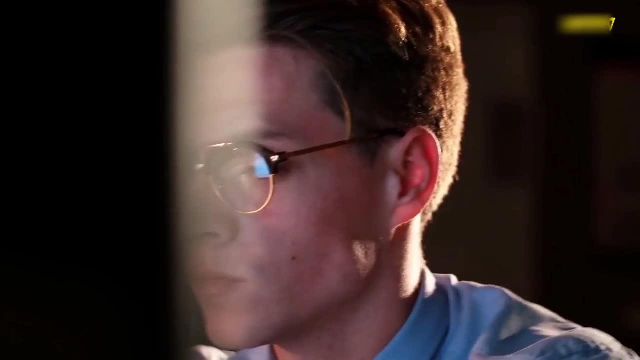 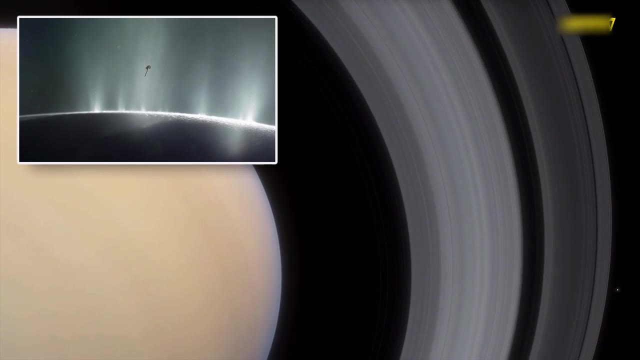 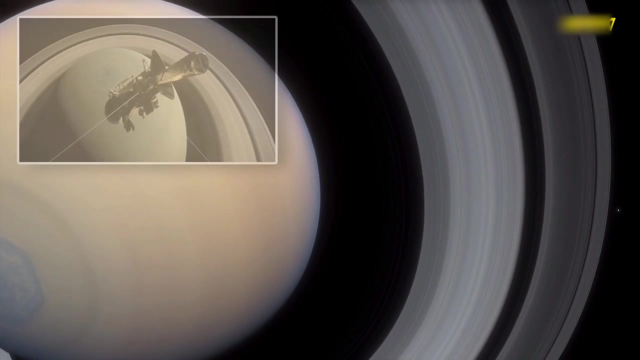 because, as always in science, the more you know about it, the more wonderful it gets. What we can see in this extraordinary image is something that is exactly like a floodplain or riverbed here on Earth. We can say this with some certainty. 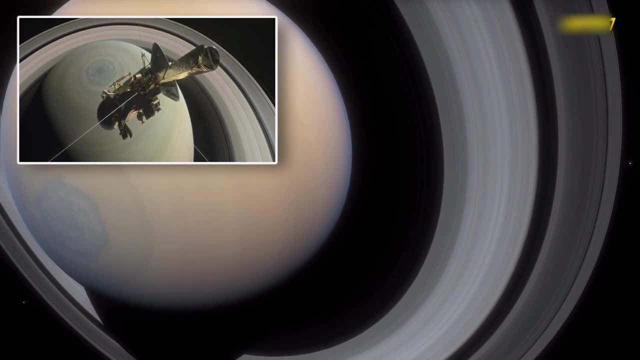 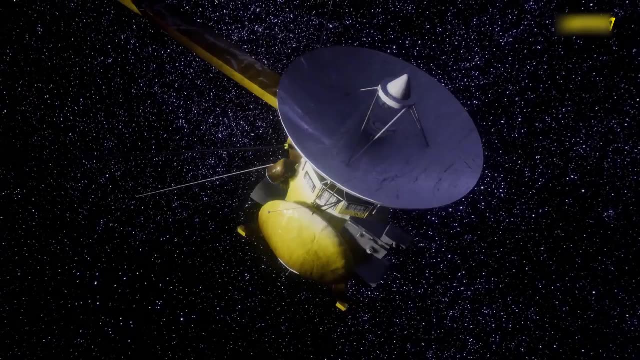 because you can see that the rocks are abraded. They've been smoothed by the action of a liquid flowing over them, But there are no rocks. Huygens was able to confirm that these are in fact boulders of frozen water ice. 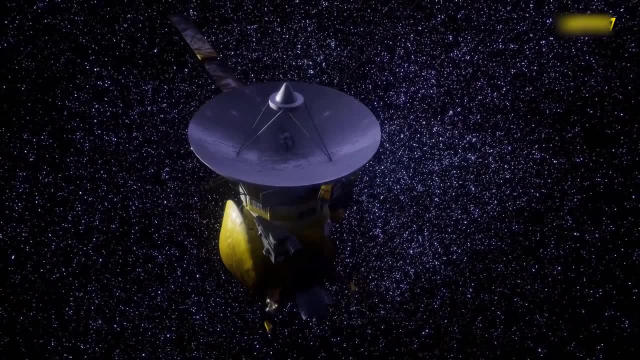 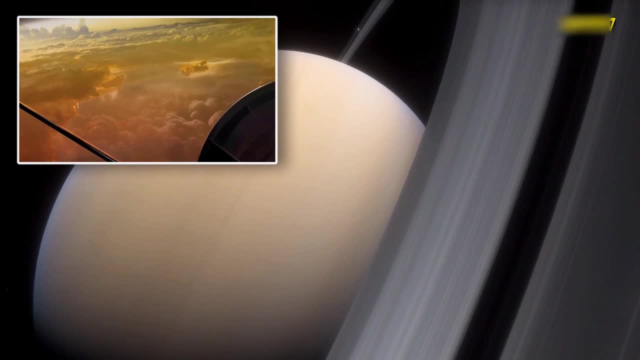 sculpted on the freezing temperatures of Titan's surface. These rocks of ice are sitting on a surface that, as one Huygens scientist described, it, is like snow that has been frozen on top. If you walk carefully, you can walk as on a solid surface. 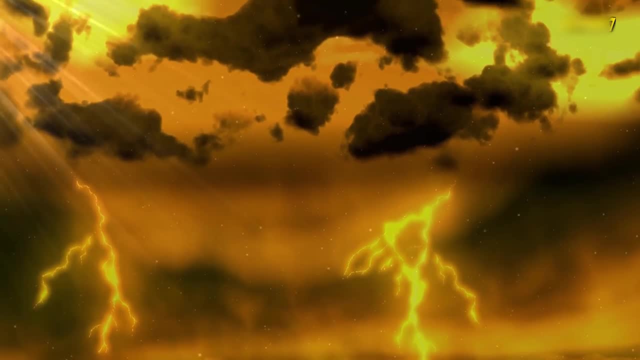 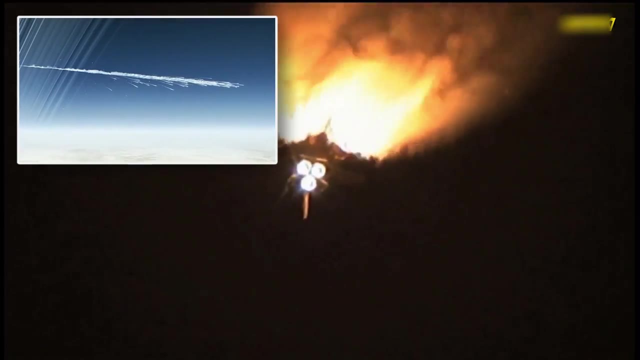 But if you step on the snow a little too hard, you break in very deeply. So if the temperature is so cold on Titan that rocks are made from water, what liquid is flowing over the rocks of ice, carving the riverbeds and floodplains directly there? 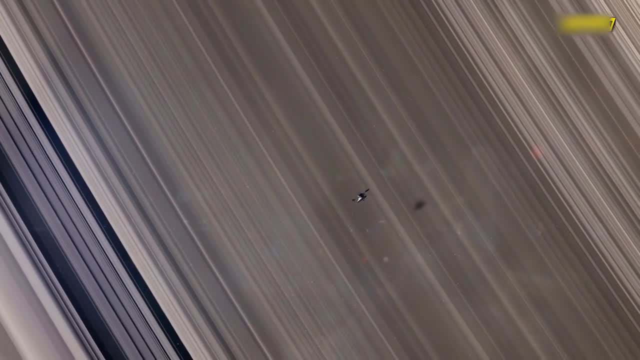 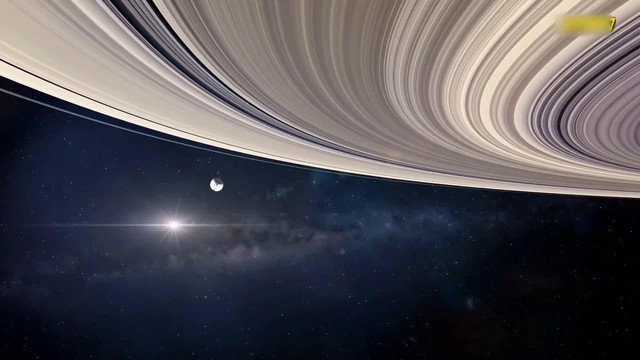 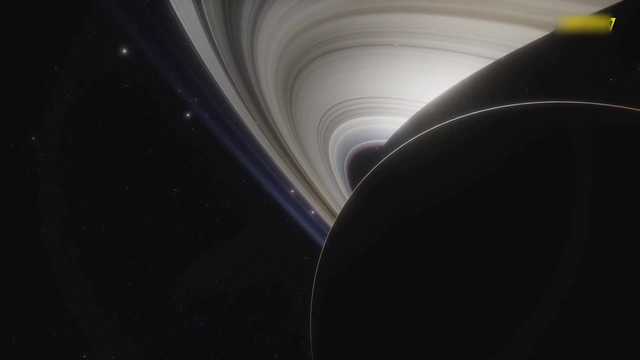 But we can imagine a time in the far future when the sun has heated up to the point where the inner solar system has become uninhabitable, where Titan may become quite cold, That methane greenhouse will become more powerful as the sun gets hotter and at some point that icy crust will start to melt. 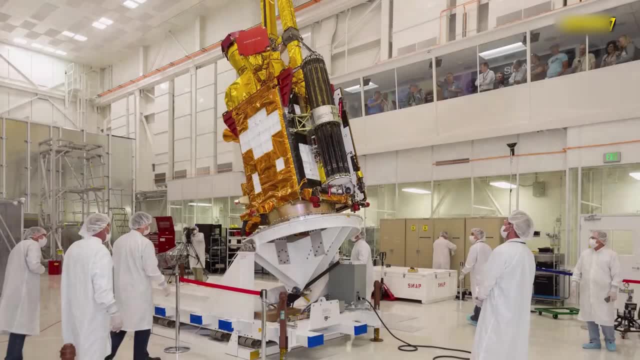 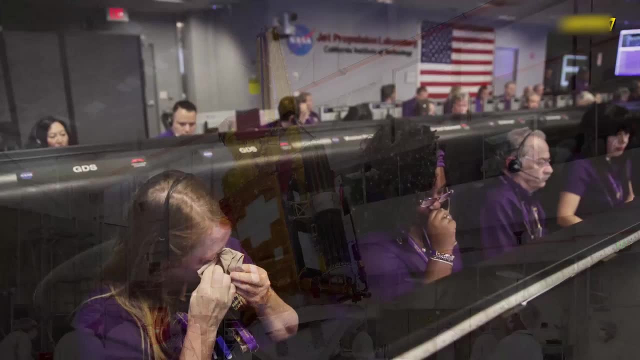 and you'll have large pools of liquid water on the surface full of all those complex organic chemicals, and that is a recipe for the kind of place where the origin of life can happen. So even if Titan doesn't have life today- and that's something we still have to search for- 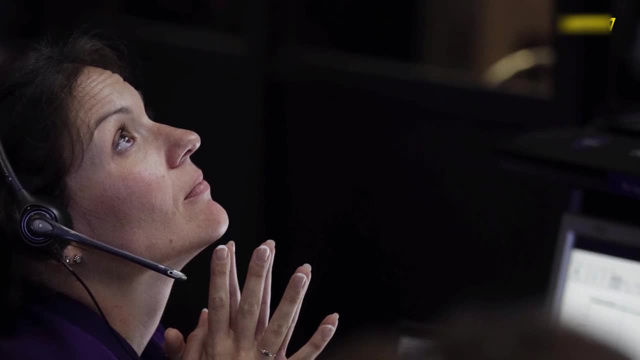 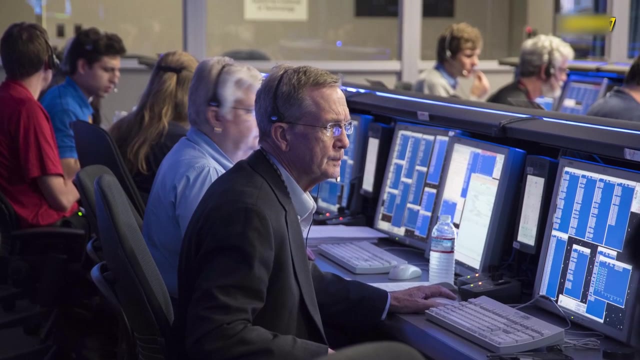 there's every reason to imagine that at some point in the future it could be a great place for biology. It's easy to think of habitability as a permanent feature of worlds, a defining characteristic, if you like. Earth is habitable because it's in the Goldilocks zone. 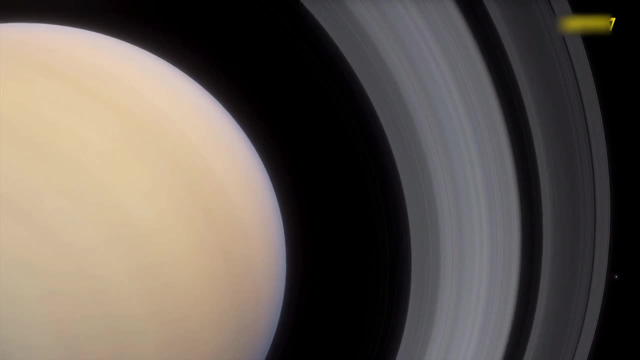 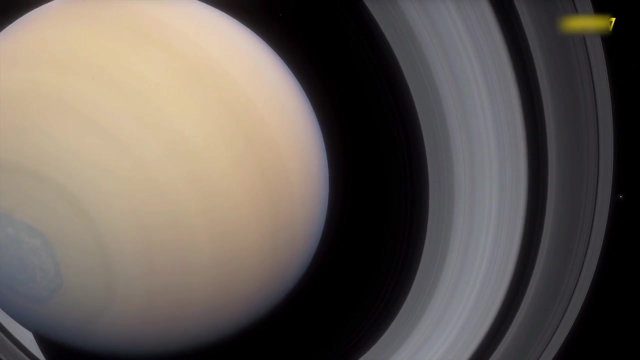 around the sun, not too close and not too far away. But it's more complicated than that. Solar systems are dynamic places. Over long timescales, planets change orbits and their parent stars evolve, and worlds that were once heaven can become hell. 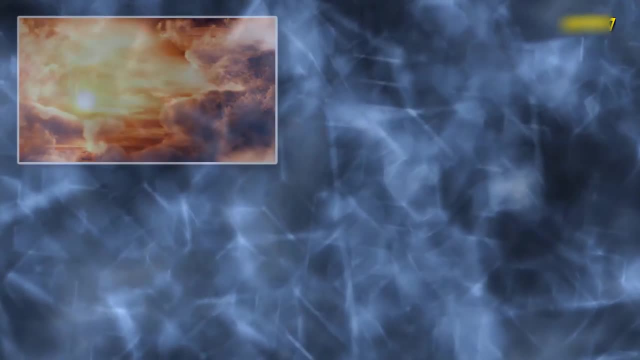 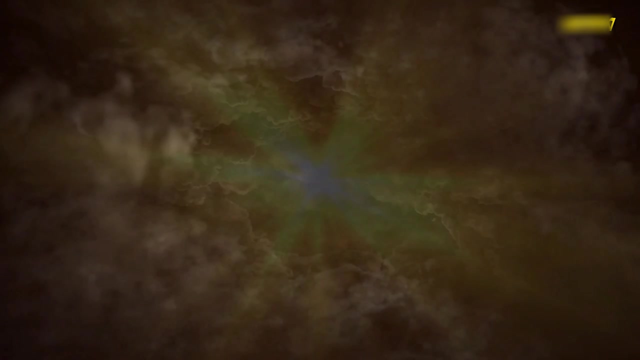 We now understand that Earth is a planet. we now understand that Earth has been a fortunate world, an oasis in a constantly changing solar system that's maintained a stable climate, perhaps against the odds, For the four billion years it's taken complex living things to evolve. 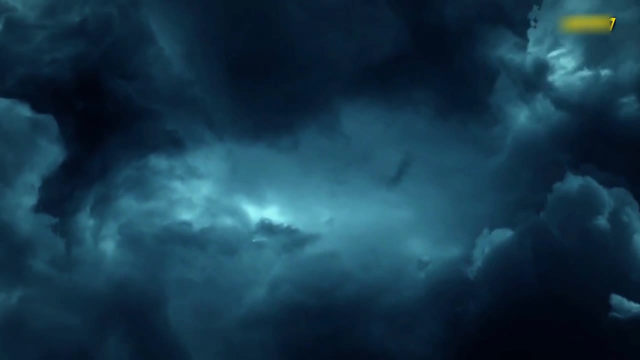 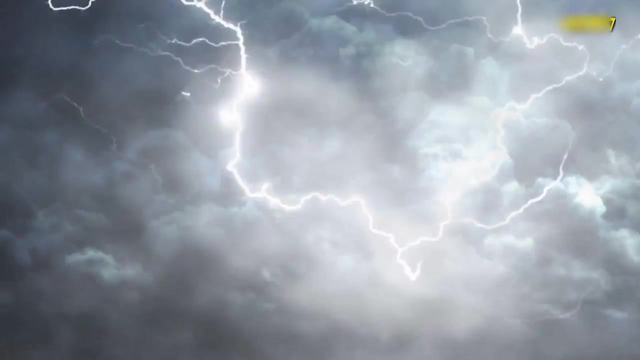 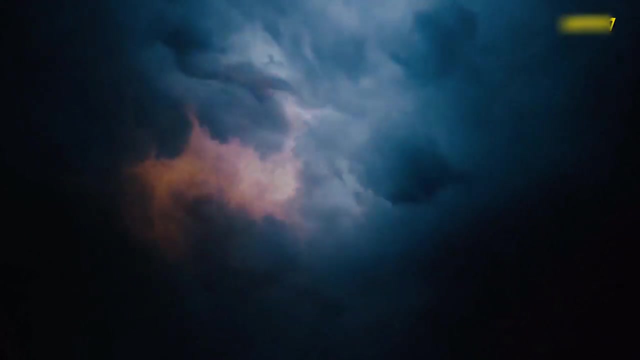 We don't know how many planets like Earth are out there amongst the stars, where the ingredients of solar systems have assembled into structures capable of dreaming of other worlds, But we must consider the possibility that there are very few, and that would make Earth and us. 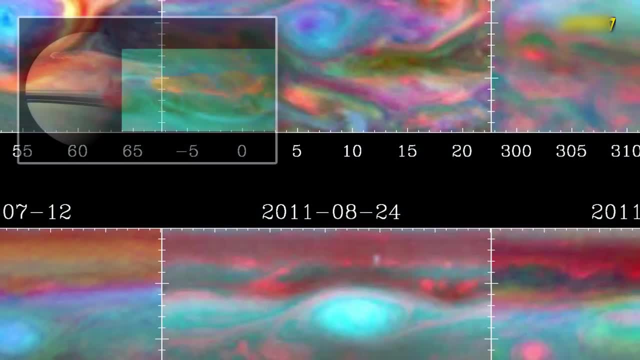 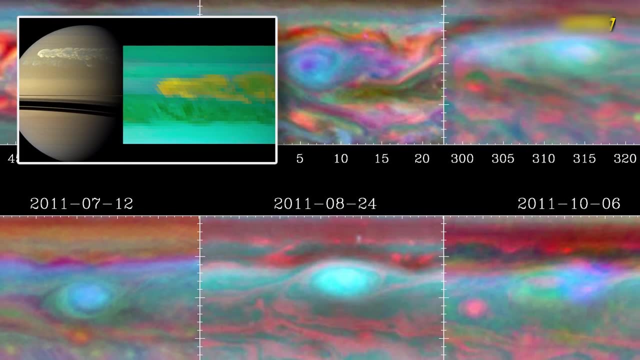 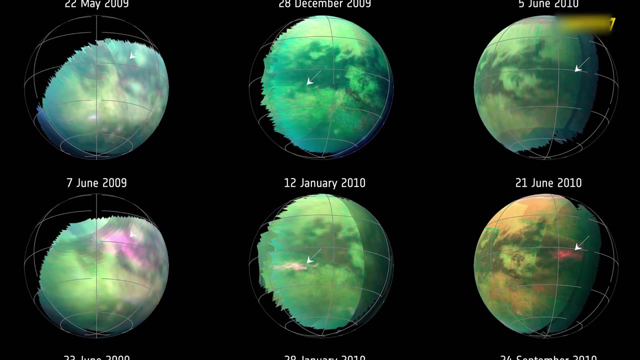 extremely rare and precious. Nearly a billion miles from the warmth of the sun, on the outer edge of Saturn's rings, lies the icy moon of Enceladus. A small moon about the size of Iceland, Enceladus is the most reflective object in the solar system. 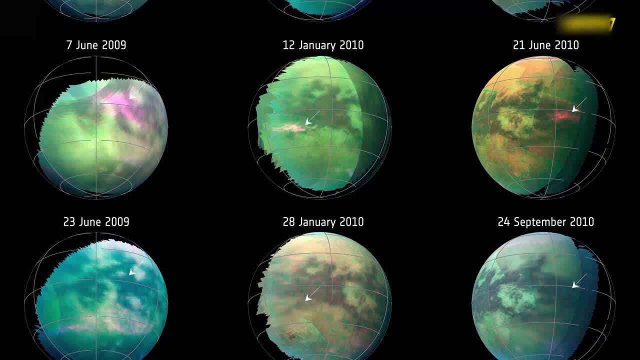 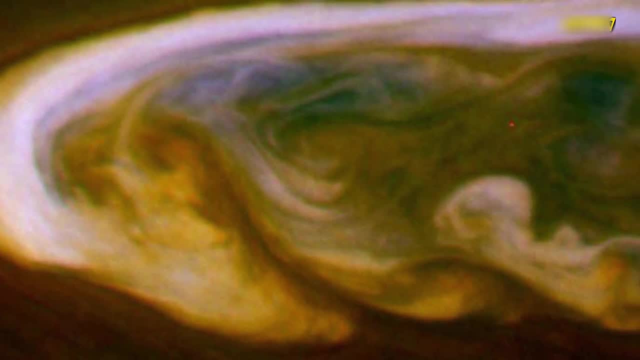 Over 90% of the light that hits it bounces back. That's because the surface of this icy moon, this covered moon, is covered by crevasses, just like we see on the surface of glaciers here on Earth. But on Enceladus, these cracks in the ice 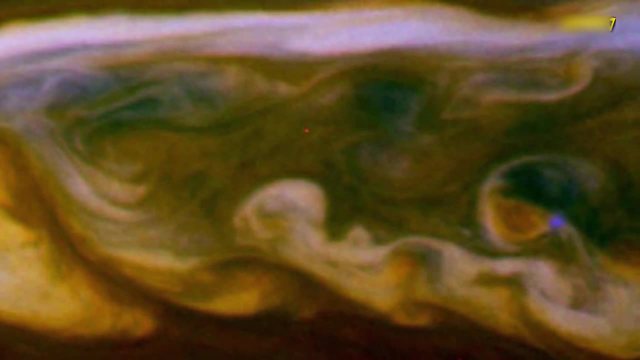 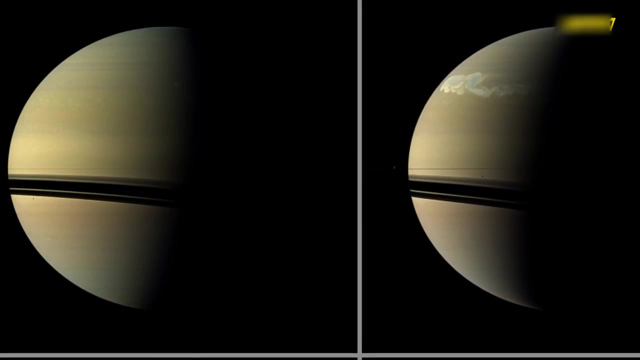 occur on a much grander scale, with some stretching for over 100 kilometres. But for all that's going on on the surface, it's what we discovered beneath Enceladus' shell of ice that must rank as one of the greatest surprises. 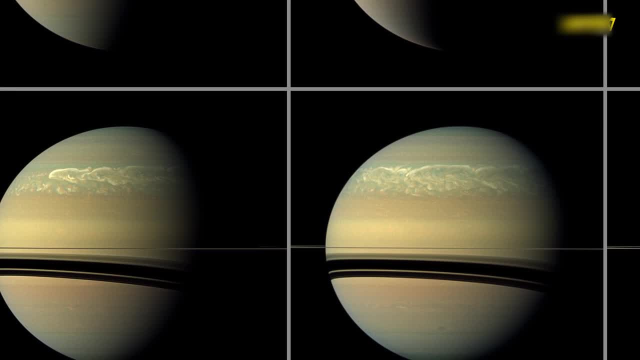 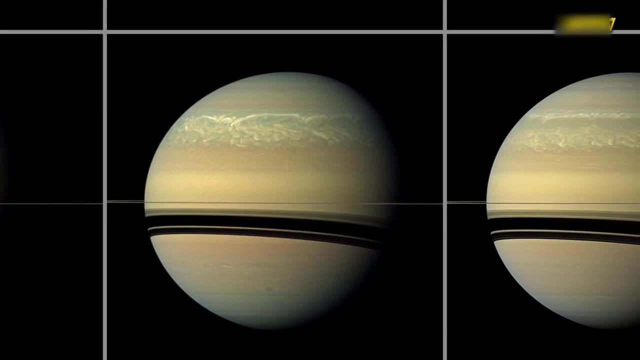 in 21st-century space exploration, a surprise that had been hiding in plain sight for decades. The first photograph of Enceladus was taken by Voyager 1 in 1980. It was actually captured unintentionally- a moon photobombing the planet. 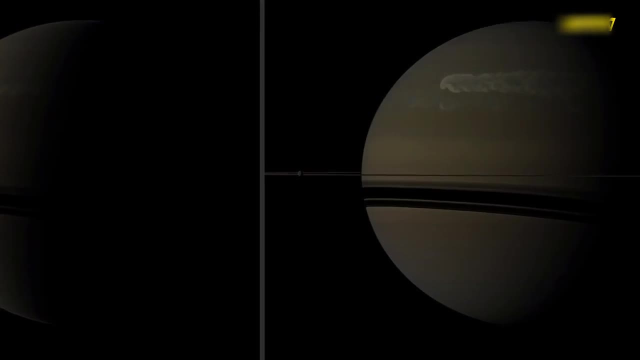 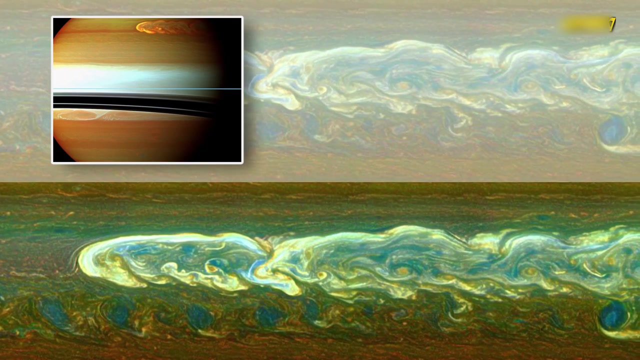 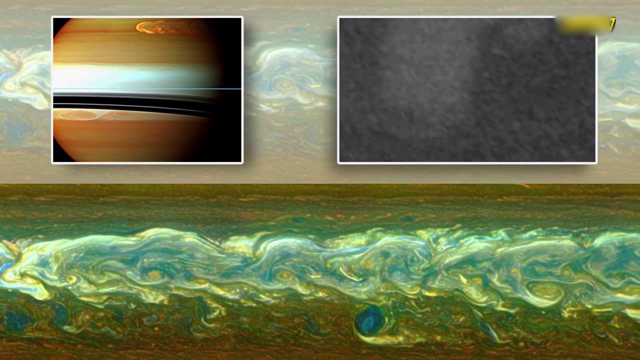 and nobody even noticed Enceladus until over 35 years later. But when the image was eventually enhanced, a remarkable feature- no more than a misty blob- began to emerge on one side of the moon. 24 years later, Cassini saw exactly the same picture. 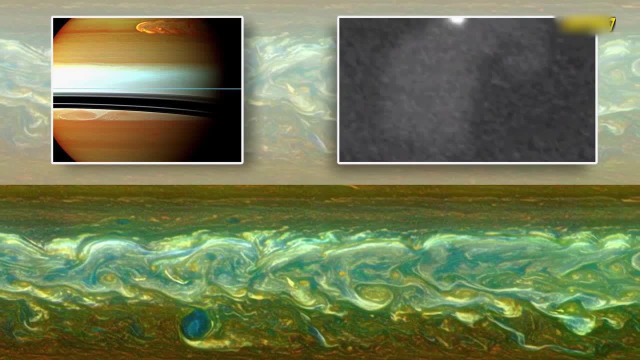 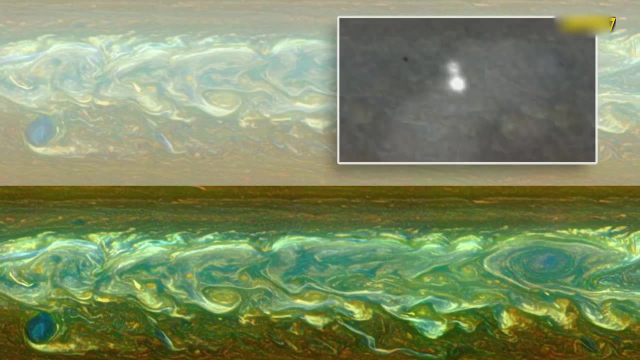 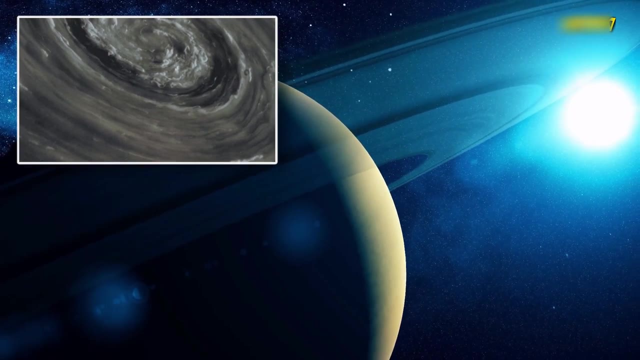 but this time in much more detail. As Cassini approached Enceladus, the anomaly revealed itself: Giant plumes of water, vapour and ice were erupting from its surface. Over 200 kilograms of material was being released every second, feeding one of Saturn's outer rings and helping to replenish it. 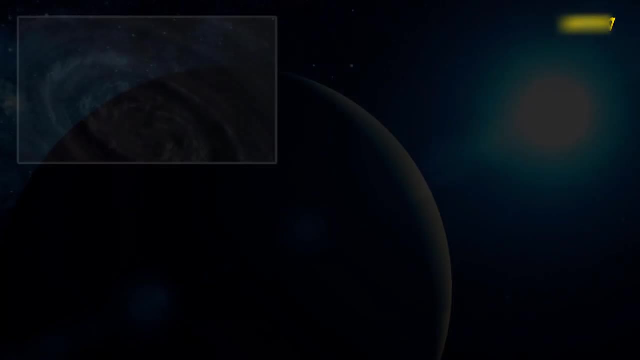 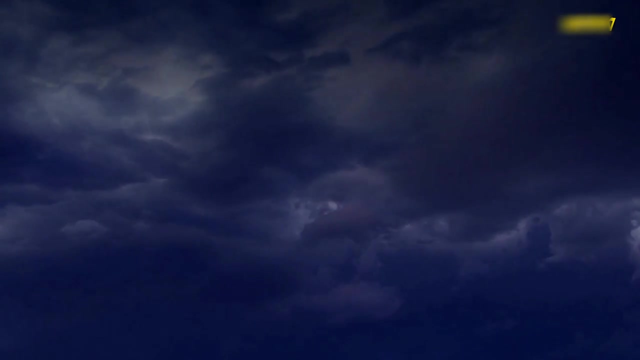 These discoveries inspired the Cassini team to take an audacious risk. Piloted from nearly a billion miles away, Cassini was guided dangerously close to the plumes and, using its cosmic dust analyser, was able to actually touch the plumes of ice. 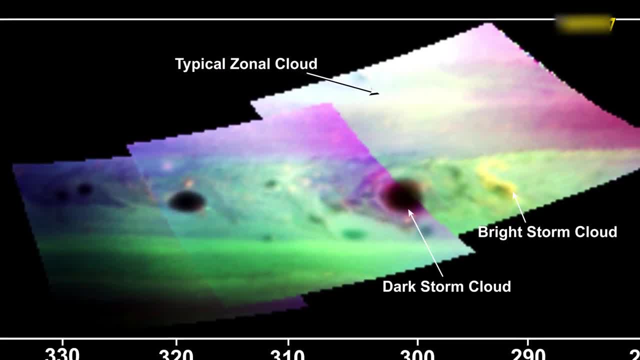 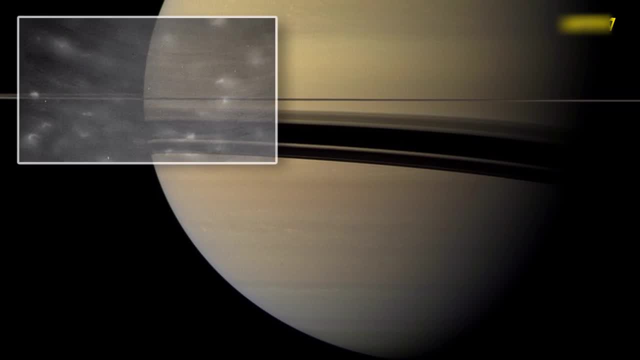 and collect a sample from one of the eruptions. As Michel Doherty, scientific leader on the Cassini project, explained the really close flyby that we had of Enceladus, where we were 25 kilometres above the surface, 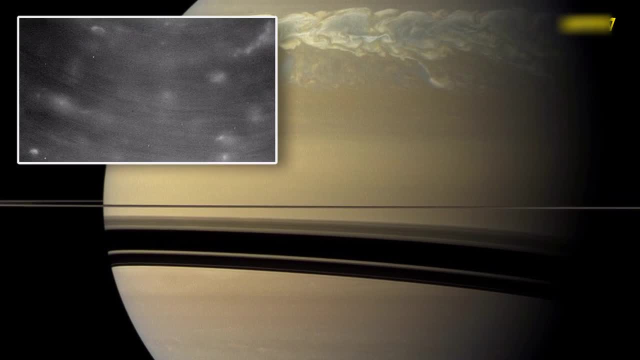 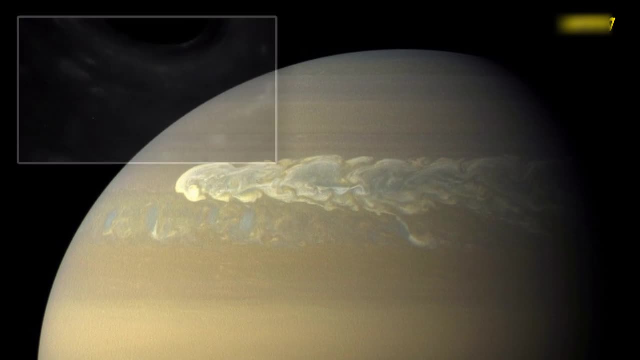 is probably closer than any spacecraft has been to a planetary body before, And the Cassini mission team said they'd never do it again because we were in the atmosphere, well, in the plume, which was really dense. They didn't lose control of the spacecraft. 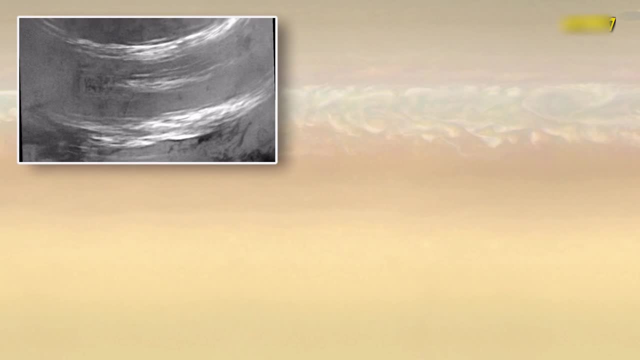 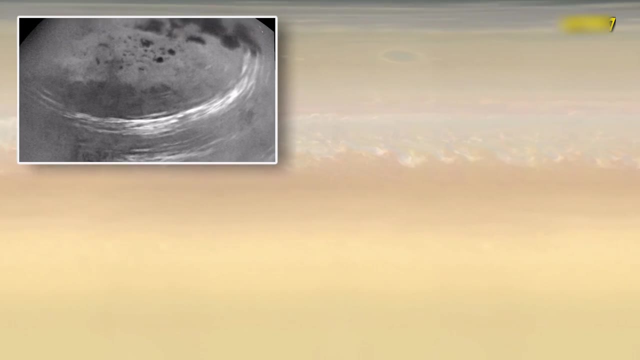 but they felt they might, because the mag boom used to stickle from the side of the spacecraft, and that almost started tumbling the spacecraft. What the scientists discovered, though, thanks to this and a series of similar flybys, was breathtaking. 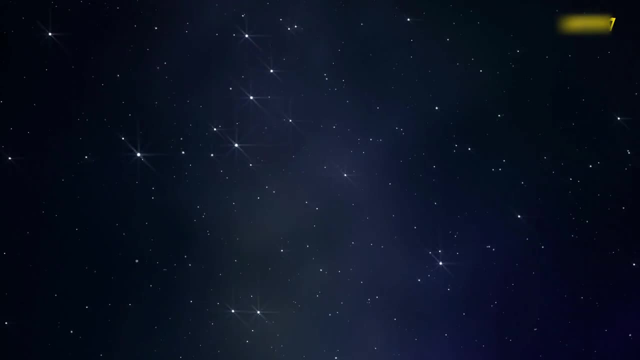 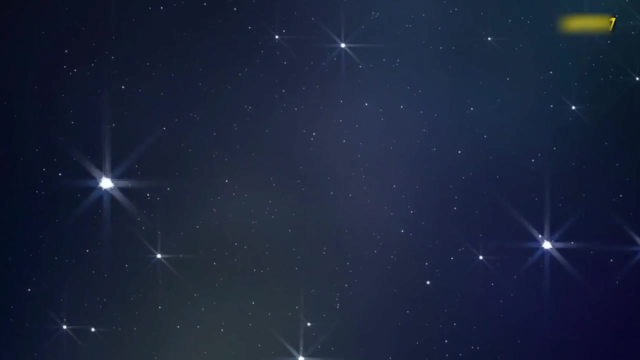 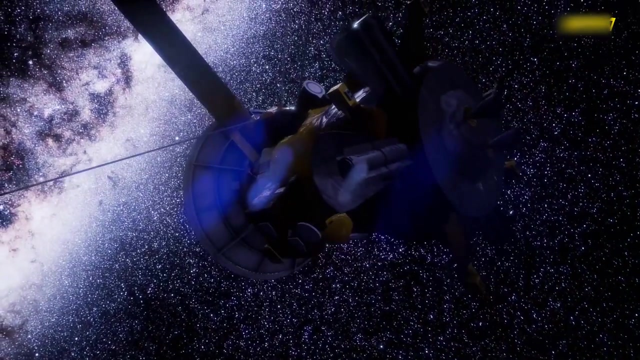 The plumes were spewing out of fissures known as tiger stripes, being projected from deep within this ice world, rising up from an ocean of salty liquid water beneath the ice. How could such an ocean exist in the far frozen reaches of the solar system? 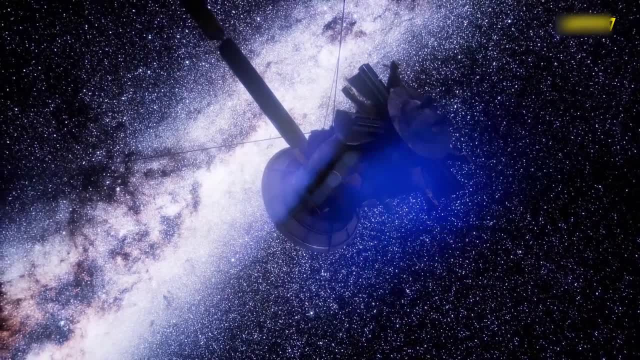 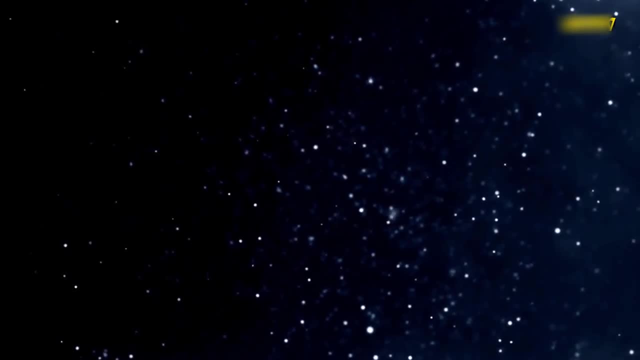 The answer lies once again in the power of Saturn to control the destiny of the moons in its dominion, Unlike the long-lost moon of Veritas that was destroyed by the might of Saturn to create its rings in the case of Enceladus. 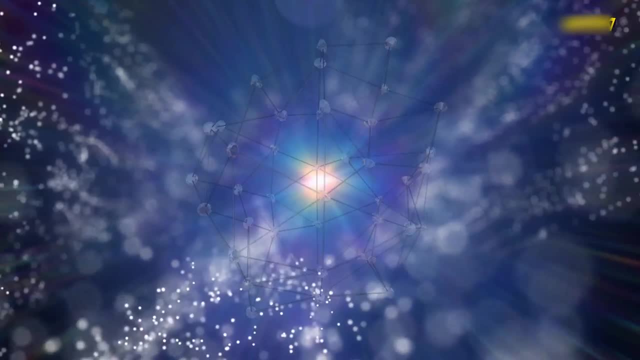 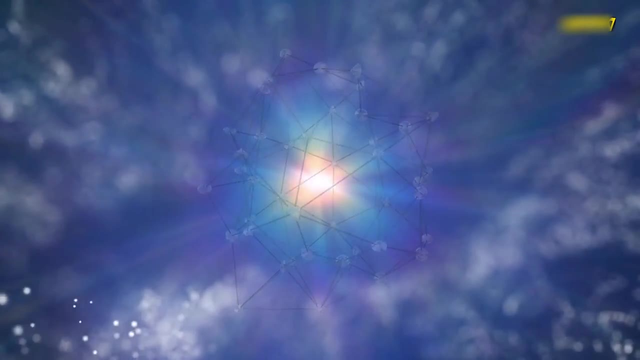 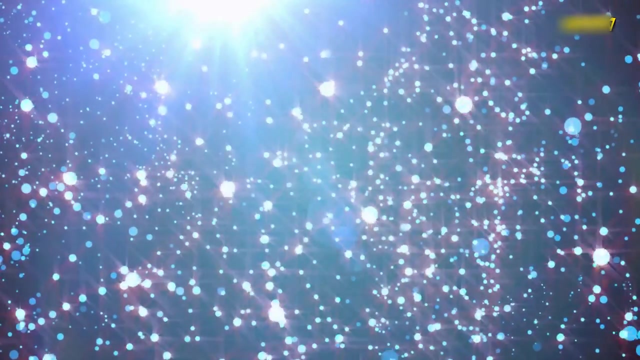 its mother planet has breathed life, not death, into its structure. Enceladus orbits Saturn and the planet's vast gravitational force pulls at the moon, holding it in orbit. But every couple of rotations another larger moon called Dione aligns with Enceladus, drawing it back. 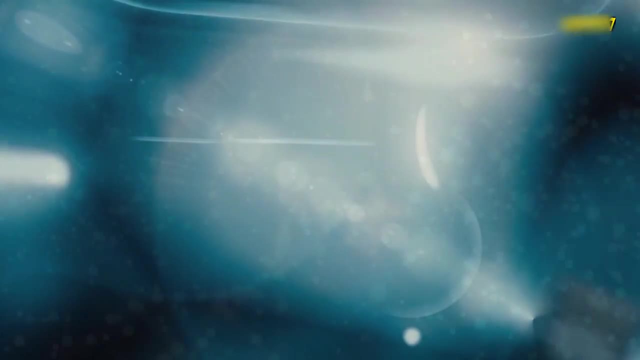 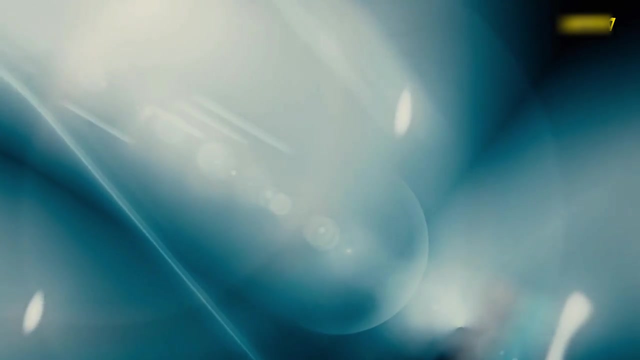 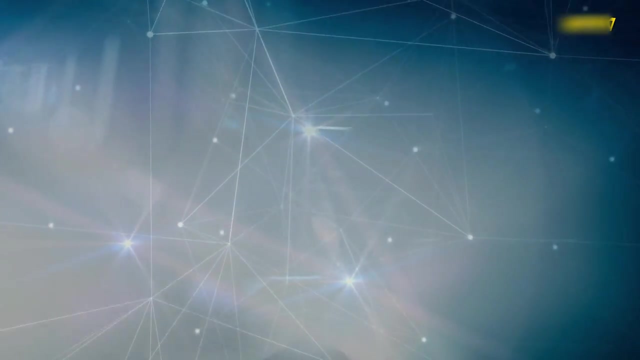 This repeated tug of opposing tidal forces stretches and squeezes the moon, warming its core and melting its icy interior. Exactly the same gravitational forces that destroyed one of Saturn's moons are now breathing life into another, But it's what Cassini found in the chemical make-up of the plumes. 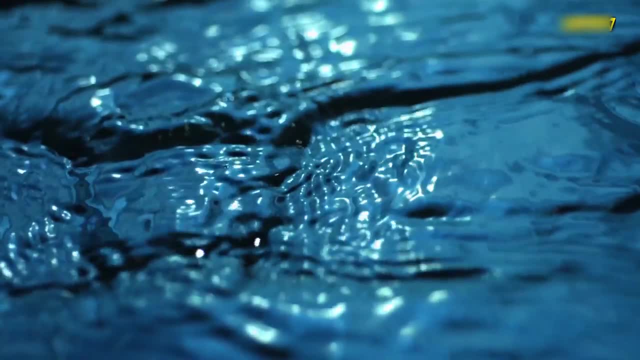 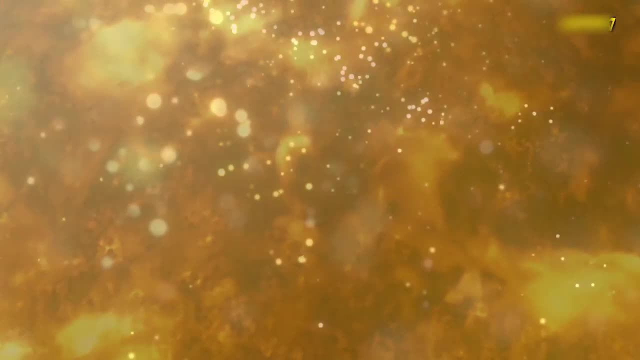 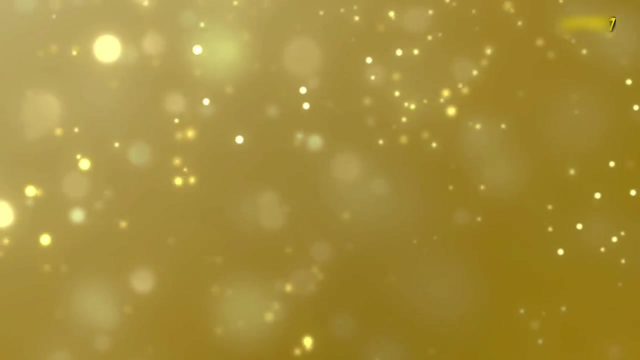 that changed everything, Because, as it analysed the columns of water, it discovered complex organic compounds and silica particles, Direct evidence that deep below the ice, at the bottom of a salty ocean of water, there were hot hydrothermal vents exactly like the ones from which we believe. 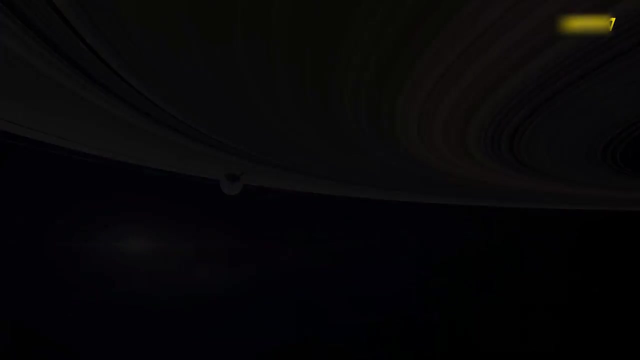 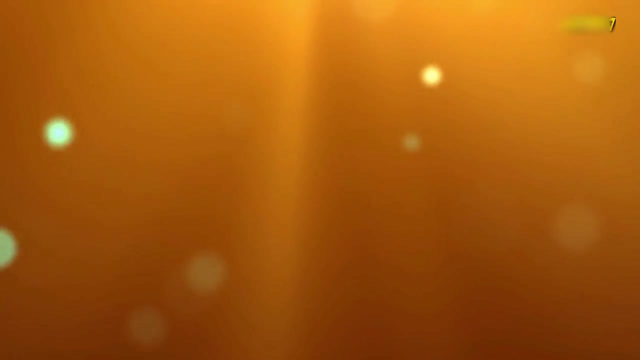 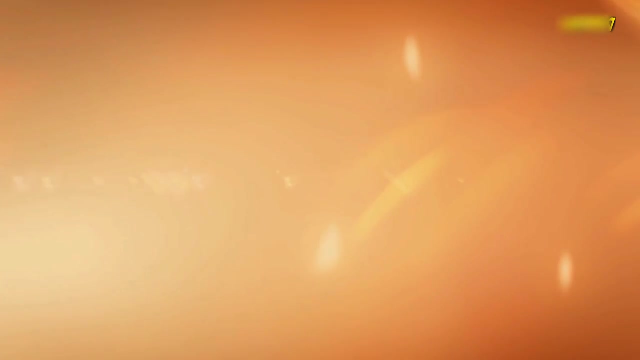 life emerged on Earth almost four billion years ago, Out in the frozen outer reaches of the solar system. Cassini has given us a glimpse of the world beneath the ice on Enceladus and revealed a warm, watery oasis, a world in which it really is possible. 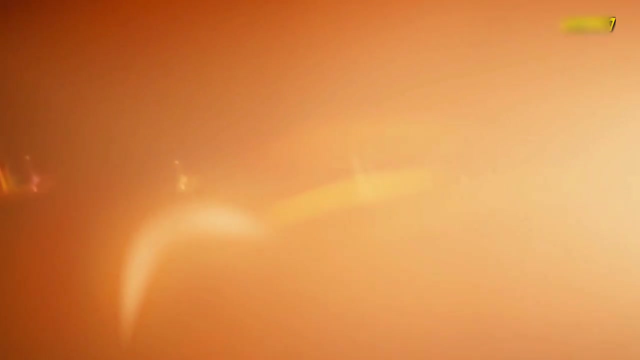 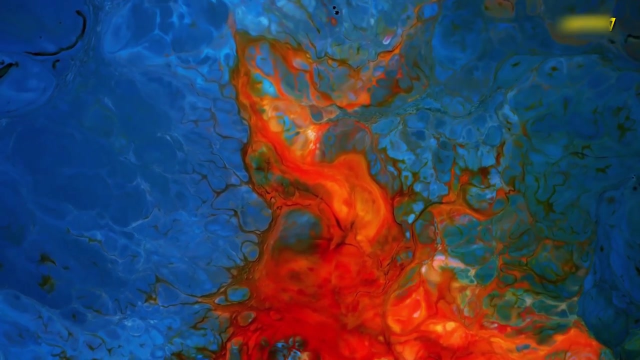 that life could exist. Exciting though the prospect of life in space is, if it is out there on Enceladus, it's likely only to be home to the simplest and most primitive organisms, And given how violent and changeable Saturn's past has been, 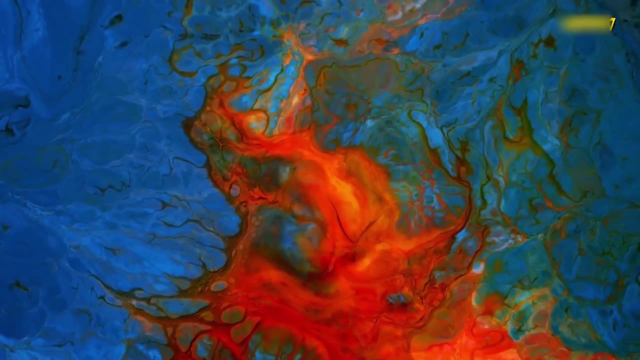 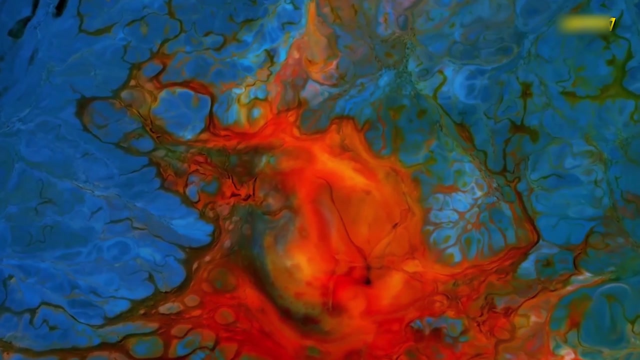 this world may have arisen relatively recently. We don't know how long Enceladus has been active, but if it's only tens or even hundreds of millions of years, that might not have been enough time for life to get going. And despite all the caveats, 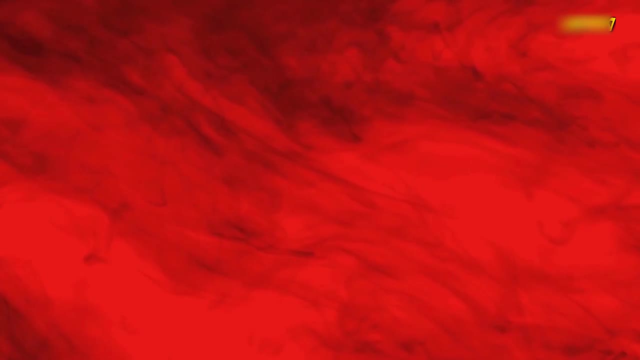 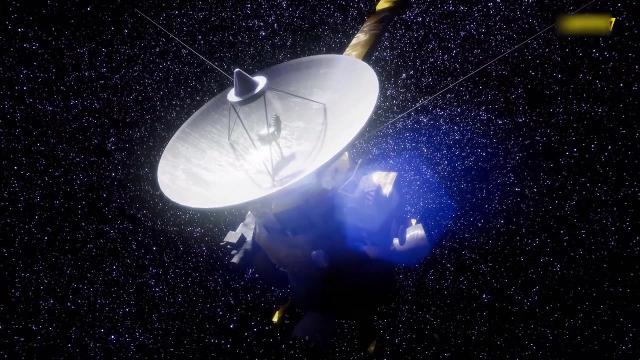 the very fact that the Saturnian system holds the potential to host life is a truly remarkable discovery, and one that compels us to explore even more. But for Cassini, the brave new world under the ice of Enceladus was a bittersweet discovery. 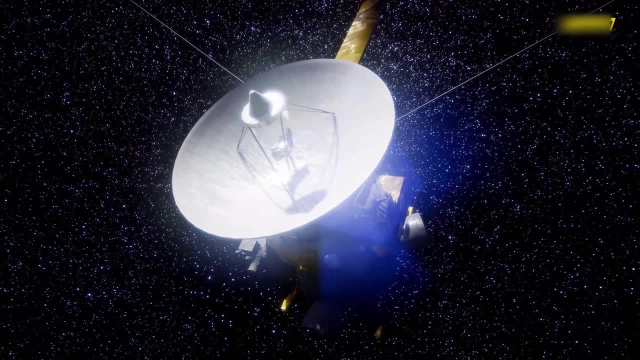 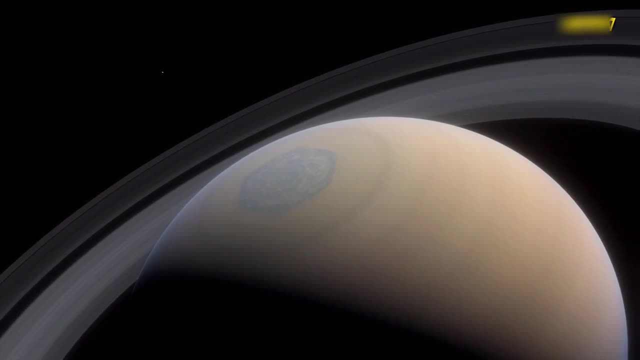 Thirteen years after it arrived in orbit around Saturn. as Cassini's fuel finally began to run dry, the team at NASA realised it couldn't risk letting this probe crash-land on Enceladus and contaminate a potential habitat for life. 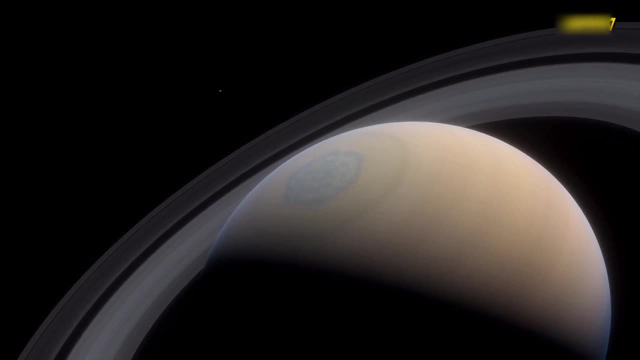 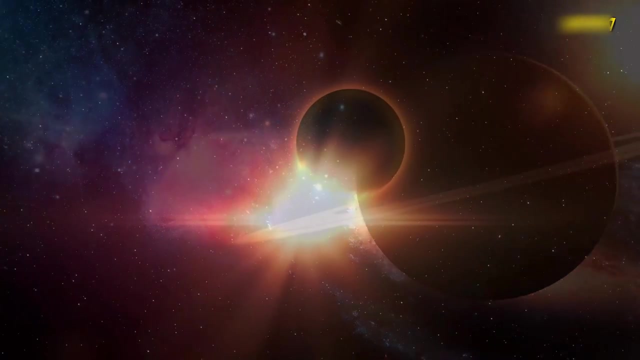 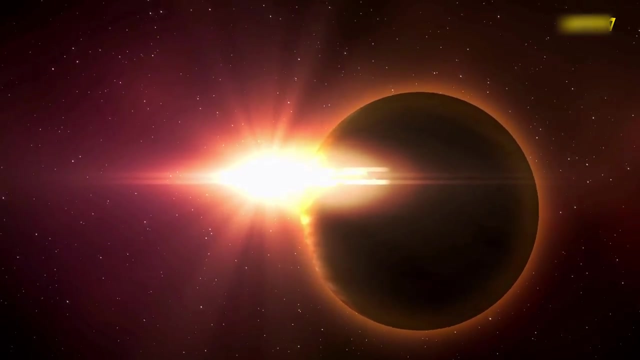 As Carl Munger, as Carl Murray explains, because we now knew Enceladus was a potentially habitable environment, we couldn't risk Cassini crashing into it or coming near it because there might be microbes hitchhiking on the spacecraft and we couldn't allow contamination of Enceladus. 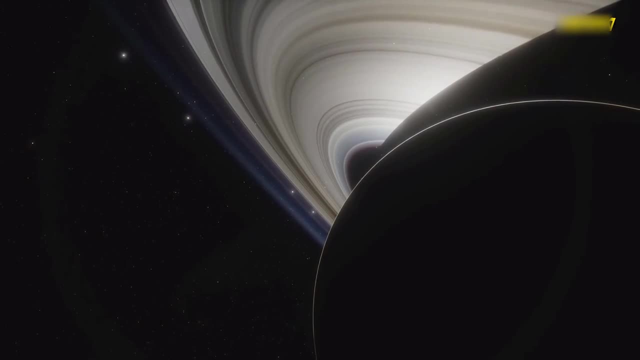 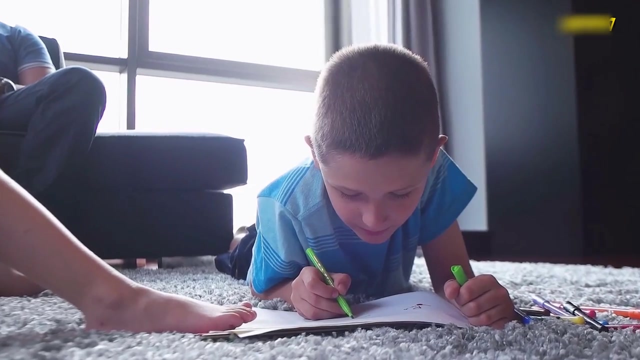 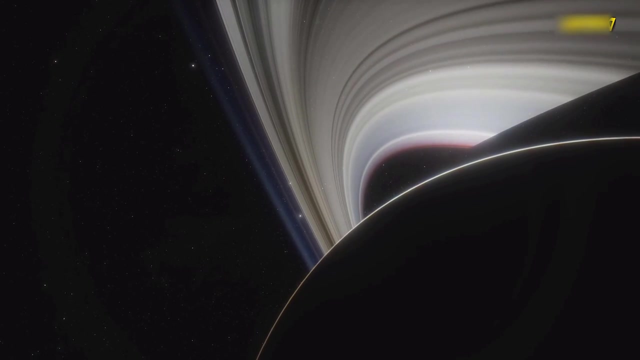 So we consciously picked an end of mission that would use up its fuel and then send the spacecraft into the giant planet itself. We journeyed out across space to Saturn to see this great beauty up close, But in the end we were rewarded with insights. 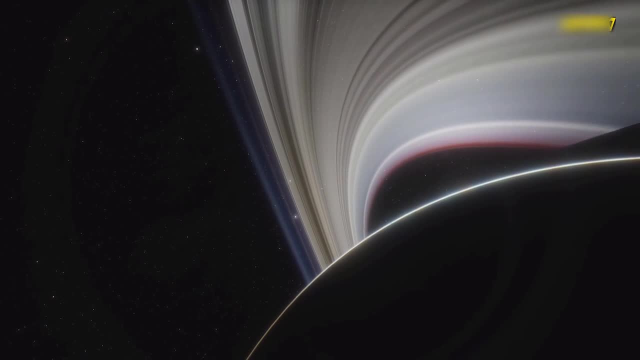 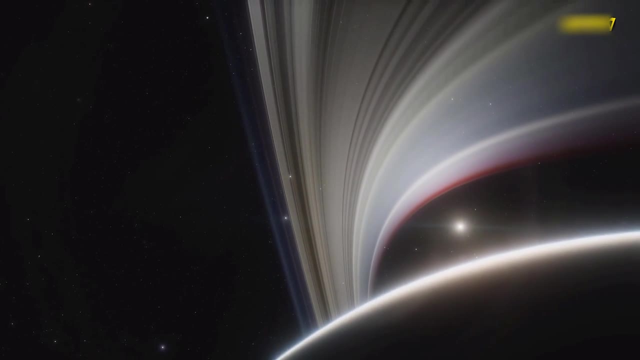 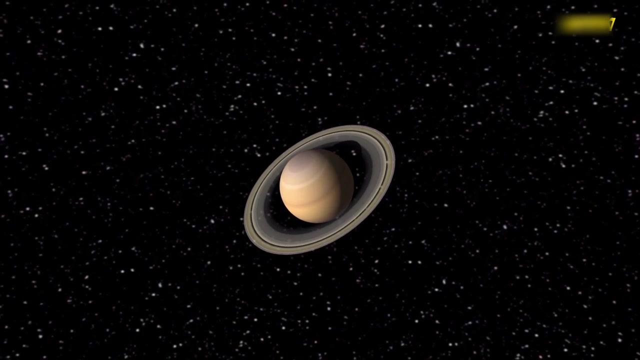 that hit far closer to home. As is so often the case in exploration and science, the real treasure was found in the unexpected shadows. On this mission, it was in the shadow of the rings, because there we found a tiny world with the potential to harbour life. 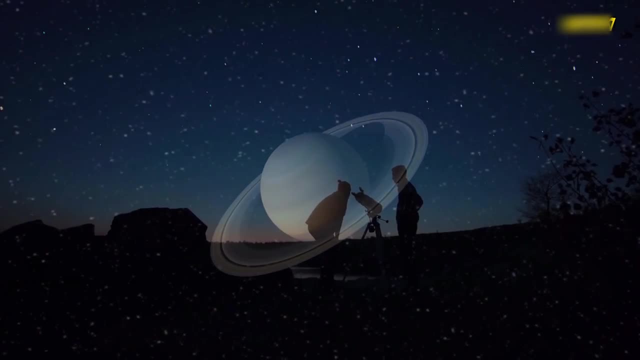 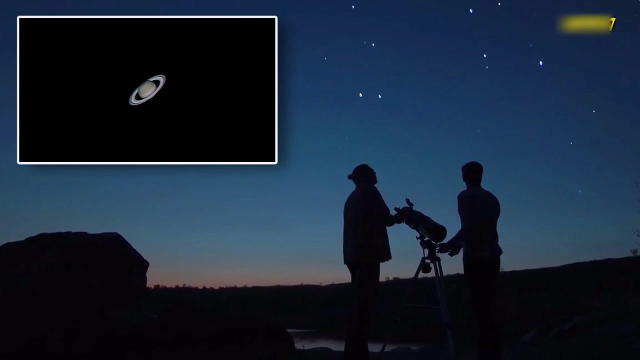 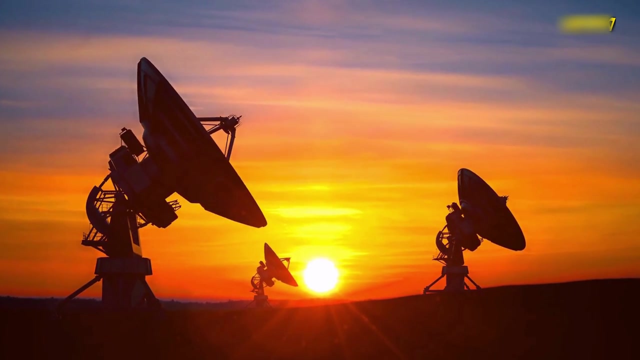 to provide reassurance that, for the first time, we might not be alone. Would such a discovery matter? Yes, it would. At this moment in history, we are, I think, in need of reassurance, or perhaps a reminder that there is great beauty and knowledge. 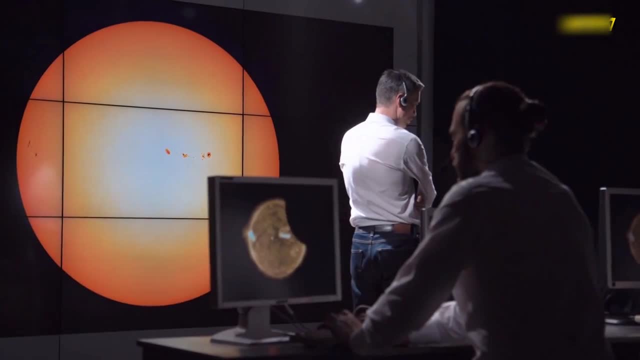 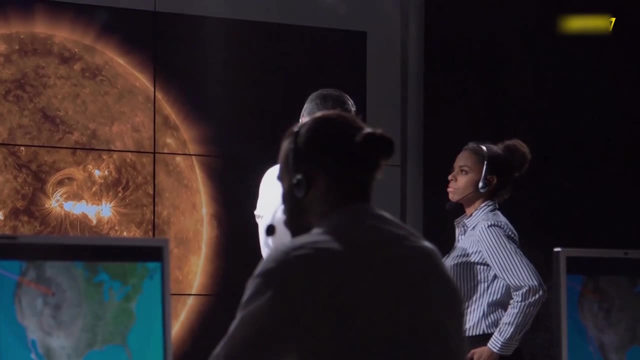 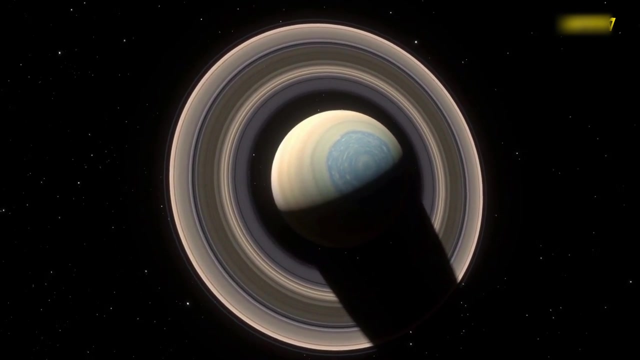 and perhaps even life and meaning beyond our shores. We will, I'm sure, go back to Saturn and its moons, explore deeper, stay longer and maybe one day even visit there ourselves. We don't yet know what we will discover, But we can be sure.